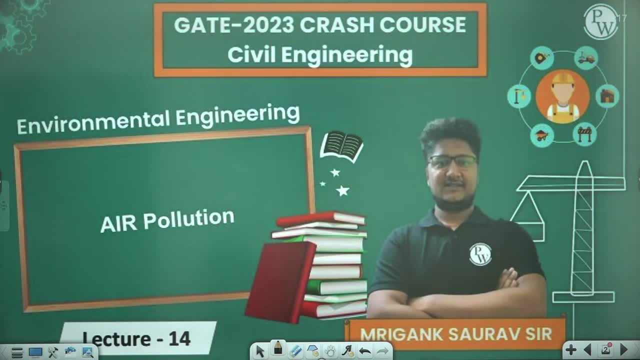 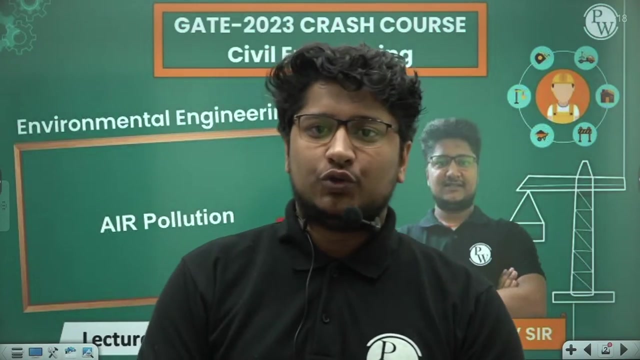 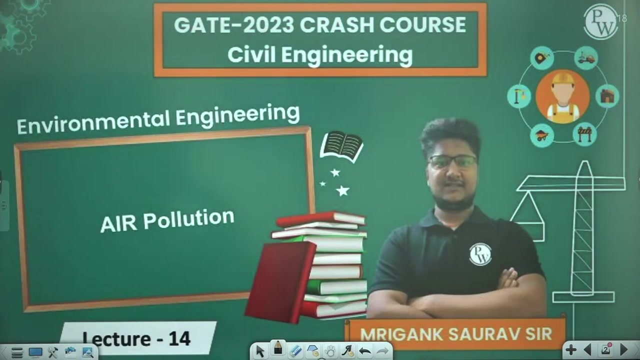 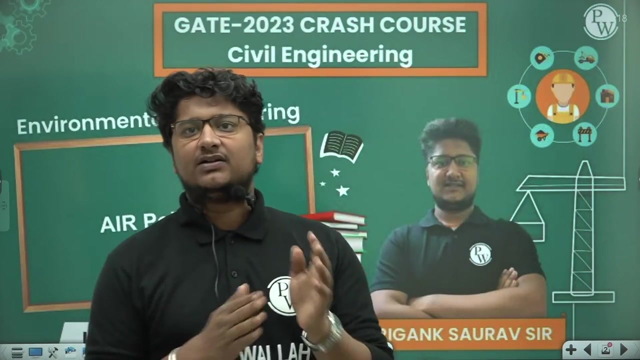 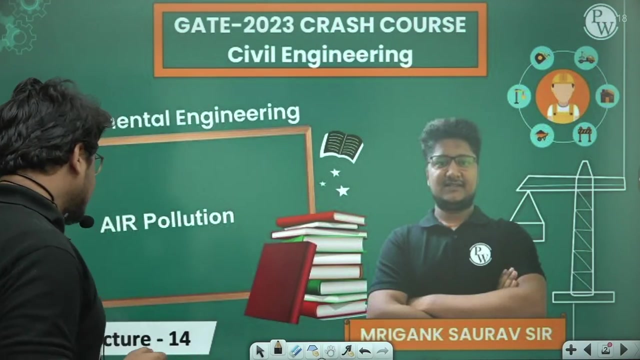 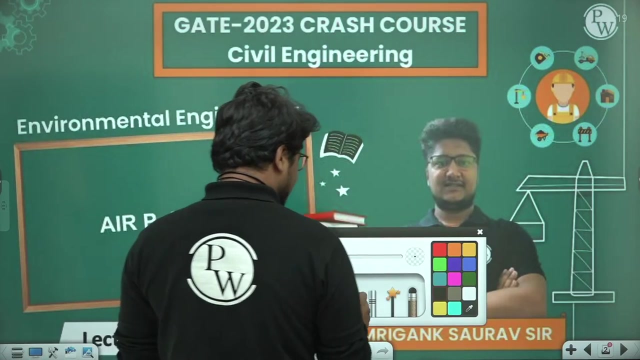 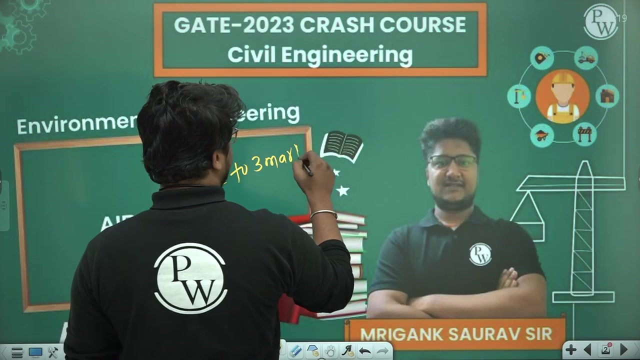 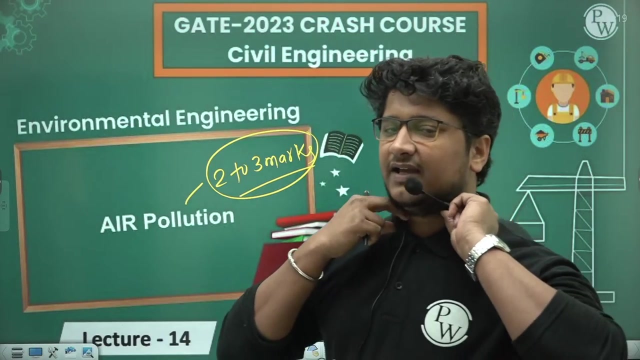 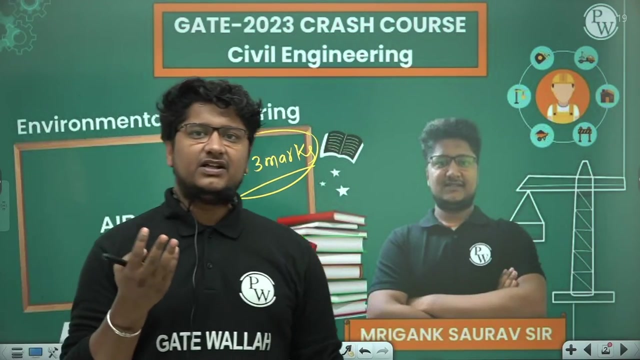 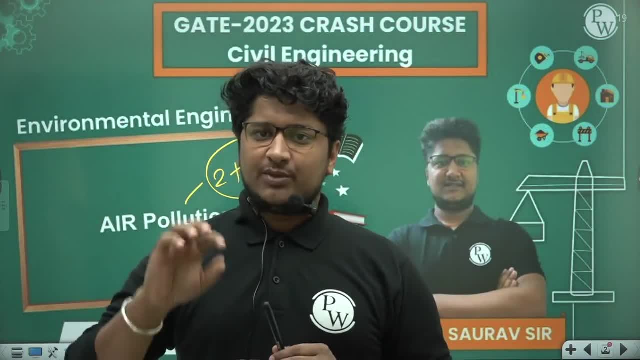 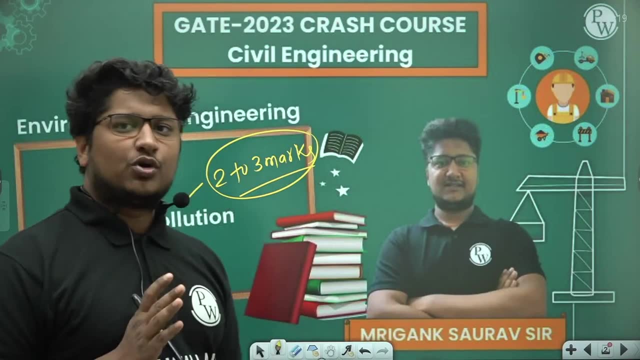 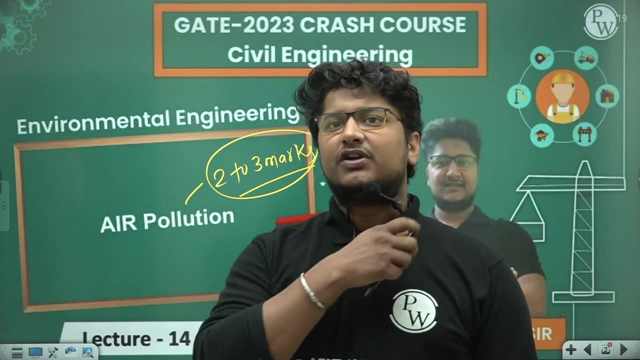 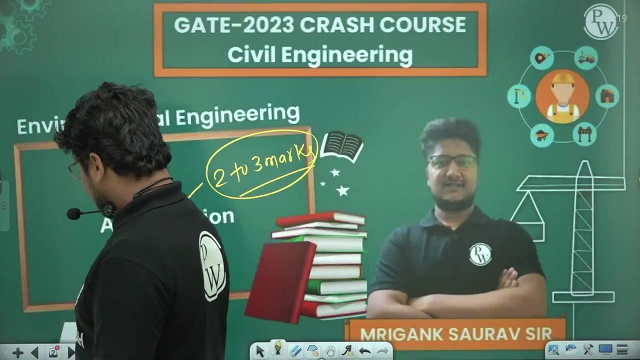 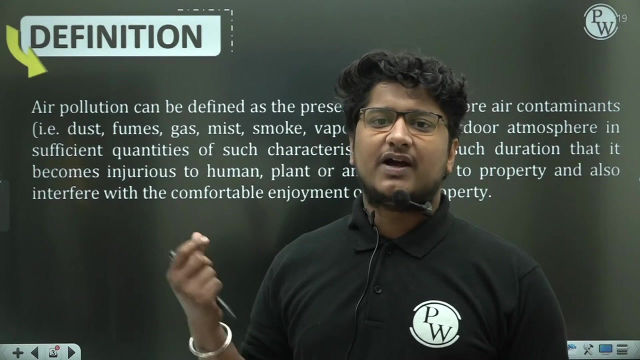 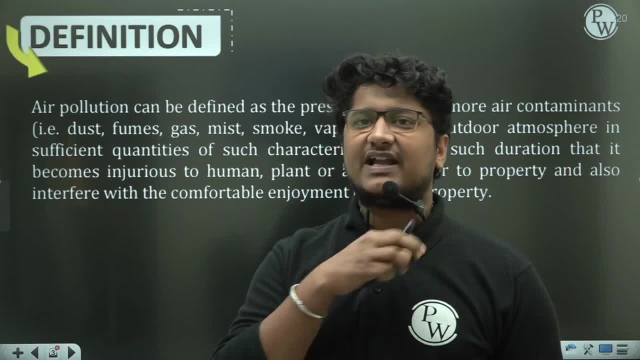 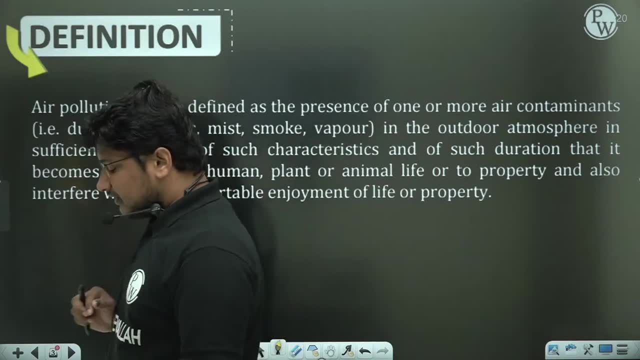 And do the numerical part with me. You will have to do the calculation part here. So we are going to talk about this chapter as well. Let's go Now when you talk about air pollution. So this is not a word that you have not heard till now. 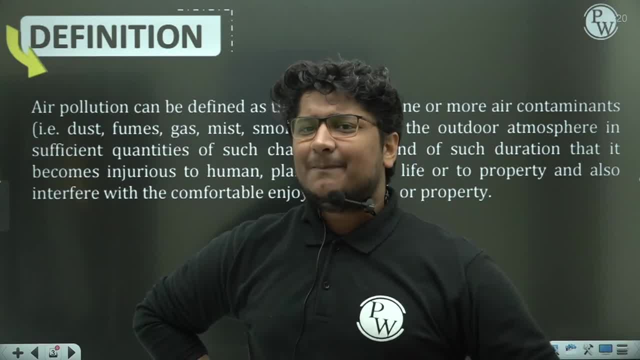 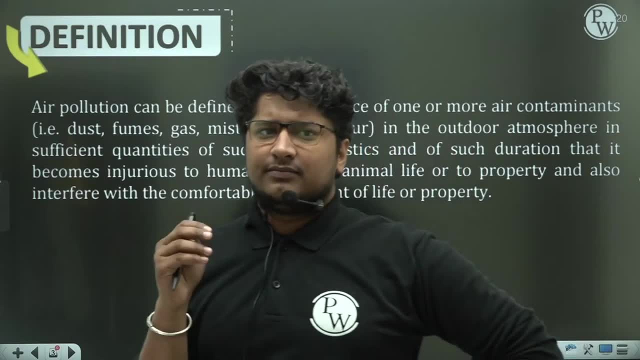 You all must have heard about air pollution before The basic thing that I am explaining to you, which you always know. So when someone asks you that, sir, the air is polluted, Or when you say that, sir, this is air pollution, When do you say that? 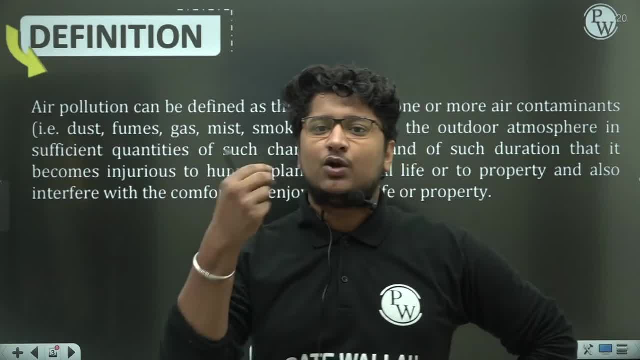 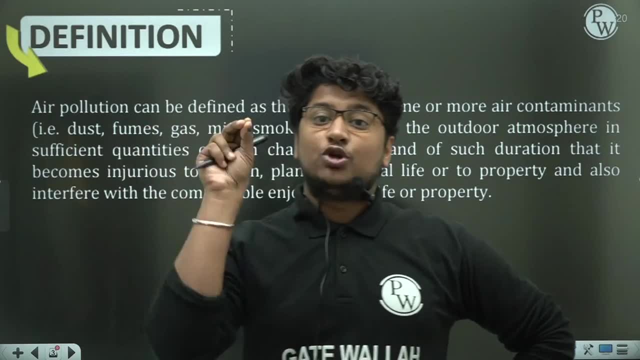 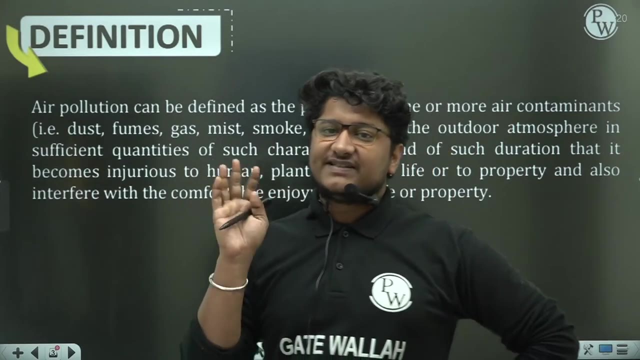 Generally, human being talks about air pollution, water pollution, soil pollution, noise pollution only when he feels uncomfortable in his own life. When that person, that human being, is feeling uncomfortable, then we talk about air pollution. So remember that when some of the same particles, some of the same pollutants get mixed in your air, 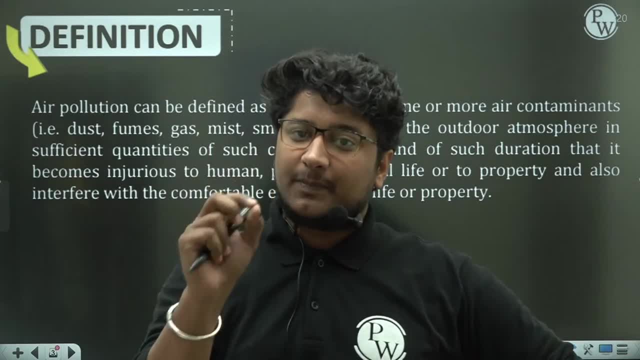 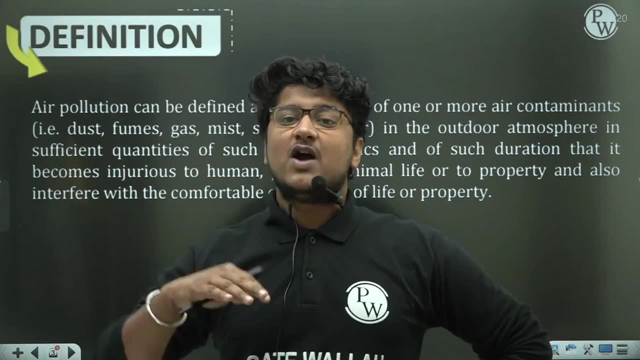 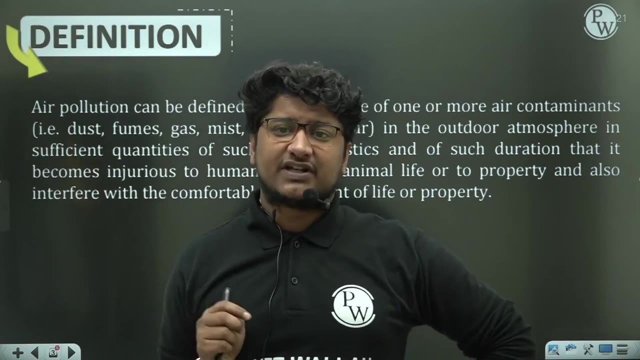 Which will affect your personal life, Which is creating a problem in your public life, In the sense it can also have a direct effect on you, Whether it is an indirect effect. Indirect effect means your house is getting damaged, For example, your Taj Mahal is getting damaged due to air pollution. 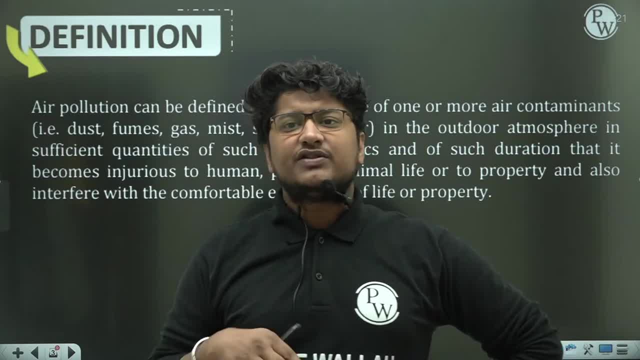 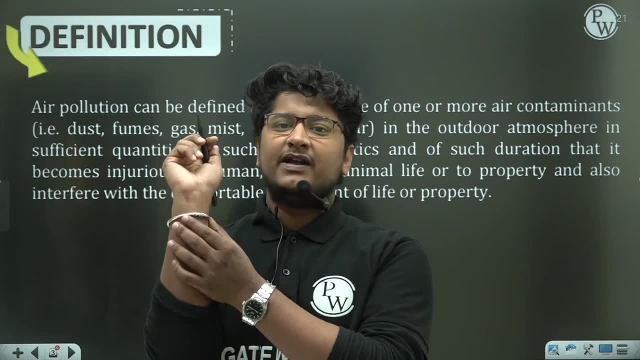 Some of your outer metal is getting degraded, So you will get to see a lot of problems. You must have seen it many times. By the way, I don't want to name it, But where is it? You all know where it is. 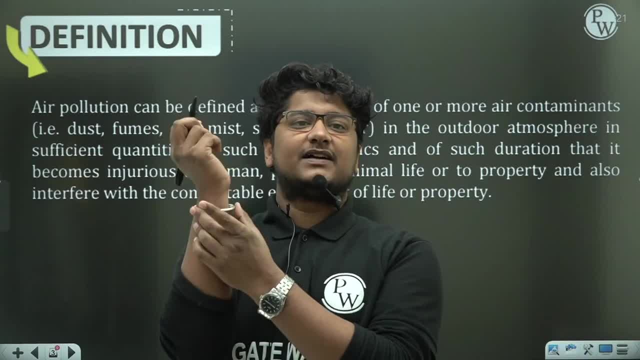 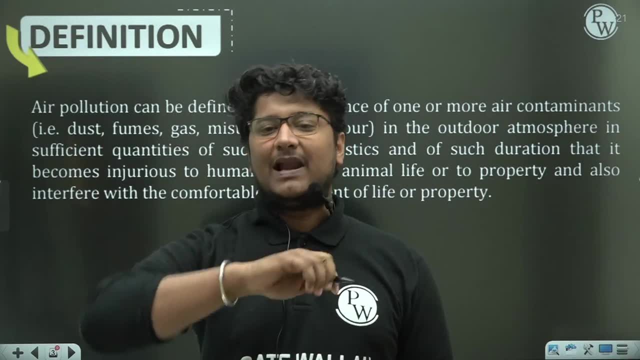 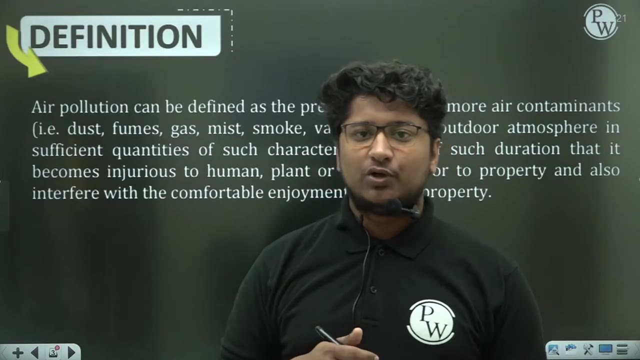 There is one place in Delhi. There I washed my hands with municipal water. After sometime my whole body turned black, So there was a reaction. Silver reacted. So why is that happening? That is nothing but because of water pollution. Many times you see that you leave a metal like this and it quickly catches rust. 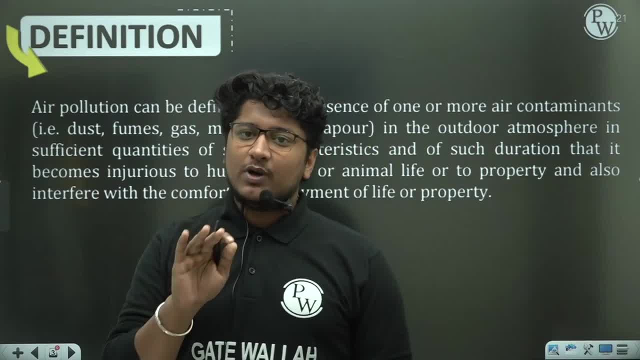 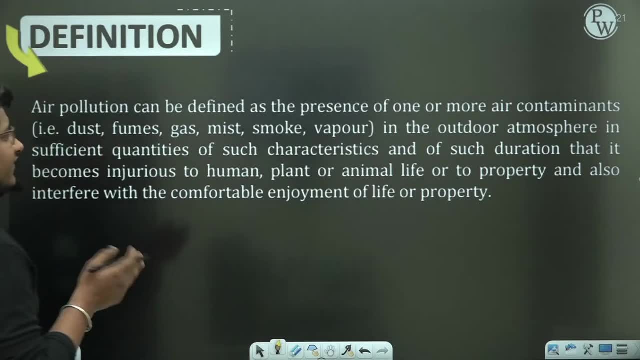 So what is that? It is the cause of air pollution. You call it pollution when you feel that discomfort. Same thing I have written here also: Air pollution can be defined as the presence of one or more air contaminants. That is, either dust, fumes, gas, mist, smoke, vapour. 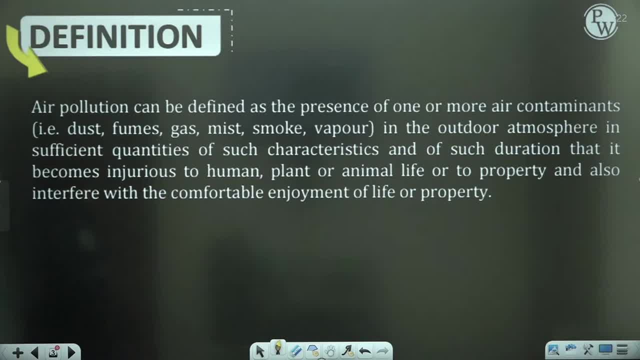 In the outdoor atmosphere Insufficient quantities, of such characteristics and of such duration That it becomes injurious to human, plant, animal life or to property And also interfere with the comfortable enjoyment of the life or property. So when did you say air pollution? 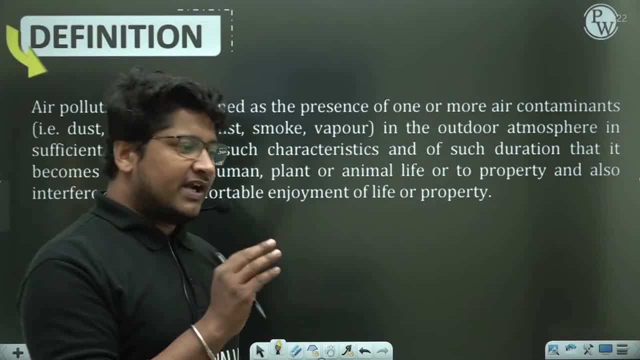 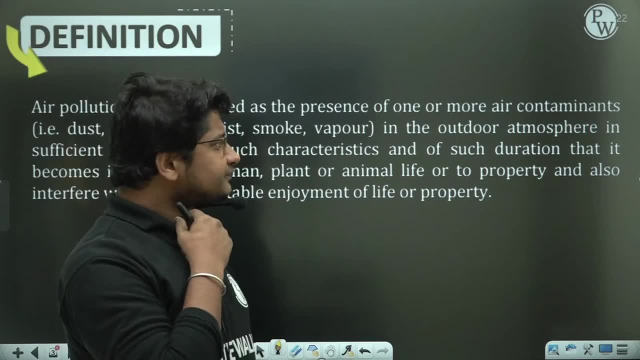 When you had a problem. If any pollutant is in such quantity And it has so many characteristics that it is affecting you, So we are also able to call it air pollutant. So you understood the topic of air pollution. Now, when we are talking about the atmosphere, 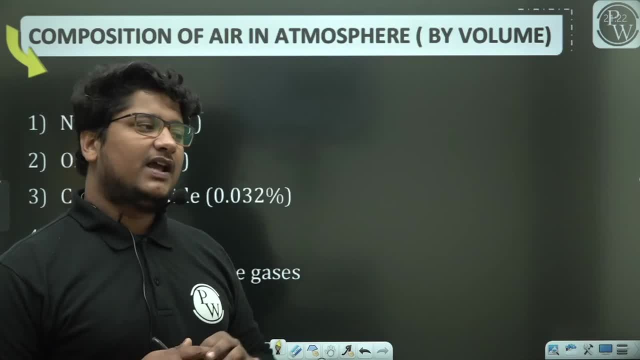 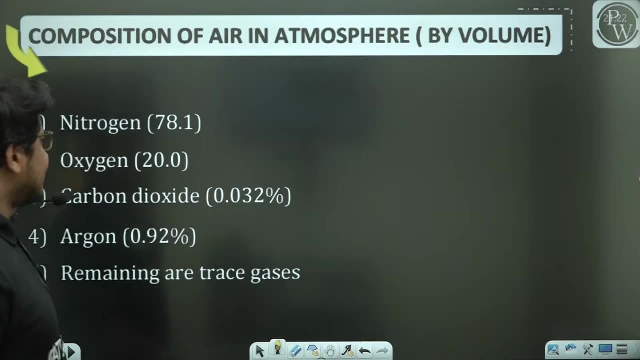 When we talk about air pollution in the atmosphere, obviously. So let's recall some basic things about the atmosphere. Like in the atmosphere, you have 4-5 things which are present. Gases like Nitrogen is approximately 78.1.. 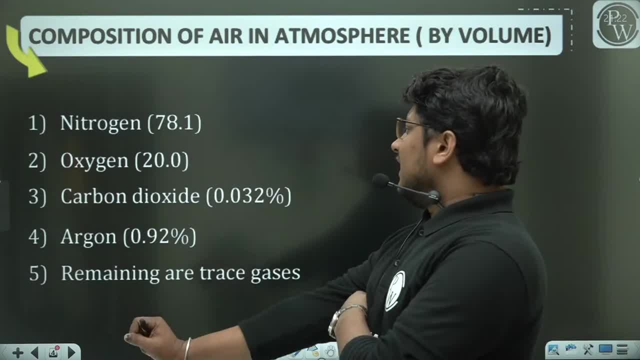 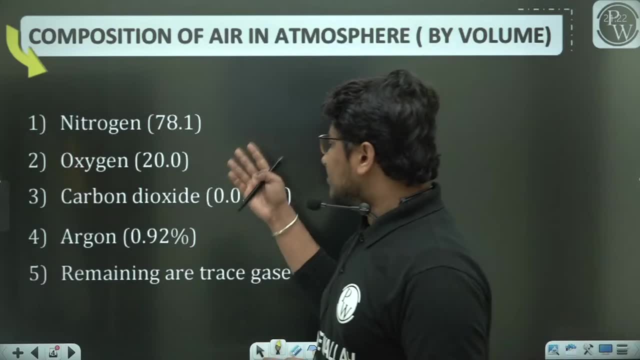 Then Oxygen is approximately 20.. A little more: Carbon Dioxide is 0.032%. Argon is 0.92%. The remaining are traces of gases. So this is your general composition of your atmospheric air And similarly, your atmospheric layer is different. 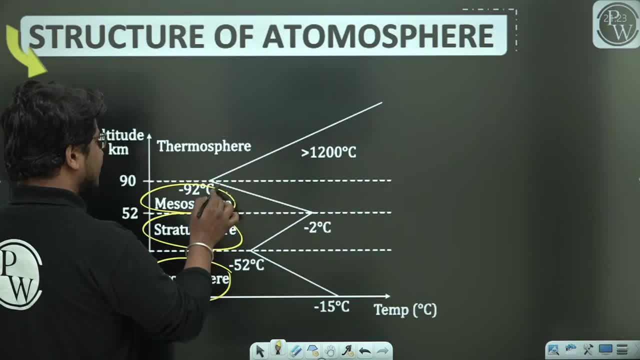 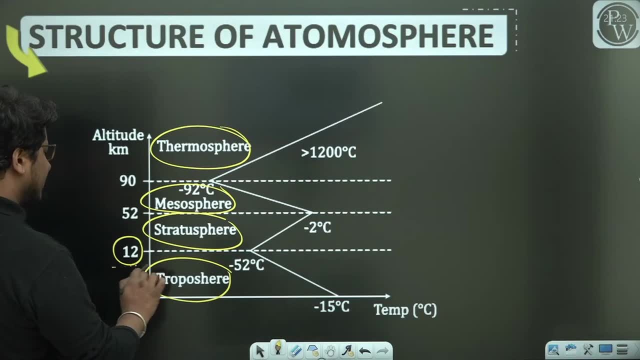 One is your Troposphere, Then your Stratosphere, Then Mesosphere, Then Thermosphere. You have different layers And what you have seen is that a particular range of different layers. For example, you have Troposphere up to 12 km. 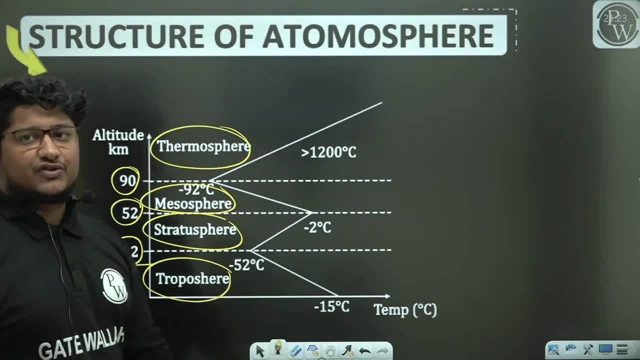 Then you are saying Stratosphere- up to 52 km, Up to 90 km. You are saying Mesosphere. It can be a little up or down, You don't have to worry about it, But the thing you have to understand the most here is this: 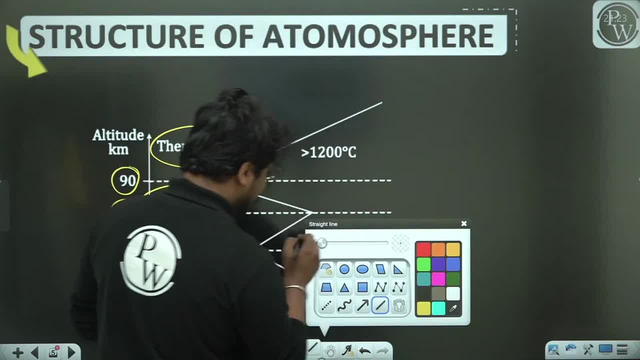 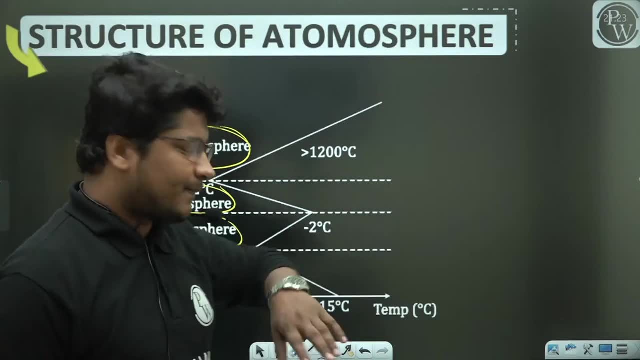 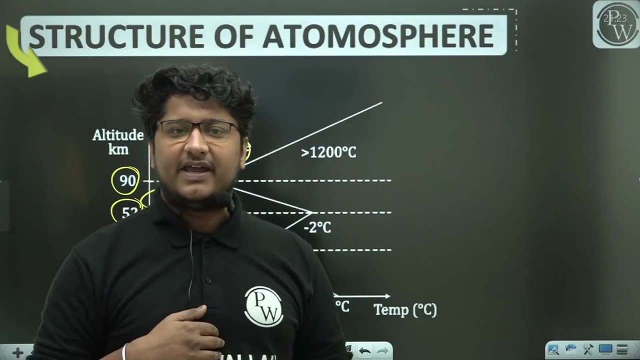 How is the temperature variation happening? This is the most important thing you have to understand Now. understand what is happening with the temperature variation. If I talk about the Troposphere, So in the Troposphere, as you go up, Like you all are in the Troposphere. 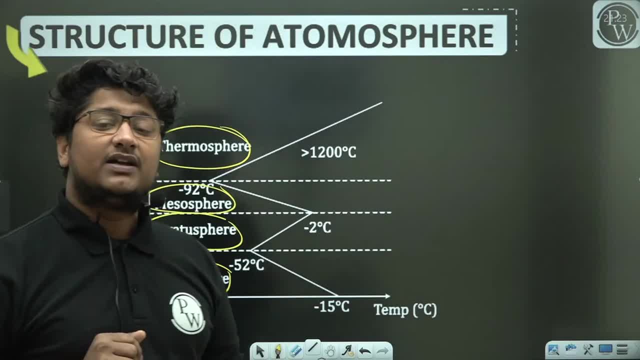 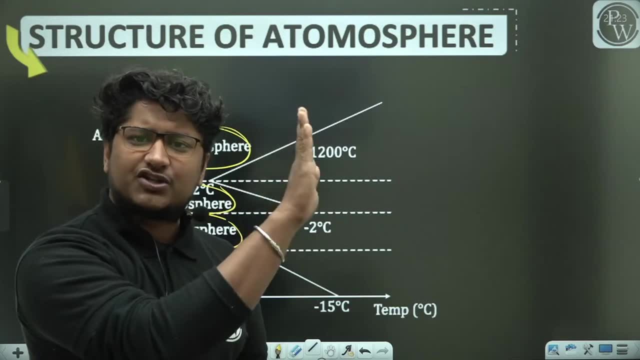 So, as you go up, does the temperature decrease or increase? Sir, the temperature decreases, You know, even if you see normally Like if you are going on a flight, If you are going on an aeroplane, So its glass is dry. 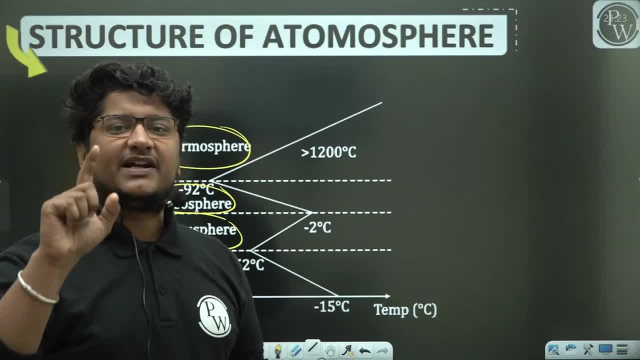 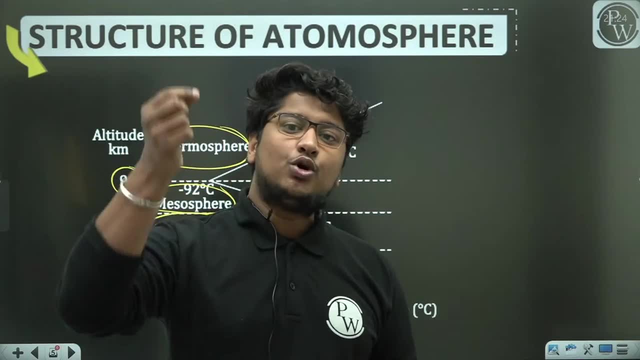 You will feel cold. So as you go up, your temperature decreases. Keep this in mind Now understand the reason for this. The reason for this is that the more pollution you have in the city, Or the more heat you have in the construction area, 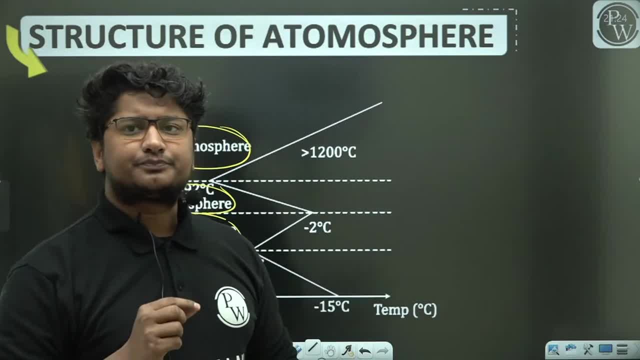 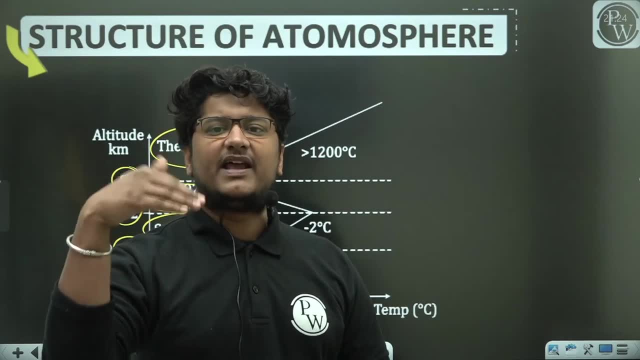 You will be able to relate with that Understand. If you go to the mountains, Or you are living in a lower innocence in Delhi, Or you are living in Mumbai, Or you are living in Kolkata, Or you are living in any city. 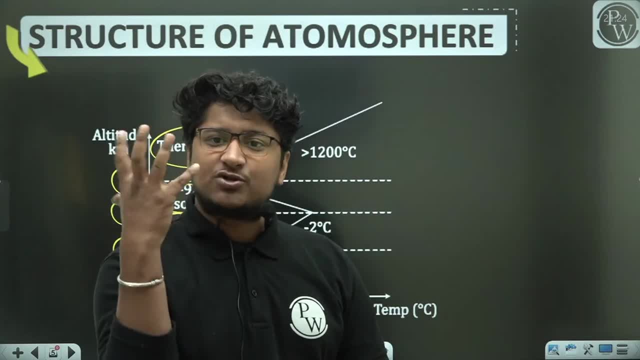 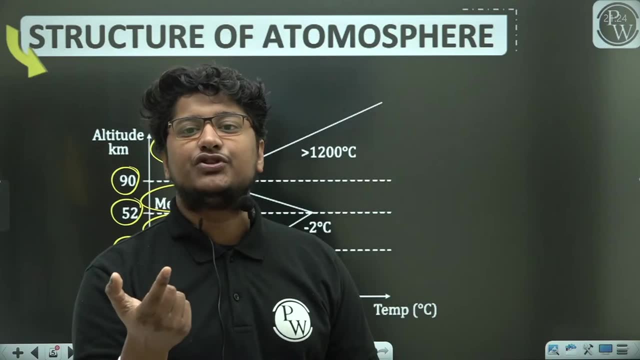 So when you live at a lower level, So in that case the air you have There will be a lot of particulate matter in it, Where there will be more particles. Particles have a tendency of, Or particles have a characteristic to absorb light. 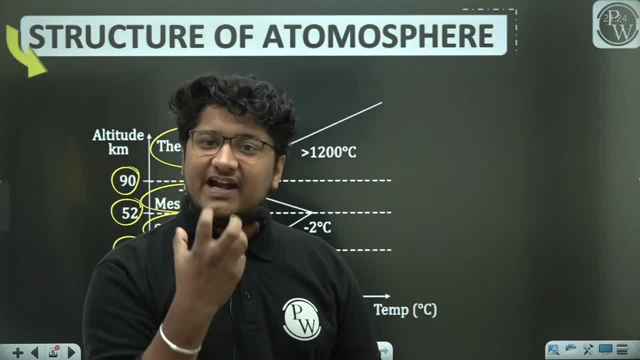 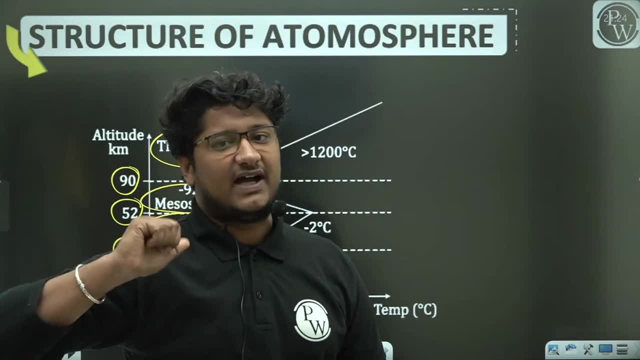 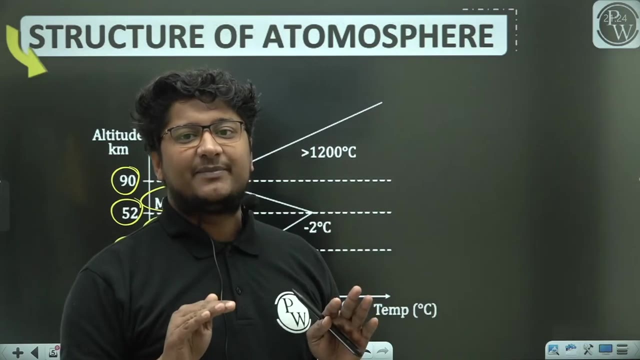 So the more particles there will be, The more that light will absorb. And if the particles around you have absorbed more light, Then no doubt your temperature also increases. Now this means that the ground surface, below Which is your earth surface, It remains at your highest temperature. 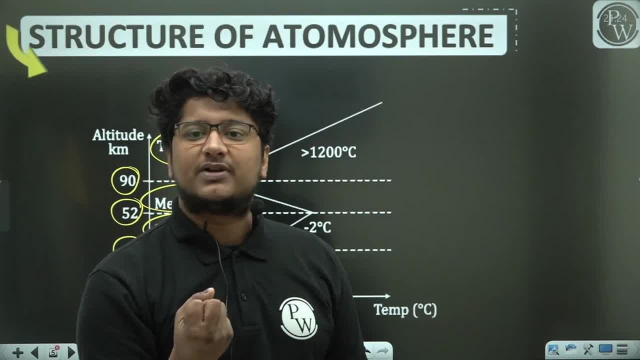 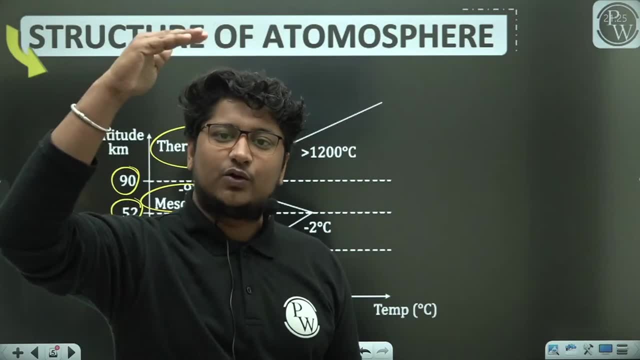 Because light comes from the sun. There are particles, All the particles absorb light And it remains hot. So as you run away from the earth surface, As you run away from the earth surface, You are going away from the earth surface. In that case, what happens? 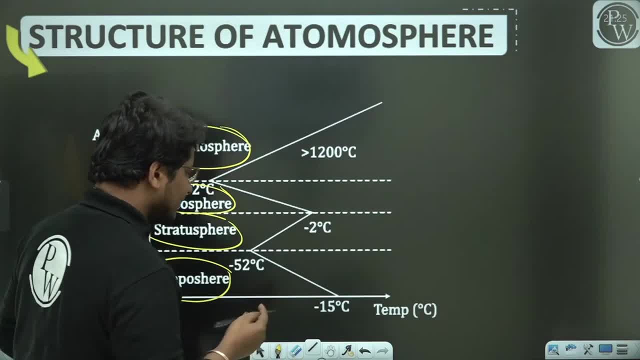 Your temperature will go down And that you can see it here. This is not minus. This is your minus. This is not your minus. Your curve is going down from 15 degree Celsius, Something like, Something going like this. Then what did you see? 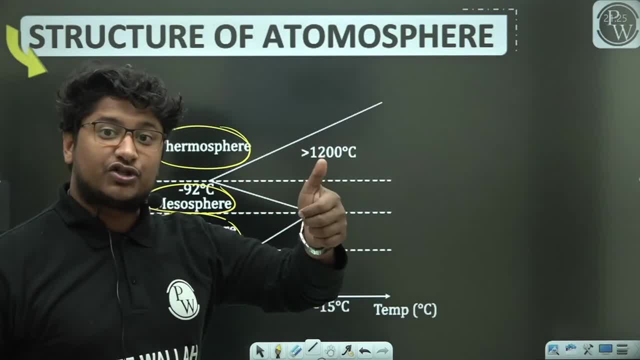 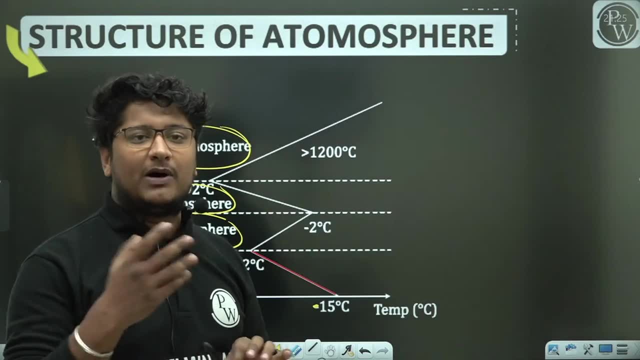 In the stratosphere. Now, what is there in the stratosphere? There is a beautiful layer in the stratosphere. We call it the ozone layer. Now, what is the ozone layer? Now you know what the ozone layer is, But let me tell you again. 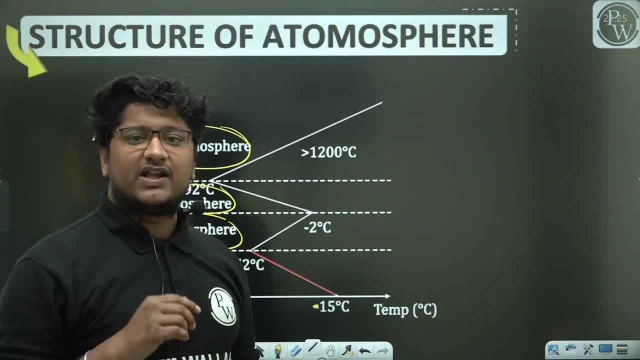 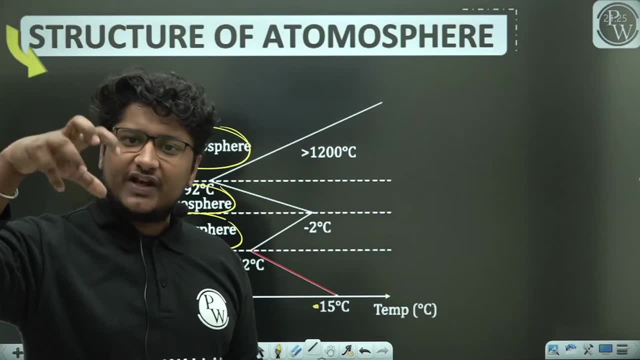 What is the ozone layer? There is a layer of O3 in the stratosphere Which does what? Which stops the UV rays coming in your sunlight, In the sense, It keeps the UV rays there. Now again, If someone is absorbing the sunlight, 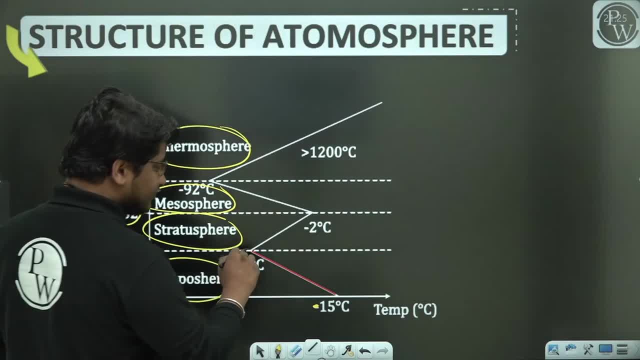 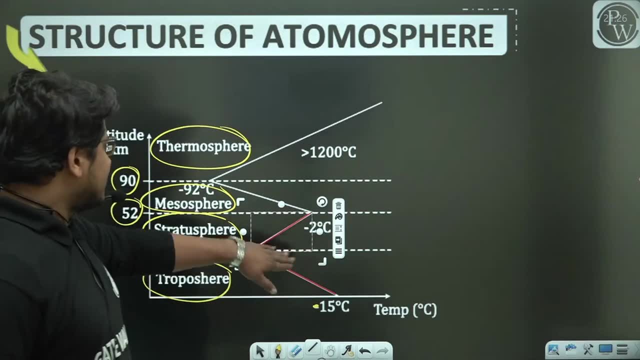 Then its temperature will be very high. Now, if you are going near it, If you go near any hot thing, Then your temperature will increase again. Okay, Next, coming to the mesosphere. Now its reverse: If you run away from a hot thing, 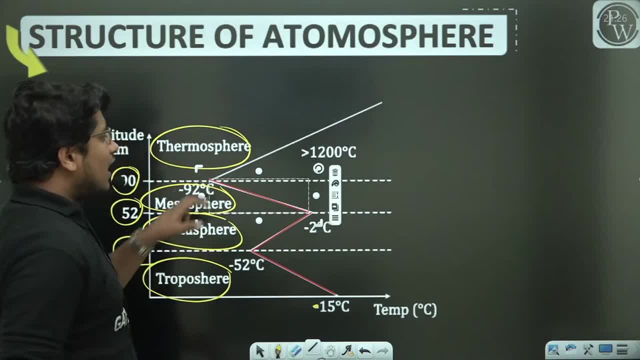 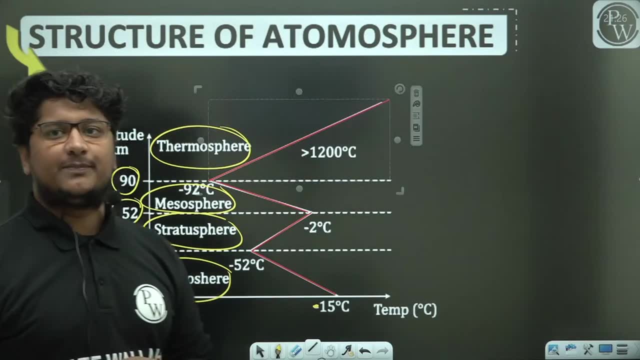 Then your temperature will be degrees again, And now, in a thermosphere, You are getting closer to the sun, So definitely the temperature will Keep on rising. Temperature will keep on rising. Who is this idiot? Secondary air pollutant? Did I talk about him just now? 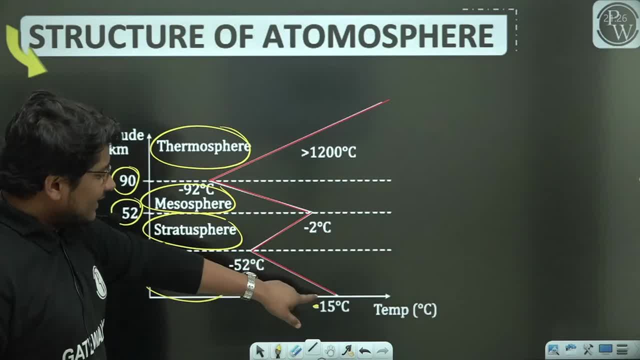 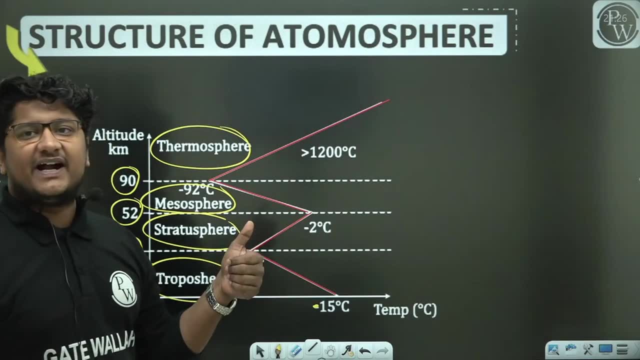 Don't give your own knowledge here. So what did I talk to you If you see, In every layer Your temperature is changing differently? Now I will ask you: Which layer are we going to talk about Out of these four layers? 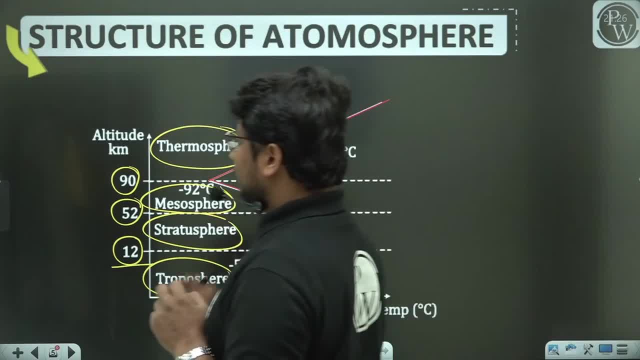 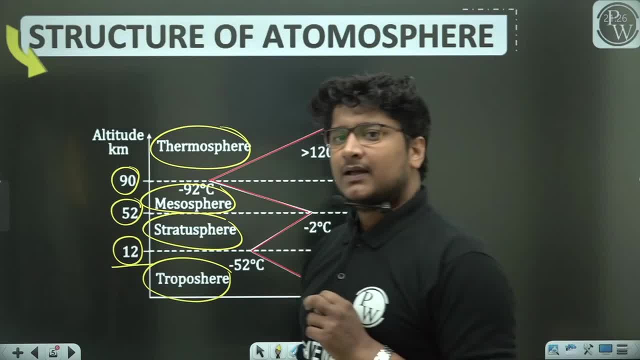 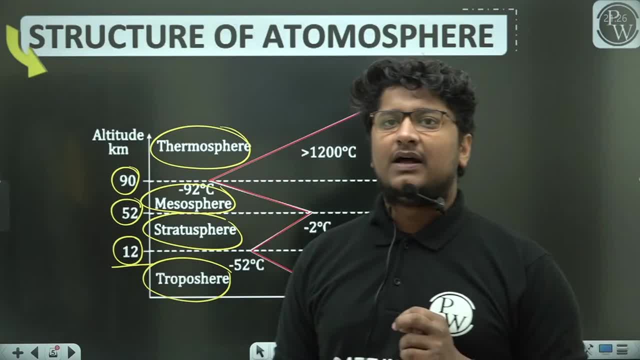 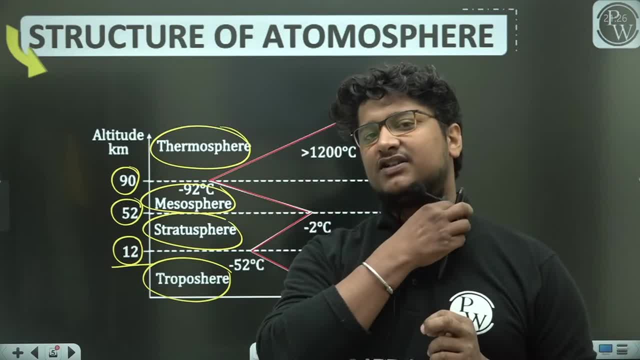 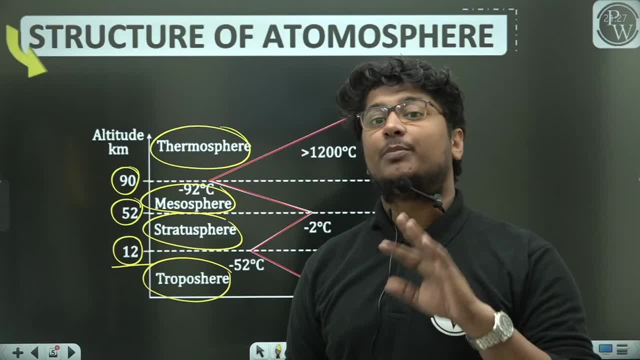 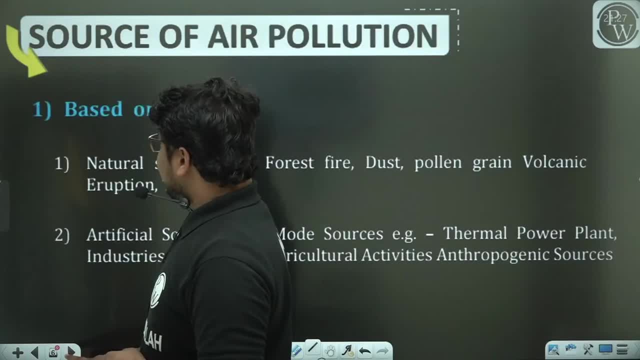 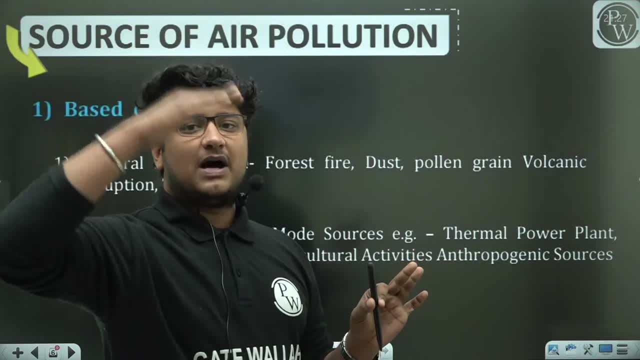 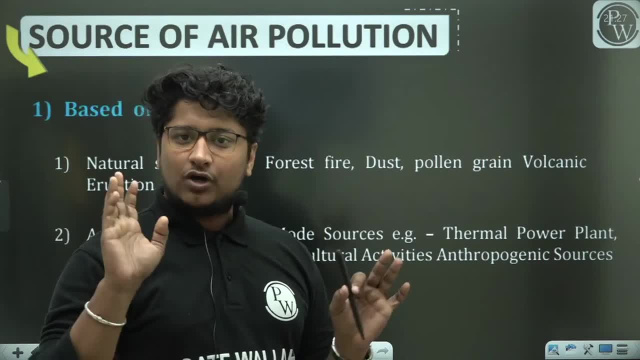 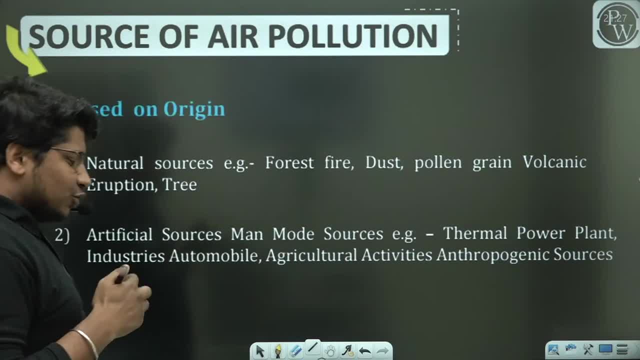 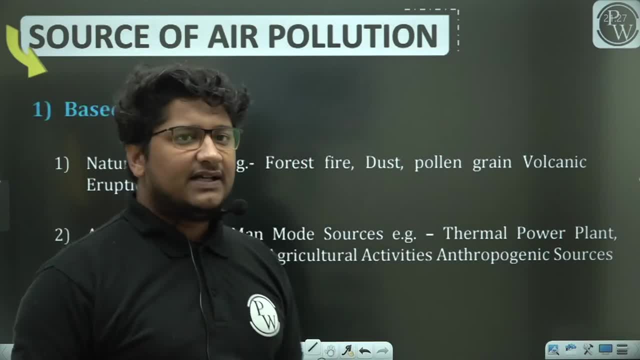 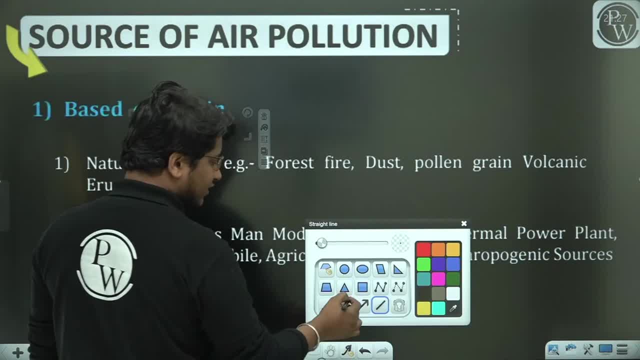 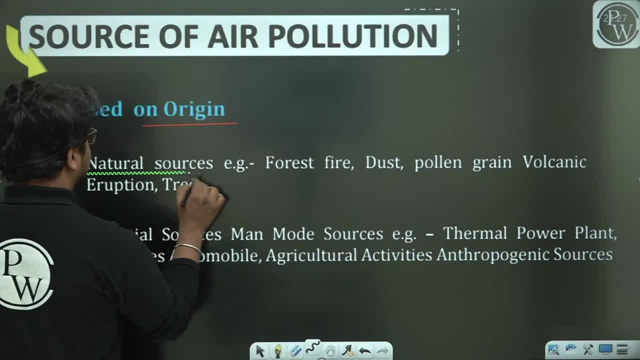 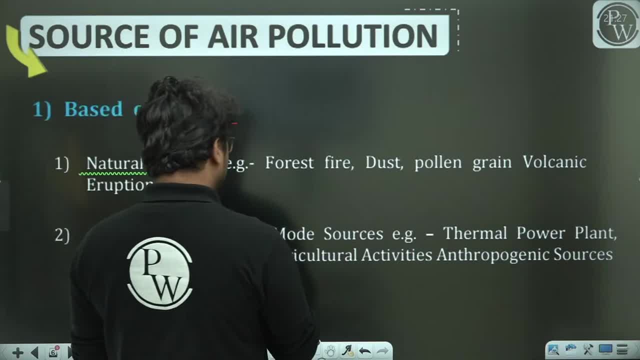 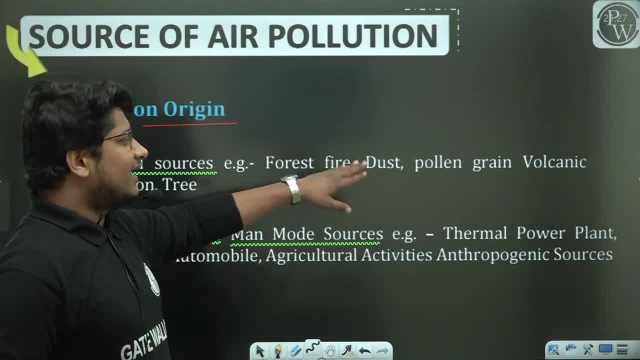 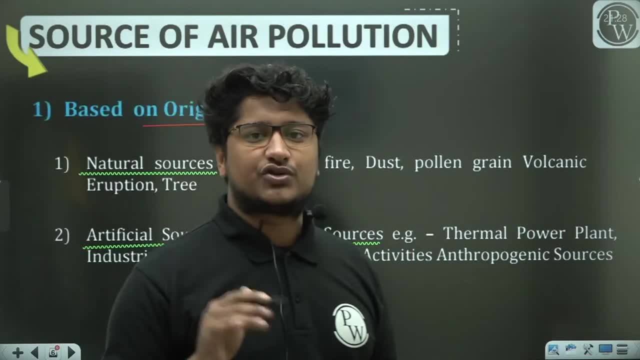 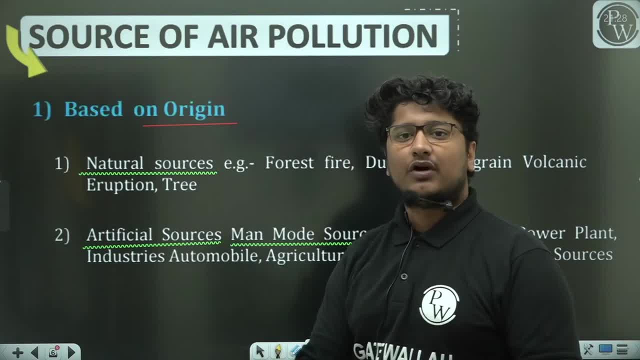 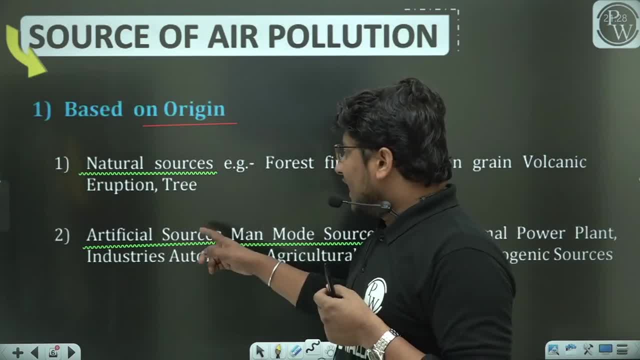 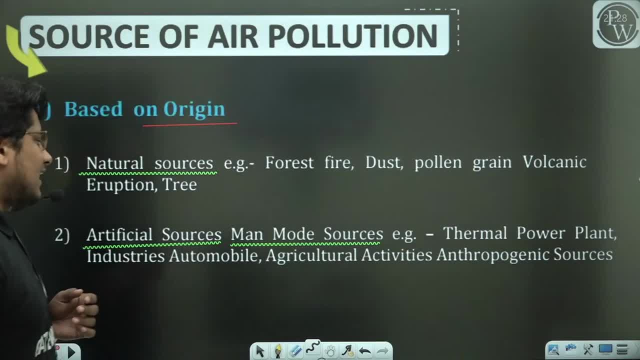 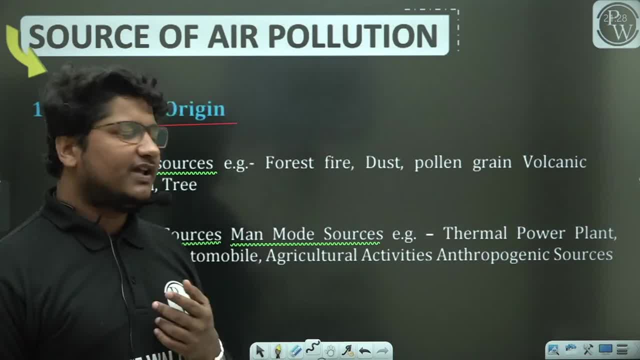 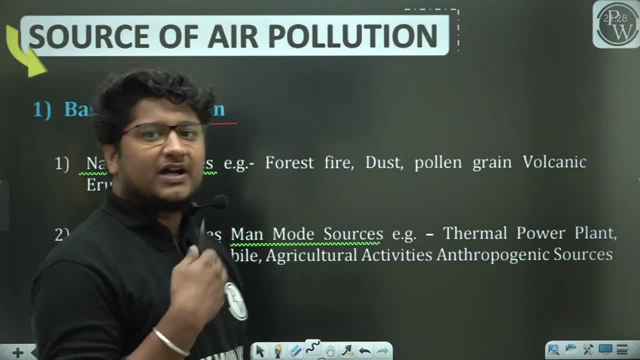 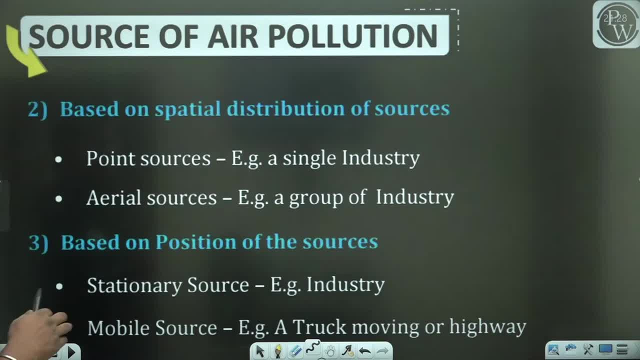 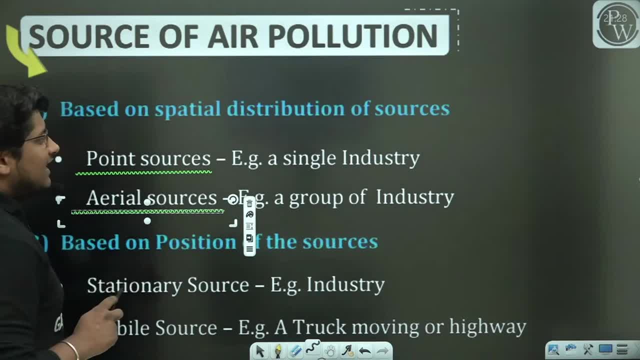 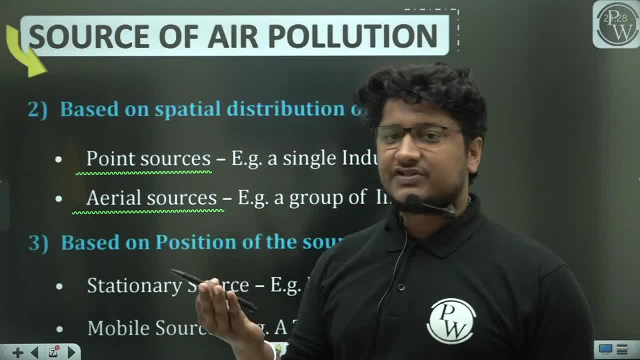 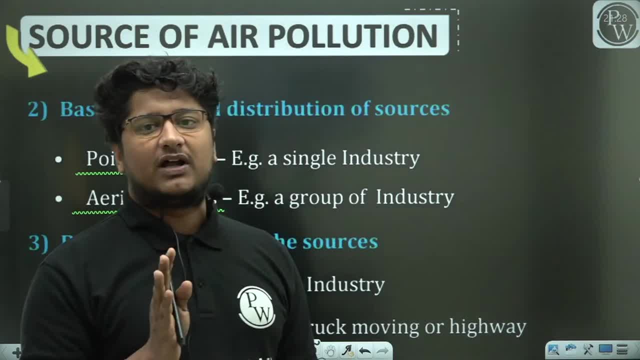 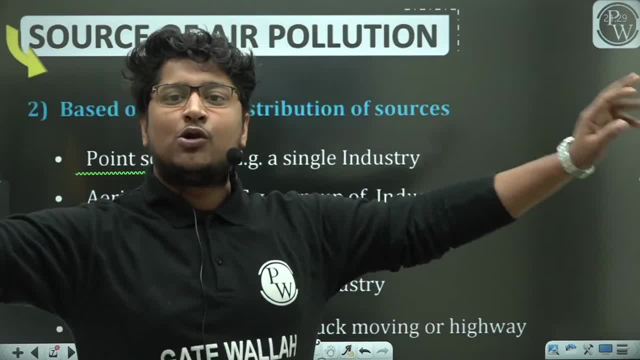 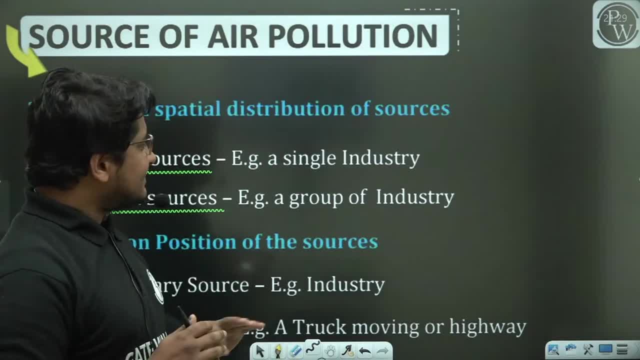 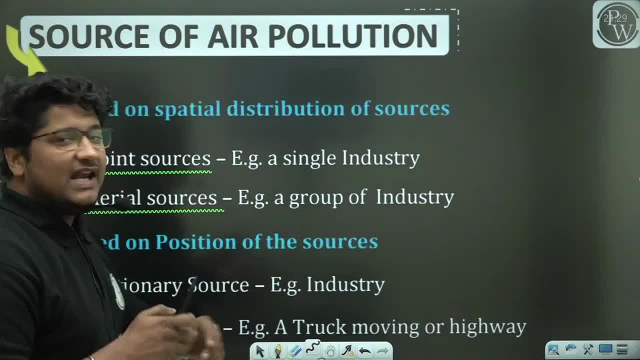 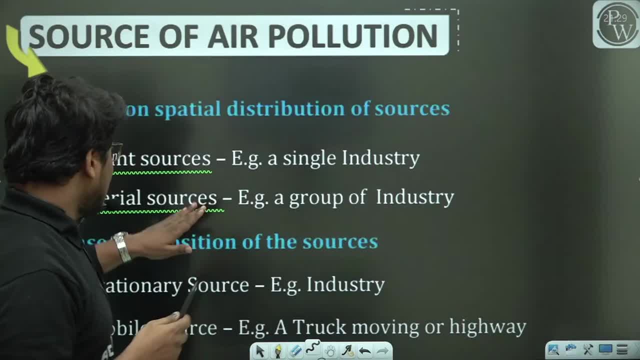 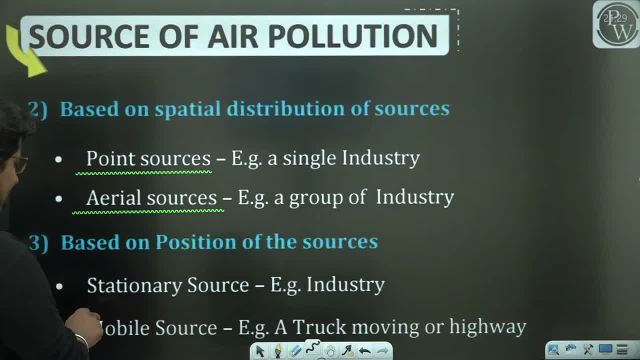 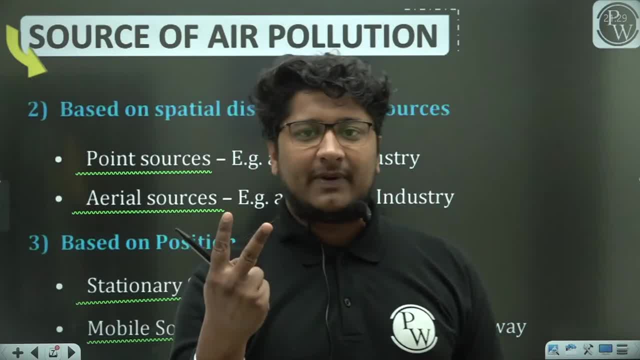 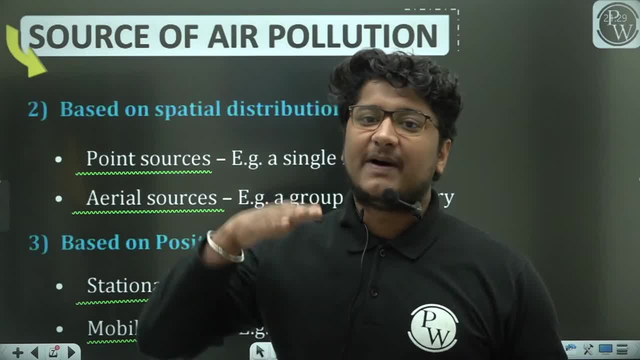 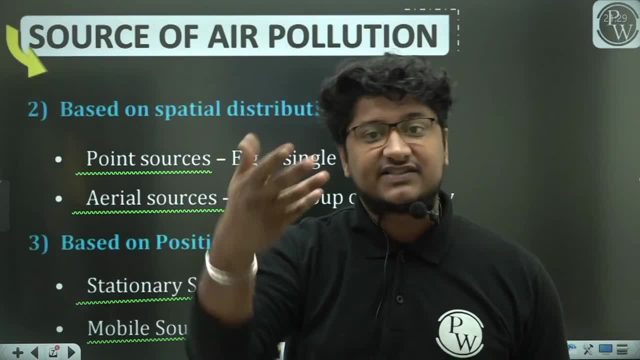 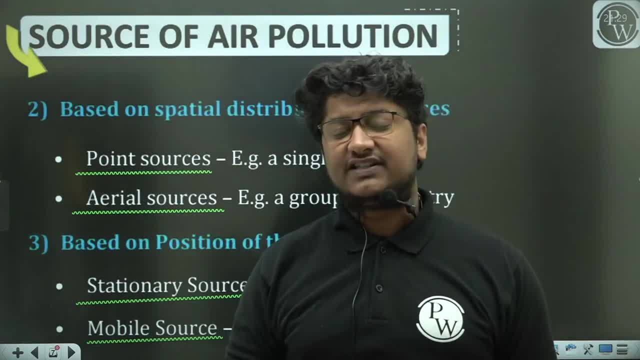 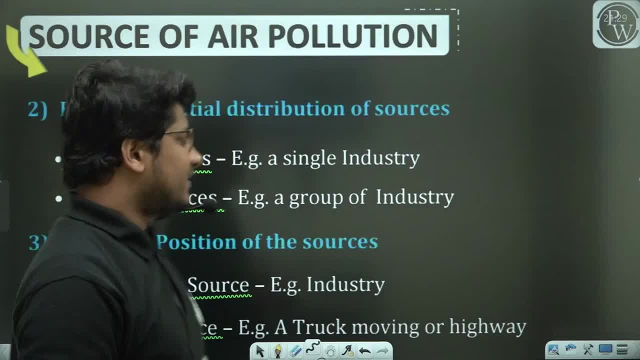 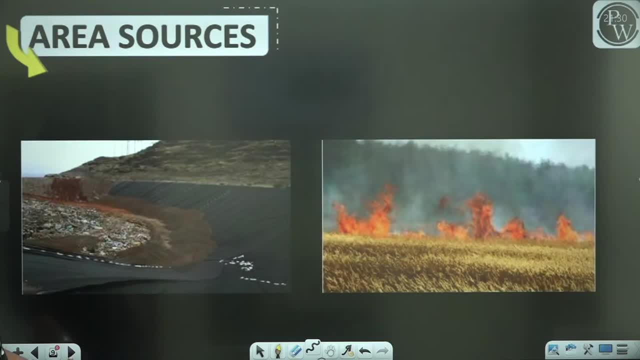 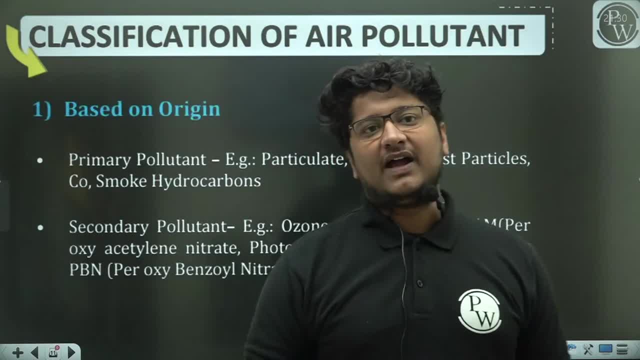 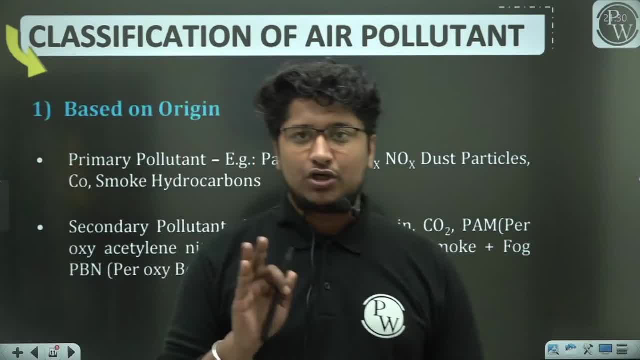 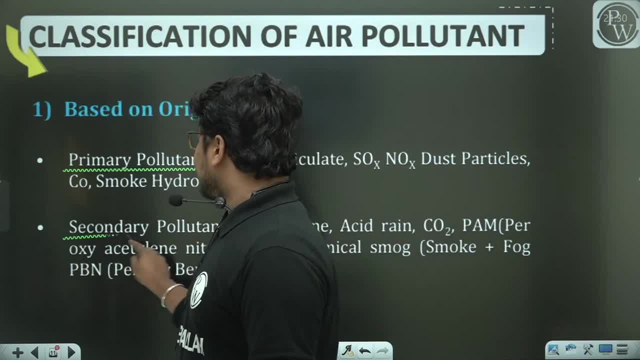 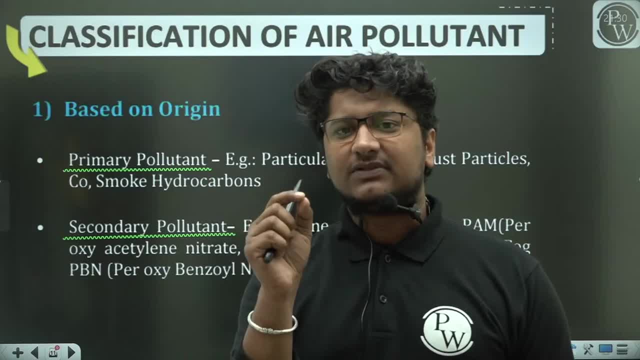 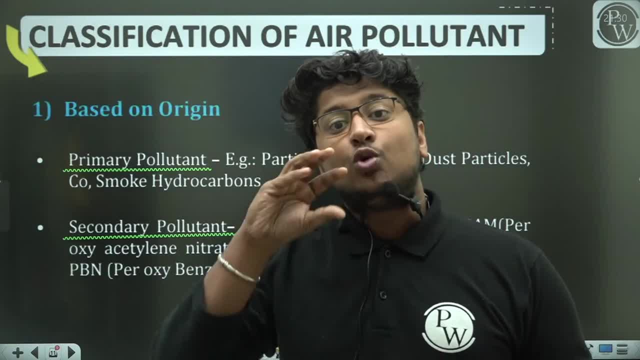 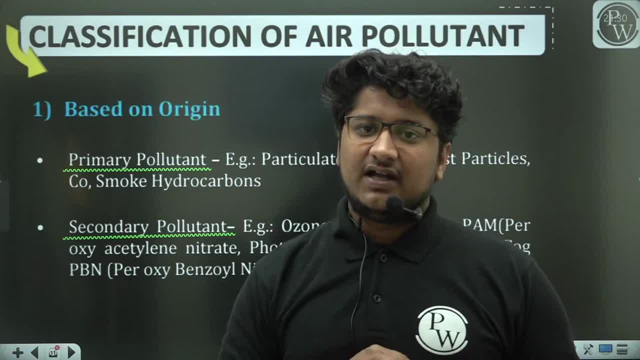 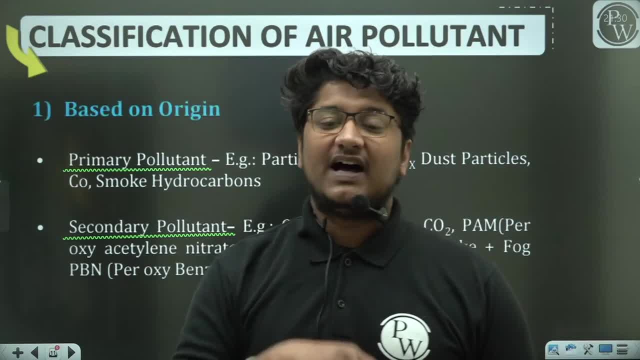 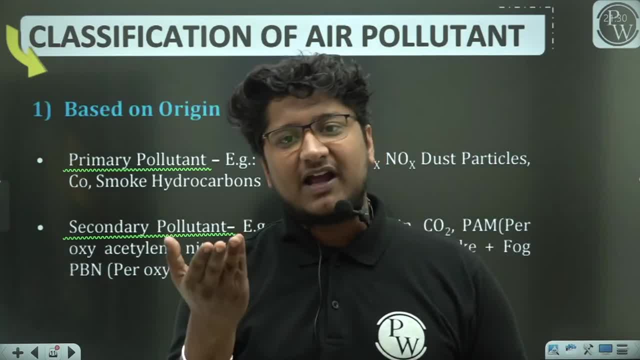 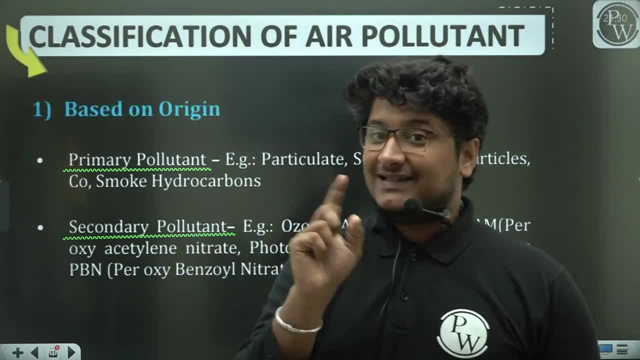 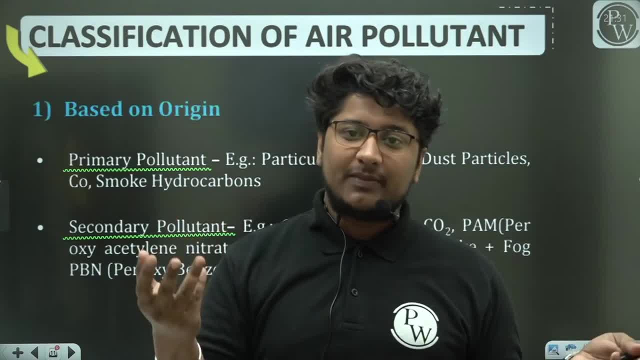 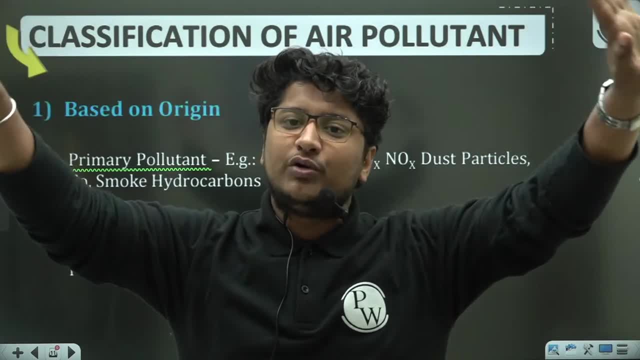 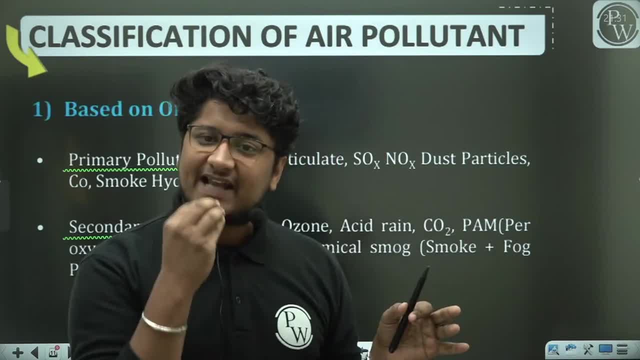 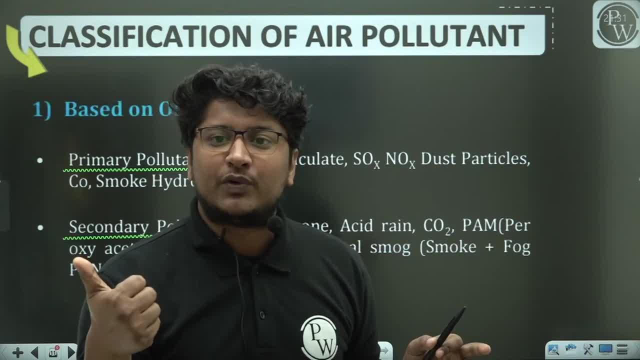 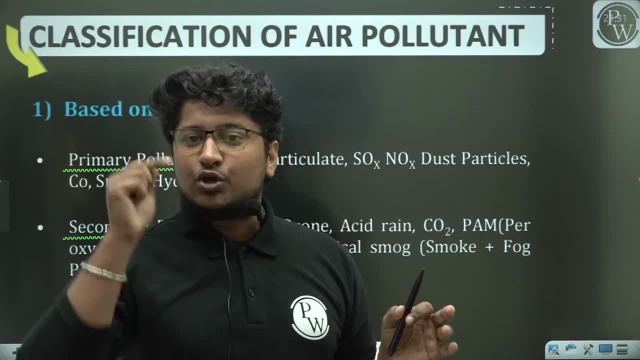 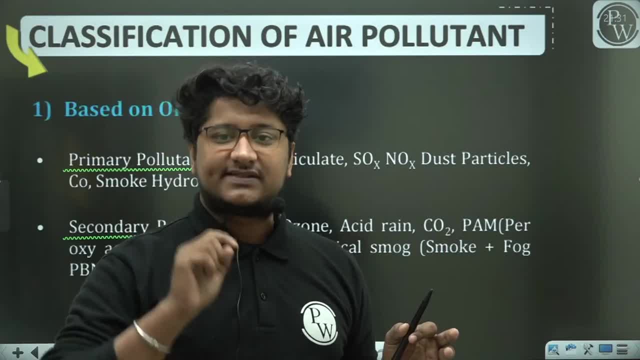 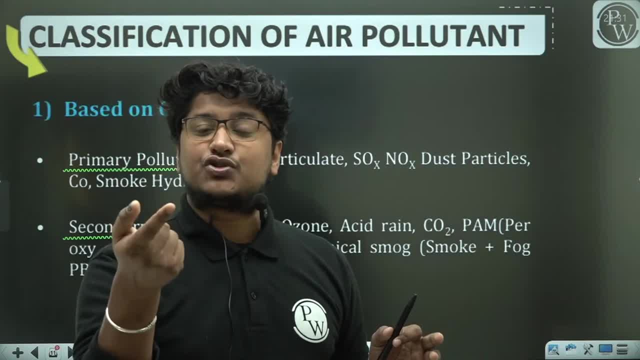 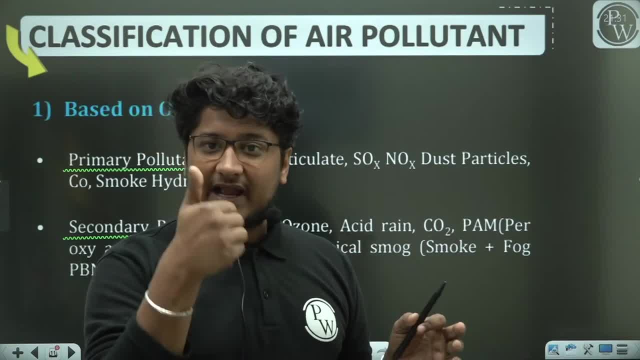 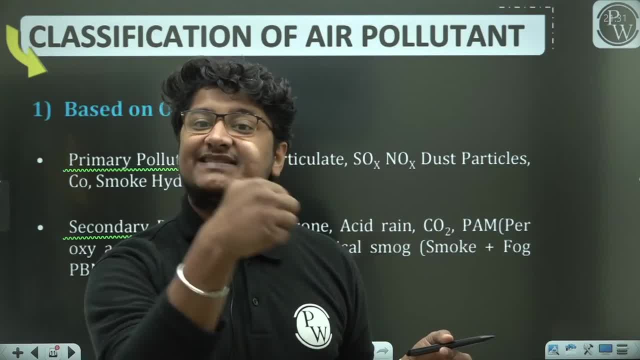 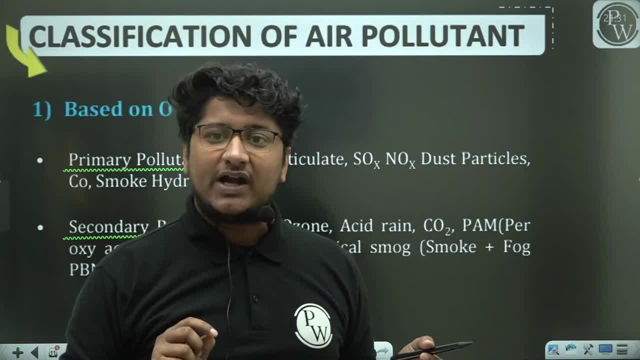 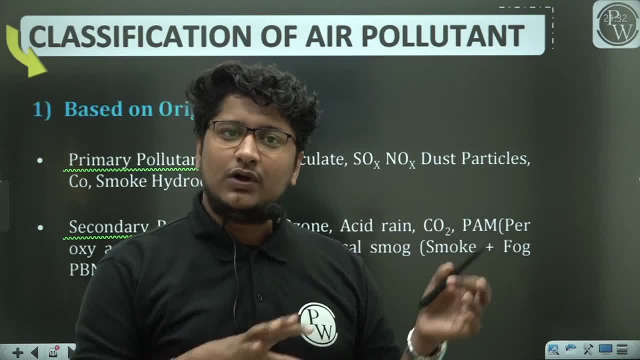 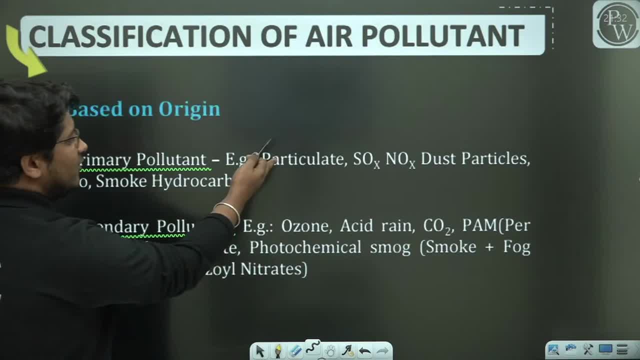 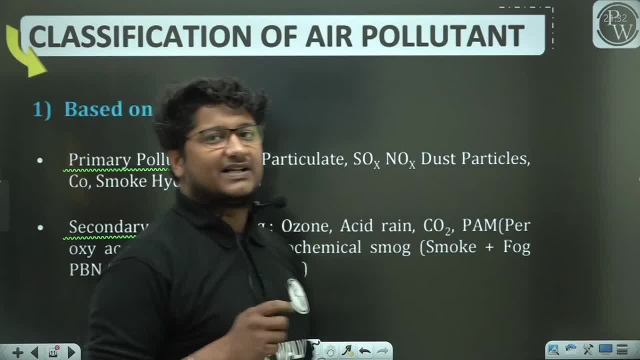 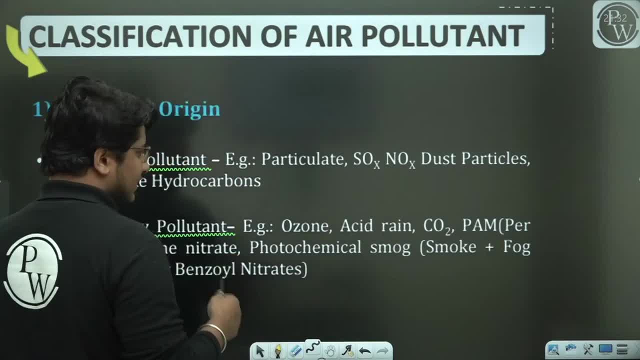 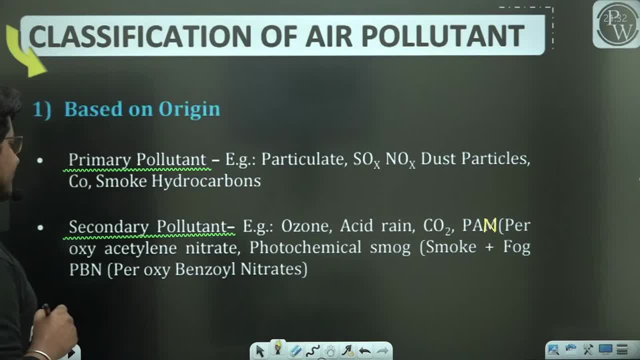 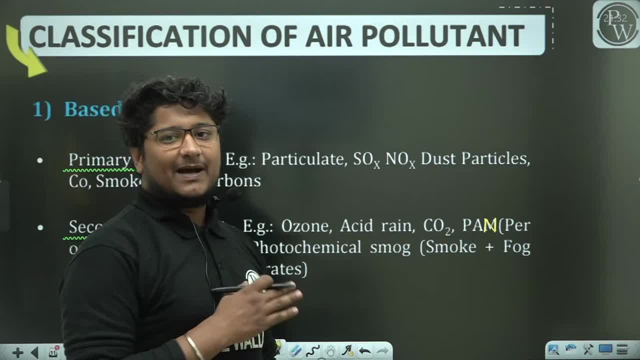 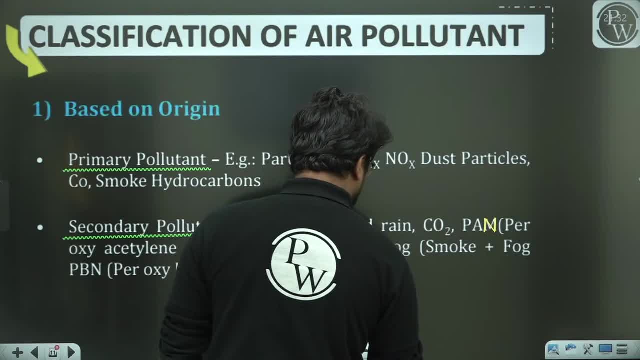 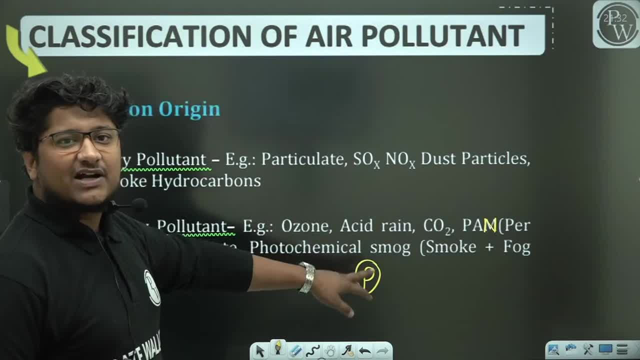 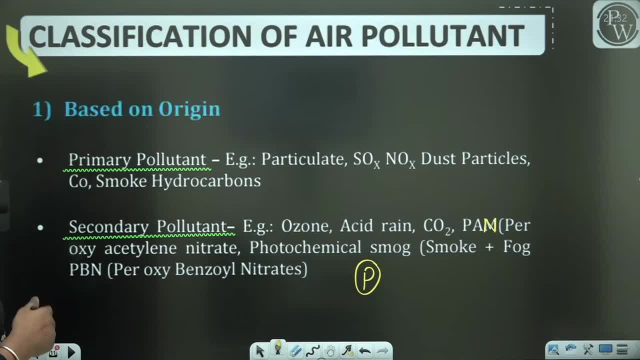 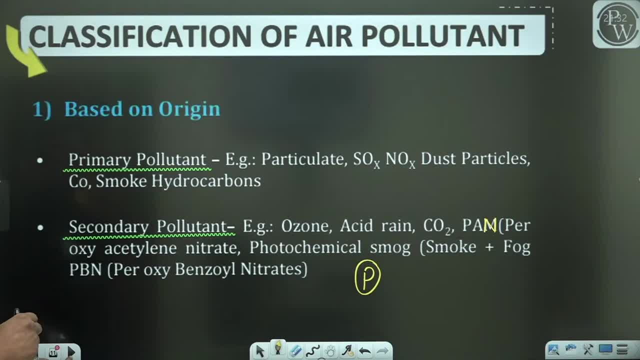 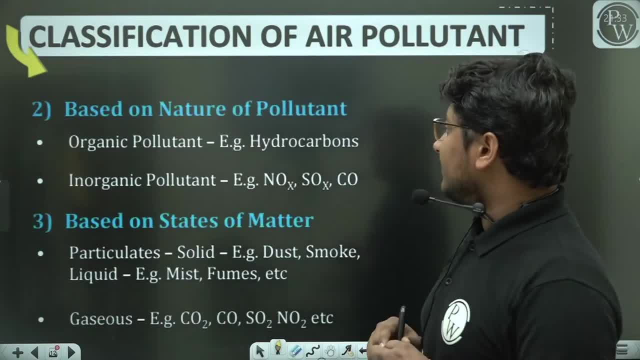 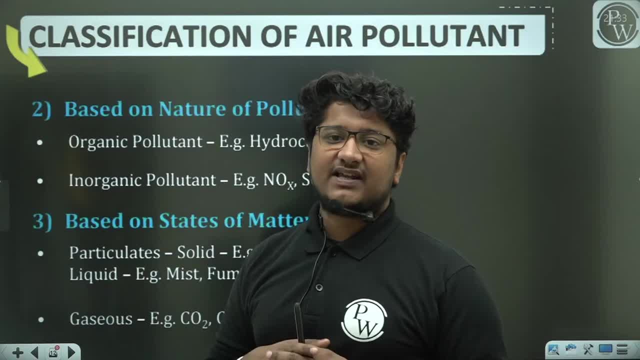 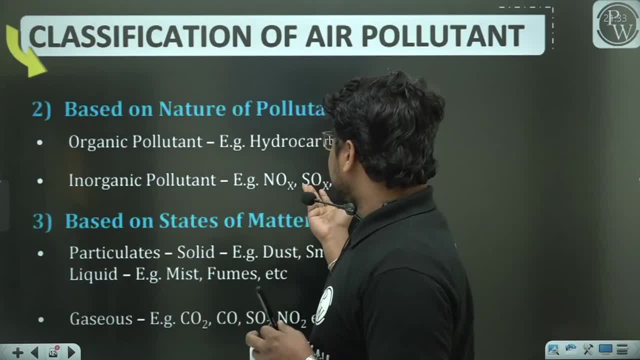 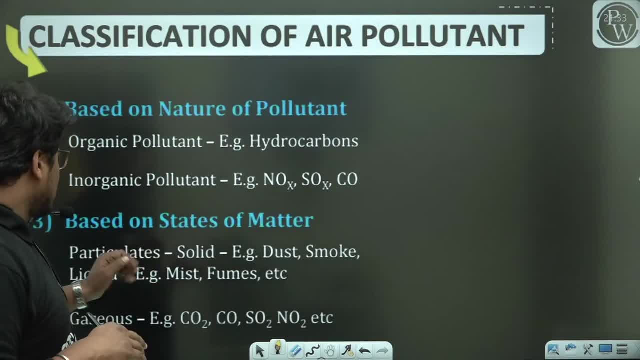 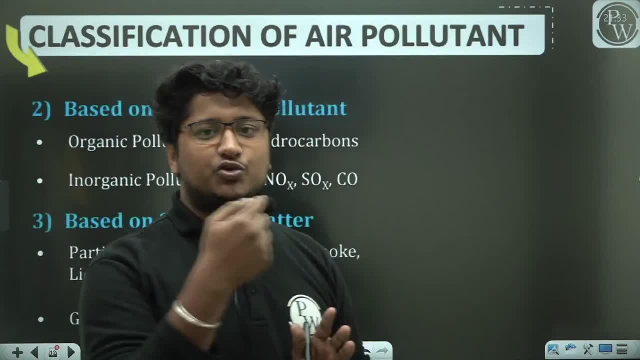 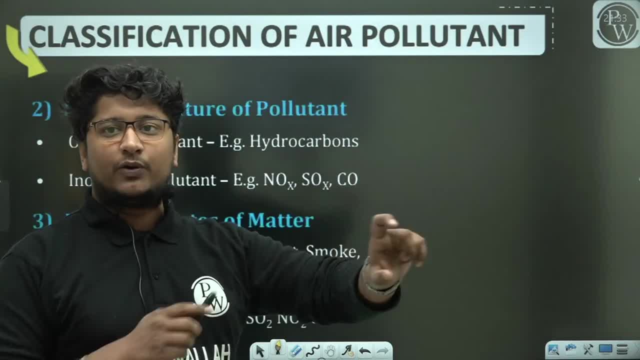 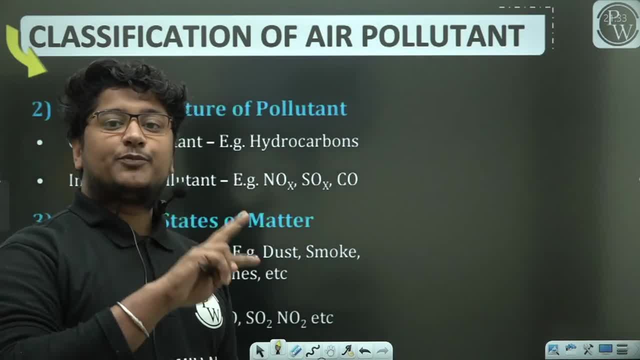 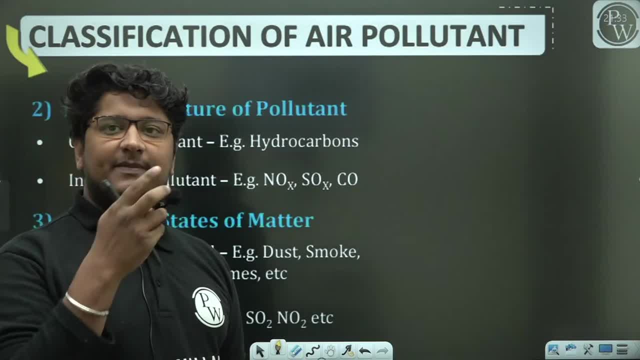 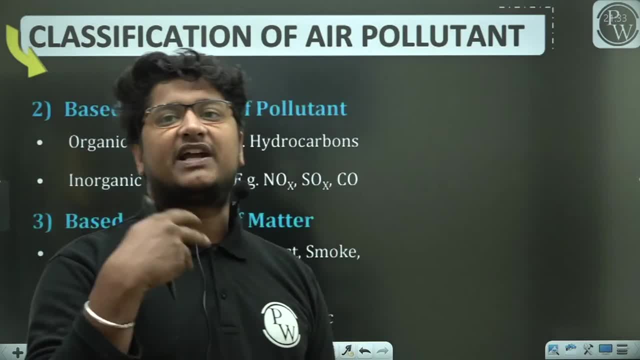 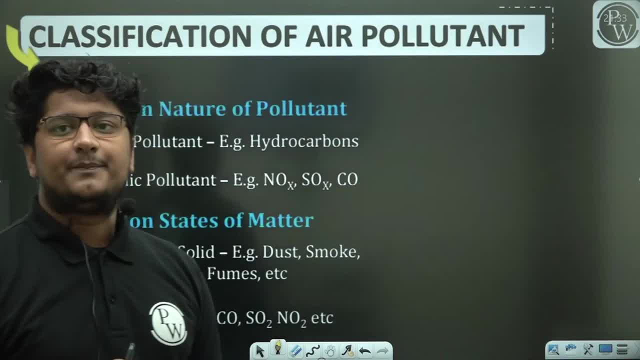 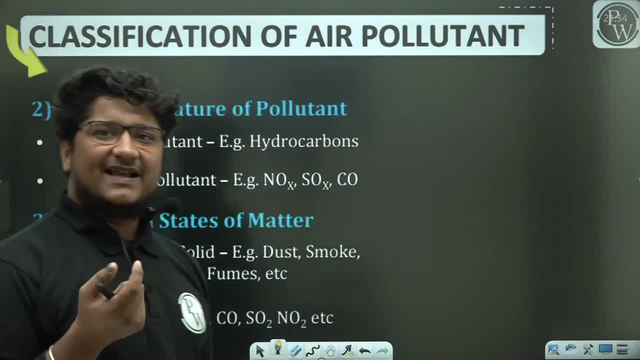 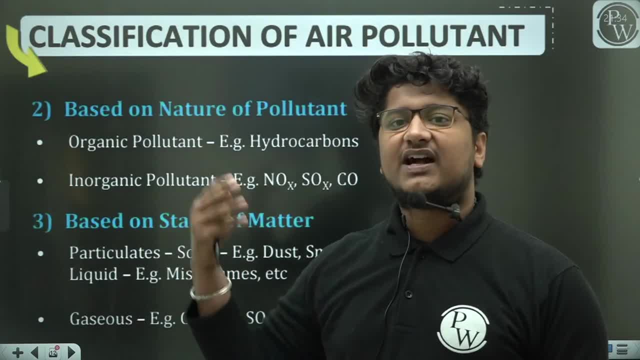 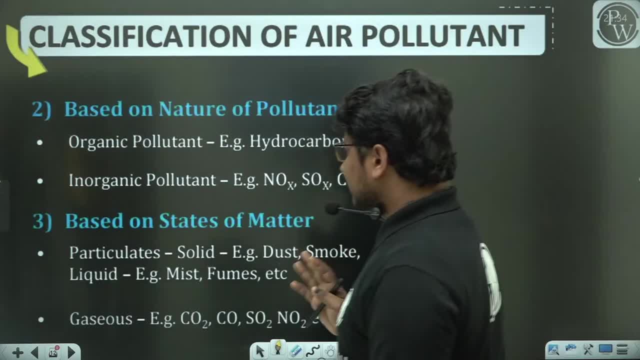 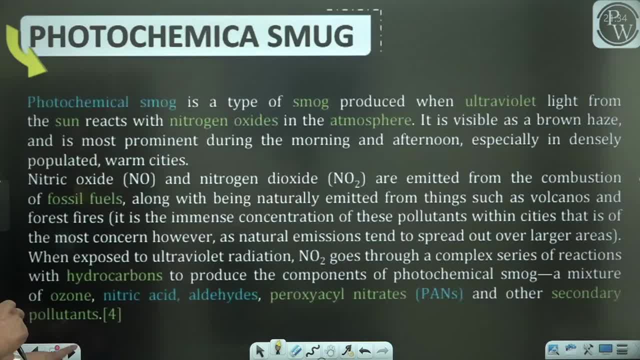 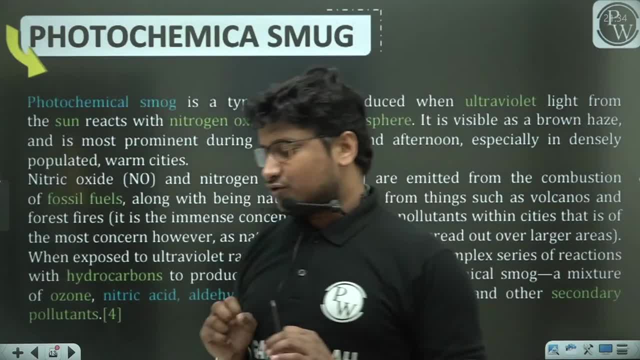 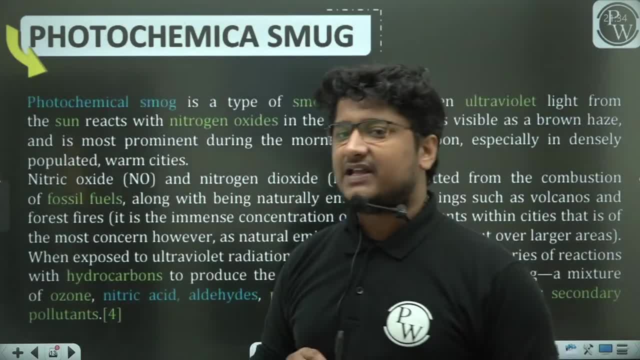 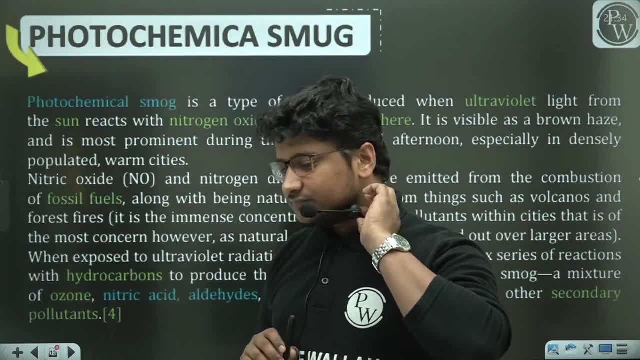 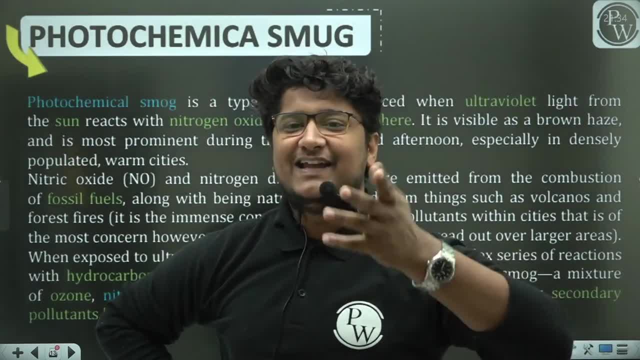 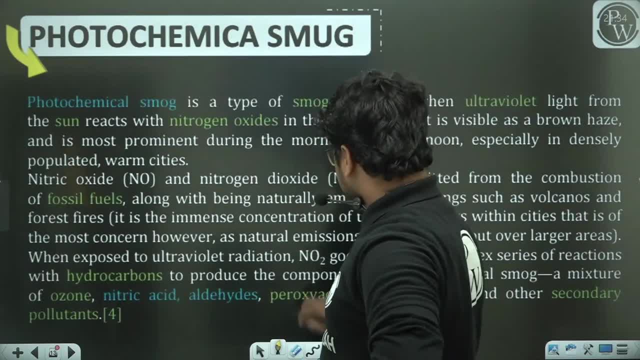 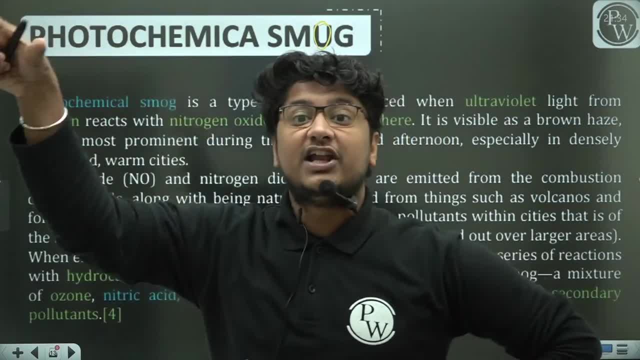 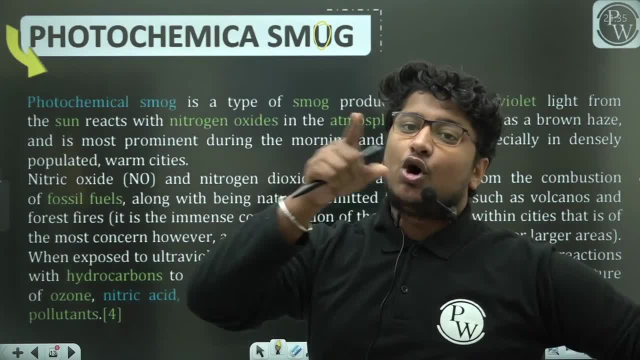 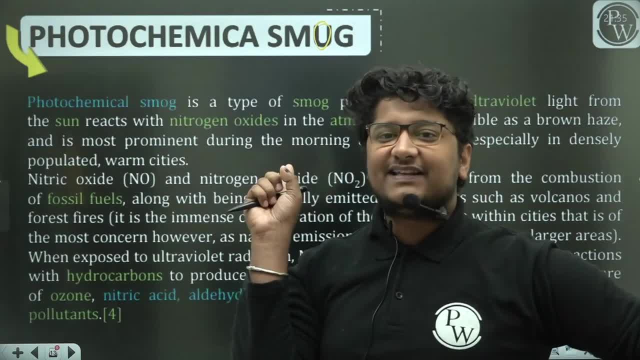 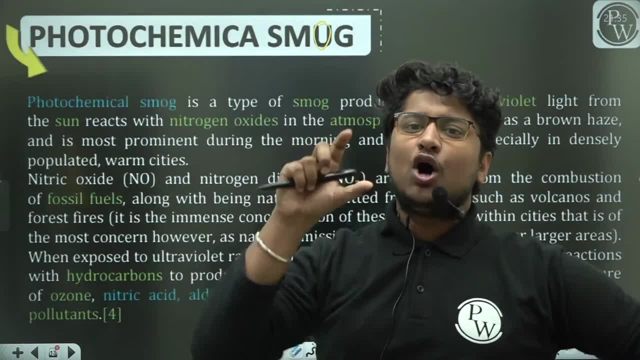 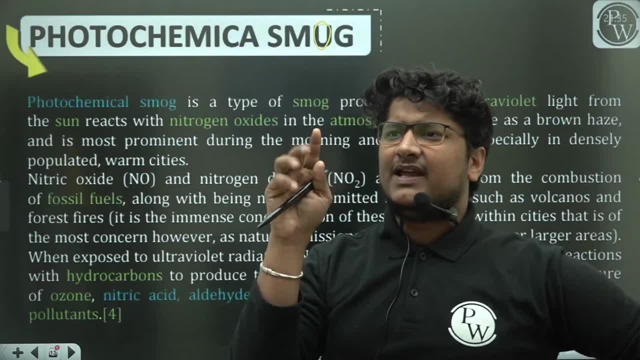 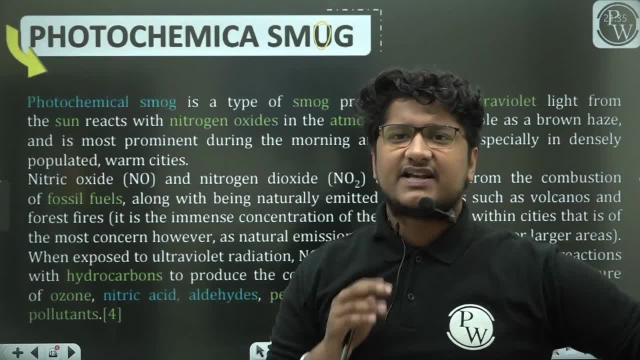 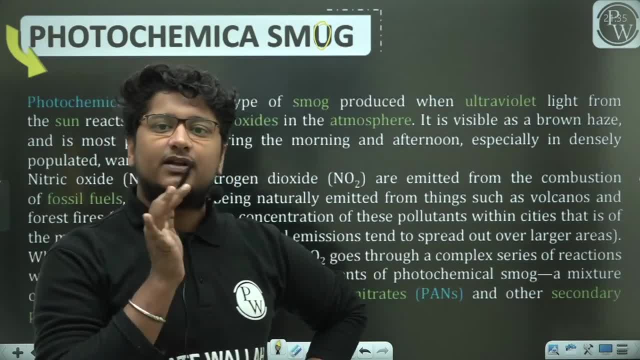 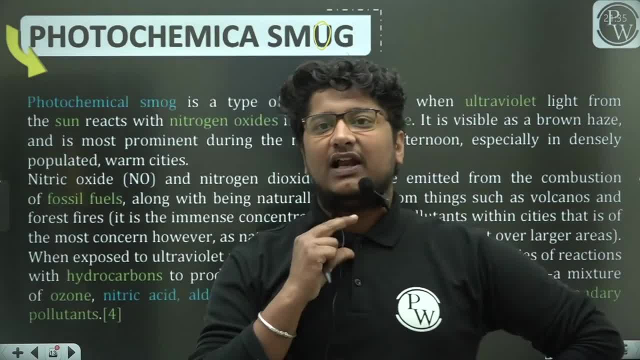 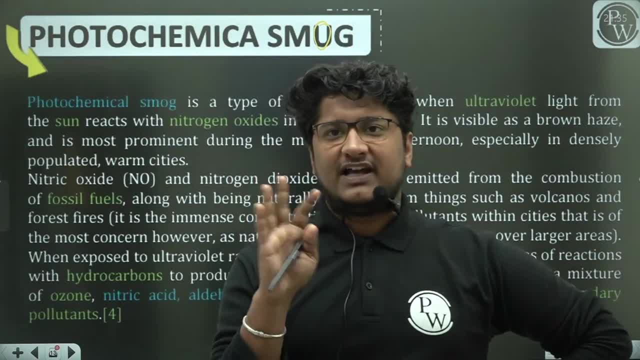 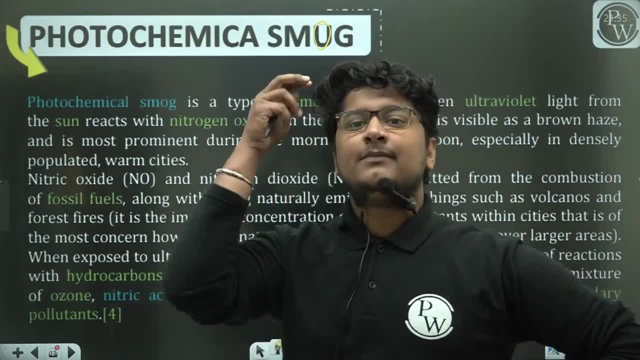 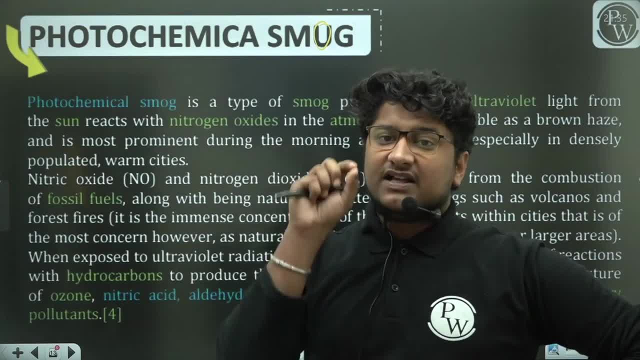 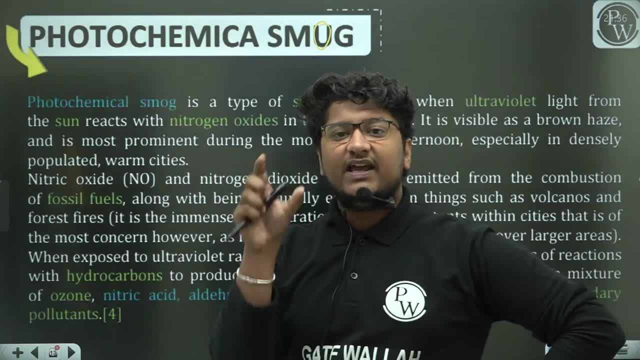 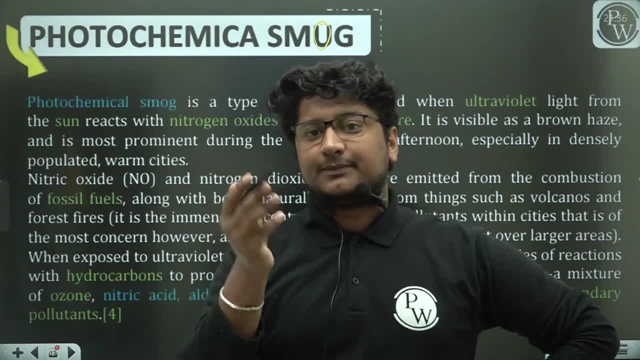 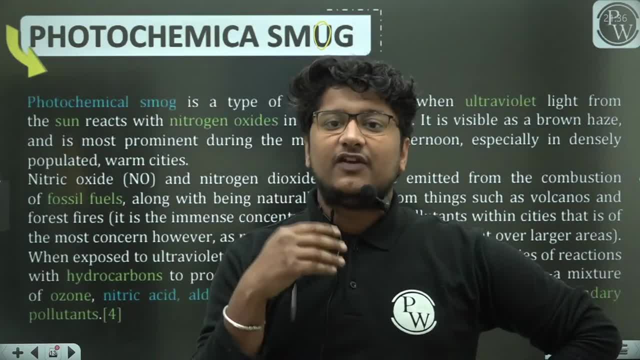 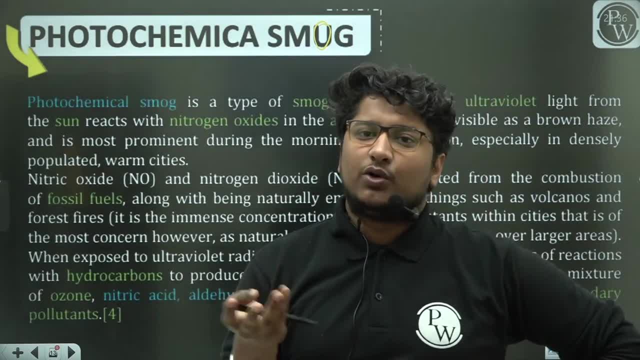 Which layer we are going to talk further. Which layer we are going to talk further. As long as you can resist, you can do it. then you die. So these things happened, which we call London Smog, Another type of smog that we call as Photochemical Smog. 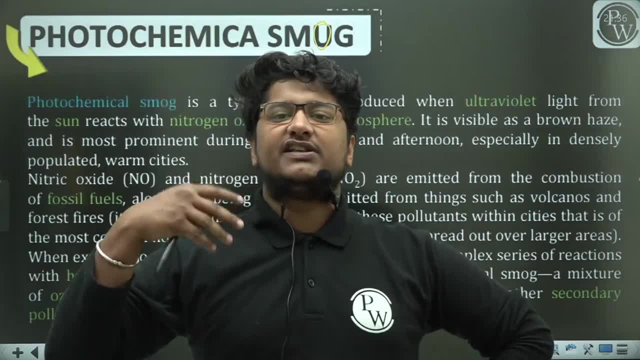 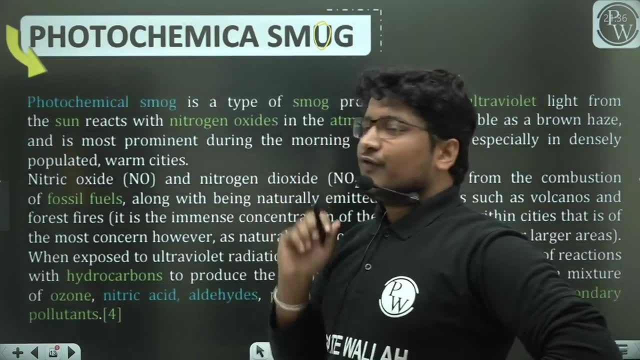 Or it is also called Los Angeles Smog. Earlier it was seen in Los Angeles. That's why Nowadays it happens in India too. There is nothing like that. So Los Angeles Smog is your Photochemical Smog. Now see what is happening in this story. 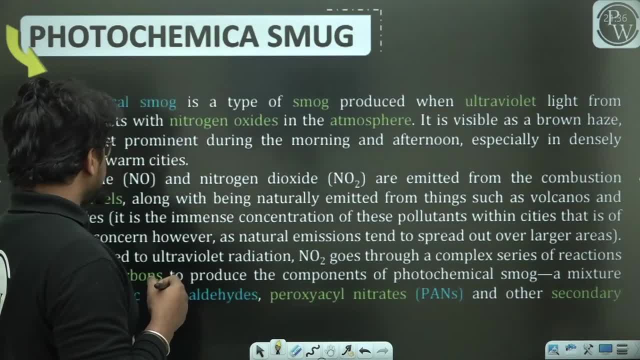 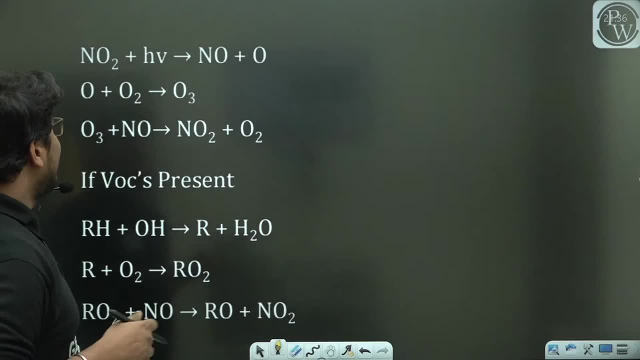 See this story of three chino. See this story. I will show you its reactions. You will understand it better. What is happening here? what is happening here? understand it from the reaction, Then I will also tell you in the figure. 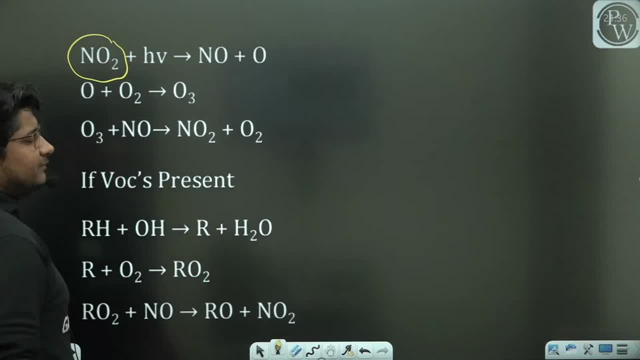 See, what happens is that you get NO2 from your automobile Nitrous Oxide. Okay, Now this NO2 part of yours, this NO2.. What happens to you? in the balance of sunlight, It broke in NO and O. 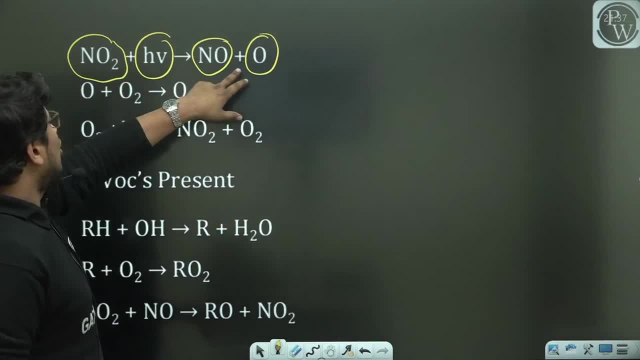 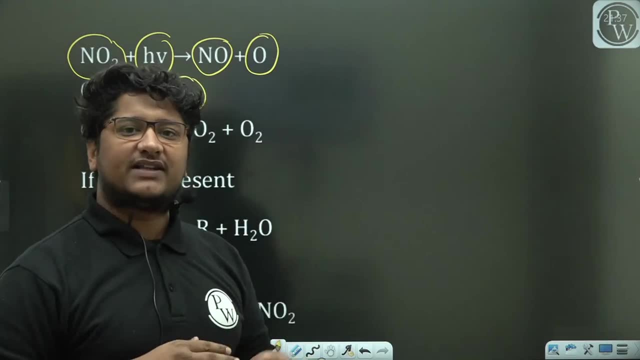 NO and O broke. Now this O makes O3 along with oxygen In the lower atmosphere zone. in a lower zone Means in a lower atmosphere zone. What happens to you at this height? Ozone is also there And means oxygen is also found. 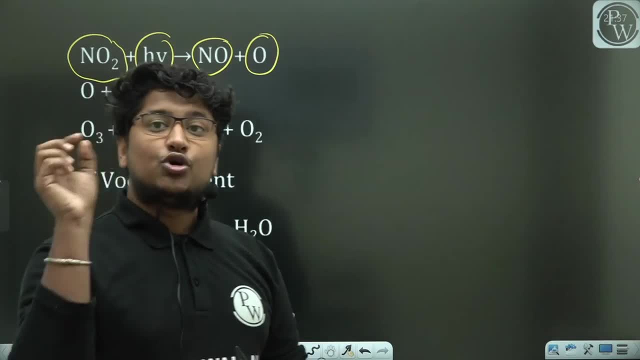 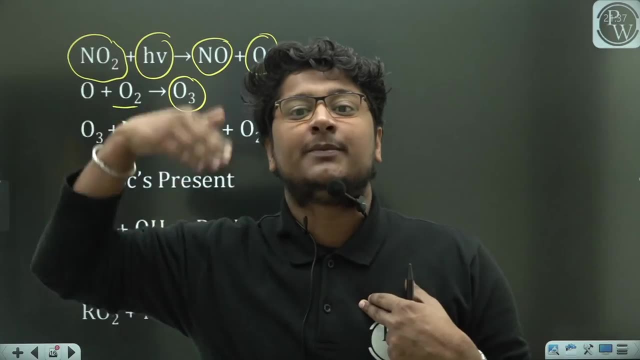 And you also have O. Both are found. O3 is made. Now what is the problem with ozone? If ozone is in stratosphere, it's good for you. We want more ozone to be made in the stratosphere. They want it. But if the same ozone is in your troposphere it's harmful for you Because it will cause you skin cancer. itching Ozone can cause you a lot of problems. So ozone is good when it is in stratosphere. 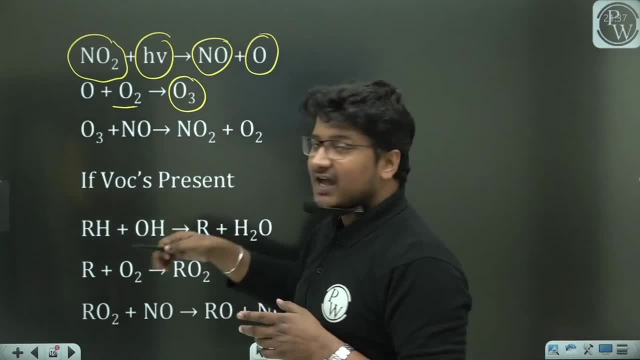 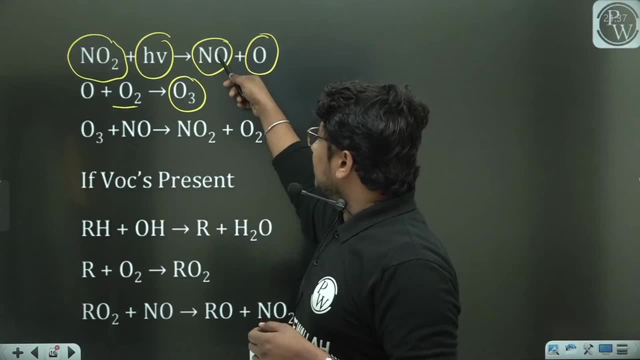 Not in troposphere. So now your O3 is made at your lower level. Now what does this O3 do? Reacts with NO. Now, if O3 reacts with NO again, what will it make? NO2 plus O2.. 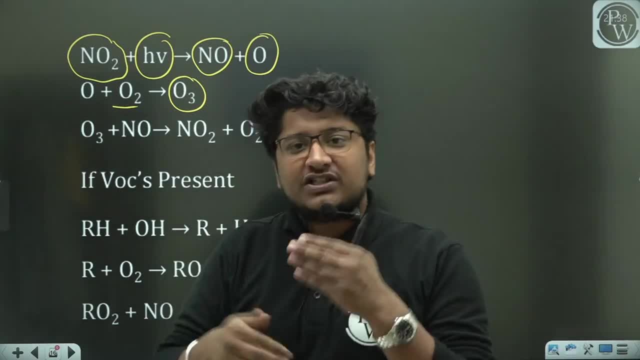 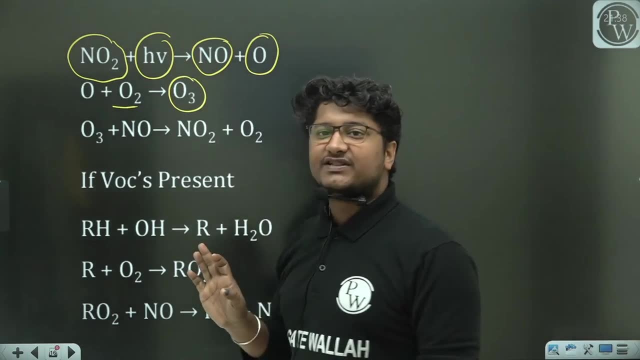 Means what has been seen in the story: Whoever made your O3, it reacted with NO again and made NO2 plus O2 very quickly. So you also got oxygen. Your NO2,, as it was NO2, was made again. 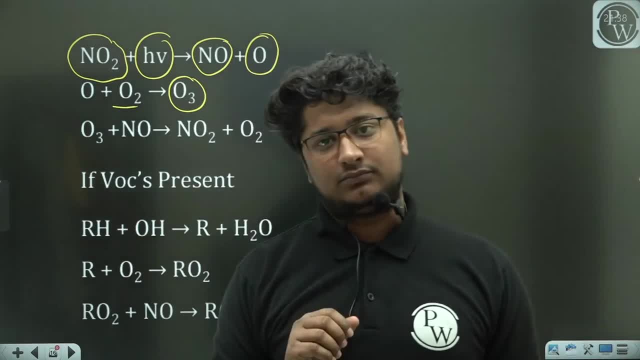 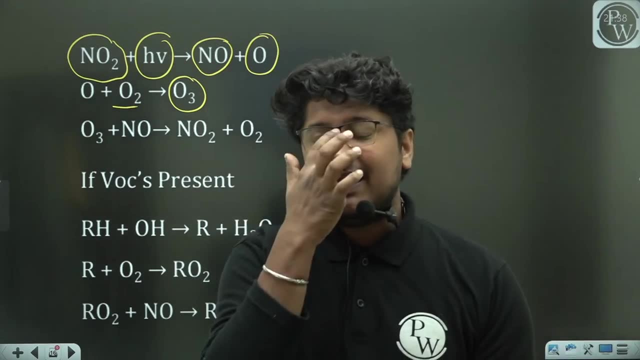 And this ozone. it also did not stop for a long time, So in the atmosphere zone. So if any poisonous thing is coming in the atmosphere but for a very short time, its residence time is very less, then it won't be a problem for us. 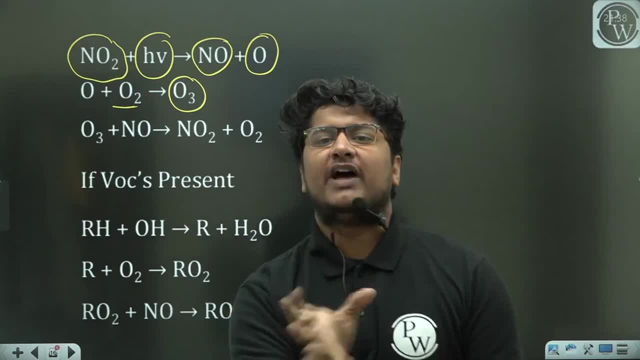 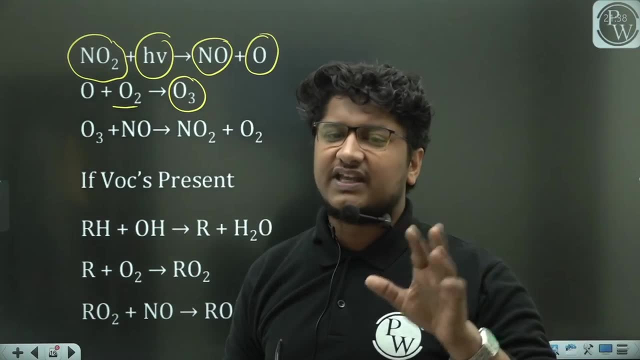 It won't be a problem for us that much. If the poison comes and it is immediately diluted, then it won't be a problem for us, The people who are living nearby where it was generated. there may be some problem But in general it will not be a problem for the large area. 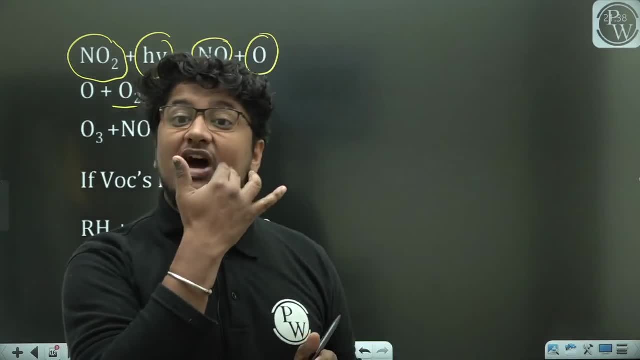 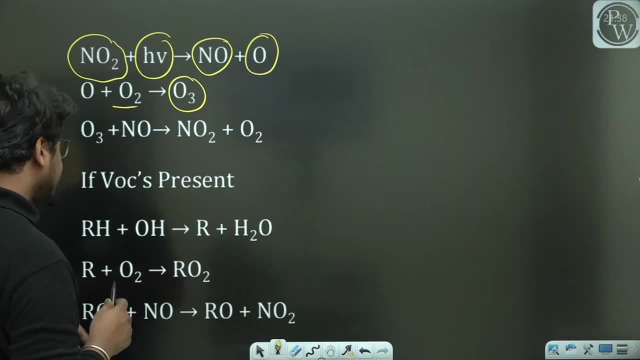 Now, what happened to the second problem? At this time, if you have some hydrocarbons in the form of volatile organic carbon, then if you have some hydrocarbons, then what are they doing? See the reaction that the O2 you got from here is reacting. 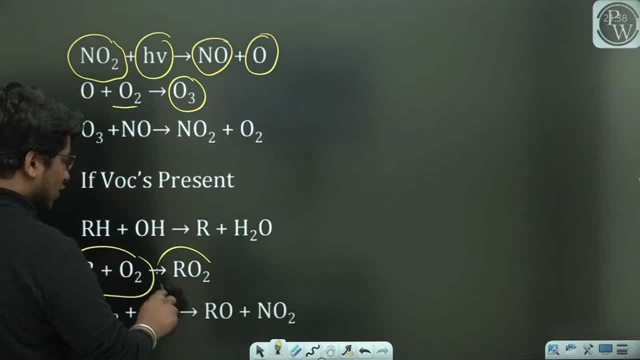 The R part is reacting with the hydrocarbon part, So you made this RO2.. Now this RO2 went from NO and went around. This NO that came out, this RO2 went around and made it RO plus NO2.. RO plus NO2.. 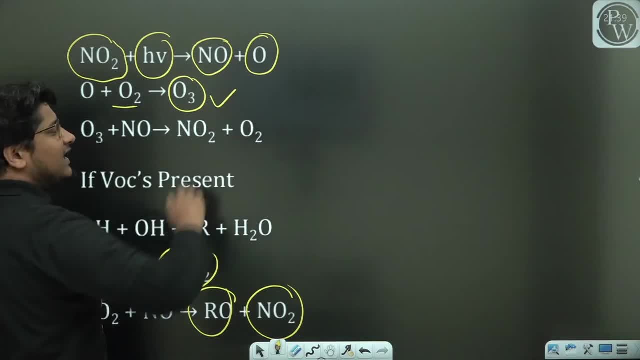 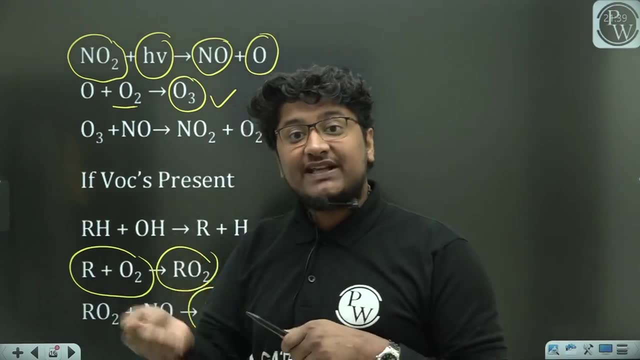 Now, what is happening in such a case? See that the ozone you got here in the troposphere. no one reacted with it. No one reacted with O3. Now, if no one is reacting with O3, then where will O3 be? 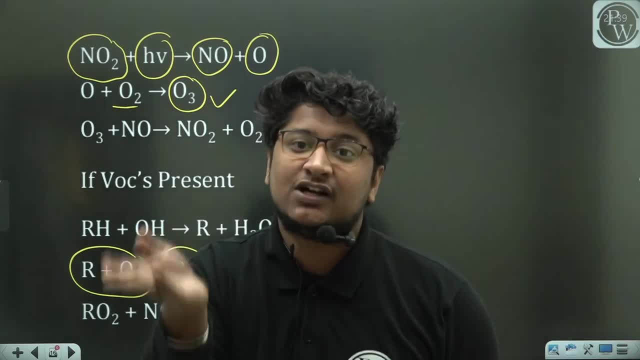 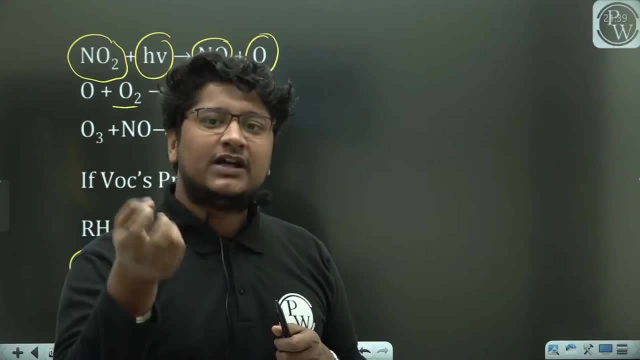 It will be in the troposphere And in the troposphere. if ozone will remain for a long time, then what will it do? It will create a problem, So that photochemical smog is your ozone plus hydrocarbon plus NO2.. 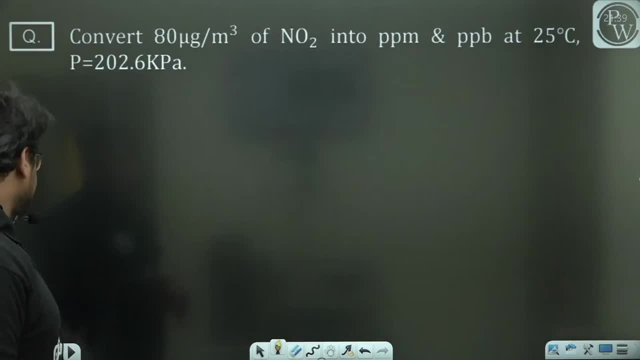 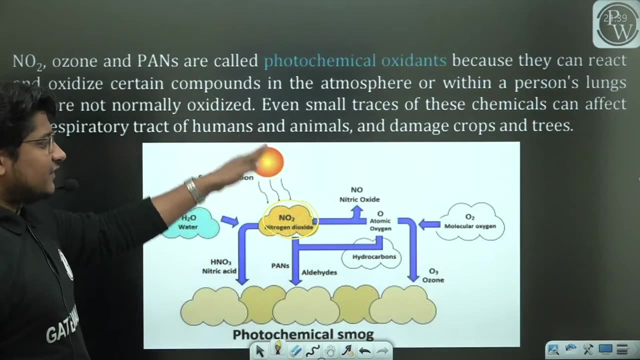 It is a combination part of all of you, So in that case, if you look at it in the figure, you will be able to see it a little better here. Look at this: This was your NO2.. OK, In the presence of sunlight. 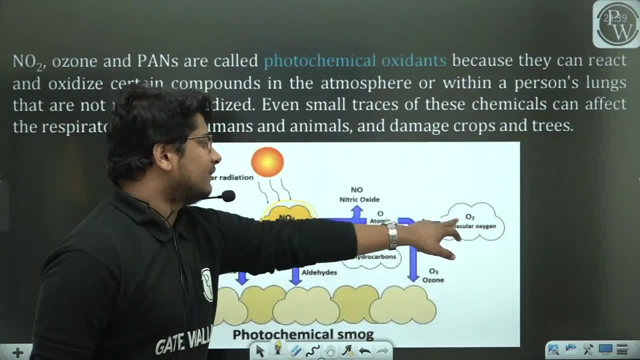 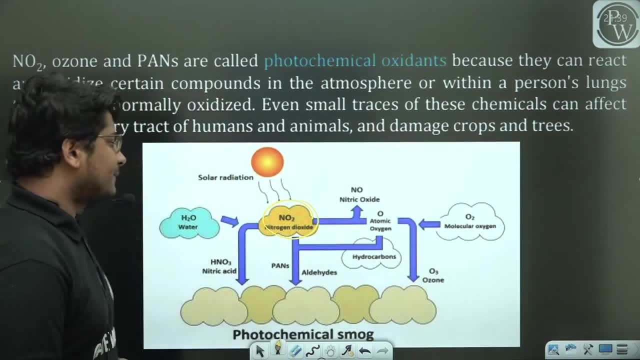 it broke in NO and broke in O. Now this O2 and this O, which is your nascent oxygen and your molecular oxygen O2, both made O3 together, so you got an O3 part. Now what happened from here? this is the nascent oxygen part. 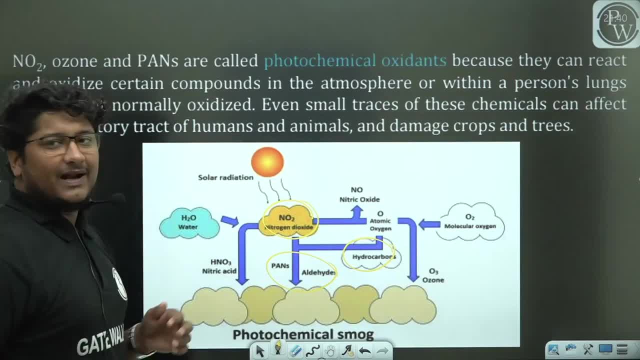 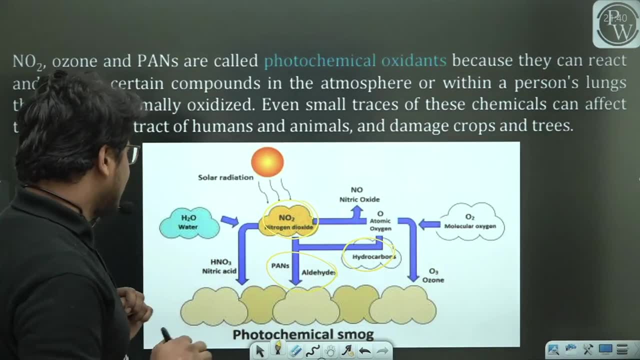 Hydrocarbon reacted with it again and you made PN or L-dehyde or PN- whatever it is- Peroxyacetyl nitrate or aldehyde. Basically, what did you make? You made a hydrocarbon part On top of that. your NO2 was reacting with H2O. 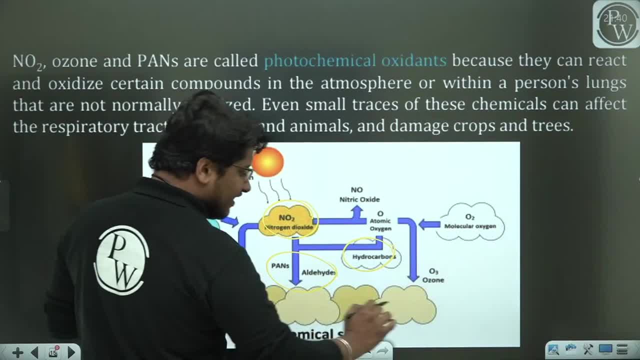 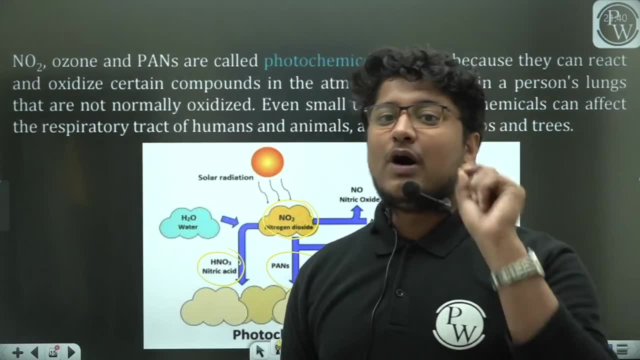 and making the HNO3 part. Now all this combination that is being made. you call it photochemical smog. So what can you see in photochemical smog? NO2 can be seen. You can see hydrocarbons. You will have ozone. 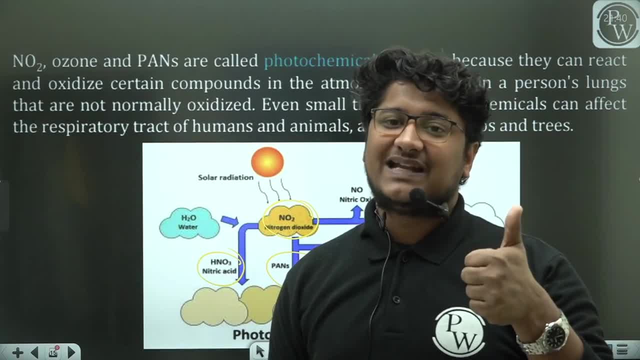 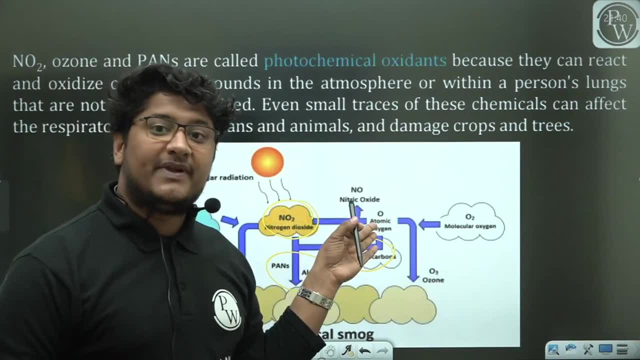 And along with that, all these things will be in the presence of sunlight, because sunlight will act as a catalyst, So this is called photochemical smog, And that is a very much problem in nowadays, because what is the main source of NO2?? 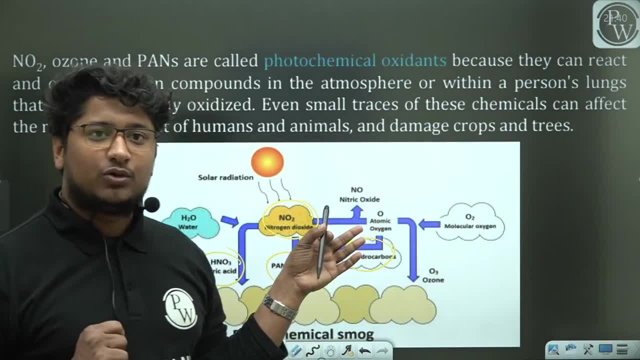 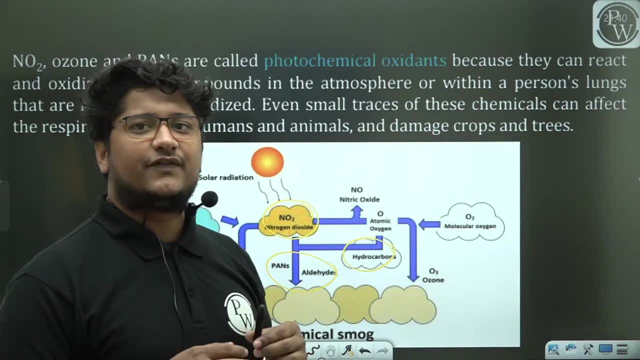 Can someone tell me What is the main source of NO2?? Can someone tell me Where do these things generally form nowadays? Where do all these things generally form? Anybody who can tell, Who has a little idea regarding the NO2 generation. 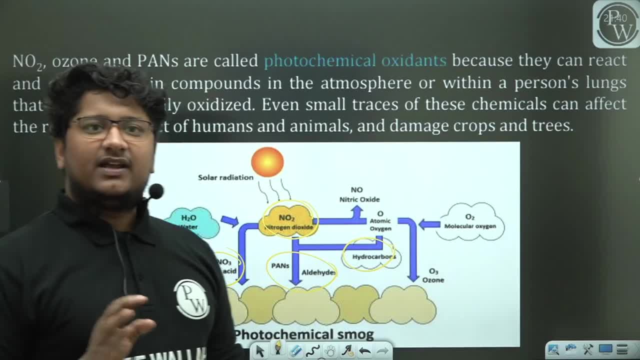 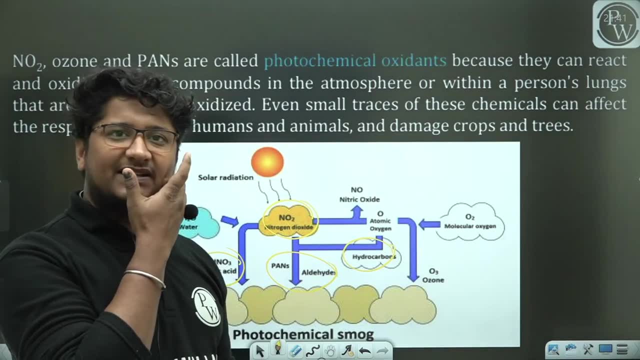 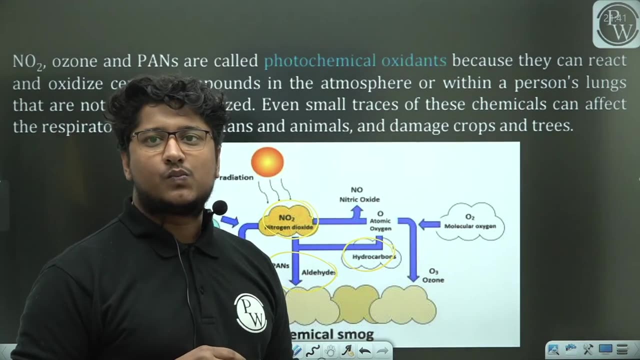 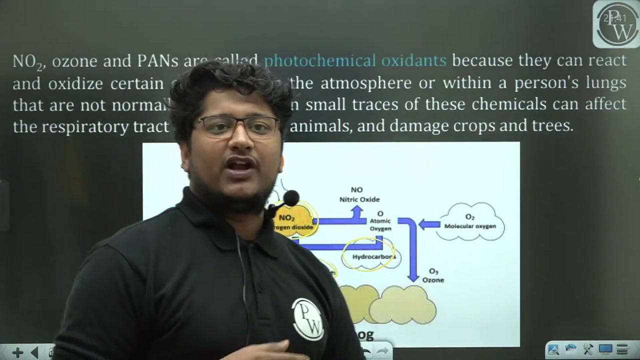 Can someone tell me? Easy, There is no hurry. I want the answer with a very clear mind. Generally, what will be the sources of NO2?? I have just talked about it, If I have been able to get a hint. So all these things are very good for you. 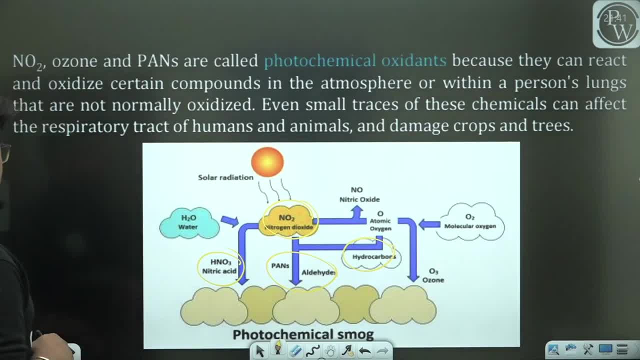 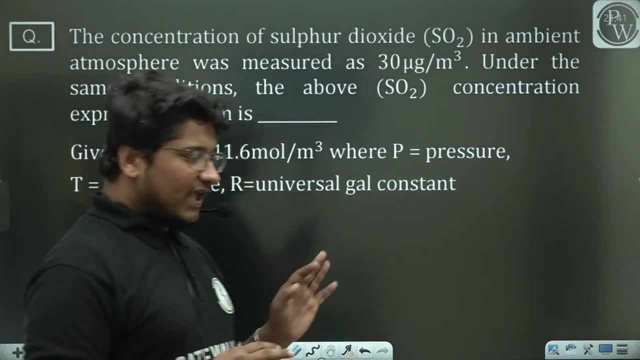 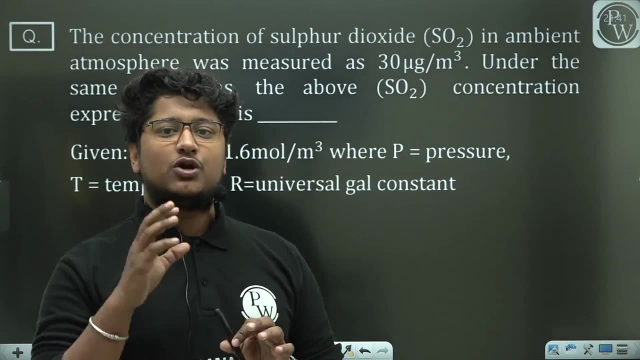 Very good, very good Automobile. The major source of NO2 that is creating problem for you is your automobile, Or you can call it as vehicular pollution. Now, this is yours, One thing which you understood, that, sir. classification of air pollution. 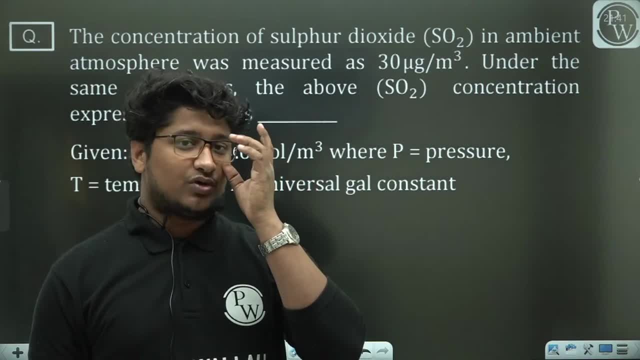 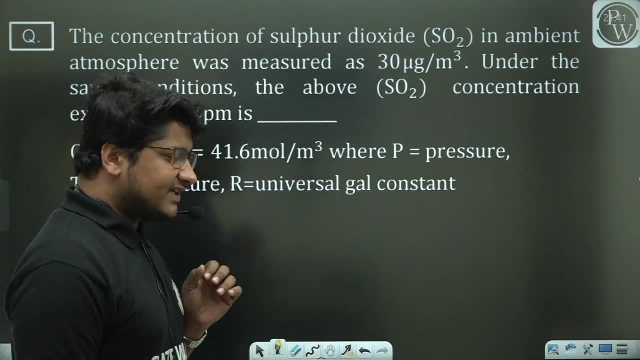 We classified the sources And second classification we did. Sir, I don't think so anybody will have any problem. Now, after this, there is a small problem which is often asked by unit conversion. Do this unit conversion with me? It is basic unit conversion. 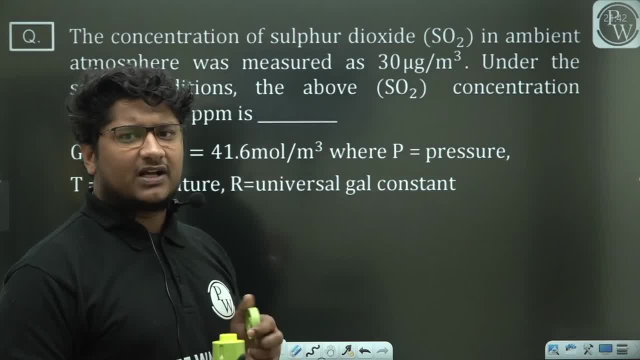 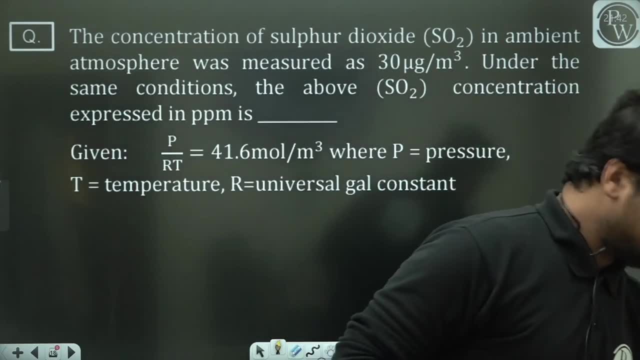 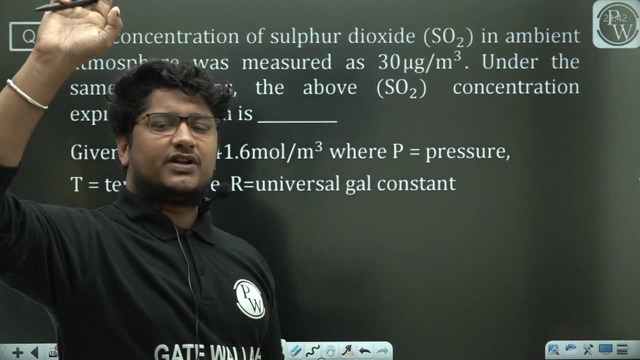 I will tell you easily And I will tell you in such a way that you will never forget again, And then I will give you the question. Then I will give you the question. Will it work? Ready, Ready. All of you are ready. quickly show the green sign. 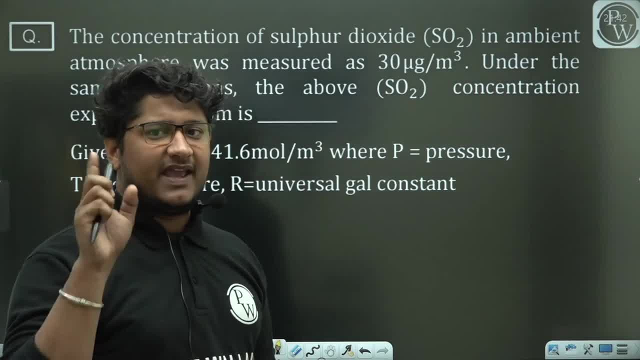 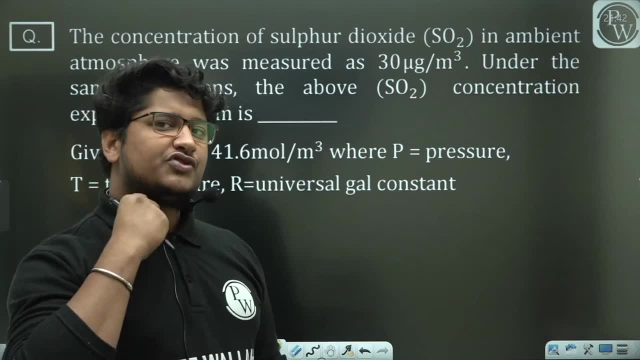 All of you are here, Everyone's mind is here. I will explain it once and then you have to make the problem. I will explain only once, Quickly: all the children, everyone's mind, everyone's mind, in the comment section, Because this conversion- you are often confused. 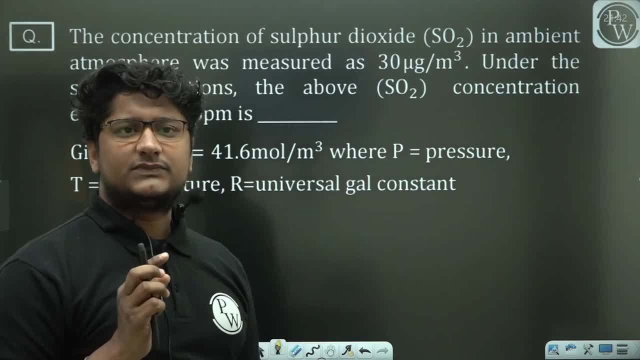 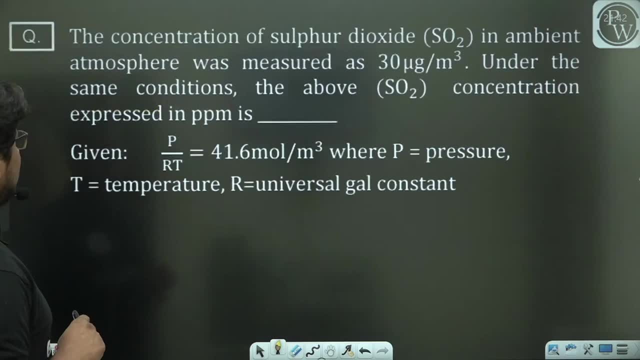 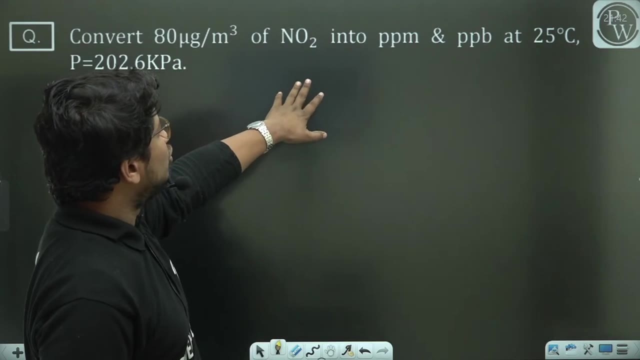 You trouble me outside. Okay, I am telling you easily. There is no problem with me. Let us take a question, Dear sir. Yes, Take a question. What is the question? 80 micrograms per meter cube of NO2 into ppm. 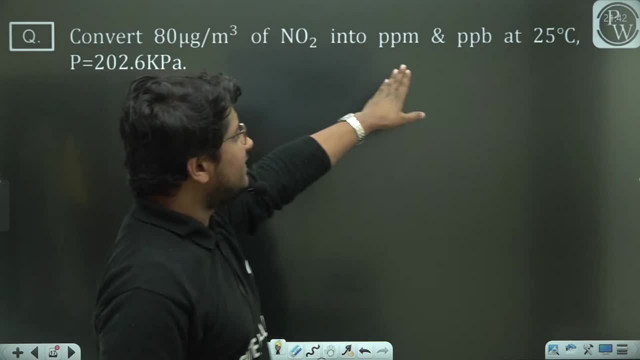 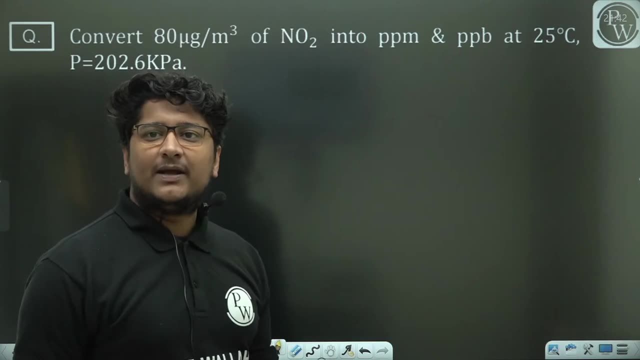 They want to convert micrograms per meter cube into ppm Or ppb. At 25 degrees Celsius And pressure, they have 202.6 kilopascal. This is Punya Pratap ji. What happened? Why are you showing your teeth? 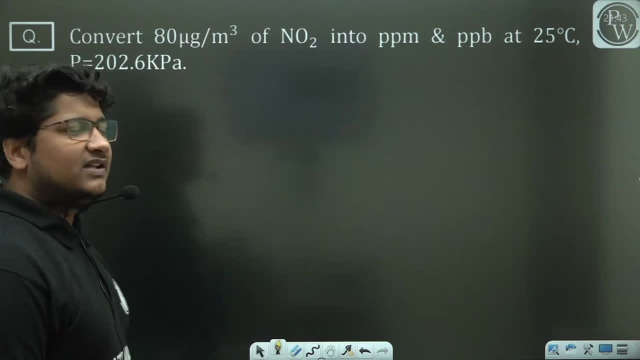 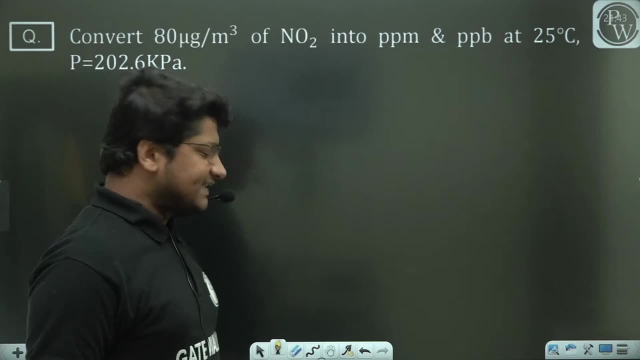 Okay, You have come after brushing. What does it mean? Will you show your teeth? Come on. 202.6 kilopascal. This is yours Now. see how it is made in a basic way. Let's take a little extra slide. 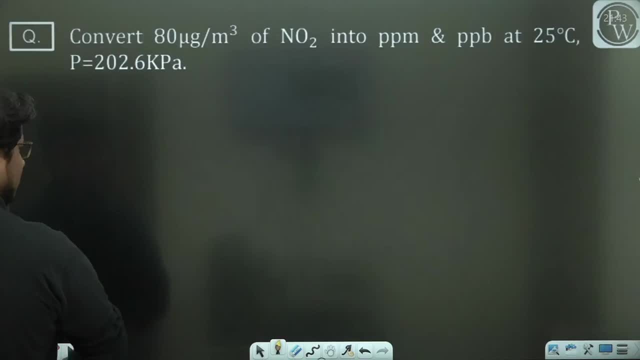 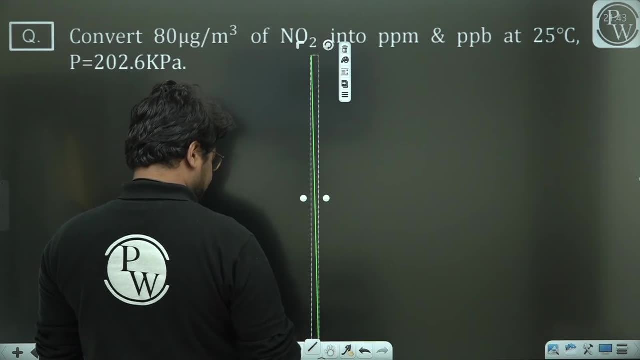 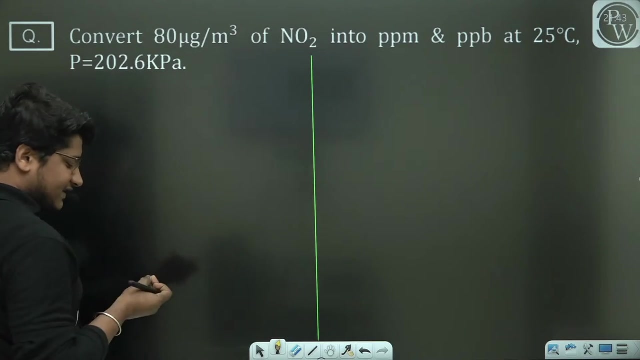 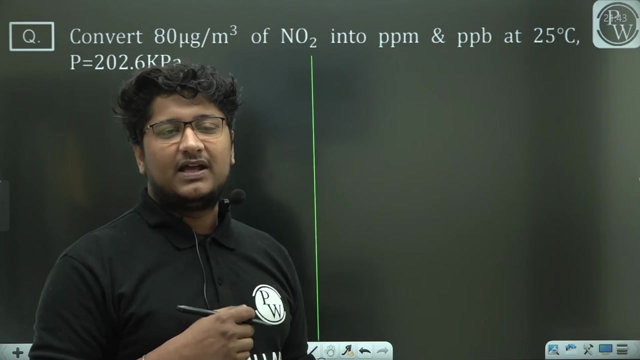 Let's take a little extra slide, Because first of all, you will have to understand Some children who do not know. Those who know, it is a good thing. Sir, what is ppm? You are going to do conversion, But what is the meaning of ppm? 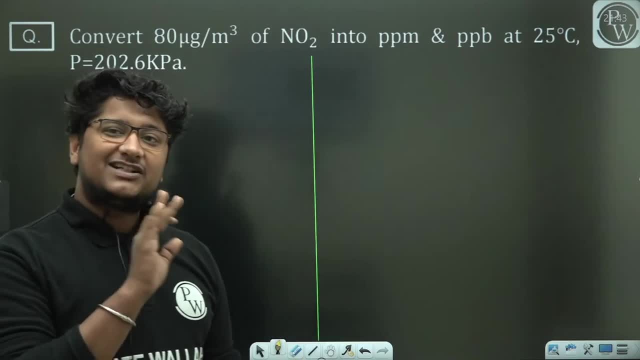 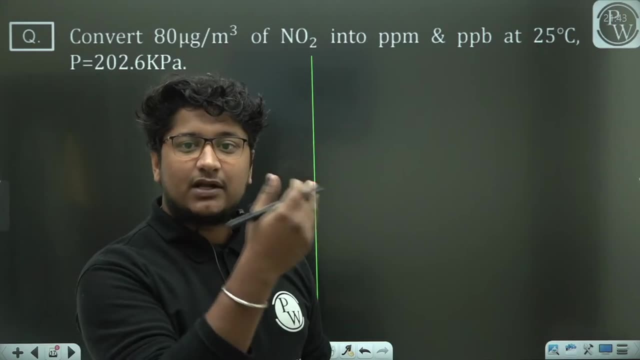 So ppm means parts per million. Now what is the meaning of parts per million, Sir? how is it different from concentration? So what unit of concentration did you take? Micrograms per meter cube. So basically, in a numerator you have mass And in a denominator you have volume. 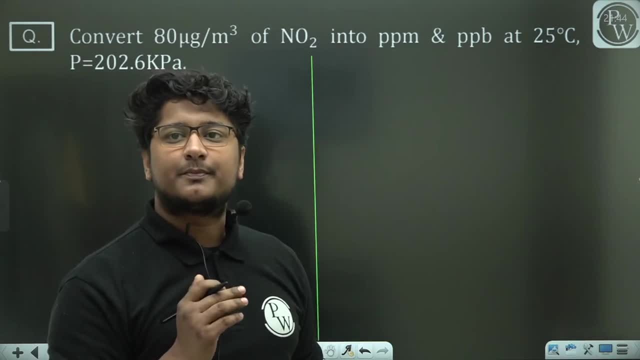 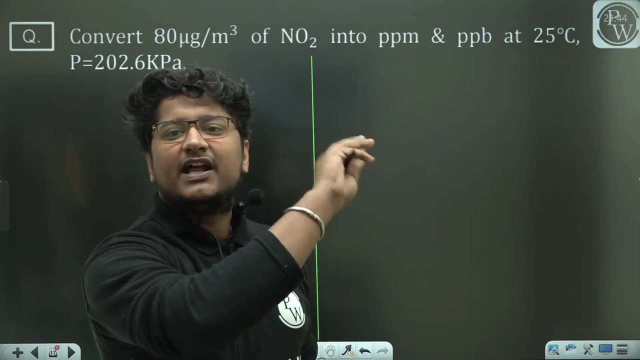 So it is mass by volume. It is mass by volume. Are you understanding? When you talk about ppm, It is part, like, In essence, number, of part of solute Divided by 10 to power 6: part of solvent, your solution. 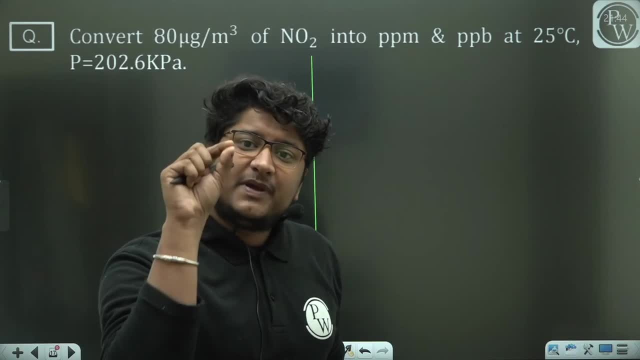 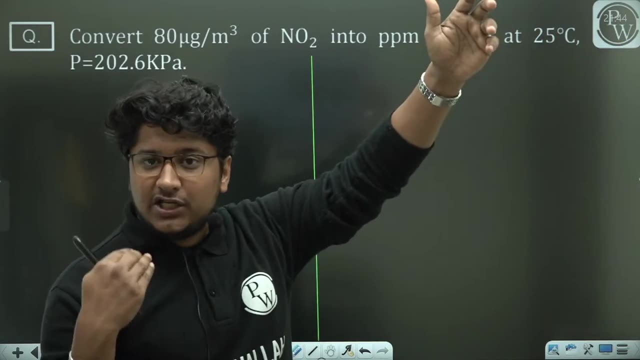 So in that sense you will have to understand When you talk about ppm, So part per million. In essence, what is the numerator for you? Same unit, Denominator: also same unit for you. So here there is no discussion of unit Either. it will be volume by volume. 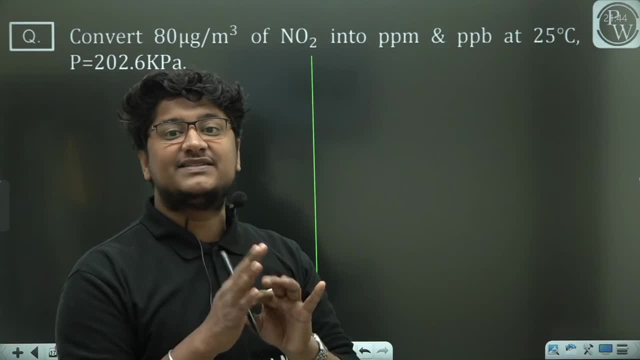 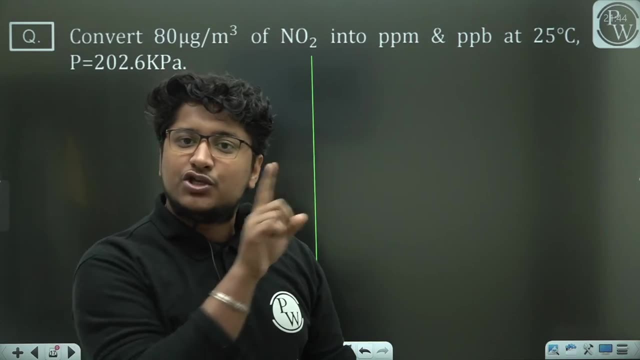 Or it will be mass by mass, But there will be no chance On which you are talking, Where you are talking. You are talking That it will be mass above And volume below. There is no such discussion, There is no discussion of unit with you. 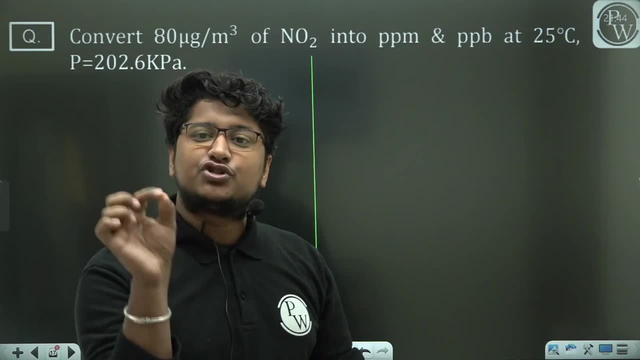 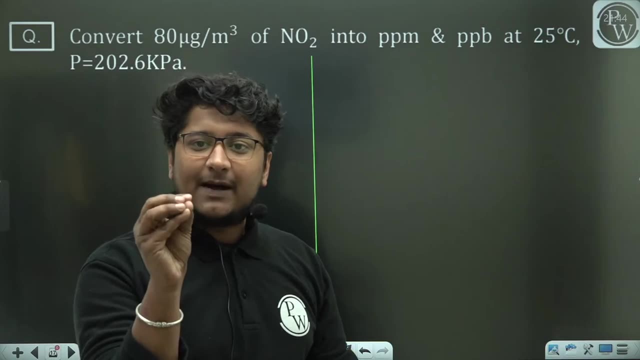 So, in essence, if you have to understand That if I have to convert anything into ppm, So this unit game will have to be removed, You will have to understand this with guarantee. So what is your part? per million means How many moles of solute you have. 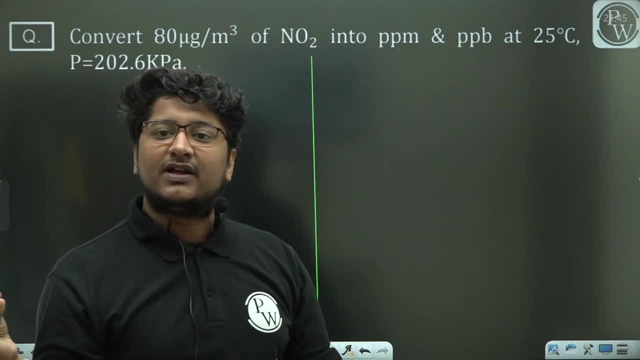 Or how many meter cube of your solute In how many solutions, And how much solution should be 10 to power 6.. Is that clear? So I am going to do the same thing, I am going to replicate the same thing. 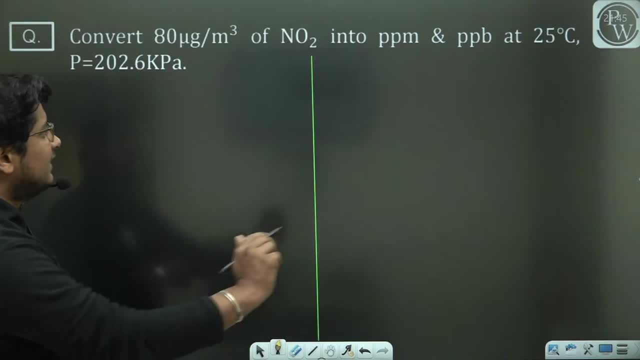 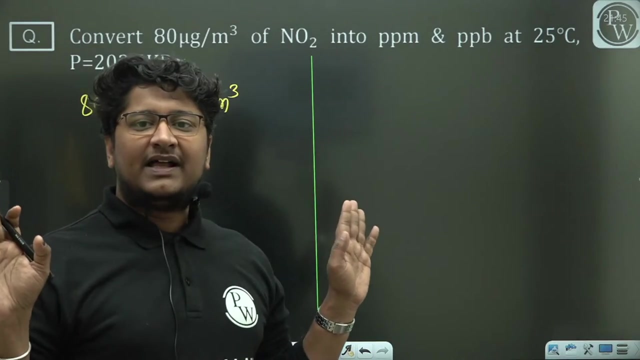 Which you can understand easily. Now see here. Those who have understood a little ppm, See here. What is the question, brother? Question is saying: Sir, 80 microgram is present in 1 meter cube of solvent, Yes or no? 80 microgram of NO2 is present in 1 meter cube. 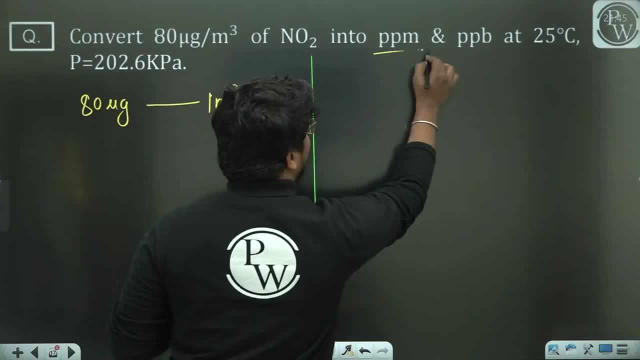 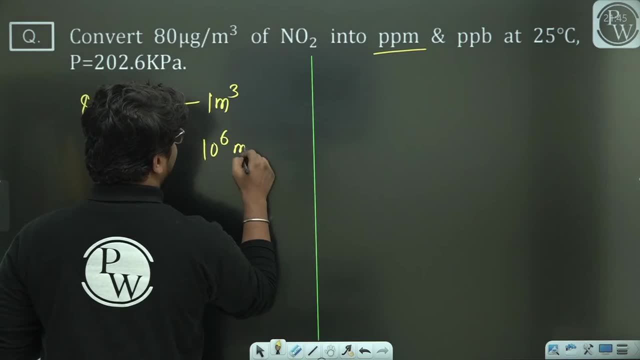 This is what it is saying. Parts per million means, Brother, How much is present in 10 to power 6 part? So if I talk in 10 to power 6 meter cube, If I talk in 10 to power, 6 meter cube. 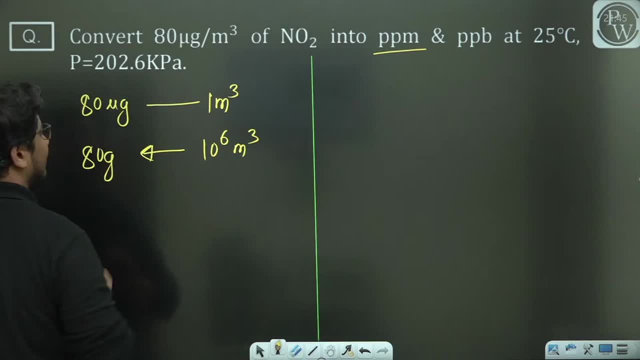 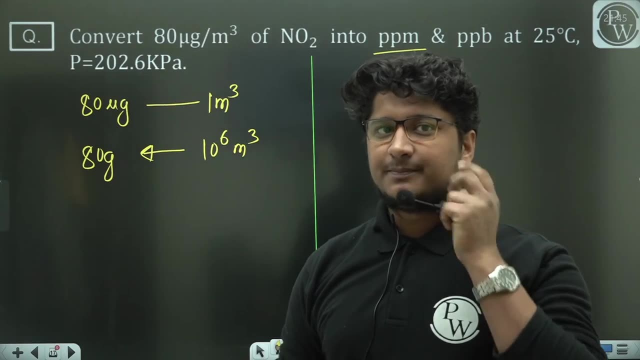 So how much will be present, sir? Will it be 80 grams, Yes or no? Will it be 80 grams, Yes or no? So, Mr Mesh, answer quickly If 80 microgram is present in 1 meter cube. 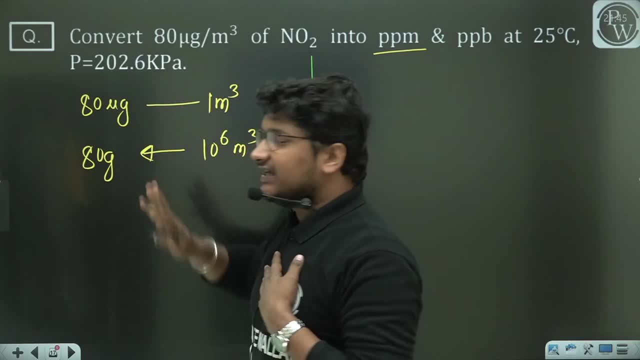 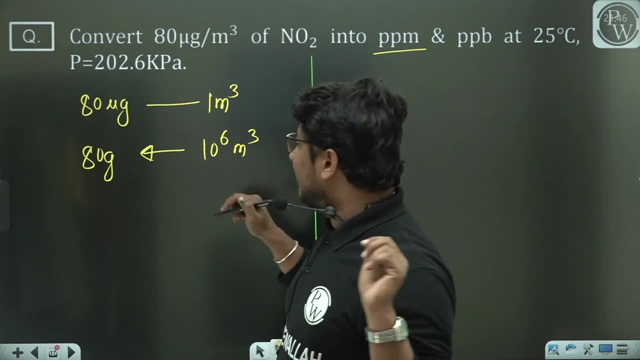 So if I talk about 10 to power, 6 meter cube, So 80 grams will be present. There is no doubt in this. Now see, If I want to get ppm value. So what will I have to do, Sir, this gram in any way? 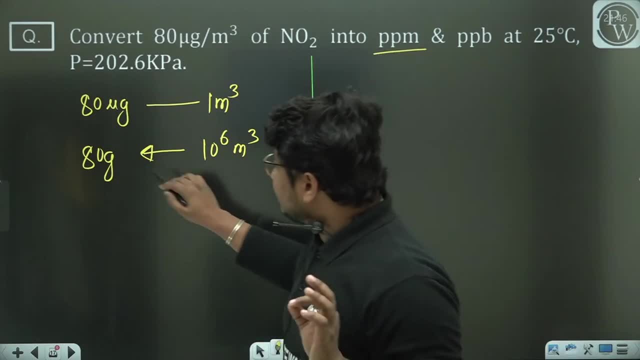 If you convert it in meter cube, If you convert this gram in any way in meter cube, So it will happen That this much meter cube is present in 10 to power 6 meter cube. So whatever meter cube you will get, Whatever meter cube you will get, 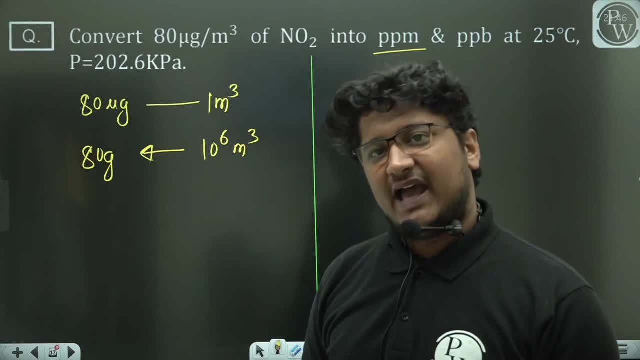 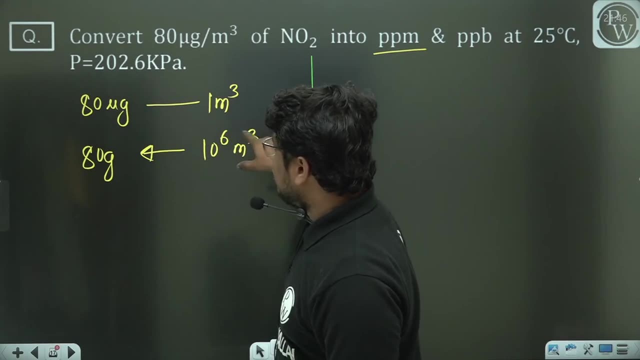 That will be nothing but the ppm. Is this thing understandable? Is this logic understandable? I am asking this to all of you. That means Whatever For 10 to power, 6 meter cube, Whatever meter cube, you are getting In place of 80 grams of NO2.. 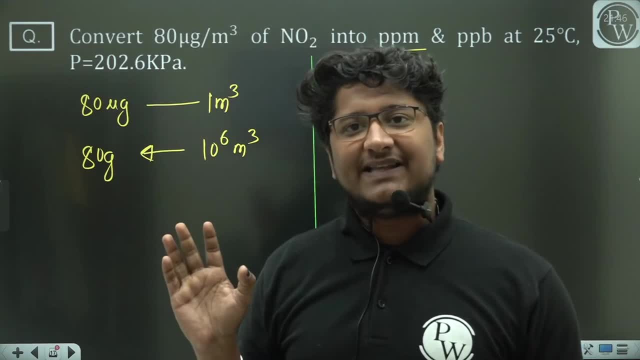 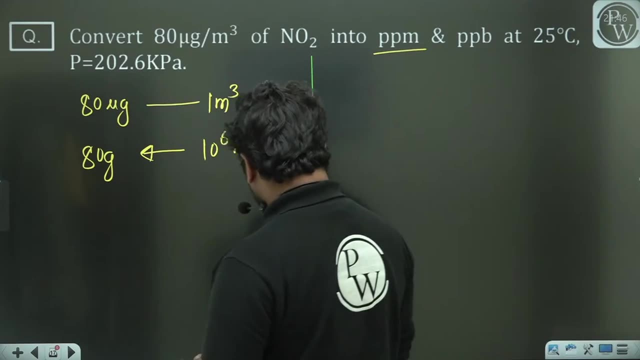 That will be nothing but the ppm value. That will be nothing but the ppm value. Is that clear to all of you? Did you understand the thing easily? Now see here. So what is our problem? Our problem is that We have to convert this 80 grams in meter cube. 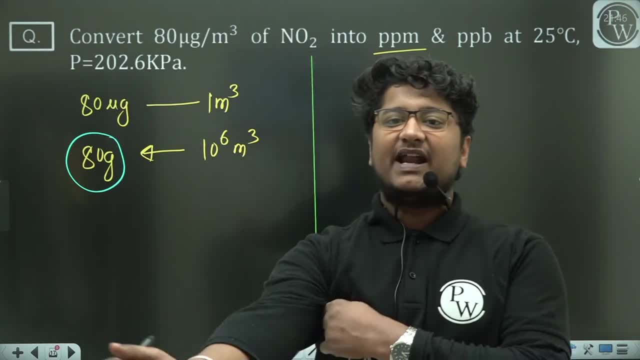 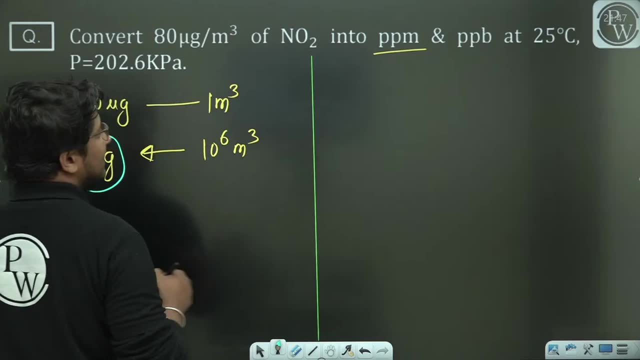 I want to convert this 80 grams into meter cube, So here we will not do direct If we want to convert mass into volume For gases. So we have a formula that we call as PV equal to nRT. You have read a formula. 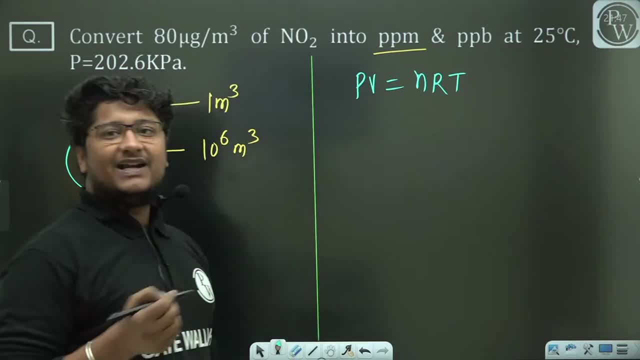 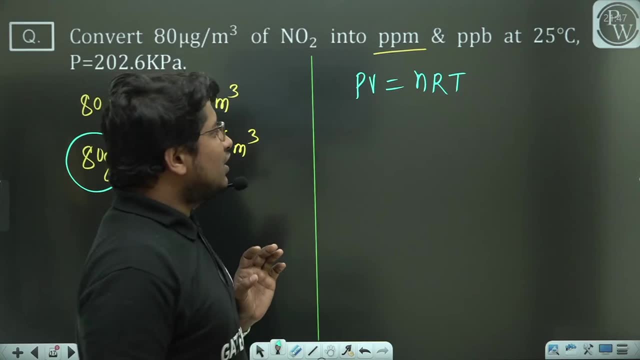 PV equal to nRT. Now, R is what It is, a universal gas constant. P is the pressure, V is the volume, N is the number of mole And T is the temperature. So first thing first Is that you need to find out R. 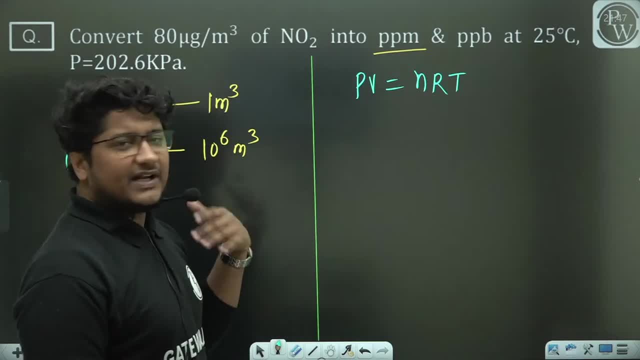 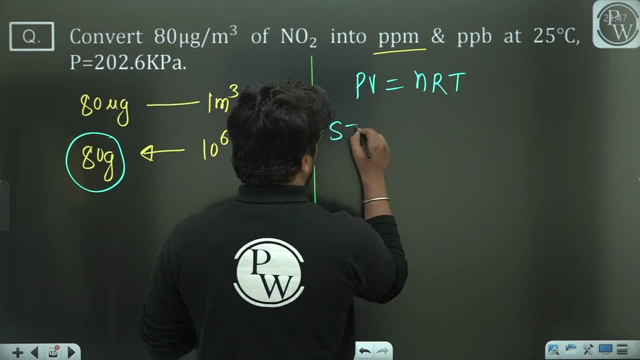 That is universal, That is universal gas, constant value Which can be rotated, Which you can rotate, And even if it is not rotated, Then also it will work. So what is the condition you have? So you have, Let us say, we are using STP condition. 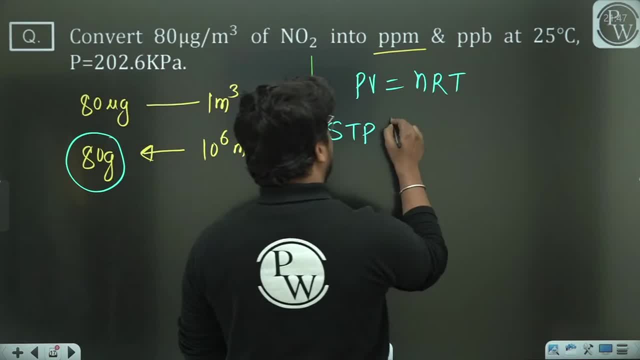 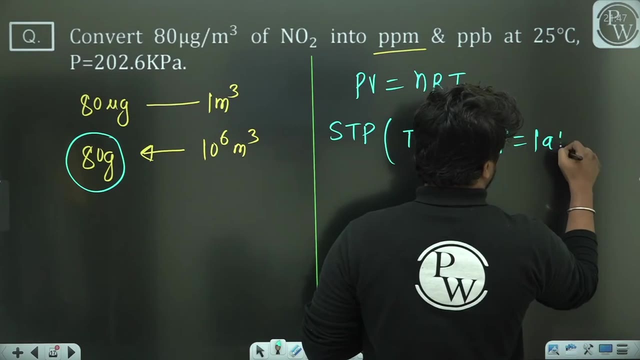 Standard temperature and pressure condition. So the condition you will have is You have T is 0 degree Celsius And what will remain? 0 degree Celsius And pressure will remain 1 atm. Pressure will remain 1 atm, For your kind information. 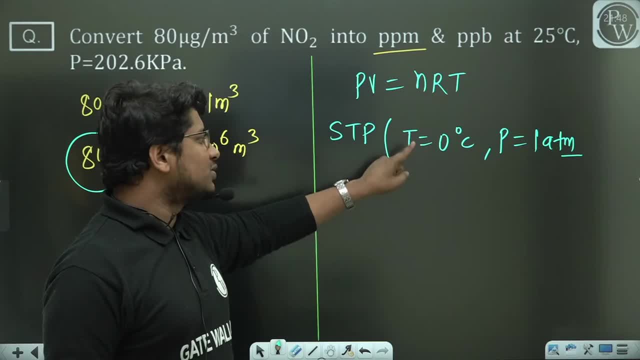 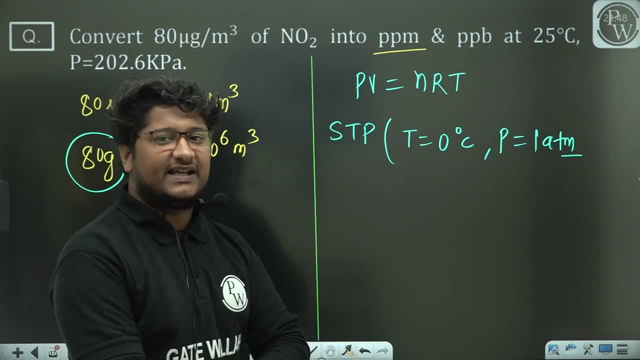 This is the condition of the old STP. Now the new STP condition is 0 degree Celsius And P is 1 bar, So the new one is 1 bar, But we are still taking out the value of R from the old one. 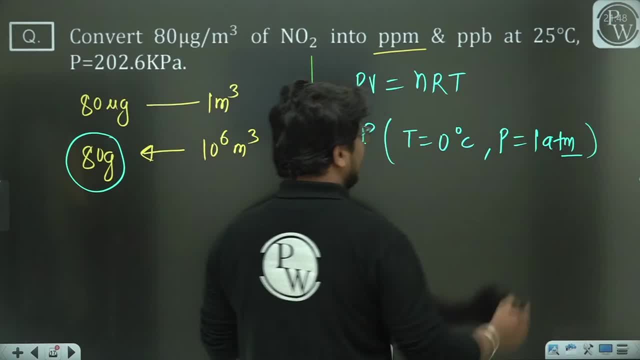 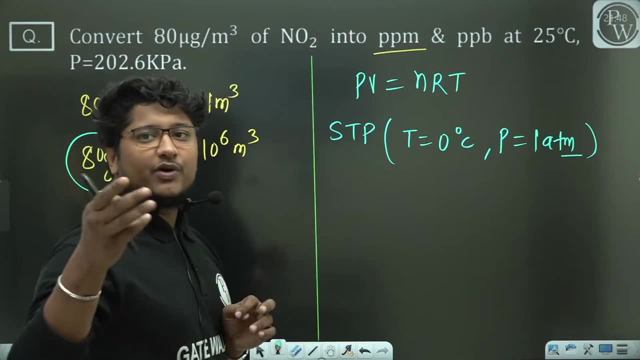 So you guys stay clear in this thing: T is equal to 0 degree Celsius And P is equal to 1 atm. Till then, tell me Who tells you the STP and NTP condition. Tell me by commenting quickly, What is the STP condition? 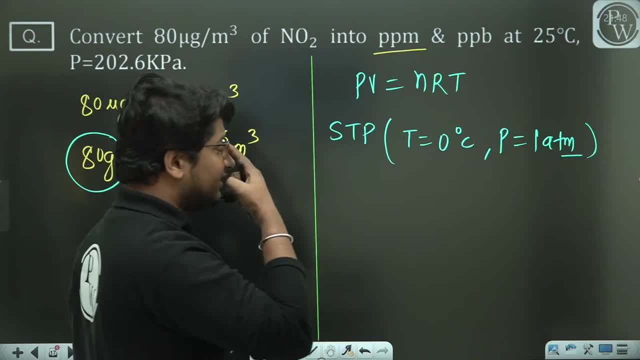 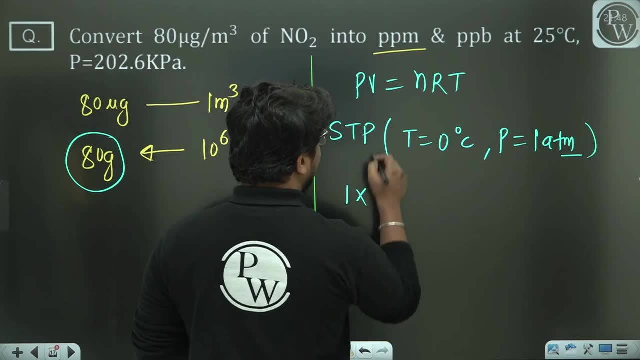 What is the NTP condition? Who decides it? Which organization tells it? Let's go Next For STP condition. If you see, PV is equal to NRT, So you keep PV as 1. 1 atm V is. 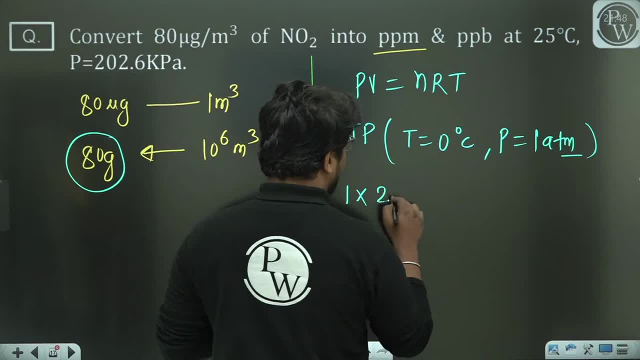 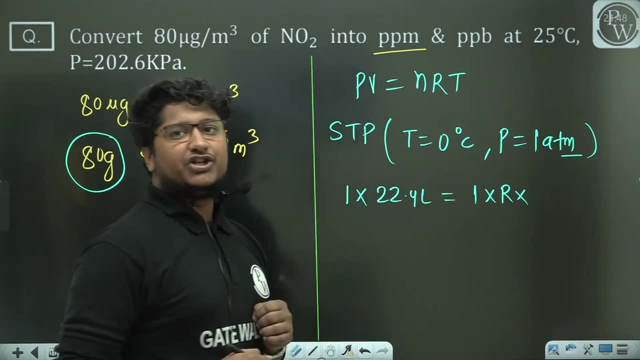 If you are talking about 1 mole, Then V will be 22.4 L, The number of moles is 1.. R is And temperature. Temperature is 0 degree Celsius, But we will always represent it in Kelvin, So how much will it be? 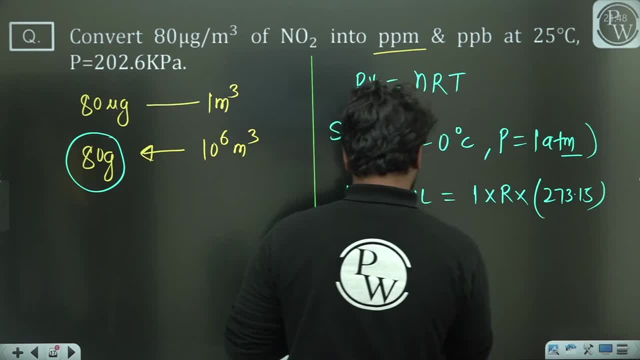 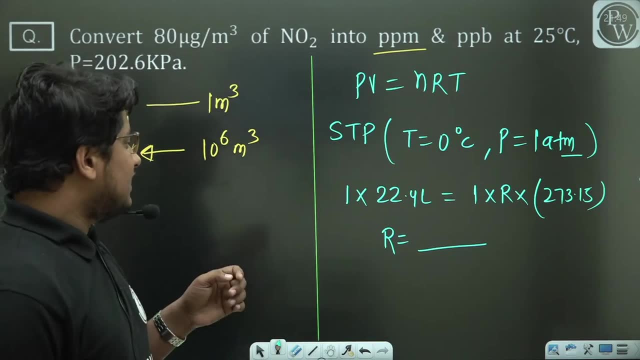 273.15 Kelvin. So if you calculate R value, What is R? Please answer me, If you, all guys, will. Yes, IOPSC, Absolutely correct. Indian Union of Pure and Applied Chemistry. What is the value of R? 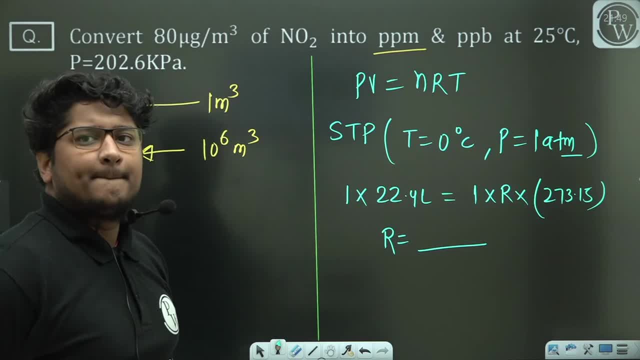 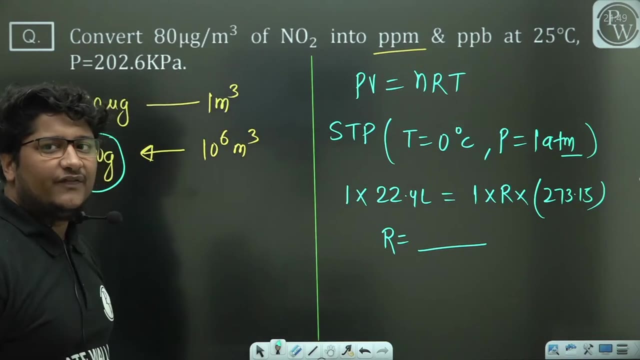 Tell me What is the value of R. All of you, What is the value of R. Tell me, by commenting, What is the value of R. What is the value of R you guys are getting. What is the value of R you guys are getting. 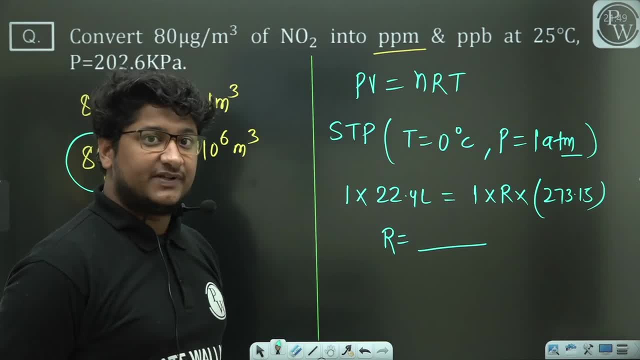 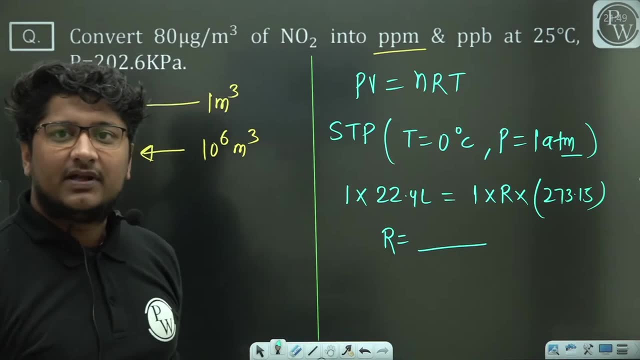 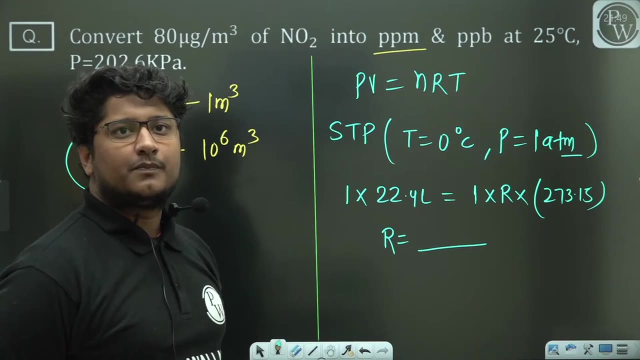 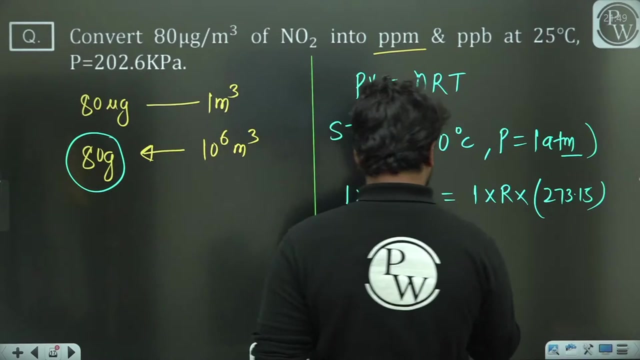 Do it together, Because I am doing this problem with you, I will do the next problem with you. I will give the solution in the next problem. Never expect this. What is the value of R 0.082.. As you all guys are telling, 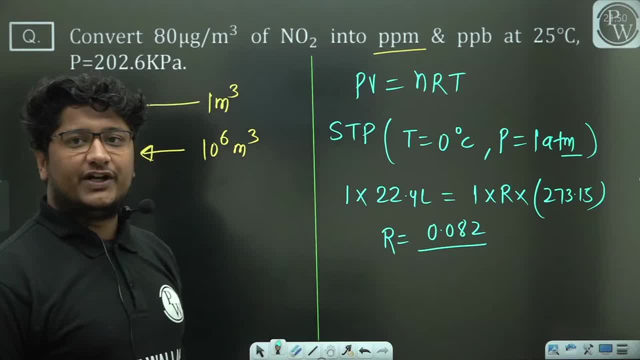 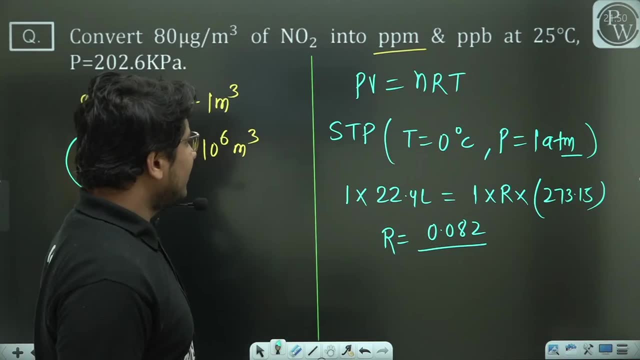 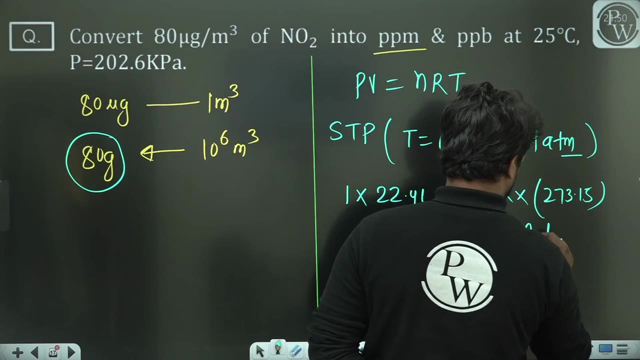 As you all guys are telling, 0.082.. 0.082 is around 1.. It is around 0.082.. Take care of the unit. Unit is very important. So what will be the unit? Atm Liter. 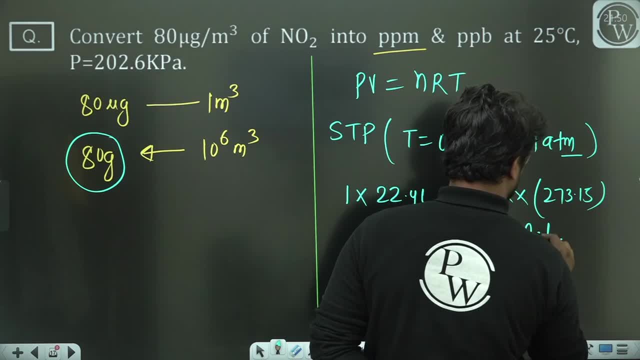 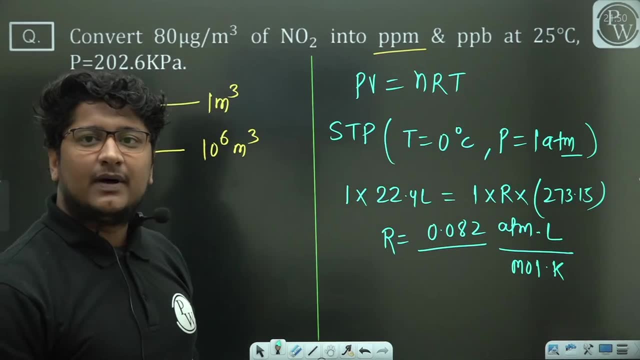 Divided by Pole per Kelvin. This is your unit. So once you got R, Sir, how to do P in Atm? Yes, So how to do Pascal in Atm? This is what you are asking. That means you have not studied fluid mechanics. 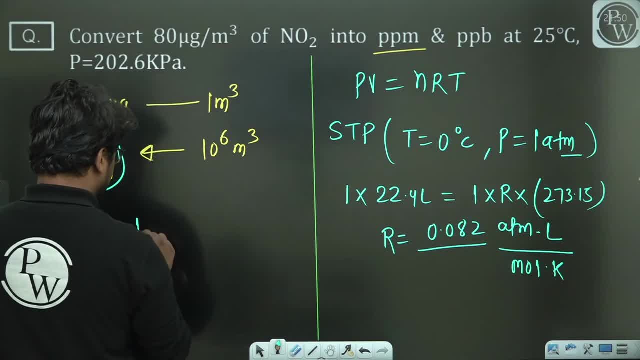 If you have to tell me these things, Then this is wrong. What is 1 Atm equal to? Tell me quickly in the comment section. What is 1 bar equal to Tell me quickly. And what is 1 Pascal equal to? 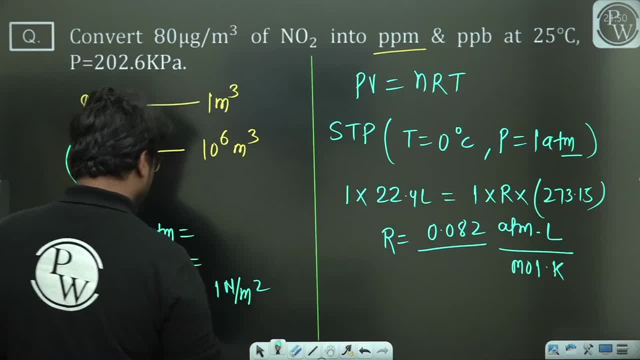 So 1 Pascal is called Newton per meter square. 1 bar equal to 10 to power 5 Newton per meter square. What is 1 bar equal to? It is called Newton per meter square And 1 Atm is 1.01325 bar. 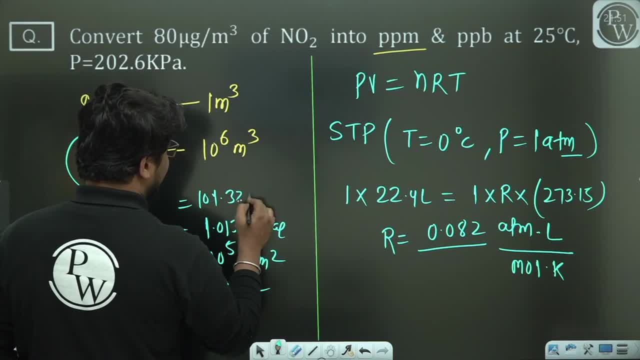 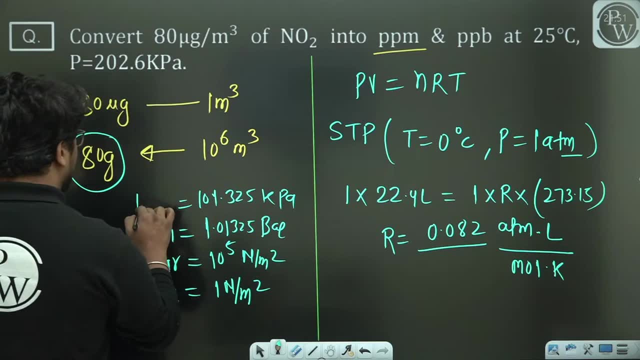 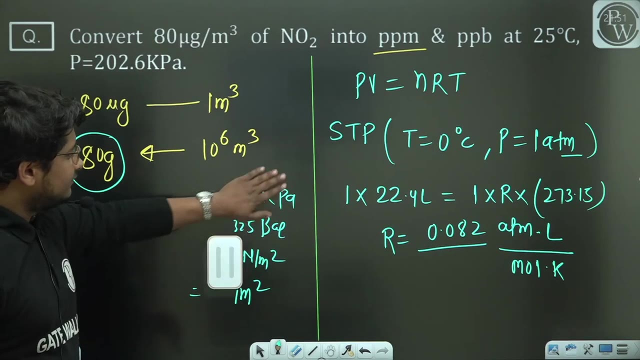 Many people write it as 101.325 kilopascal. Ok, You write this 1 Atm like this. Now, I have already discussed these things with you, So here I will not write again. Ok, Now pay attention here. Now pay attention here. 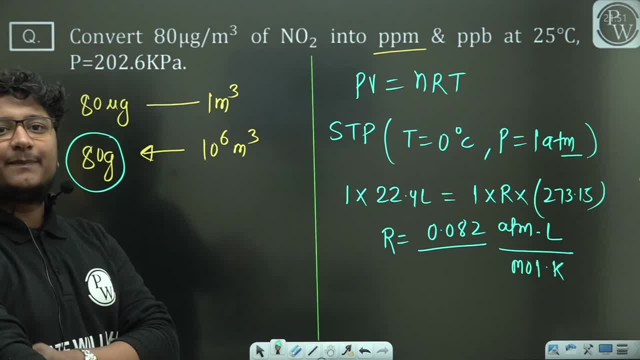 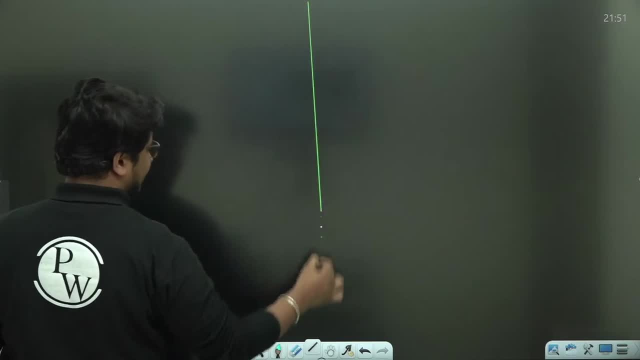 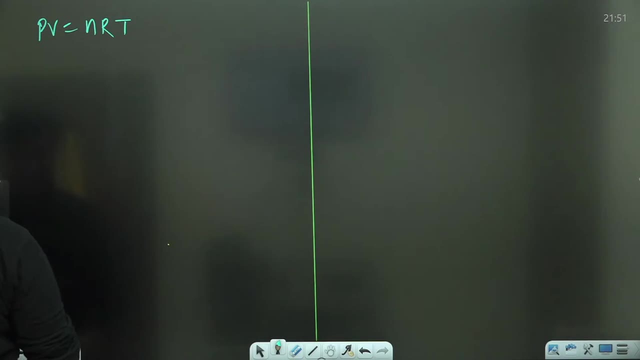 So you have got R value. Now we can easily write our PV equal to NRT formula. Let's go. So now let's write our formula PV equal to NRT. So we have PV equal to NRT. What is there in our condition? 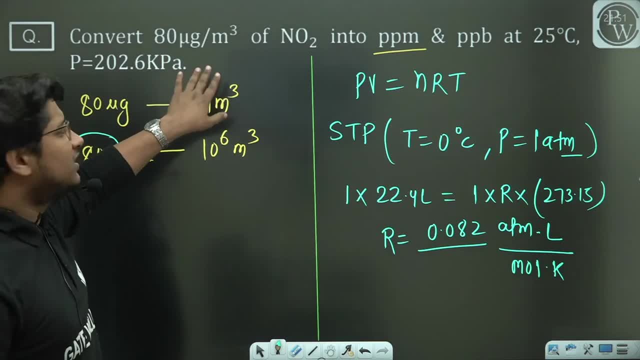 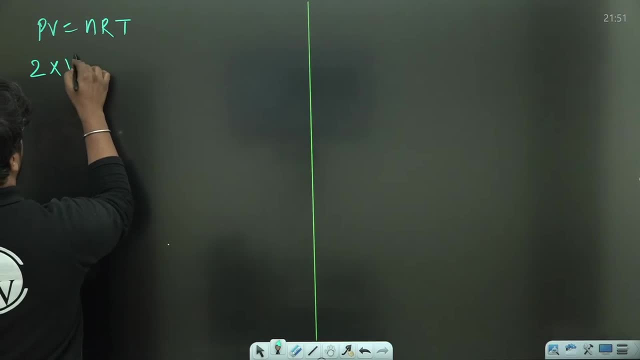 Sir, in our given condition P is 202.. That means, can I take it roughly 2 Atm? Yes, sir, We can take 2 Atm Into volume. Sir, we have to take out the volume. Sir, we don't know the number of moles. 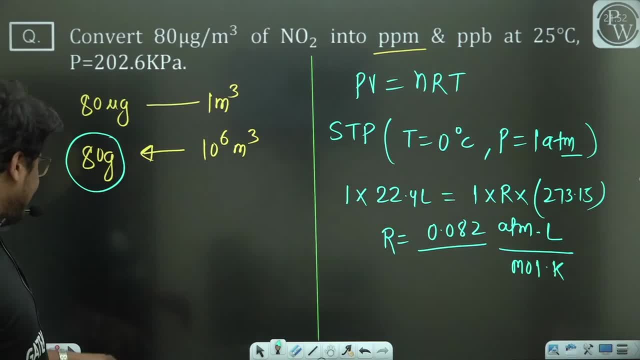 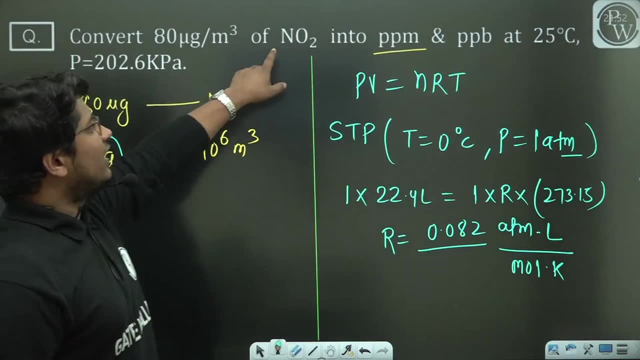 We will have to take it out. So for how many grams are you talking? Given mass is 80 grams. So 80 grams divided by its molecular mass, Number of moles. So what is the molecular mass of NO2?? Tell me by commenting. 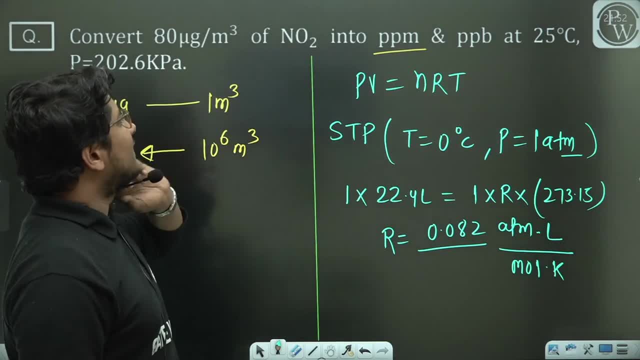 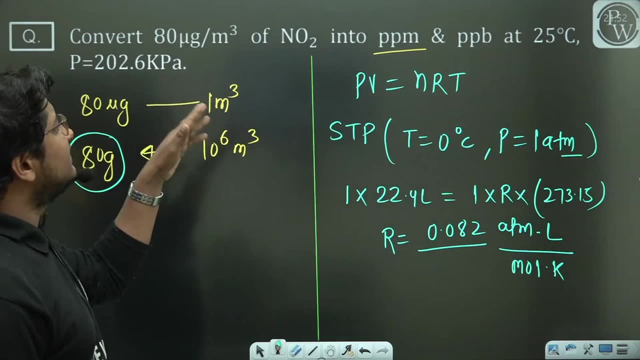 How much will it be approximately, Approximately? your nitrogen will be around 14. And your oxygen will be 16 and 32.. So approximately 32 and 14.. It will be a little more than 46 or around 46. See the exact. 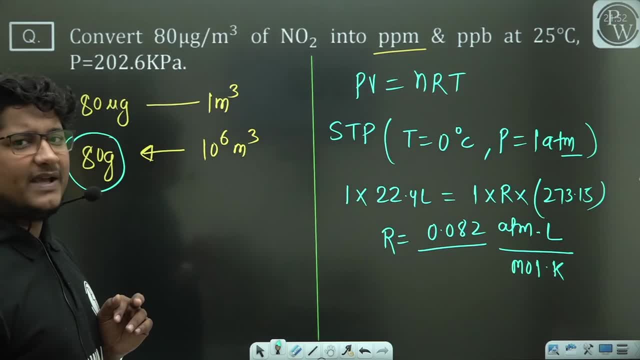 I am taking 46.. You see exactly. So your NO2 is 46.. Okay, let's go Now. did you get the number of moles? You have given the value of R as 0,, 8,, 2, 1.. 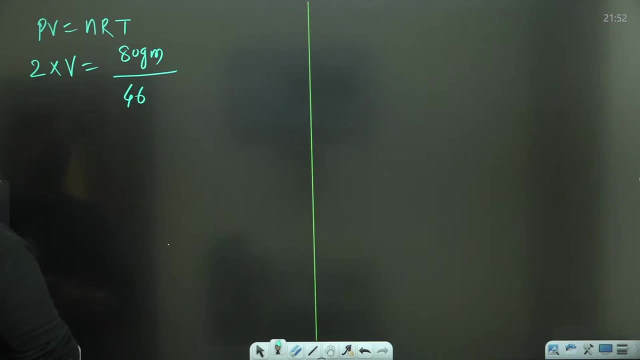 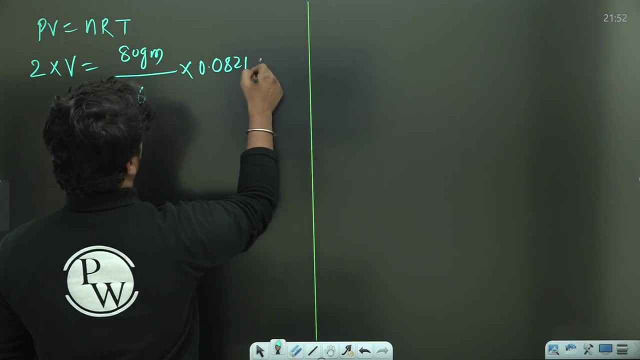 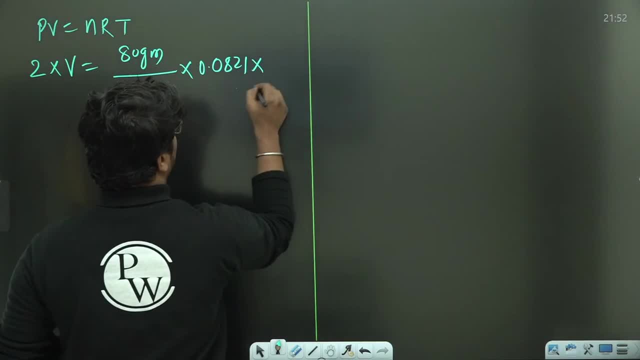 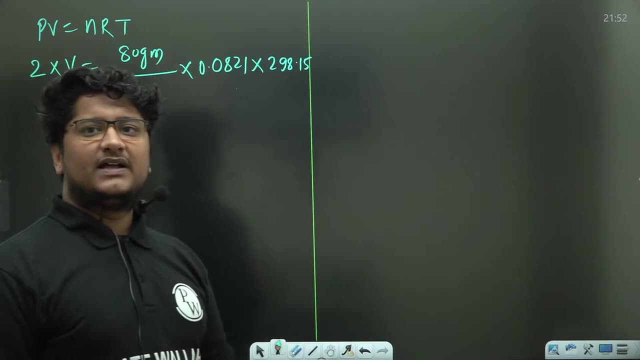 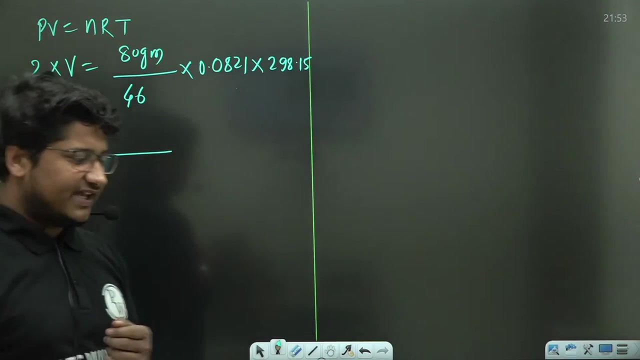 Then it will be 298.15.. Where is 20?? It is 298.15.. Okay, There is no problem. Let's go Now. how much is the value of its volume from here? Tell me What is the value of volume. 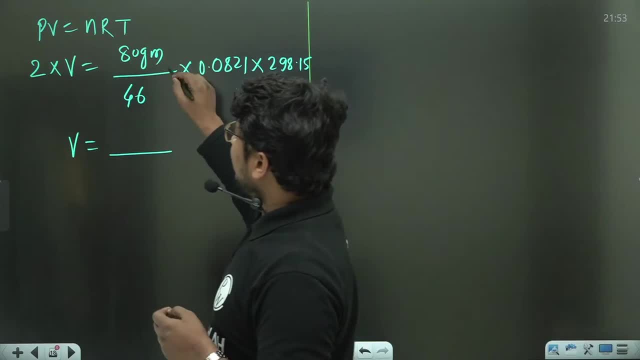 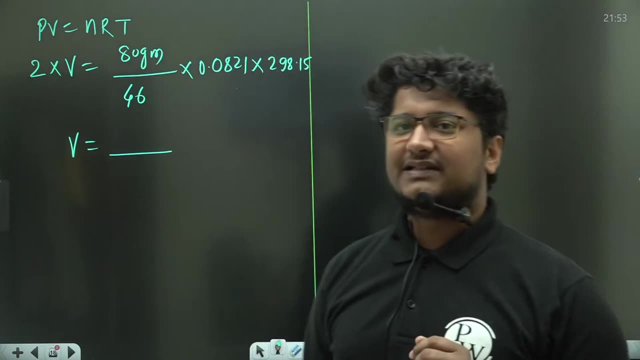 Tell me to all of you This formula: basically what we are doing: we are converting this 80 gram into volume. We are converting this 80 gram into volume. That's what we are doing. That's what we are doing. That's what we are doing. 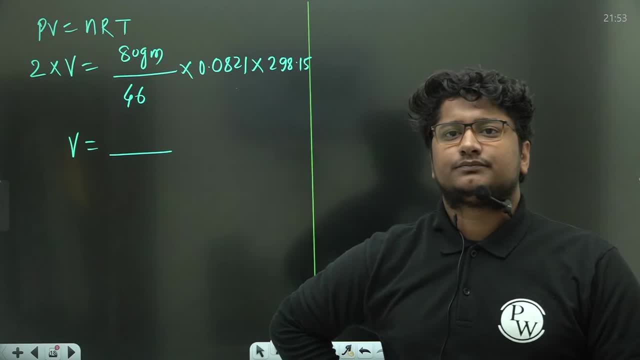 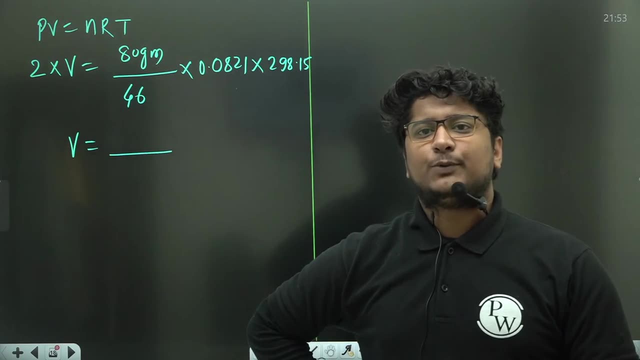 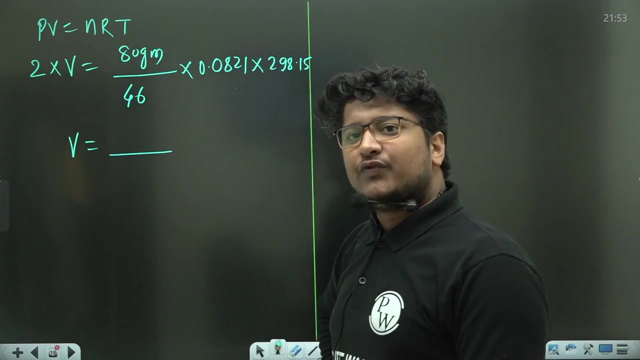 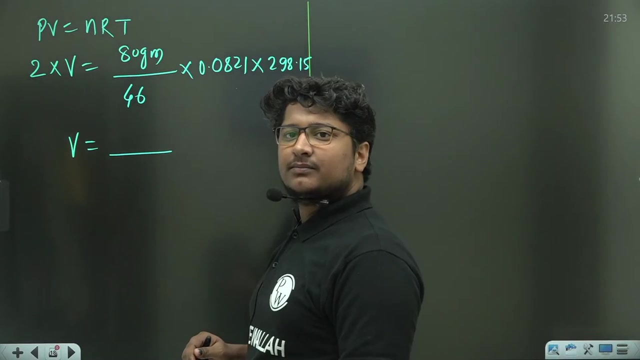 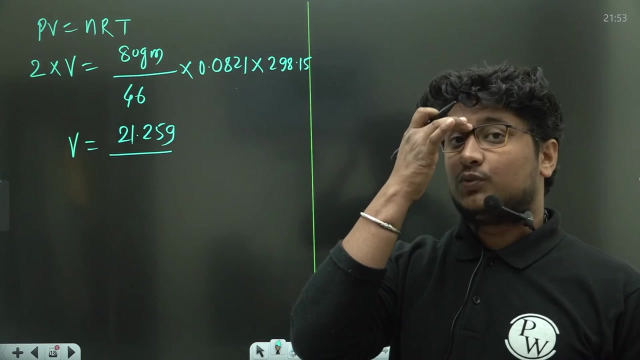 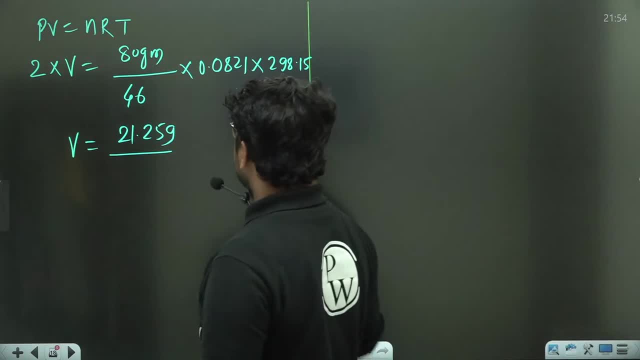 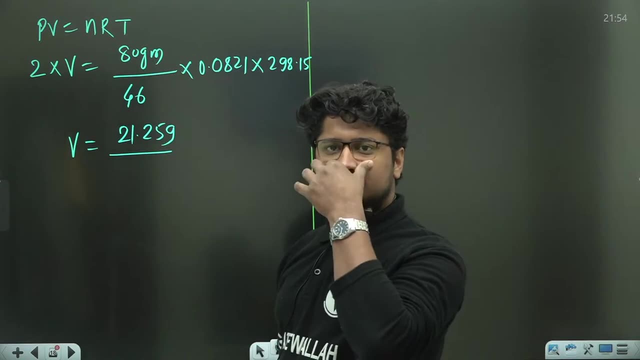 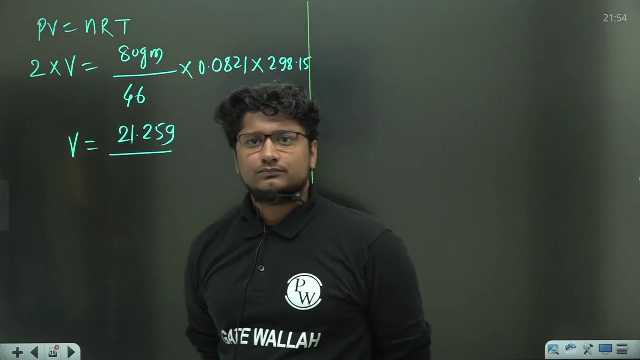 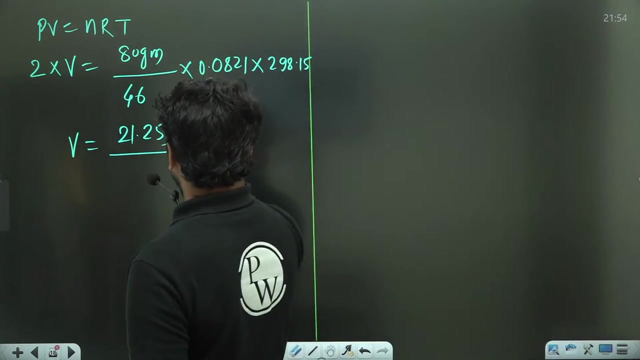 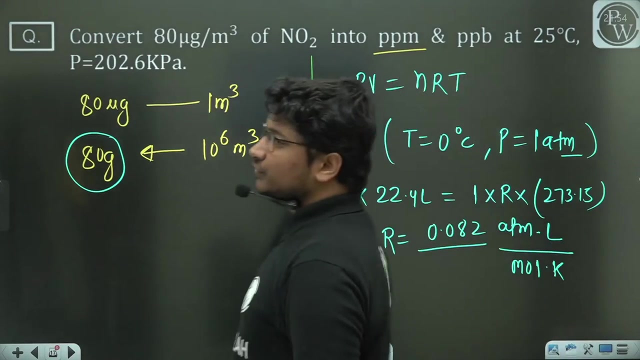 21.259, 21.259 in liters. okay, why did you keep it in liters, sir? why did you keep it in liters, sir? because, sir, you kept the value of r in liters. you kept the value of r in liters. so, obviously, sir, the volume will also come in liters. 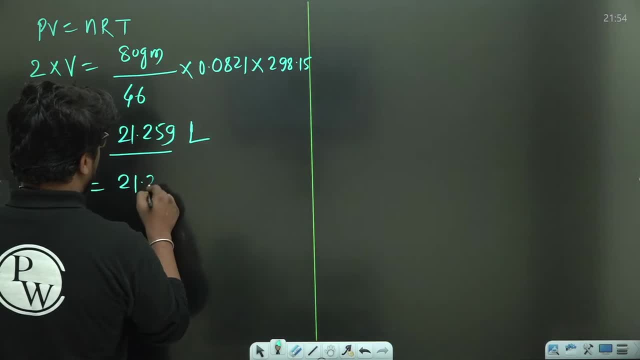 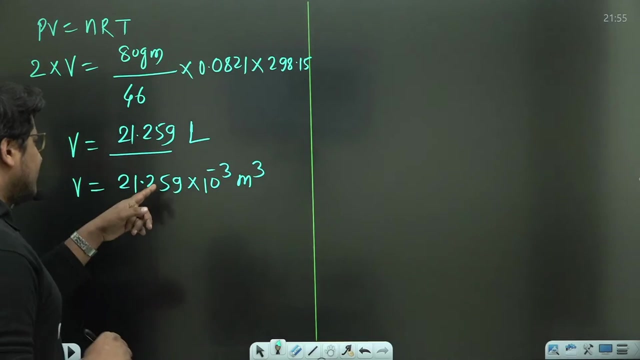 if I want to convert the volume into meter cube, then what I will do: 21.259 into 10 to power minus 3 meter cube, 21.259 into 21.25 into 10 to power minus 3 meter cube, that means this 80 gram is actually equal to. 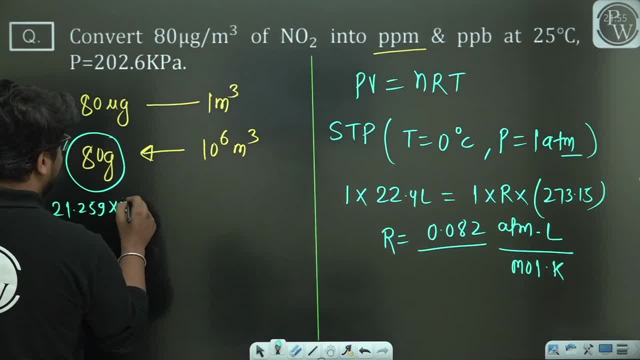 21.259 into 10 to power minus 3 ppm. okay, meter cube, now 10 to power, 6 meter cube. this much meter cube, you get NO2 here. this much meter cube, you get NO2 here in 10 to power, 6 meter cube. 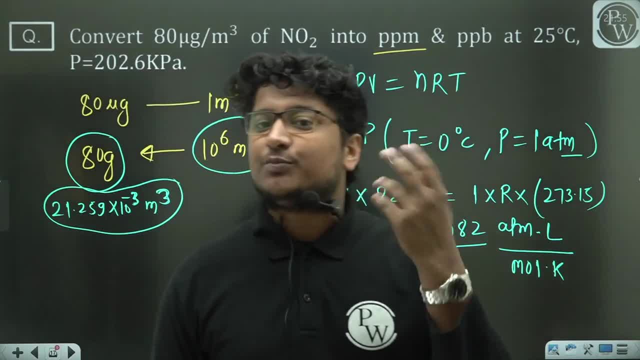 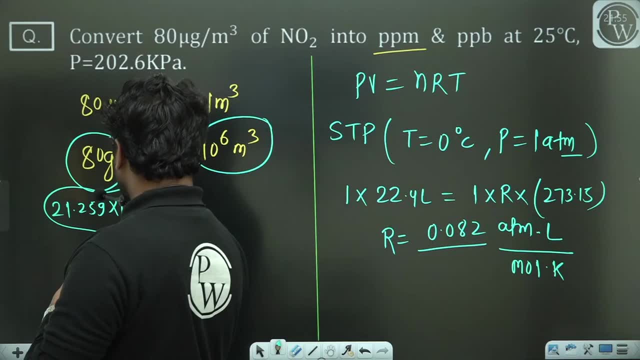 this much meter cube, you get NO2. so now someone will ask you what is the value of ppm? so you know it yourself, sir. answer will be 21.259. 21.259 into 10 to the power minus 3 ppm. what do you say? 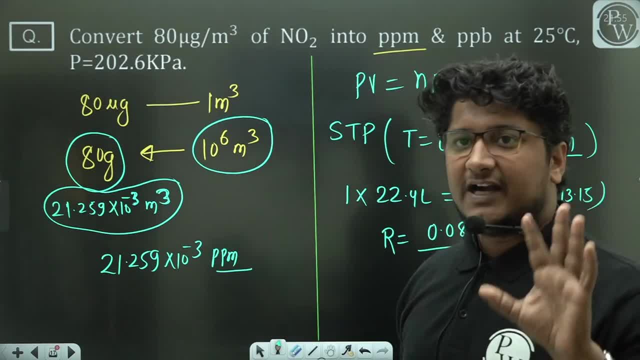 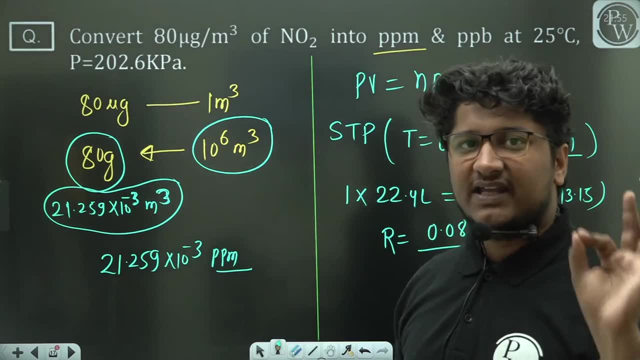 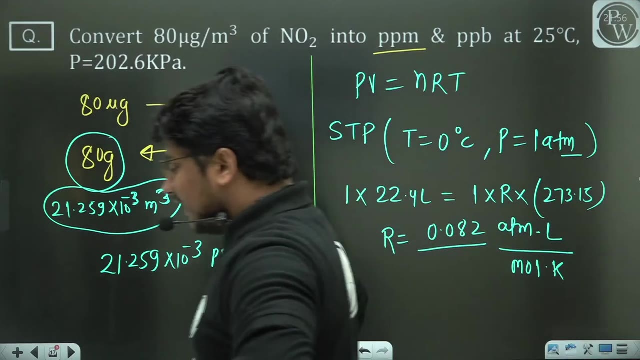 did you understand? how many people understood the ppm part completely? yes, sir, I understood. yes, sir, I understood line by line what you told me. conceptually, I understood. I didn't print it out. I solved it with you, sir. how many of you have understood completely? sir, I didn't print it out. 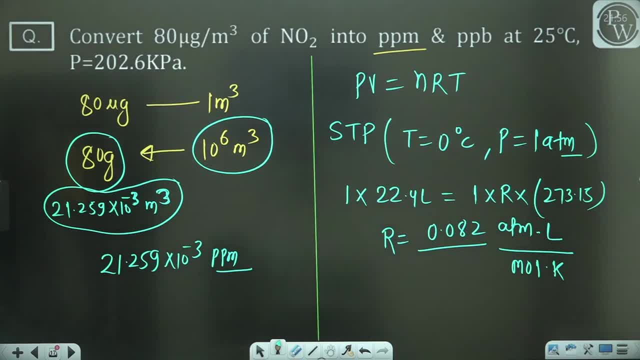 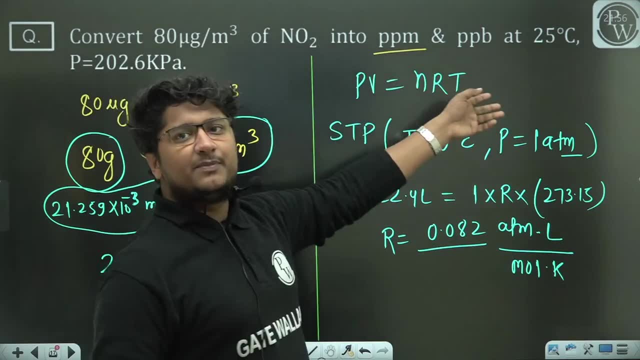 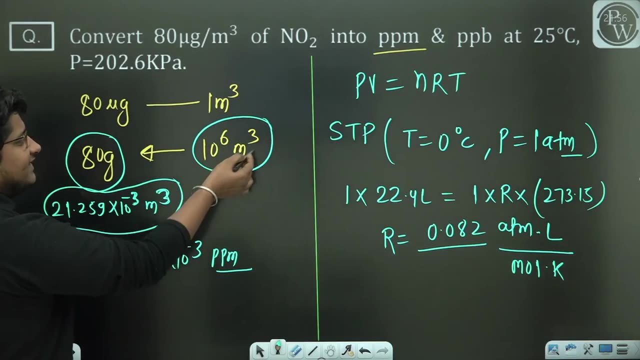 I solved it with you, ok. so once you got the ppm value, second part, pp is also asking you. that is for 10 to power 9, he is talking to you. 5 to the power of billion, he is talking to you. so you see, if it is so much present in 10 to power, 6 meter cube. 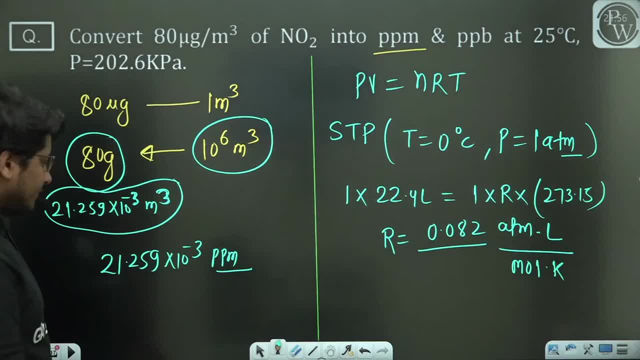 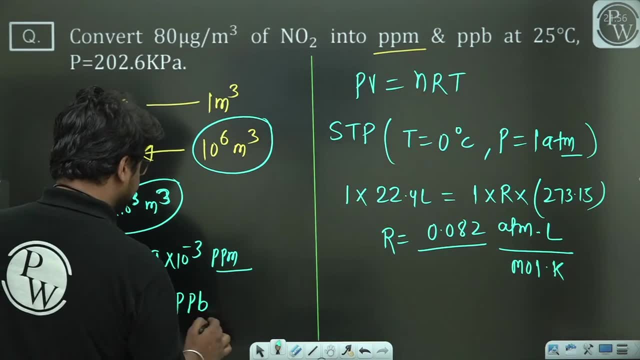 then what will happen in 10 to power 9 meter cube? just multiply it by 10 to power 3, so if I talk about your ppm, it will be 2.259 ppm. now tell me, if no one has a problem, how many people have understood this thing. 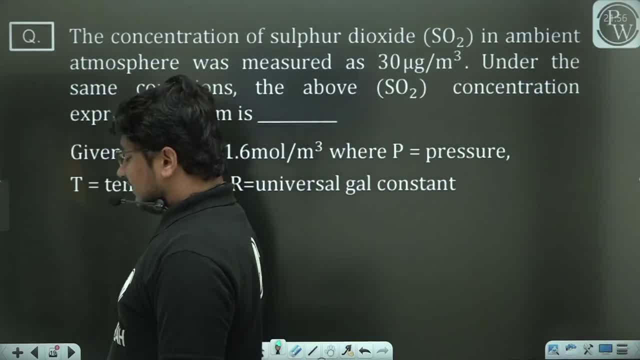 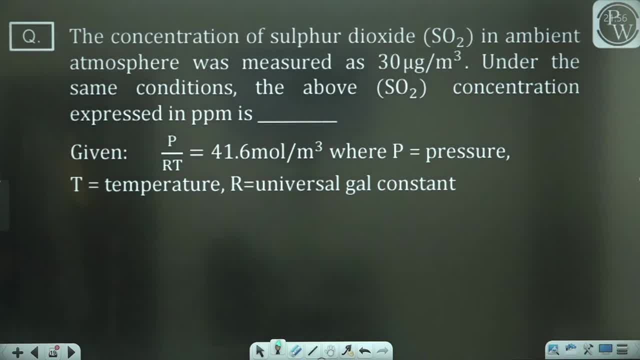 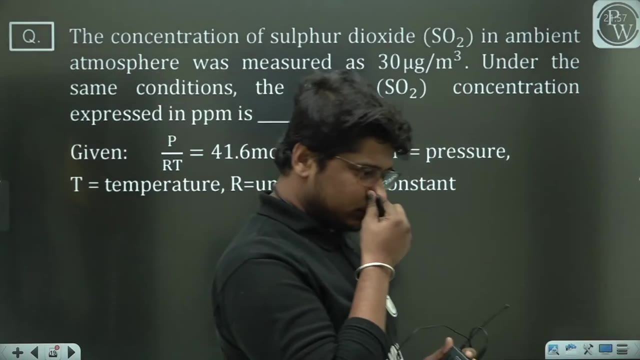 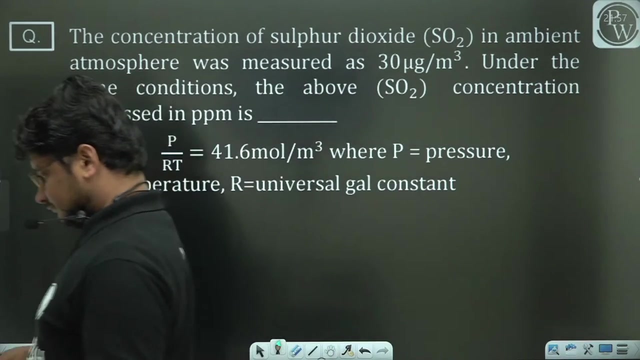 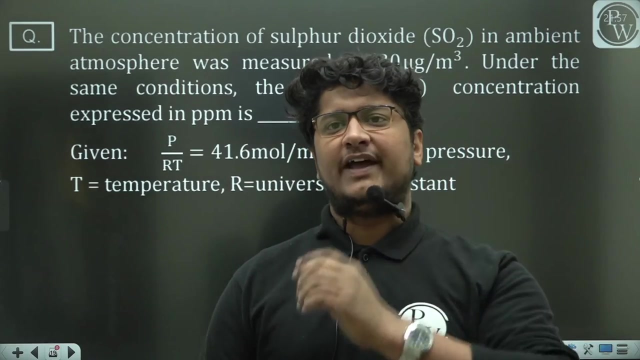 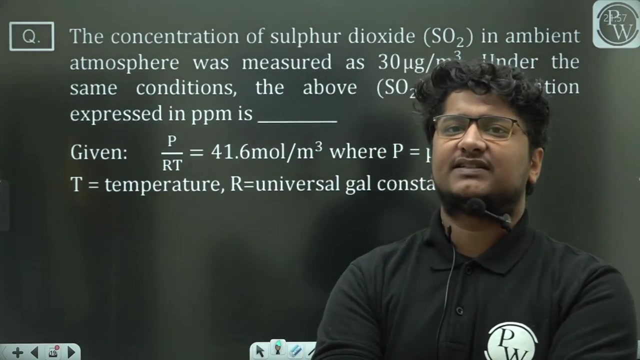 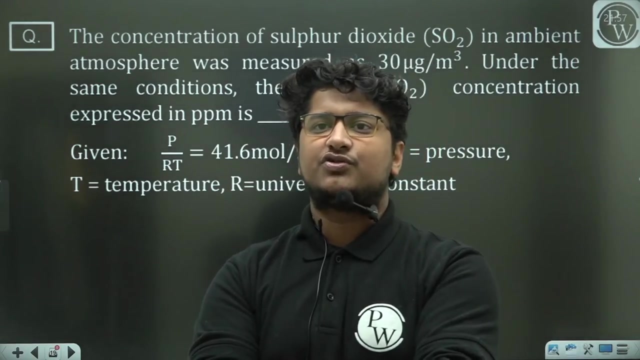 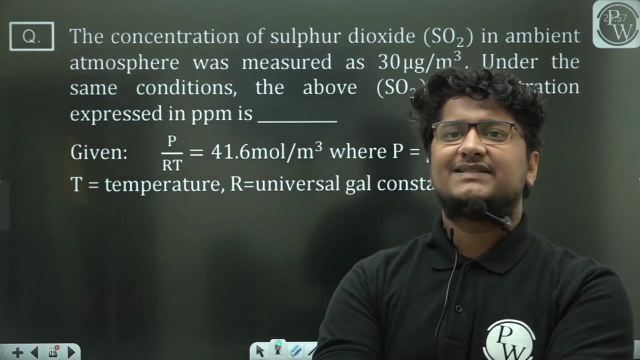 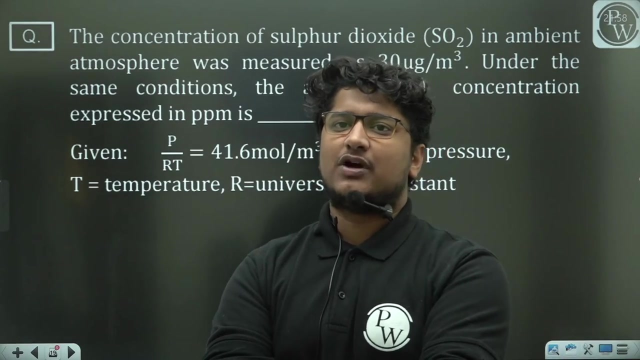 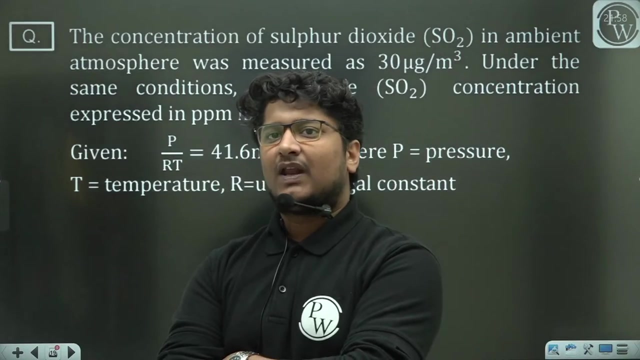 All the people who will not answer: that means you have not understood the previous question. All the people who will not answer: that means you have not understood the previous question. All the people who will not answer: that means you have not understood the previous question. 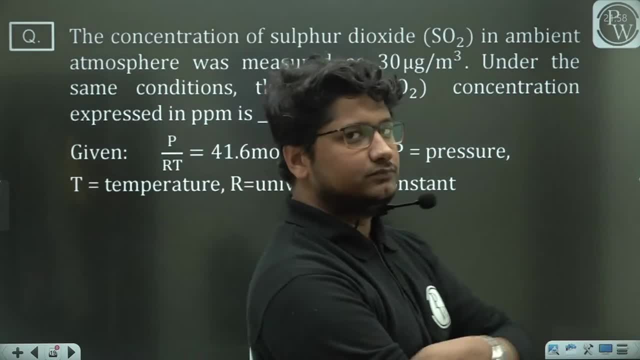 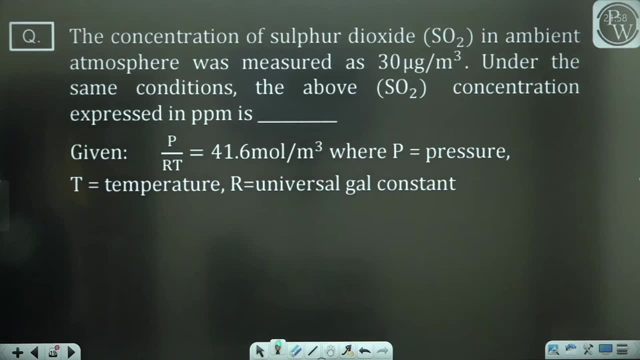 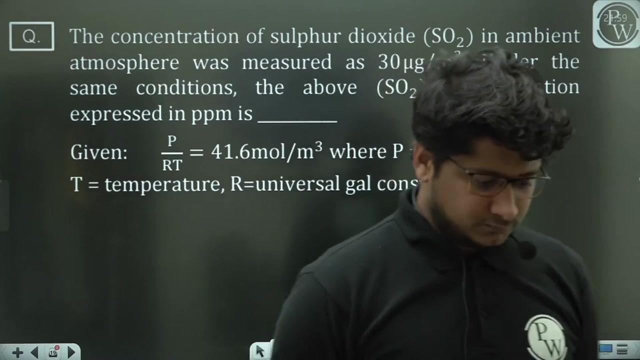 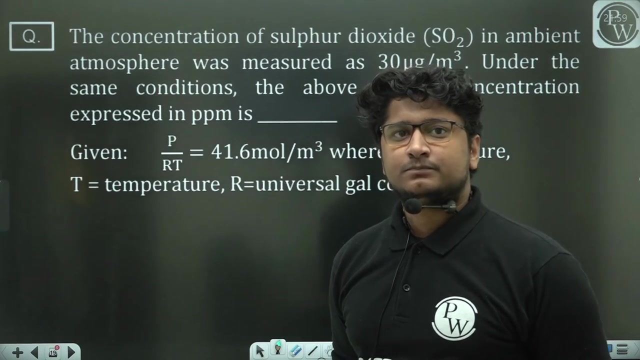 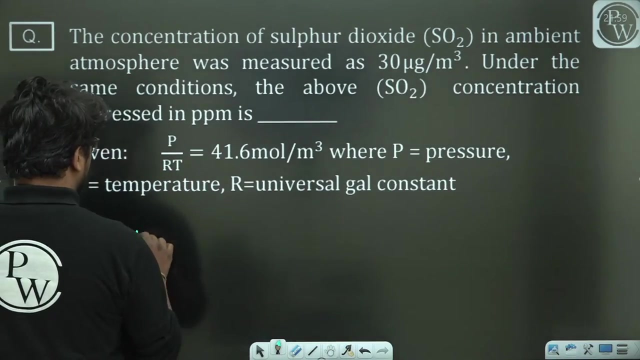 Thank you. You, I think, Sumesh, Gaurav, Vivek Akash. people are giving a simpler answer: Nothing. It's a simple question, Sir, 30 micrograms are present in 1 meter cube. You need it in ppm. 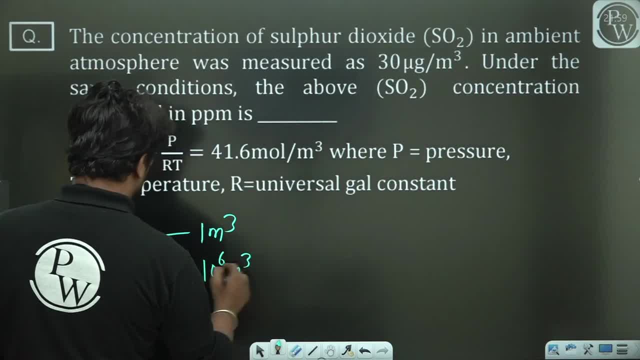 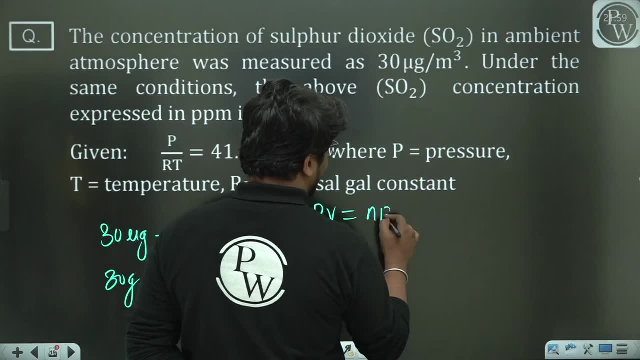 Sir, how much will it be present in 10 to power 6 meter cube? Sir, 30 gram will be present. I will just convert 30 gram. The story will be over. So pv equal to nRT In the question, sir p upon. 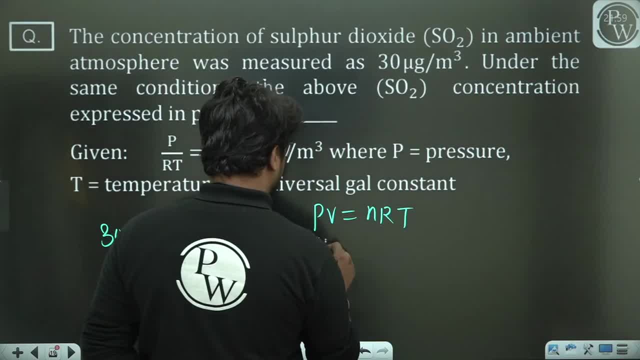 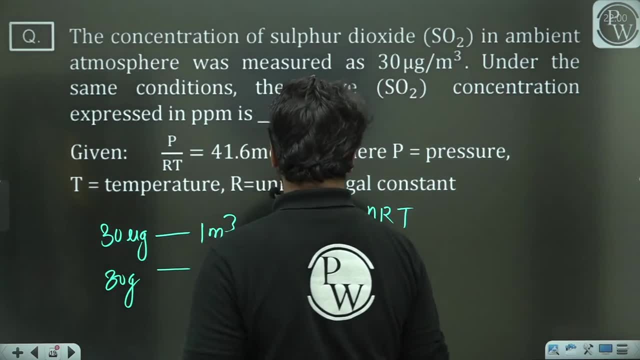 RT's value is already given. So it's a good thing, sir. p upon, RT's value is already given. Into volume And number of mole will be 30 gram. That is a given mass divided by sulfur dioxide. So it will be 32 plus 32, 64.. 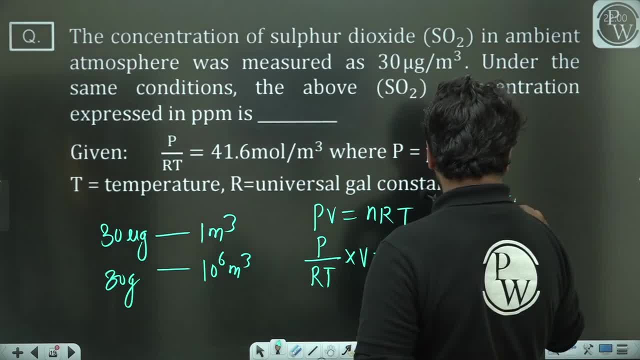 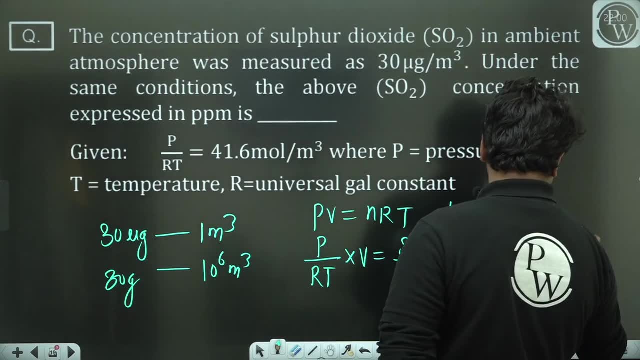 So if we are asked to subtract volume from here, then how much will it be? 30 divided by 64. p upon RT's value is 41.6, sir. So now the value you will get directly, which will you get? It will be found in meter cube. 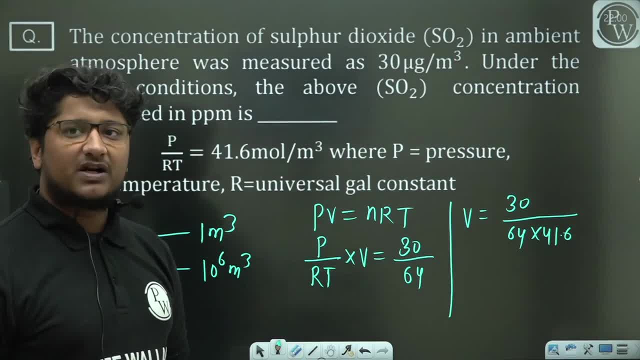 Because your p upon RT's value is given in your mole per meter cube. So whatever value you will get of your volume, it will be found directly in meter cube. I think all of you have the answer: 0.01126.. 0.01126. 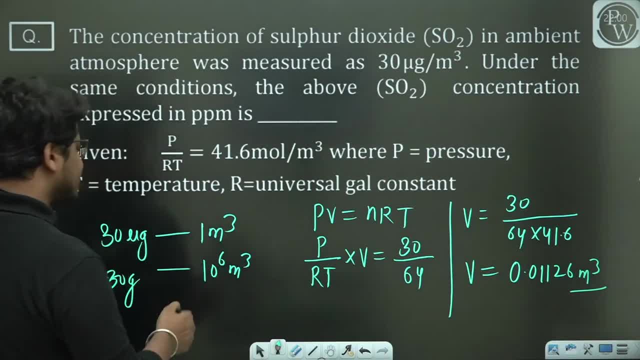 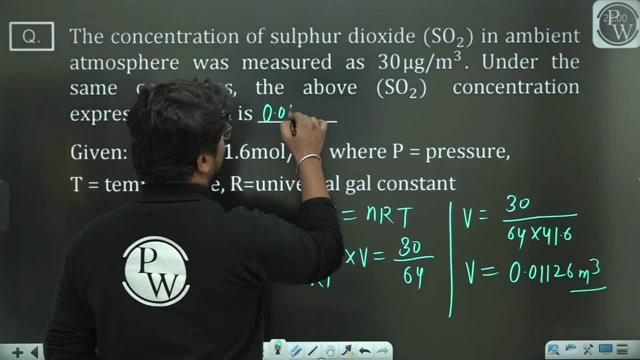 meter cube. Now, this much meter cube is present in 10 to power 6 meter cube. That means that much ppm we have, So final answer will be 0.01126 ppm, And this question has been asked in GATE 2016 for 2 marks. 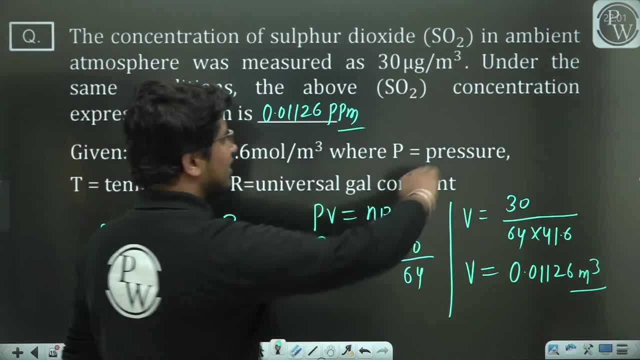 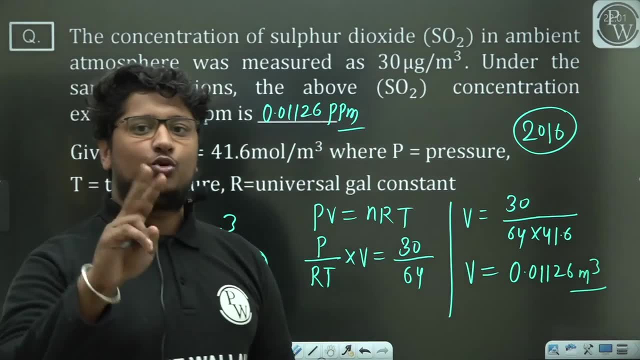 Now tell me how easy is this question? This question, I think I am not sure, but it was asked in GATE 2016 for 2 marks. So how beautiful was the question? How beautiful was the question? Within 2 minutes, you all can answer. 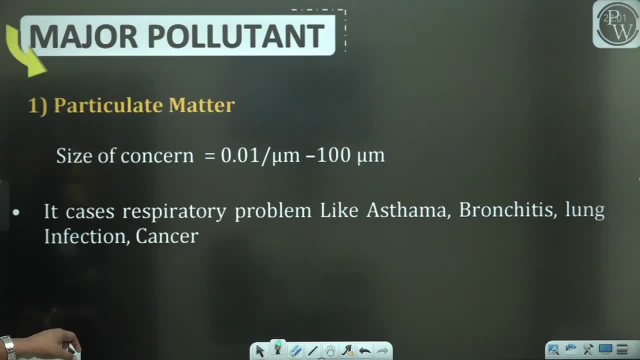 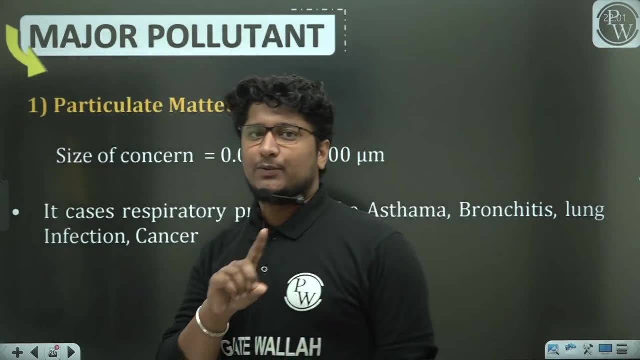 Within 2 minutes, you all can answer. Within 2 minutes, you all can answer. Now we will talk about some major pollutants. The first question can be asked from here in air pollution. It was asked in 2015.. So correct it. 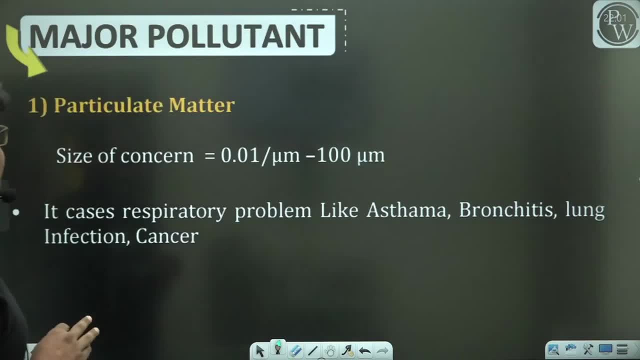 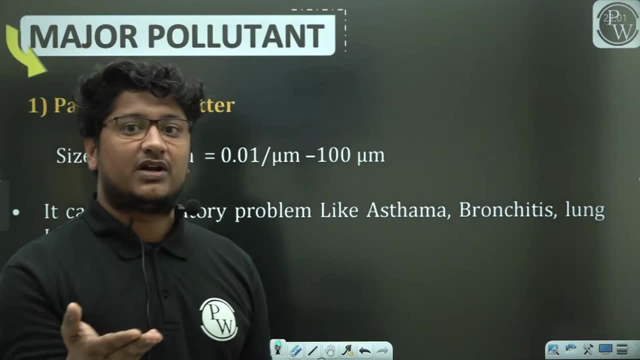 I knew that it was a question of GATE. Now we are talking about major pollutants. So the first part was the question from where it can be asked. I have explained it to you. Still, questions are being asked from there. 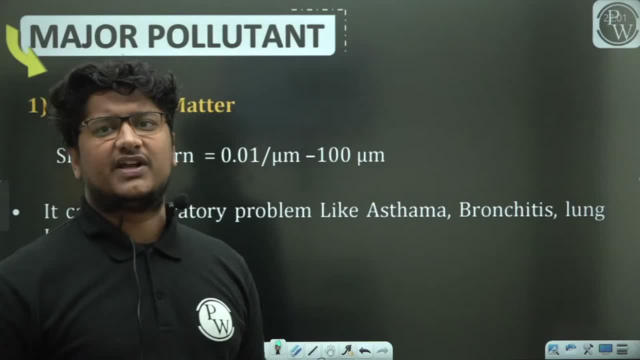 You have said that it has come in 2015 as well, And still recently- I am talking about 2019 or 2020,. I have seen a question which has come to you on this concept, So this is a very basic concept. 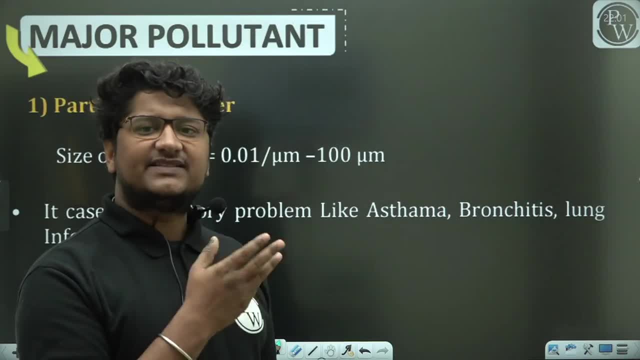 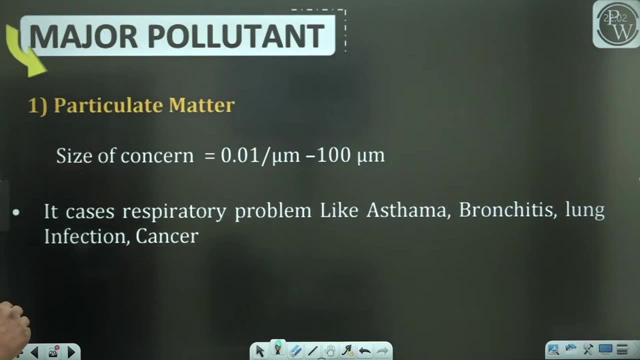 How we convert microgram per meter cube into ppm. That is the basic conversion. Everyone has to know that Next part is in major pollutants, particulate matter. So generally what is shown is the size of concern. Size of concern means. 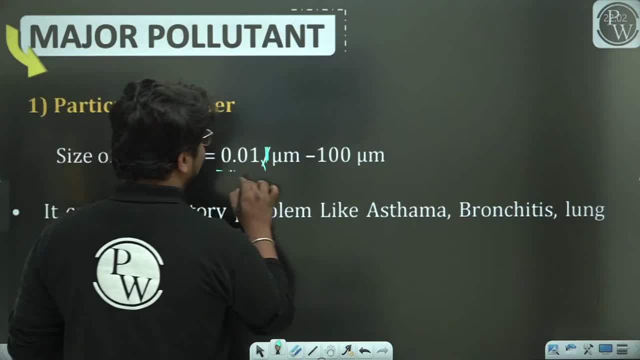 the effect on which you focus more. That is 0.01 micrometer to 100 micrometer. That is 0.01 micrometer to 100 micrometer. That is 0.01 micrometer to 100 micrometer. If we are thinking about. 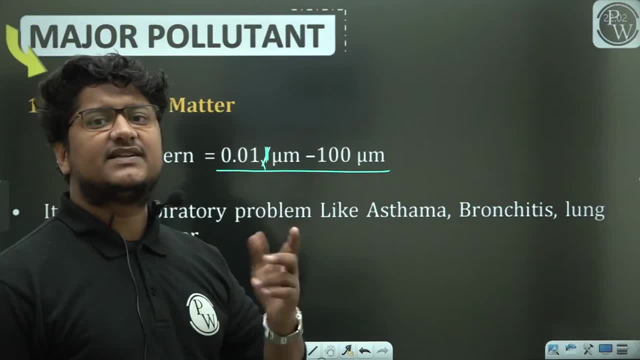 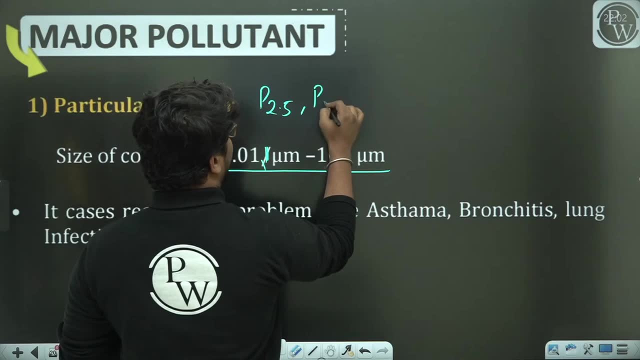 every particle. Does that harm us more Or do we have more concern for that? Generally, you keep two type of particulate matter in mind. One is PM2.5 And the other is PM10.. Your PM2.5 And your PM10. 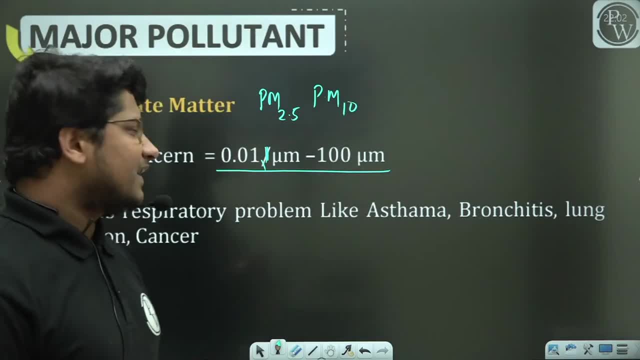 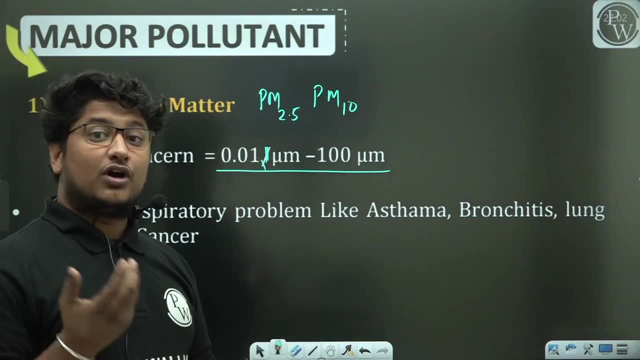 I will tell you the last. What are they? Both of them are particle size, One for 2.5 micron particles And other for 10 micron particles. who is more dangerous? because both of them listen. and you people, sir. pm 2.5 concentration. 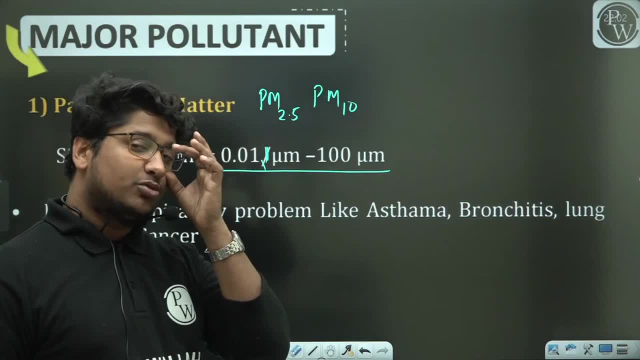 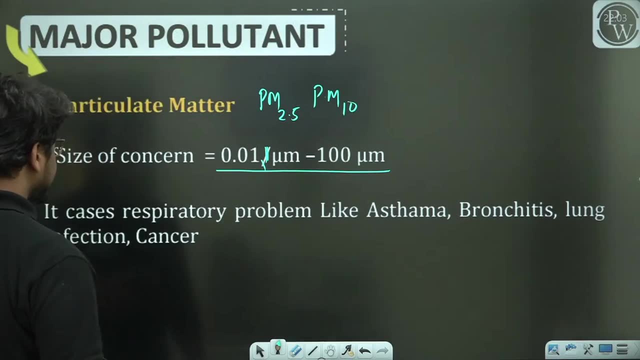 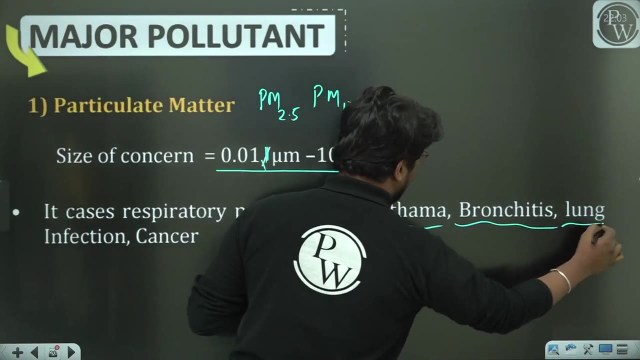 is so much in the atmosphere- pm 10, you are so much in the atmosphere. who is more dangerous than both? for you as a human being, who is more dangerous than both? the rest particulate matter. what problems do you create? you already know, like asthma, bronchitis, lung cancer, lung. 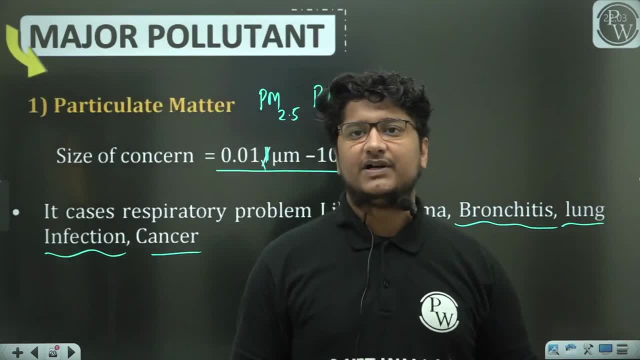 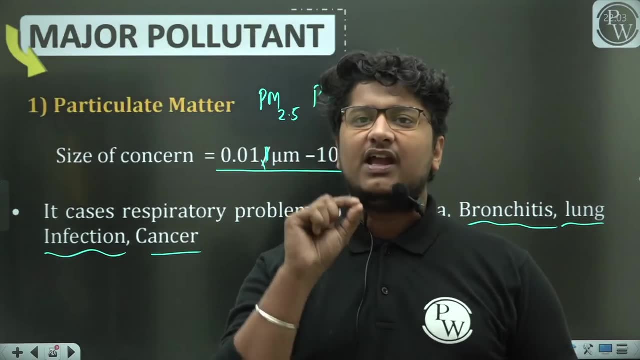 infection. all these things can happen to you because of this, for the particulate matter, 2.5 more dangerous for us. what is the problem? that we have nostrils inside the nose, which you have hair inside. it is called nostrils, so nostrils, that is yours, it can stop pm 10. 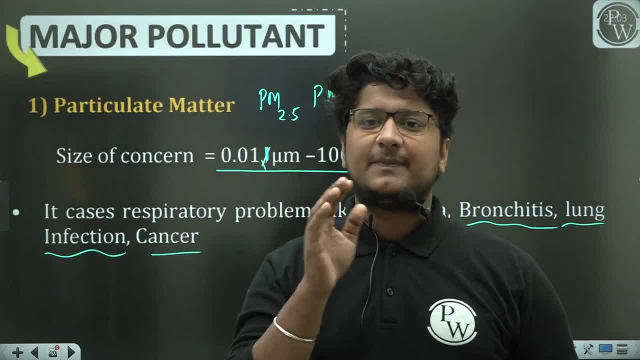 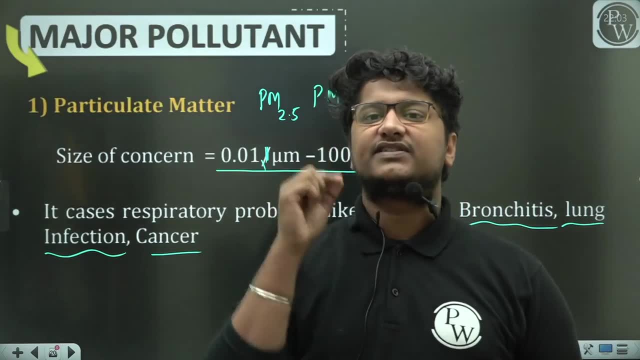 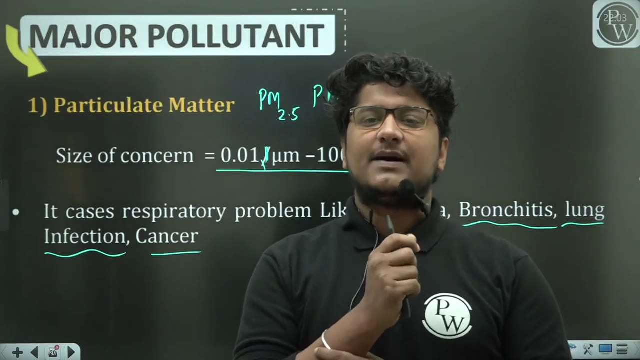 its capacity is that it can stop the particles of pm 10 or the big particles of it, but the particle of pm 2.5 they cross our nostrils. then what is that directly goes to the lungs and if you have something like that, so what will it do to you? if you have something like 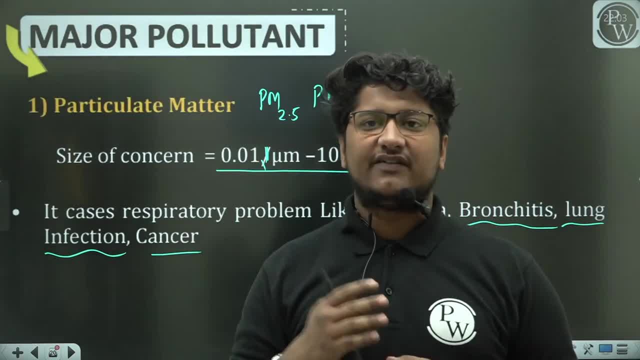 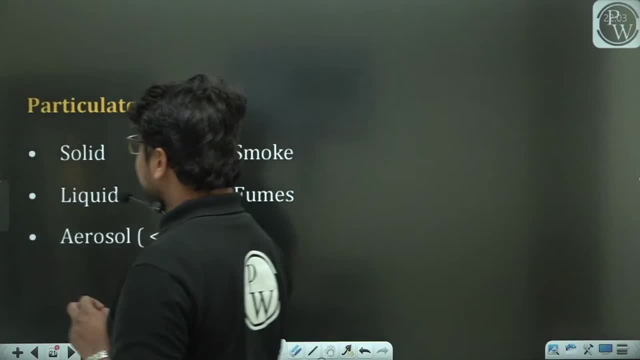 this, then what will it do to you? if there is something like this in your lungs, then can also cause infection in your lungs. PM2.5 is more dangerous compared to PM10, keep this in mind. Rest, you have different types of particulate. one is your solid, which I had told you example. 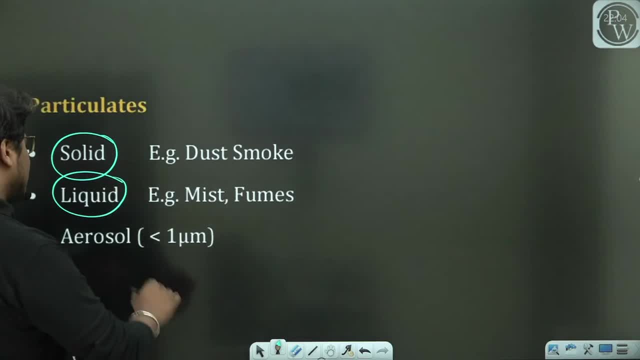 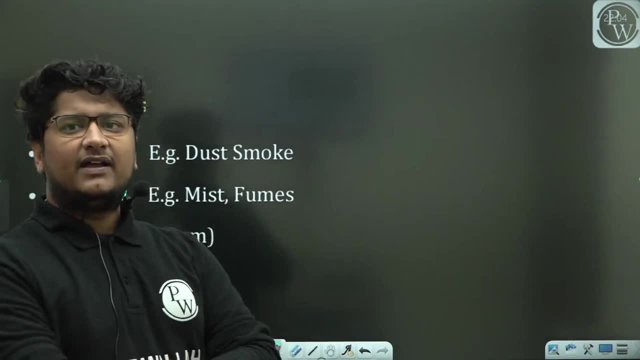 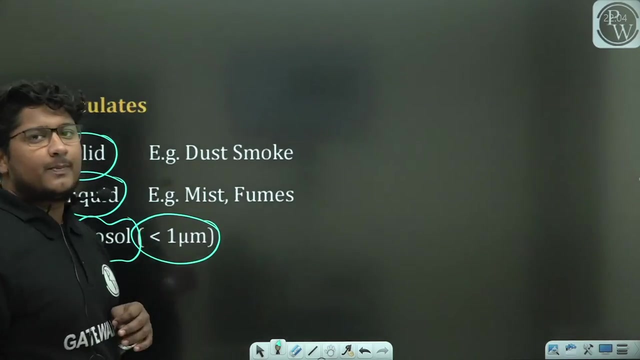 also. second is in liquid mist or fumes. and the third one which is new to you nowadays. it came in research a long time ago, but now, in local language, it has come a little late. that is your aerosol. what is aerosol? you call it less than 1 micrometer particles. 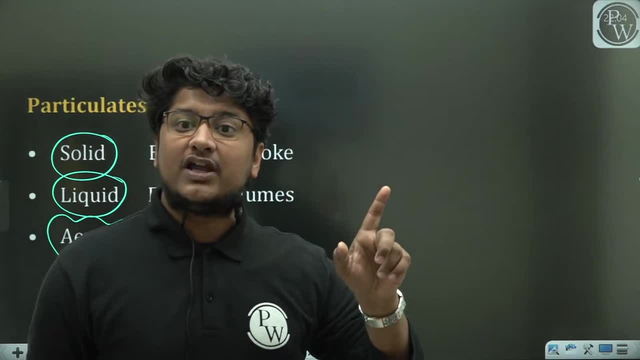 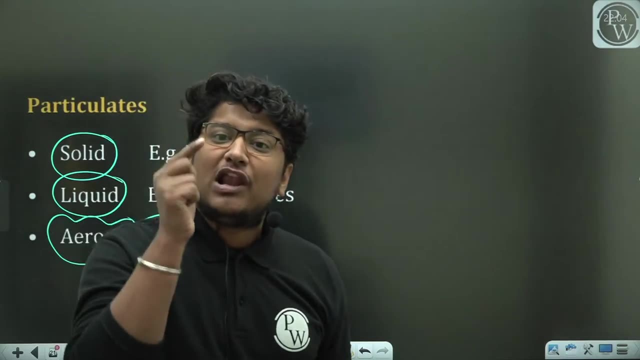 now. it is such a small particle that you will see many times. you will not be able to tell exactly whether it is a solid particle or a liquid particle if you have a size of less than 1 micrometer particle- and I give you that, whether it is of water or soil, will you? 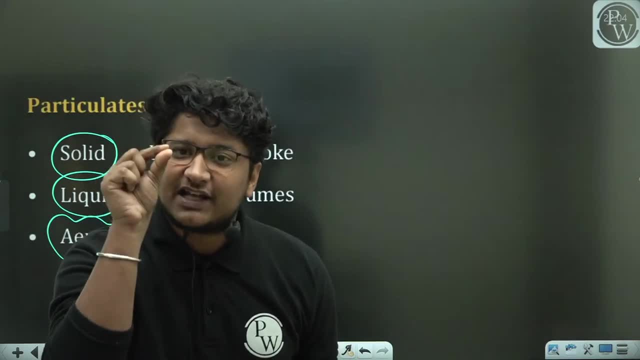 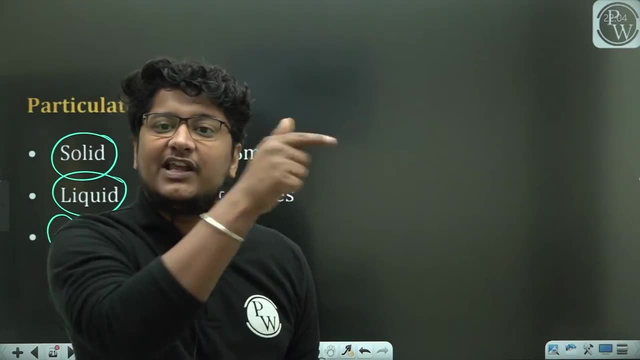 be able to tell such a small particle, such a small particle so exactly you are not able to tell, not knowing that, what type of behavior it is showing? it is showing the behavior of solid or the behavior of liquid? that exactly you will not be able to tell. so in that case, 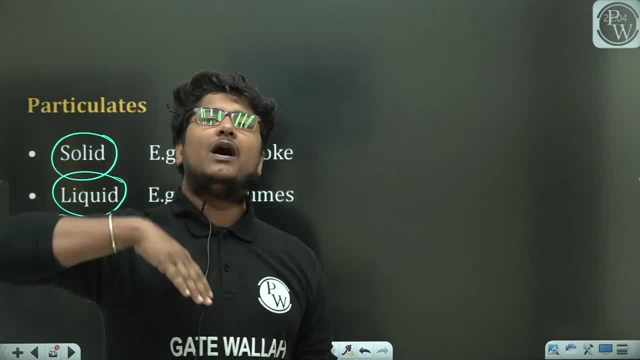 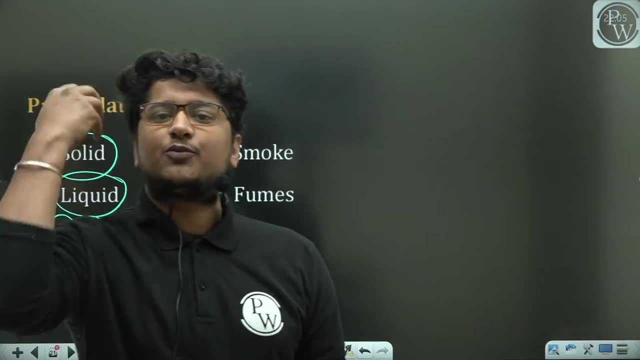 the aerosol generally. what happens to you? such a small particle always remains in the atmosphere in suspension. it will settle very rarely because such a small particle always remains in suspension. so this is your aerosol. a lot of research is going on on. 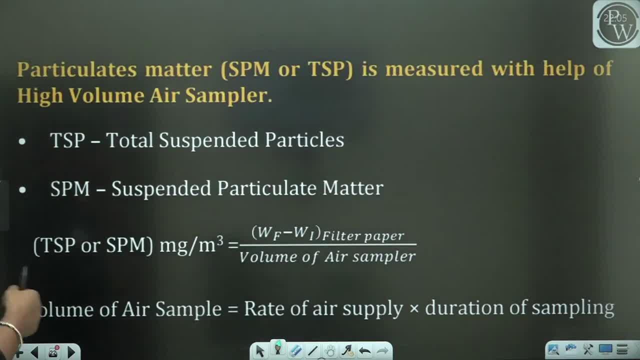 it nowadays. next now, let's talk about your particulate matter. Next now, let's talk about your particulate matter. Next now, let's talk about your particulate matter Generally. many times we call it SPM- suspended particulate matter- or total suspended particulate. 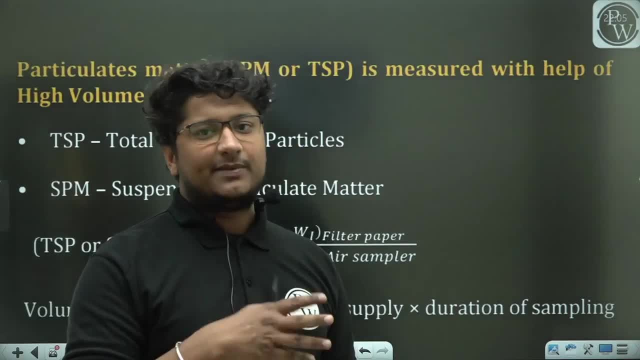 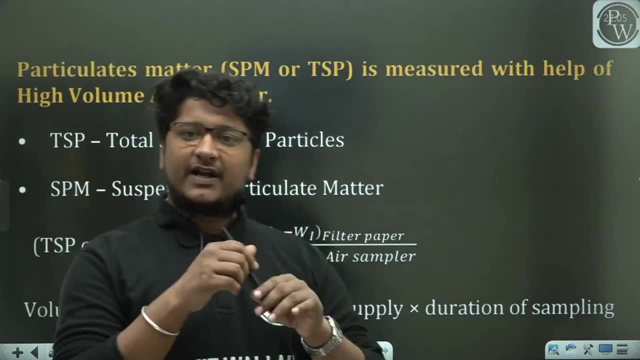 so the way to find out this is also very simple, and I have seen you asking questions from it. what is the simple way? see that, brother. what do you do? take a filter paper, take the weight of the filter paper. dry the filter paper, take its weight. that is the initial weight. 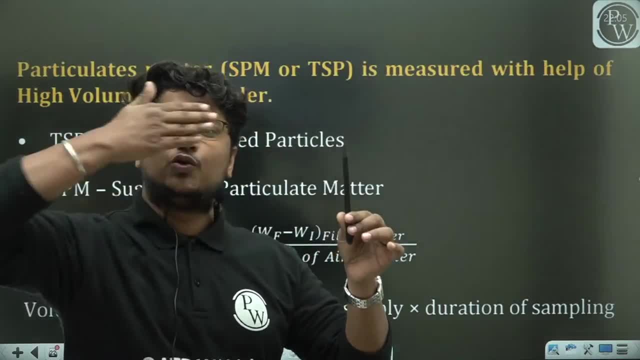 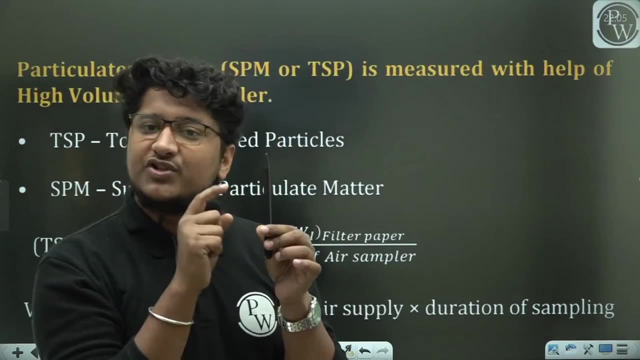 now pass air with this filter paper. whatever your flu air is, pass your flu gas. when you pass air, then what will happen in it? whatever your particulate matter will be will be retained in it. now your entire spare air stopped. now wait again for this filter paper, if it is. 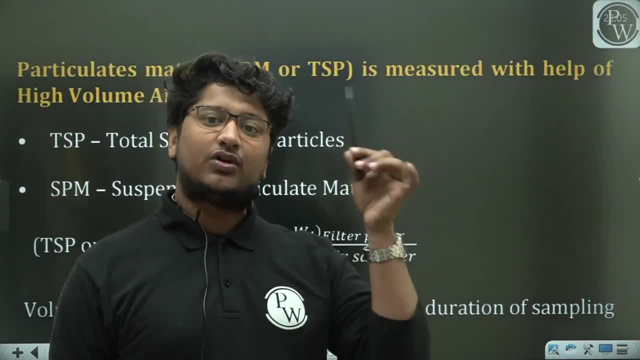 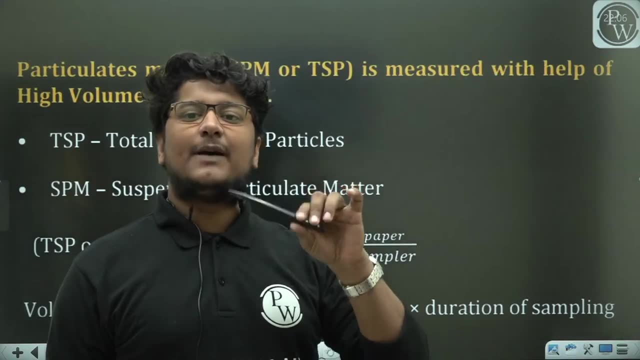 bad weight. dry it, but if you have wet it again, then you are being again. then the weight you will come. you will come late compared to our first weight. now try to find the difference between the two. then who brought the difference the way? now it is Committee. 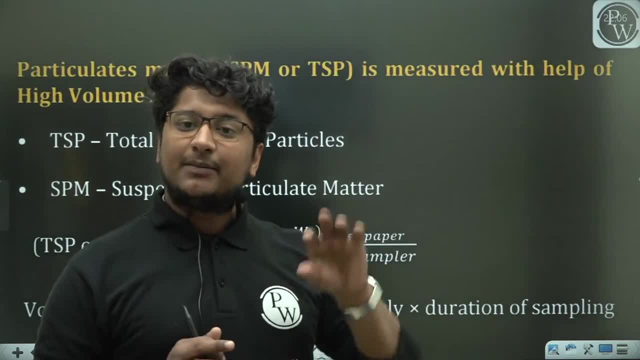 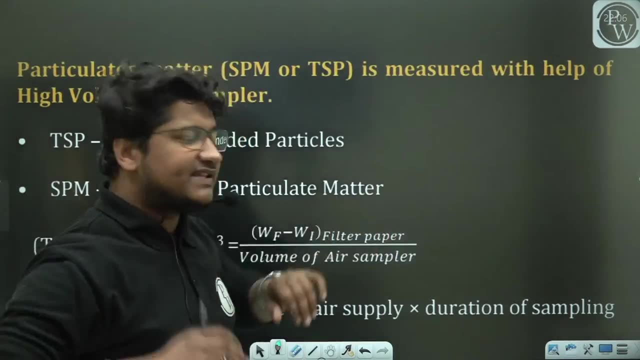 matters Just Cuz now because of particulate matter. now, now you have come to the air. So whatever difference you get, that is nothing but the given mass for the given volume of flue gas. Now how will we get the given volume? So what did we do to get the given volume of air sampled? The rate of air supply into duration of sampling, Rate of air supply into duration of sampling, will give you the volume of air sampled. So whatever difference you got, divide it by the volume of air sampled and you will. 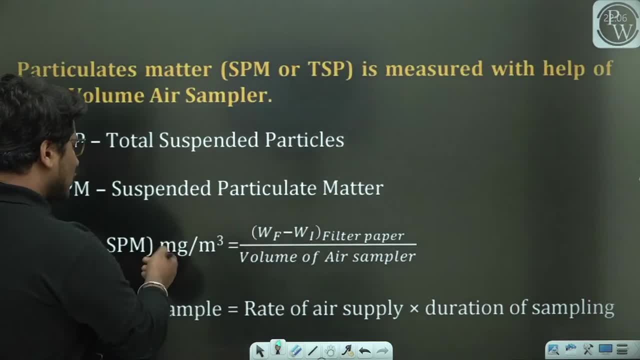 get TSP or SP, whatever you call it. In that case, if you want it in milligram per meter cube, then you will get it. or sometimes we tell it in microgram per meter cube, then you will get it. So this becomes a basic formula which you have to keep in your mind. 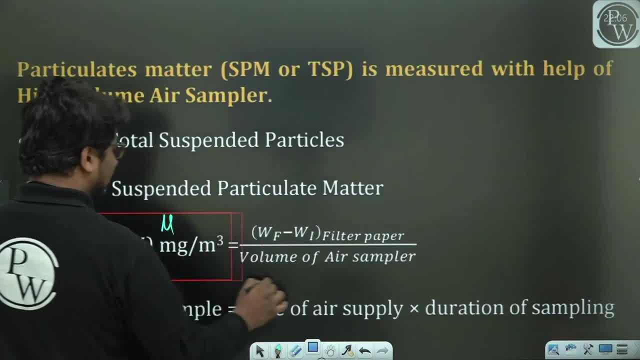 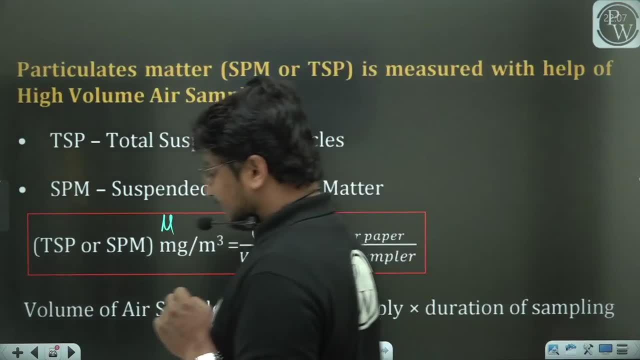 I don't think so. it is a very, very difficult formula for you to remember. Very basic formula. I have also asked you a direct question in the exam. keep it directly in your mind. Any difficulty in understanding this? Any difficulty in understanding this? 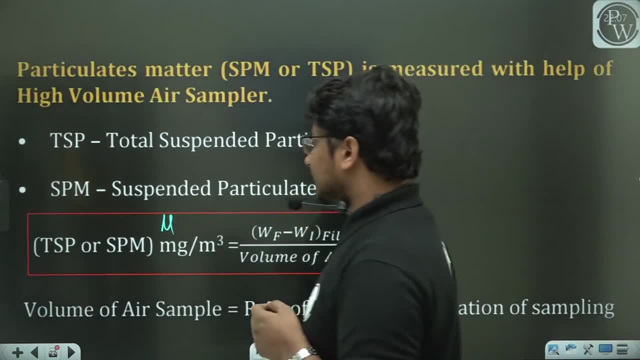 Anybody having any difficulty in understanding this, Any difficulty in understanding this formula. Any difficulty in understanding this formula. Any difficulty in understanding this. Any difficulty in understanding this formula. Two things, the same thing. we did, suspended solid, when I was teaching you in water quality. 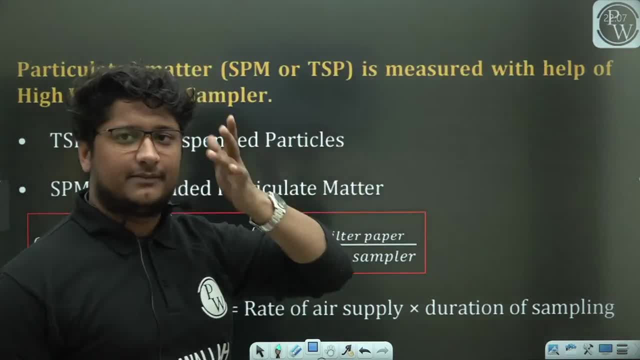 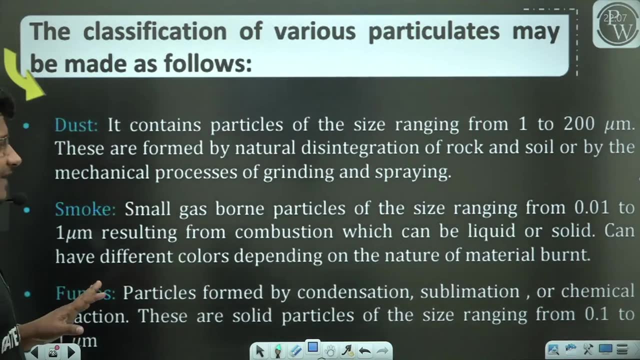 there. I did the same thing in filter paper. Same formula is also here. Same formula is also here. Nothing more than that. Now you have different types of particles which you live in the market, What you have to keep in your mind, their range, 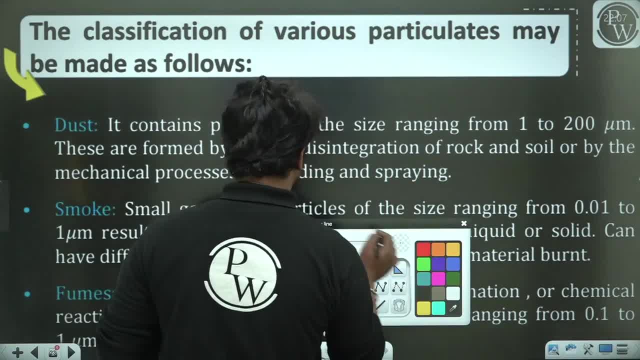 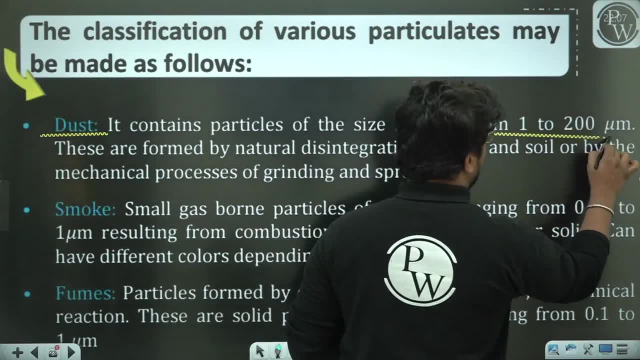 The size of the particle will be kept in your mind. That is enough. So see what is your dust. So what is your dust particle? What is your dust particle generally? your small rocks or soil part will be 1 to 200 micrometer. 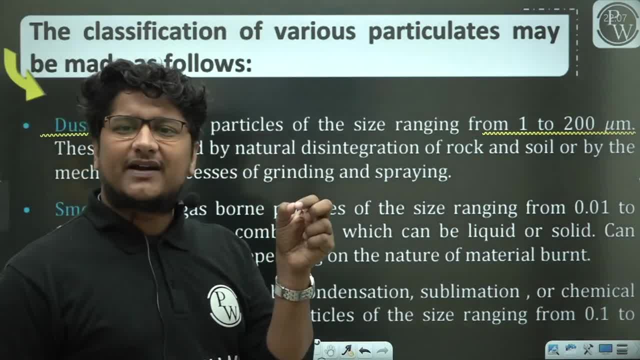 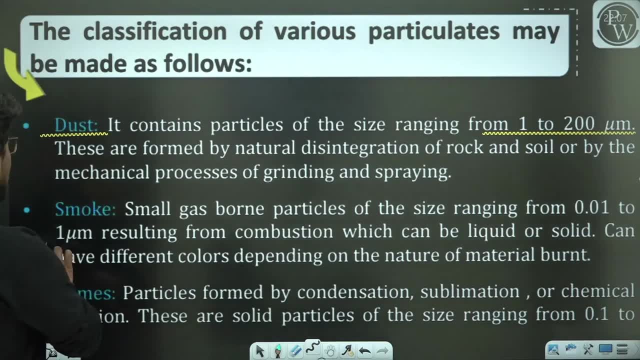 generally dust what you say. either it will be the broken part of the rock or the part of the soil, so it will be in the size of 1 to 200 micrometer. second is your smoke. its size is 1 micrometer and from 0.01 micrometer to 1 micrometer. 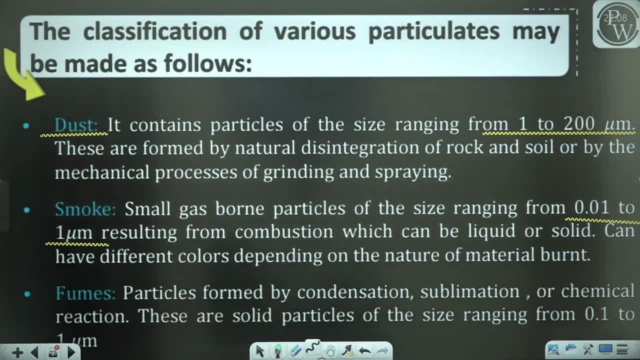 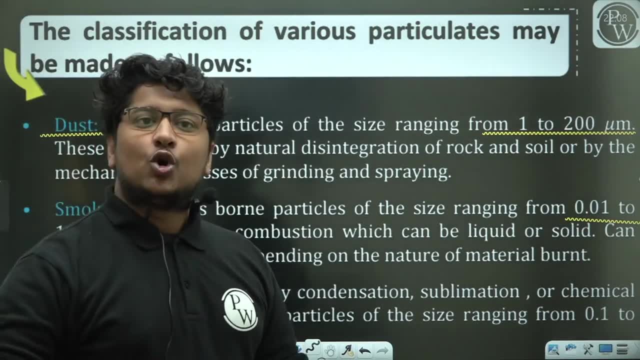 it will be in this range and this smoke is generally from where it comes out. if you see smoke, if you are burning wood, you get a different smoke. if you are burning coal, you get a different smoke. if you are burning something else, you get a different smoke. 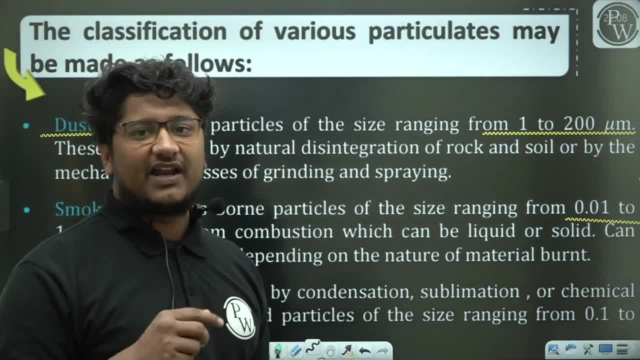 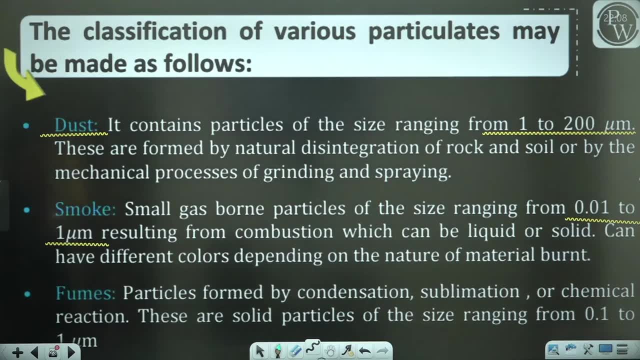 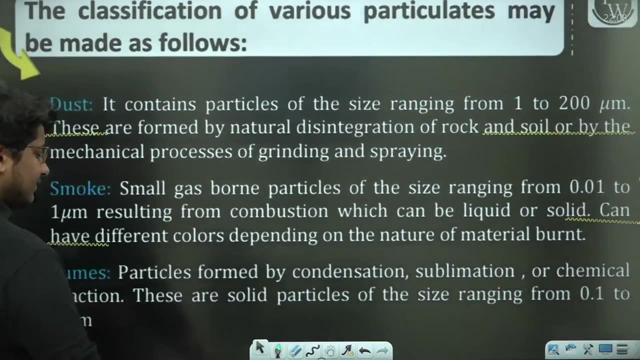 so the color and the type of the smoke depends on what you are burning. next is fumes. fumes are particles formed by the condensation, sublimation and chemical reaction. these are solid particles of size ranging from- keep this range in your mind. 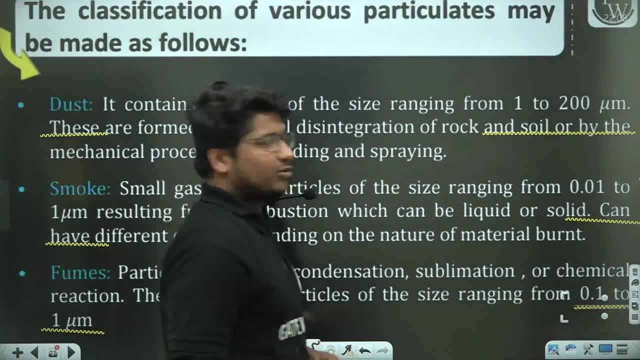 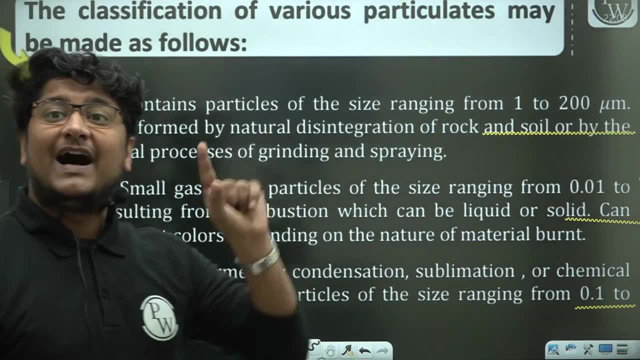 so its range is from 0.1 micrometer to 1 micrometer. range is often asked to you, Sir, for dust 200 micrometer, but for PM have a range of- yes, Arpit child, pay attention. I did not say the range of particulate matter from 0.1 to 100. 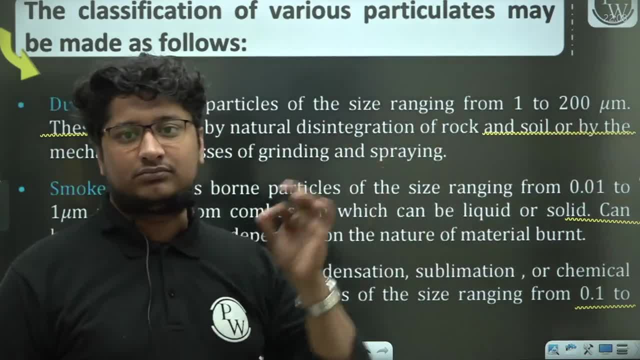 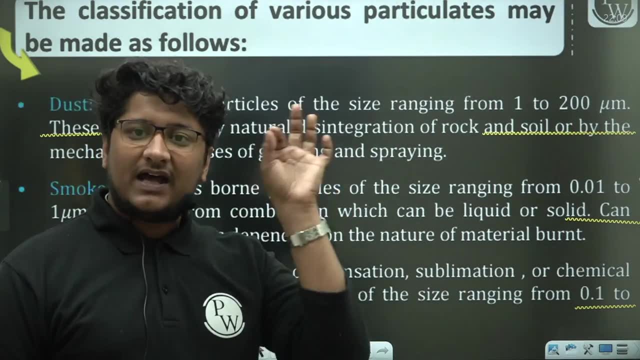 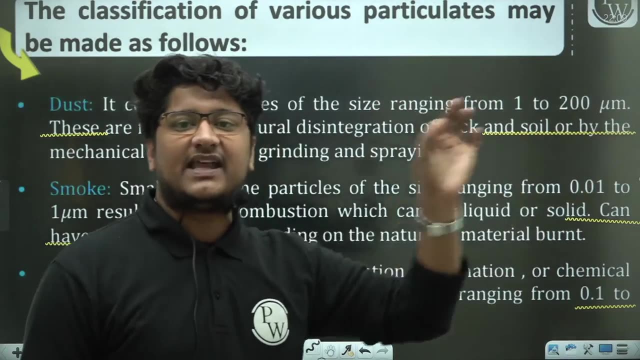 what I said in that size of concern. can you understand the point? can you understand the difference in both? I gave you the size of dust, that is, range of dust, the range I have given to you, what I gave in particulate matter, the size of concern. 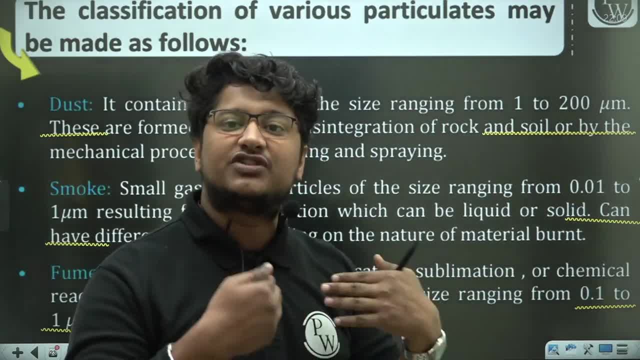 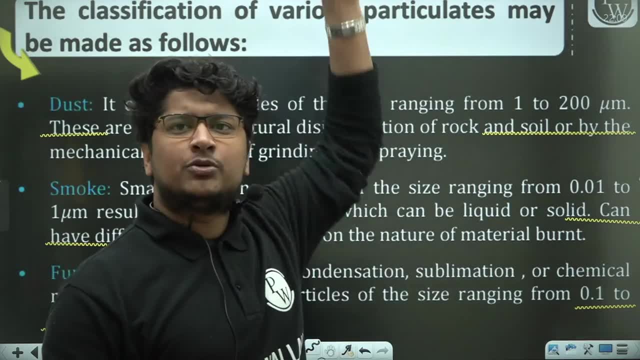 it means the size. we will study about it. they trouble us more. we will study about them. ok, it can be 200, 300 micrometer also can be. it can be up to 300. there is no such fix that particulate matter will be of this size. 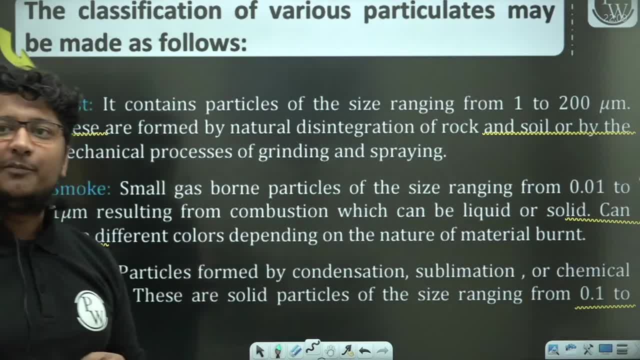 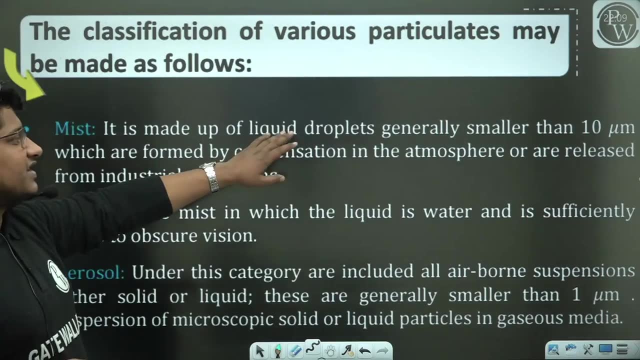 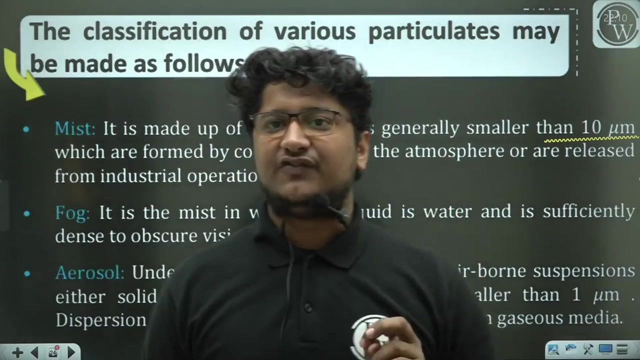 ok, it also comes in burning coal. yes, yes, now your coal is burning. so because of a 광, it is alright. ok, k 만, ok, ok, ok, yes. may for a confused with a mist or fog may confuse with a similar cheese. a but a key back to the hand up at the high he. fog is also a mist in which the liquid 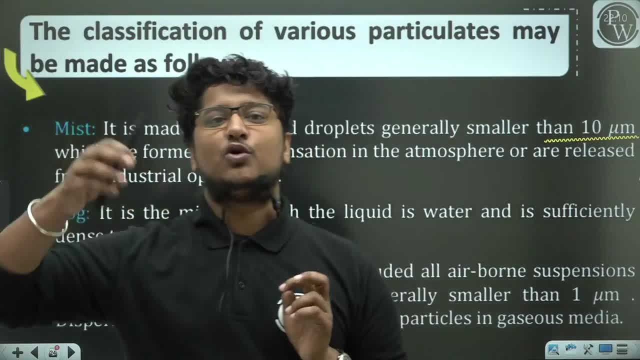 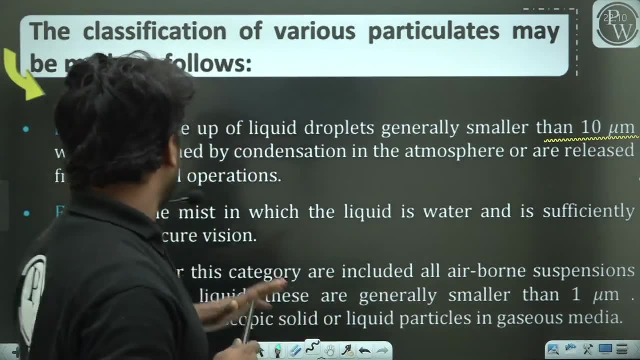 is water. that means mist. to have us me liquid do so, Robbie was at the high, for example. kerosene to be missed was at the high. kerosene to be up, co mix was at the high, so it's not quite gonna kick off kerosene to be up come this one's at the 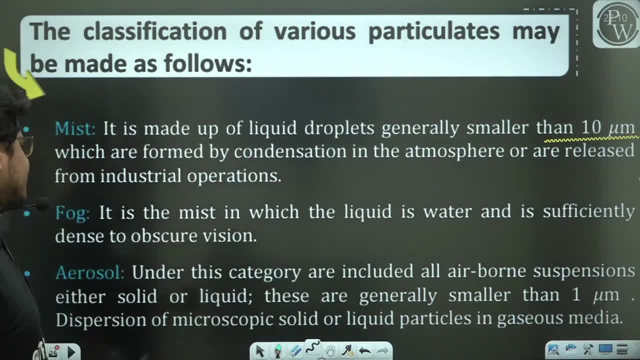 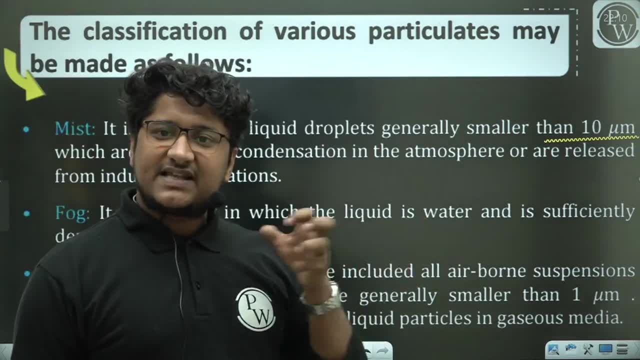 high, take a hum, just keep for key. I got bad. carry on to particularly water can kiss me up. go bad curry or fog may. it is all because at the high key to up key density that you go boho jada ready in city jada reiki to a pool of the sea bath. a up to visible knee decage, a up 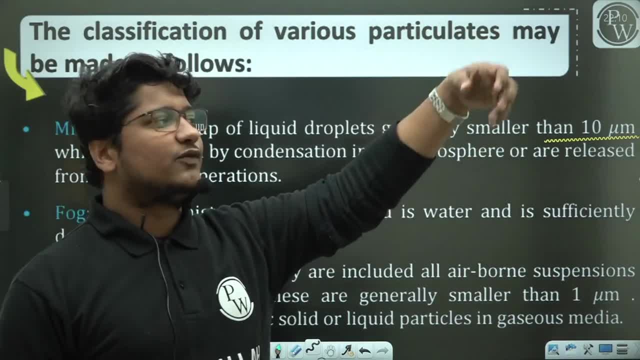 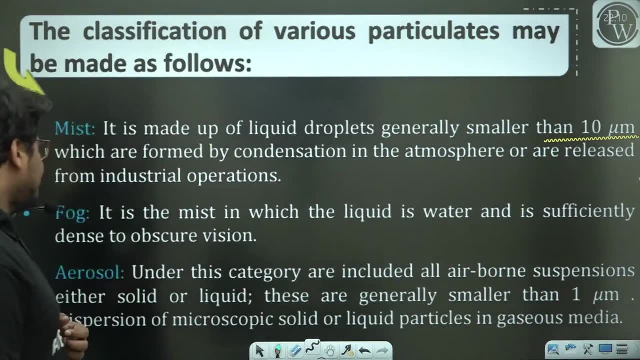 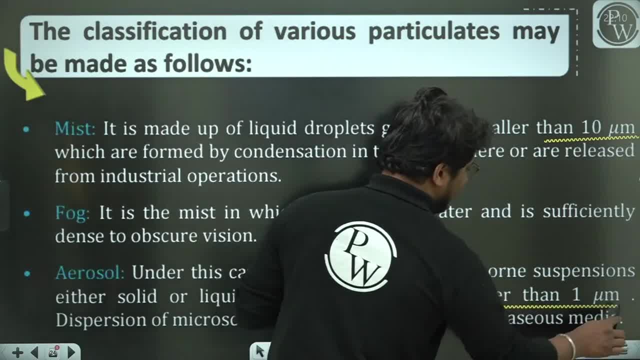 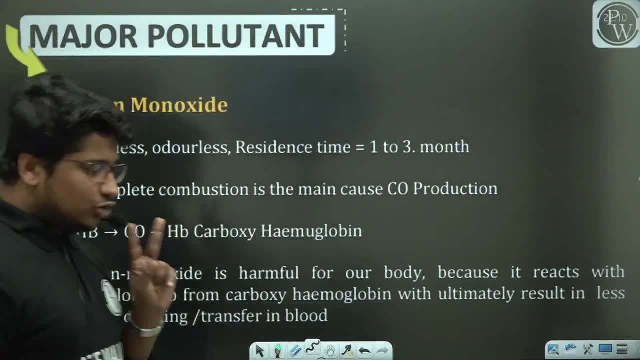 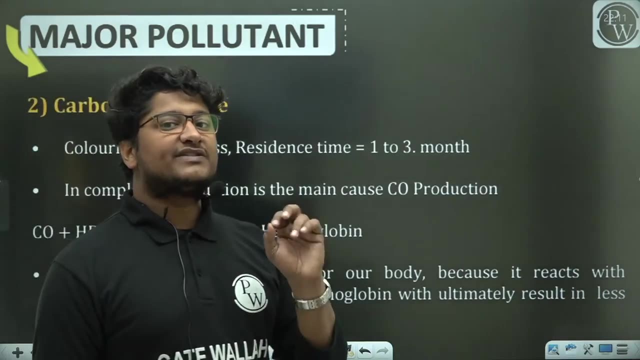 cup of idea is kidding joy. smaller than ten, one micrometer, corner than one micrometer to escape. regarding the aqua range, many, but I did tell you to Sarah Joe, I've got pollutant, a job key, the mark miracle, a poor Samajana head, that is carbon monoxide. I've carbon monoxide, key beauty, can I? 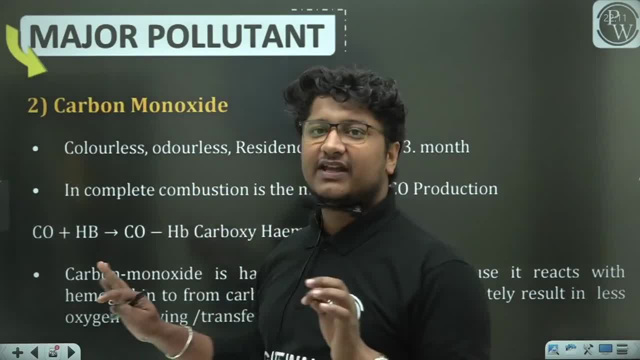 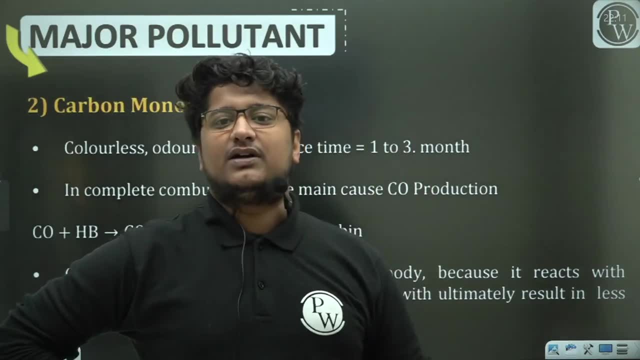 decode he a colorless hair order. less hair is up to take it. take this key beauty kiya he is sir, is key. residence time. boho jada haute abha batana kissy, be kissy, be pollutant car, agar resistance time jada hoga residence time. 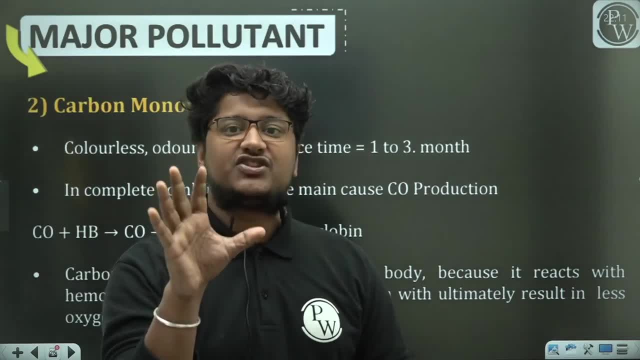 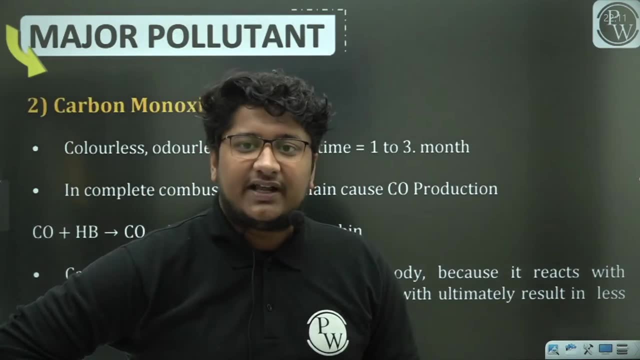 jada hone ka matlab hai. he was same same same nature, me same form me. jada time, tak atmosphere may retain rata to walk Lee honey karak, jada karega, which jada loko effect, karega, jada loko expose, may I exposer, may I go to in that case up. 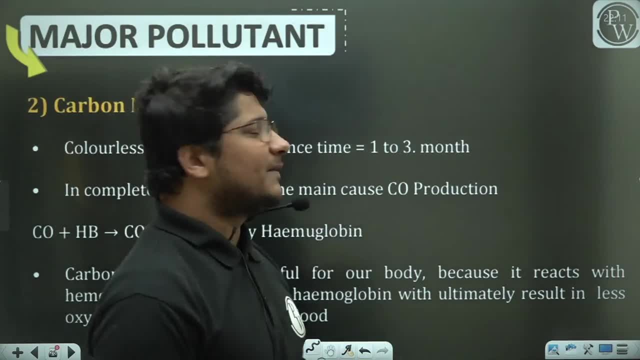 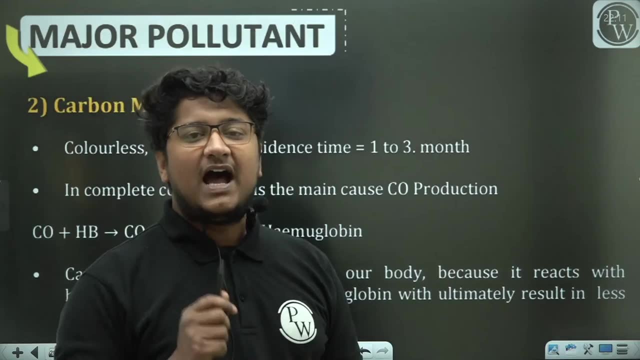 samajhi aga that case up samajhi aga kajapa carbon monoxide about key residence time up key one to three month, hey, or ye, is he ways a jada honey karak be up kelly a jada problem me create content about the key, only key job her may are. 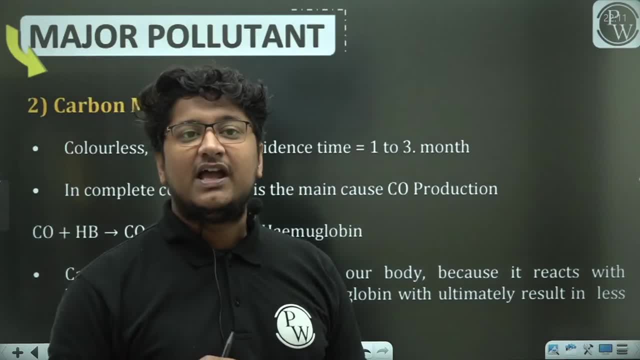 lucky a to do chuti-muti are lucky to palomar and all the budget. a ticket a little close, buddy, I got lucky, lucky a to up. kya bolte hai ki media. nickel low up, nickel, low top, keep jeb. he appogad me. 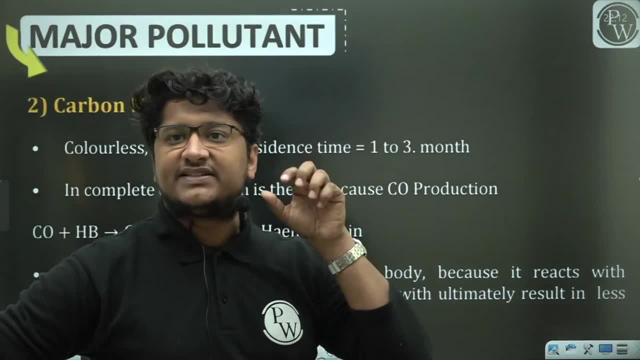 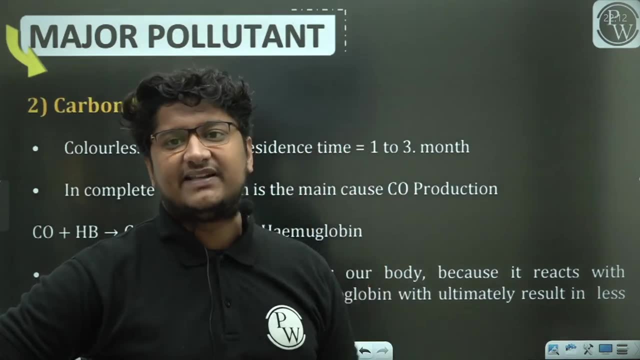 I get you up to a certain limit. the couple oxygen major lega the carbon monoxide. there a fidget sign: oxygen key. comey hoogie jesse apk ox and keep a meho Gavo up to carbon monoxide in la gia to starting my job. talk oxygen hair. 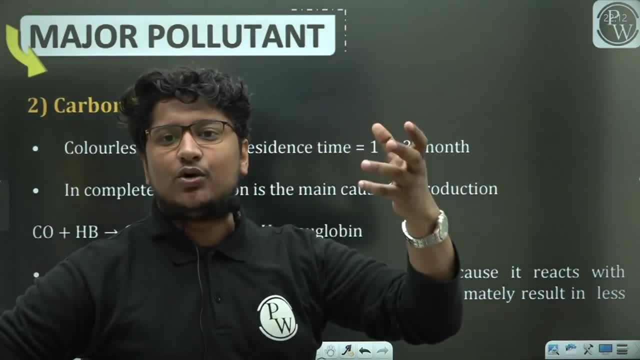 that the tech. carbon dioxide, you say oxygen key coming. who give a carbon monoxide, nickel in a league a or carbon monoxide a grab jada in hail? apne body maker. Lee, like 40% care, I should have taken a look at how I got my body okay I. 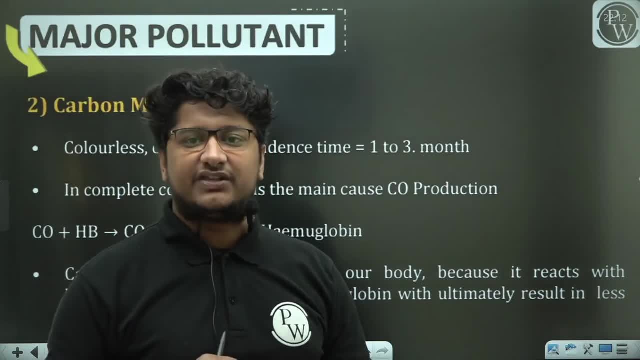 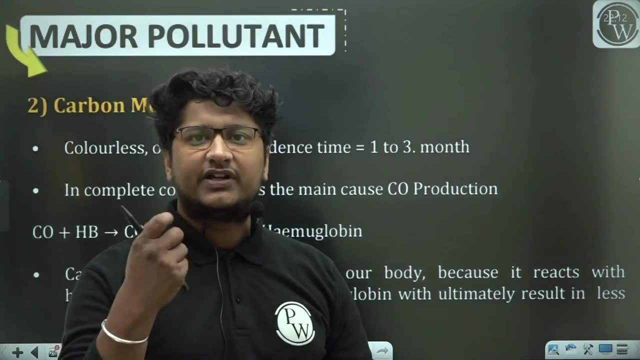 If you have carbon monoxide around you, then your death is certain. there is no problem. you will die easily, Do you understand? So that is a very dangerous death. You suffocate and die. So you will understand what carbon monoxide does. 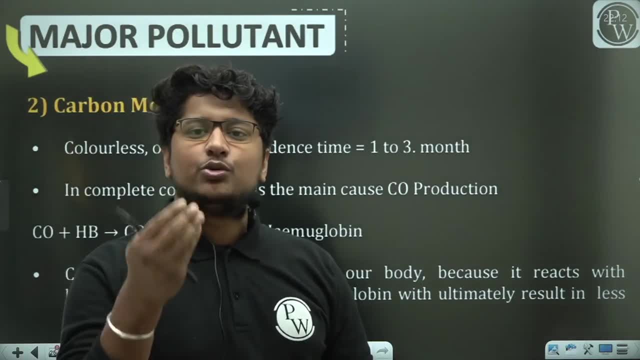 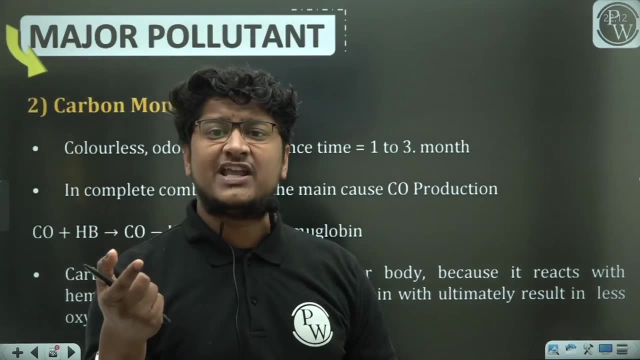 When you inhale carbon monoxide in your body, then what happens is that it is found in the blood. Now, one of your favorite things in the blood is called hemoglobin. What is the function of hemoglobin? It has an oxygen carrying capacity in the blood. 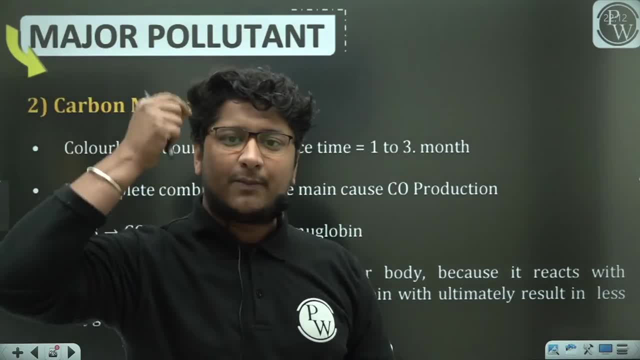 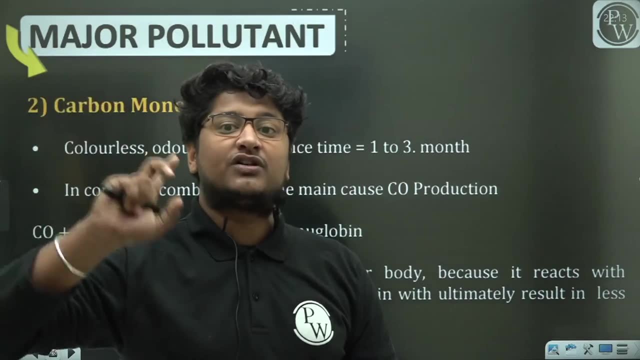 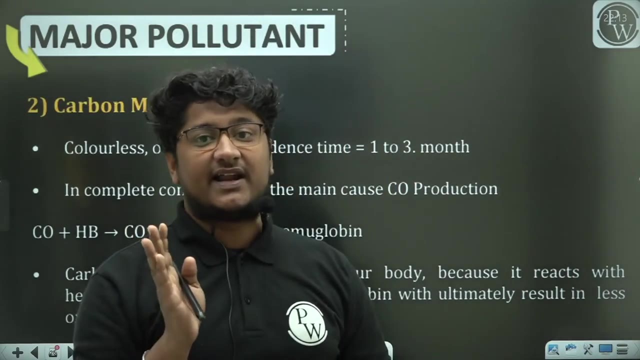 It carries oxygen to every part of your body. Now your hemoglobin is very much in love with carbon monoxide. So if carbon monoxide comes in your blood, then this hemoglobin and carbon monoxide will start doing different things. So carbon monoxide and hemoglobin together will make your carboxyhemoglobin. 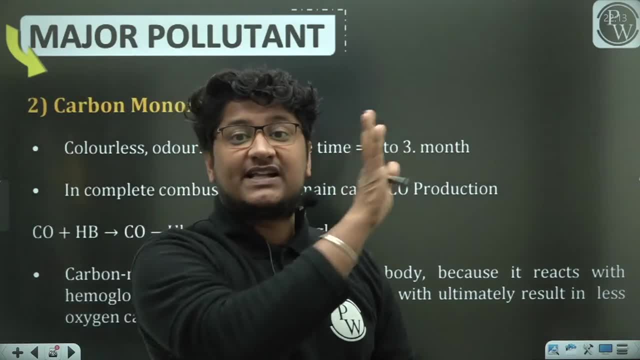 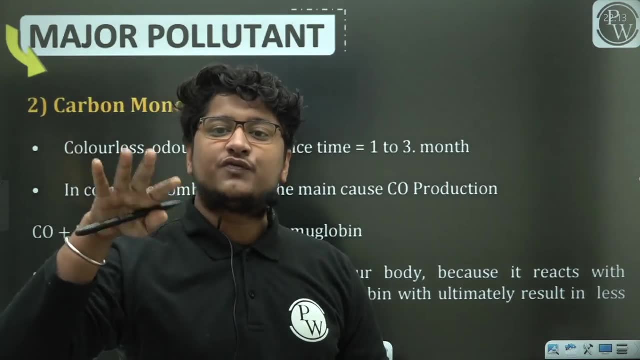 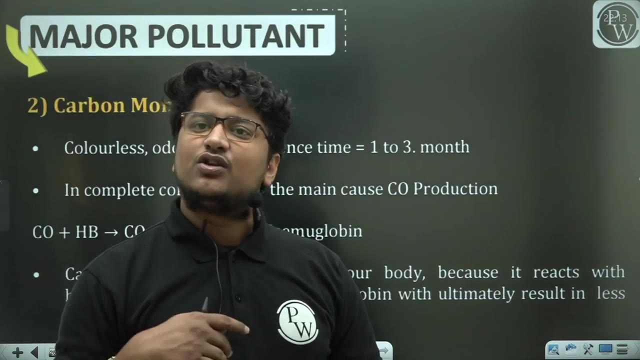 Now, if hemoglobin is present in your blood, then who will do oxygen supply? There is no one to do that, And if this happens to you, if your blood part is exposed to carbon monoxide, then you can die very quickly if you do not get treatment instantly. 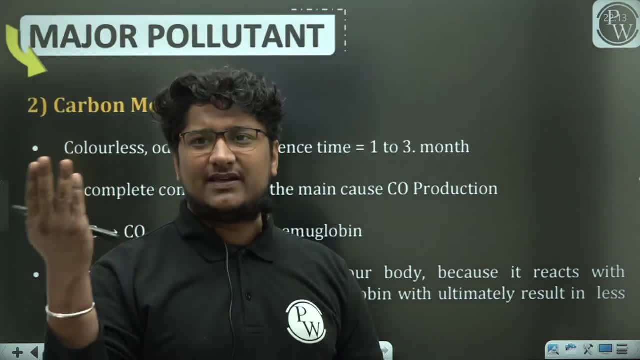 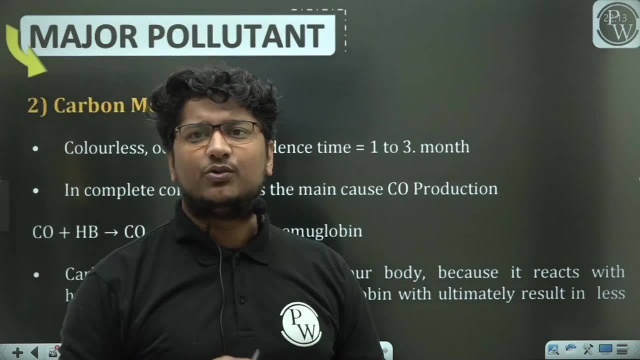 So pay attention to this. That is why you must have seen a very tragic incident in Surat. Many children had jumped from there. That is a very bad incident that happened. It is their fault, We will not come to that, But why did the children have to jump from there? 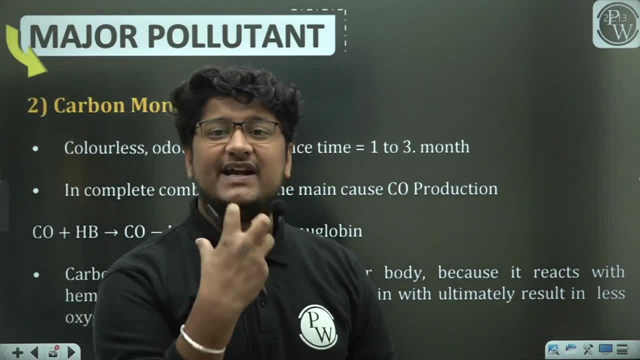 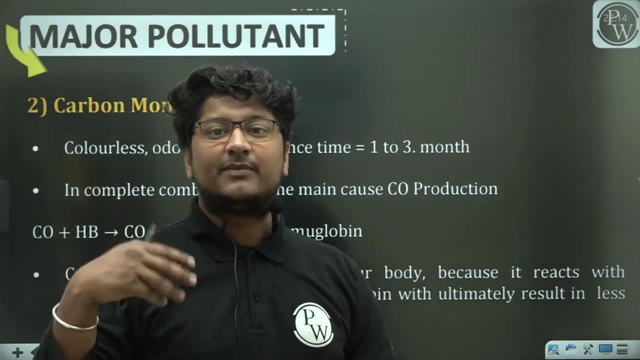 Or why do some people have to jump Because they were inhaling carbon monoxide? If they would have inhaled more carbon monoxide, they would have died anyway, So they would have been forced to jump. So understand this thing. These things were wrong. 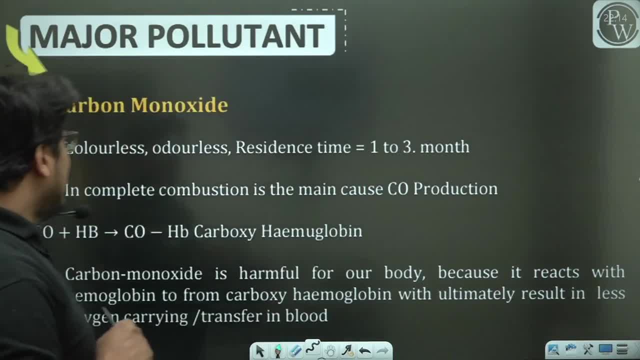 But I will give you an example to relate. So you have understood this thing. Now, how do you analyze carbon monoxide? regarding carbon monoxide, So there is an analyzer for this. It is not mentioned here. That is why I will write it. 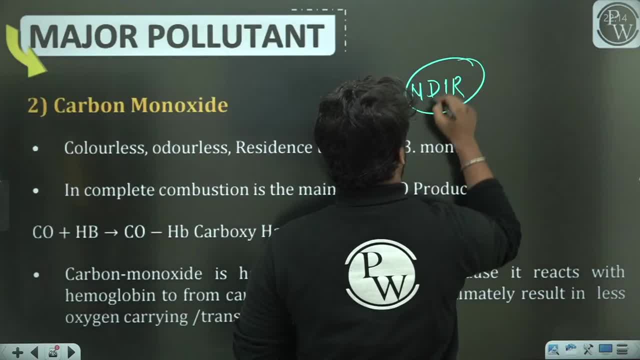 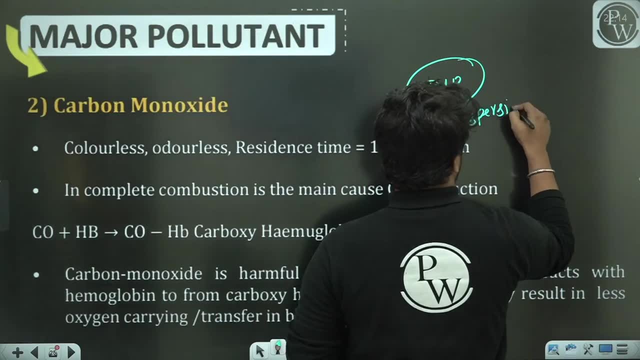 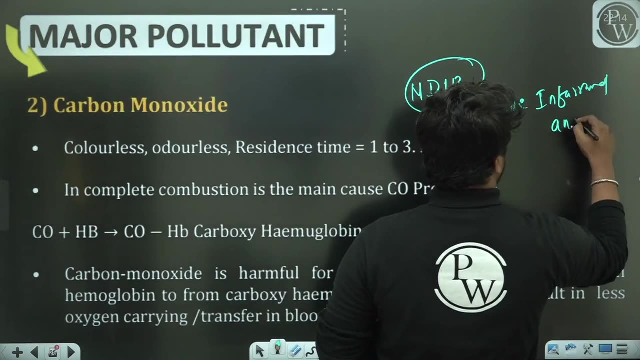 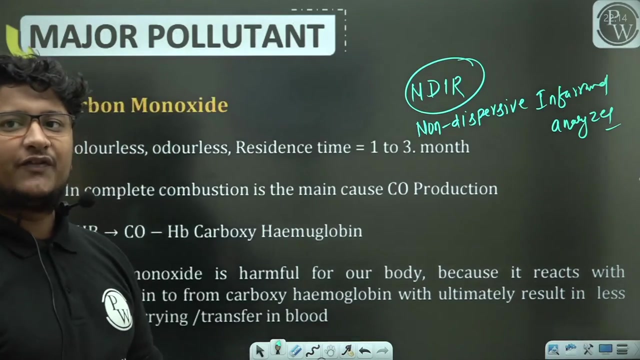 We call it NDIR analyzer In short form. we call it NDIR In full form. we write it as non-dispersive infrared analyzer. Is that clear to all of you? If you will keep your breath in this way, then your face mask is effective. 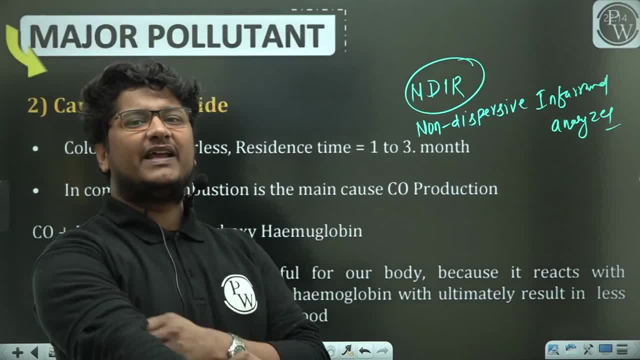 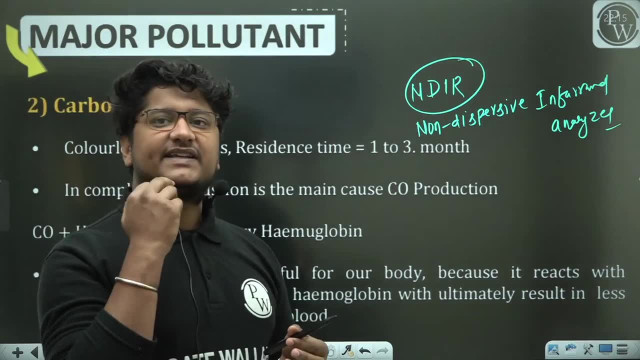 If it is technically made with carbon monoxide, then it will be effective, But carbon monoxide is a very lighter part, So you will be inhaled. You will be inhaled with the air. In such a case, the best solution remains that you should go out. 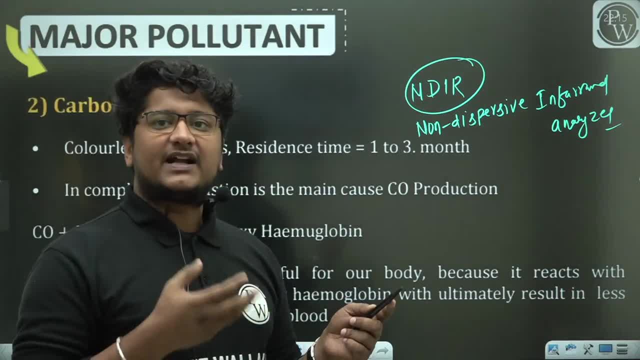 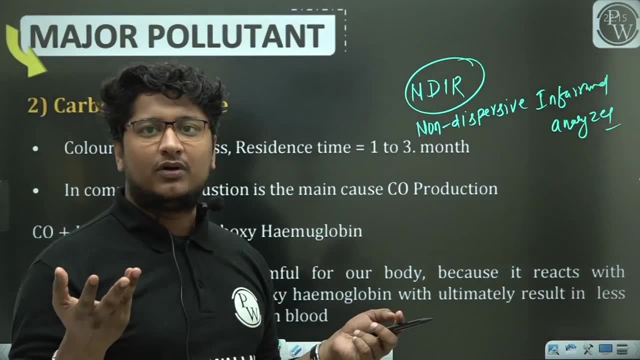 So it is better, Because how long will you keep your breath, Or how long will you keep it? Because there is no oxygen in it. Wherever you will have a problem with carbon monoxide, you do not have oxygen in that air. 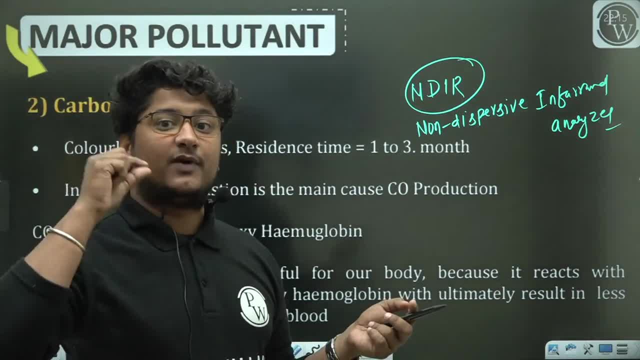 Can you understand this point? This is a different thing. is that you are taking your oxygen part separately in it, then it is a different matter. otherwise you do not have oxygen in that room. then what will happen to you if you put a mask there, or what will happen to you? 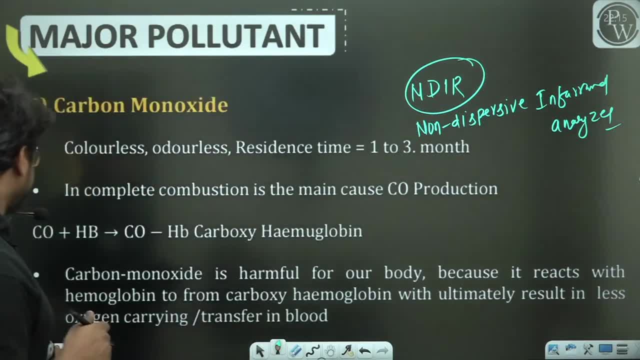 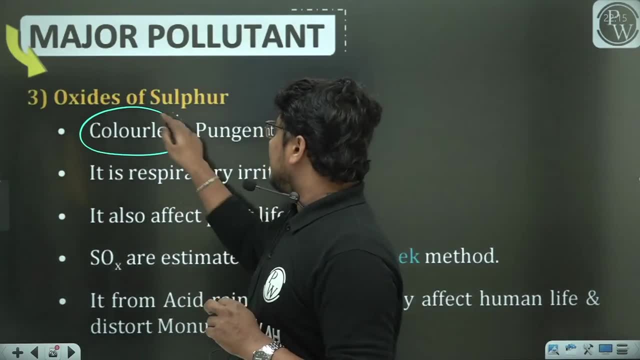 otherwise it is decided. next we talk about oxides of sulfur. now what is in oxides of sulfur? this is also orderless to you. this is also a pungent smell to you. it has a very bad smell, and this also. 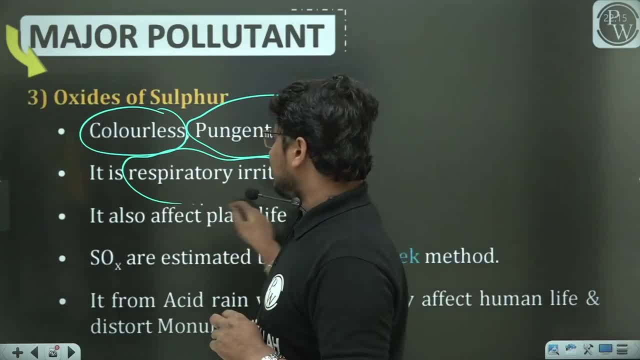 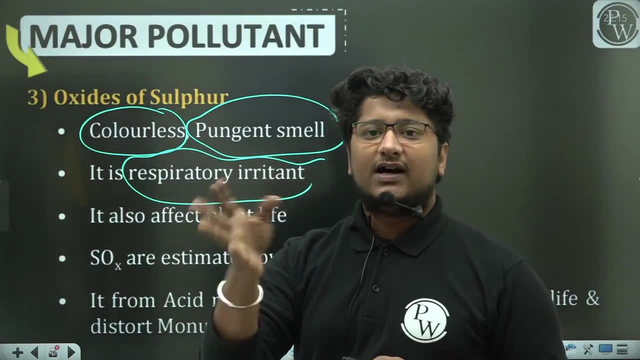 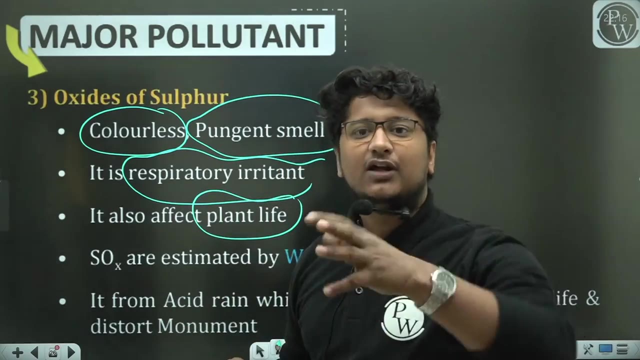 creates many problems for you, like in your respiratory system. it will provide you with irritation here. Apart from this, if you have got socks from H2 o, then you will have AC drain in it. it will affect your plant life too, because if AC rain falls on the plant, it will almost end. 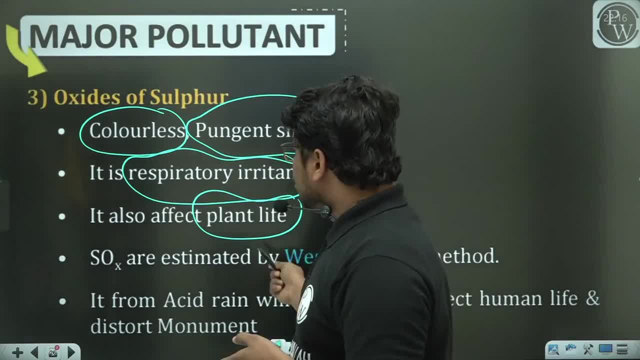 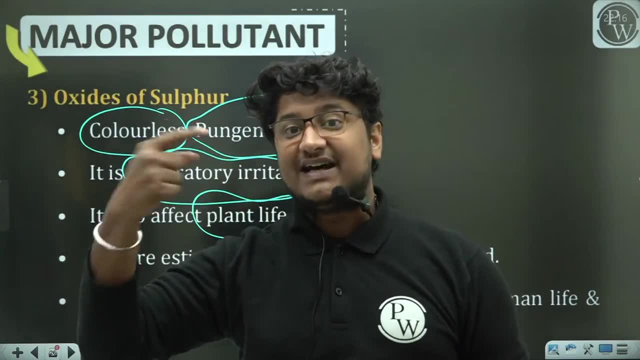 especially for small plants. It is very dangerous. if this AC drain has fallen on you in agriculture land directly, then it will do ACD. if your agriculture land will be more acidic, then productivity will be down in the same case. you will have seen many times that the village area must have been. 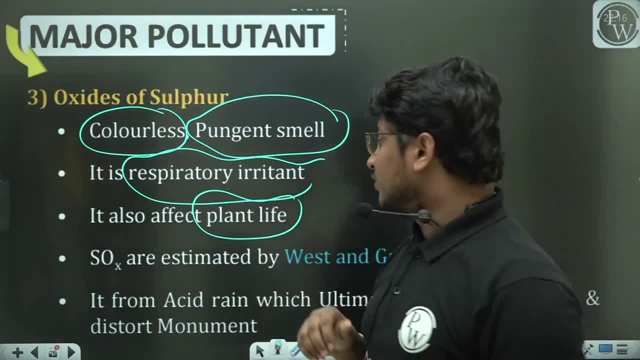 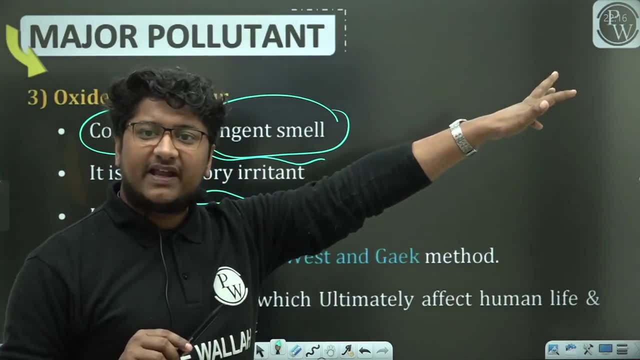 Sometimes they mix lime. So why do they mix it? you must have understood Now. apart from Sox, this is the acid rain. If it falls on the marble body, then it also reacts to you. You all know that if there are more Sox in the atmosphere, 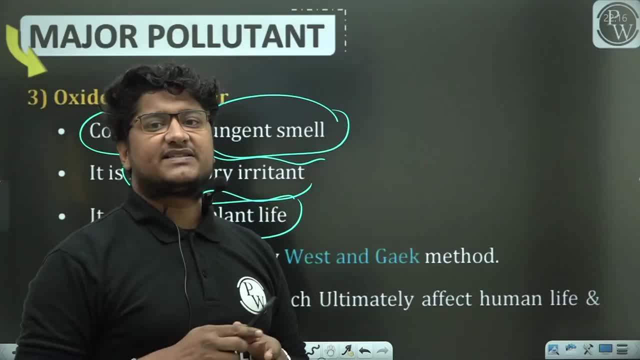 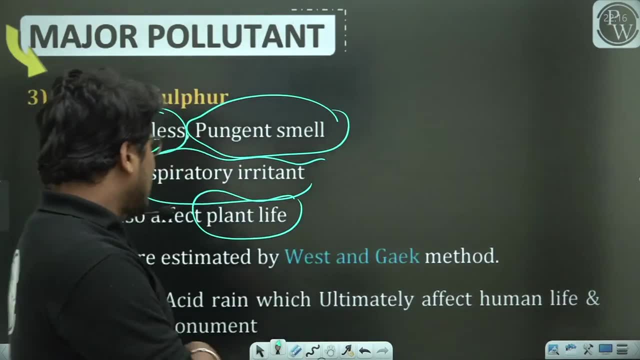 you will see the area of Taj Mahal. around it, the Thamapao plant is taken care of, Because if they are emitting more Sox, then it has an effect on Taj Mahal. Now, what is the method of this? This is the Western Gaik method. 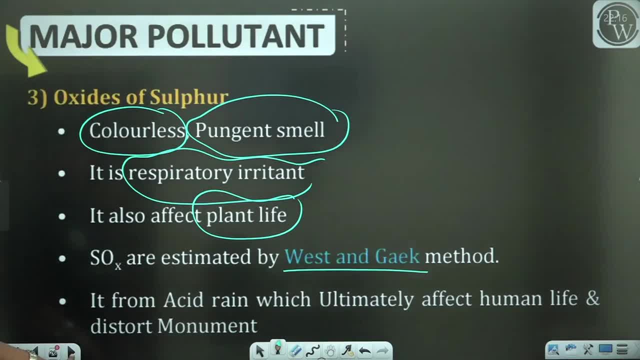 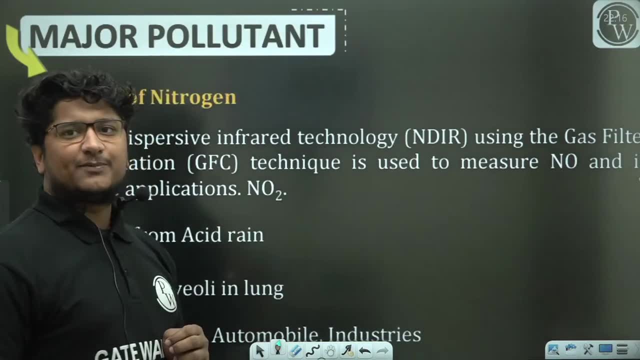 These are the names of the two scientists, So it is a method created by them. There is no need to tell. Next is the Oxides of Nitrogen, NOX. You know that the major sources of NOX are automobile sources. And what does it do? 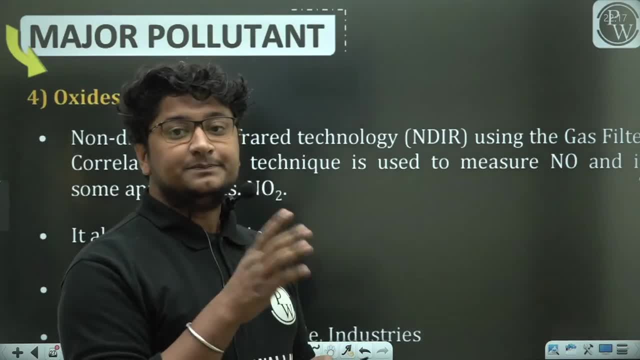 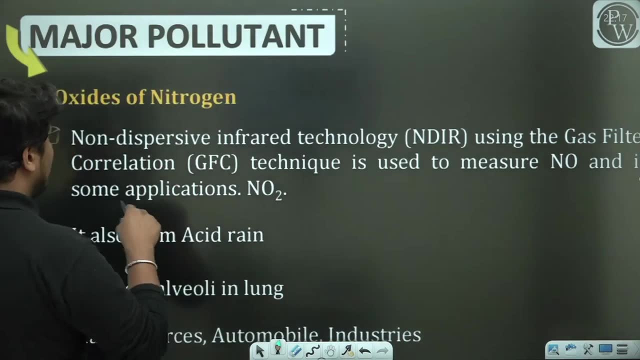 First, it makes you an acid rain, And the second thing it makes you is nothing but photochemical smog. These are the two things that put the greatest effect on you. Now keep in mind that the method of removing this is that you have to. 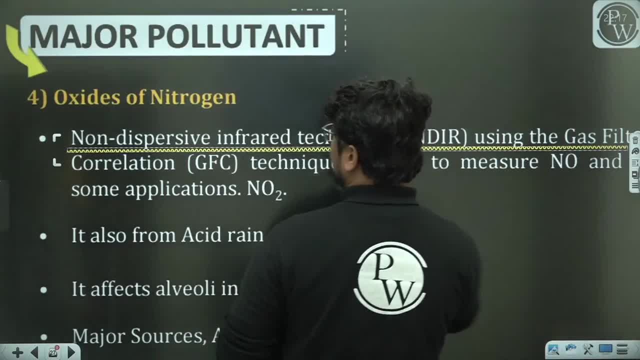 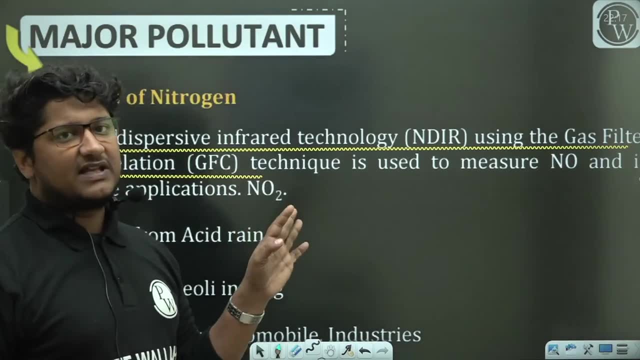 use a non-dispersive infrared technology using gas, while chlorination- GFC you call it. So keep this technique proper in your mind. Sometimes you are asked in match the following: What is the technique? No one is going to ask you anything. 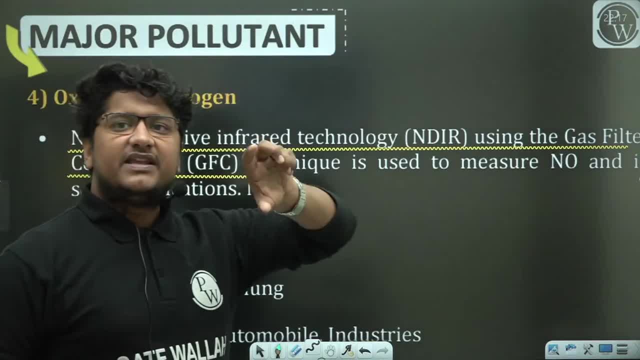 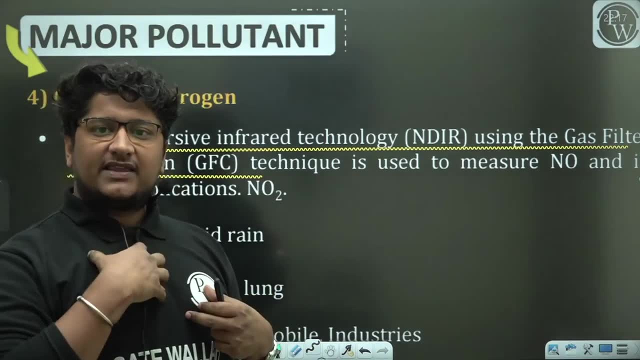 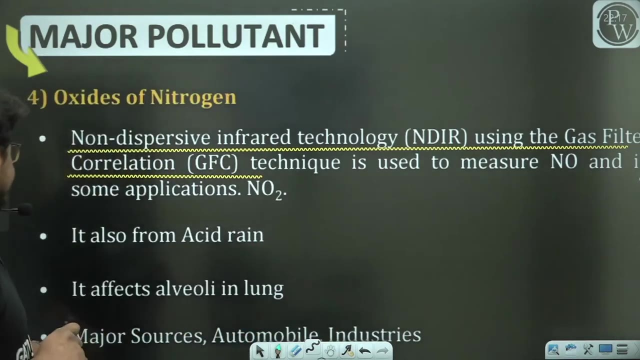 And the problem with NOX is that if it goes in your lung, then what is left in your lung Alveoli? What does it do When you breathe? it traps oxygen from the air. It spoils it. So keep this in mind. 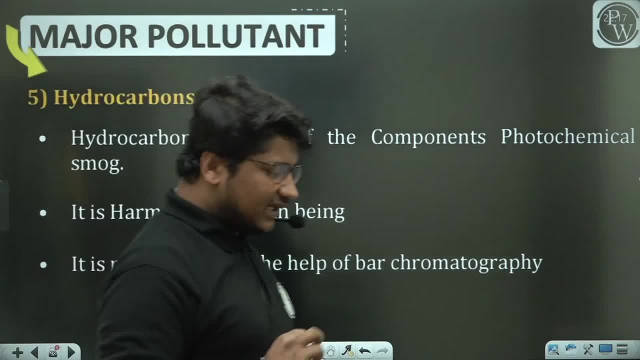 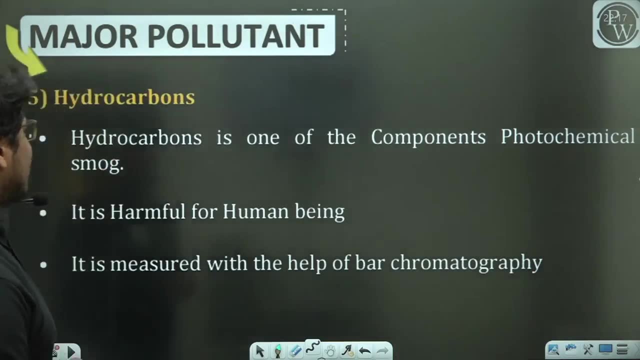 Next comes hydrocarbons. Now, what is hydrocarbons? It spoils you. You know the source. There are many sources of hydrocarbons. The one you measure you generally do it with gas chromatography. You have not seen gas chromatography yet. 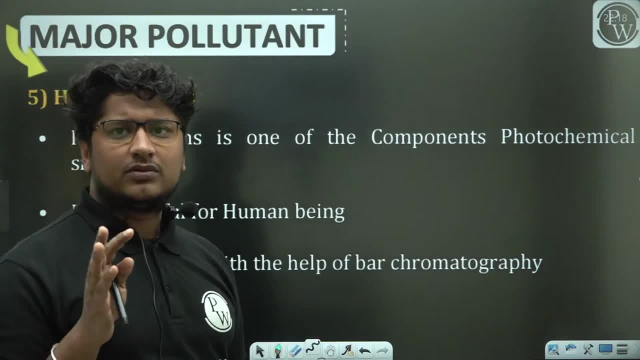 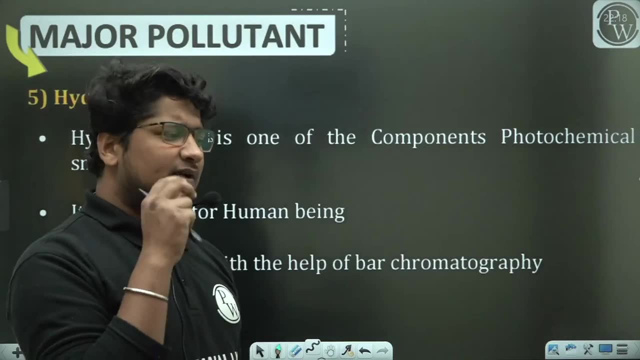 You will work on gas chromatography in the master. Have you heard of chromatography technique? Have you heard about chromatography technique Anyone? You will do it in the masters. I am giving you a general idea. There is no need to know. 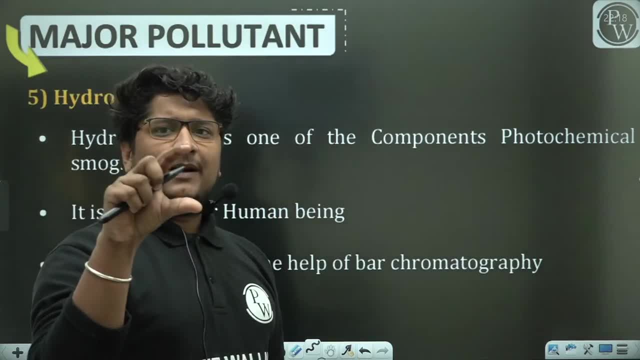 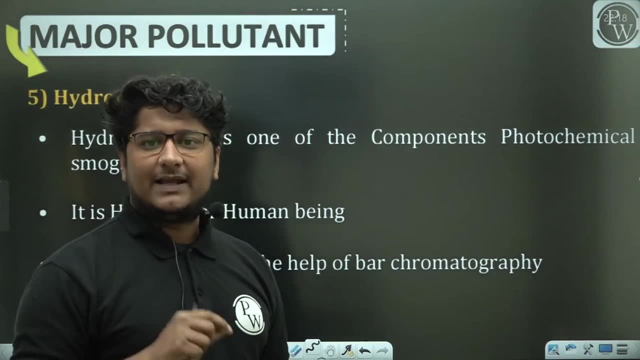 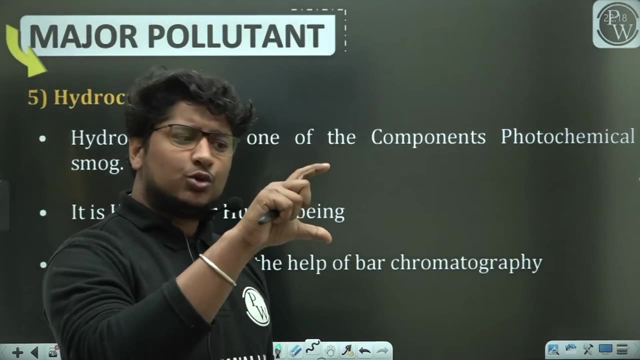 For your extra knowledge When you work on chromatography technique. then what is in it? Every organic compound has a particular temperature on which it comes in the form of vapor. It is not color matching. It is not color matching. So what will it be? 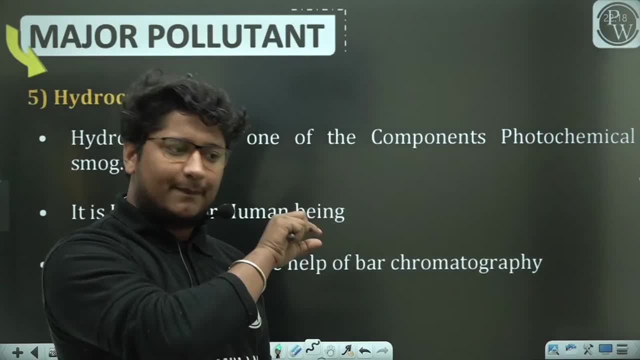 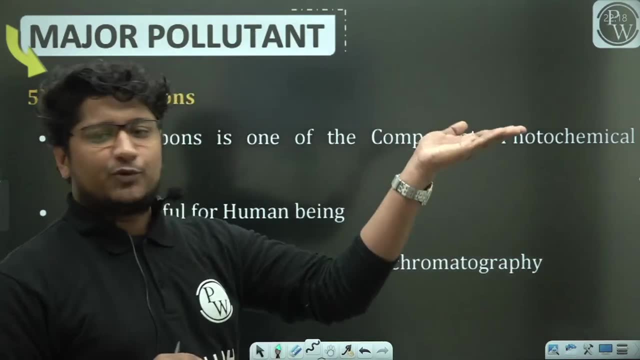 When you put input from one side, your fumes are burning. You put input In that way. you will be hit at different times, Different temperature, The whole curve will keep moving from your face And you will see peak at different times. 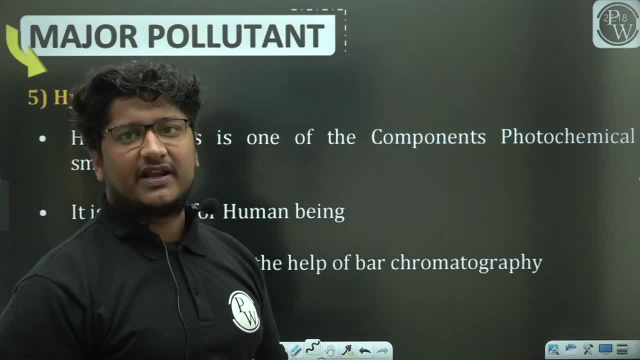 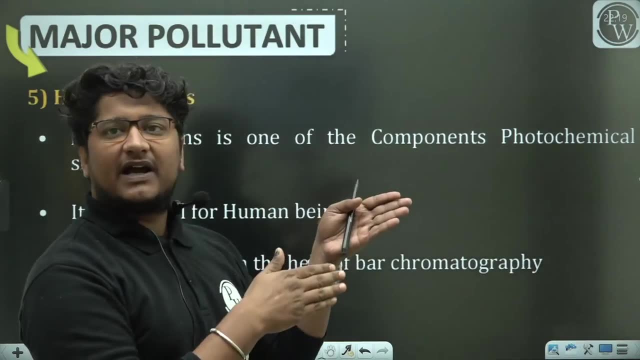 And then you can calculate it there. How much is its concentration? So what is this technique? Different time of vapor change Different time. For example, if you have toluene in hydrocarbons, It will come in gases at different times. 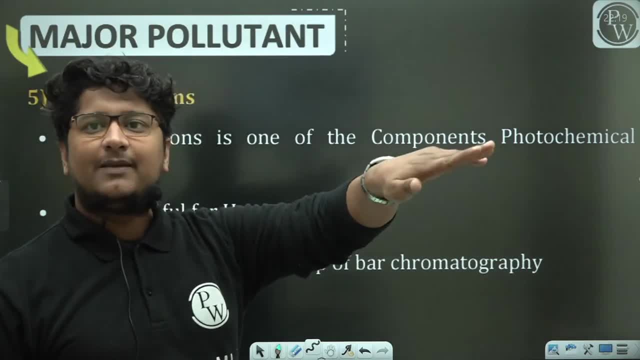 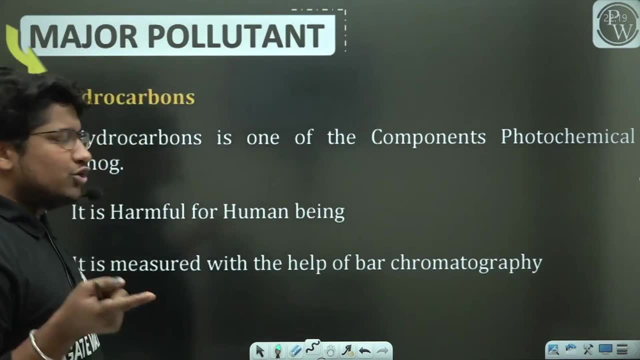 If you talk about formaldehyde, it will come at different times. This is chromatography technique. You will know it in more detail. I just gave you a basic idea. So chromatography technique in the sense if you talk about gas, chromatography. 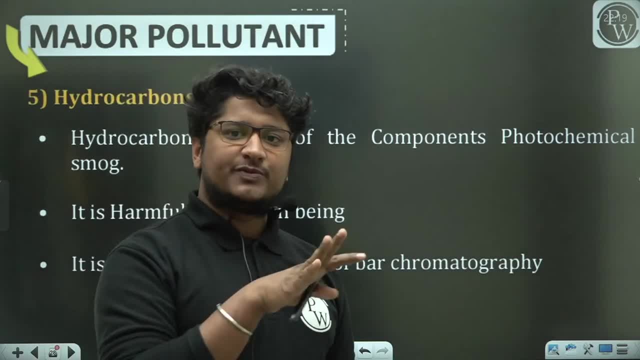 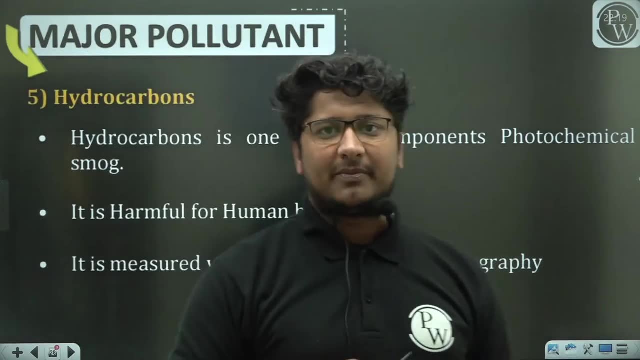 then it will be the same. If you work on liquid HPLC, then it will be the same. So this hydrocarbons, you can find out from GC, There is no problem. You can find out from gas chromatography. Now let's talk about 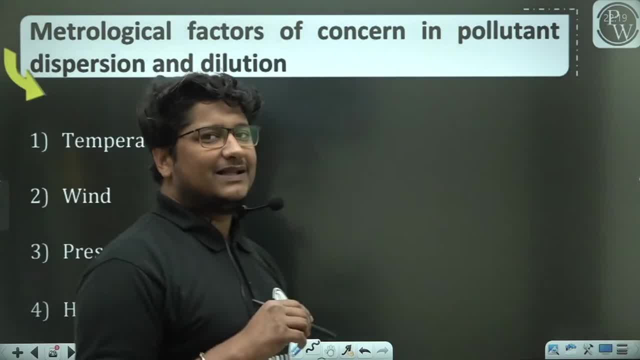 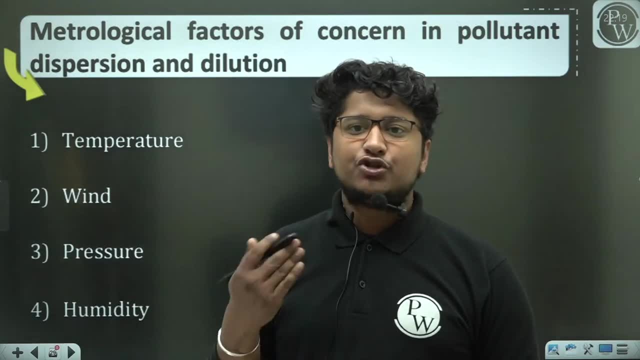 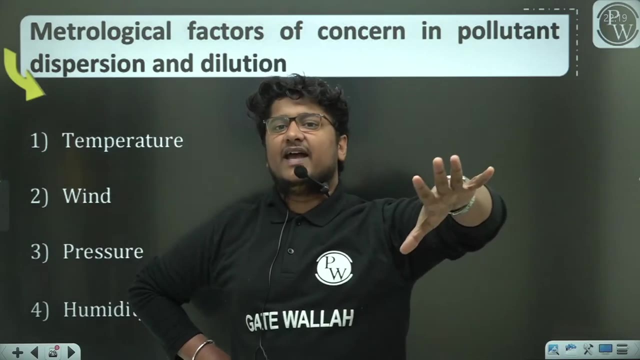 next is your metallurgical factors. Now, whatever we were talking about in this video, one thing is sure: that you will get pollutant. You can't close the industry completely, Because industry is useful to you. So when we assume that pollutant is sure to come out, 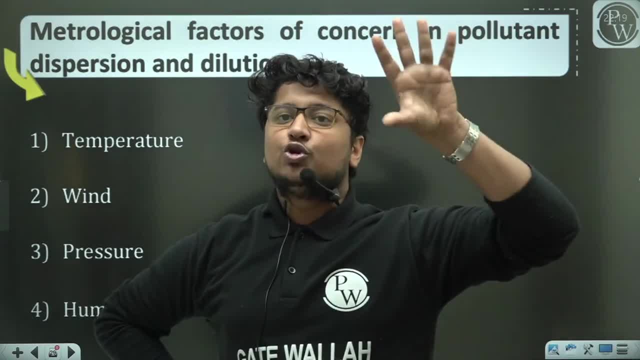 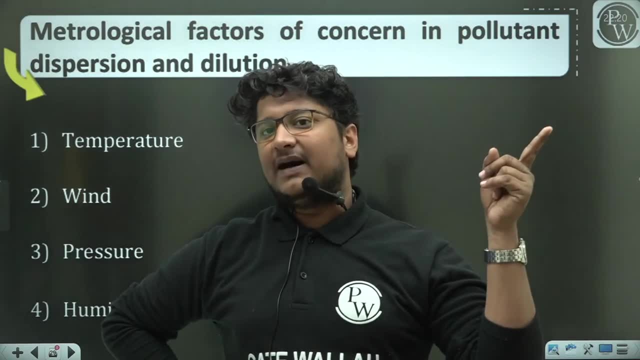 So now, sir, tell me, if pollutant is coming out, then how can you disperse and dilute it better? Now, these are two words about which I talked to you yesterday. So dispersion and dilution are very basic things that you have to understand. 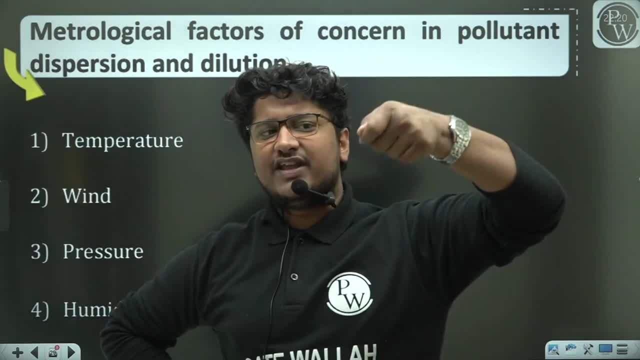 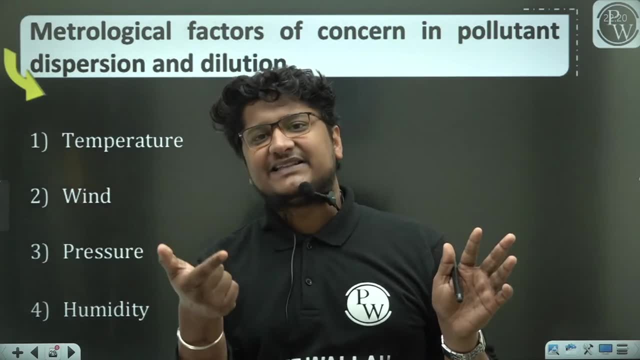 I told you that there is a coffee. You put one spoon of sugar in the coffee. Now you leave it. What happens to the bottom part? It becomes sweet automatically. That is nothing but dispersion. And if it is coming from bottom to top, 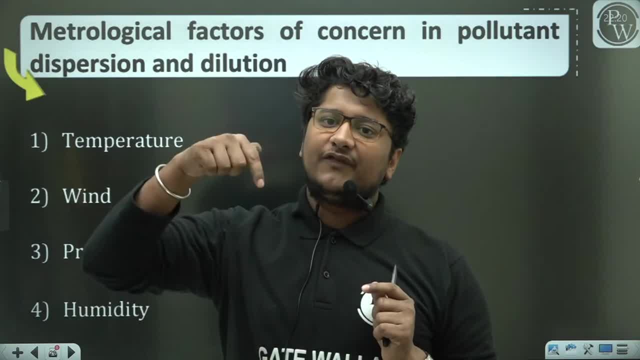 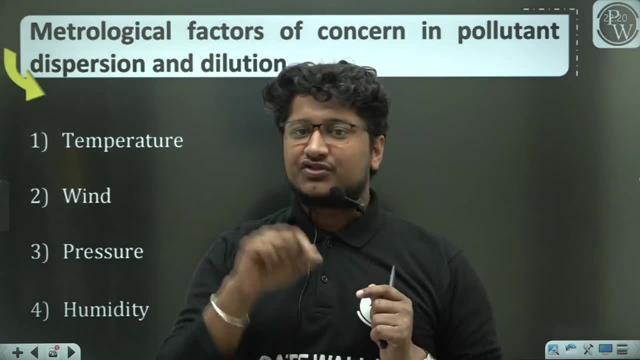 that is nothing but the dispersion. You have not done any mixing. Now, in the same coffee glass, you mix up from spoon to spoon. Now that is dilution. There is a very thin line difference between dilution and dispersion, So you have to understand it clearly. 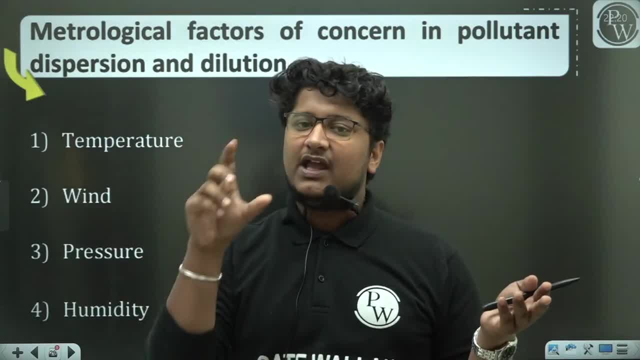 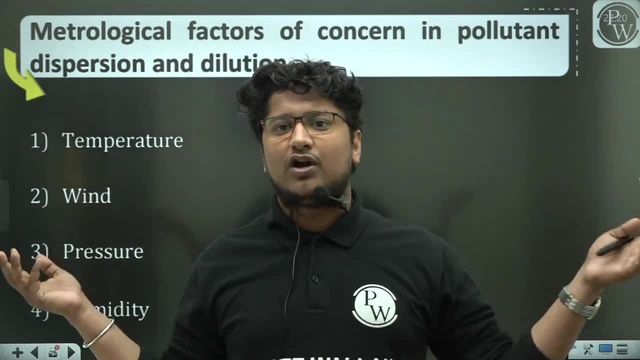 In the second example. I told you that, for example, you are doing that there is air in the room In that in one corner someone put perfume And just in the opposite corner you are getting its smell. or in some other corner you are getting its smell. 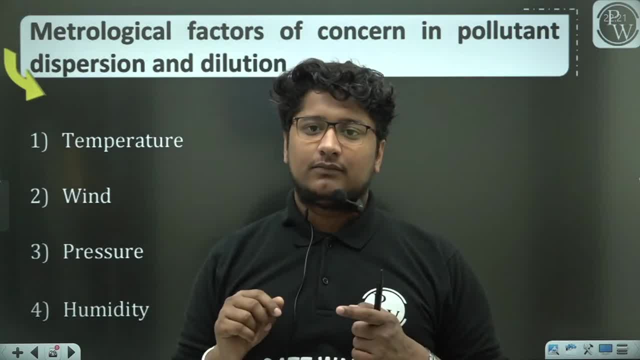 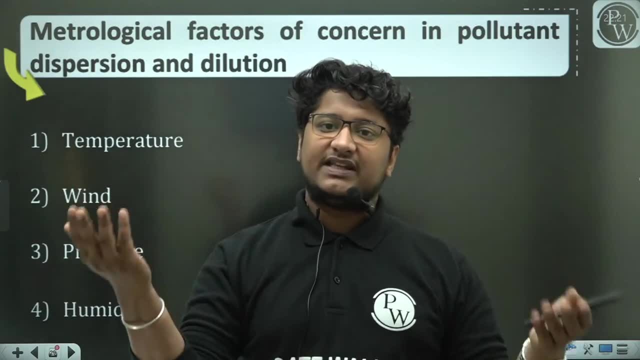 That is dispersion. Now you put the same perfume in the room and you started the fan. Now the mixing that happened, that is the dilution. So the concentration is decreasing in both the dispersion and the dilution. So, whether it is dispersion or dilution, 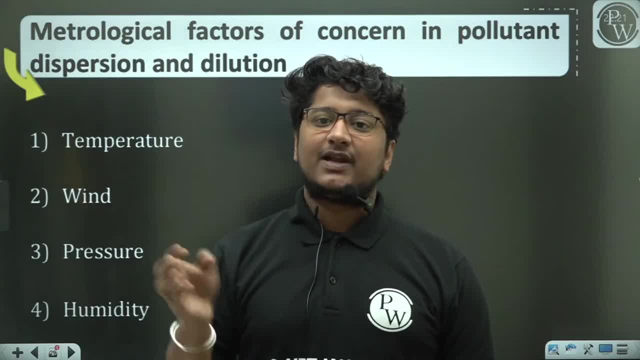 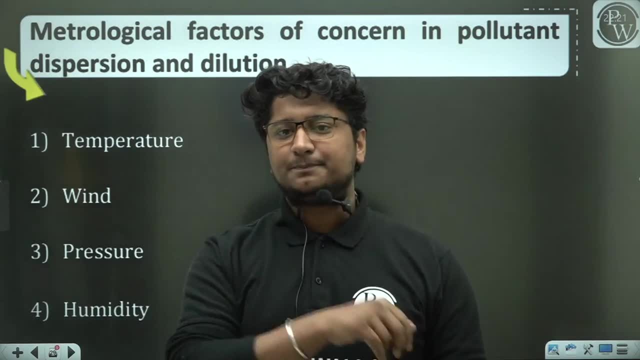 the concentration of pollutant is decreasing in both, And if in your atmosphere dispersion and dilution of pollutant is happening well, then you see, there is a lot of benefit for us. For your example, if you talk about Bhopal gas tragedy, So in Bhopal gas tragedy, 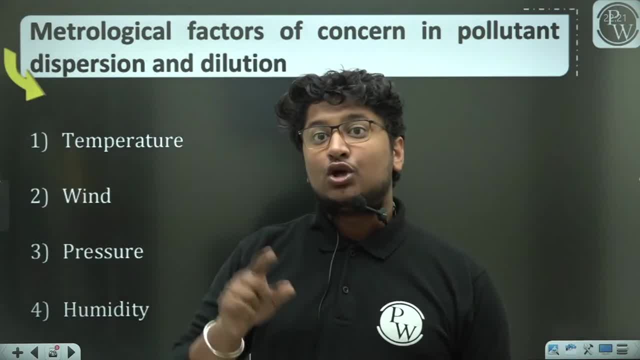 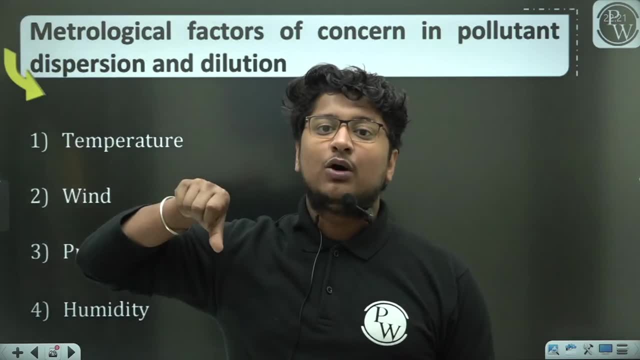 the gas leak happened somewhere in the night and its effect was shown more in the morning time, Because in the morning time there is inversion, which you will read further. So if there was no inversion in the morning time, then maybe so many people would not have died. 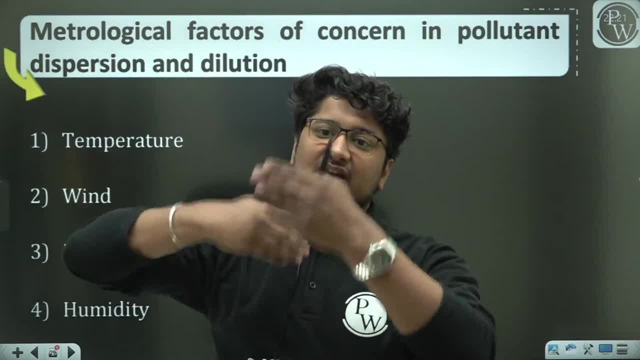 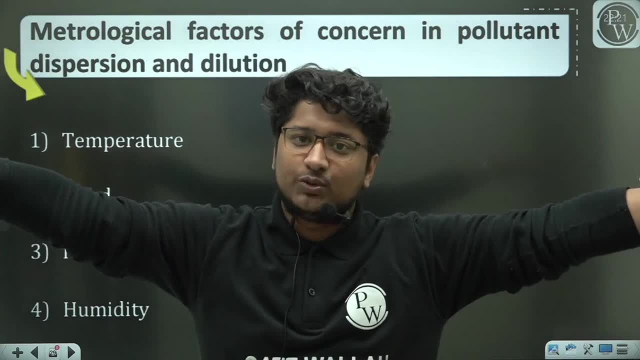 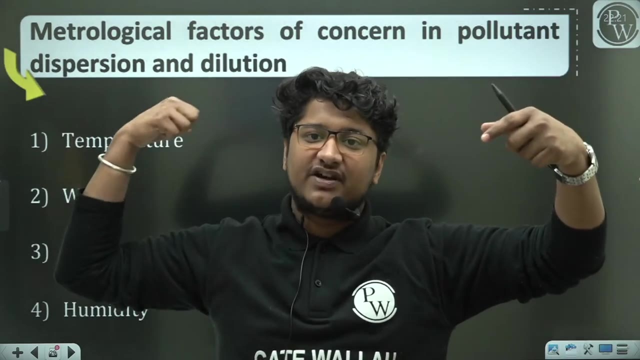 So if pollutant dispersion and dilution had happened well, vertically, then those gases would not have spread more urgently, And if it would not spread more urgently, then less people would have died. So dispersion and dilution is very important. If in such a condition 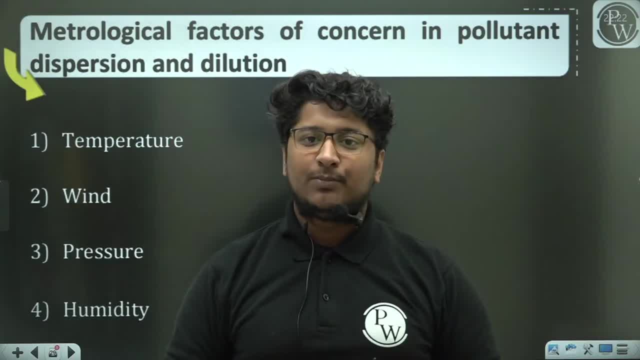 like in inversion condition. if any industry releases its pollutant in such a condition, then there will be no dispersion and dilution and it will come in direct exposure. that is not good. So to understand dispersion and dilution, why did it come in our syllabus? 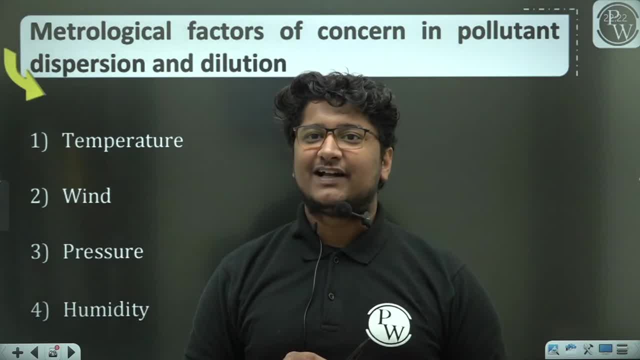 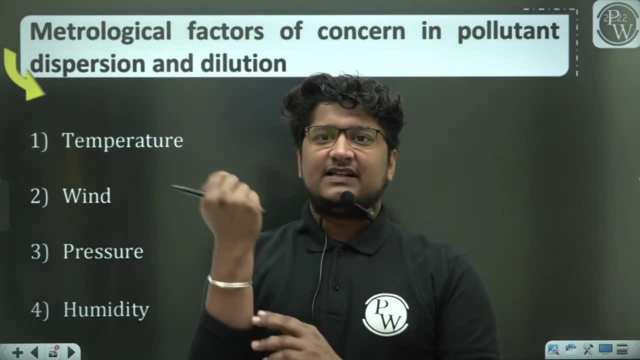 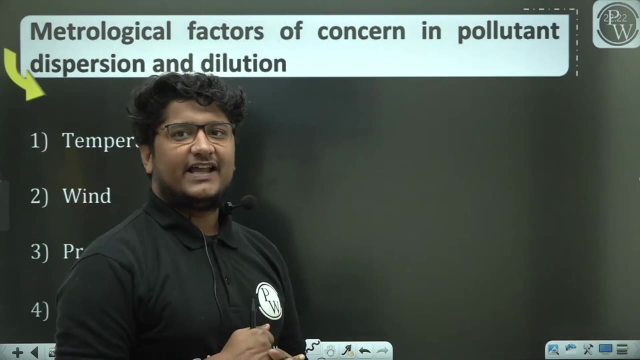 that gas leak is called methyl isosinide. Can anyone tell the name of the company? No one will tell the name of the company. Don't search google, Let's see if anyone remembers or not. Company name Anybody? Ok, So there are four factors. 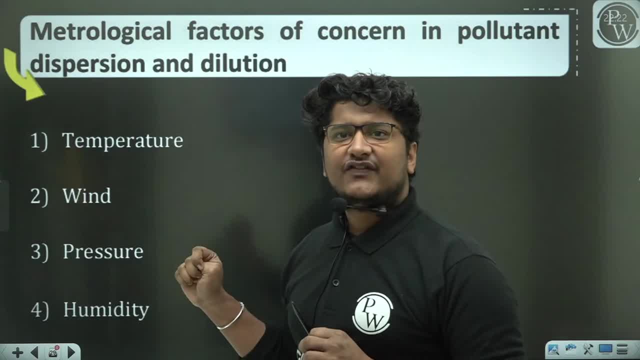 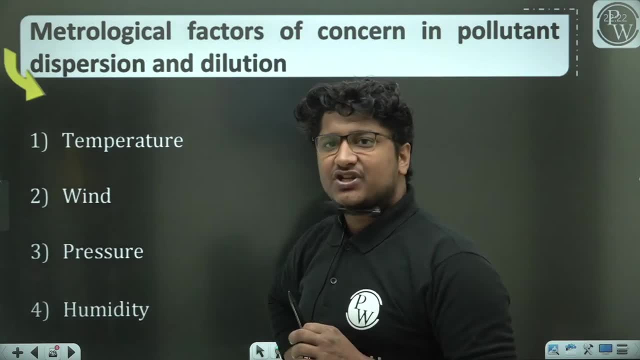 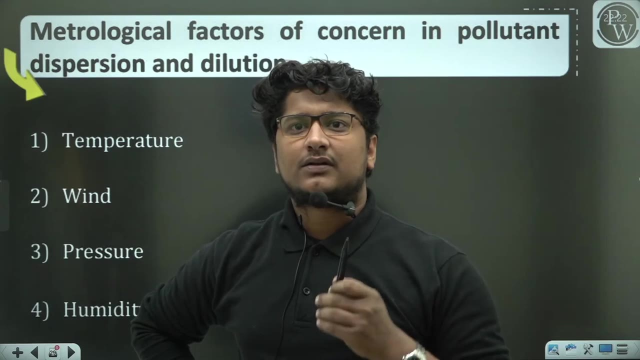 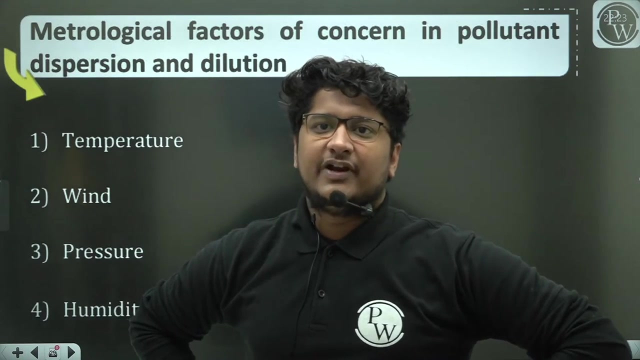 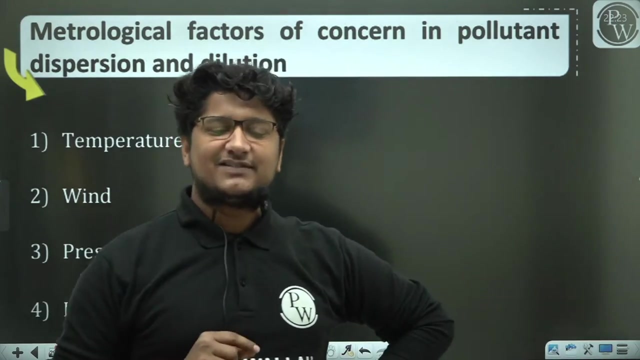 that actually affect dispersion and dilution directly. Pharma company- Company name was not pharma. There are four factors, basically: temperature, wind pressure and humidity. Ok, Ok, Union Carbide Very good. But when the incident happened few days later, they changed the name of the company. 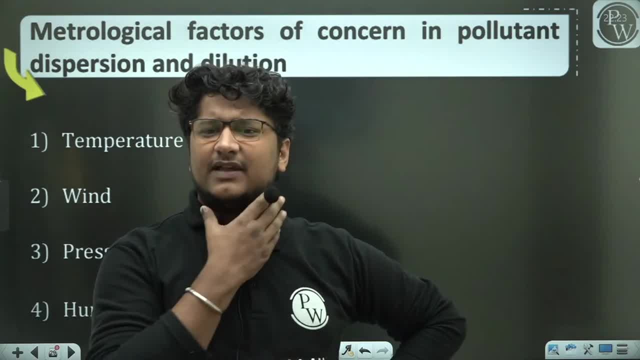 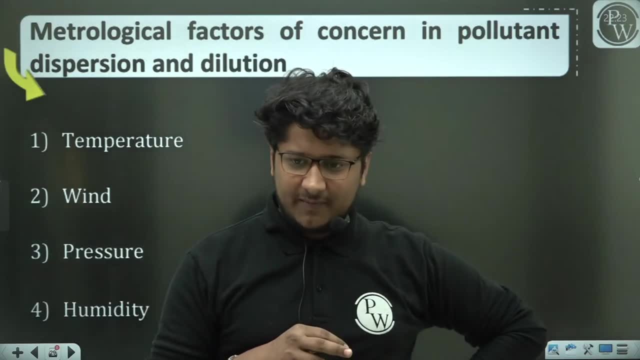 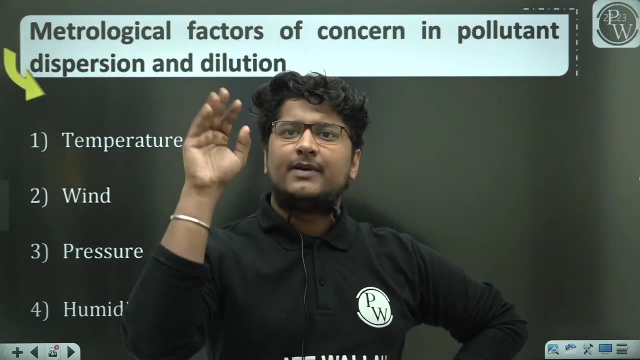 People use that company today Every day. Is it every day or every day? It is every day? The battery that comes. Is it in my house Every day the battery comes. So now your Union Carbide factory has been changed In foreign. it is still called Union Carbide. 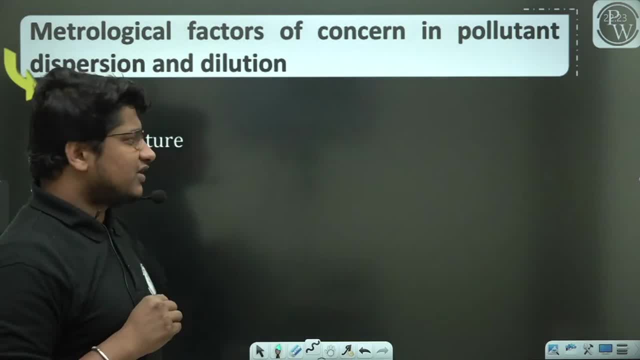 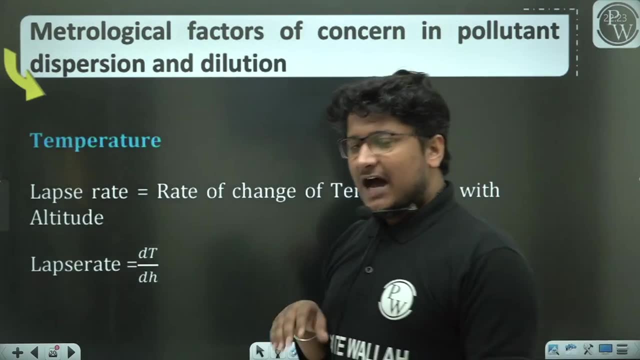 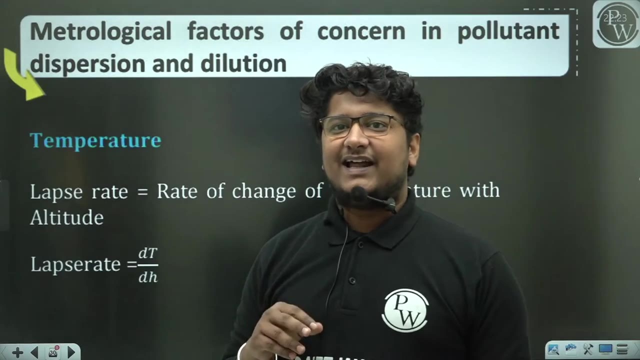 But in India its name has become every day. Ok, So let's start First. let's understand one by one. First, if we talk about the factor, then Temperature. Now, to understand the temperature factor, To understand the temperature factor- Hey, Akshay adds useless, Just for your general knowledge. 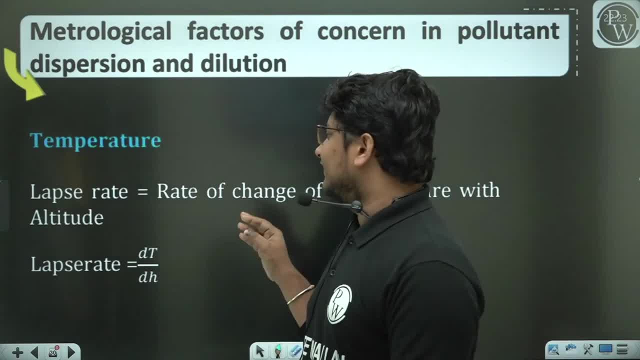 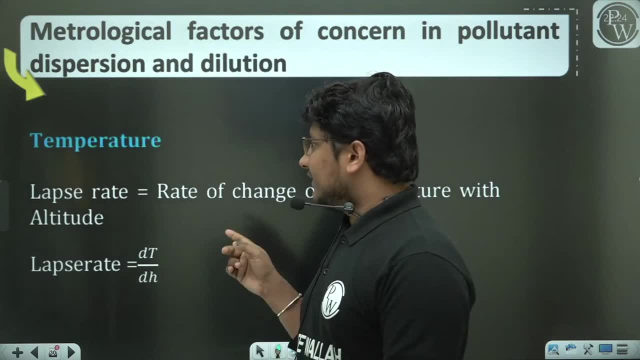 I told you. Akshay adds that: what does he do, Bicot? all this? Where do you spend your time? Do you watch more social media? Come here, Come to the story. You get lost from the story When I am talking about the temperature. 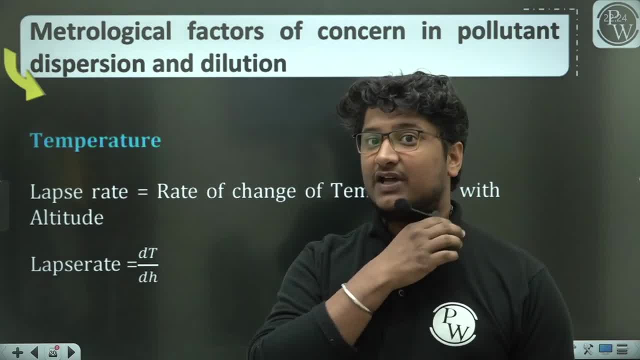 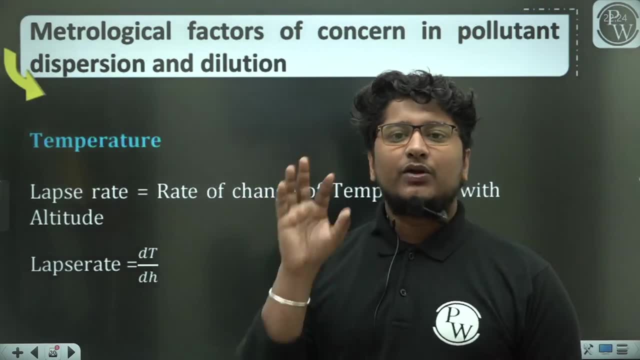 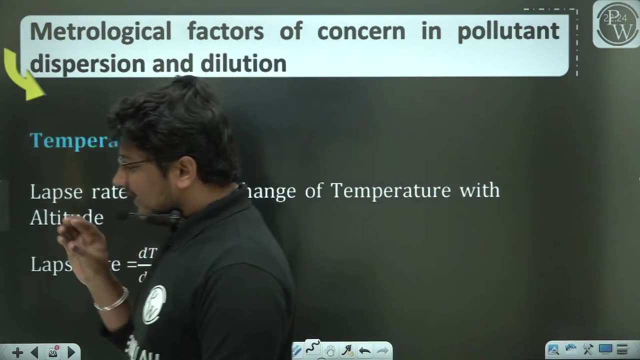 Temperature is a very big factor. Listen carefully Here. one thing is important: If you miss, then you will be in loss. If I talk about the temperature. So what is in the temperature? See one factor Which you have to keep in your mind: So that is your term, That is your lapse rate. 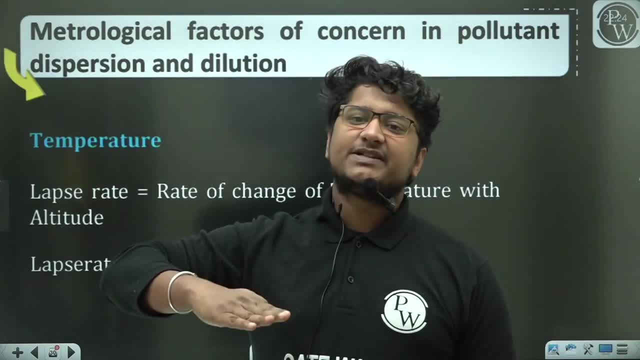 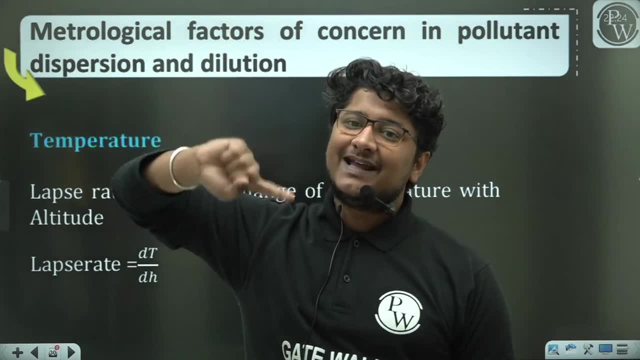 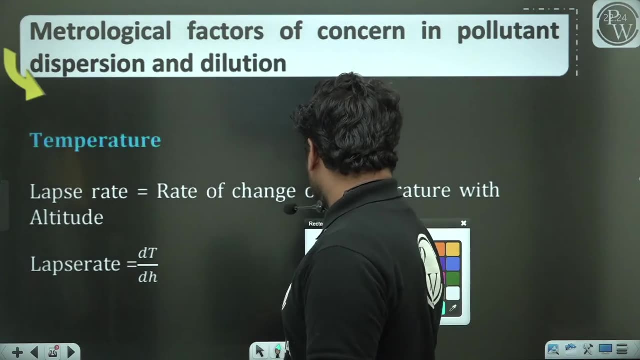 What is the lapse rate? Sir, if we are talking about the troposphere, You said that when we increase the altitude Means we go above the ground level With the temperature, With the altitude. So this change in temperature With the altitude, What we call it Lapse rate. 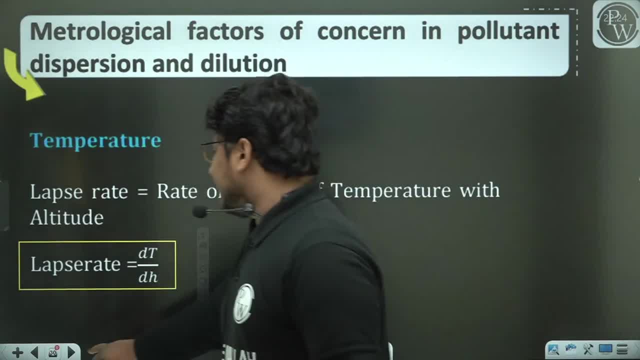 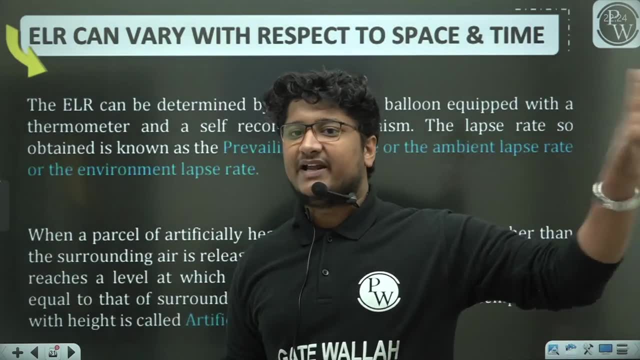 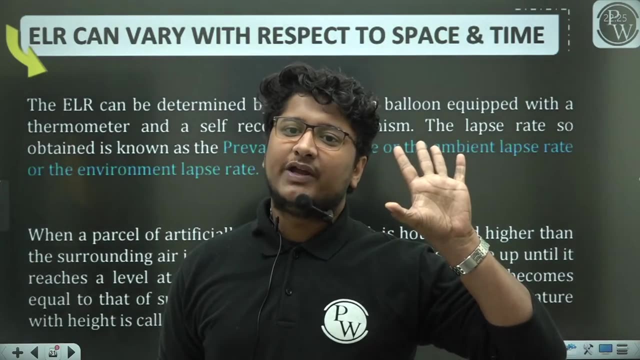 So what is the lapse rate? It is written here. I will put it in the box for you. That is DT upon DH. That is DT upon DH. Now, this is the game of the lapse rate, Everything. Two lapse rates are found in the corner, Which is called ELR. 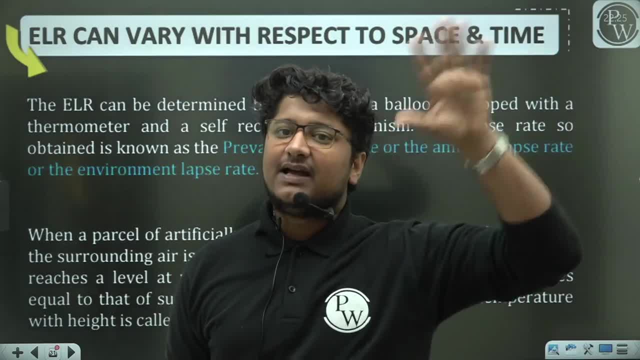 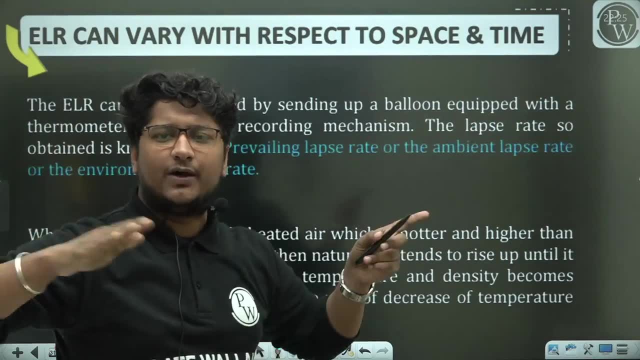 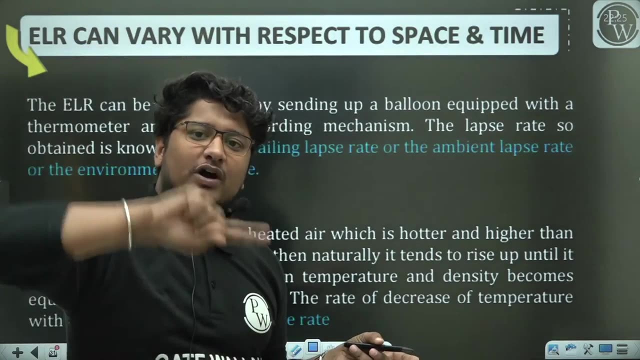 Which is called environmental lapse rate Or ambient lapse rate Or prevailing lapse rate. What happens is simple: In any area, In any particular time or location, When you go up, You find a change in temperature with the altitude. So if you calculate that, If you calculate DT upon DH, 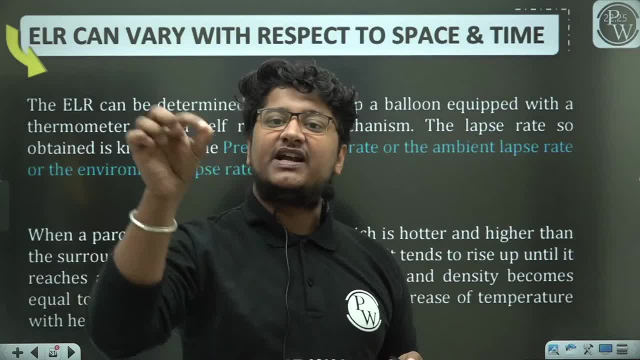 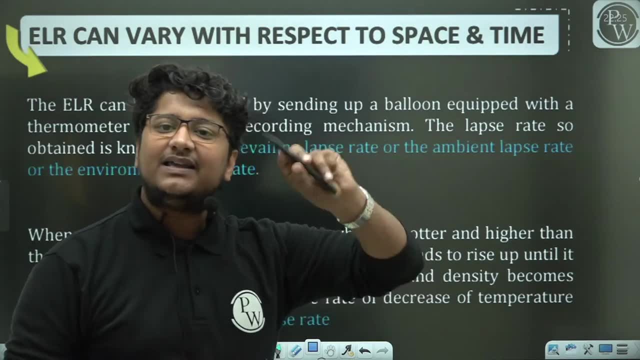 That we call as ambient lapse rate, Or environmental lapse rate, Or you will call it prevailing lapse rate. Now, if I ask you, What is ELR? Will it be constant Or will it change according to time and distance? Will it change according to time and location? 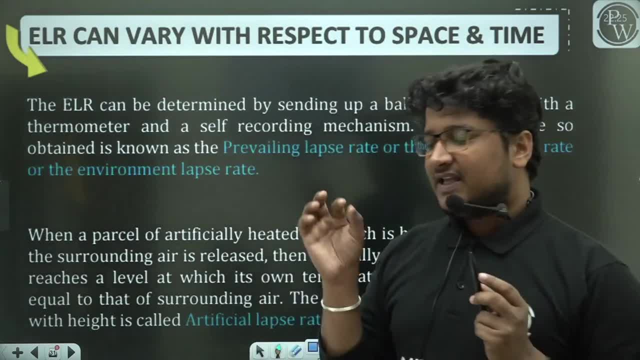 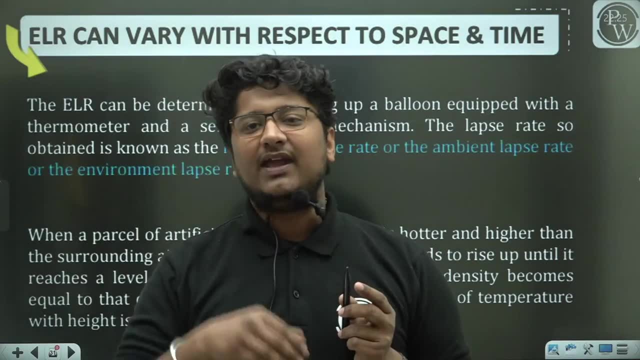 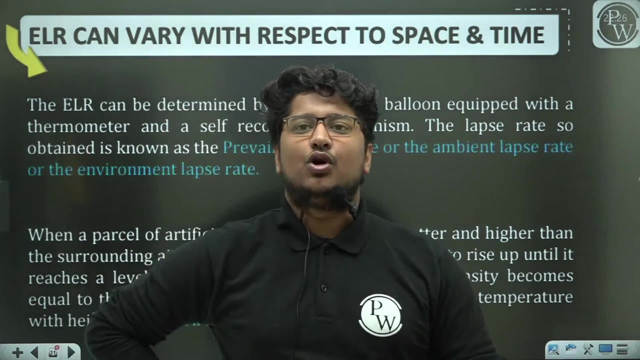 Those who understand ELR, They will reply quickly. If I talk about ELR- Environmental lapse rate, Will it change according to location and time? Will it remain the same? I am asking this to all of you. I am asking this to all of you. Listen carefully and reply. 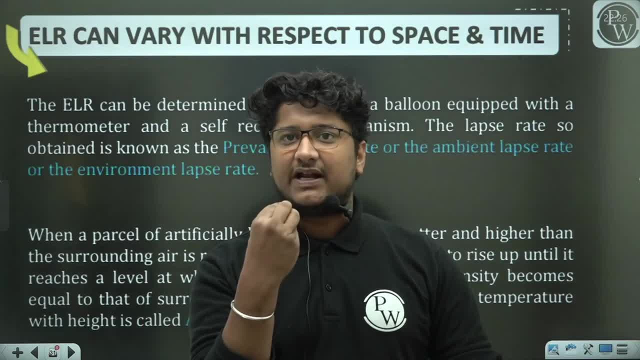 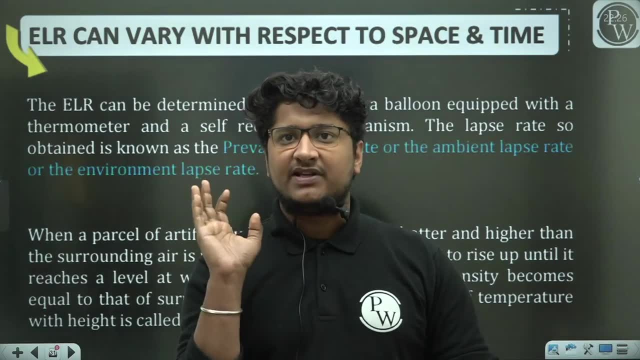 Here PDF is going backwards. You have to pay attention to my words. If you go up and down even once, Then I am not going to repeat further. I am frankly saying I am not going to repeat it Because today syllabus is big So I don't have time to repeat. 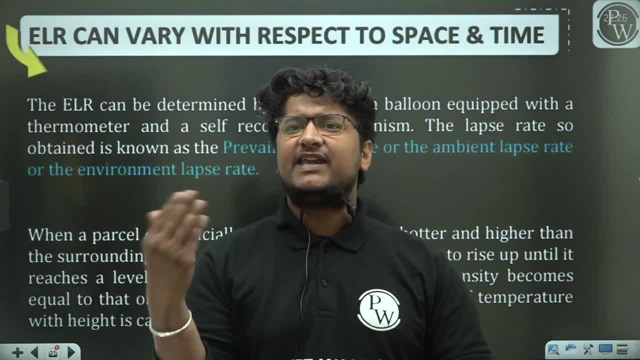 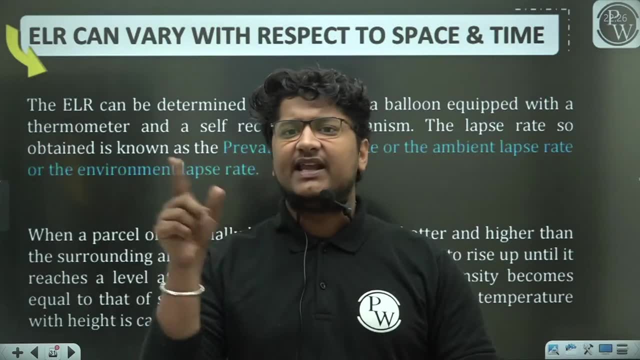 It will change. It is obvious that If we see in the morning at the same time, Then we will get different. If we see in the evening, then we will get different. If we see Kolkata, then we will get different. If we see Delhi, then we will get different. 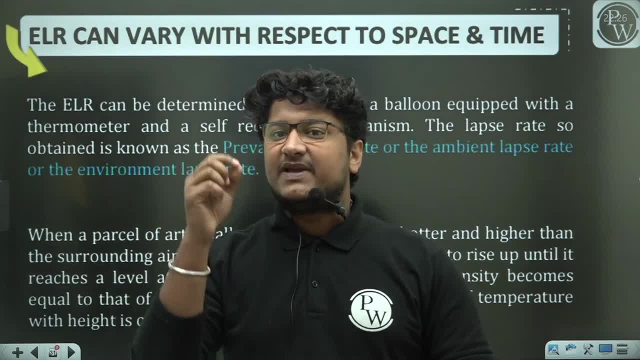 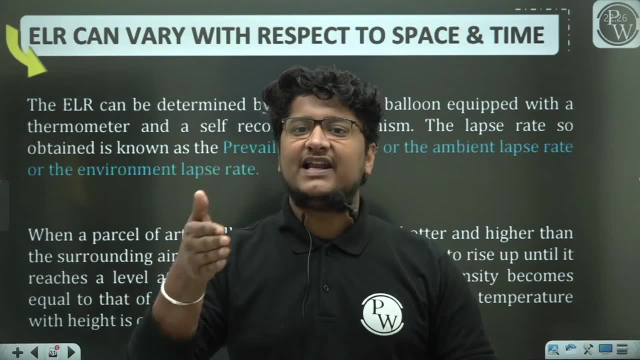 So ELR will change Based on the location as well as based on time, But if you talk about the second, It is nothing but the ELR. We call this full form Adiabatic lapse rate. Now, what is this? For example, you must have seen chimney. 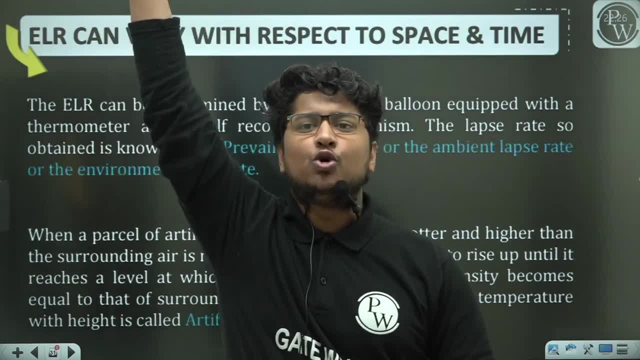 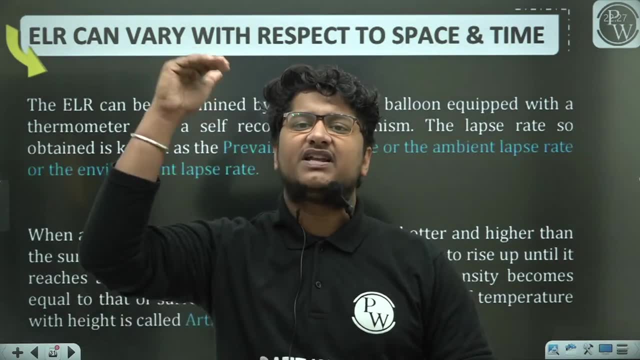 So the smoke coming out of the chimney, It is going up, Yes or no, sir? Why is it going up? Because, sir, it is a warm air parcel And any warm air parcel wants to go up. When will it go up, sir? Till the time the density 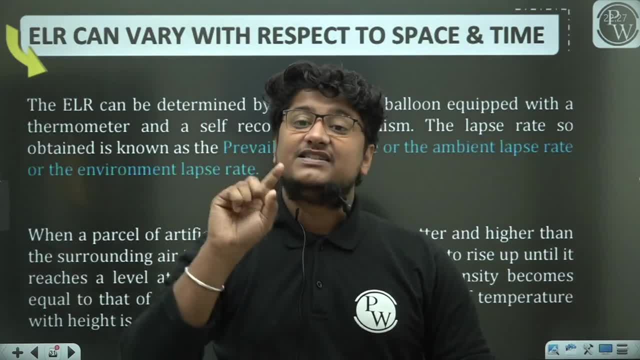 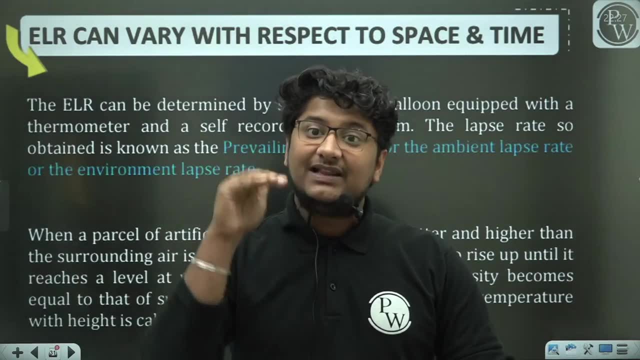 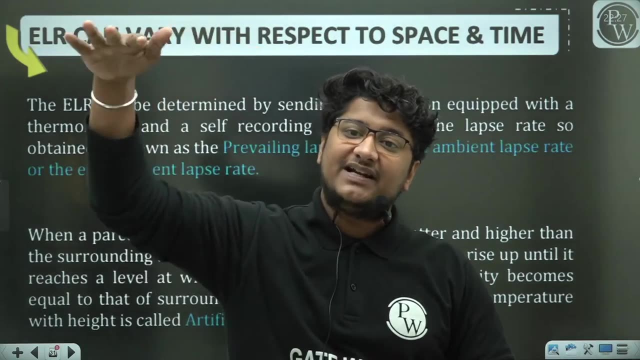 And the surrounding air density is not the same, Or till the time Its temperature And the outside environment temperature Is not the same. Till that point it will go upward, So that warm air parcel Which is coming out from the chimney It will go upward till a point Where the density of that plume 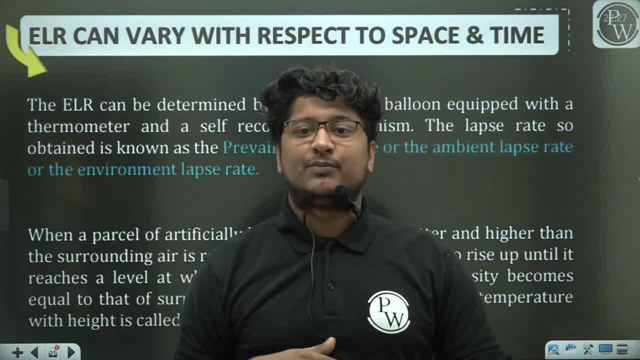 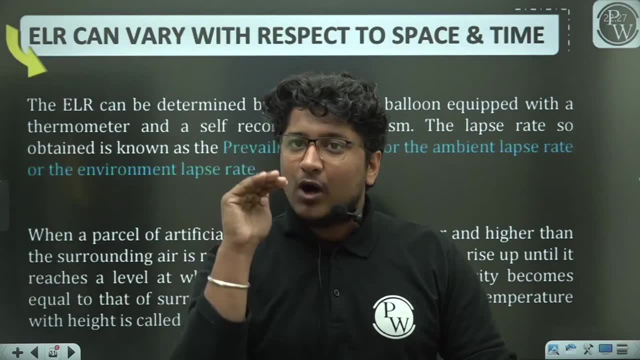 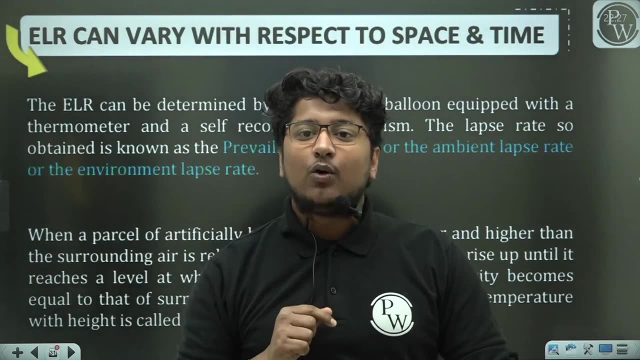 Is becoming equal to the Outside atmospheric air density. Till then it will go upward. Till then it will go upward, Same thing with that temperature also. So when it is going upward, It is a warm air parcel. It is going upward During the course of that motion. What will happen to you? 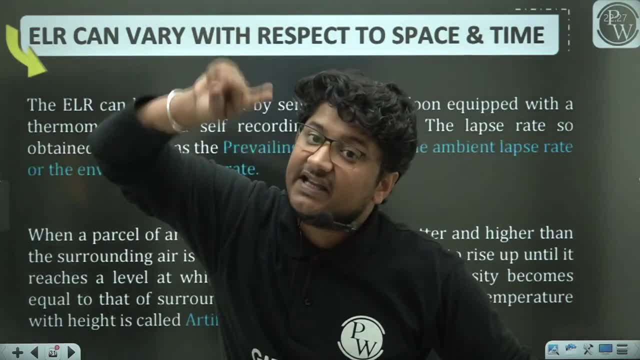 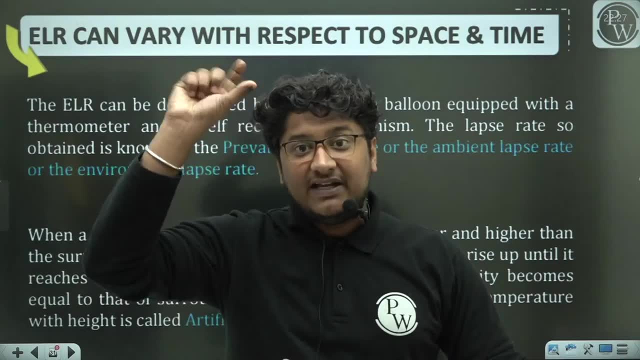 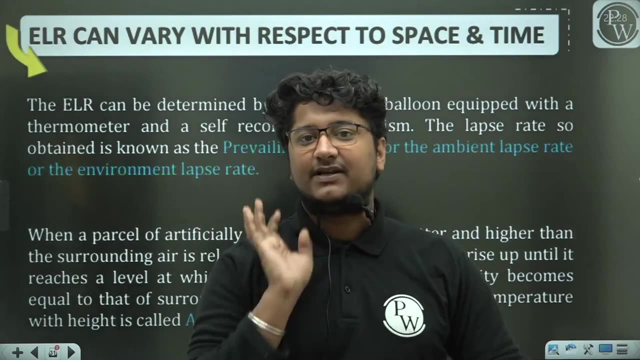 It will decrease its temperature, And when it is decreasing its temperature, That means there is a decrease in temperature With respect to altitude. There is a decrease in temperature With respect to altitude. So where DT upon DH comes, It becomes a lapse rate And this particular type of lapse rate. 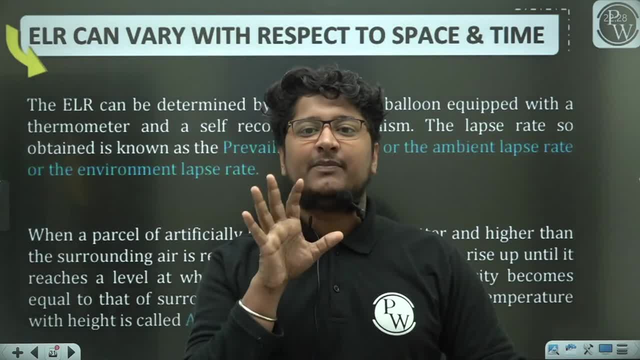 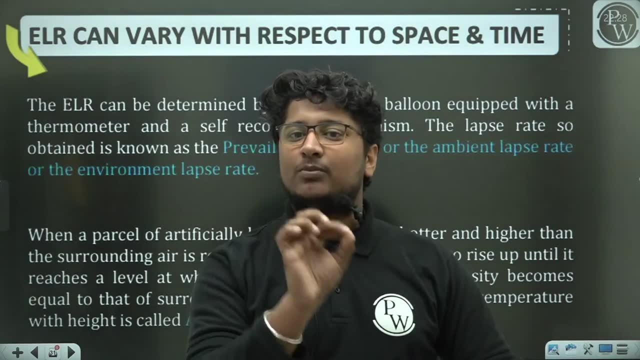 And it is a thermodynamic property And it will always be constant. For a dry condition It will be somewhere around Minus 9.8 degree Celsius per kilometer, And if you have a wet condition, Then you have to keep minus 6 degree Celsius per kilometer. 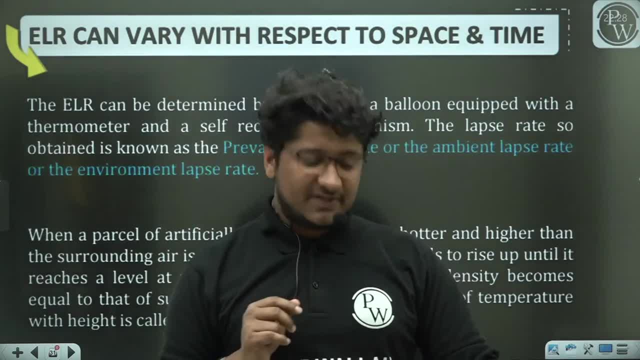 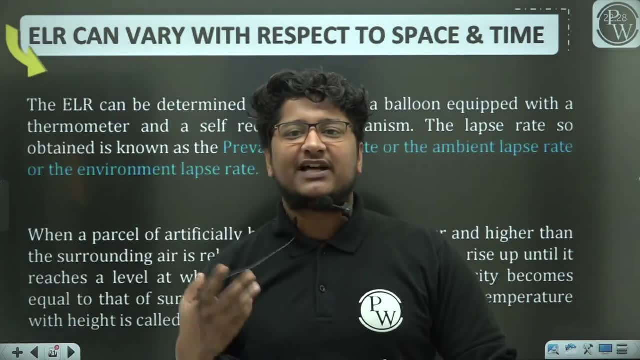 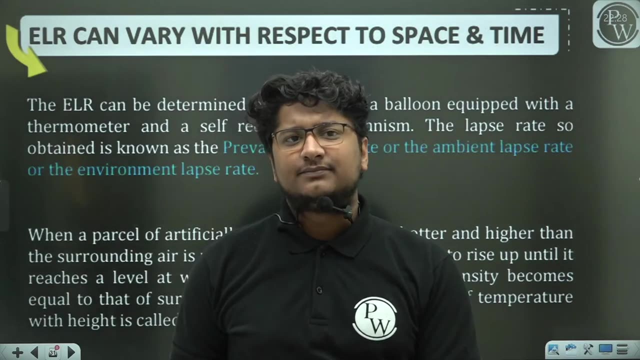 I will make you note these things Now here. you have to understand That. how is your ALR Constant? Try to understand it with some examples. How is your thermodynamic property? What is your constant? Will it not depend on the volume of the warm air parcel? How much volume is there? 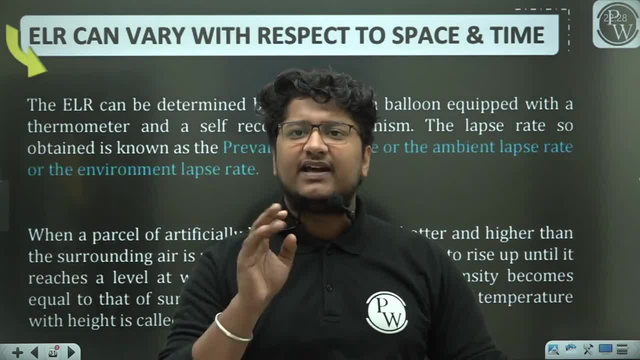 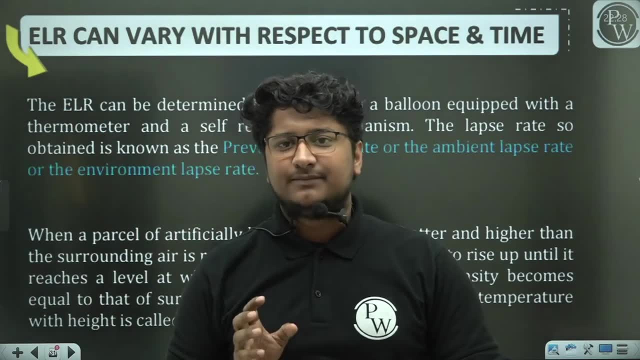 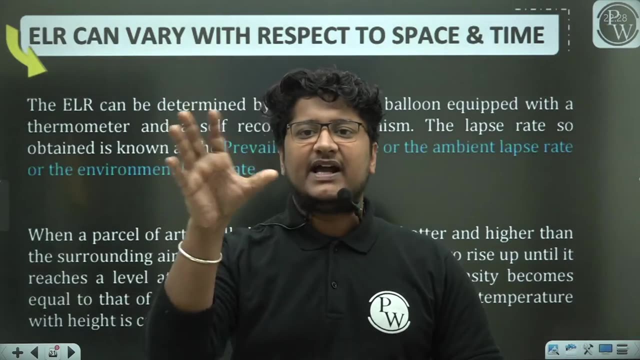 It should also depend on that. It will not. For example, There is a 5 liter milk. 5 liter milk we have And then 1 liter milk we have. I have heated both at the same temperature. Let us say both are at 60 degree Celsius. Now I have left both to cool down. 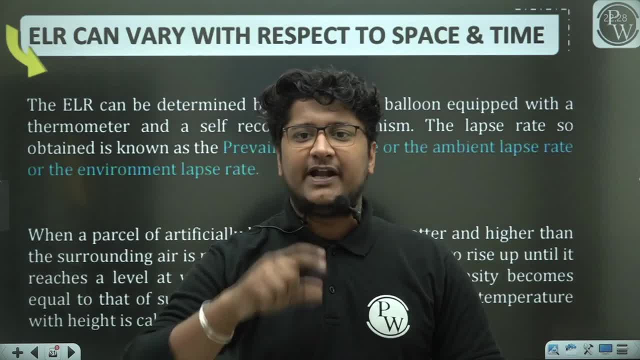 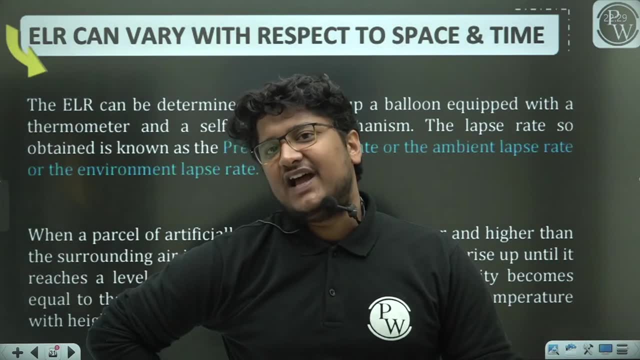 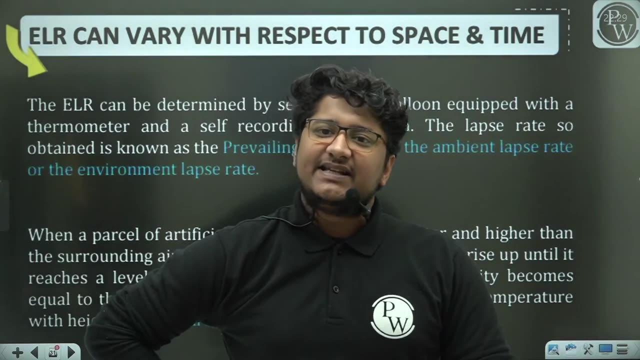 I have left both to cool down. Who will be the first to cool down? Comment and tell. First case: We have 5 liter of milk. Second case: We have 1 liter of milk. Both the milk I have heated, both at the same temperature: 60 degree Celsius. 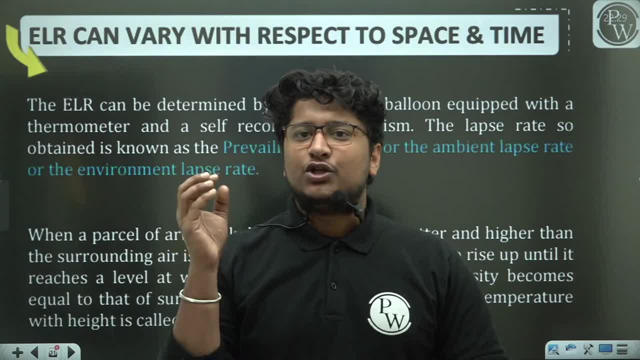 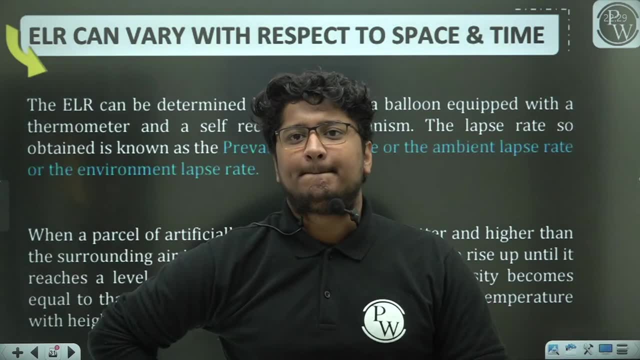 60 degree Celsius. Now I have left both to cool down. So I am asking: Who will be the first to cool down? Who will be the first to cool down? Who will be the first to cool down? Vivek Bachcha is telling case 1. 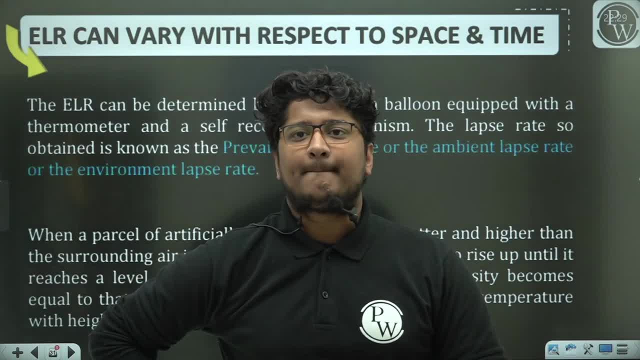 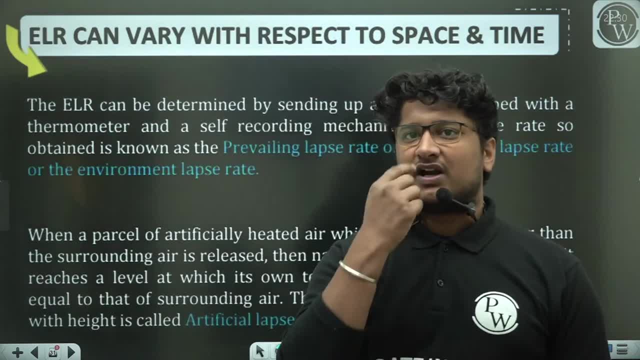 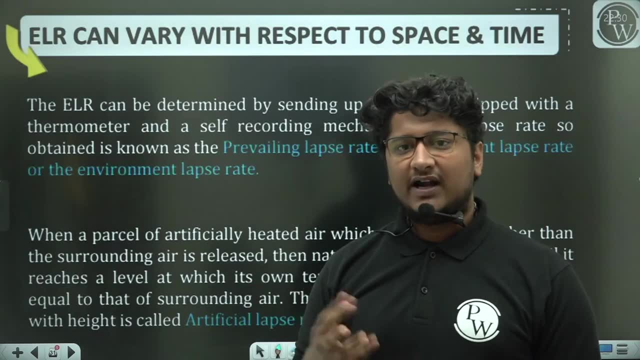 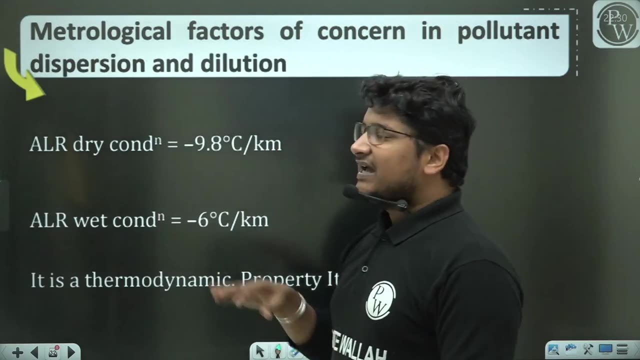 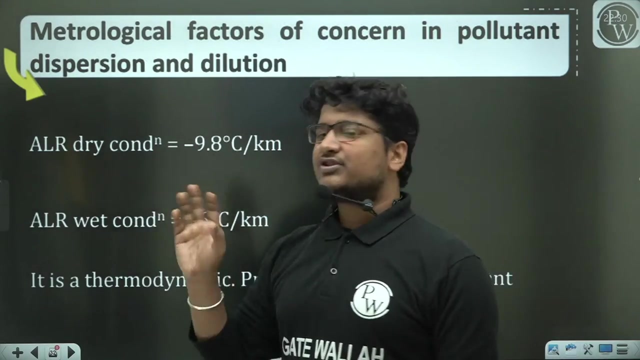 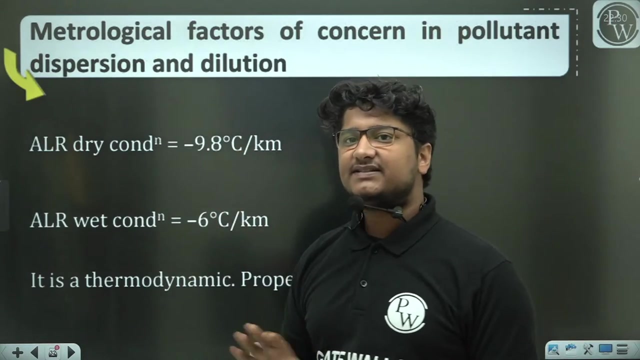 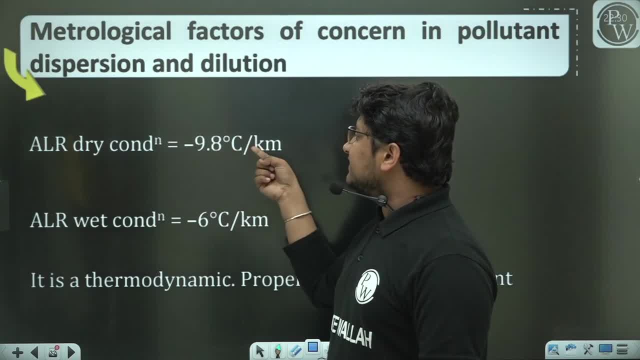 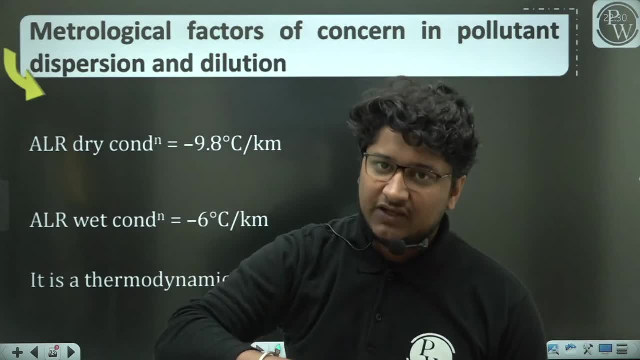 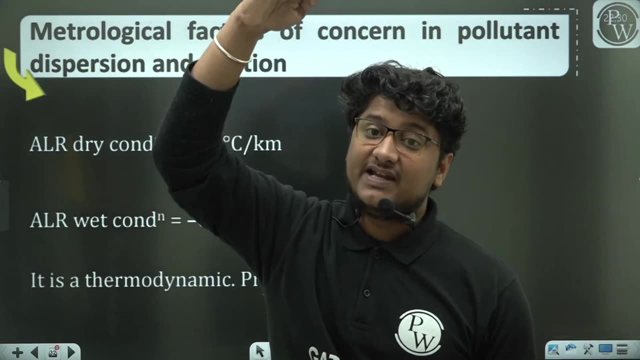 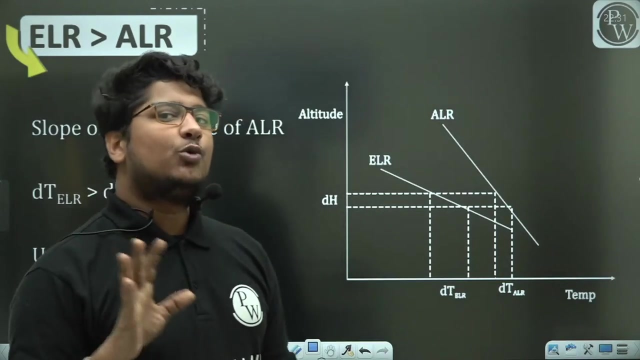 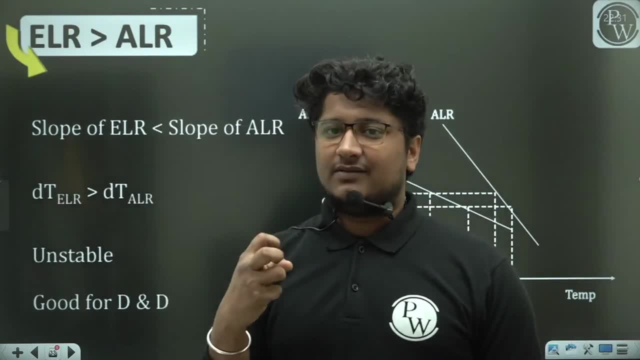 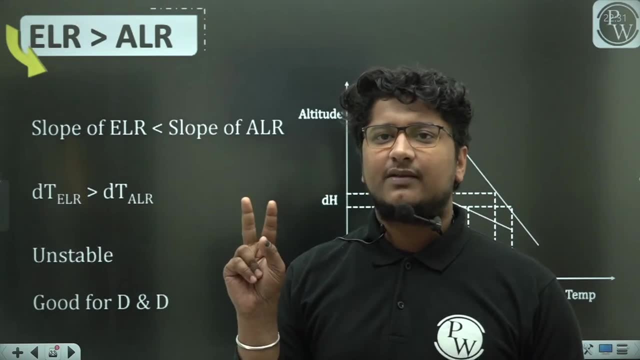 please give me an answer to yes or no, Because he is a hero. If you don't understand the hero, you will play the whole movie in the wrong way. It is important to understand these two heroes. So if you don't understand the difference between ELR and ALR, 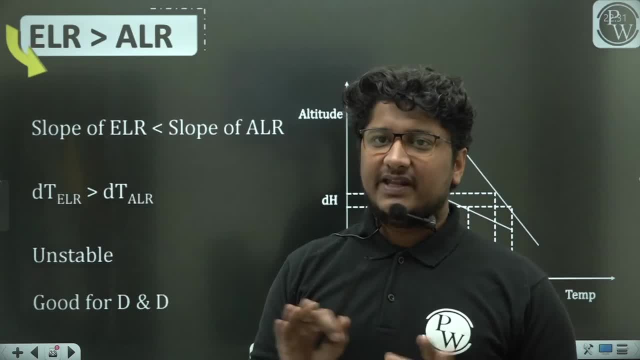 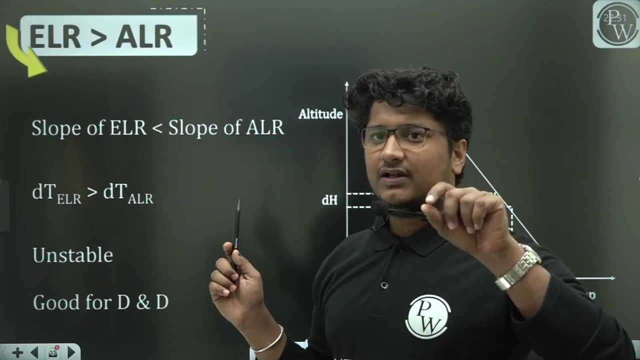 or you don't understand ELR and ALR. anybody, frankly, tell me, Because if you don't tell me, the pain will remain in your life. I'm telling you. If you're not going to tell me, sir, I have a problem with ELR and ALR. 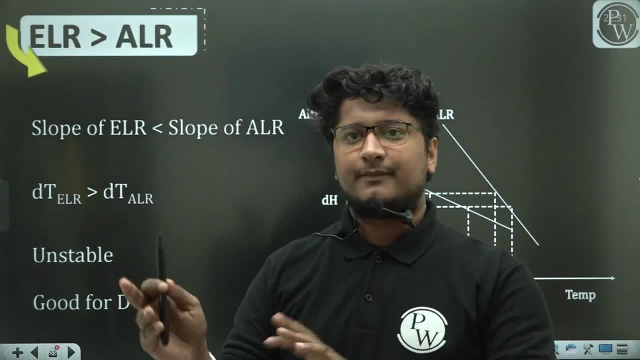 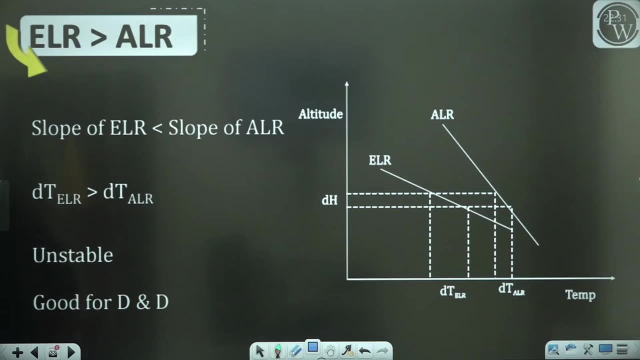 then I will clear it here, Because you will live in pain in the future. So if a child has a problem with ELR and ALR, please tell me, And if it is clear, then also tell me. It's not that you and I don't have a lot of connection. 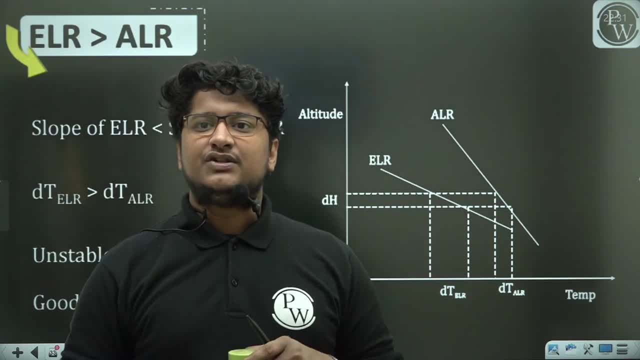 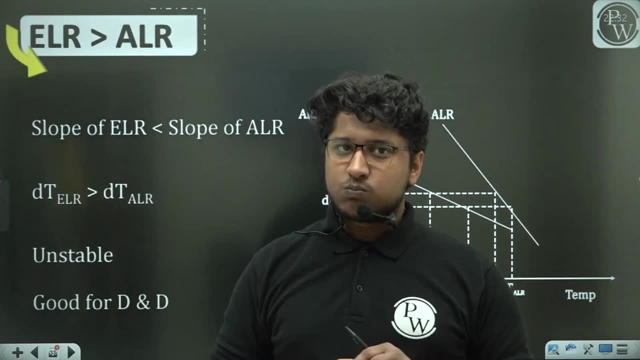 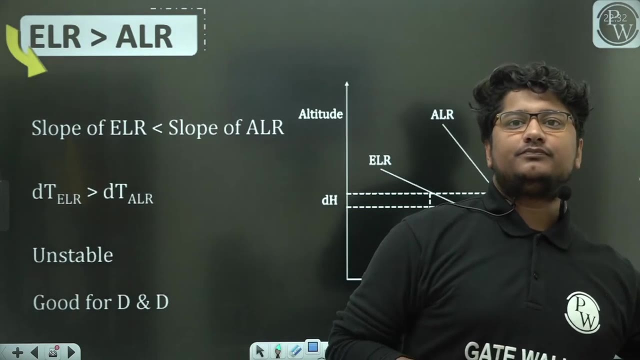 Do you. I will know what you are thinking in your heart. So if you understand ELR and ALR completely, please tell me Full repeat, please. Sahabaz bacha, this means you didn't pay attention here. I have told you so many things so easily that there is no chance of repeat. 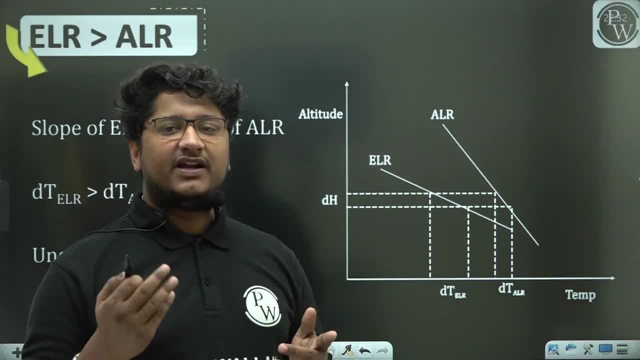 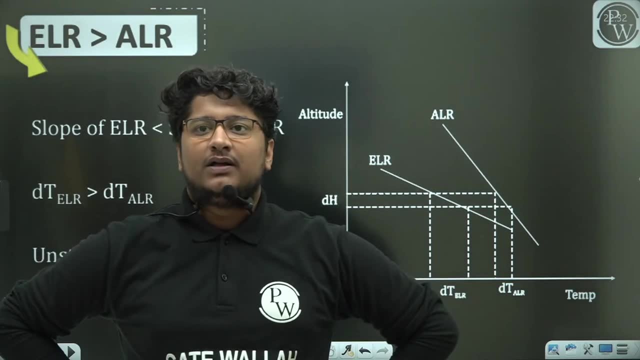 I am repeating again only for Sahabaz. I will not repeat these things again and again Because there is a class of cross-course left. I don't have so much time to repeat these things to you. Listen carefully, I am telling it very slowly. 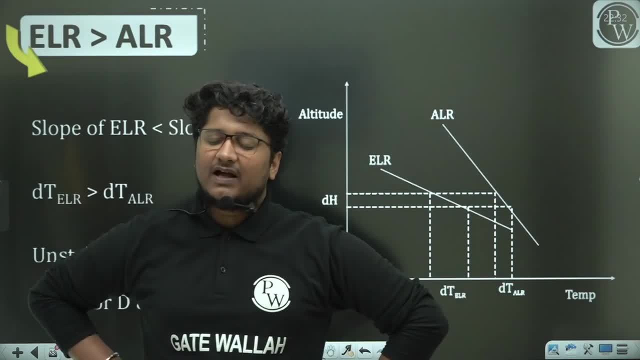 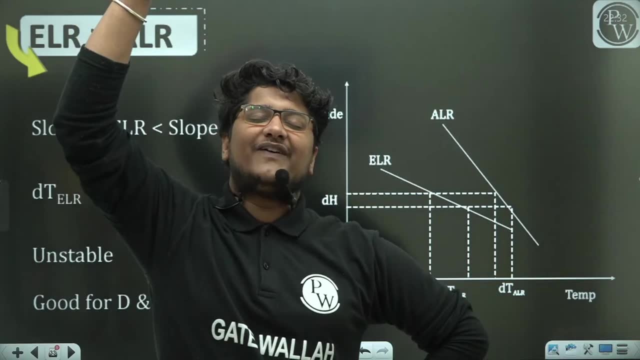 ELR means that in natural environment, if you go from one floor to two floors, from two floors to three floors, from three floors to five floors, from six floors to ten floors, when you are going up you will find a change in temperature. 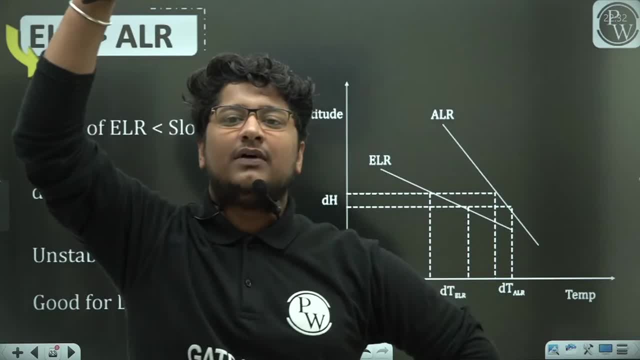 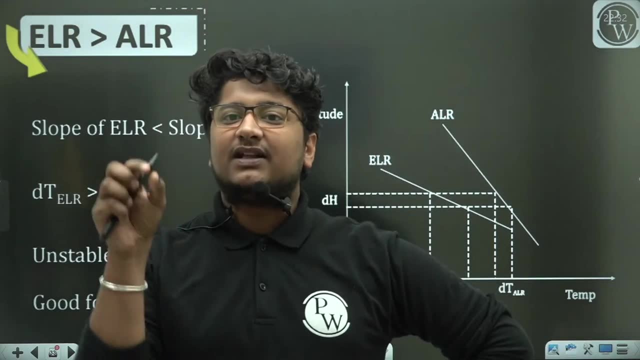 And that change in temperature with the height we call as ELR And that can change based on the location, based on the time. But if you talk about ELR, ELR is nothing but when a warm air parcel which is artificially heated up. 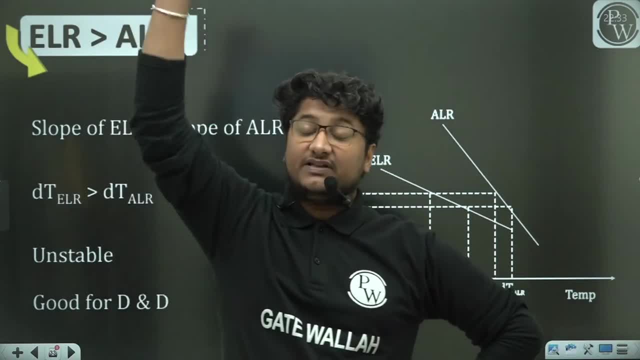 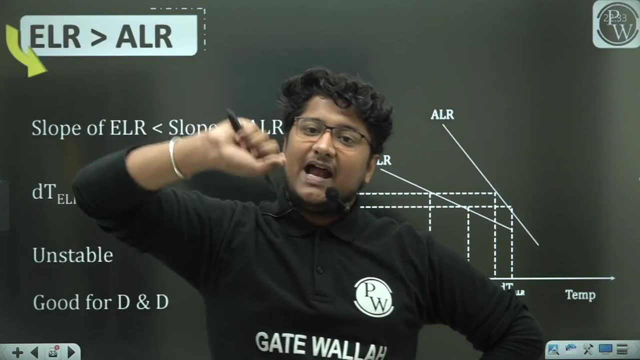 and that air is going upside, that air mass is going upward. In that case, what will happen? It will change its density, it will change its temperature And during that, what will happen? There is a change in temperature with the altitude. 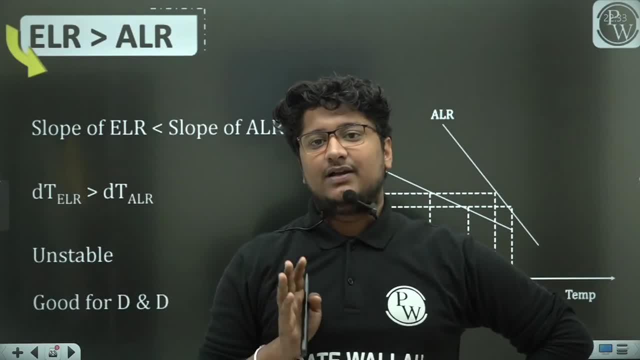 That change in temperature with the altitude we call as ELR. So now ELR will be constant because it's a thermodynamic property. It will be constant and that value will be minus 9.8 degrees Celsius per kilometer for that time. 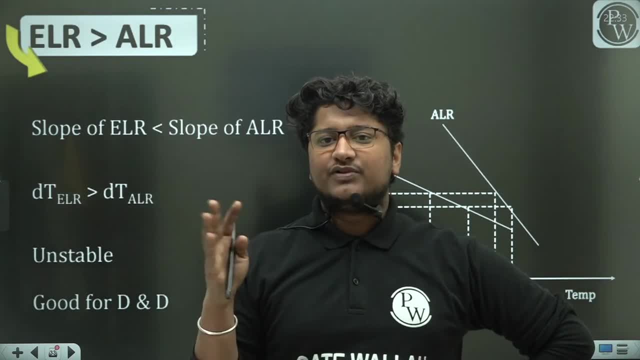 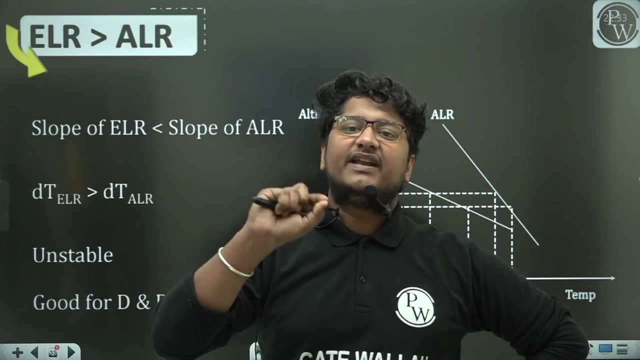 It will be a dry condition and somewhat lesser, around minus 6 degrees Celsius for the wet condition. Keep this thing in your mind. So ELR will be constant. ELR will vary according to your location and time. Now, this is the game of these two heroes. 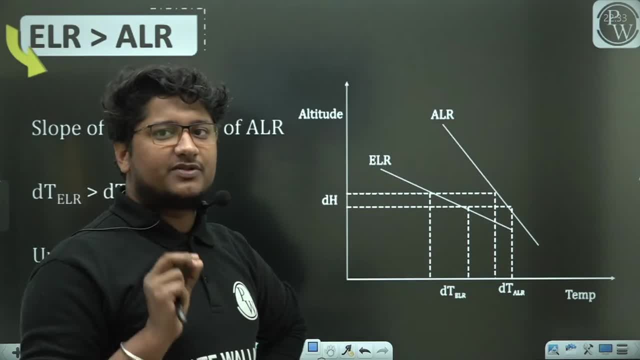 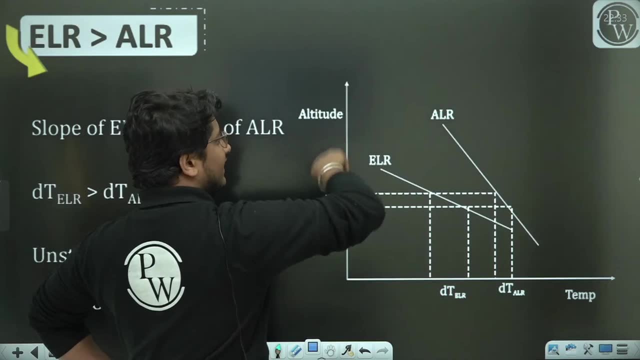 This is the game of these two heroes. If you understand it easily, then you will understand it. The first case is: let us say: what did you do? Pay attention, What did you do? You put one here. altitude in y-axis. 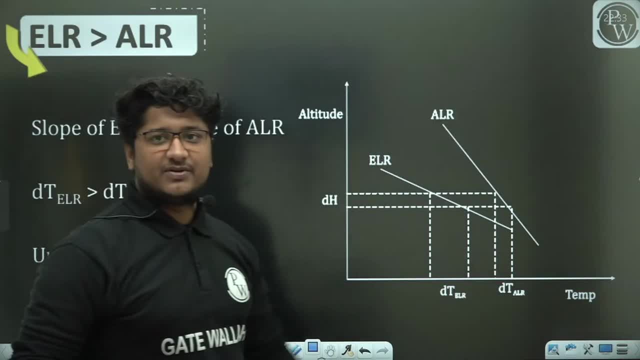 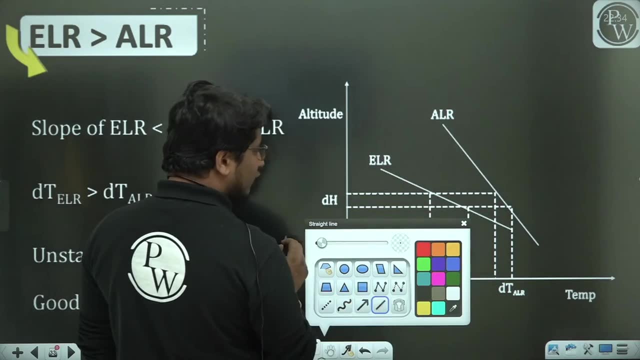 Means, you have kept the height And in x-axis, you have kept the temperature. Okay, Keep this in your mind, The red line that I will draw. I will draw it with the help of ELR. So what did you do? 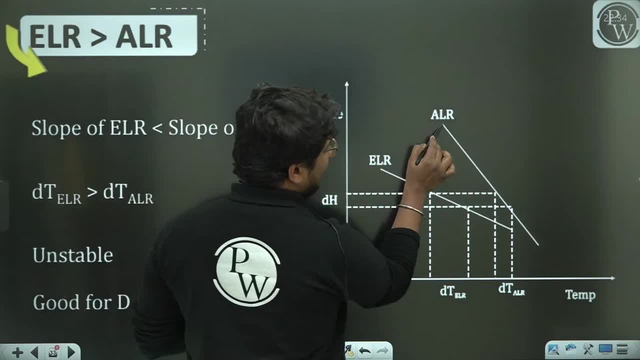 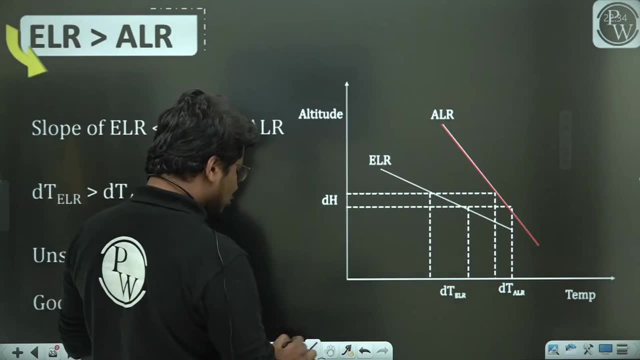 You plotted and you drew a red line, Red line. whenever I will draw, it will be showing you the ELR part And the second one. I have drawn a blue line. That is for ELR part. That is for ELR part. 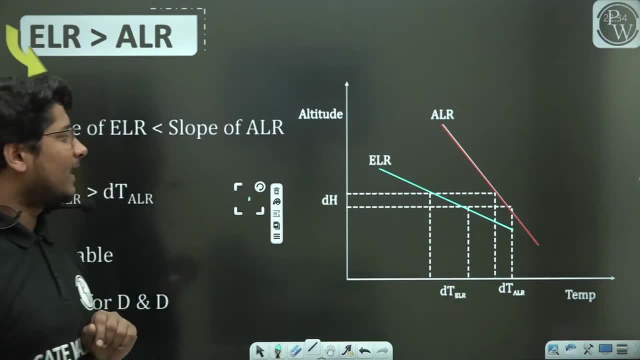 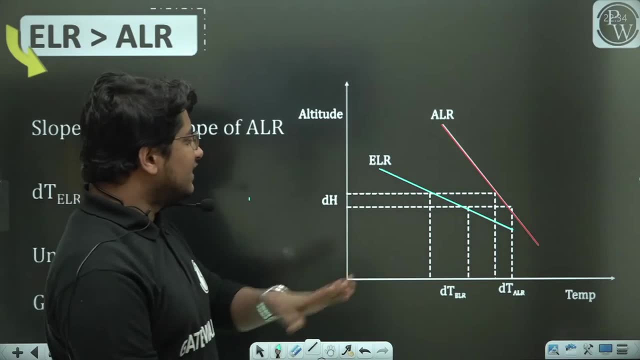 Okay, Now this red line and the ELR part, the blue line that you have drawn. you have to understand this game, Sir, how did you draw this? Some people ask, sir, how did you draw this? So, son, I did not do anything here. 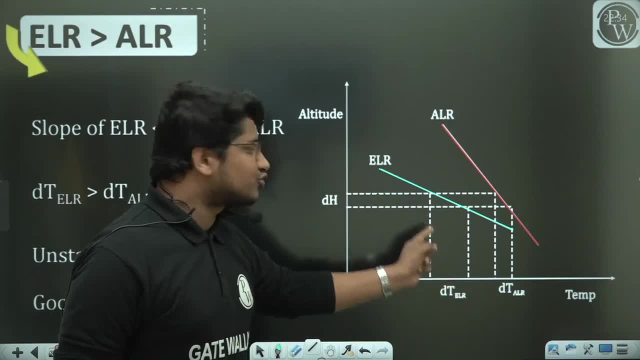 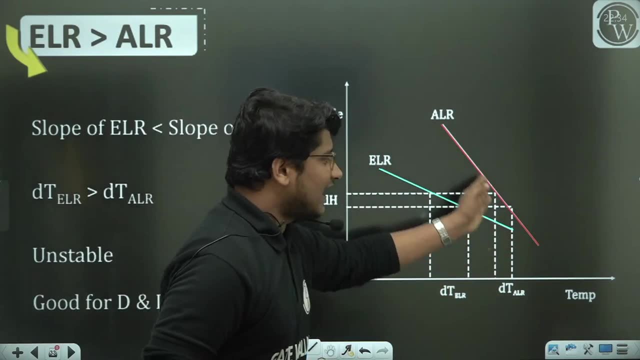 Plotting the different temperatures at different heights. Plotting the different temperatures at different heights. This line will be drawn And the ELR line is always constant. That is, minus 9.8 degree Celsius per kilometer. You will always see the ELR line being constant. 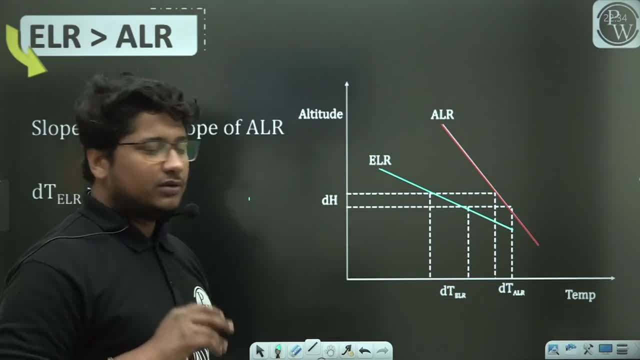 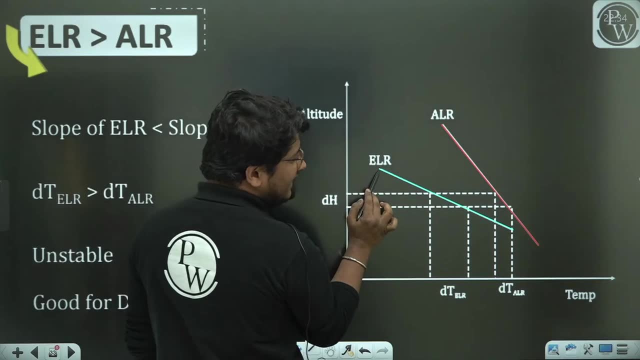 The ELR line will vary according to your time and distance. Now, if I draw both of these, Now if you look at both of these curves, then you will forget what the case-wise is. Tell me whose slope is more in ELR and ALR. 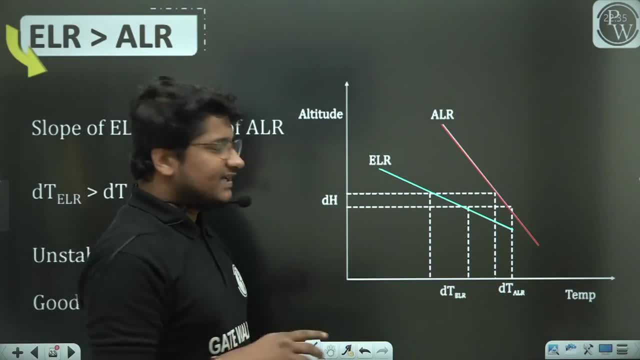 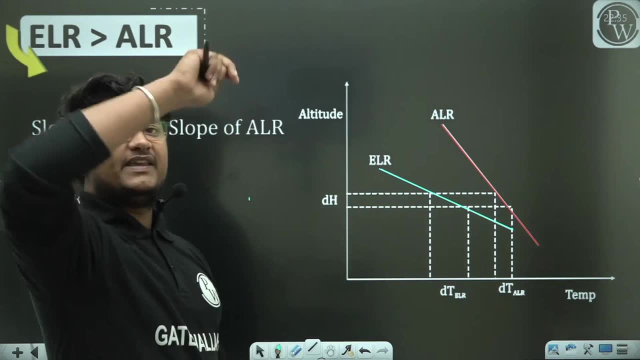 Just look into this diagram. Just look into this diagram and tell me slope of ELR is more or slope of ALR is more. Slope of ELR is more or slope of ALR is more? Answer it easily, Because you have to read 8-9 cases ahead. 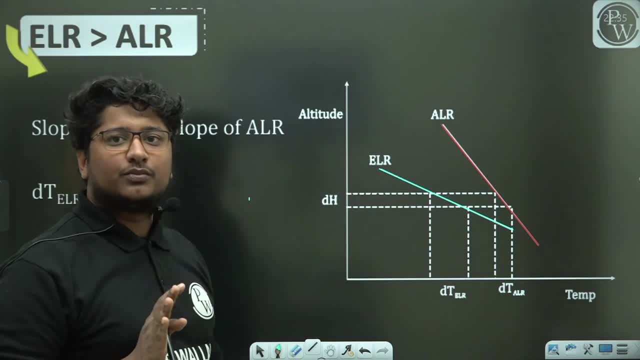 So if you do not understand, you will rot For sure. Try to understand. Try to understand. Do not keep it. The slope of ALR is more. The slope of ALR is more. Okay, Very good. Who is Vivek Chaudhary? 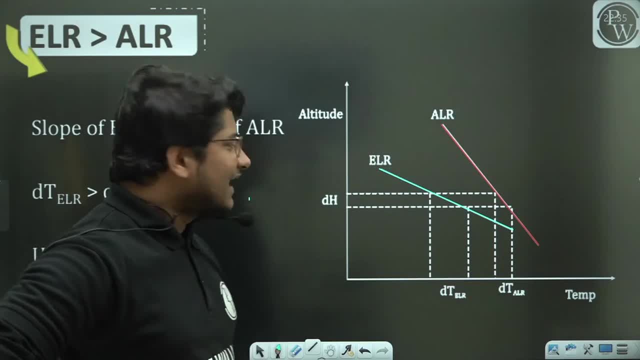 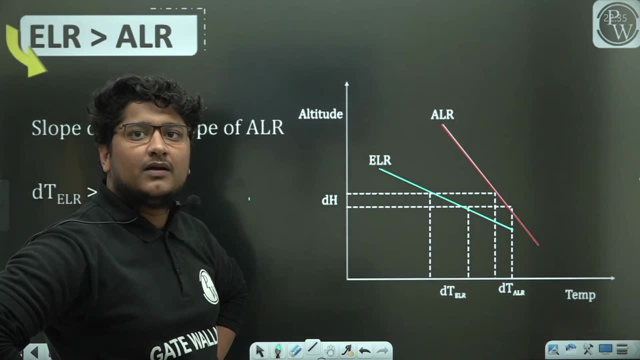 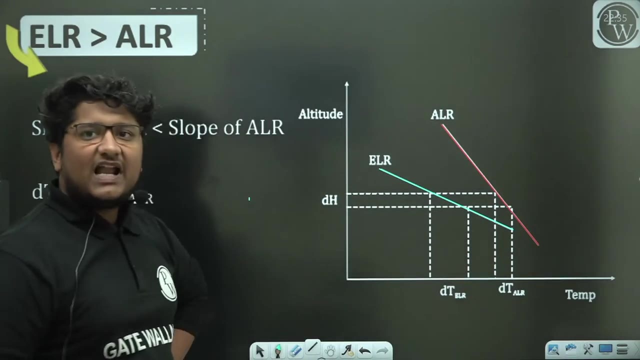 Do you eat and sit Useless? It is clearly visible that the slope of ALR is more, So he can see ELR. So now see, the slope of ALR is more compared to ELR. Ok, Now if you compare in both, 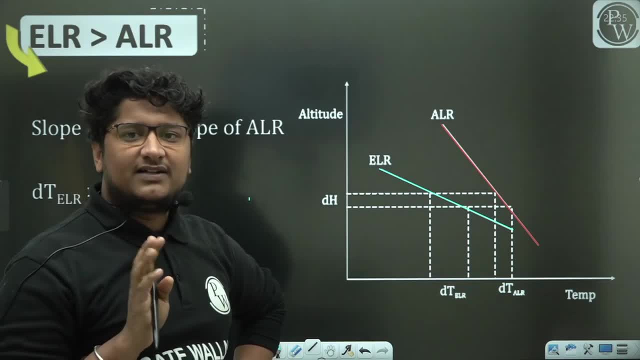 when you compare in two things, then you will give one data to same in both, right. If you want to do comparison in two people, then you will give both resources also same. So if I want to compare in ELR and ALR, 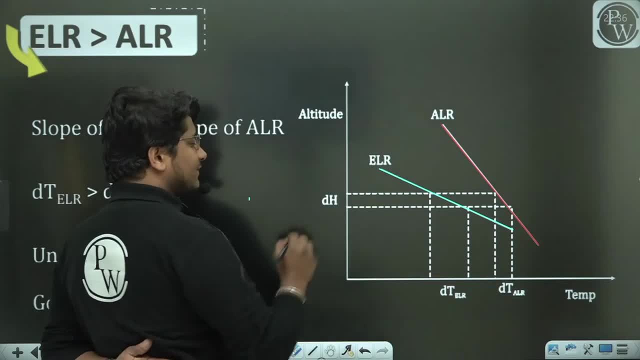 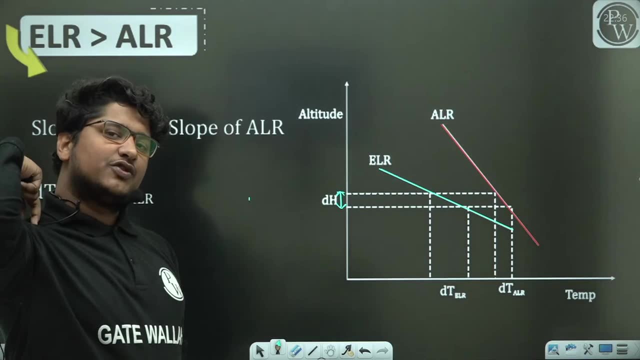 then what did I say? That do one thing, that give height in both. Give height in both. That means give your elevation difference. what is the elevation difference you give? You give same. One second kid, Where is he roaming? 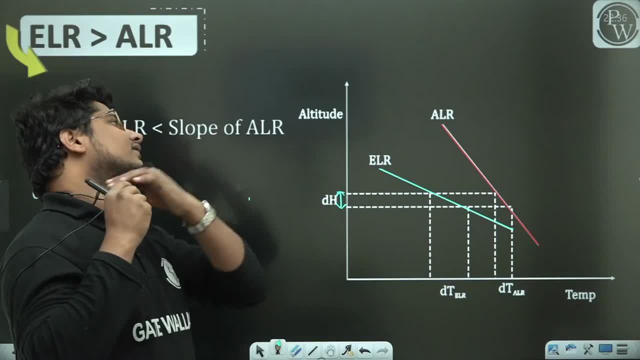 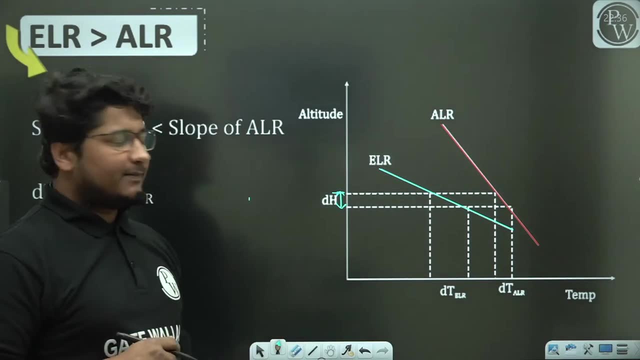 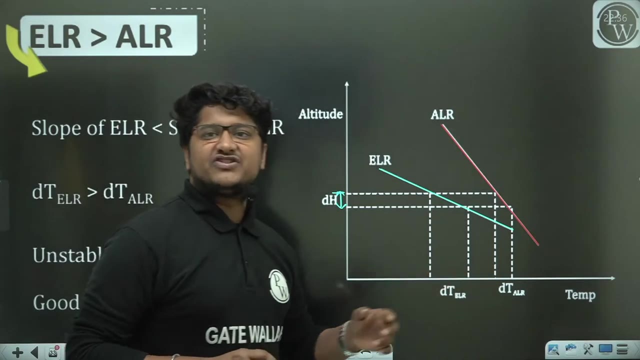 Where is he roaming? Where is he roaming, Where is it rotating? So what did you give? We talked about same elevation difference So that we can do comparison, that if we keep same elevation difference in both, then see how different temperature changes. 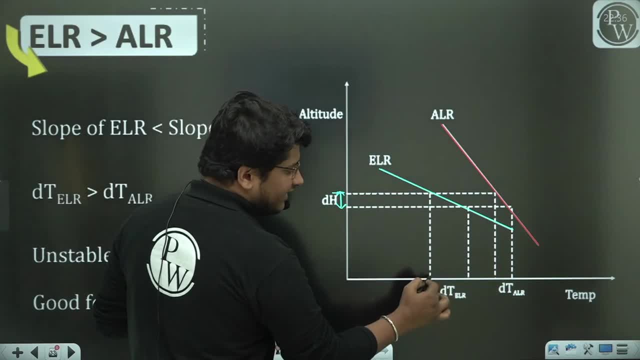 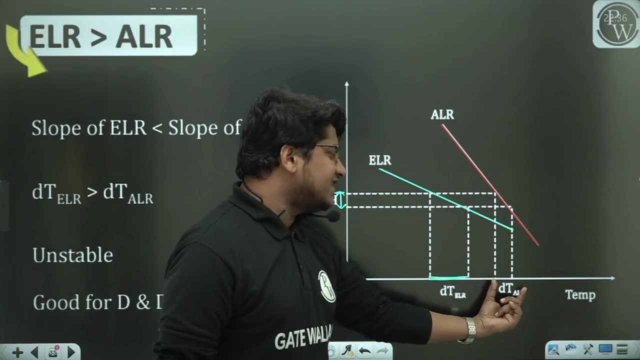 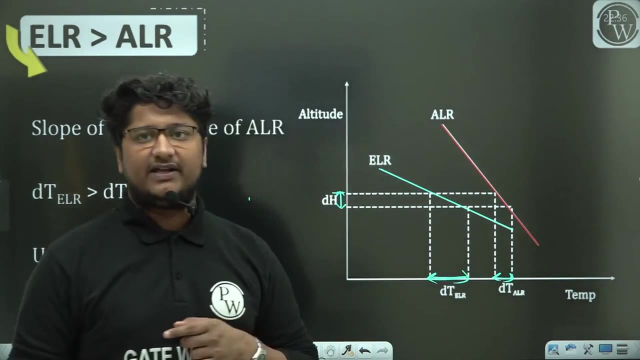 So what did we do? If we plot same elevation difference in ELR, then we got this much value. This is nothing but the DT ELR. And if we project the same thing in ELR, then we got DT ELR. Now I don't need to tell you that here ELR is bigger or ALR is bigger. 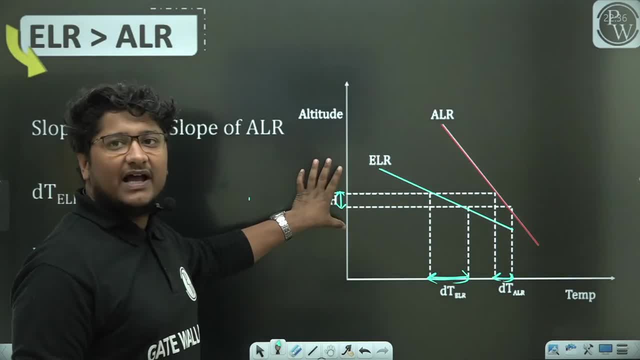 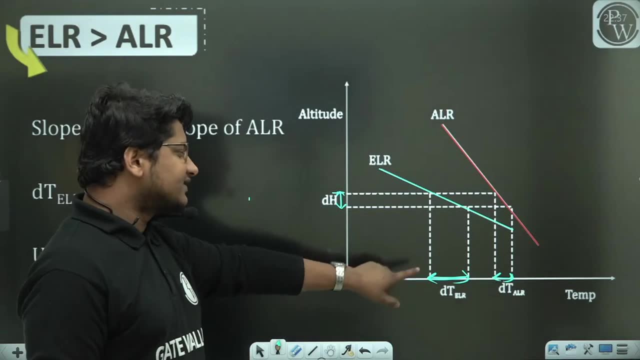 For the same height difference, for the same elevation difference, the temperature difference is more in ELR or ALR. Comment and tell me: The temperature difference is more in ELR or ALR. See the figure and tell me. See the figure and tell me. 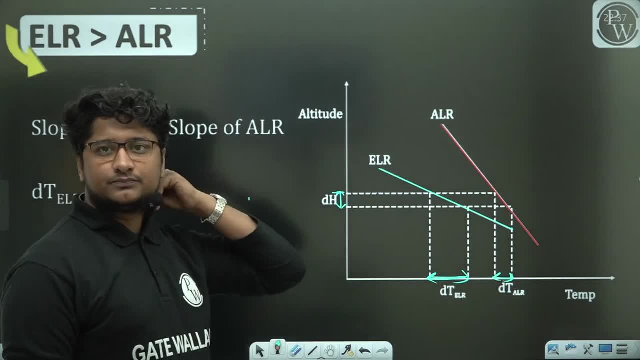 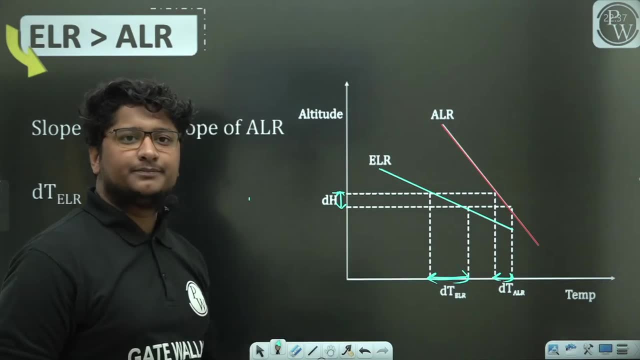 Don't see anything else. See the figure and tell me. See the figure and tell me, Did you get the temperature difference in ELR or ALR? Comment and tell me, Sir, it is more in ELR, Sir, it is more in ELR. 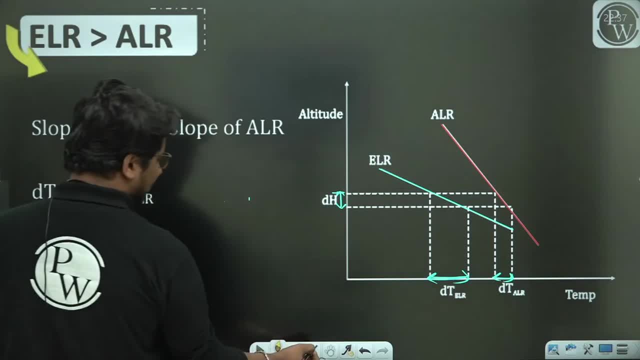 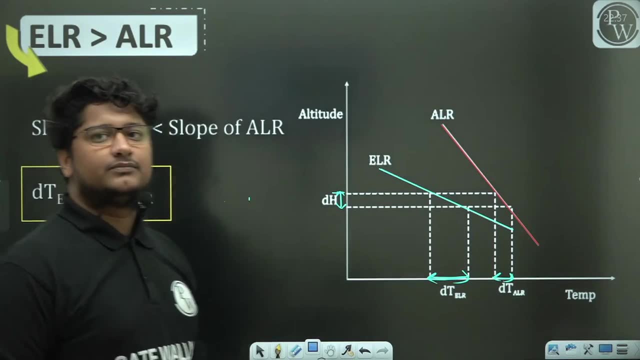 That is the reason why your case is made. What is it made of? I will put it in the box. The DT of ELR is greater than DT of ALR. So you saw more ELR in comparison to ALR. You saw more ELR in comparison to ALR. 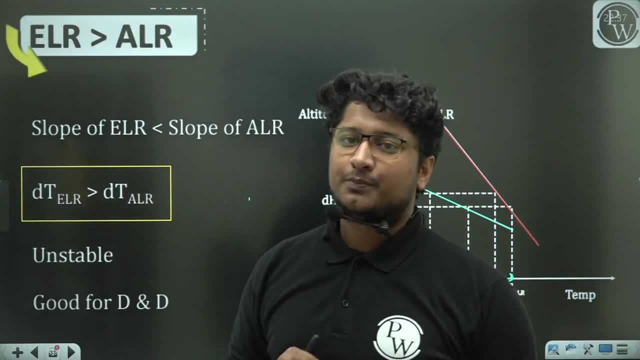 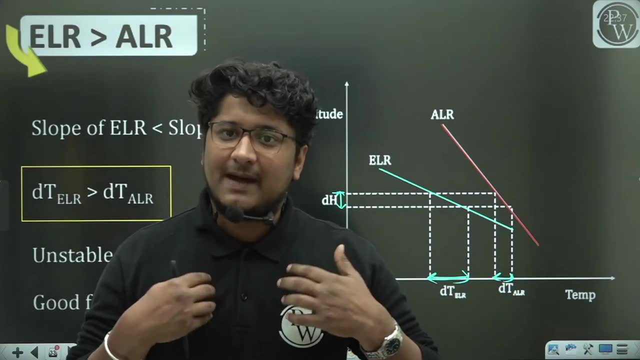 If you can understand this condition with an example. What is the example? Look, you are ALR, You are running in a race. You are ALR yourself, You are ALR yourself, You are running And ELR is the one who is going to run with you. 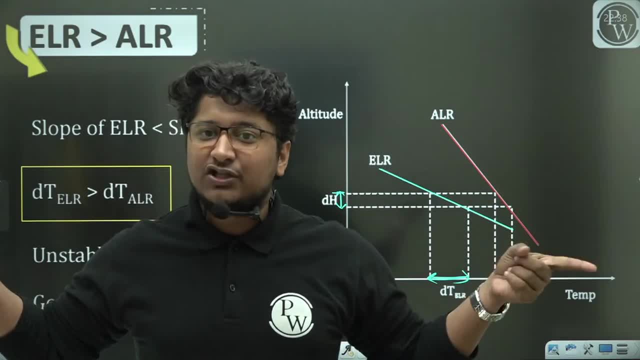 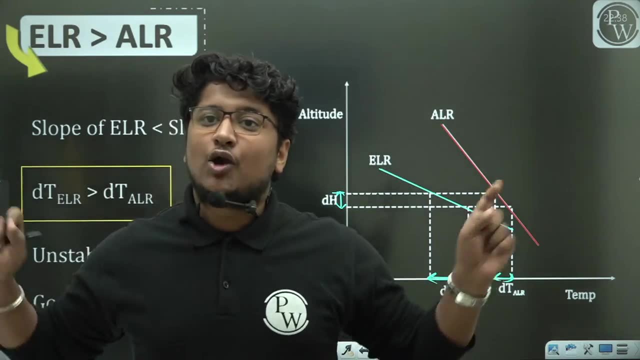 ELR is the one who is going to run with you. The one who is going to run with you is your environment. Now you understand that if you are running in a race with a 10 meter per second speed And all your friends are going with a 20 or 30 meter per second speed, 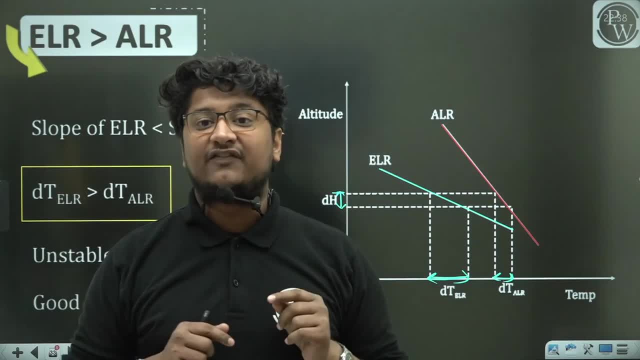 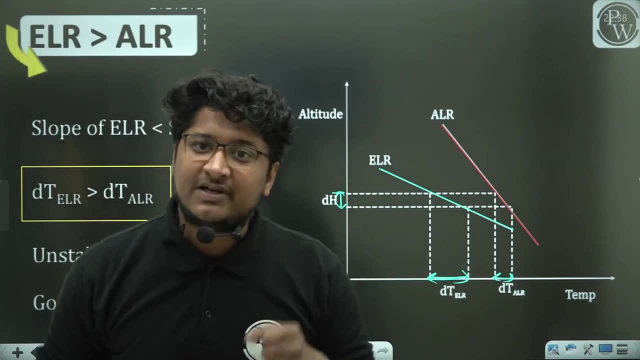 Now tell me what your mental thinking will be. What will be your mental thinking? You want to increase your speed. You want to decrease your speed. You are going with a 10 meter per second speed. That is nothing but the ALR. 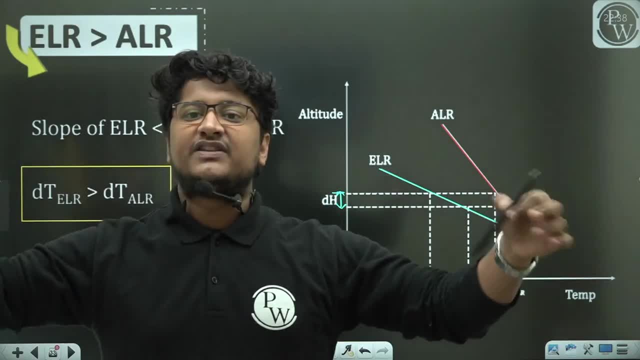 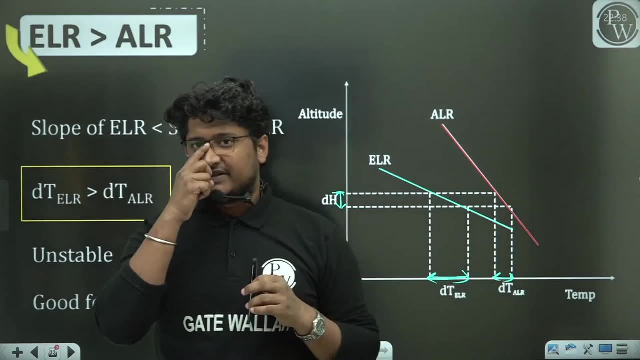 That is nothing but the ALR. All your friends are going with a 20 or 30 meter per second speed. What your thinking will be at that point of time? Tell me fast. With a simple example, you will understand. With a simple example, you will understand. 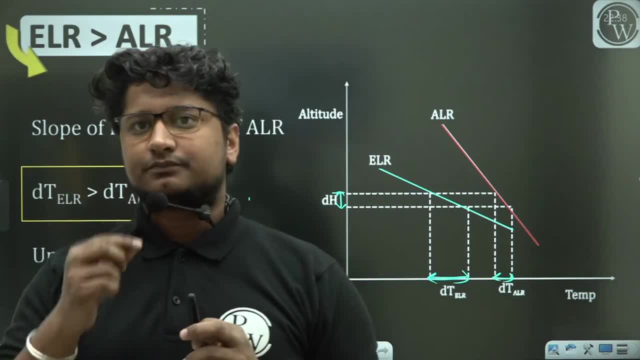 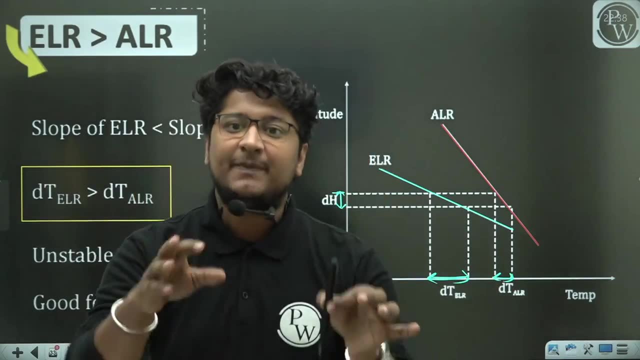 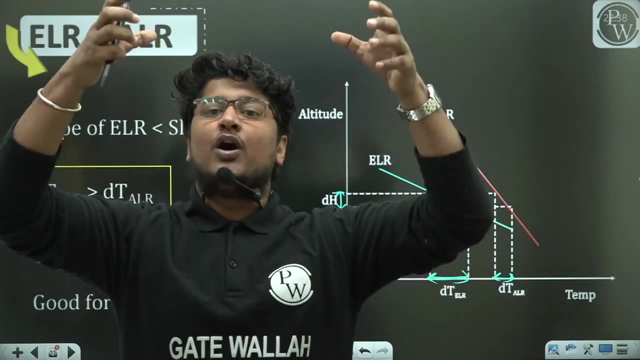 Quickly. I want reply quickly. I want reply quickly. You will increase your speed, You will increase your speed. That is what happen when a warm air parcel comes out of the stack or a chimney: That warm air parcel is going upward, But that if ELR is more than the ALR, 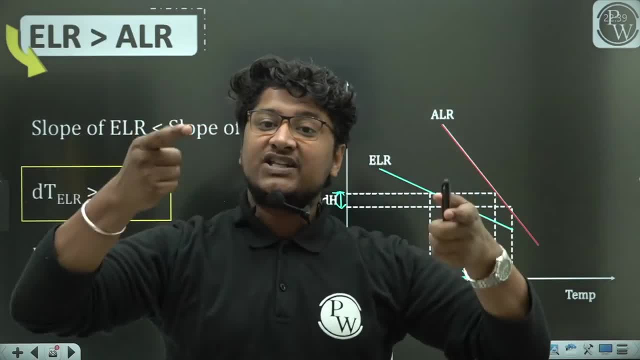 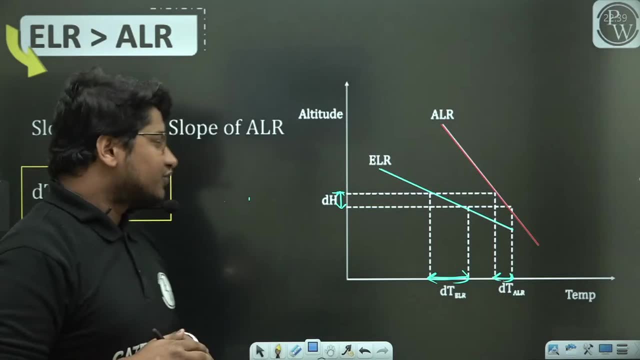 That warm air parcel will go with a certain more height. In that case, what will happen? It will give you more turbulence. It will give you more, better mixing, Better dilution, Better dispersal. That condition is basically unstable condition. That condition is basically unstable condition. 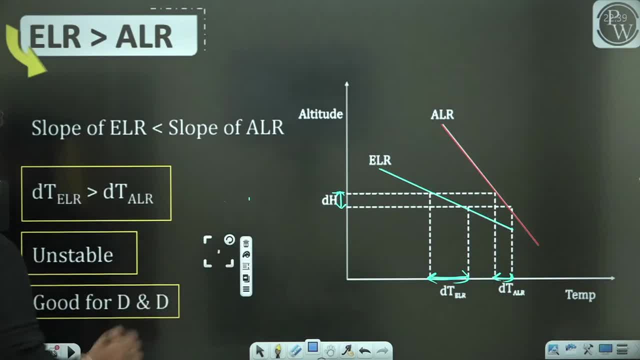 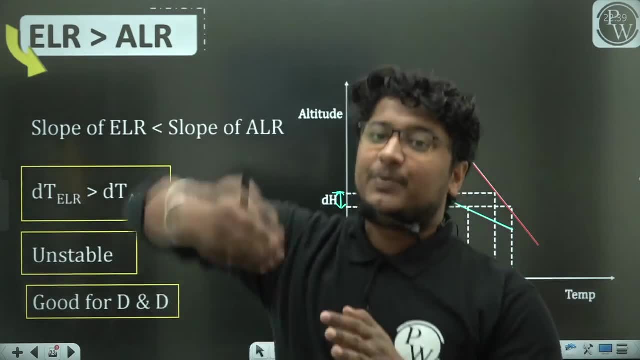 And that is good for. It is good for DND. DND means do not disturb. I am writing in the short form of DND. It means dispersion and dilution. So the more you move vertically, I am talking about temperature, dispersion and dilution. 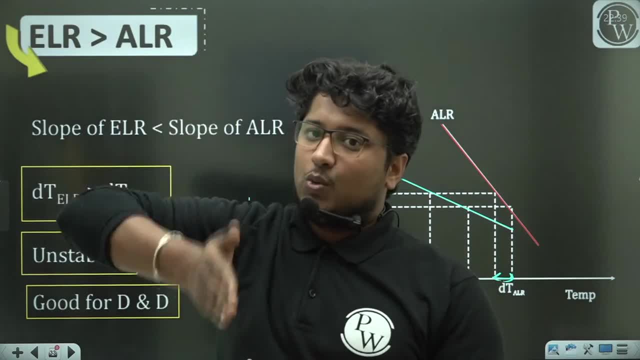 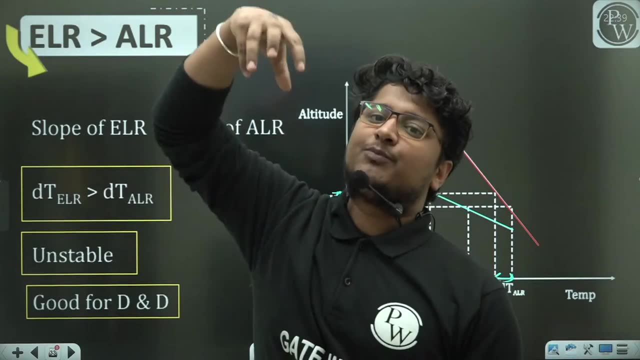 I am talking about temperature, dispersion and dilution. I am talking about vertically mixing. I am talking about vertically mixing. So the better your air, The more air you have The warm air parcel, you have The plume that has come out. 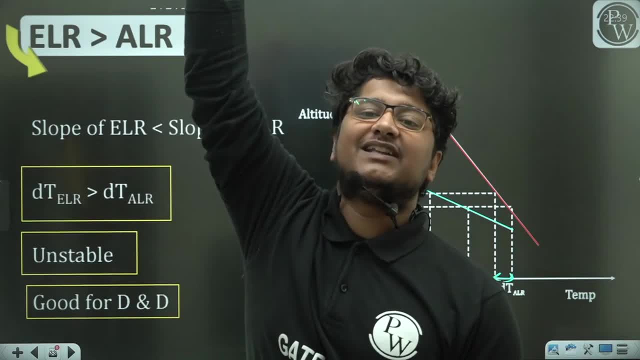 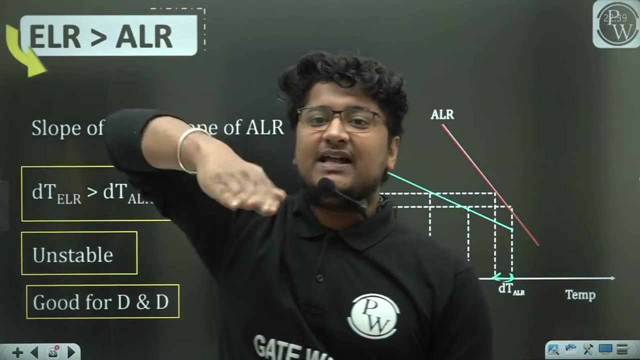 The smoke that has come out of the chimney. The higher it goes up, The better the mixing will be, And that is good for us. That is good for us. So in that case, The higher it goes up, That means vertical mixing will get better. 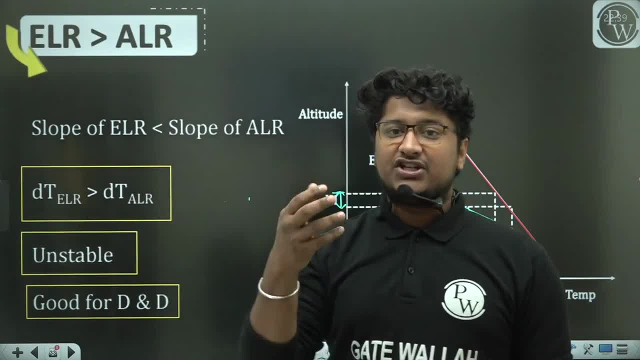 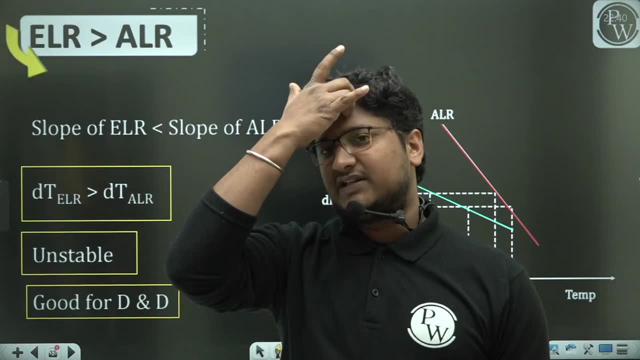 And this condition is basically unstable condition. Unstable condition is good for us. You all know that if there is a symptom of defective progress, Don't become more defective of performance, Otherwise you will get more progress. But those who do not get much defective performance do not get progress. 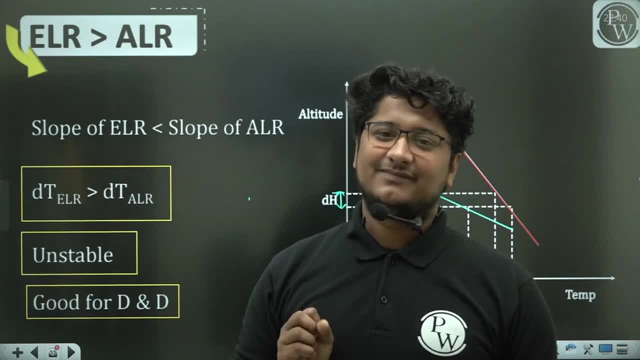 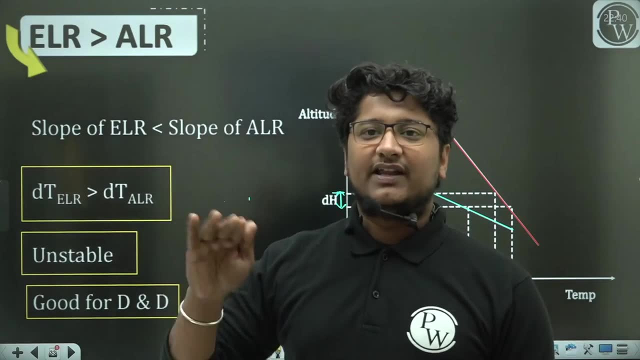 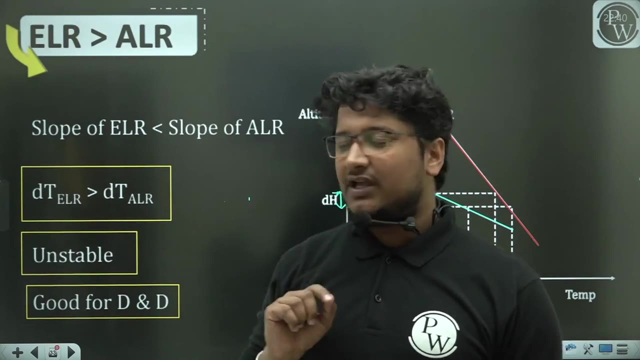 It's okay, We will live our life in one pen. Why work hard? We will live our life in TCR. So understand that the unstable part is good for pollutant dispersion and dilution. So did everyone understand this case, This case we call as super adiabatic case? 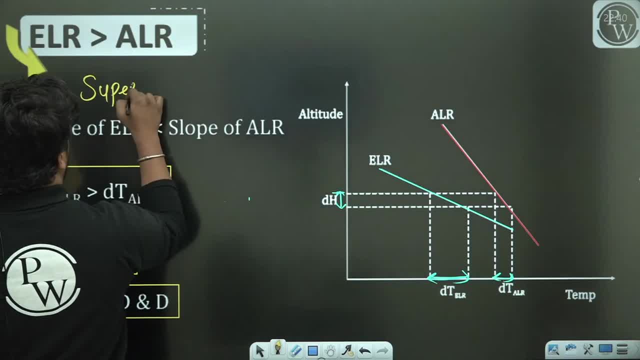 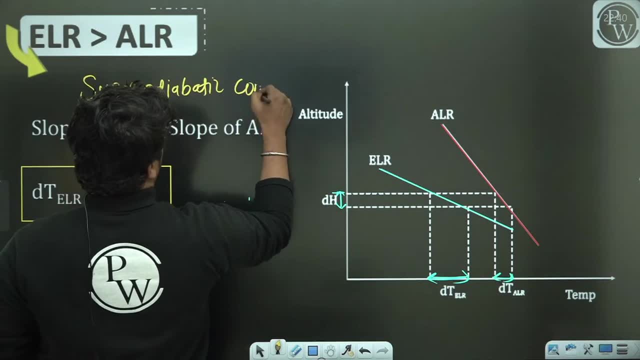 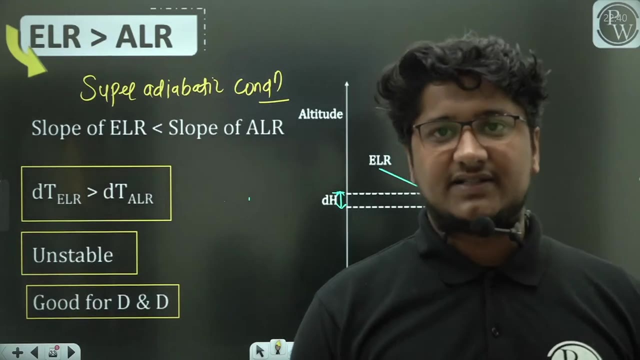 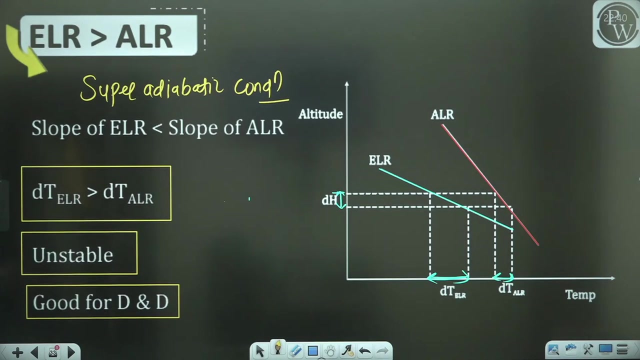 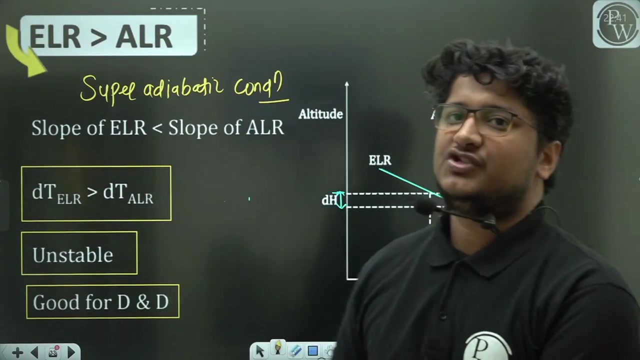 case we have named as super adiabatic condition. super adiabatic condition: Anybody having any difficulty in understanding. Tell me. if anyone has any difficulty, I will move forward one by one case. If anyone has any difficulty in understanding. If you have understood this, then we are going for the next case. 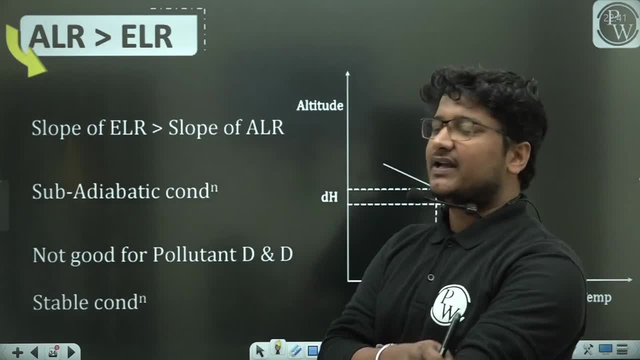 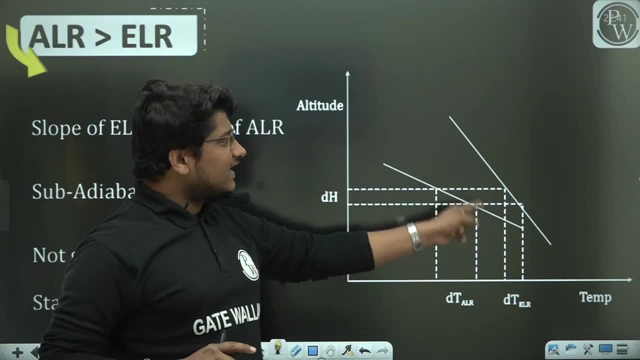 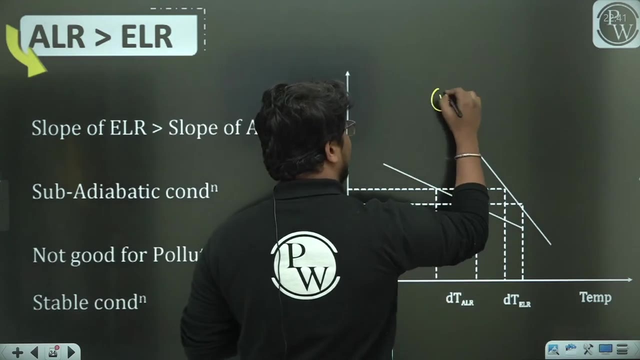 Next case is when your Alr is greater than Elr. Just opposite. Now, see here, I don't need to tell, I am just asking you that which line of these two white lines will be Alr? Let us say name. One is named as 1, Two is named as 2. 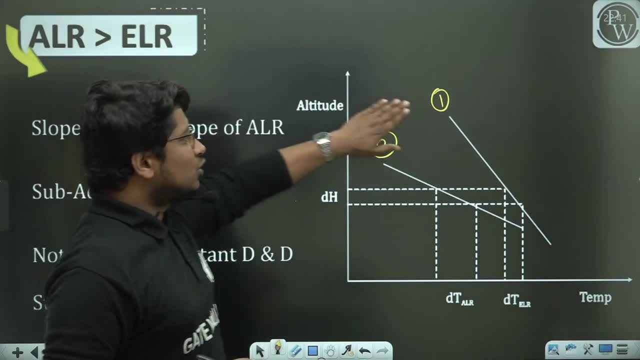 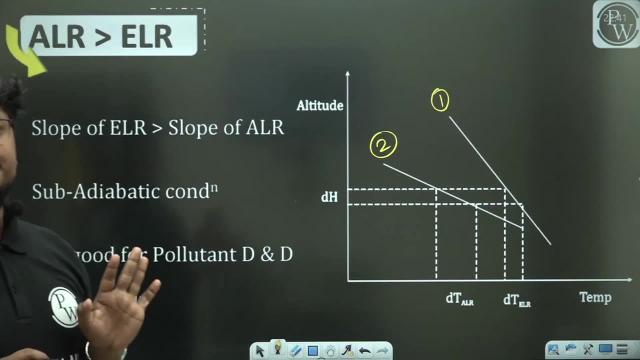 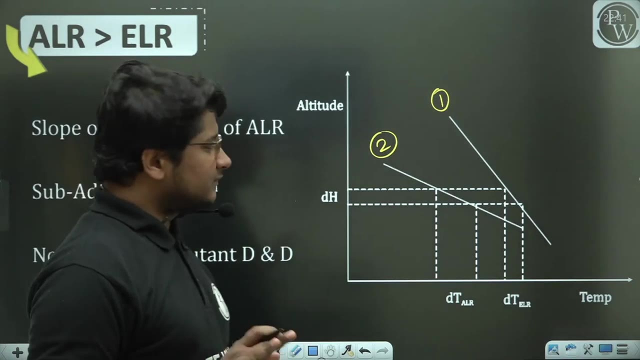 Sir, my case is Alr greater than Elr, Alr greater than Elr. So which one of these two will be showing you Alr? Which one of these two will be showing you Alr? Answer me clearly. Answer me clearly, Easy, Easy. There is no confusion. 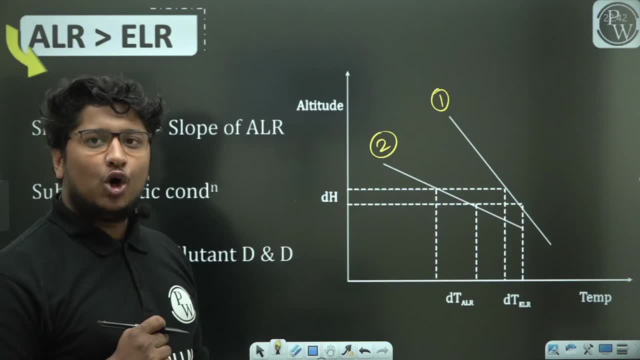 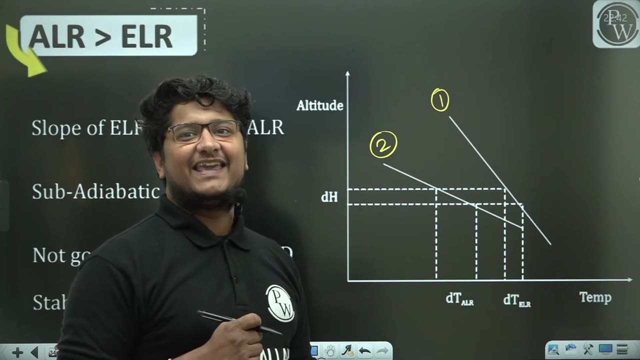 First is showing Alr. First is showing Alr. The second line is showing Alr. Very good, you are saying: First is showing This is showing which is bigger than the Elr. Yes, This is very good, Superb, You can see the sky is also movingable. 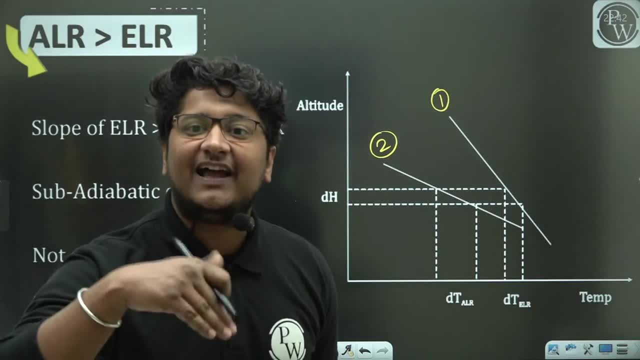 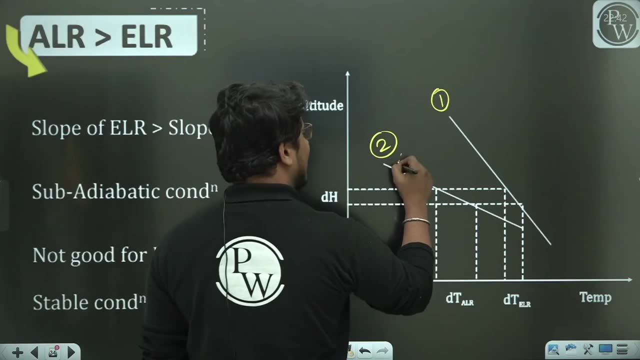 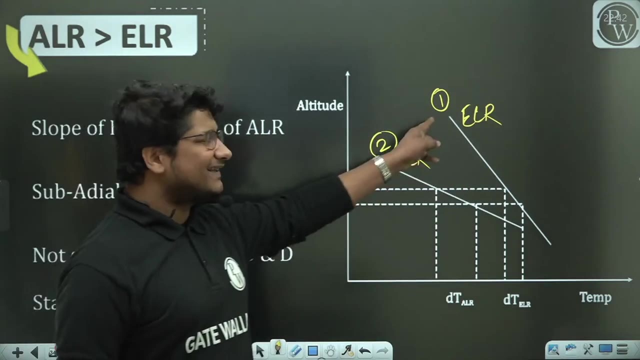 Sus, Its value is higher than that of which is faults. Sirrit, You said Alr, greater than Alr, So which is shown T slope is less. that is our ALR and this is our ELR. The one whose slope is more, its value is less, sir. 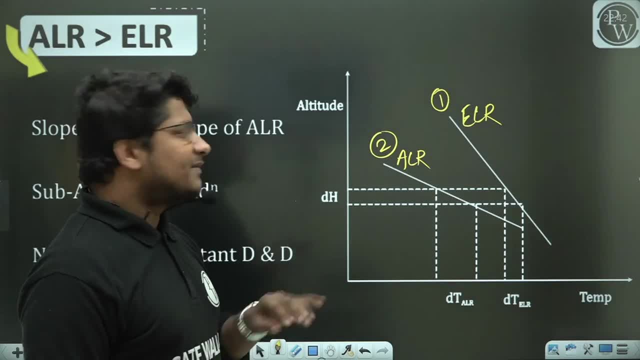 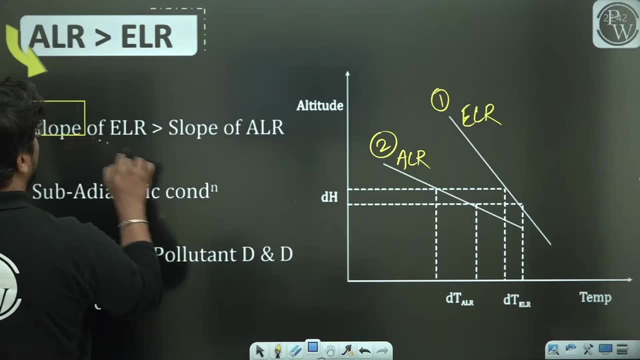 Did you understand the point or not? Okay, now I have explained this thing to you in a simple way. Now, in such a condition, you can see that the slope of- I have also mentioned here the slope of ELR- is greater than the. 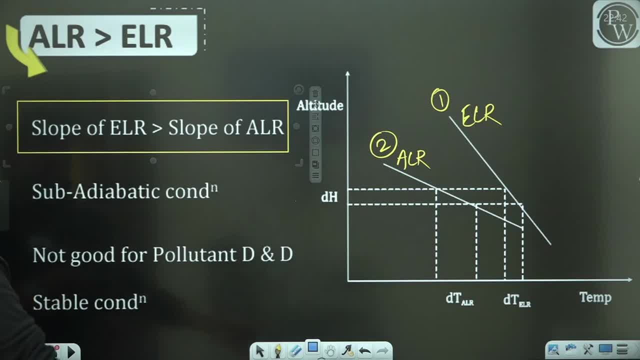 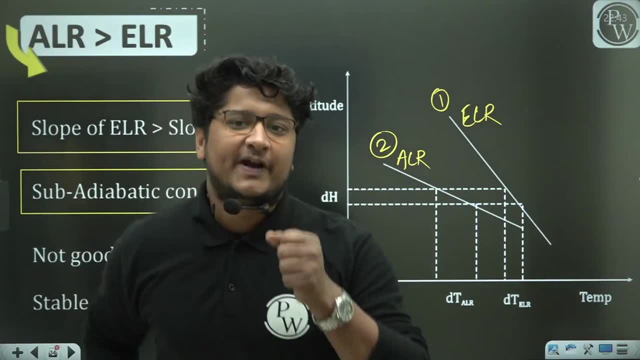 slope of ALR. Okay, what will be called in such a condition? This is your sub-adiabatic condition. Now, the obvious thing is you are running in the race with a 20 meter per second speed. 20 meter per second speed. 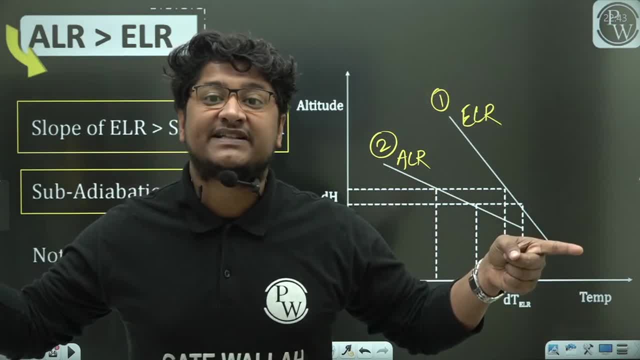 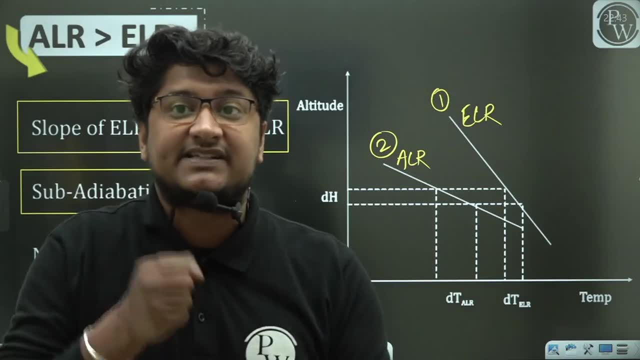 and all your friends are going with a 5 meter per second speed. What your thinking will be, Aapki thinking, kya rahegi Aap 20 meter per second speed se ja rahe hain And all your friend are, all your friend are. 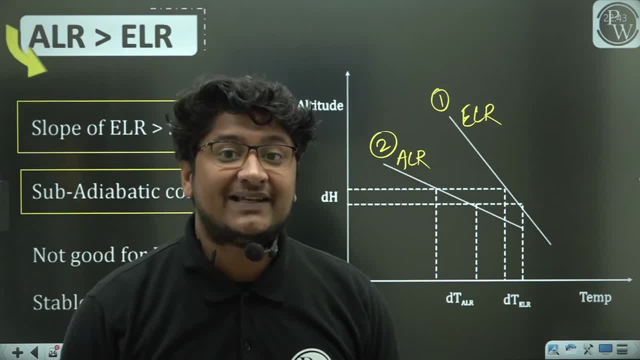 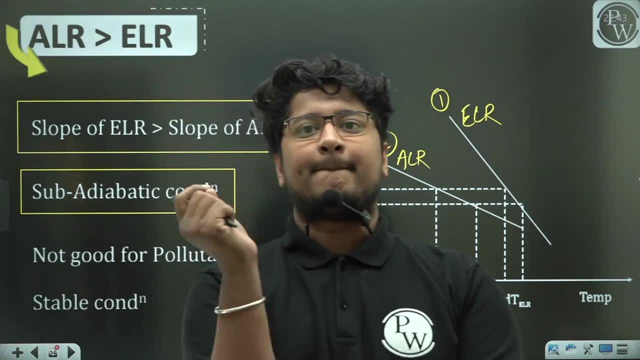 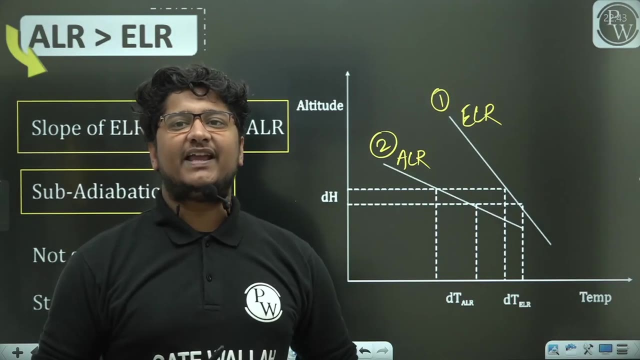 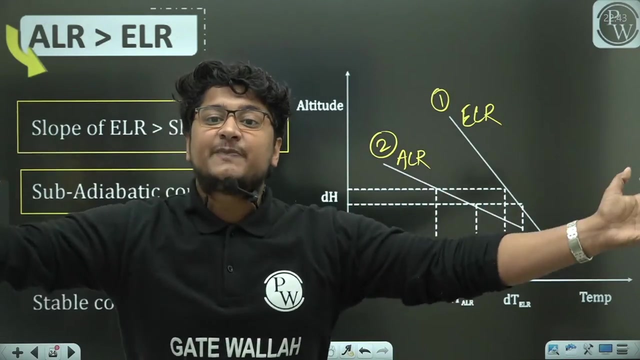 going with a 5 meter per second speed. What your thinking will be at that point of time? Quickly, Quickly, quickly, quickly. dada aapki condition: kya rahegi to decrease that part? that means, if a warm air parcel is going upward, aaspas ka jo environment ho bol raha hai rukhna. 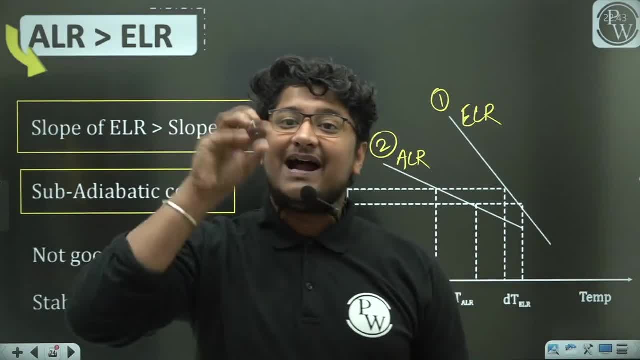 beta, kaha upar jaa raha hai, kaha upar jaa raha hai. so actually, in that case the environment is not helping you. aur jab woh help nahi kar raha hai, environment to aap, kya hoga? 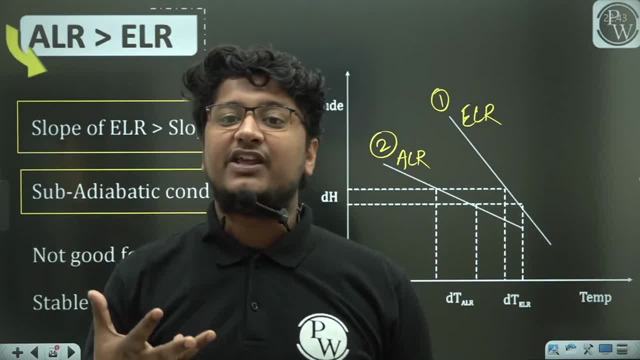 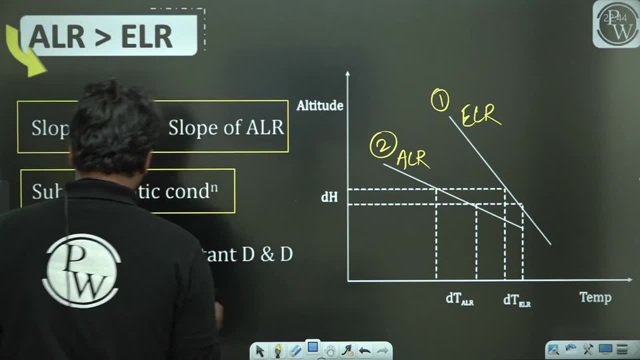 aap jaada height tak nahi jaa pahogi, but the better mixing aapki nahi ho paegi. that condition we call as sub-aerobatic, and it is not bad, but it is also not good, so this: 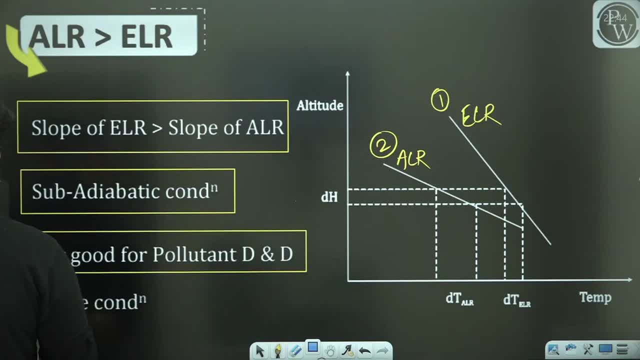 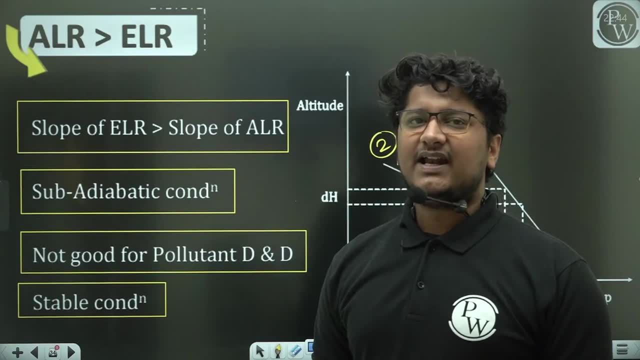 is what we have written. not good for pollutant dispersion and dilution. this condition also we call as stable condition, this condition we have named as stable condition, is that clear in this pollutant dispersion and dilution will be there, but not good. good, toh bolenge. 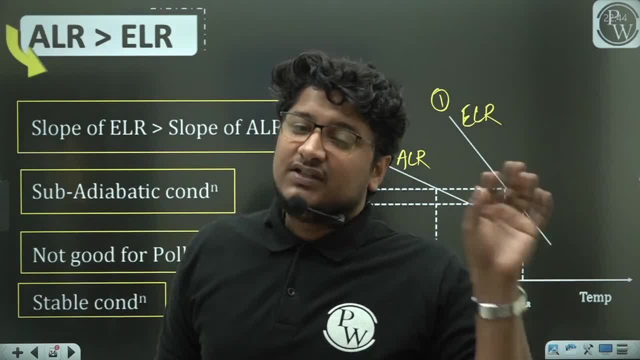 hi nahi not good, bad bhi nahi. bol rahe hain tarafat, So not good bolke chhod rahe hain toki behtar aapki isme nahi hoge, dekho ki isme aap kaise. 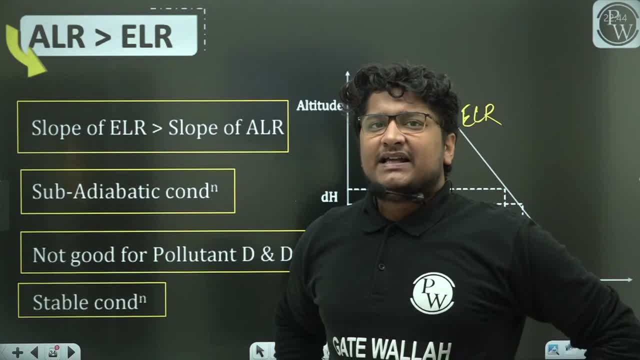 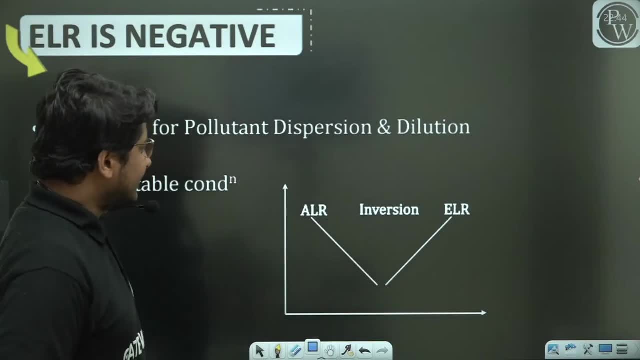 ho rahe hai. aage mai aapko u bhi show karo case samajh mein aaya, chalye going for the third case. aap dekho, third case ki beauty dekhna. ek baar third case ki beauty dekhna. 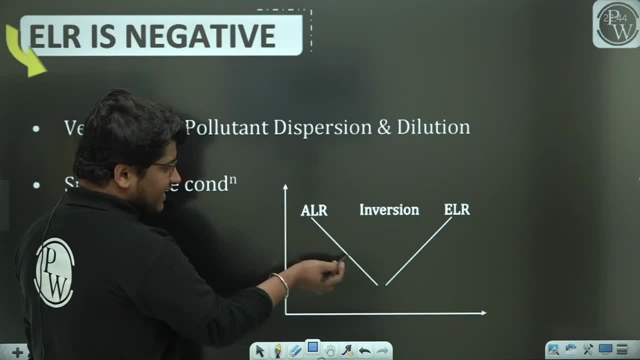 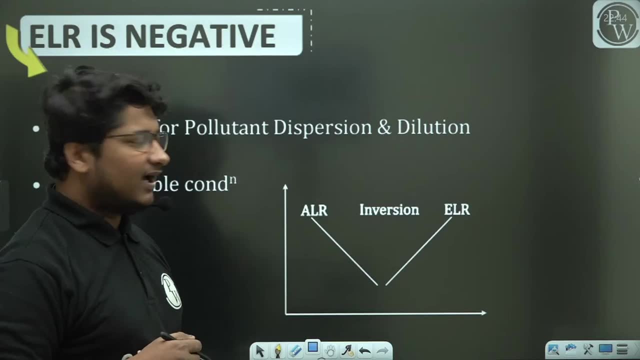 ek baar, sir, ye hamara ELR idhar gaya hai. theek hai bhot badya, ore, ore, ore, ye nalaik kya ho raha hai. dekho, ye ELR toh kuch alagi direction me bhaag raha hai. dada, dada ELR toh. 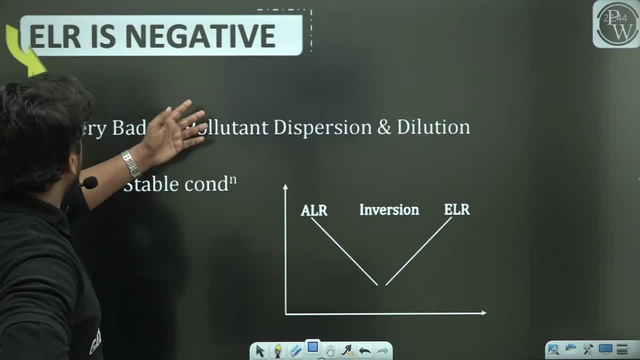 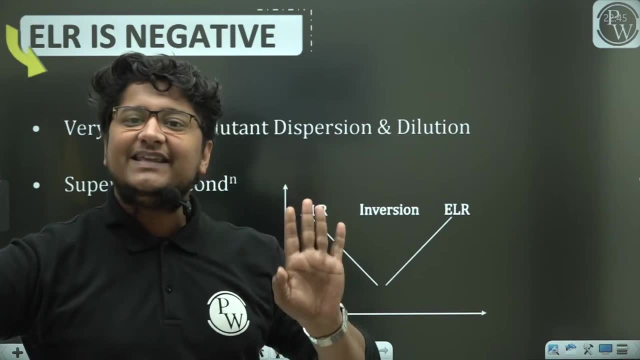 alagi direction me bhaag raha hai. Aur case ka naam bhi aap likhe hue. kya hai: ELR is negative. sir, ELR toh already negative hota tha. ye aap case ka naam kya de diye ho, toh haan, ELR already negative hota tha, kyunki. 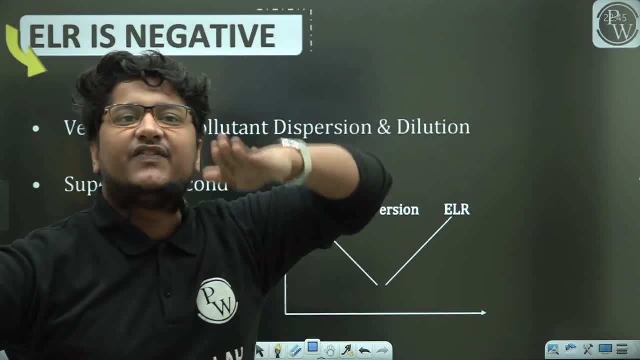 aap jaisi upar jaate, the final value aapki kam hoti thi. let us say, 15 hai usse upar gaye, toh aapko 14 ho gaya, toh ELR ka value negative hui hota tha. lekin jab o case ka. 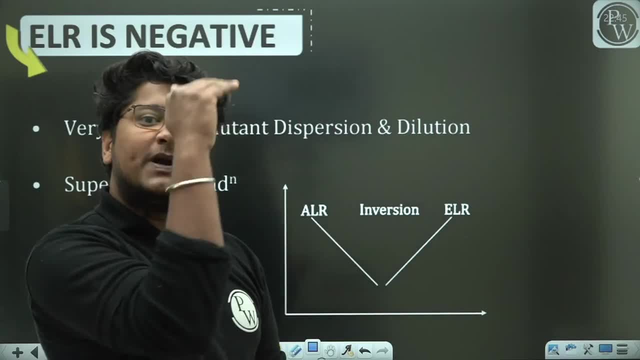 hi naam ELR negative ho gaya hai. iska matlab, jab aap upar ja rahe ho, toh temperature bad raha hai, matlab final value aapki jyada ho rahe hai. aap dekh bhi sakte hain figure. 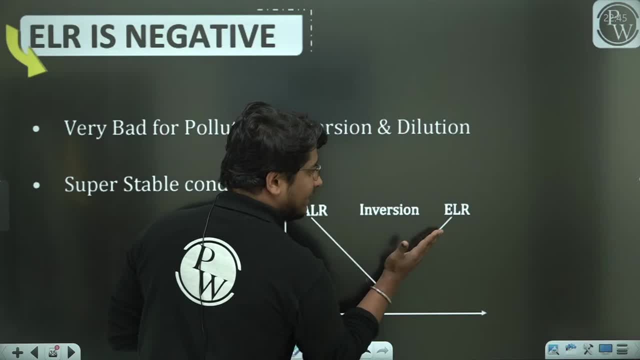 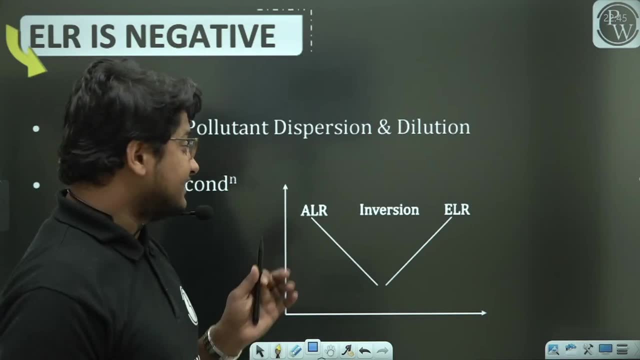 me Ki, ELR, jaisi aap height badha rahe ho, apna temperature badh raha hai. jaisi aap height badha rahe ho, aapka temperature badh raha hai. now this condition, we need this condition. 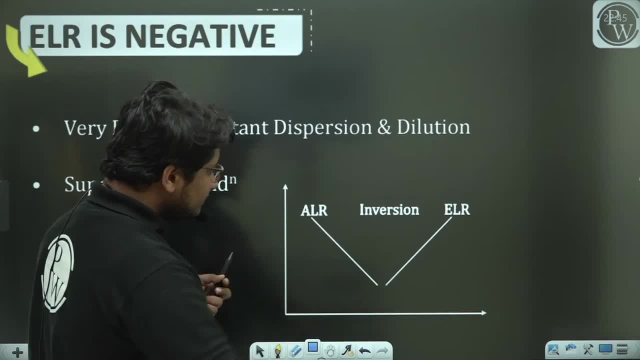 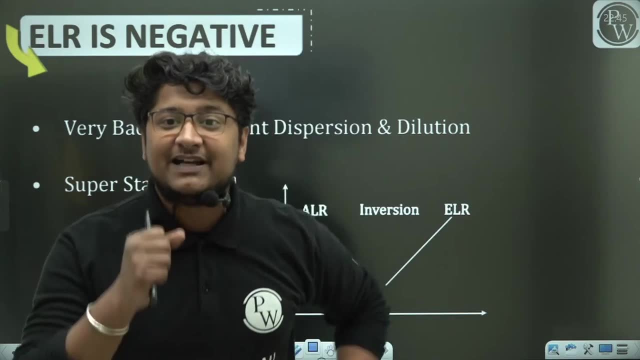 we are going to see the beauty. kya beauty hai, sir. dekho: ELR, alag, ELR, alag. ab firsai si example, ko samjho: you are going with a 20 meter per second speed in a east direction. 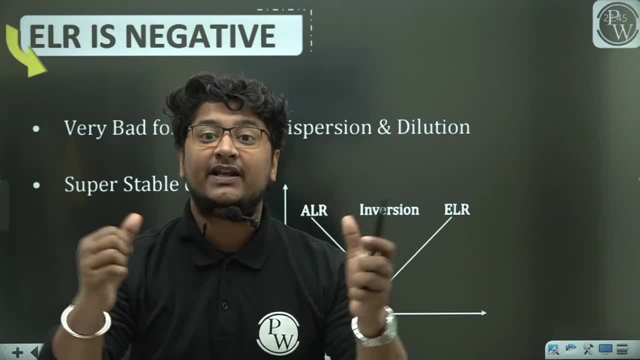 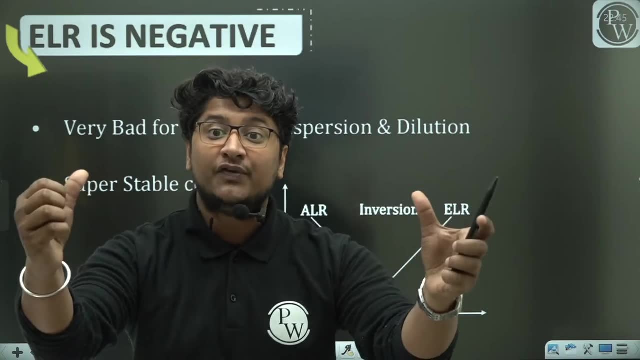 in a east direction and all your friends are going in with a, let us say, 5 ki speed se jaa rahe ho, yaa 10 ki speed se jea raha ho with any speed, but all your friends are going in a opposite direction, opposite direction. what your thinking will be at that point of 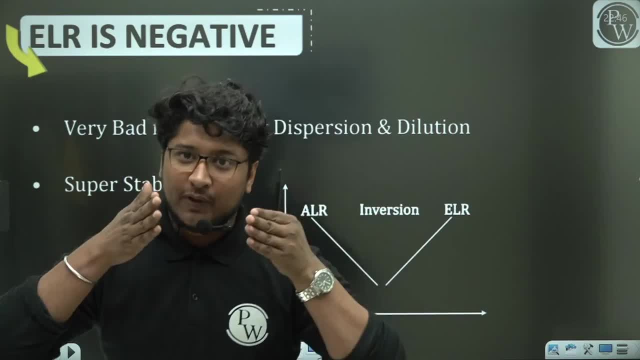 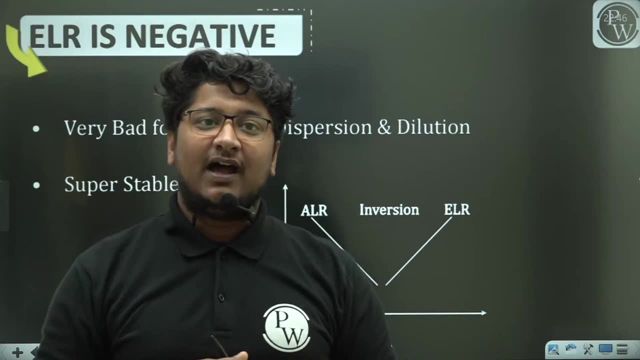 time. you are going in, you are in a race, you are going in this direction and you have seen that all your friends are going in the opposite direction. aapki thinking: kya rahegi? ah bhaiya, kahin khud pe self doubt, kahin hum galat toh nahi hai haan bakhi log. previous. 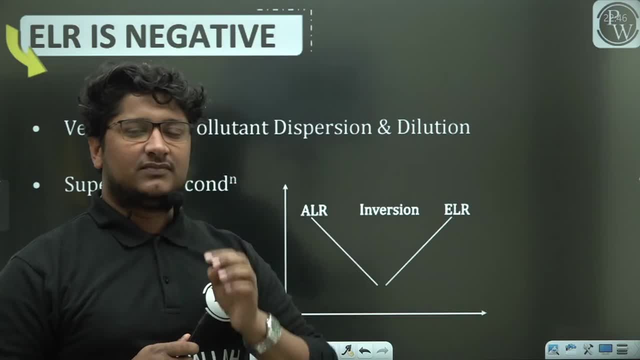 year question nahi bana rahe hain. mahi bhi nahi banata ho, yaar, ckoce previous year questionme kuchh aata raha tha. toh ye, se aapki joien aapko yaha sindhi ek hain, yaha hai, aba bhi ki kar hit bhi toh. 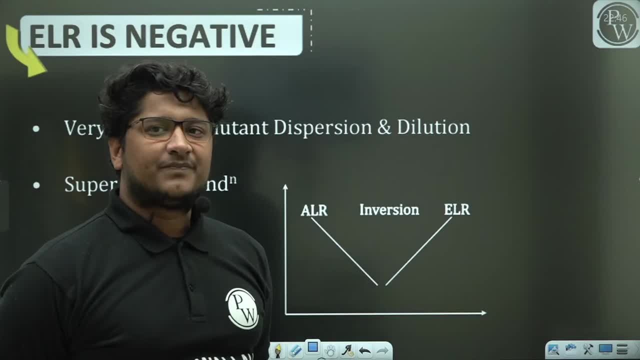 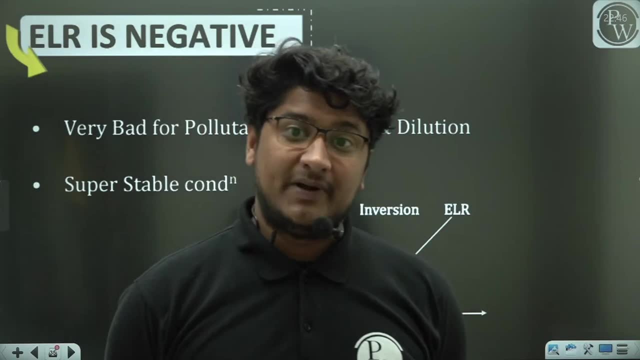 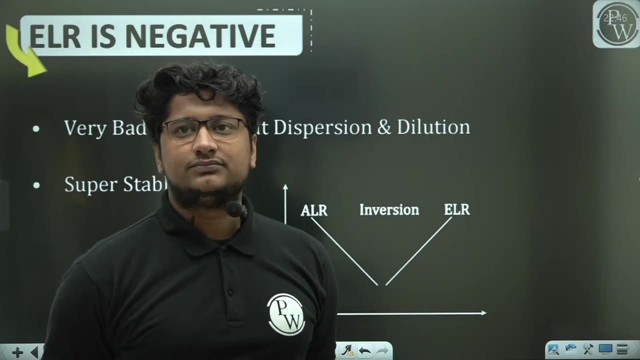 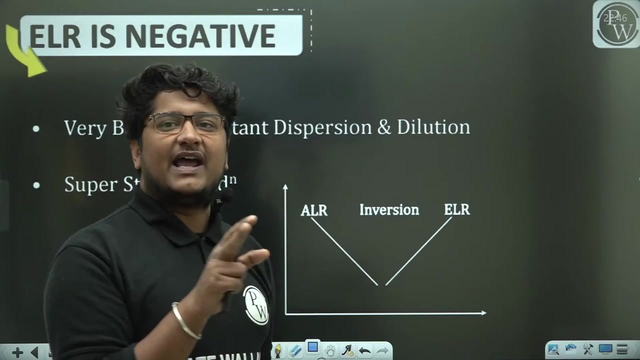 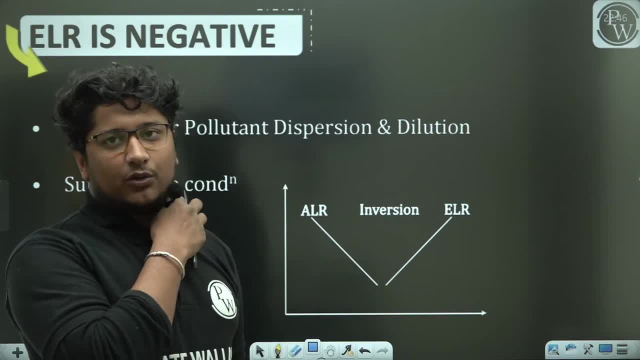 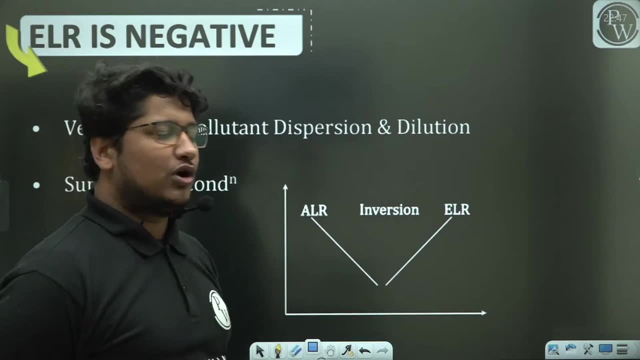 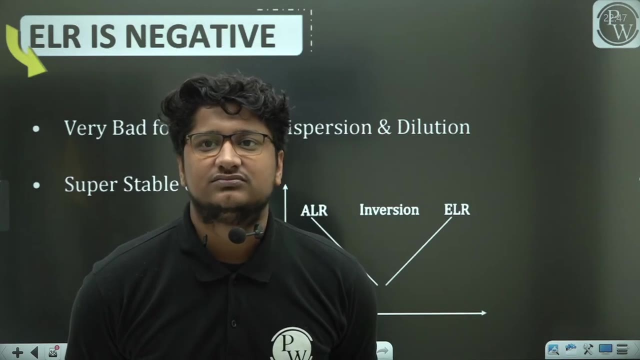 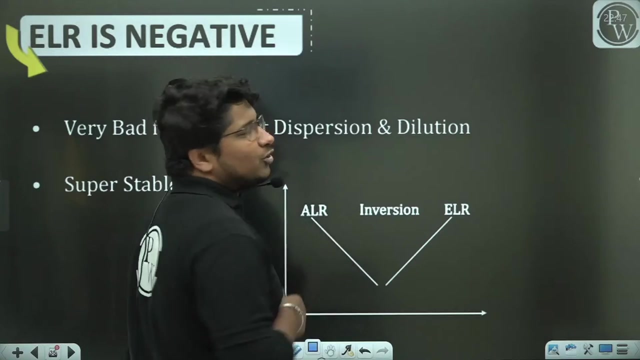 If you have a friend who is a motivator, someone who is a guide, there should be a proper group. then make that group. it will be made slowly, some people will be made in college. so what is happening in this way? that, brother, we have self-doubt. brother, it seems that we are going wrong. let's go back and start walking again. so, brother, we were going right, the rest of the neighborhood was going wrong, so we also took the wrong. it happens. 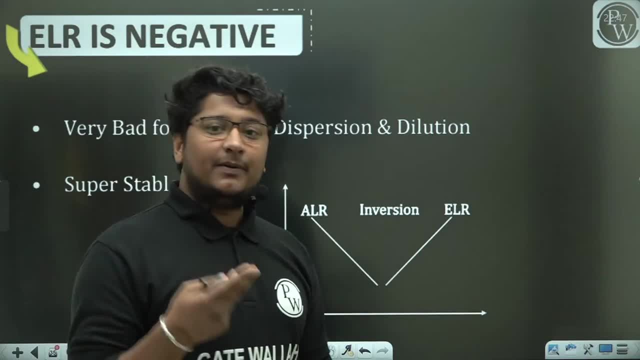 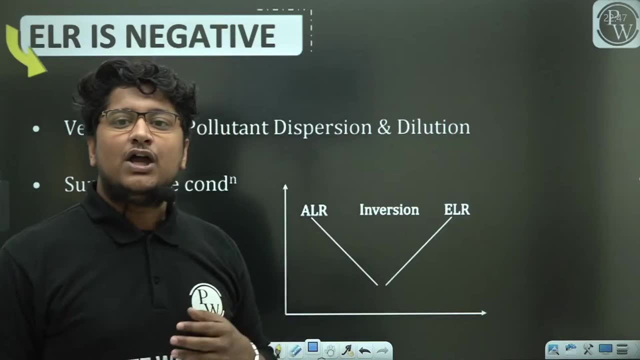 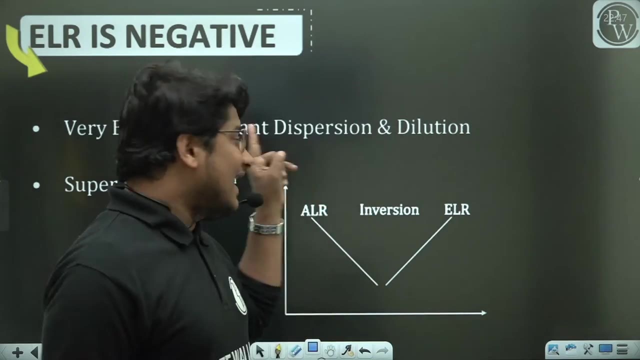 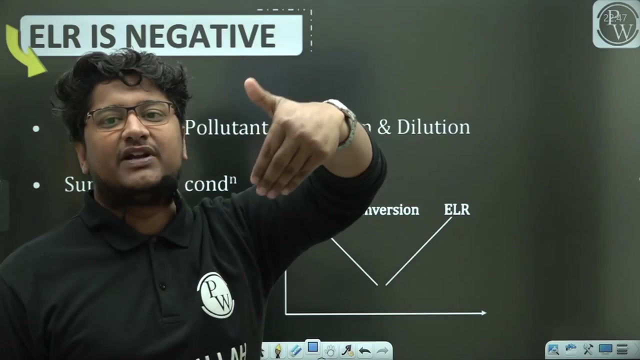 The same thing will happen with the gases also, that now he has his own ALR, but he got the ALR upside down. he got the ALR completely upside down. so you think in such a case there will be any mixing. this case we call as inversion and this case only happened generally happened in the morning time and that same case happened to you, which was released after the release of methyl acesonate. this same condition was developed in the morning, due to which more people died. 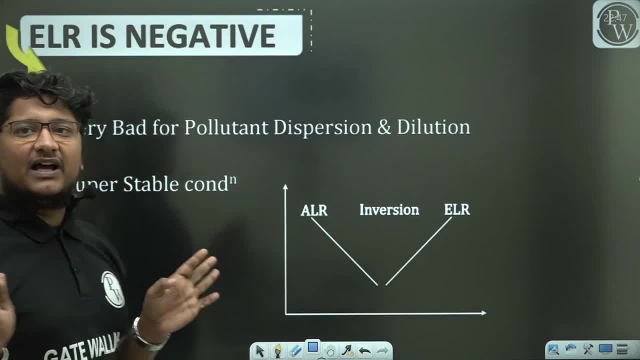 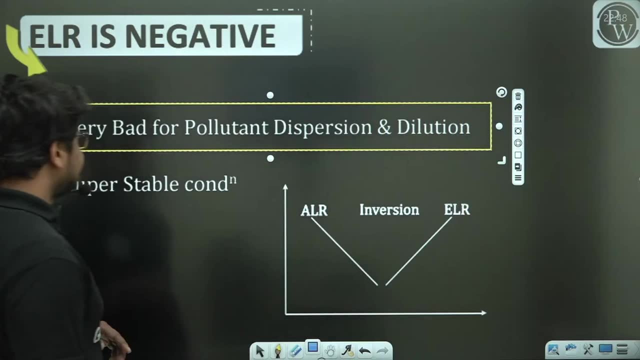 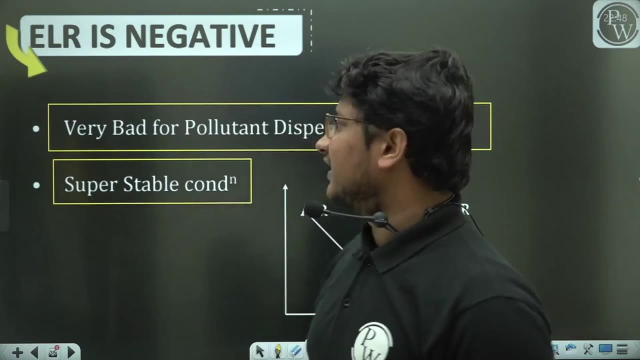 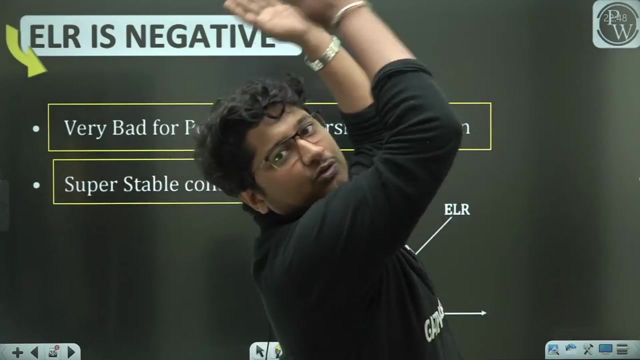 So you see, in this condition- in this you will also get wrong to say bad- this is called very bad, very bad for pollutant dispersion and dilution. it is super stable condition. no doubt, in this too, very stable condition, there will be no vertical mixing, no mixing like pollutant. you will remain the same. if your air is going in this direction, then air will move along with it. if air is going in this direction, then air will move from the air. no vertical mixing is allowed. 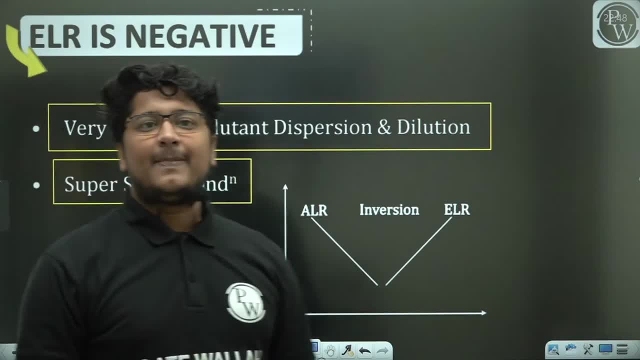 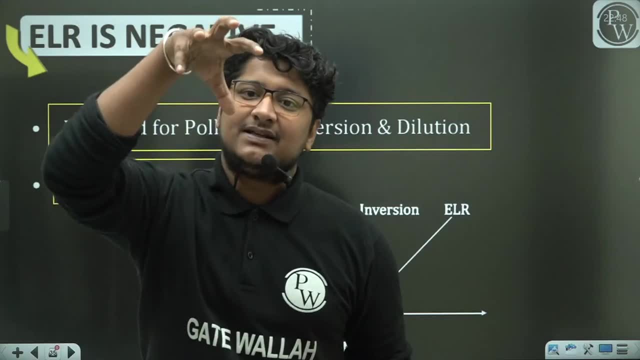 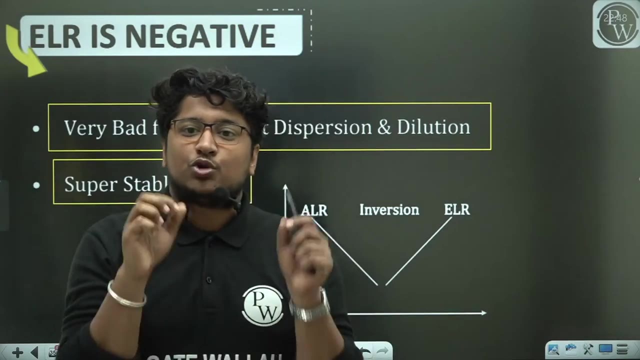 mixing. generally when this condition develops in the morning, when you go for running you feel slightly cold and sun is about to rise. when sun is in the part about to rise, then sun is sending its rays to you. so the upper air mass is little hot. the lower mass 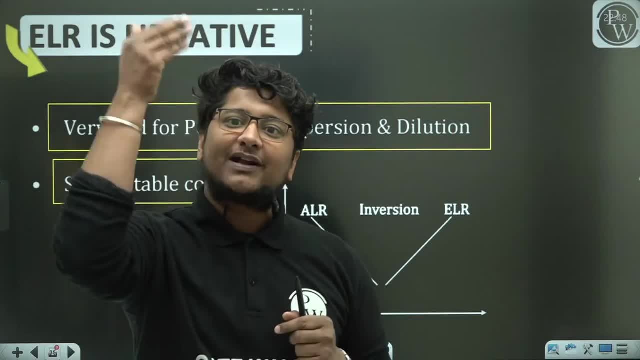 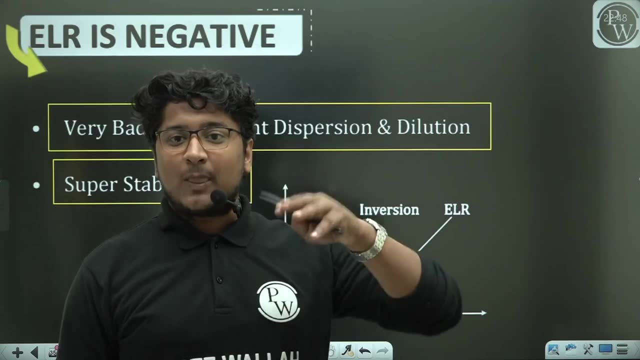 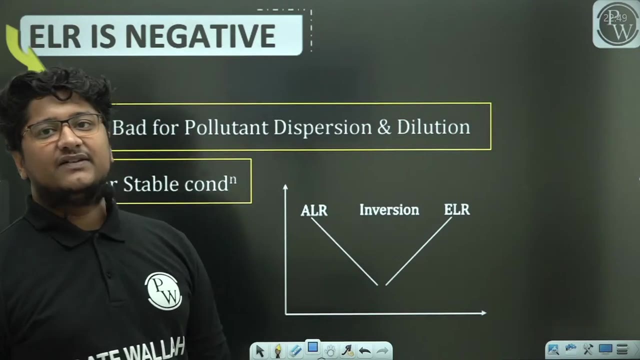 is still cold. so the lower cold and upper hot as you go up your temperature will increase. so in that case you will find ELR is negative. that means when you go up your temperature is increasing and this condition generally happens in the morning time. so we call that condition inversion. 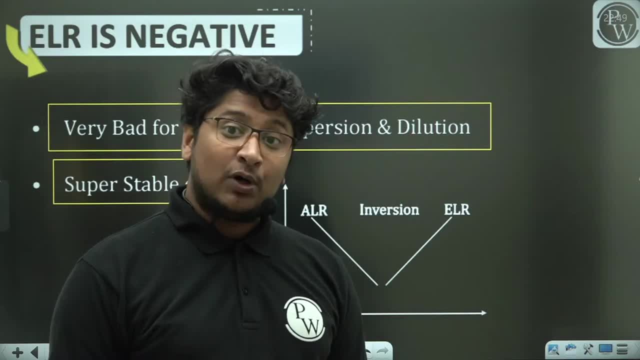 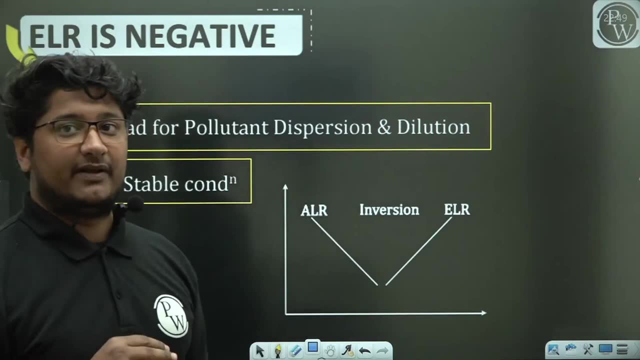 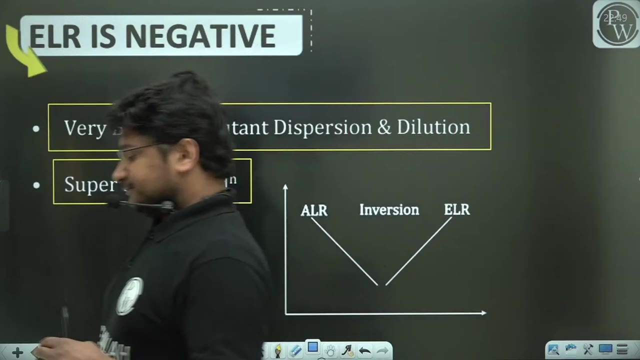 condition and nobody is allowed to emit any pollutant during this condition. if you emit pollutant in this condition, then it is illegal. it is dangerous for the human being or for any life. is it clear? is that clear? is that clear? is that clear? did you understand? 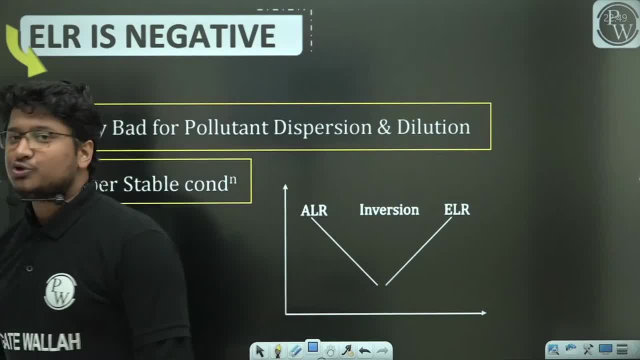 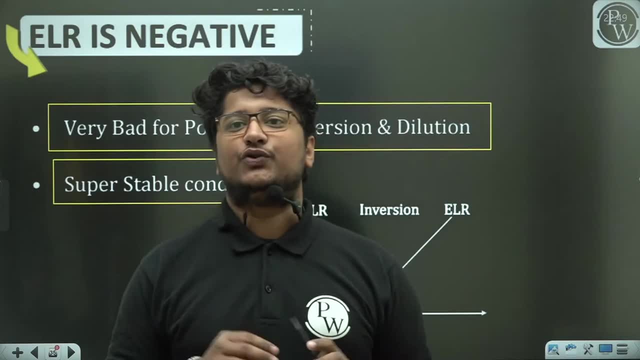 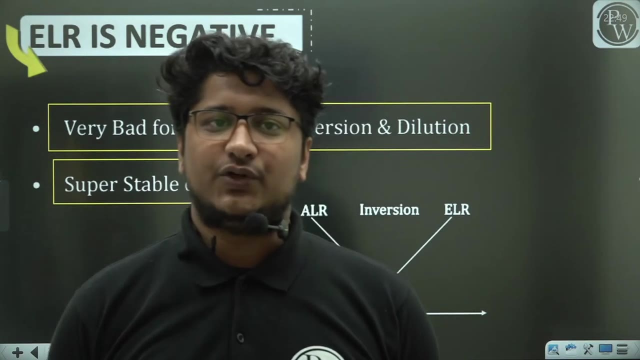 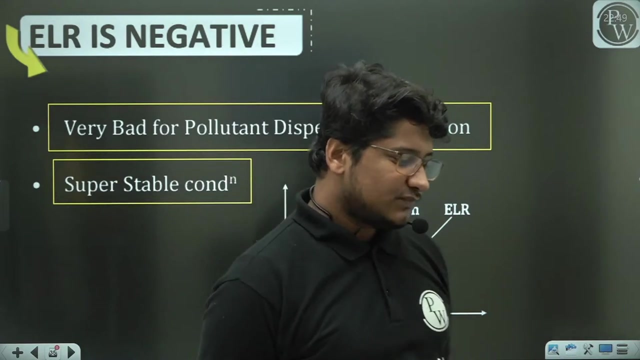 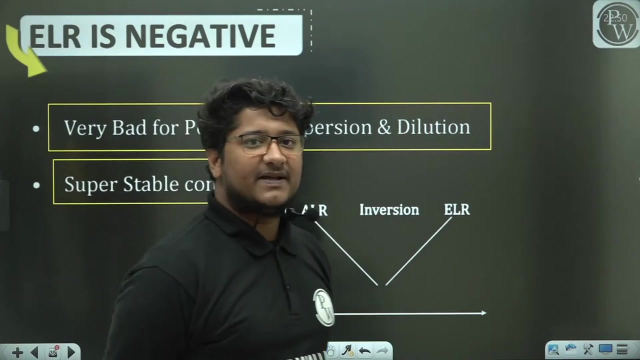 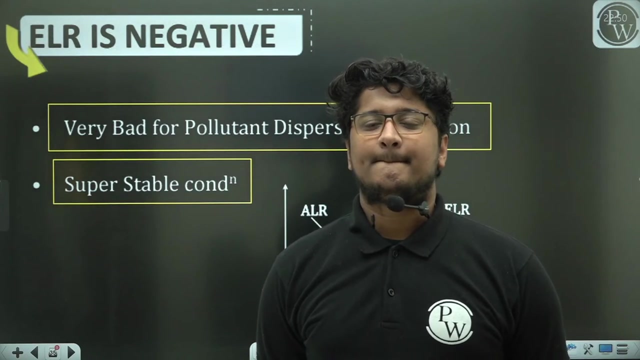 lets speak. did you understand? so if i ask you, in those three case that i have taught you which case you find beautiful, which case you find best for you, which case you find best for you, which case you find best for you, which case you find, case you find, but out of these three, so you have read three, so which one is the best? 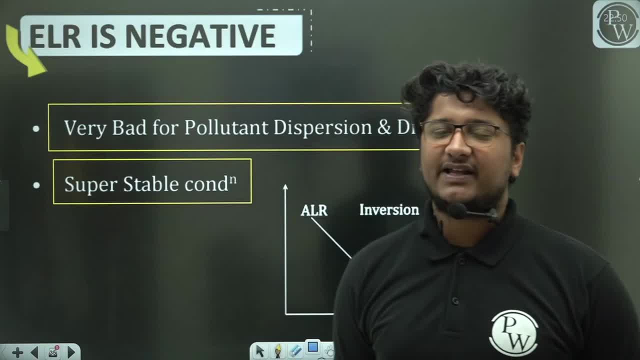 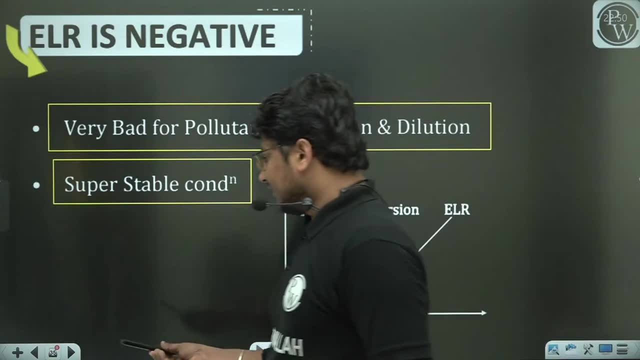 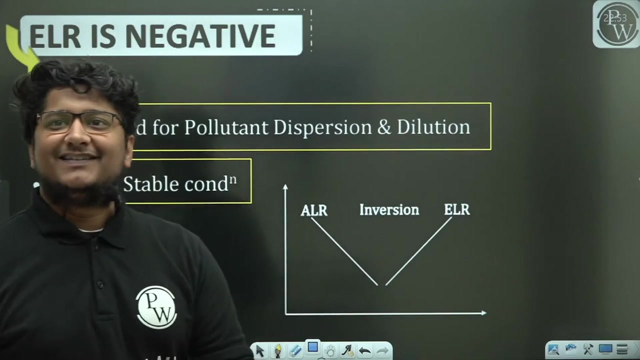 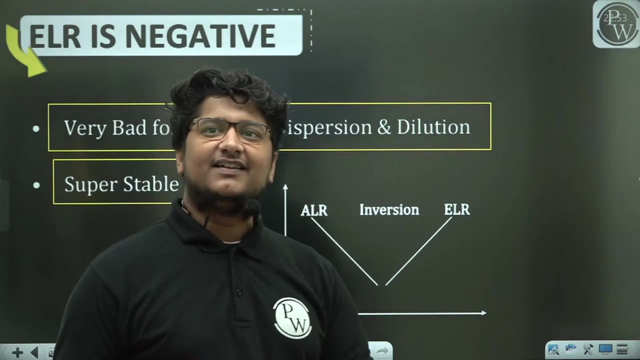 that is nothing but the for adiabatic case. for adiabatic case, that is the best. okay, just wait for two to three minutes. I will be coming back. you, you, you, you, you, you, what you, what you, what you, you, you, what you got. 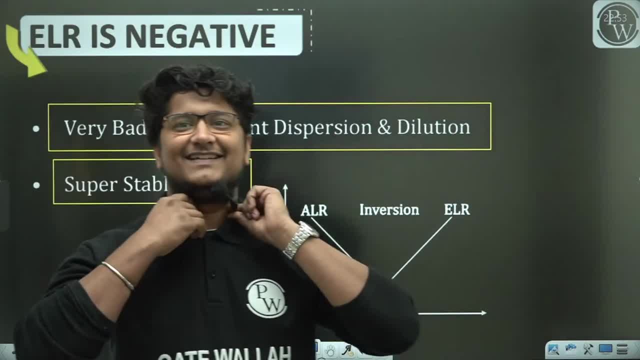 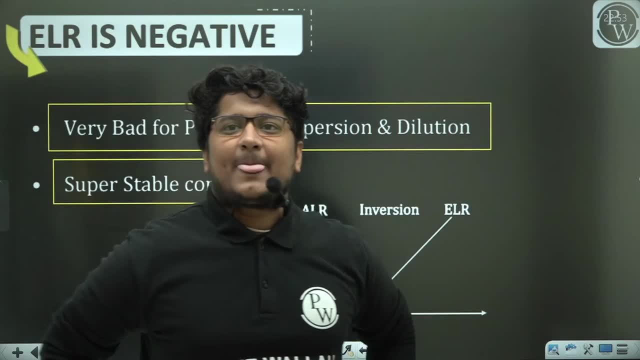 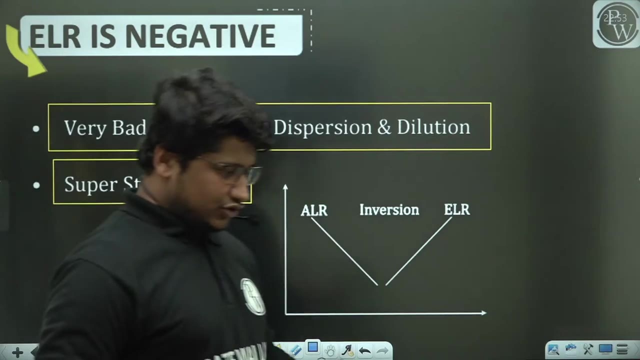 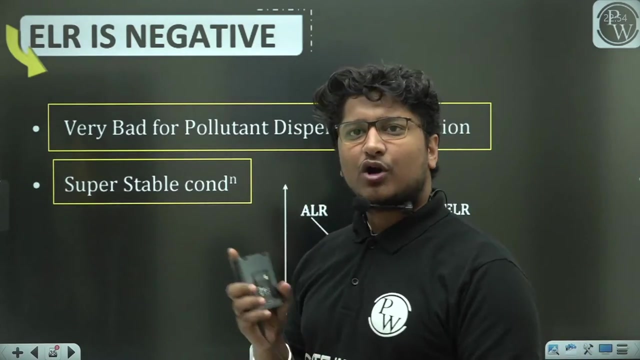 get ooh Big Chaudhary Saigas ki hai Chalo theek hai Start karen kahani. hai Chalo To hum log baate kar rahe theki regarding mock test, ki aap log baate kar rahe hai. 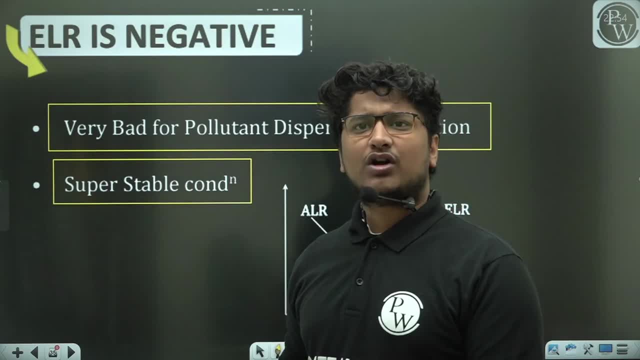 Mock test laga rahe ho testries. I think aapka 2 mock test kitne ho gaye, 4 combined test ho gaye hoge Kal hi raat, maine, kal raat Kal aap log ki class lini ke baad mai. 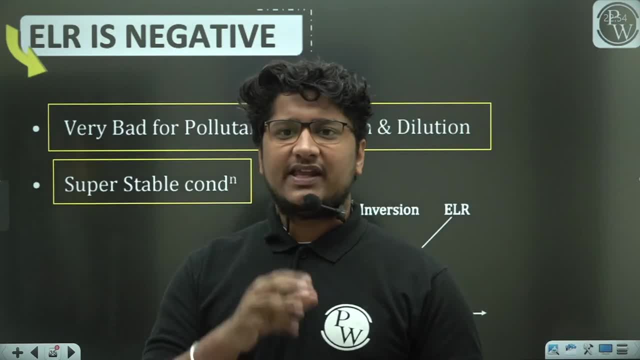 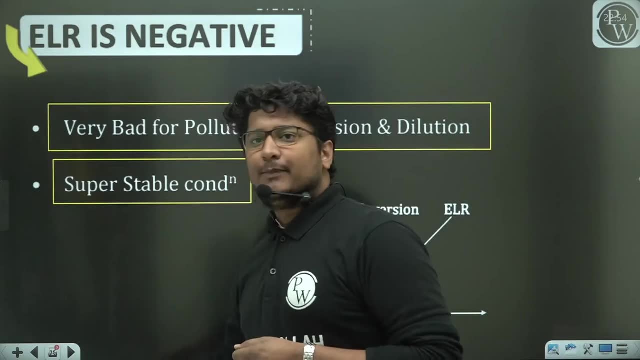 jo mock test second hai. uska maine recording kiya hai. kal 3 sare 3 ve raat tak wahi chalo Kal aapka mock test ka recording kiya tha. Aap log ki. class ke baad maine bola tha na aap log ko. 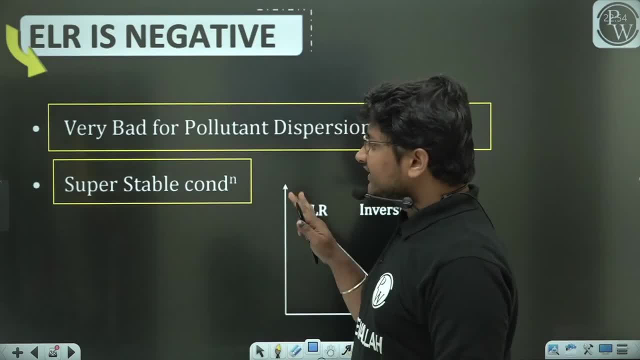 To baat karte hain. hum log Out of these 3, aapko pasand aaya kaunsa Super adevitic wala case wo aapko pasand aaya tha. Ab iske aage ki baat karenge. 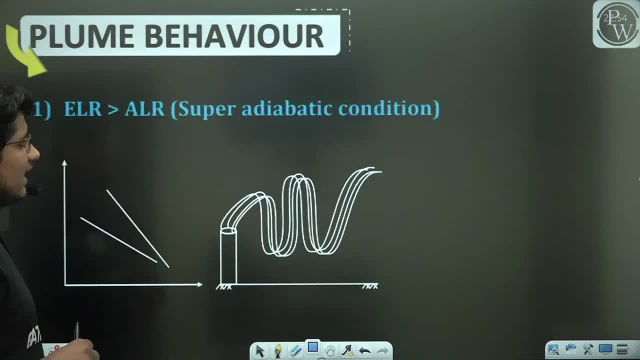 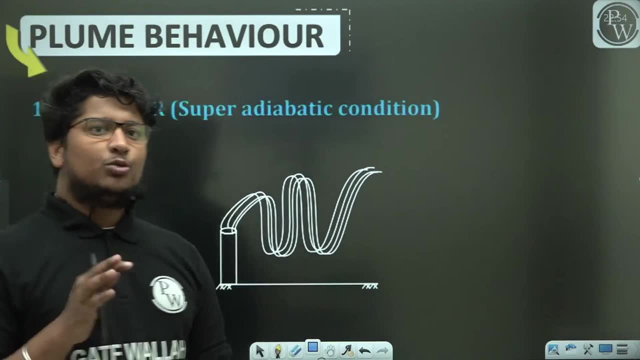 thora, so aur se To aap aata hai aapka plume behavior. Now next thing comes, which is plume behavior. To baat karte hain, agar plume behavior ki To plume behavior hai. kya, sir? 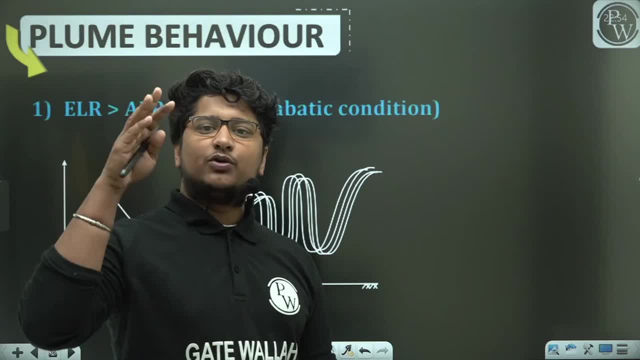 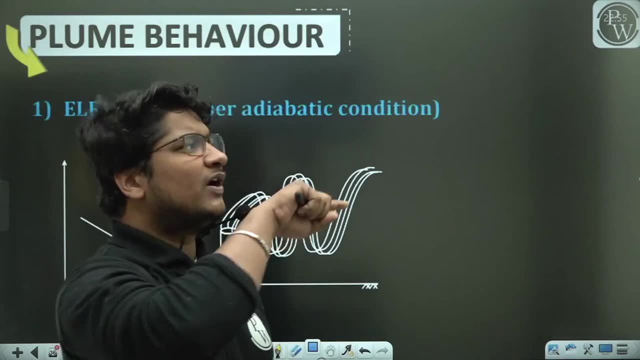 Pahle plume. kya hai? yahi samajh lo To aap log ne kabhi aise notice kiya hoga. Ek isse ghar mein, agar batti bhi jalate ho, na To aap dekho, usse dhuwa nikalta hai, kuch is tarike se. 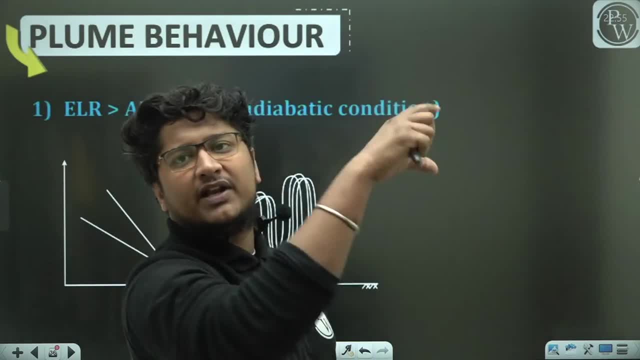 Yaar, fir jo log chimney ko dekhi hongi, usme dekhi hongi aapka dhuwa nikalta hai. Have you seen that thing? Dekhe hi hoge, notice nahi kiye hoge, Otherwise dekhe toh sab logo ne. 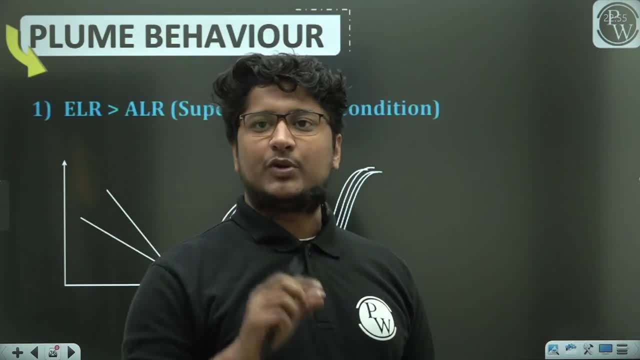 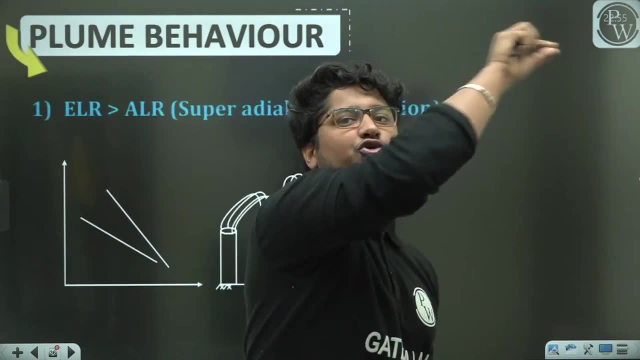 To wo jo aapka dhuwa hai. na usko, hum plume bol rahe hai. To ek technical word mein hum log plume bol rahe hai. Ab, wo jo plume hai, na wo din ka alag, alag time mein aapko alag alag behavior show kar raha hoga. 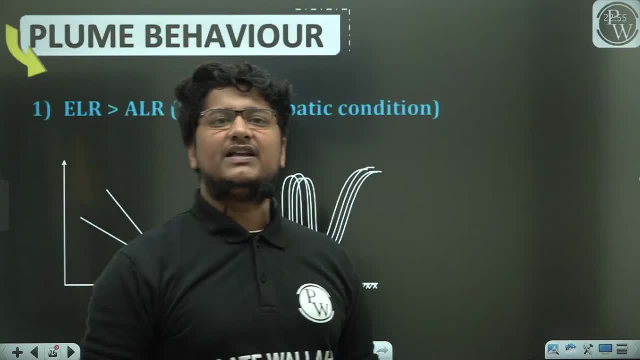 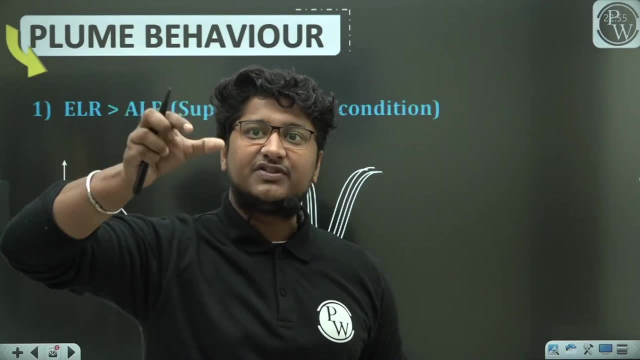 Smoke and plume are same nahi. Smoke jo aapko generally, jo koi chee aap jalate ho, na similar aapko dikhega Dekin. plume jo aap jisko bol rahe hai, Plume specifically hum kisko bol rahe hai. 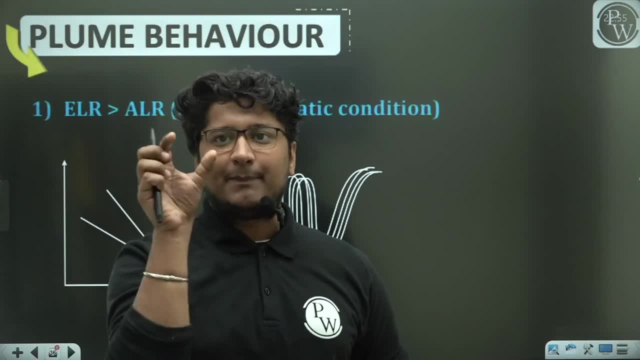 Jo aapki chimney se toh aapko dhuwa nikalta hai. Usse Usko aap, particularly aap, kya bol rahe hai? Plume bol rahe hai, Ab is baad ko samjho. 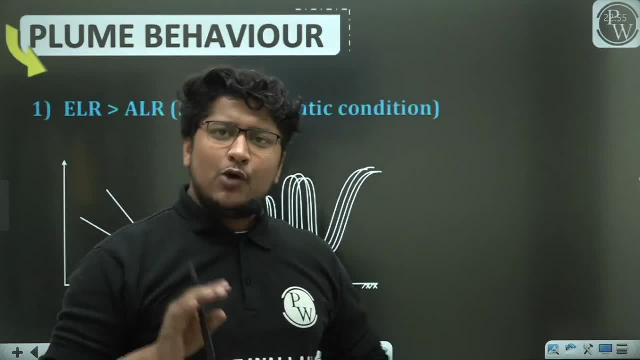 Yeh cheeze aasaani, se aapko samajh mein aajayi, Wo jo plume. aap dekhte hoge chimney, se aapko kayi baar idhar bhaag raha hoga. 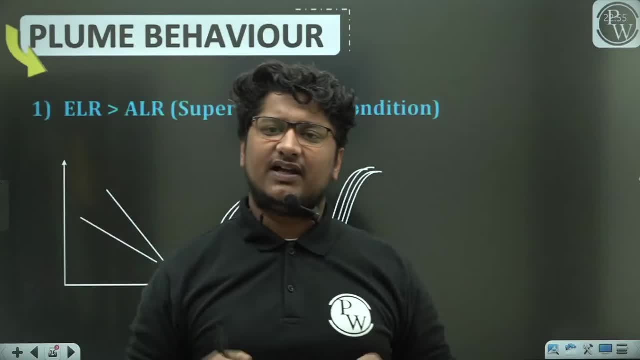 Kabhi aapko upar niche jaa raha hoga. Alag alag behavior show karta hai. To wo jo alag alag behavior show karta hai, Wo bhi kahine kahine depend karta hai aapko ELR aur ALR value pe. 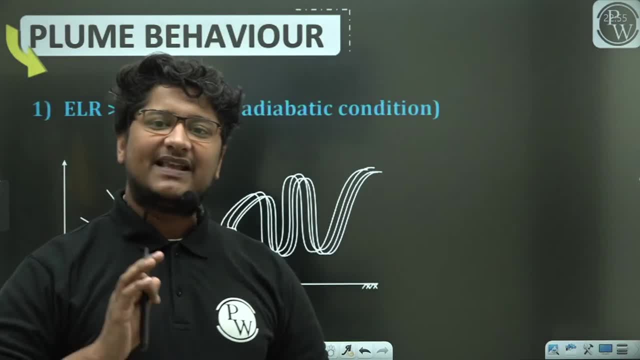 To ELR aur ALR pe aapko kaise depend karta hai, Uski behavior, kaise kaise change hoti hai, Ke baare mein baat karte hai, toh, Toh, pehla case aapka jo tha. 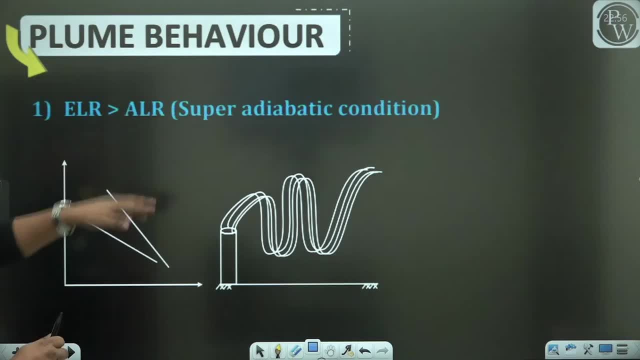 Super adiabatic wala case. Wahi case leke chal raha ho. mein ELR greater than ALR. Batani ki jorat nahi hai, Mujhe yaha pe kaunsa ALR hoga. 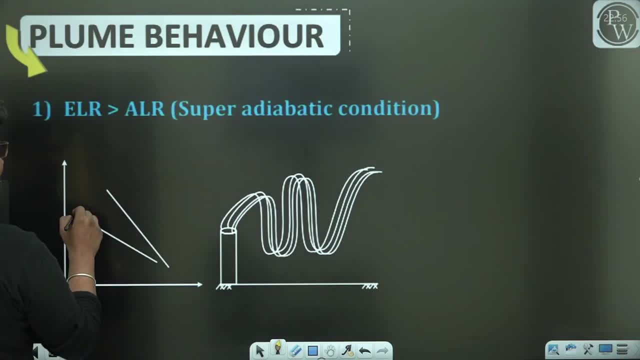 Kaunsa ELR, Jab aapka ELR bada hai. ALR se toh obvious hi baat hai: Yeh aapko ELR hoga Aur yeh aapka ALR hoga Aise case mein, agar aap koi pollutant emit karoge. 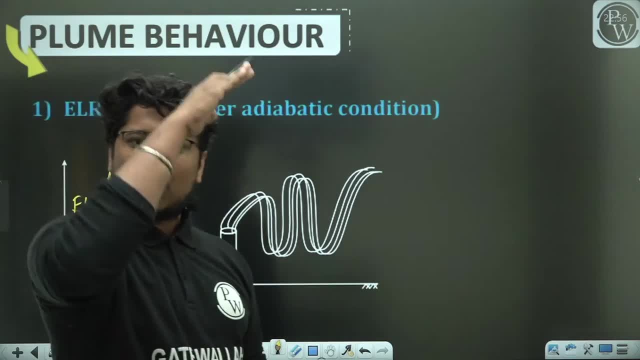 Toh yeh pollutant. dekho kya hoga Aise case mein. kya hai Vertical mixing bohot badyaan ho rahi hai. Toh aise case mein aapka pollutant niche bhi jayega. 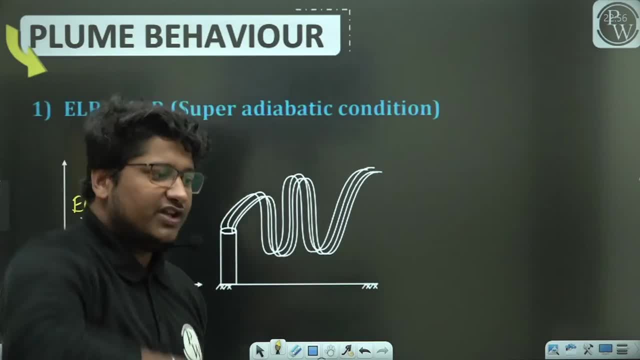 Upar bhi jayega Vertical mixing mein se upar hi jayega, Aisa thodi hai Niche upar, niche upar, niche upar. So it is something going like this. It is something going like this. 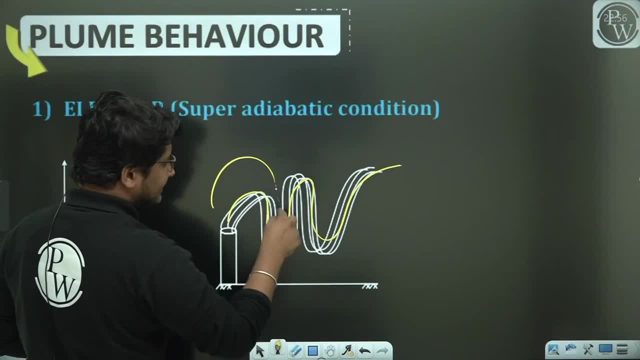 Toh, yeh jo aapko kya kar raha hai, Woh looping kar raha hai, Toh is case ka naam bhi kya hua, aapko Looping, Aur aise case mein, Aise case mein. 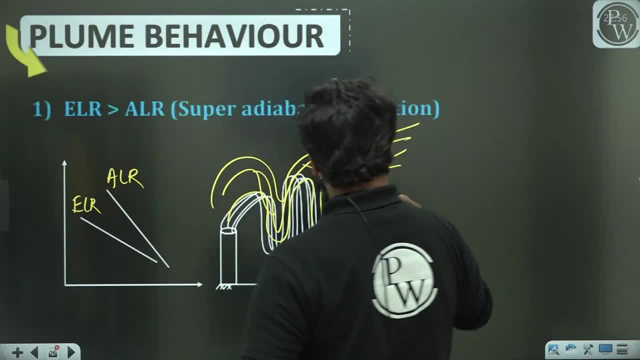 Agar hamare Vivek Chaudhary bhaiya Yaha pe. Agar hamare Chaudhary ji Chaudhary Bhagalpur side se hai kya Udhar Chaudhary Chaudhary. 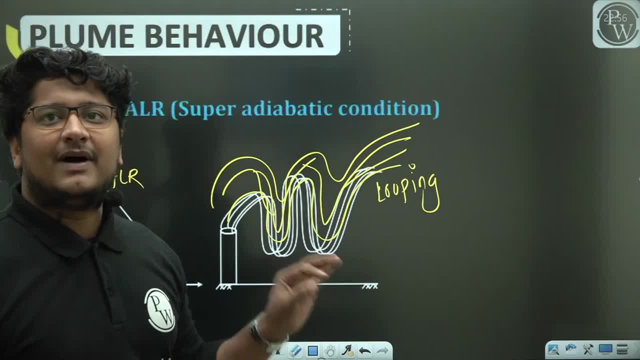 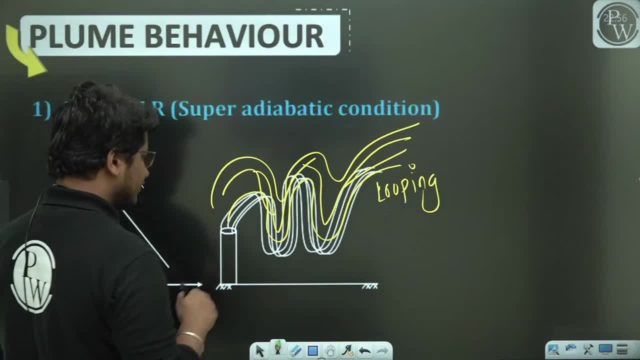 Yaha pe Agar hamare Chaudhary ji Chaudhary Chaudhary Bhagalpur side se hai kya Udhar Chaudhary rahte hai Jiada tar Chalo Agar hamare Chaudhary ji yaha pe hungi. 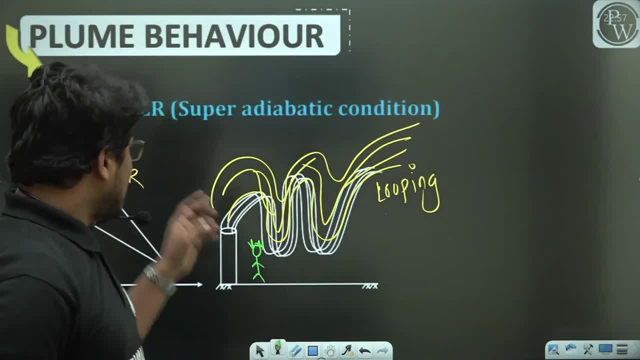 Toh aaapko lagta hai, Chaudhary ji kal ki class mei rahe paayenge Aise condition mein, agar Chaudhary ji yaha kharre hoke brush kar rahe hongi subbh, subh. 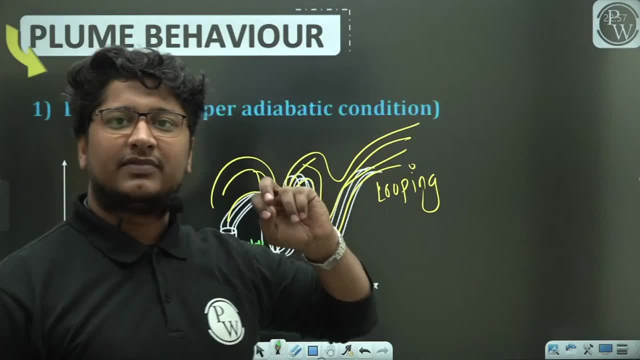 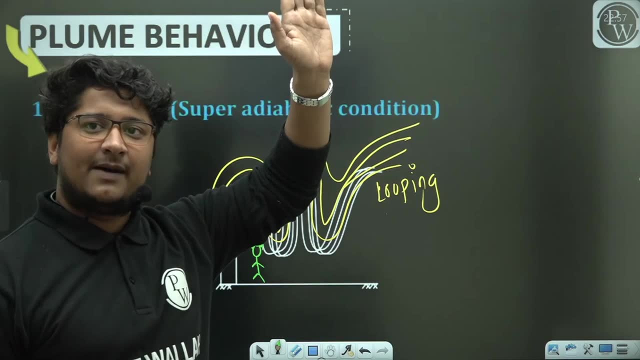 To lagta hai ki kal ki class mei hu brush kar paayenge. How many people think that Mr Chaudhary will be able to brush? Tell me quickly. Mr Chaudhary is not from Marwal, Let me tell you. 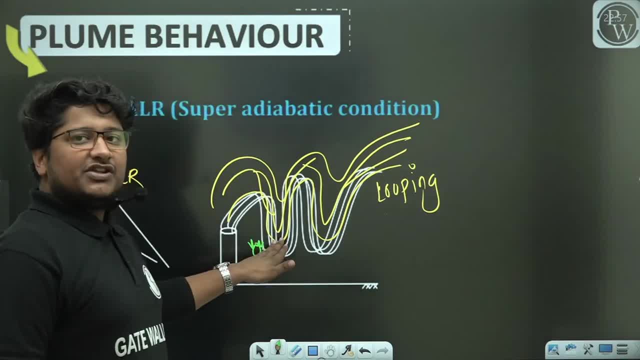 Mr Chaudhary is from Agra. OK, Very good, Let's go Now. you will understand that if Mr Chaudhary is in Agra and was brushing and he got such a condition, then will Mr Chaudhary stay in Agra tomorrow or not? 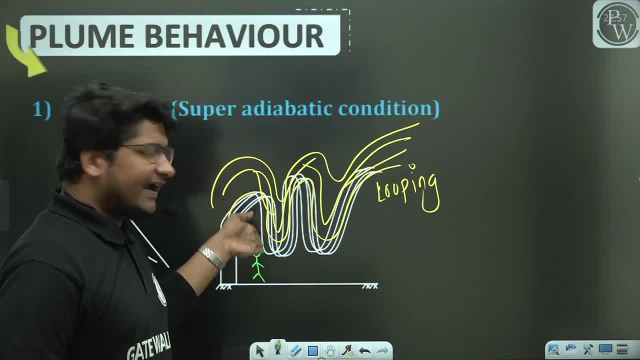 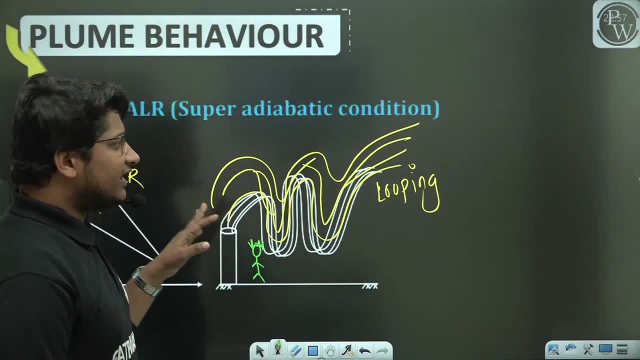 Will he come to class tomorrow or not? No, he won't be able to come Because, sir, he will have such a dangerous exposure. then it will be the last brush, Do you understand? So we call this condition looping And you were calling this condition the best condition. 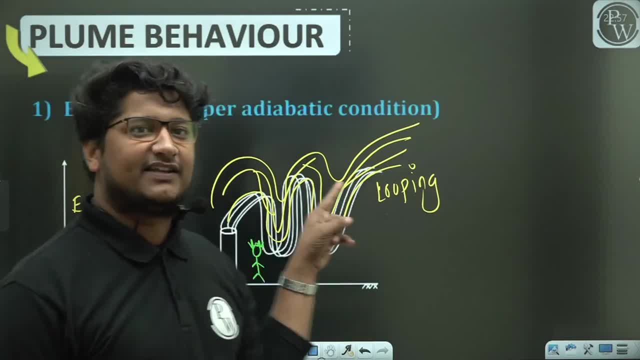 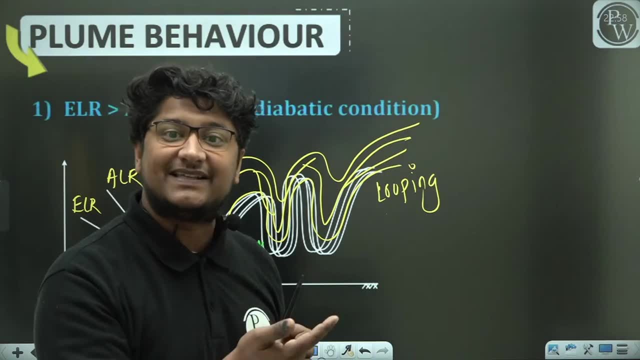 After understanding half the story. you were calling this condition the best condition. Who were you calling? You were calling the super adiabatic condition the best condition, Did you understand? So this is the best condition for vertical mixing. But vertical mixing, pollutant, dispersant dilution. 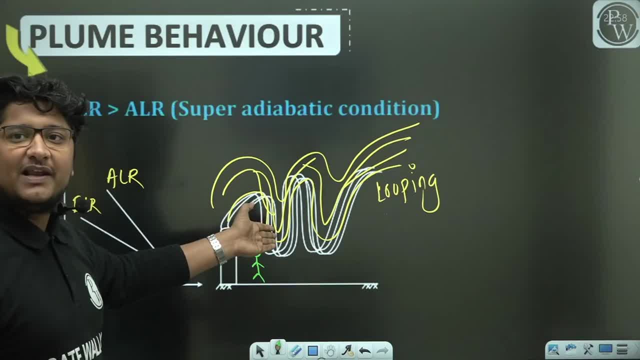 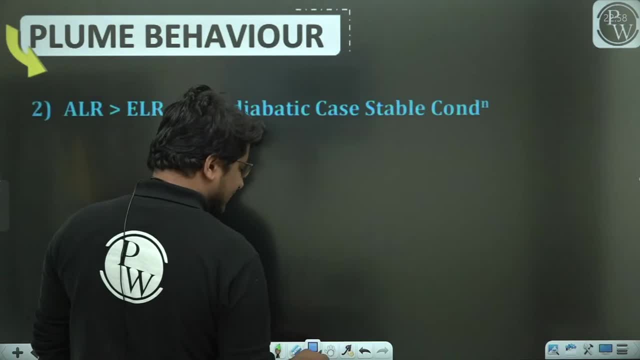 this will be good for you, But it can also be dangerous for you. It can also be dangerous. Second condition comes to you when ELR is greater than ELR, So its picture is not made. The naïve has not drawn, So we will draw. 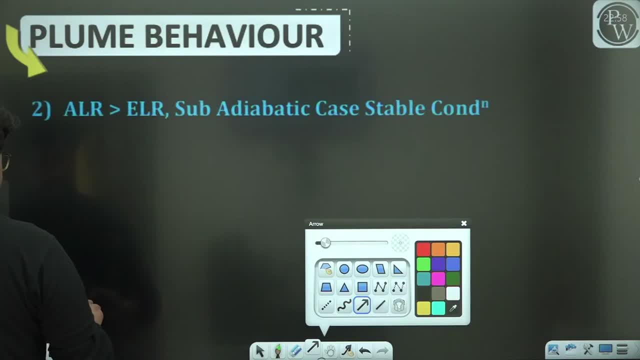 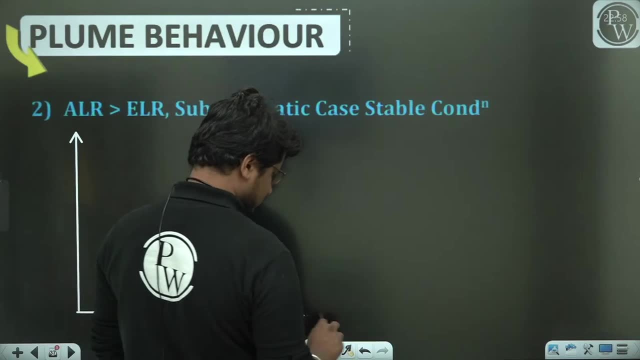 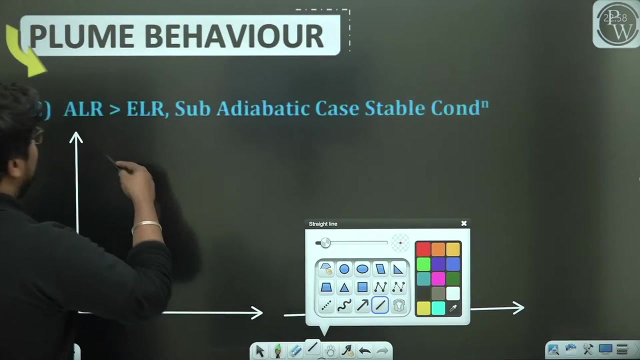 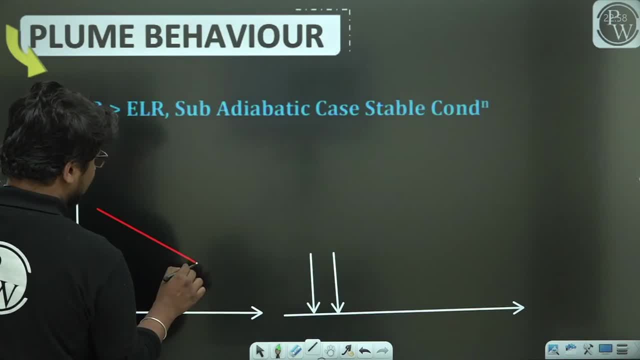 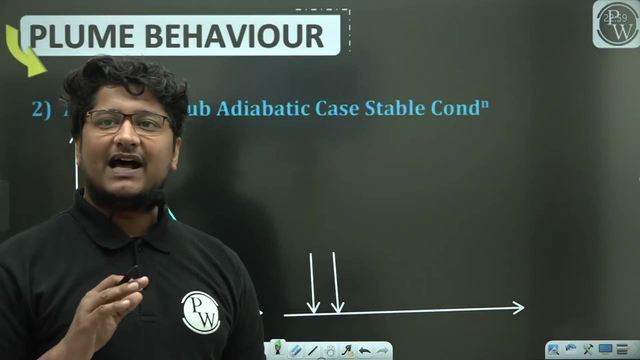 you have more ALR, then its slope is less. if ALR is less, then its slope is more upside down. let's go. what is such a condition, sir? sub adiabatic condition. now, today's syllabus will be over. no, son, today's syllabus will not be complete. tomorrow also your class. 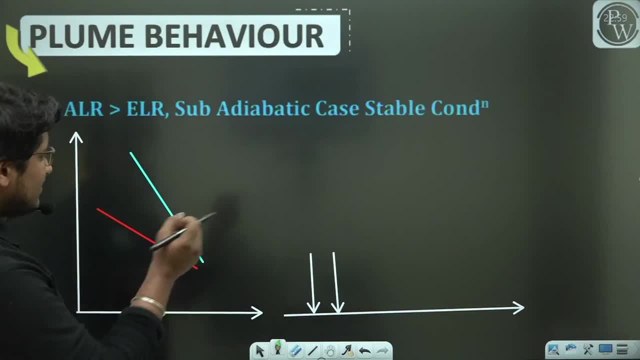 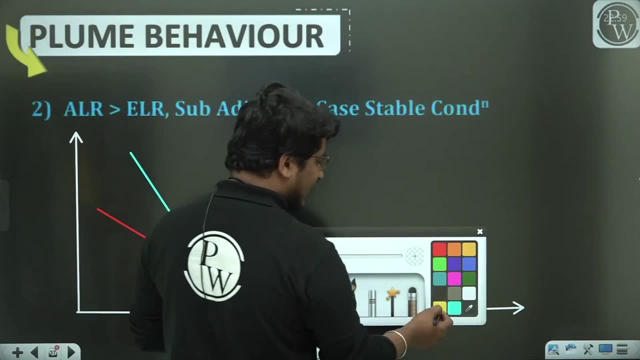 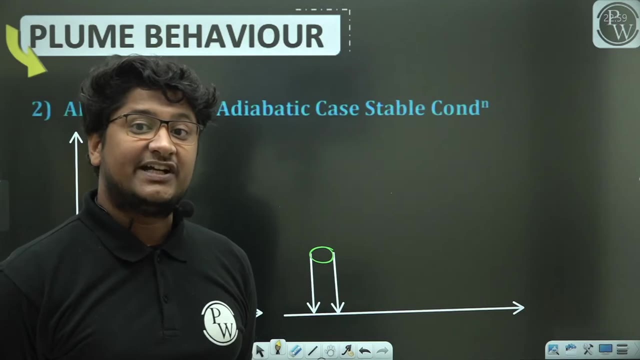 is of solid waste management. tomorrow your syllabus will be complete. now see, this is your chimney. this is your chimney. now, from this, sir plume will come out. now you tell me that in such stable condition, was vertical mixing good or bad? I gave you three conditions. 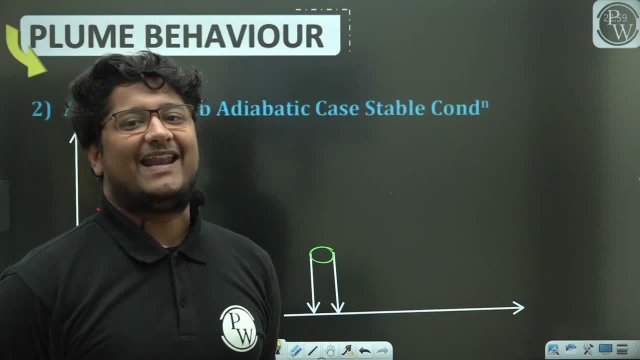 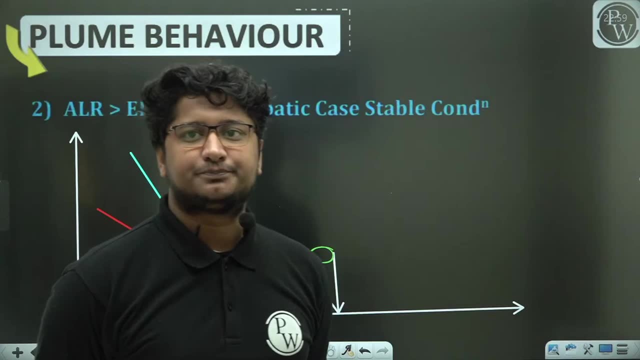 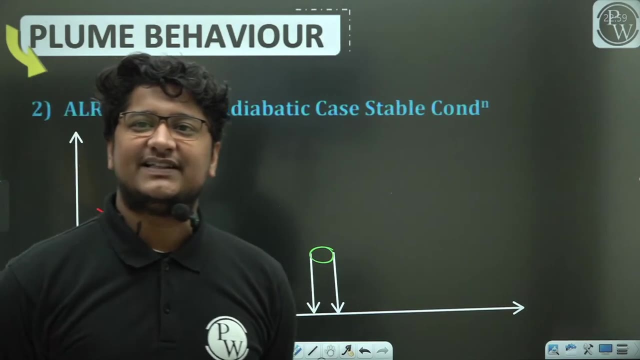 good, not good and very bad. you had three conditions. tell me which one will be: good, not good and very bad. all of you, All of you, all of you, Vikas ji, don't give your time and knowledge here. ALR equal. 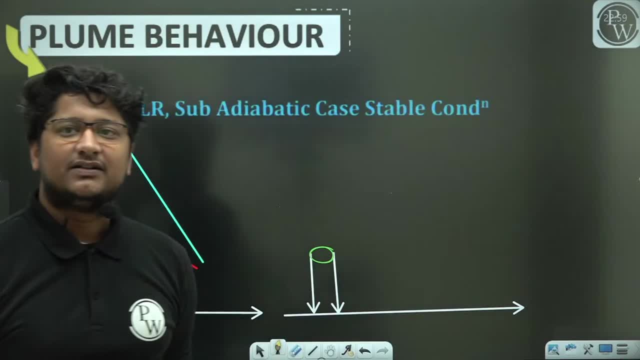 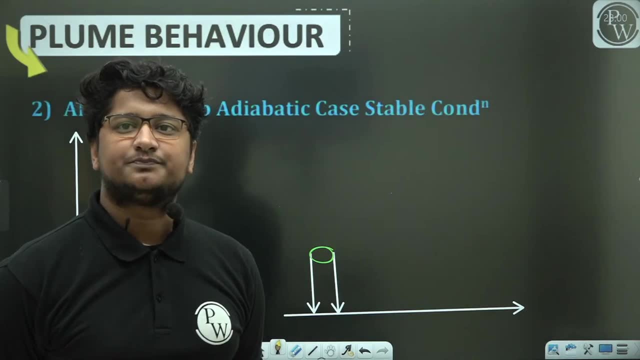 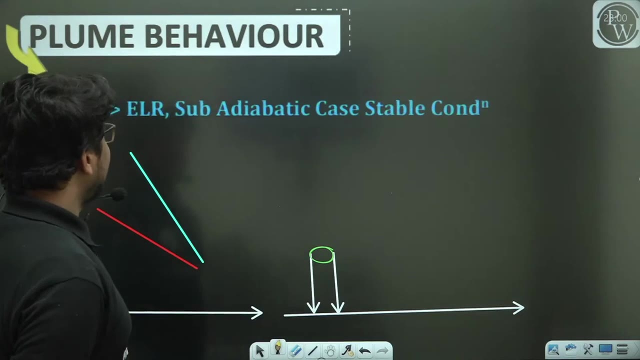 to ELR is the best condition. sir and Arpit ji, two minutes silence I will have to give for you. spelling of silence is wrong, very bad, useless. how will it be very bad. what is your condition? everything is adiabatic. not good will come in this. where will the 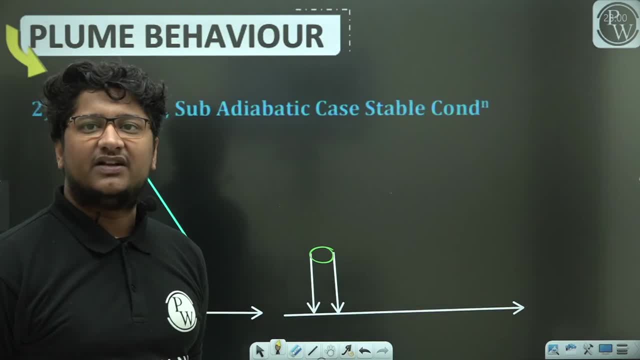 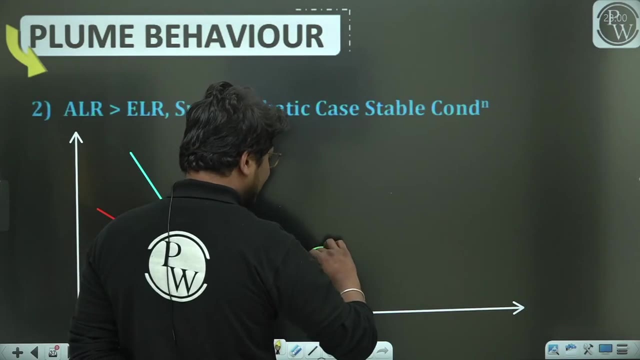 very bad one come from Adiabatic and Adit about inversion condition is not happening. it is not good condition, not good for pollutant dispersion in relation: will happen, but will small. sir, it will happen, but it will be small. so, in the sense that your pollutants coming out of here, where 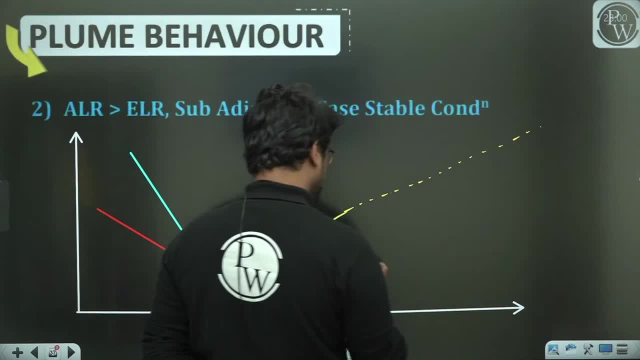 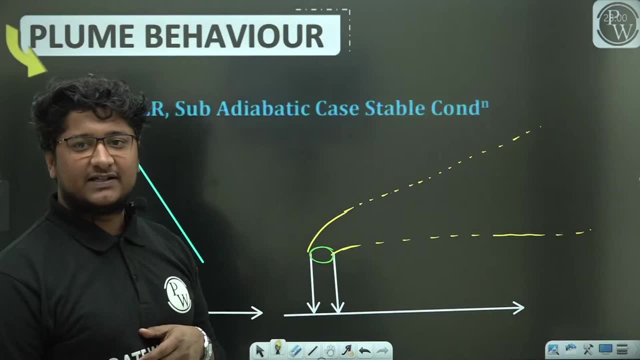 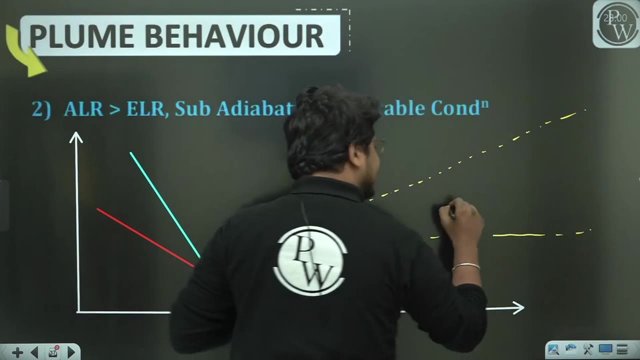 it is little bit more love. some foreigners are left. then small, small, smallா what you will do- vertical mixing. so it is something like making a cone. it is something like making a cone, so the name of this case will also be what you will get coning, the name of this case. 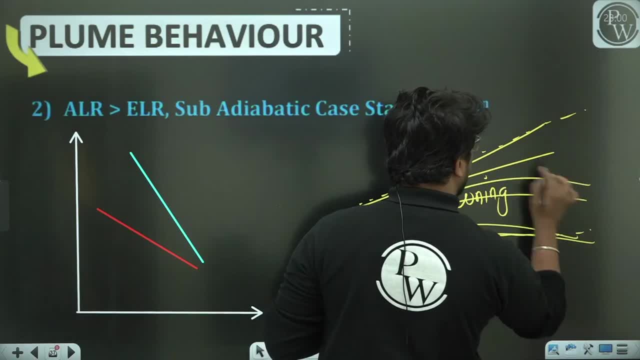 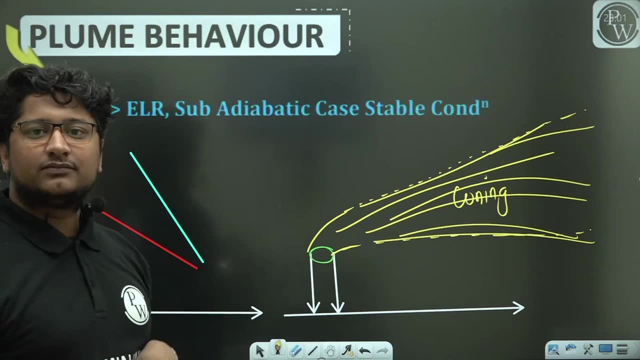 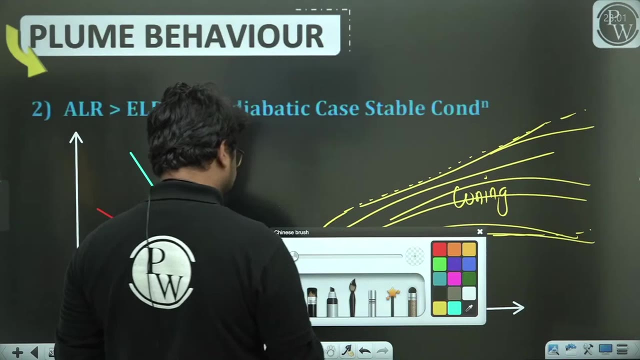 will also be what you will get: coning. in such a case, your pollutant will be going in this way. what is the name of this? coning? because it is making like a cone, so the name is also given: coning. ok, got it now again. to whom you willjoin this case? to arpatbhaiya, or to whom? 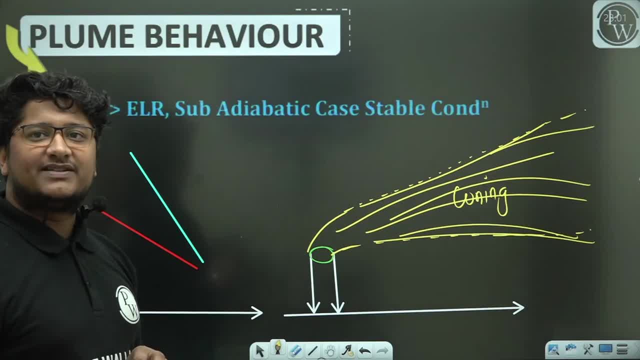 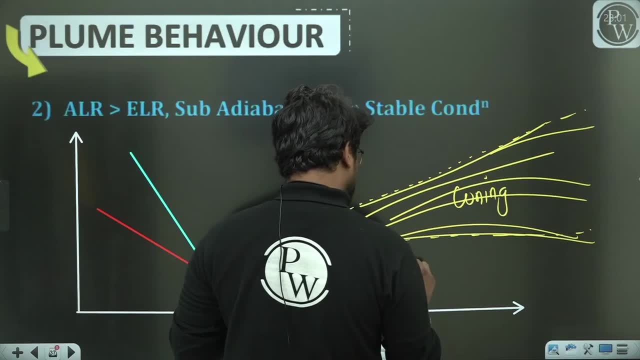 last time we joined to vivek choudhary. this time we join to Jobless engineer or pro. ok, wow, he also joined as pro in capital letter. so our jobless engineer is standing in the space. his hairstyle, I dont know. now he is female or male, I dont know. 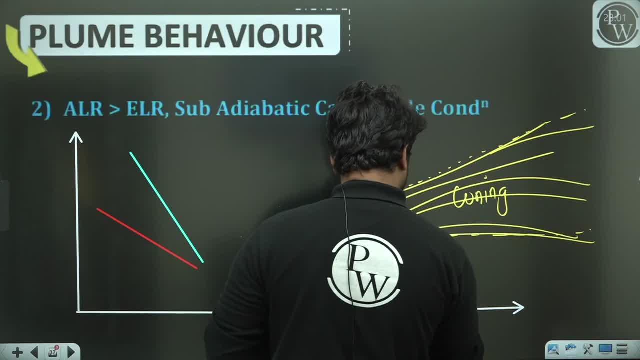 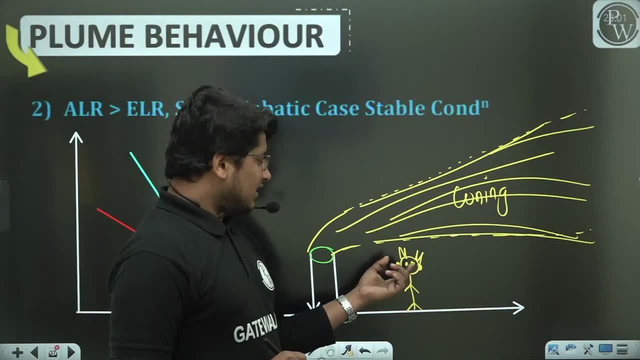 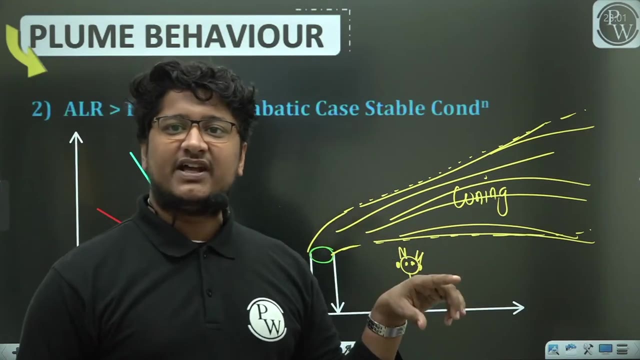 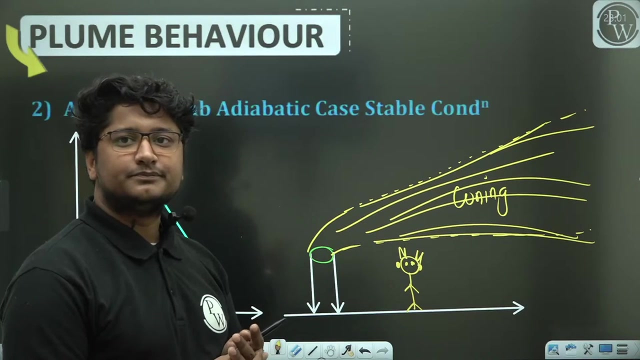 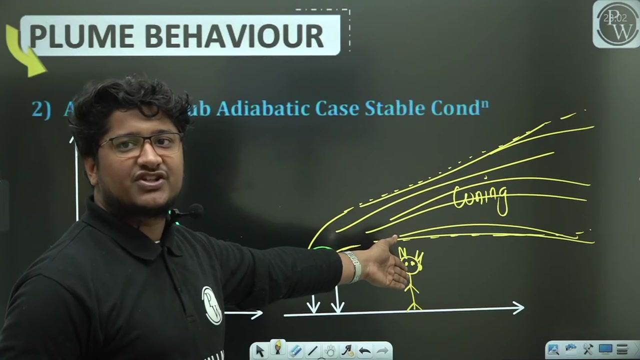 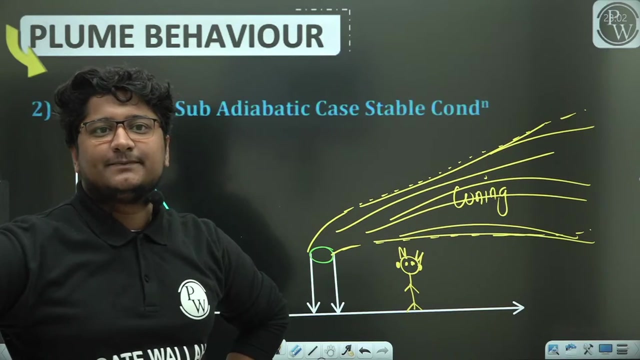 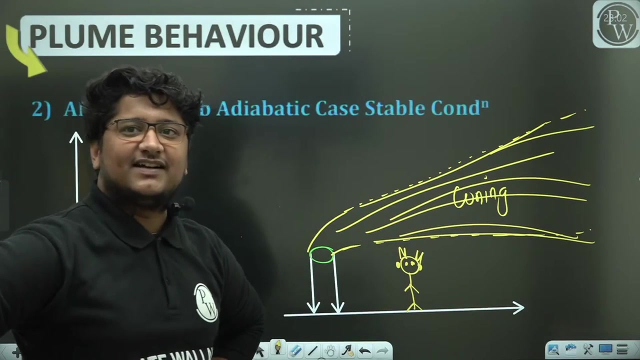 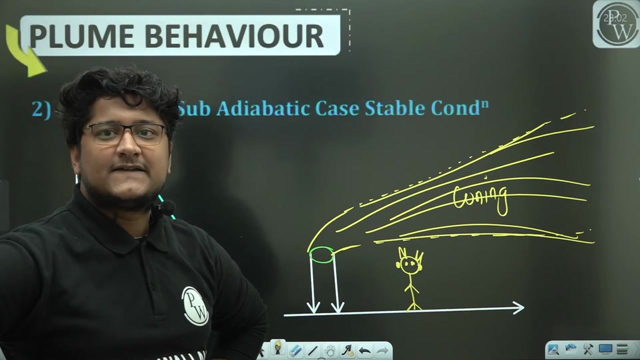 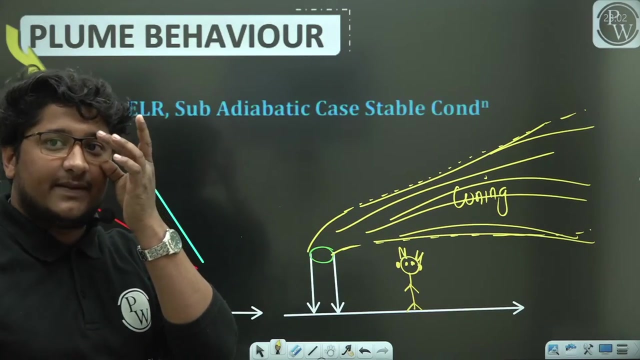 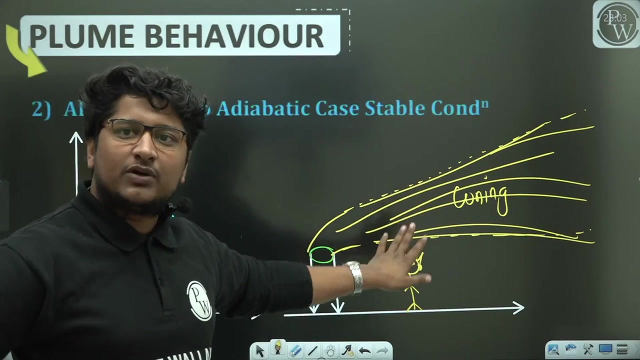 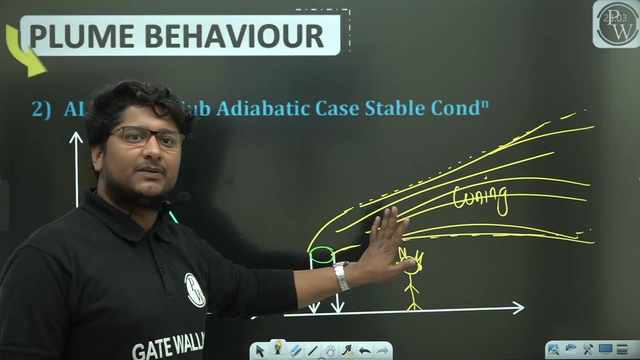 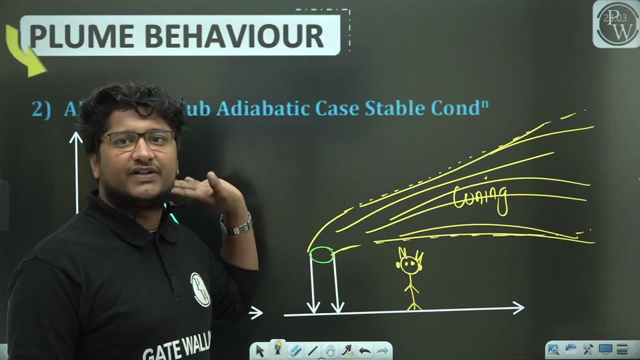 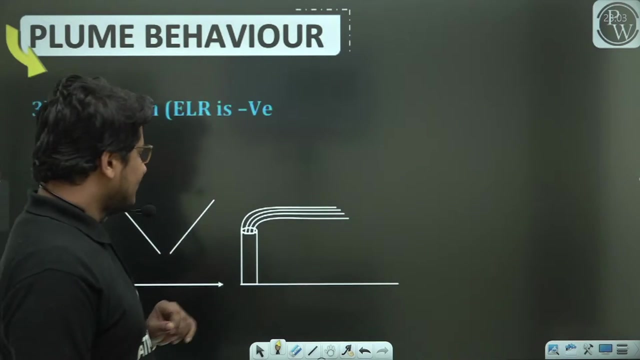 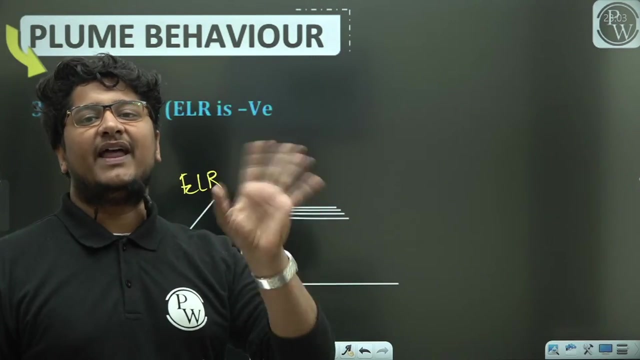 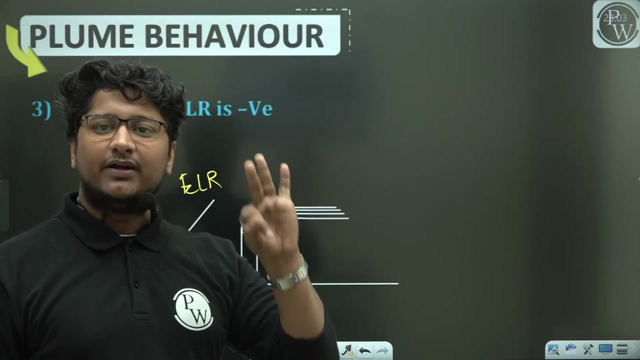 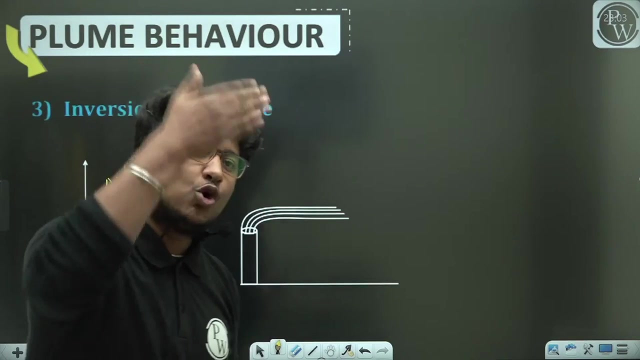 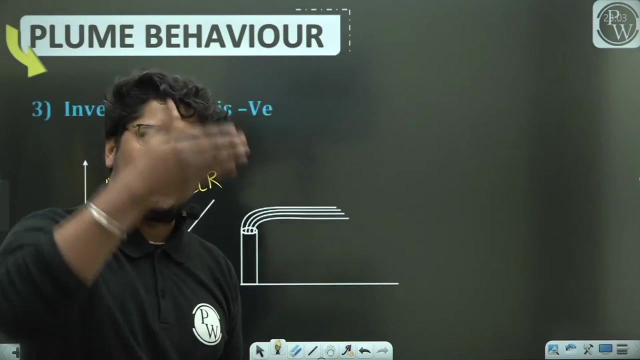 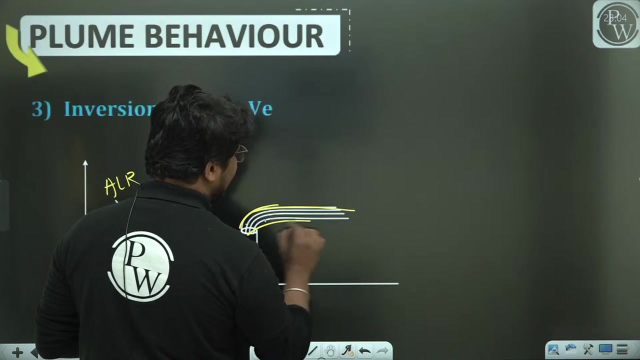 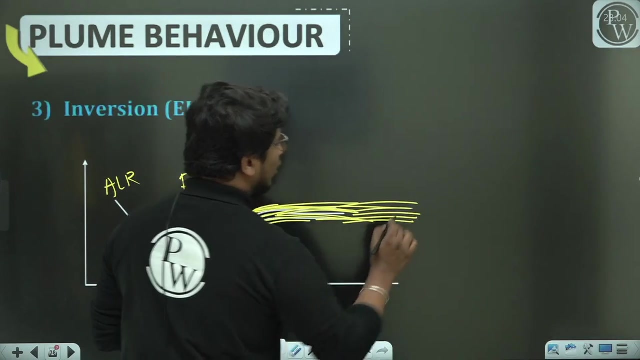 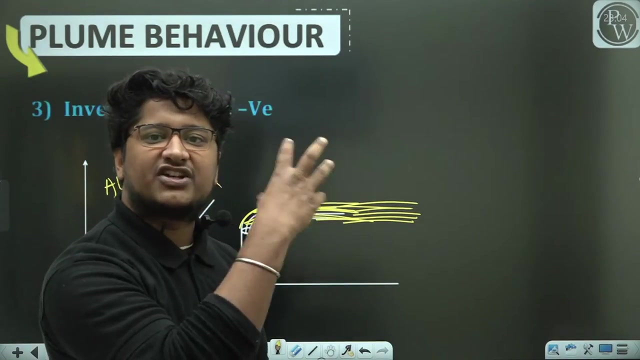 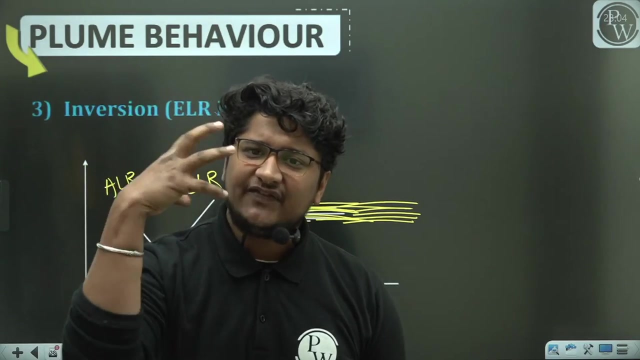 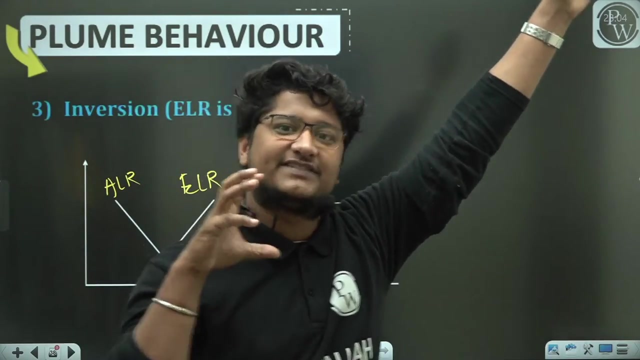 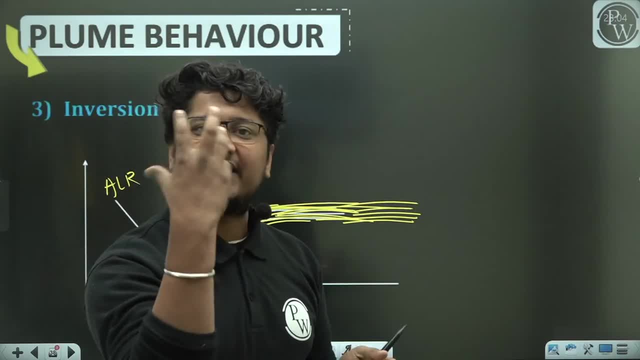 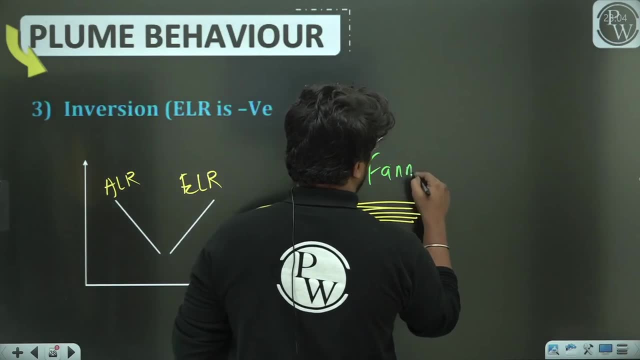 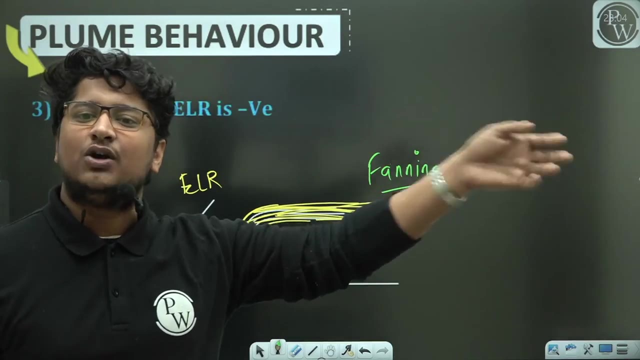 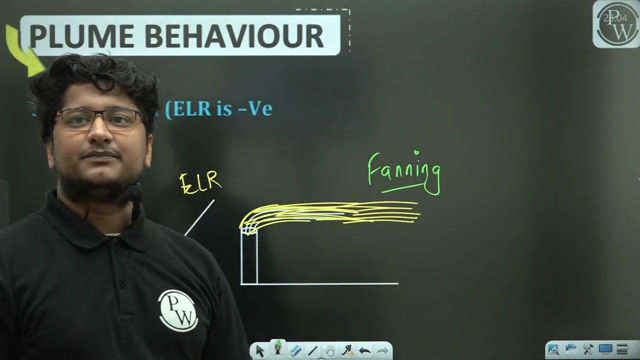 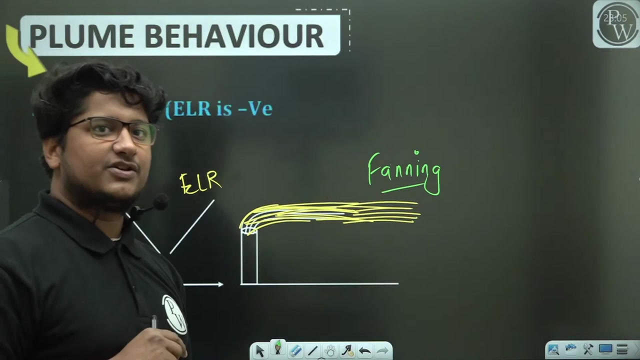 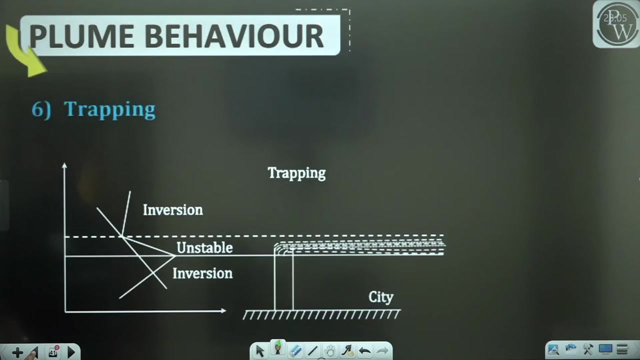 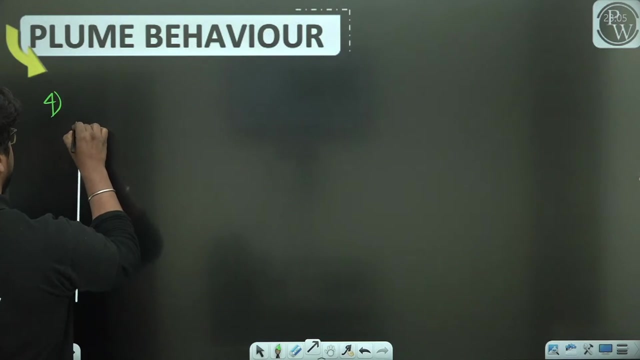 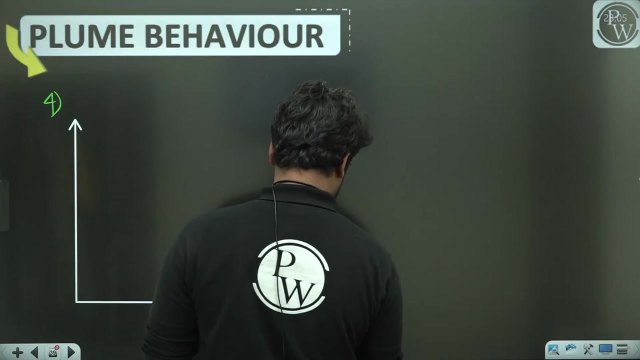 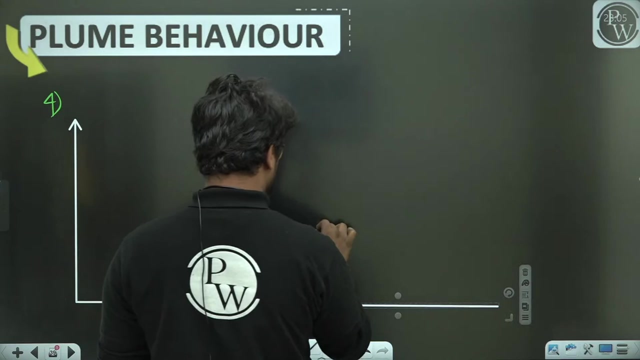 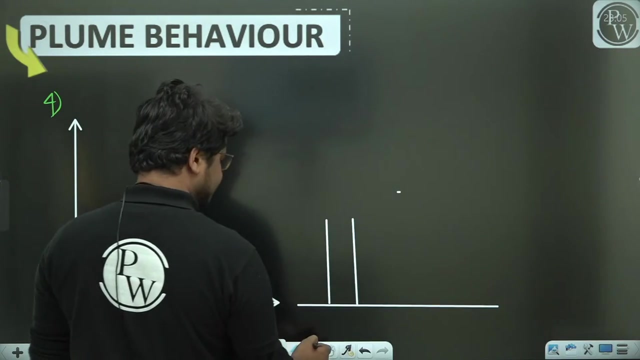 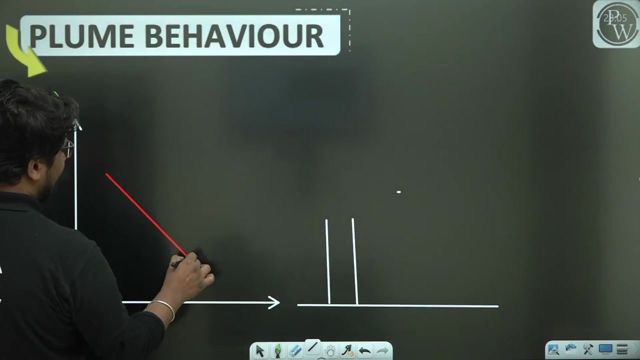 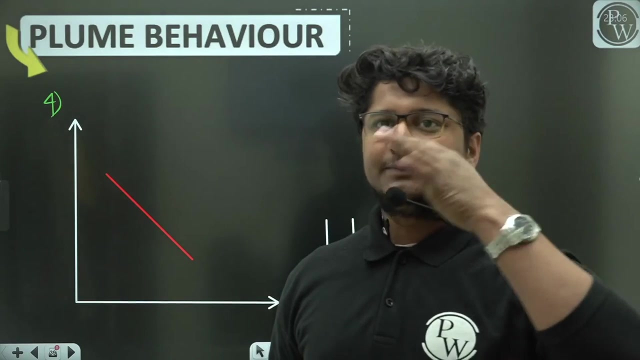 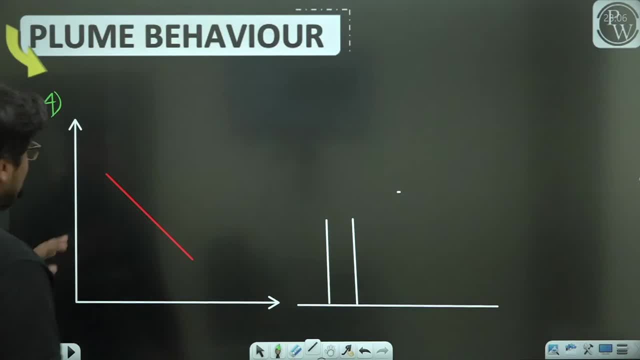 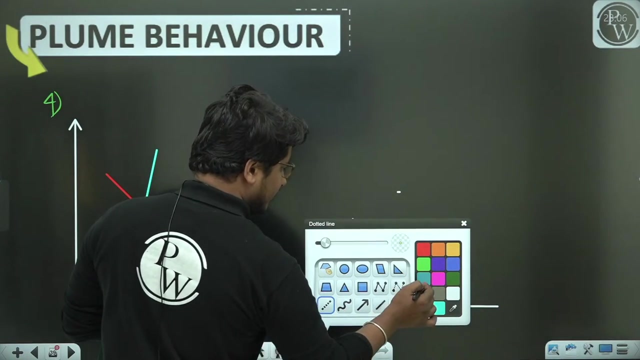 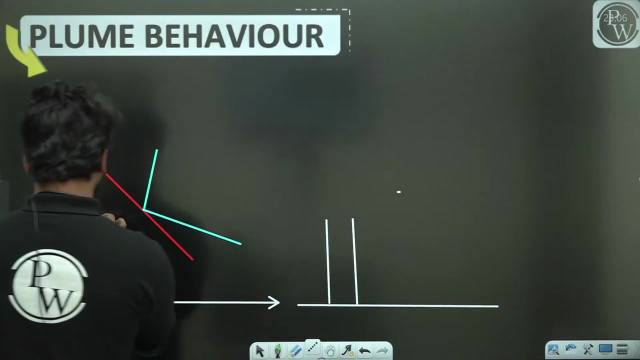 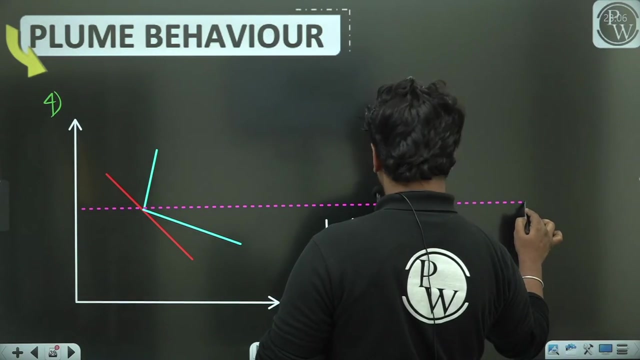 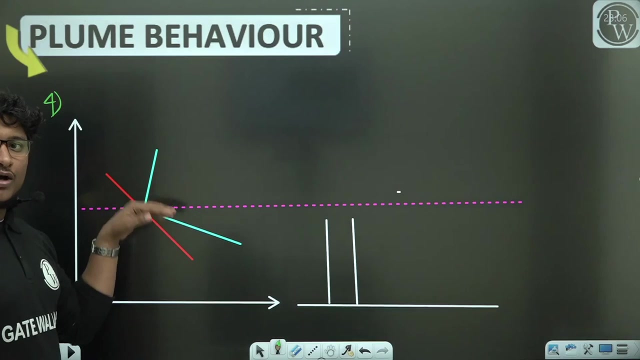 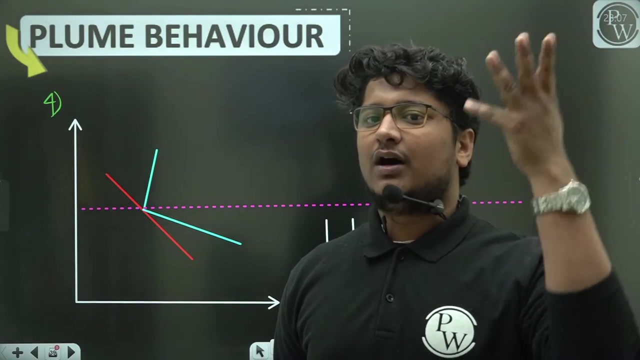 Now see how to play. this is your ELR. now, how can I play? I can't play with ELR. I can play with ELR. I can play only with ELR. now see how to play. OK, so here you see the problem. here you see the problem. I musste divide this into 2 wurdenpes. 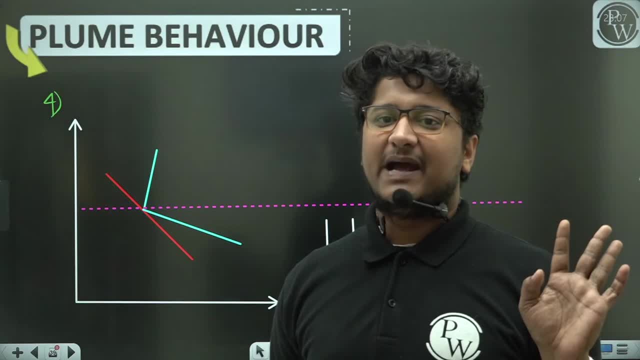 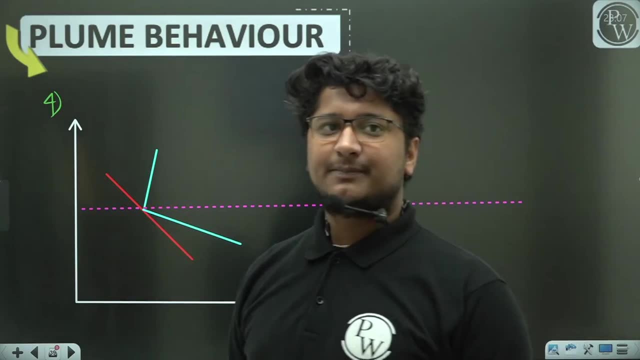 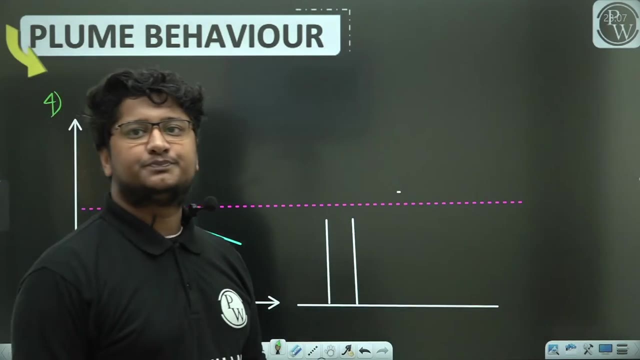 super stable means very bad condition. so above there is stable, unstable or super stable, tell me quickly. divided into two parts, one above and one below. answer in comment. answer in comment. upper inversion means super stable. Suruchi bacha is telling upper inversion. 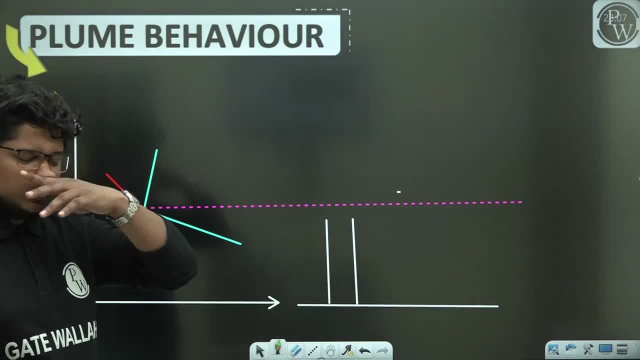 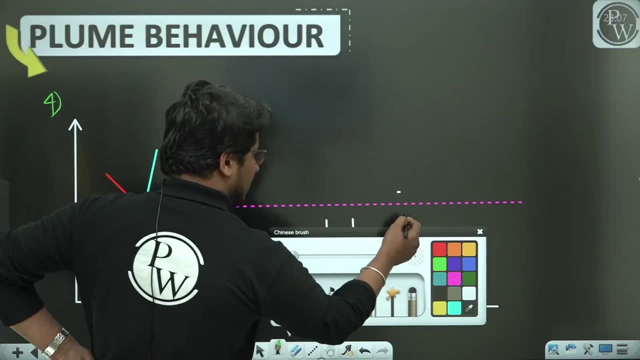 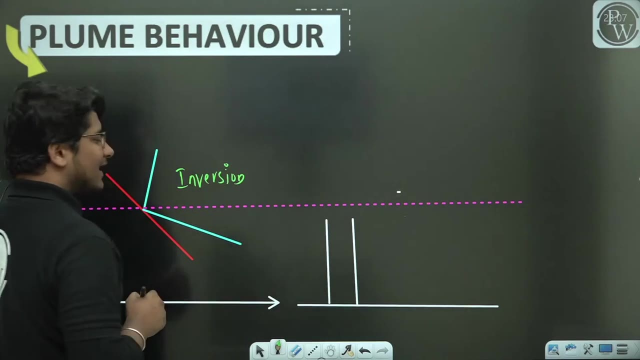 means what happened to you. it is very bad. it is very bad. so you said this one, sir inversion. okay, I accepted it, sir inversion. and what happened to the one below, sir? what is the one below? 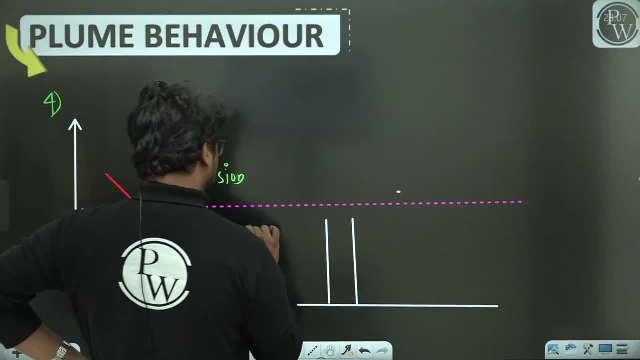 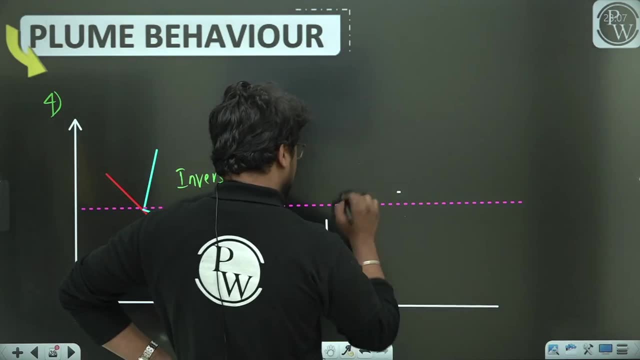 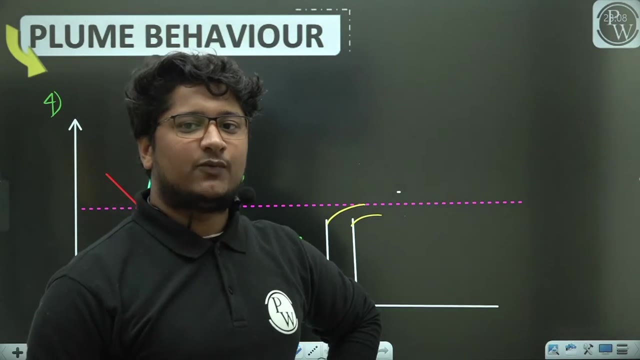 sir, unstable. the one below is unstable. it means your super adiabatic condition. in such a condition, sir, if we take out the warm air parcel, you think your warm air parcel will go up? you really think any warm? 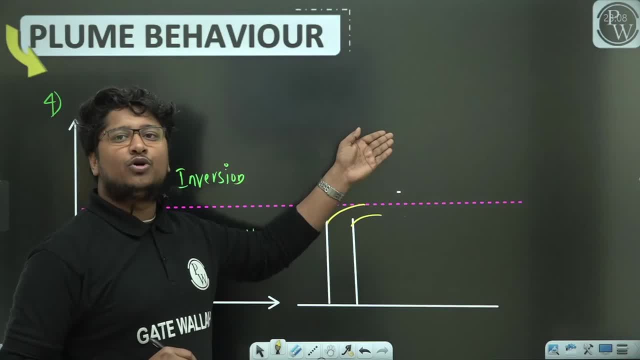 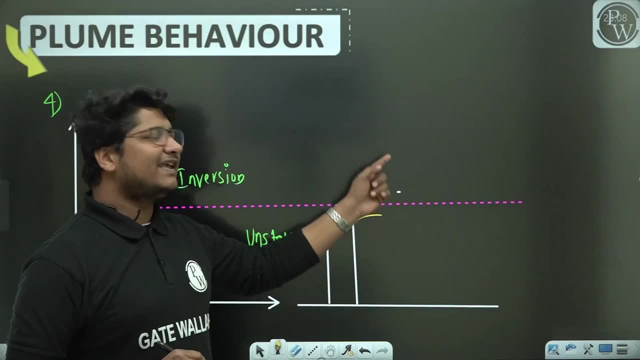 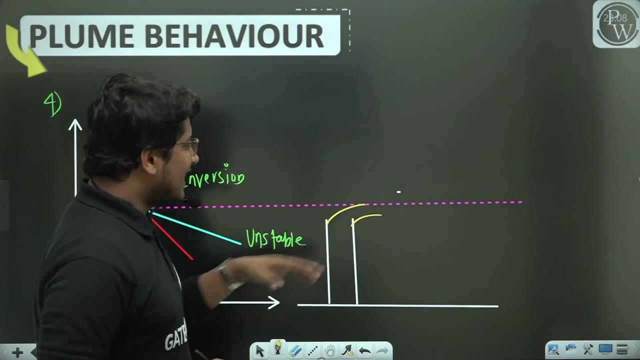 air parcel will go upside. one is you total couple restricted zone. four police officers are standing for you to sleep. one is absolutely couple free zone. you feel that even one couple will go in the upper zone. none will go in the couple free zone. no one is going to go in the restricted zone. the same thing is here. 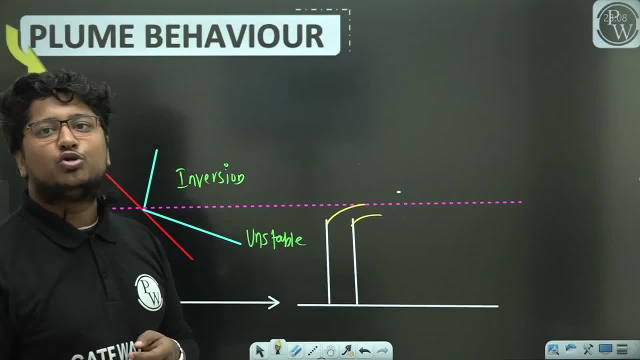 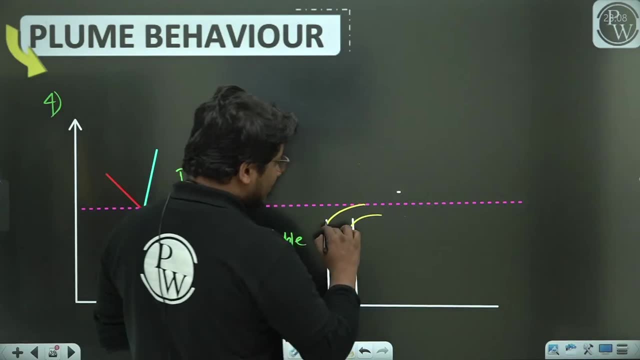 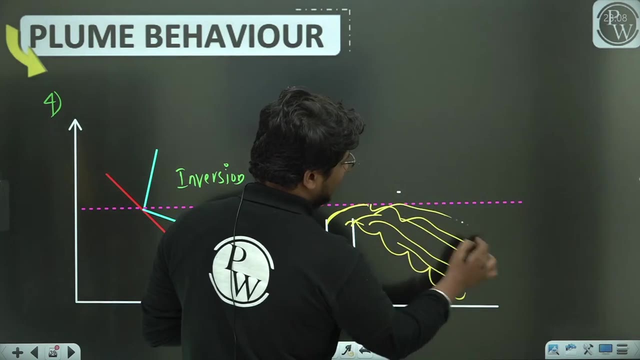 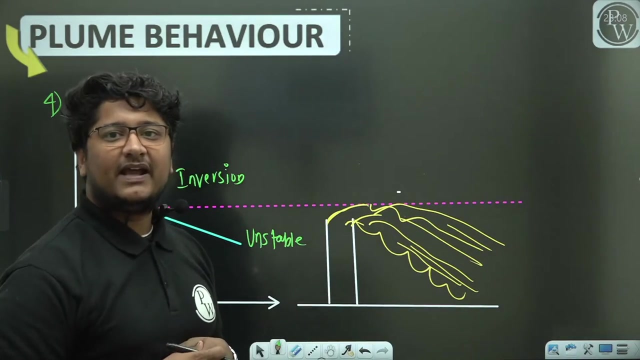 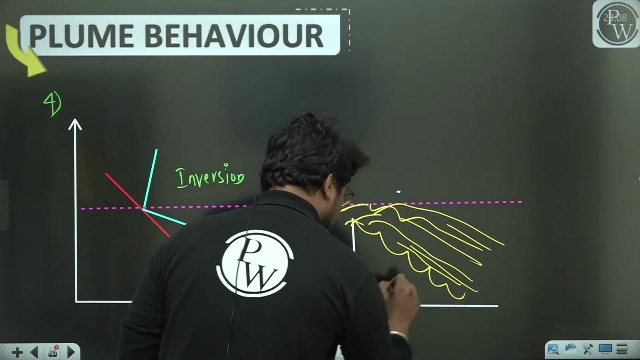 one is you in such a condition where the vertical mixing is absolutely zero. one is you? So, in this case, whatever your plume will come out, it will run all the way here. it will run all the way here. it will run all the way here. and in such a case, in such a case, in such a case, if our who is brother this time, Arpit Tiwari ji, if our Tiwari ji will be brushing here in the morning, if he will be brushing in the morning, then he will be brushing here. 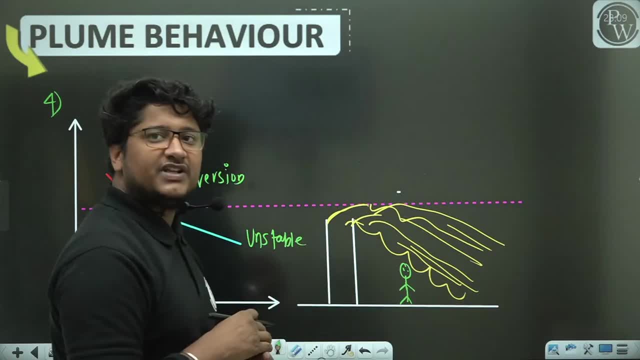 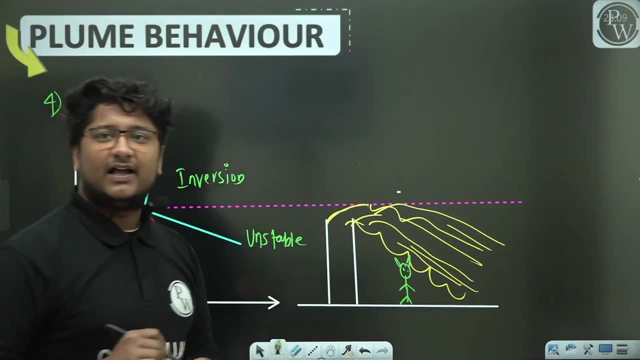 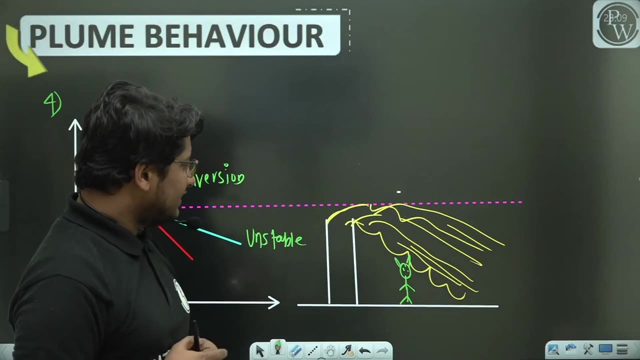 Now, Tiwari ji is a woman or a man? by name, it seems to be a man. so, Tiwari ji, what do you think? will we live tomorrow, or will we have to say that Tiwari ji was a good man? what do you say in such a case? in such a case, what will we live? will Tiwari ji live, or will Tiwari ji be a good man? 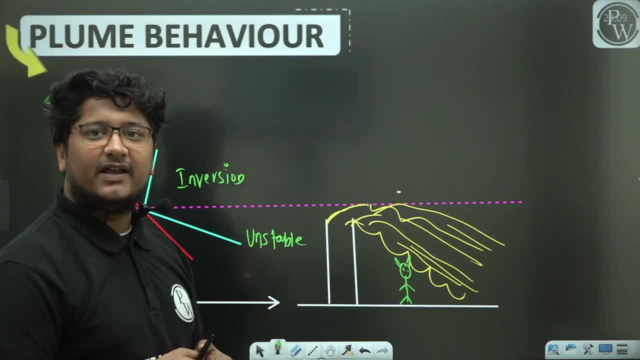 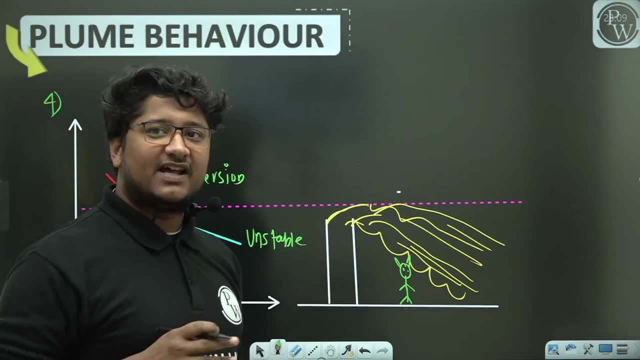 Yes, here the brush, I mean whatever our brother Arpit is. so Tiwari ji was a good man. In the comment section once, quickly, everyone will type all the children together that Tiwari ji was a good man. 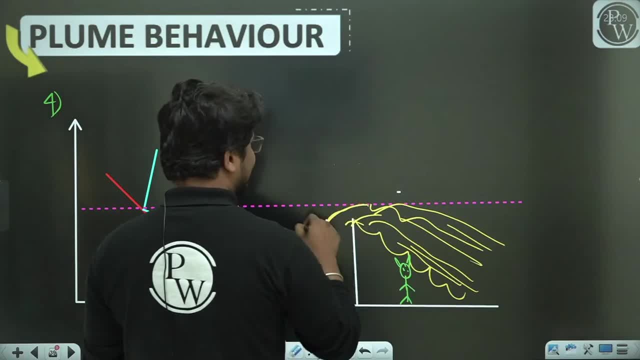 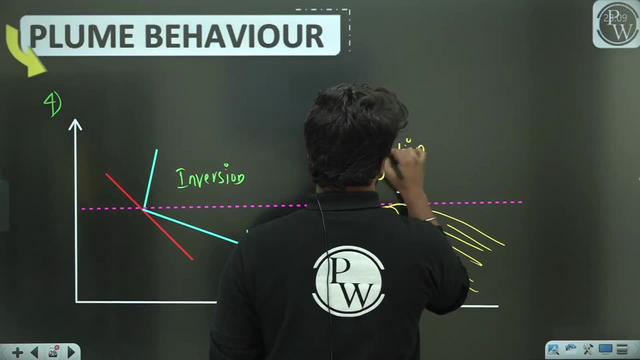 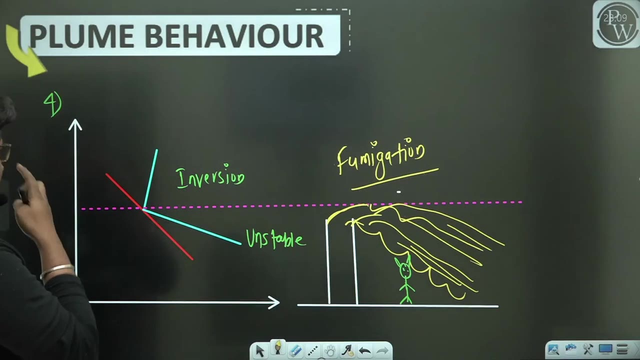 Come on, Let's name this case children. This case we call as fumigation. This case we call as fumigation. This case we call as fumigation. Okay, Come on, Let's go to the next case. 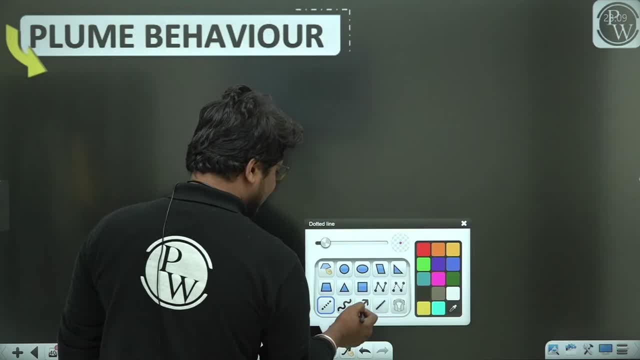 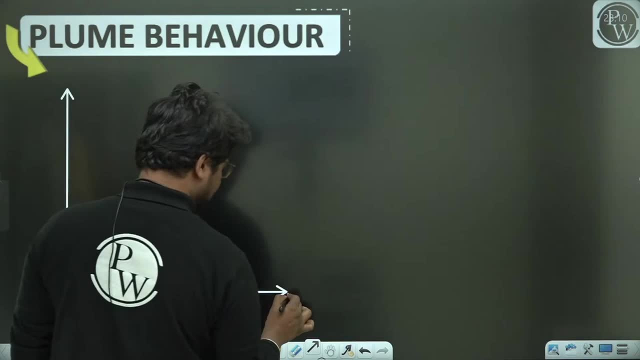 Let's go to the next case. Okay, We have to come to the comment section. all the children, Tiwari ji was a good man. He was a good man from the best. Whoever he was. he was a little naive, but he was good from the best. 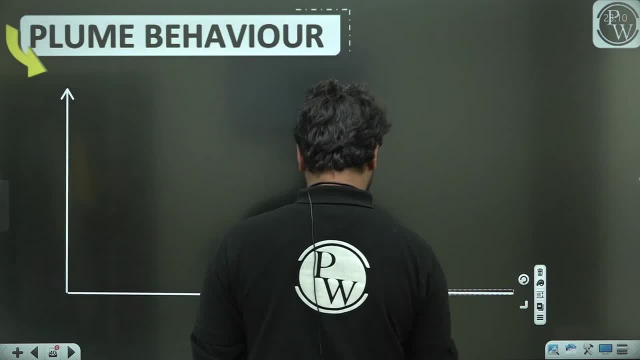 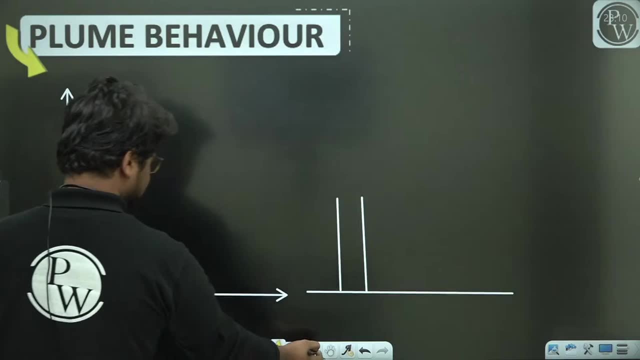 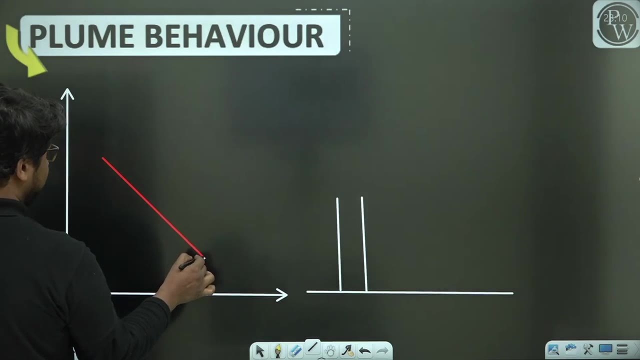 He was a good man. Yes, Mr Tiwari is a good man. okay, now come here again. our ALR is the same with whom we can play, sir, then we can play only with ELR. sir, ALR is constant, it cannot be played. so this time, how am I playing? see, this time, you guys, this time I am playing something like this: 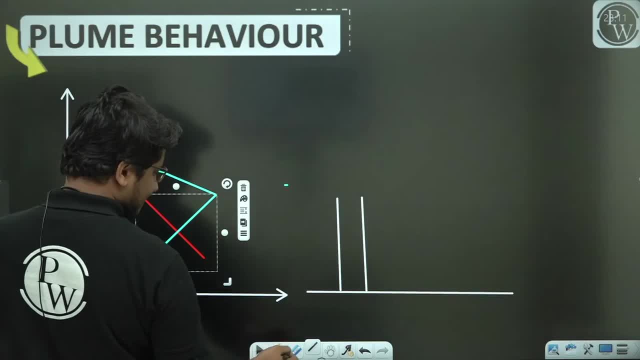 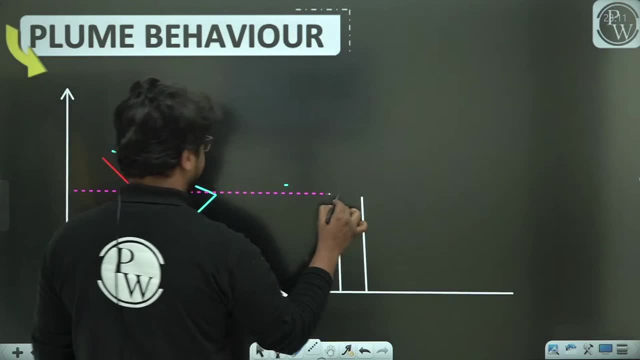 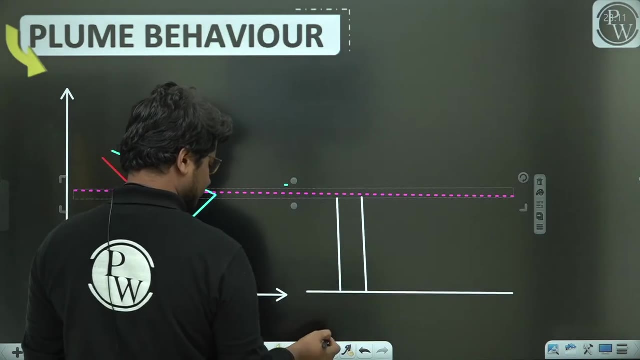 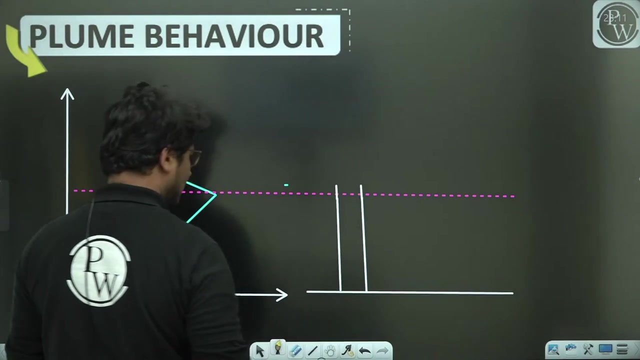 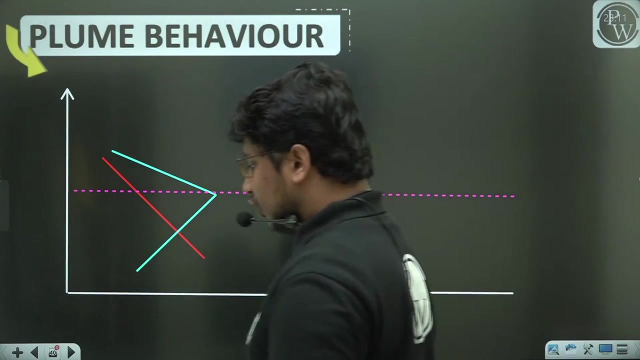 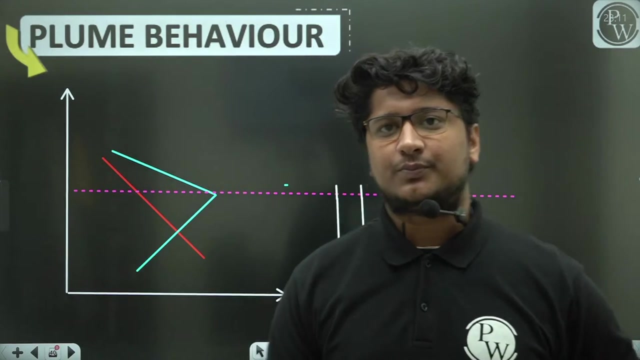 let's go again: up, down, up down. what is up, what is down? tell me quickly what is up, what is down. tell me quickly what is up and what is down. tell me quickly all the children. 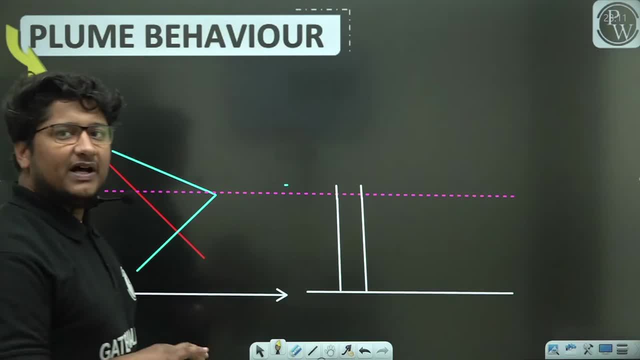 up unstable this time. up unstable this time. why, sir? because I saw only the slope. so the slope. I saw the slope of ELR less, whose slope is less, its value is more. so what happened to the upper part, sir? 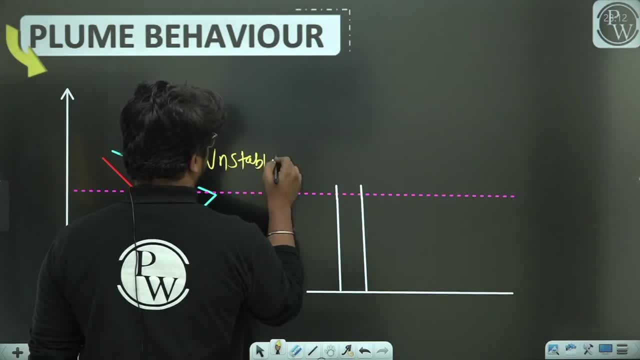 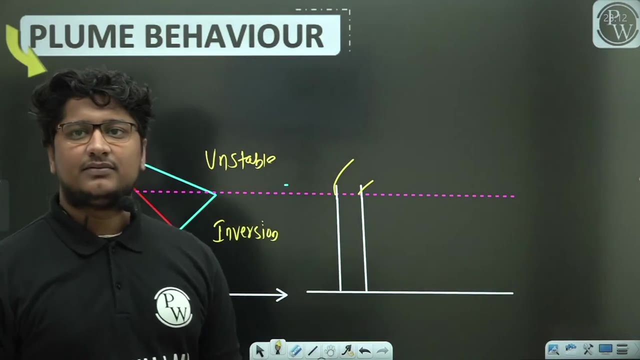 unstable. see the lower part upside down, upside down. so what happened, sir? the lower part inversion. now, if any plume comes out of here, you think it will go down. now, in such a case, if any plume comes out of you, you think it will go down. 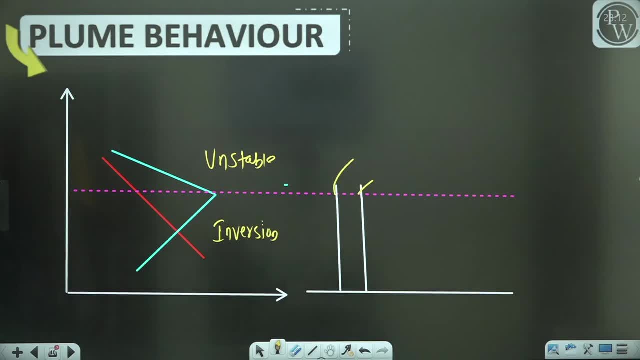 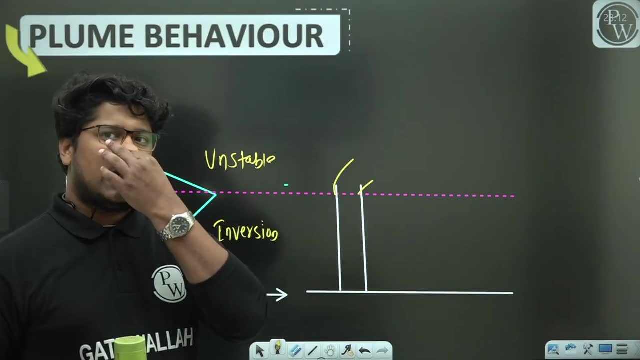 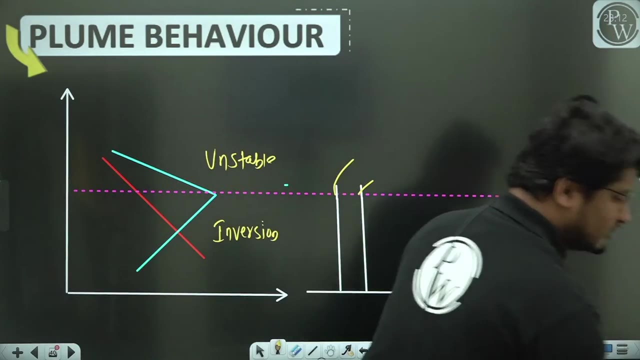 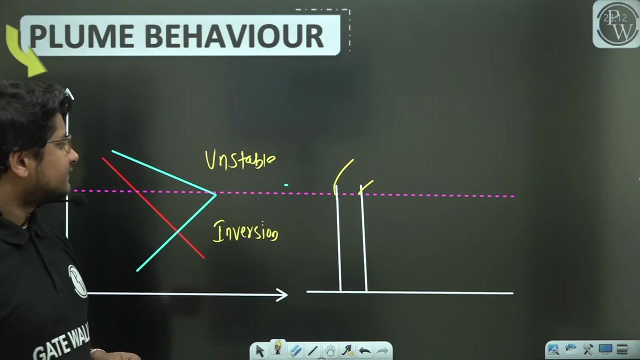 you think that it will go down? no, sir, there is no chances to go down. there is no chance to go down, sir. why it is not going down, sir? because there is inversion and at the top is your couple跟. 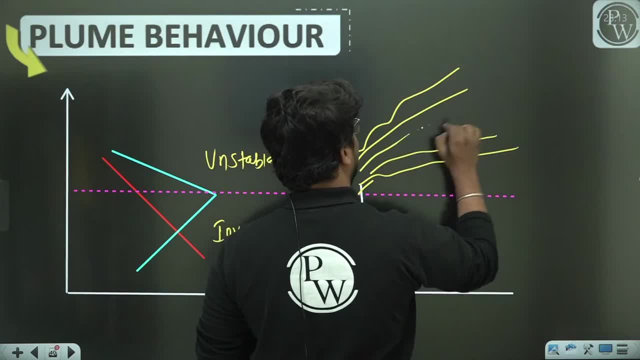 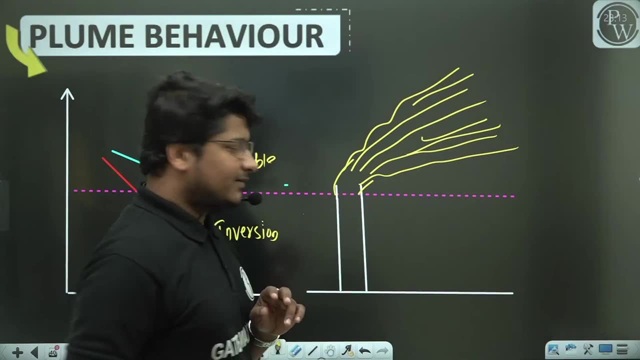 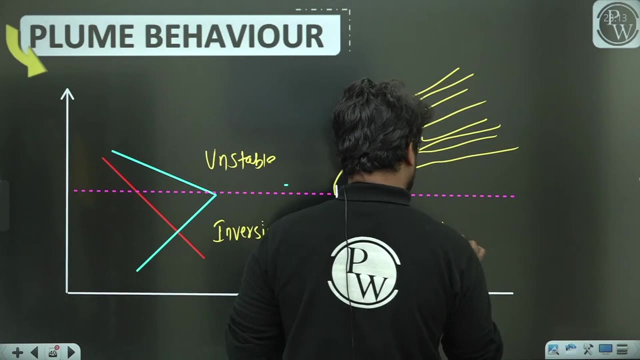 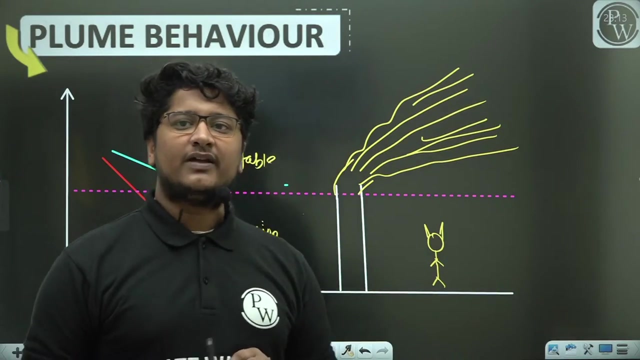 free zone going. and in such a case, in such a case, in such a case, if our brother tiwari is brushing here, if our brother tiwari is brushing here, then he will be laughing or sad. he will be laughing or he will be crying. in such a case, if our brother tiwari is brushing here, 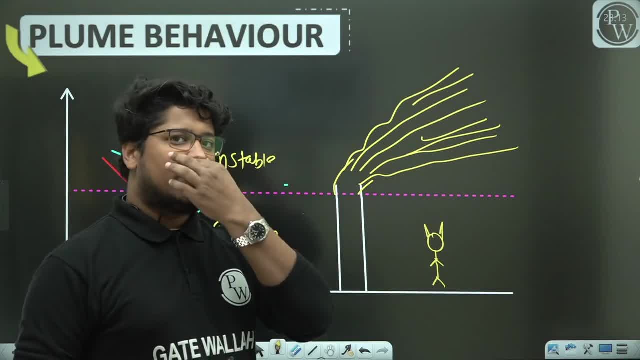 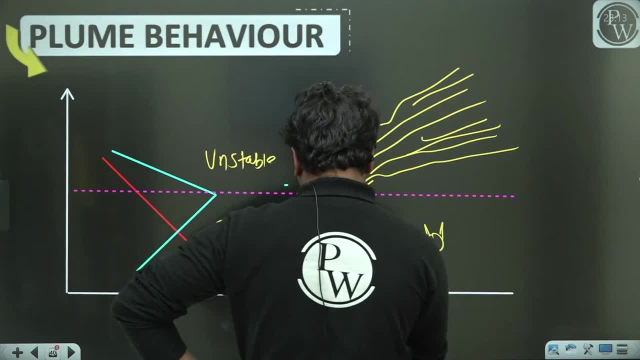 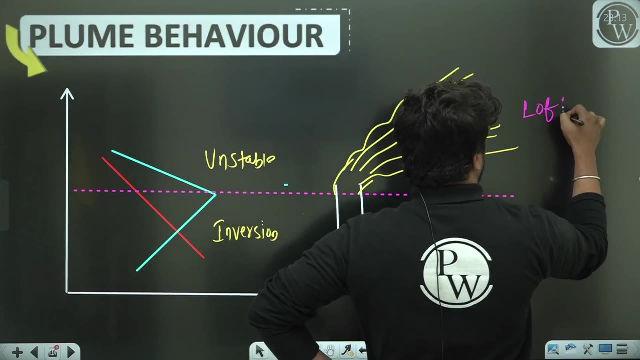 will be laughing or crying. reply with ease. will be laughing or crying. will be laughing due to this. what was the name of the case lofting? this is why the name of this case. also, What was the name of the case Lofted? What was the name of the case Lofted? 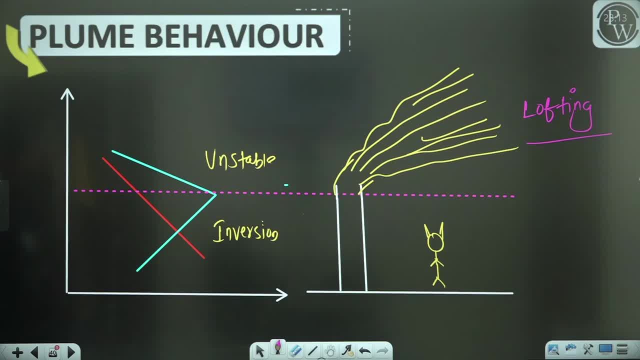 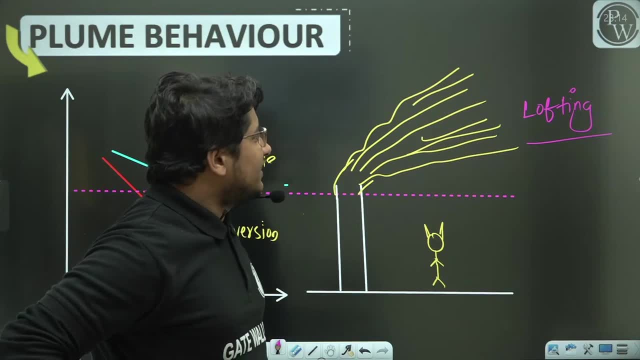 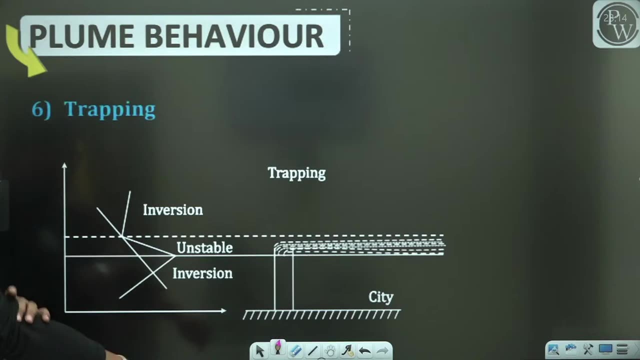 What is the name of this case? Lofty. Ok, I am very happy, By the way, Mr Tiwari is happy. Ok, what is the name of this case? Lofty. Next case, you know, is trapping. Now see what they have done in this. 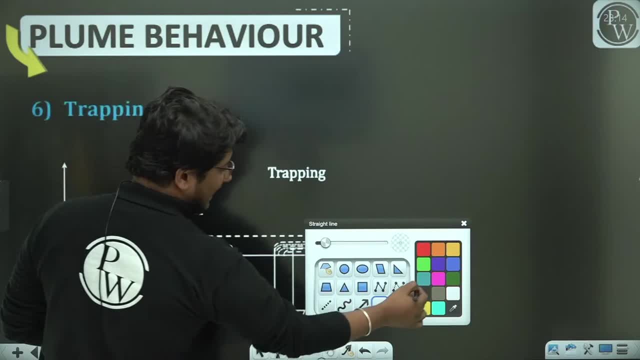 See what they have done. One is your ALR, which is constant. It is still ALR constant. Ok, after this, what did you play? You played a little with ELR. What did you play? So first time? your ELR is like this: 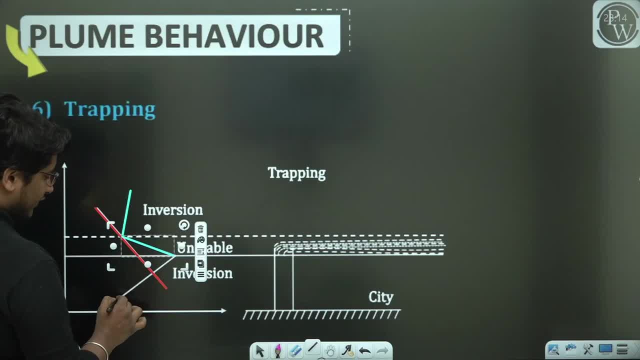 Then it is like this And then it is like this. So you will see in the above condition what you are seeing. It has spread in three parts: In the above also inversion. In the below also inversion In the middle. your is unstable. 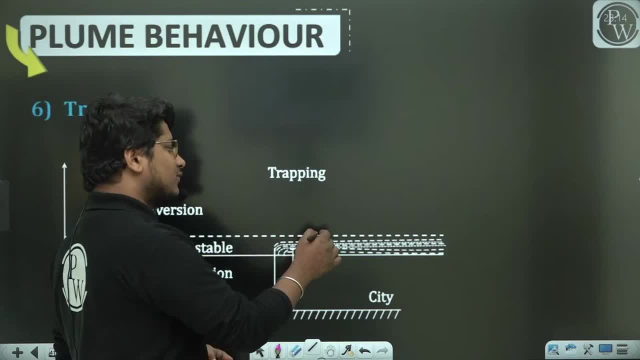 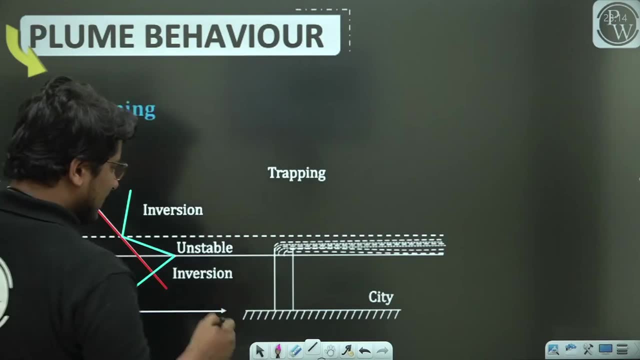 Now, in such a case, if you will release any plume, So neither it is going up nor it is going down, So it is trapped in the middle of two inversion layers. In such a case, In such a case, This time, Tiwari brother will say that you use me again and again. 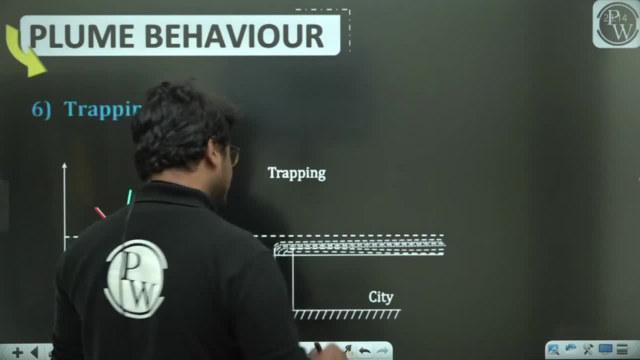 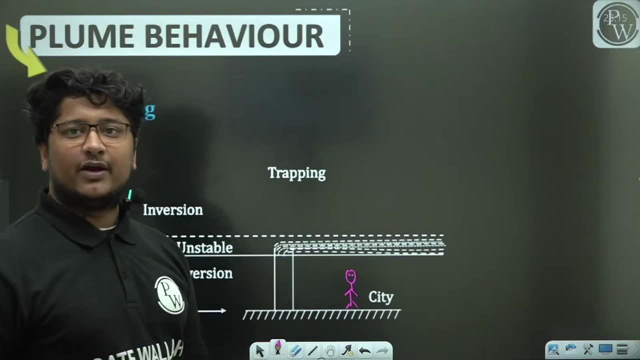 This is wrong. So this time our Vikas brother is here. So if our Vikas brother is here, If he is brushing you here, So it came out from above: Vikas brother. So this is done generally by trapping. 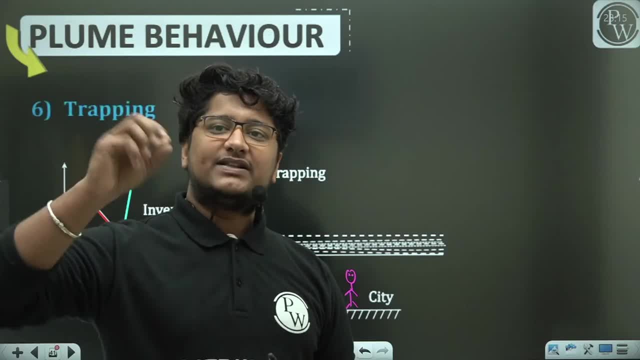 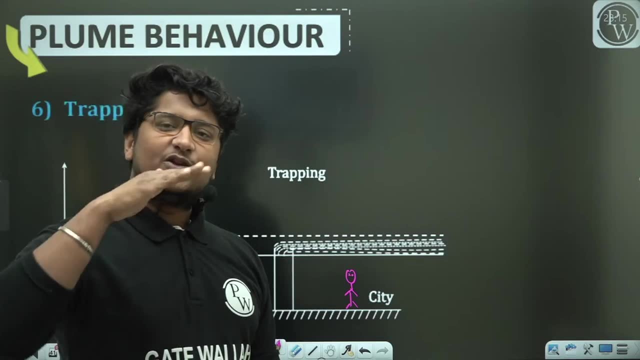 When you have a plant near any city And you want to save the pollutant from the city, That is, it is said, upside down. So you want to save the people of the city from this trend, So you cross it from above. 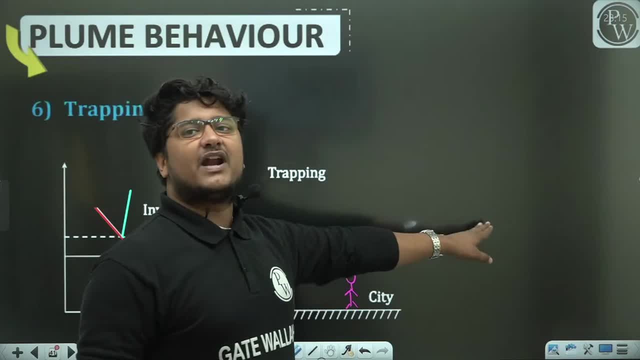 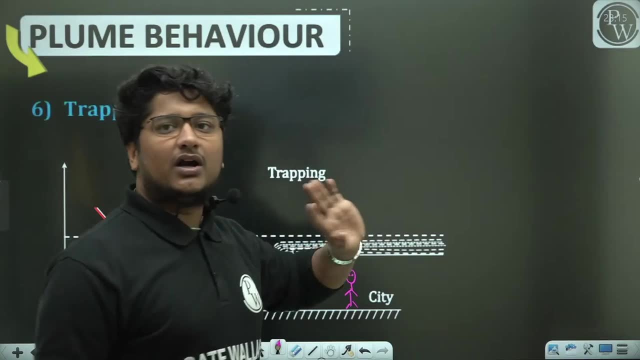 But this is not a permanent solution, Because wherever the trapping condition comes again, you will not get it. What will be the problem? That again it will create a problem for you. So this trapping condition is not the first priority for us. 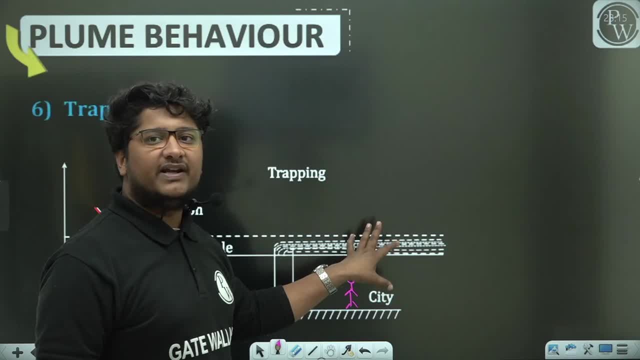 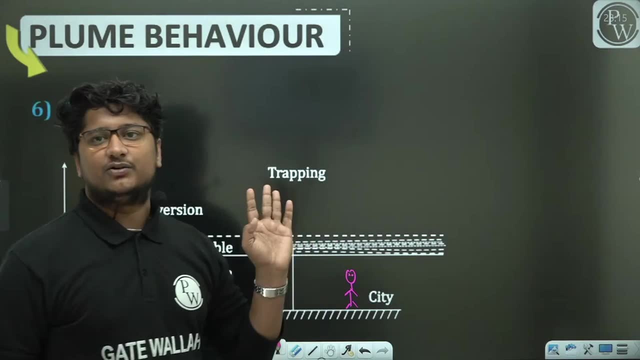 But yes, when do they do pollutant emit in the trapping condition? You have understood that When there will be a city down here, Your Vikas brother will keep brushing there. So you take it out from above. Okay, So our Vikas is saved. 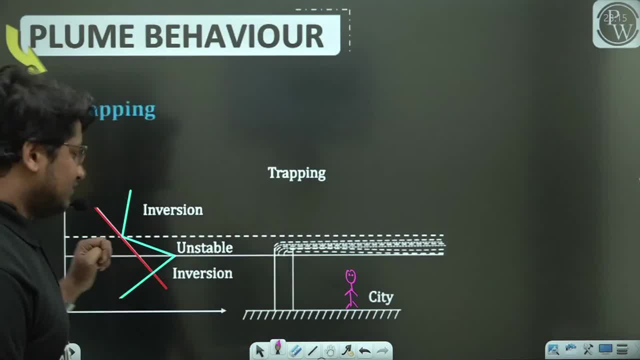 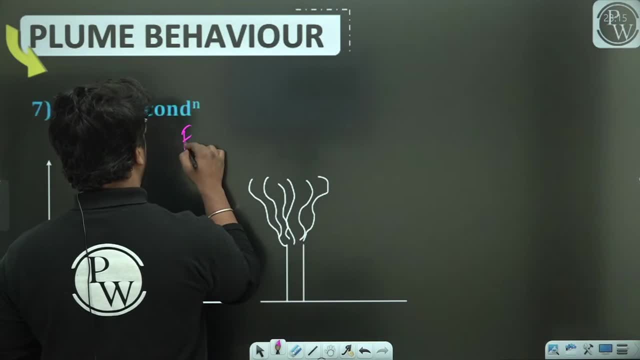 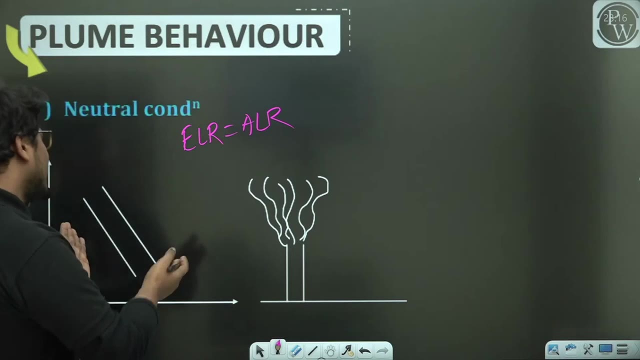 Let's go. Next condition is your neutral. This is the inherent condition. When your ELR and ALR is equal And ELR is not equal to ALR, ELR and ALR will be on the same line. If the slope is equal to both of them, then you can say ELR is equal to ALR. 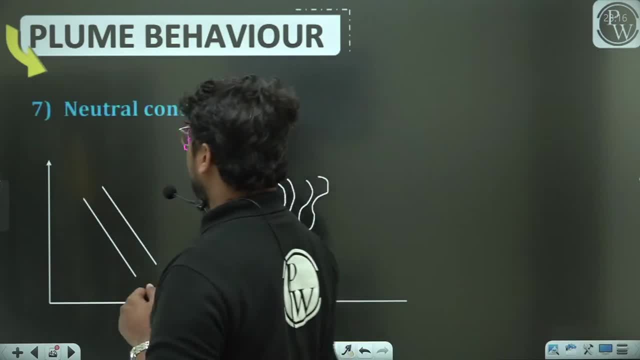 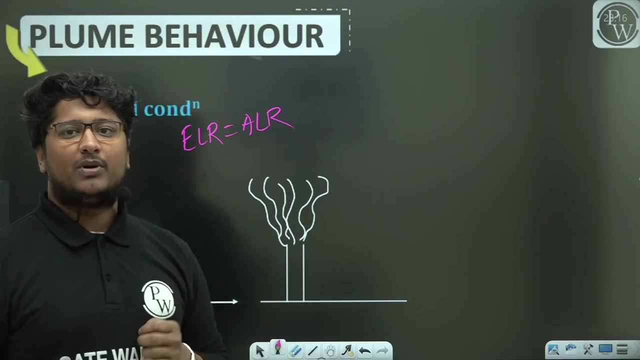 If slope is also same for ELR and ALR, You can say it is a neutral condition Here, as your warm air parcel was going. it will keep going up, No problem. So this is the ideal condition. I mean there are very few neutral conditions. 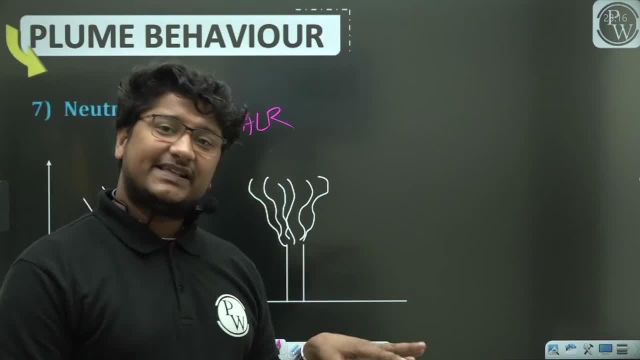 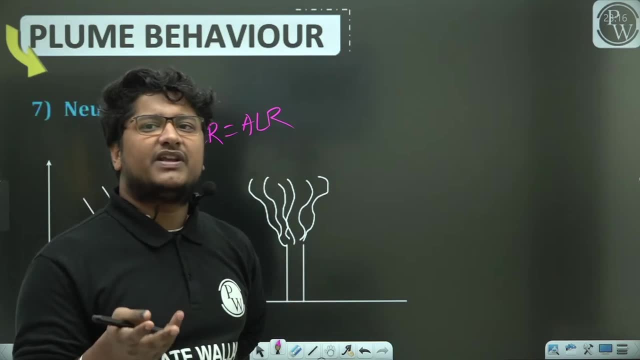 We don't talk much about it, But these 7 conditions that are there. Apart from this, many conditions are possible. These 7 standard conditions that we are talking about, All these conditions are not like this at any time. At any time, you can be at a particular location. 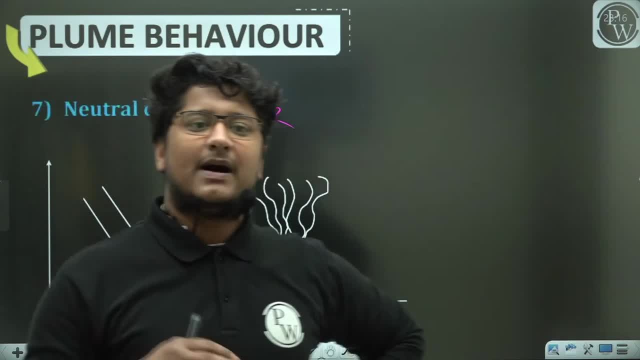 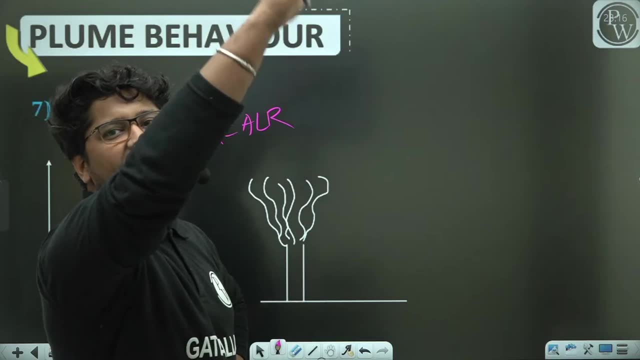 And according to that, you have to meet pollutant. So when you will be in a trapping plant, Your work will be regarding air pollution. So you will keep walking on the slide here. That brother, the temperature was measuring. You will keep running ELR. 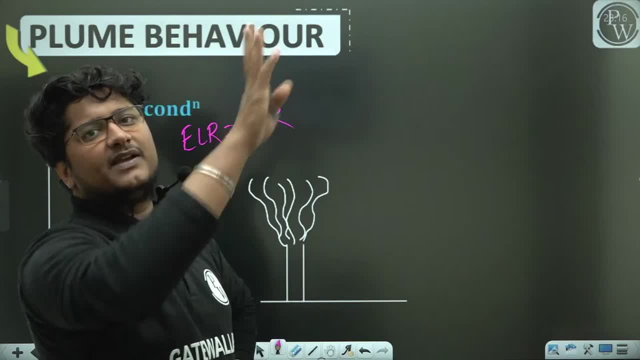 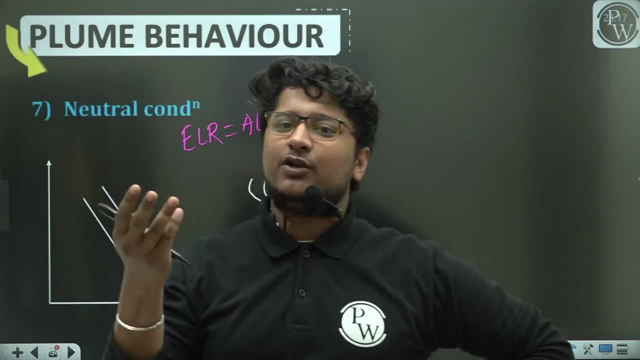 ALR will be the red line. there You can see which condition is going on right now And according to that you have to meet the pollutant. So your pollutant in the entire industry does not always emit. They emit at a particular time. 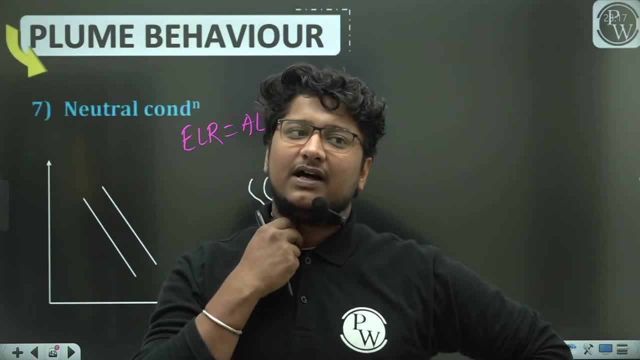 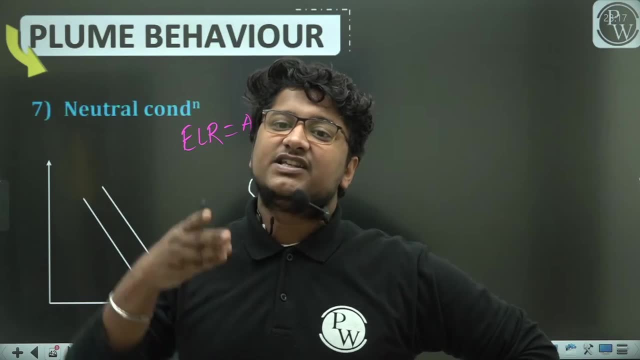 Especially those who are dangerous pollutants Which put a lot of effect on you. They emit at a particular time, Especially when there is lofting. they emit. It is not like that when the condition of fumigation is going on And people do not do it like that. 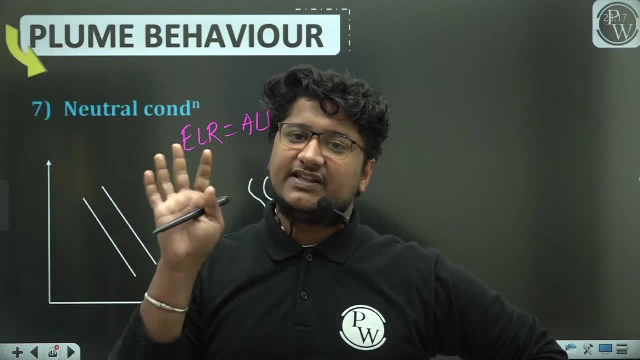 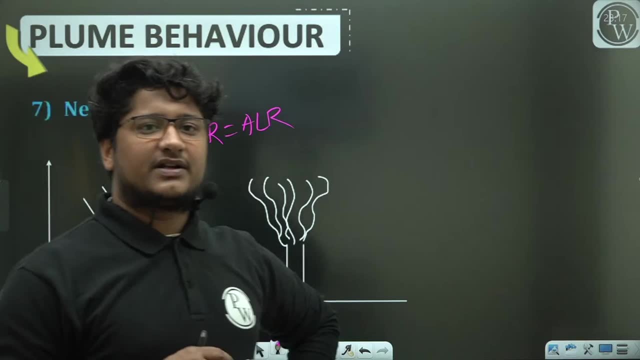 They generally keep in mind that there is a lofting condition, So that Mr Tiwari is also happy. This thing is taken care of. Out of 7 conditions, There may be more conditions. These are the standard conditions that I have told you. 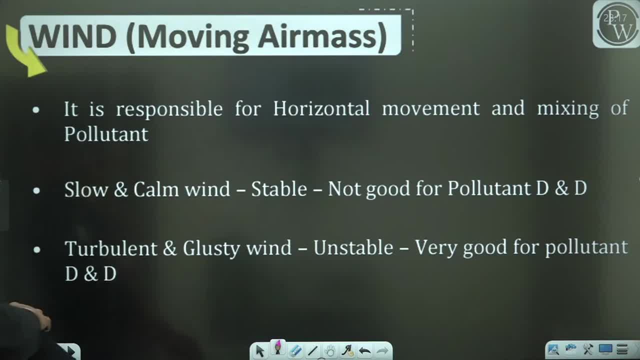 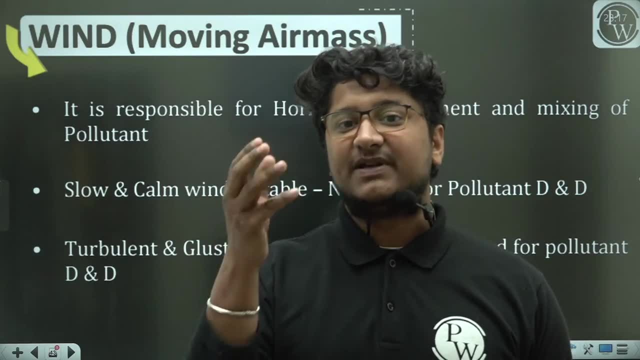 I hope you have understood 7 conditions. If you have understood 7 conditions, Then once in the comment section Tell all the children Which one is best out of this 7 conditions, Which one is best for you And which one is worst for you. 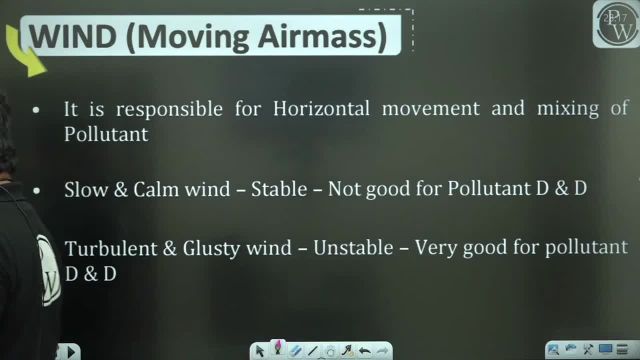 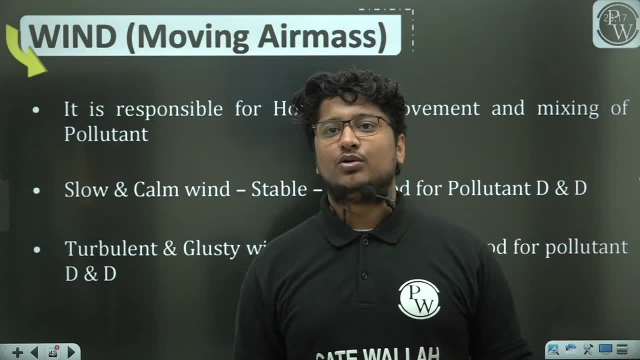 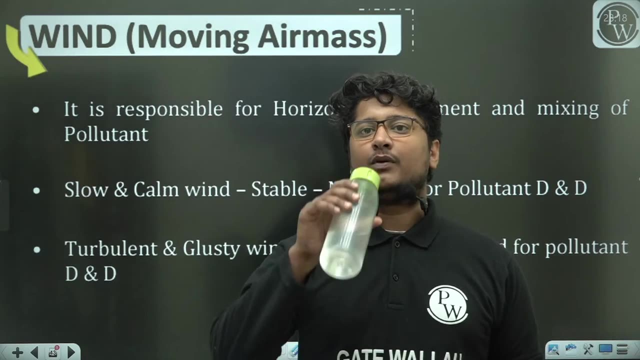 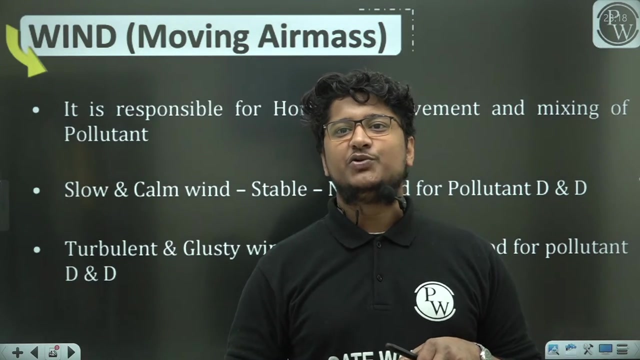 Both things. If you have understood these 7 conditions, I hope you have not looted. I have tried as much as possible That you loot this condition, But still, if you loot, It is your fault. I said neutral, It is useless. 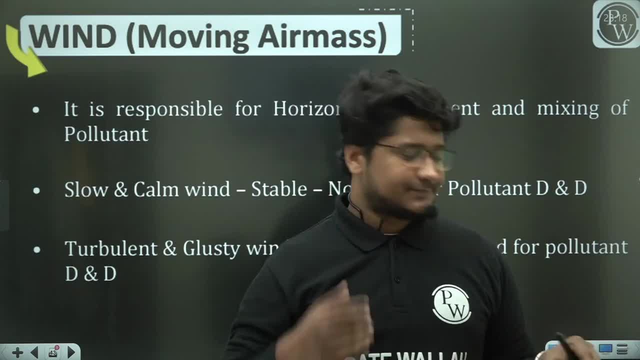 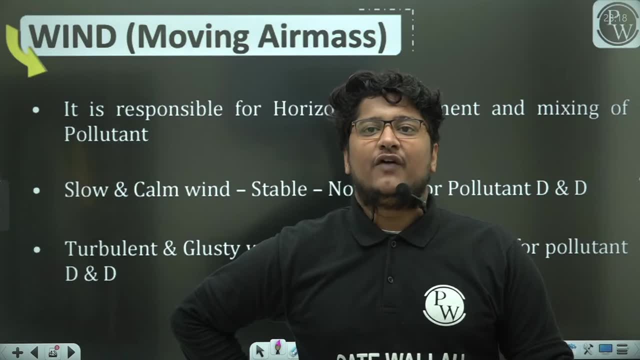 Neutral is less, It is very less. Leave neutral and say Lofting is the best Because in lofting you have the surety That nothing will come down. In lofting you have the surety That nothing will come down. 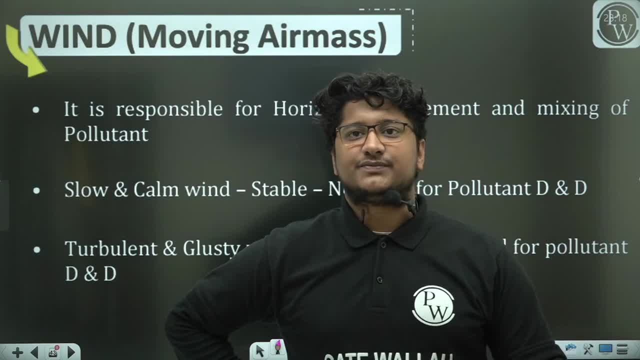 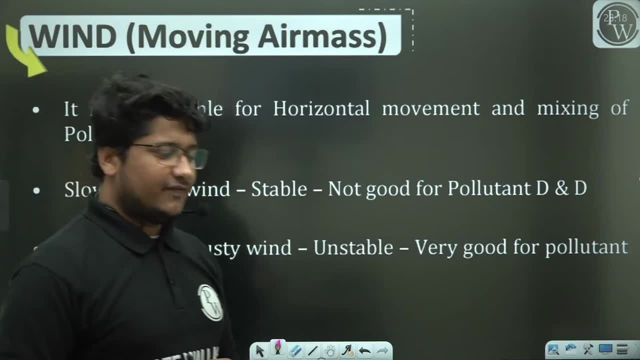 Fumigation is the worst. Fumigation is the worst. Very good, Let's move ahead Now. next is your metallurgical criteria. First was temperature. We have read this whole story in temperature. Now the temperature that mixes you. It does vertical mixing. 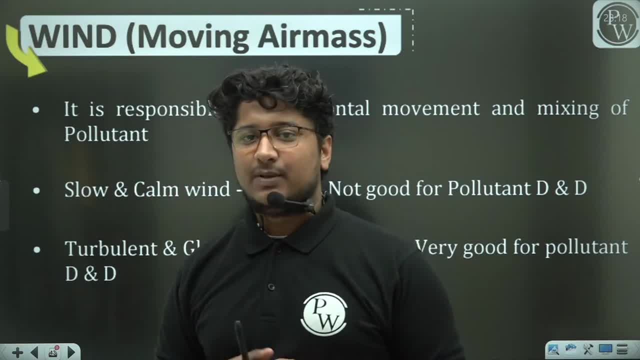 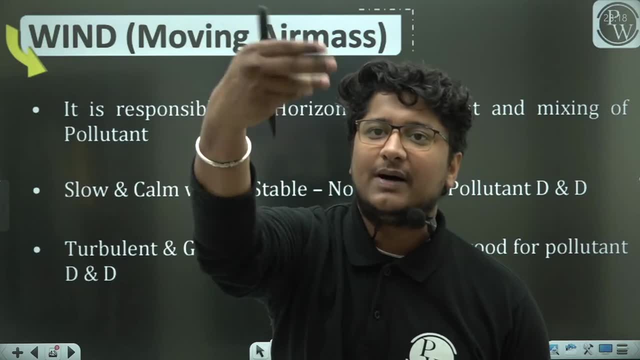 Now the second that comes to you is wind, Which you also call moving air. So what is your wind doing? It is doing horizontal mixing. If the wind is blowing here, Then what will happen to you? It will mix there If it is blowing on this side. 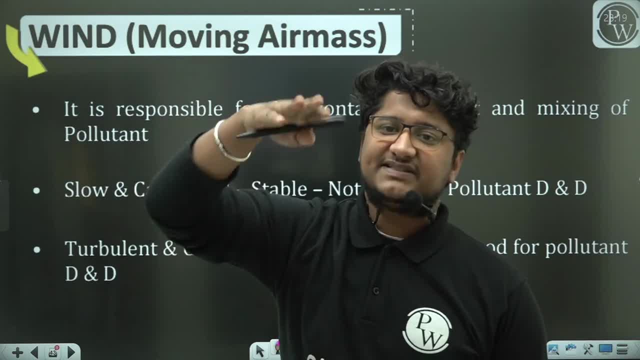 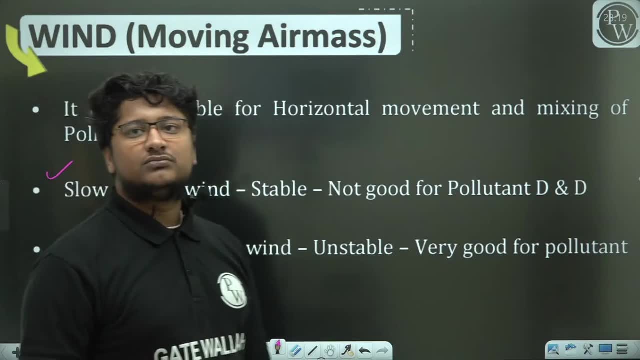 Then it will mix on this side. So the mixing it does, It does horizontal mixing. So the simple thing is, Sir, if you have slow and calm wind, Then it will be stable wind If your wind is not moving much. So in such a case, 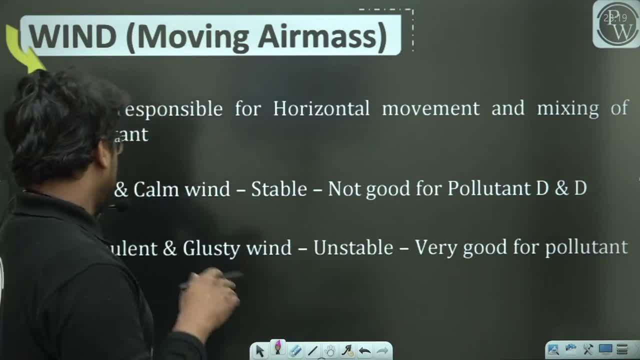 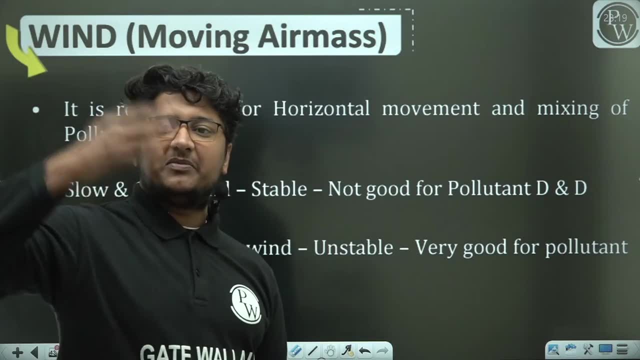 What is not good for you For pollutant dispersion and dilution? Turbulent and gusty wind. It is gusty, It is not gusty. Cut the L. So what is in such a wind? There is a lot of turbulence in your wind. 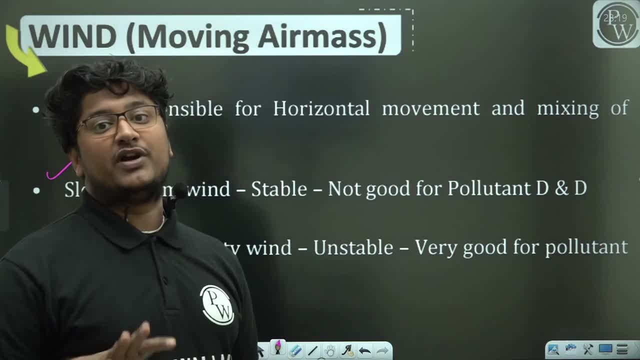 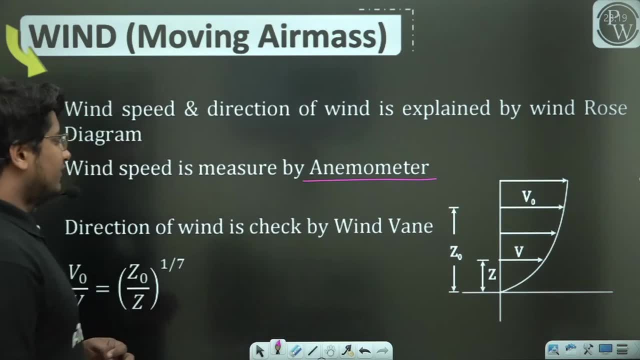 So this is the best condition for us. It is an unstable condition, Good for pollutant dispersion and dilution. Whom do you measure the wind? What speed do you measure the wind With anemometer And the direction of the wind? 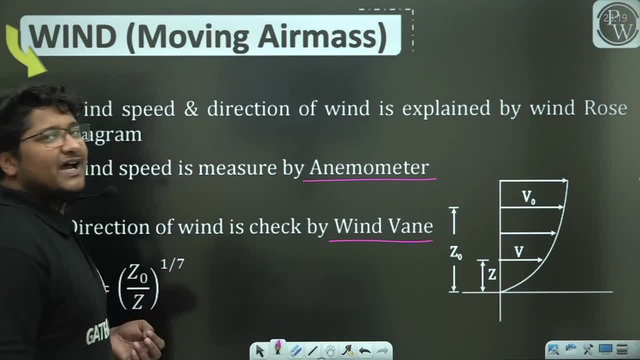 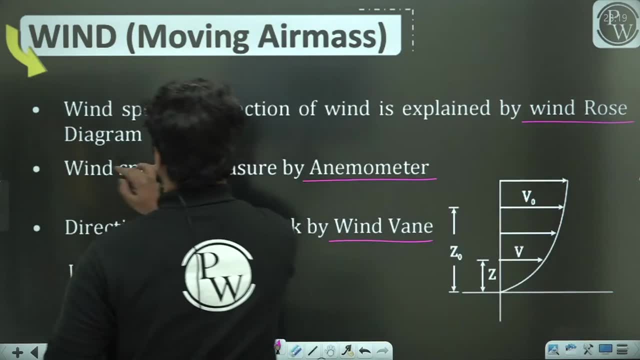 You measure it with wind vane And all these things. You can see in a particular diagram Which you will learn to make in mtech. We call it wind rose diagram. Ok, For example, The airport is being designed, So the wind rose diagram of that area. 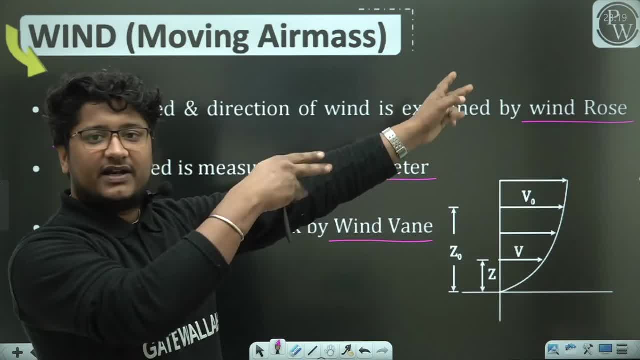 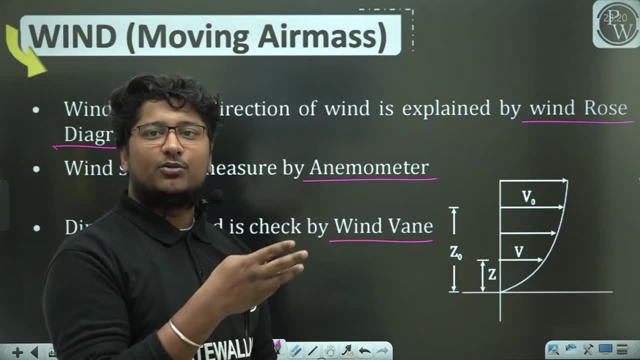 We see And in which direction Keep your runway, All those things You get to know in the wind rose direction. What is the direction of the wind In a year? Or in 5 years? What is the direction of the wind? 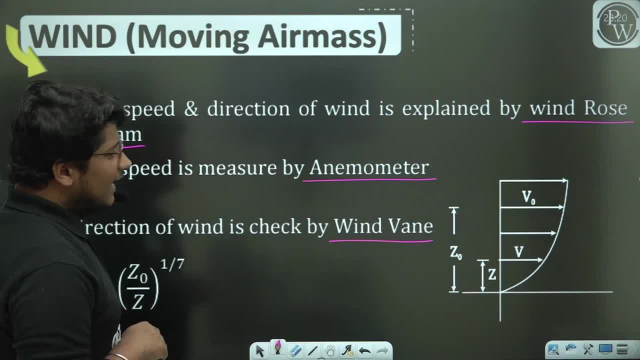 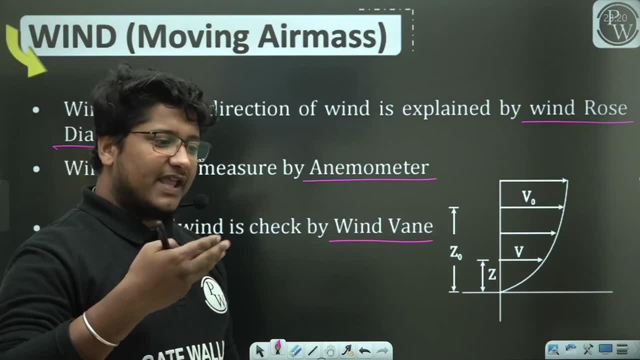 All those things You get to know in the wind rose. Now, what have you done? The speed of the wind Related to the height? Now, It is a simple thing. If you have seen That, you live at a normal height. 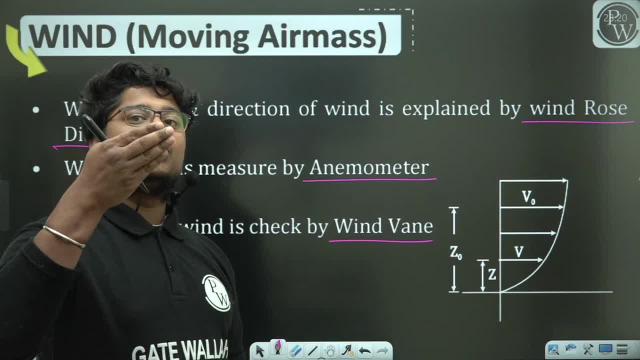 Then the speed of the wind remains different. If you go up, Then your, for example, It increases at a different level. If you go up more, Then it increases more. If you go to Burj Khalifa, Then it increases at a different level. 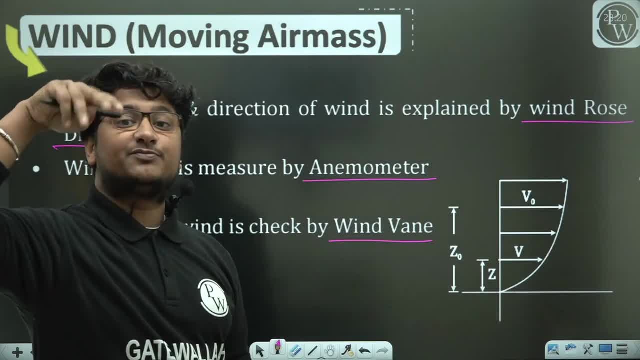 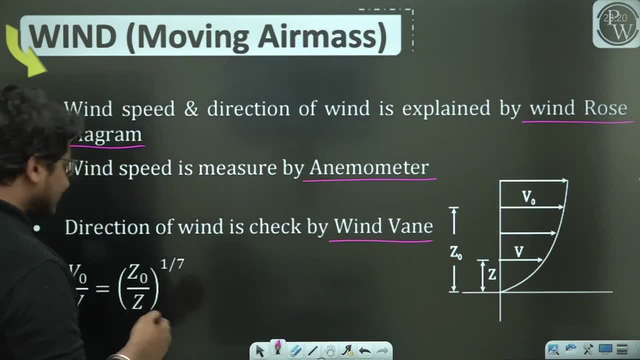 As you increase your height, The speed of the wind Drastically, Exponentially, You are increasing. So to understand that, What have you done? The relation of these two? We call it Seventh law. What is the seventh law? 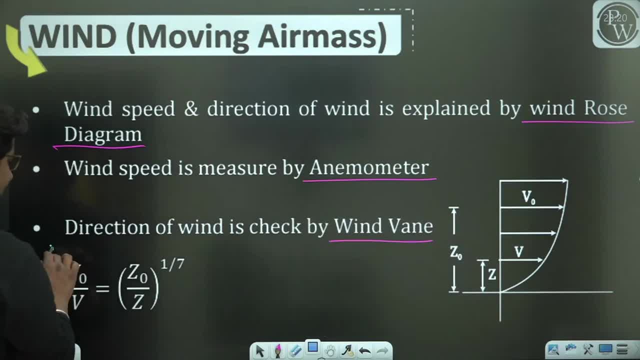 So this is your seventh law, That we is directly proportional to The direction of the wind. The direction of the wind Is directly proportional to Z, to the power One by seven. So V naught upon V is equal to. 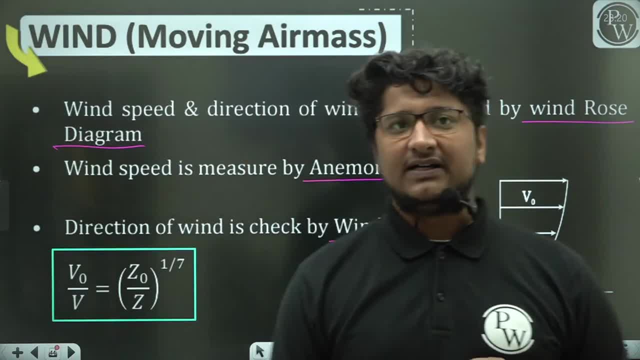 Z naught upon Z to the power One by seven. Keep this thing in mind, Because this is not a derived formula, This is an experimental, waste formula. This is not a derived formula What we have found In the seventh law. 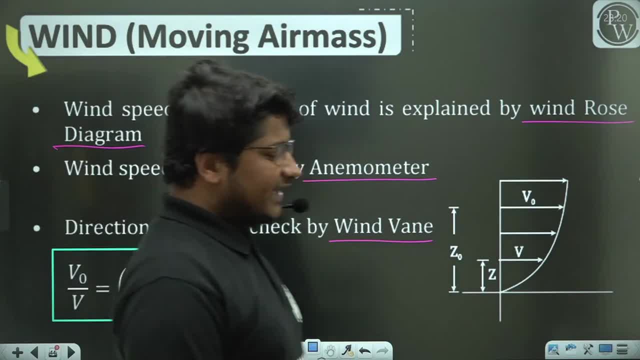 That V is directly proportional to Z to the power, One by seven. That is why Its name is Seventh law. And then we made a relation: V naught divided by V, equal to Z. naught divided by Z to the power. 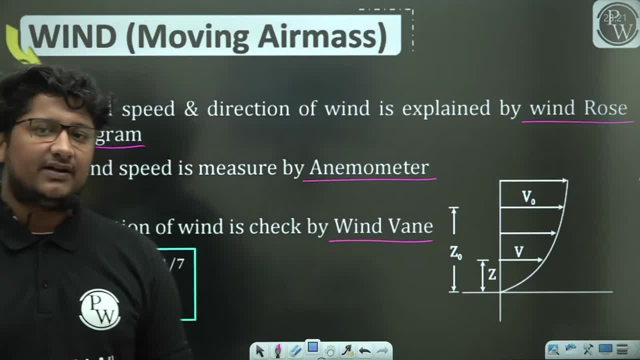 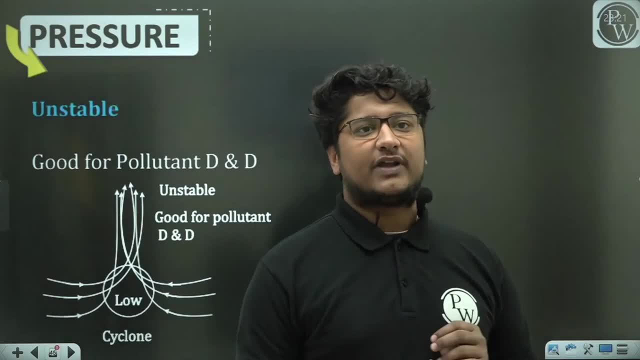 One by Keep this thing in your mind- Regarding wind. So this is the seventh law, And then we have Related to Second law. Now the second thing Is about the pressure. In the second law, Pressure will be An important role to you. 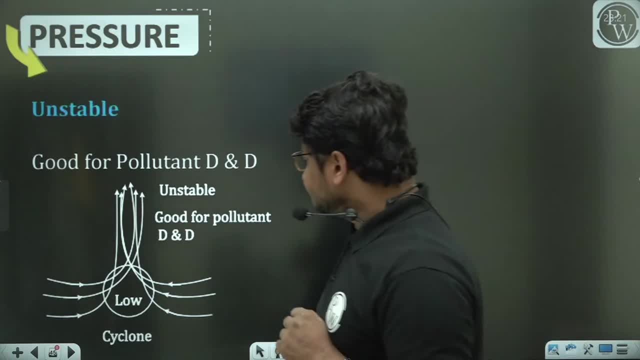 In your pollutant dispersion and dilution. How do we understand this? So what is the condition? Generally, there are two conditions: Either your area Will be in low pressure zone Or in high pressure zone. Now, if your area Is in low pressure zone, 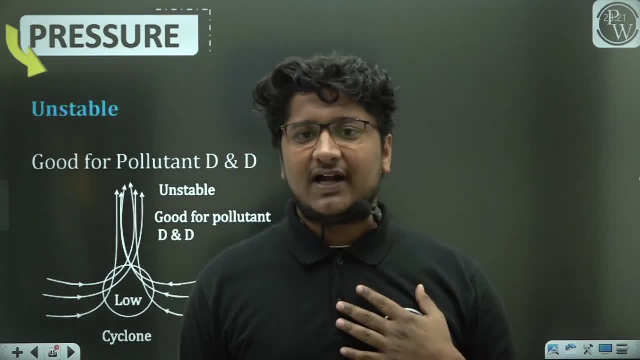 Then you must have read something simple: Where there is a low pressure zone, The air comes from the surrounding area. You get the air from the high pressure zone And the pressure is there. Now the pressure comes from the low pressure zone And the pressure is there. 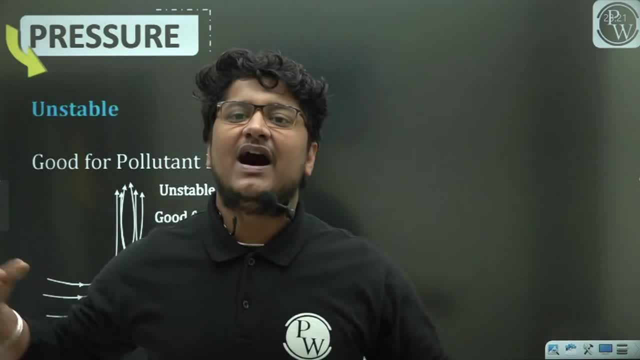 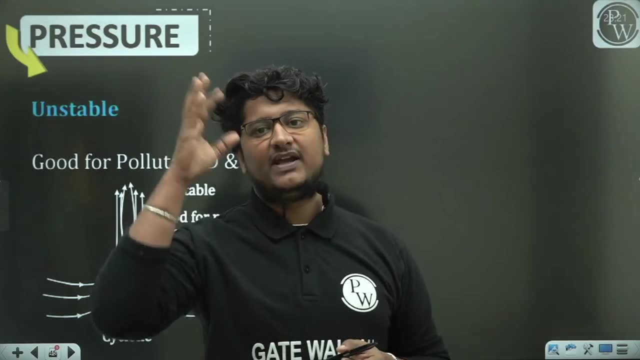 And the air comes from the air. Now you know Where there is a low pressure zone. Air comes from the air. Air comes from nearby high-pressure zones and you want to fill that area there. You must have studied geography in your childhood that if low pressure develops somewhere for 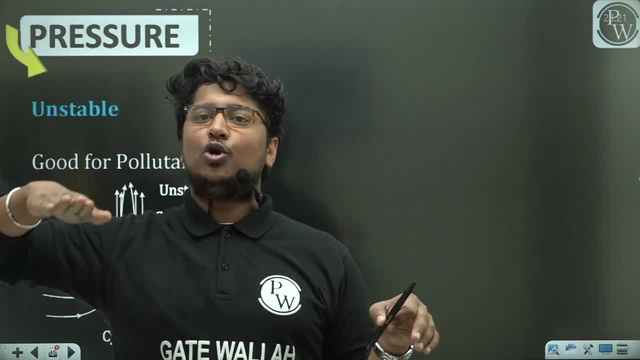 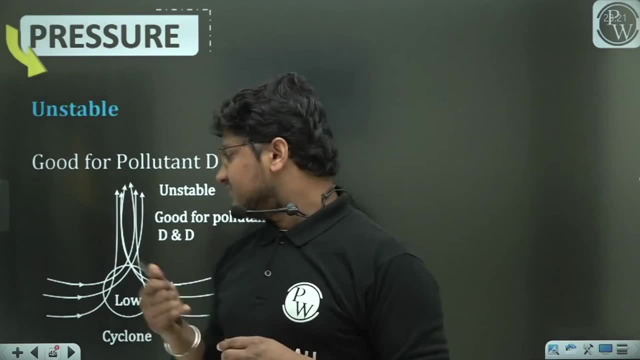 example, if low pressure region has developed in your area, Bihar, UP, then you get air from the high-pressure region of the Bay of Bengal. you must have studied all this in geography. The same thing is that if your area is in low-pressure region, then what will be around you? high-pressure. 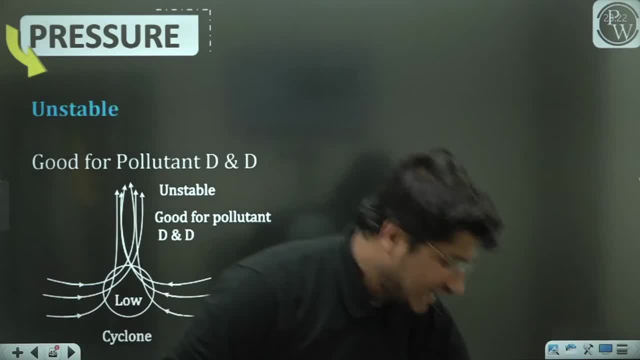 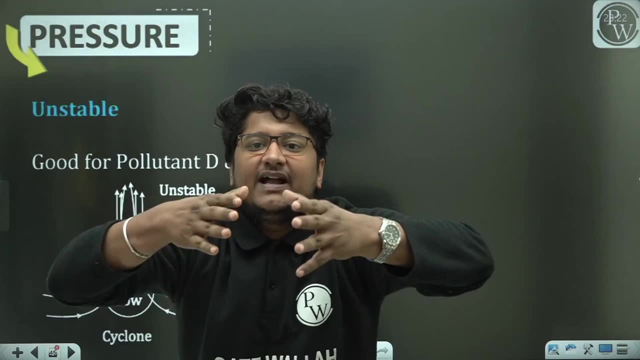 region will be then from all sides. you understand that it is like it is like air is coming from all four sides. air is coming from all four sides. if air comes from all four sides, then it will collide and can not go down after colliding. if it will collide, it will not go down, it will go only upward. 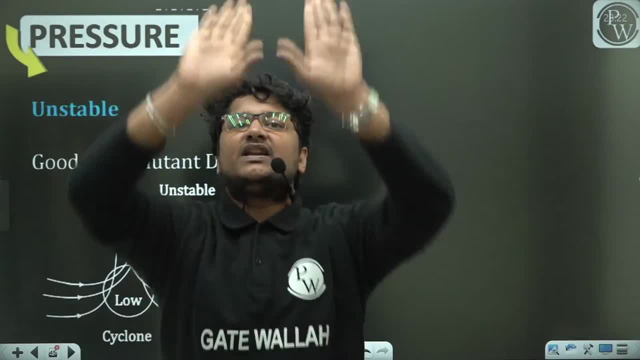 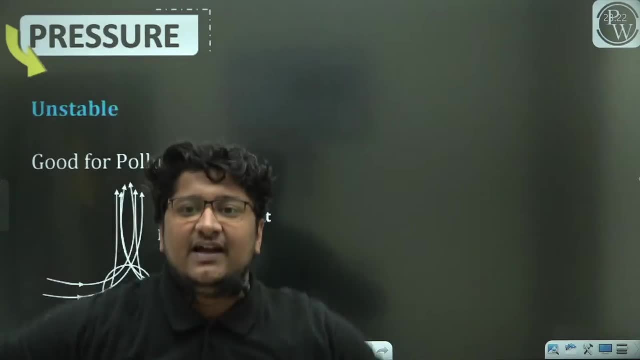 because it will not go down. So when it is going up and at that time you are releasing a pollutant, at that time, if you are releasing pollutant, then it came up with the air. it came up with the air points of view. 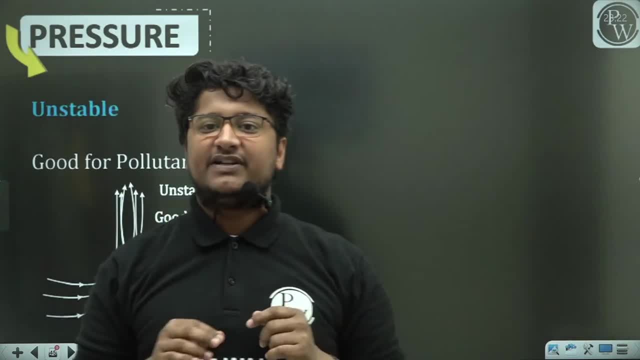 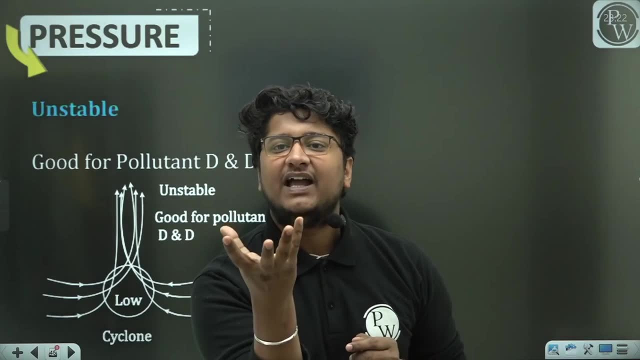 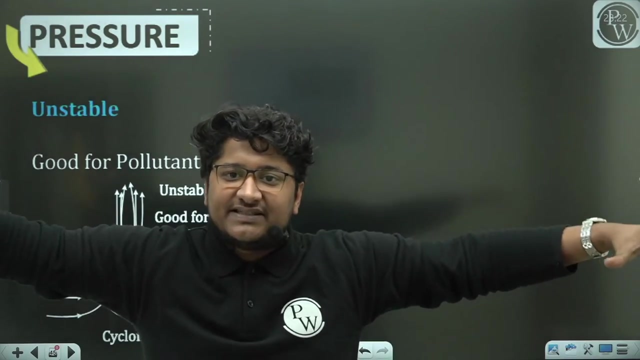 So this condition is good or bad for pollutant dispersion and dilution? You guys will comment. You guys will comment: For example, this is your area which is in low pressure region. The whole area is in high pressure region. Due to high pressure region, air will come and it will fill up this area from all the directions. 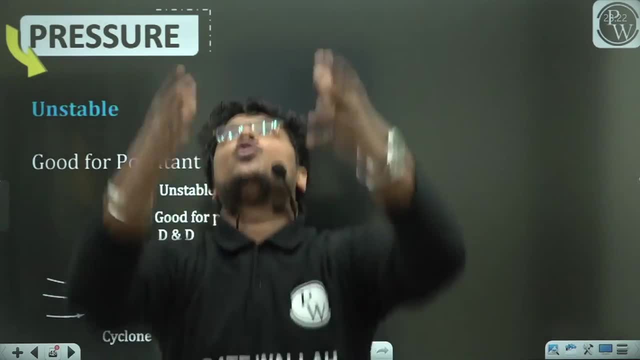 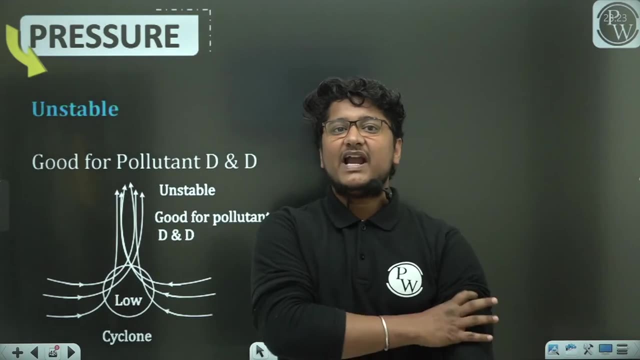 So, from all the directions, air will come from all the directions and air will come from all the directions. So in this case, if you will release pollutant, it is good or bad. It is good, It is good. So what do we call good condition? 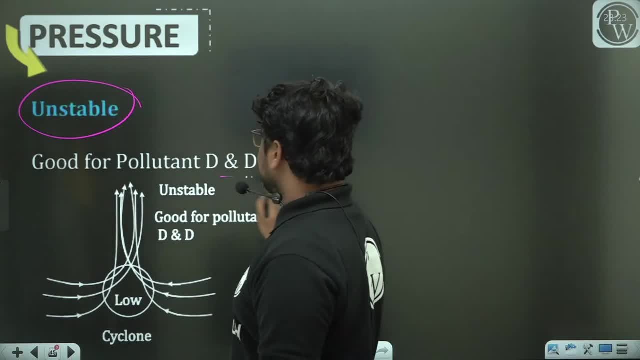 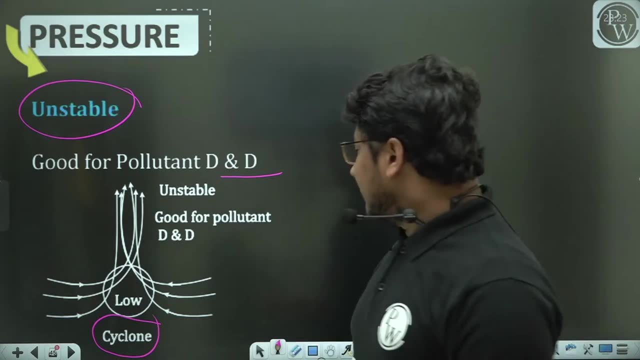 Unstable And it is good for pollutant dispersion and dilution. And what do we call such condition? Cyclone? Sir, cyclone has come. Okay, Someone's opposite, Someone's second brother. Anti-cyclone, Your area is in high pressure region. 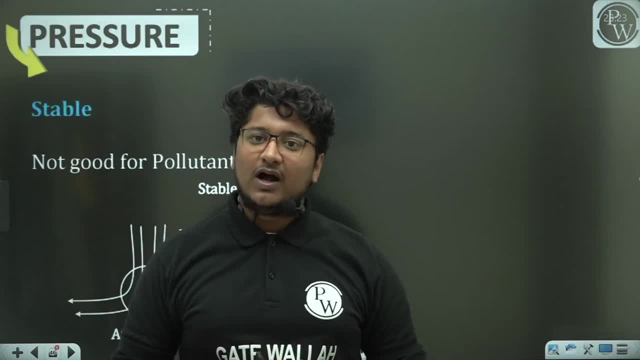 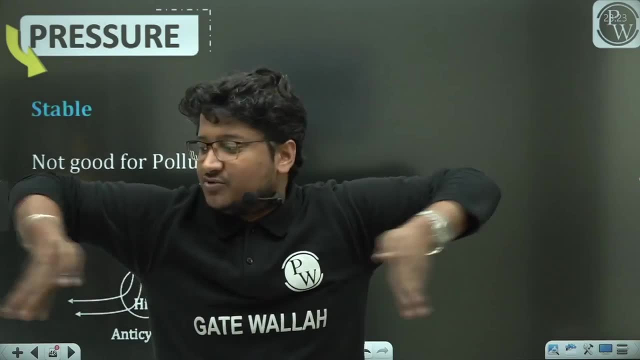 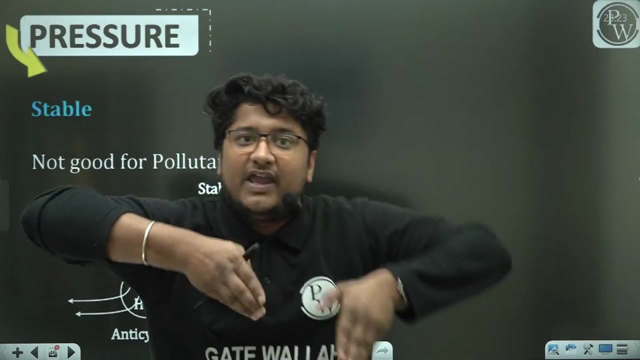 Outside area will be in low pressure region. In this case, what will happen? Air will be coming out of your area. It will be going towards low pressure region. Now, when it will be coming out, it will be moving urgently. And when it will move urgently, and if you will release any pollutant there, 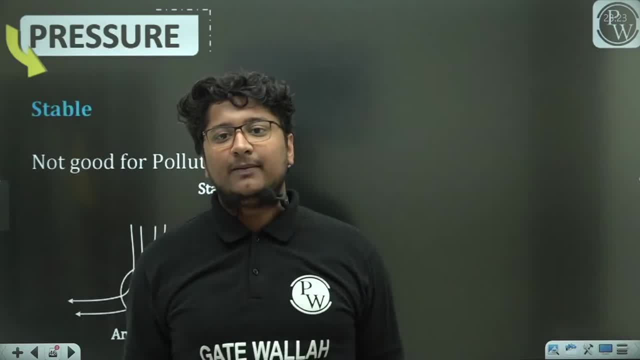 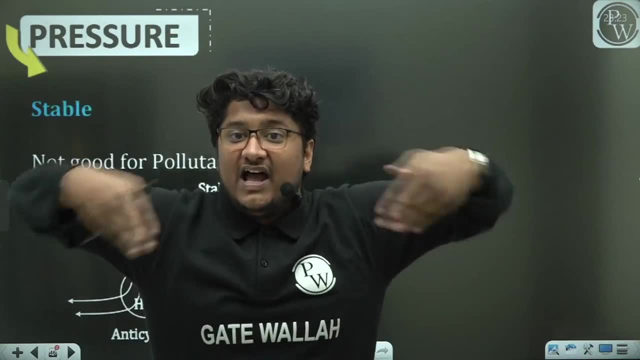 it will spread it on the horizontal level. So is it good or bad? The pollutant that you will release due to high pressure region air is coming out of there. Air is coming out of there. Air is not coming there. 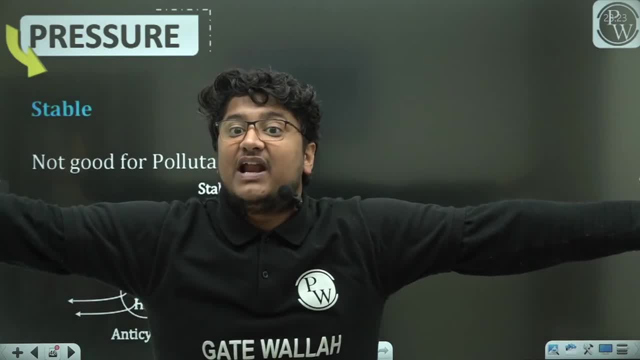 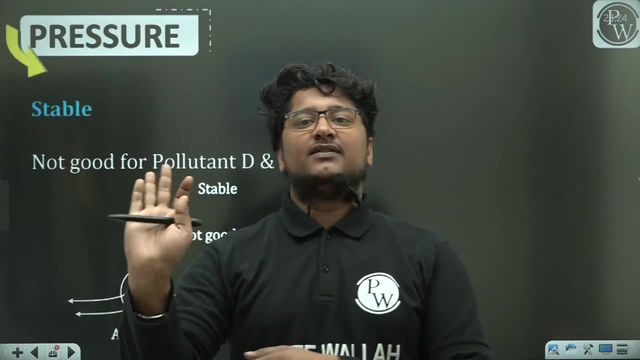 Air is coming out of there And it is gliding urgently. It is gliding urgently. So what will you do? It will spread your entire pollutant downwards. That is not good for you. It will spread you on the opposite ground level. 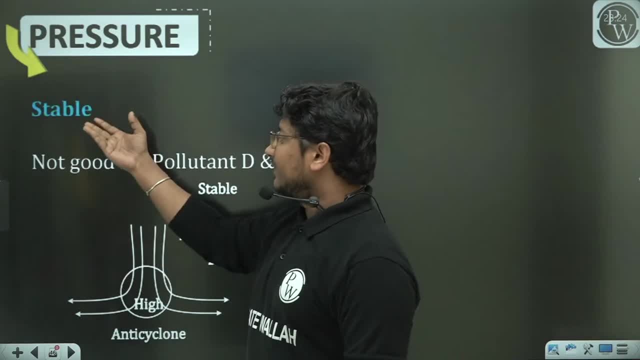 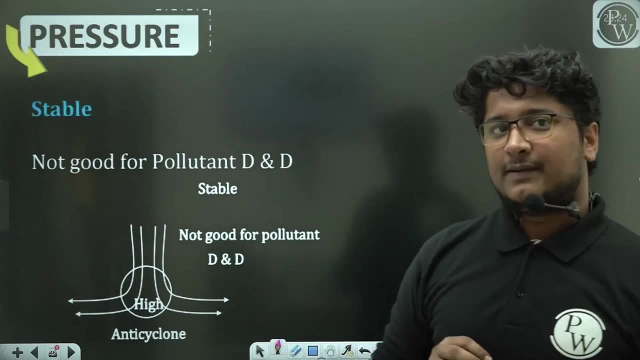 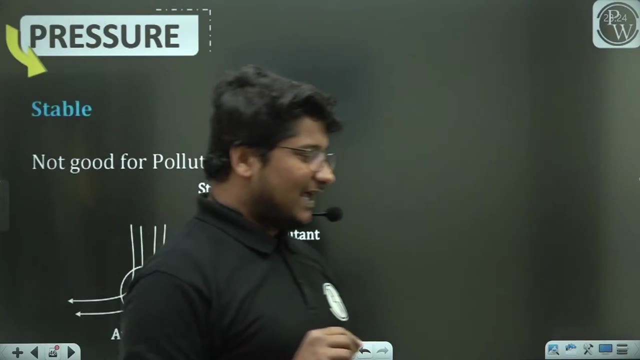 This is something that we call as anti-cyclone. Obviously, it will be stable And not good for pollutant dispersion and dilution. So you have understood how pressure impacts. You have understood how pressure impacts. Now one question from you people. 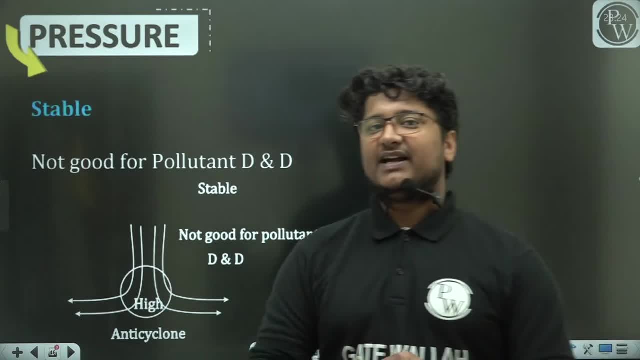 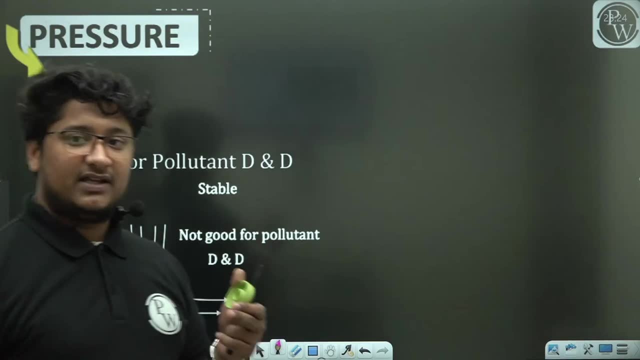 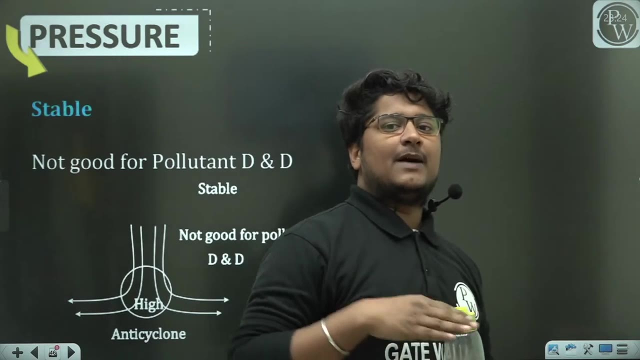 We have discussed pressure. So according to height, does the pressure increase or decrease? According to height, does the pressure increase or decrease? If you are changing your elevation, the pressure is increasing or decreasing. For example, let us say you are going up. 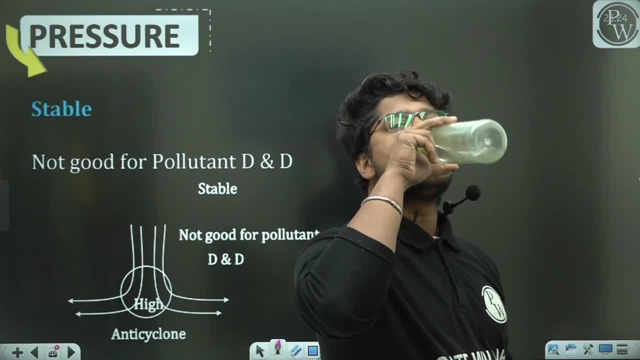 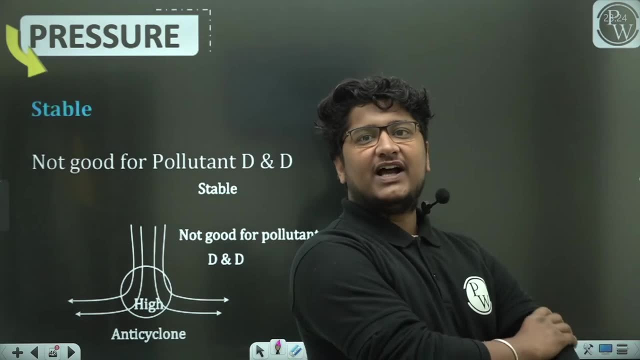 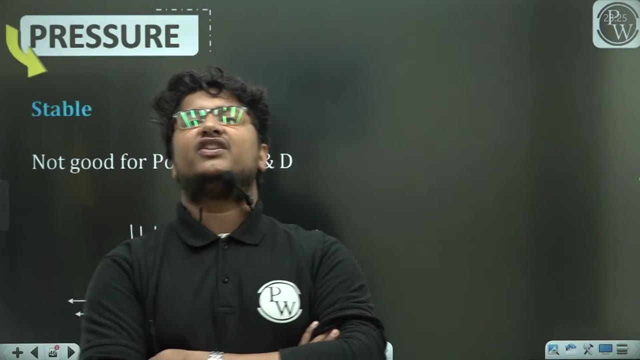 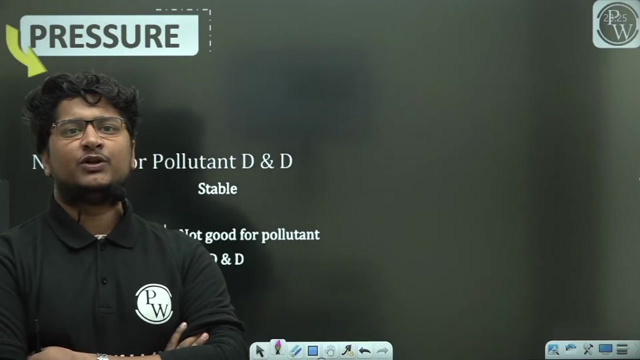 You are increasing your altitude. Tell me quickly: Does it decrease? Why does it decrease? What is the reason for decreasing? You people said that when you are going upward, your pressure is decreasing. What is the reason for decreasing? What is the reason for decreasing? 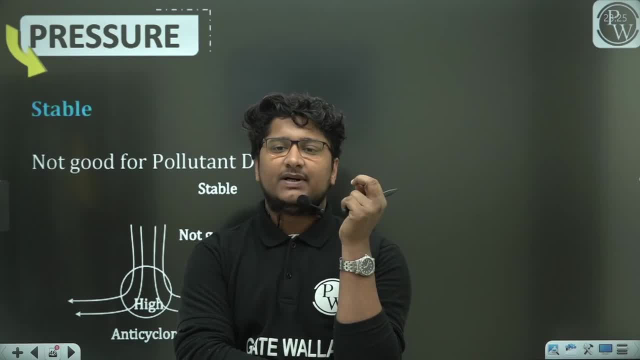 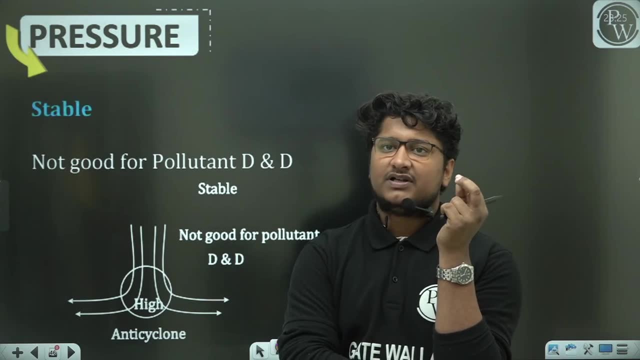 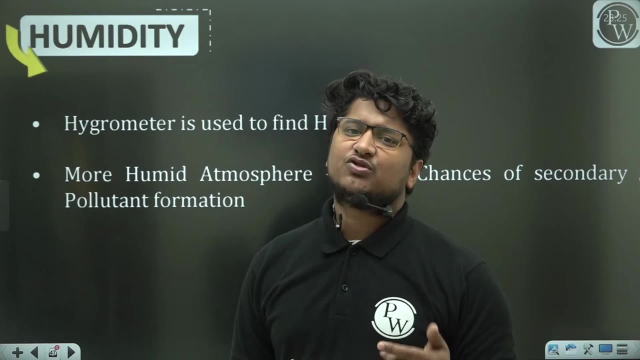 Density of air. It is nothing but density of air. It is nothing but density of air. Very good, Let us move ahead. Next one is humidity. Now, if humidity will remain in your air, then secondary pollutant will form more. 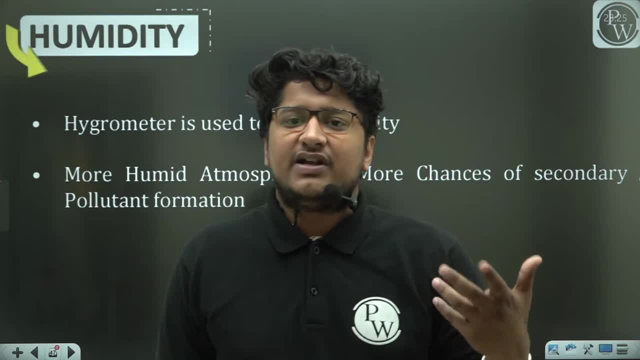 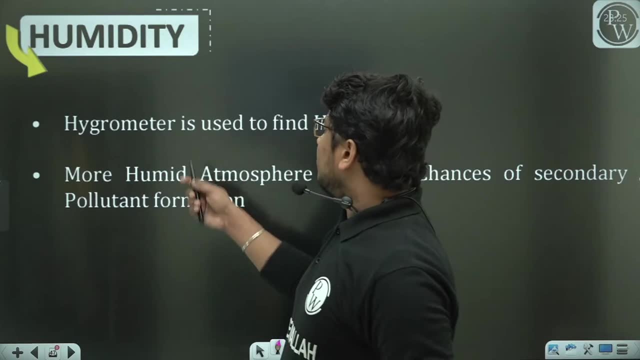 Socks and nocks were rotating like this, But if there is humidity in your atmosphere, then those socks and nocks will be converted into acid rain, So it will make you secondary pollutant. So, to measure your humidity, remember the name of your device. 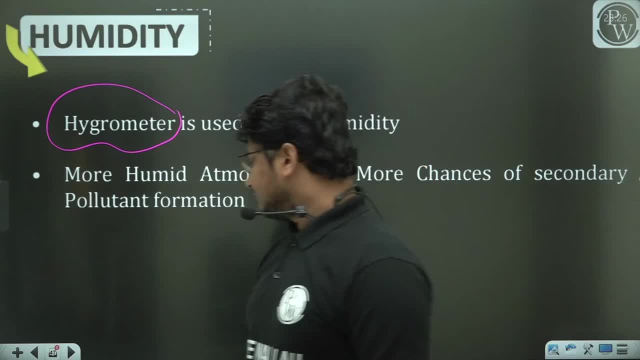 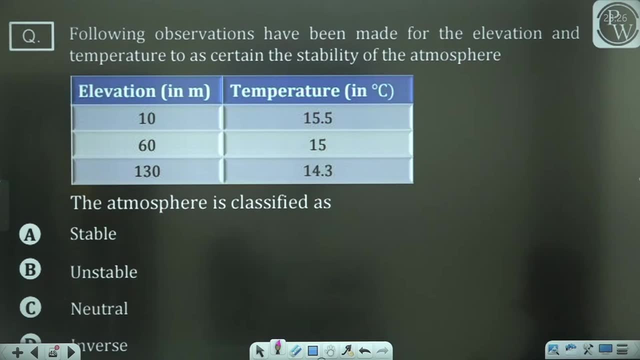 That is hygrometer. Is it clear? Let us move ahead. There is a question. Answer it easily. Now. your theory part is a little done. There is a little more theory which we will see later, But before that some questions. 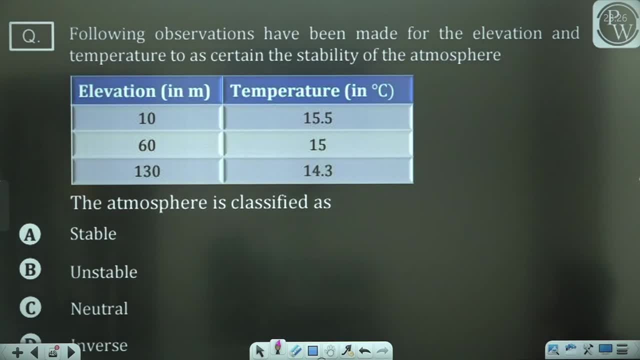 Answer it easily. There is nothing to be afraid of. Solve the question and answer it. What is Jobless Engineer saying? Does oxygen decrease, Did I ask you? I am talking about Fisher. Does oxygen decrease? Yes, Yes, Yes. 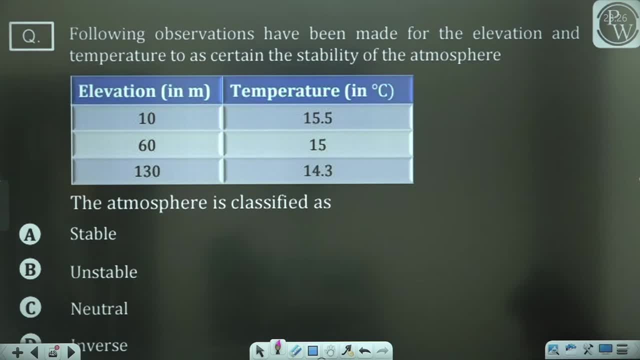 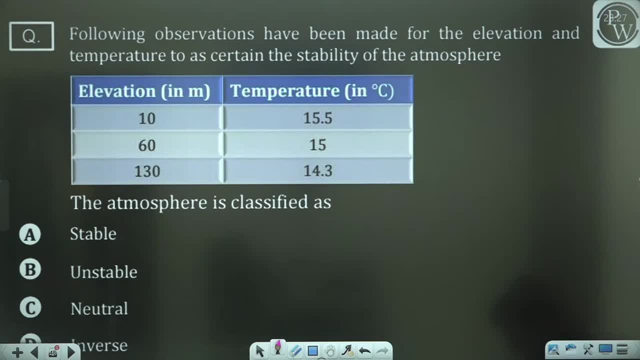 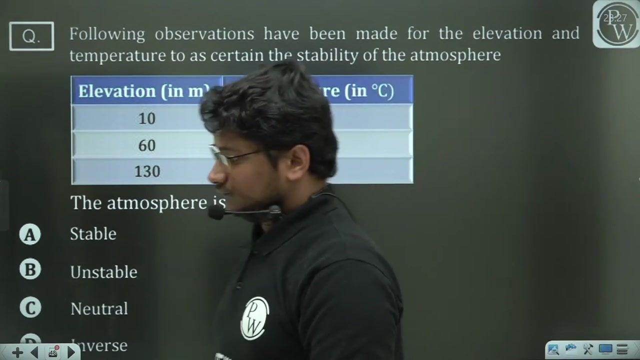 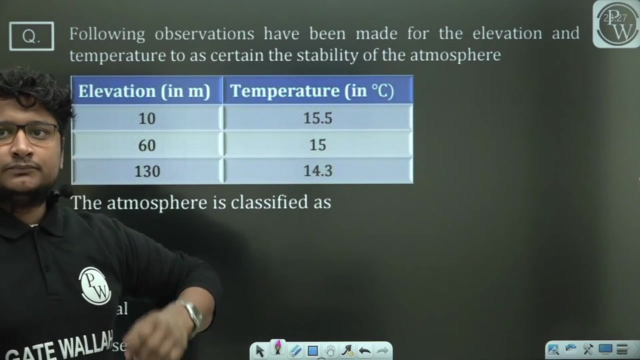 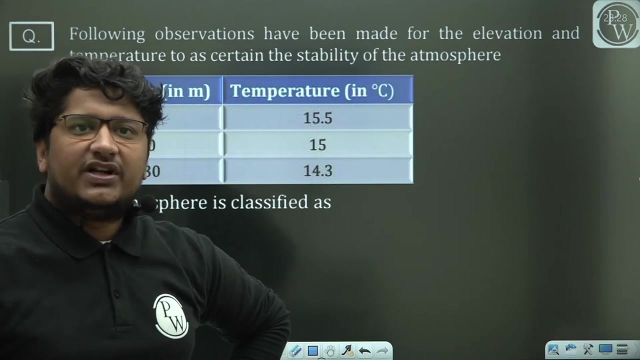 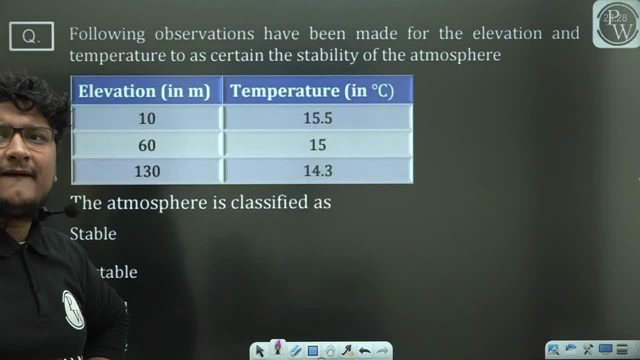 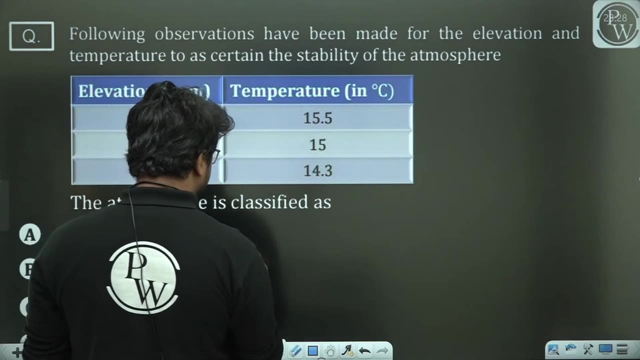 it's not sick. simple question is, sir, hum ko malum hai ki ALR to constant hai, uske regarding toh koi baat karta hi nahi hai, sir, that is minus 9.8 degree Celsius per kilometer. superb, ye, toh constant hai, sir. 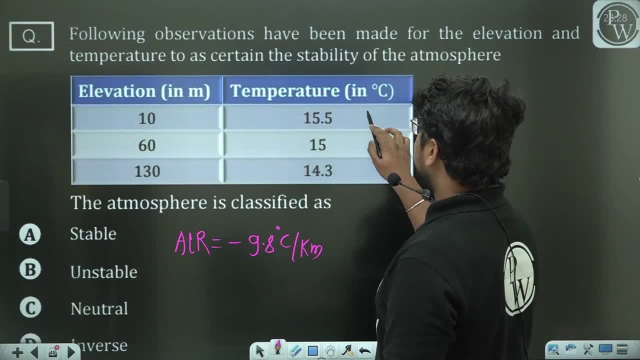 toh baat karenge, sir ELR ki. toh dekhiye: 2 ELR nikal sakta hai. ek yahan se nikal sakta hai, sir, ek yahan se nikal sakta hai. toh let us say first: ELR 1 nikalte hai. 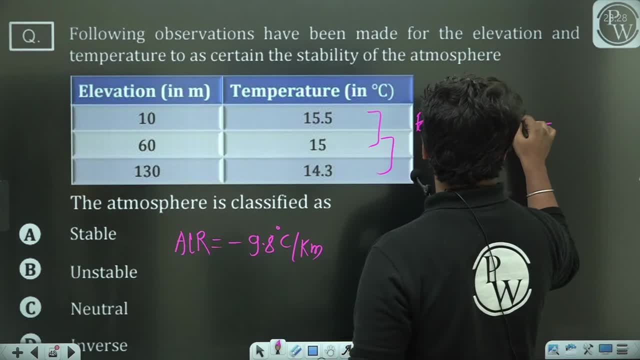 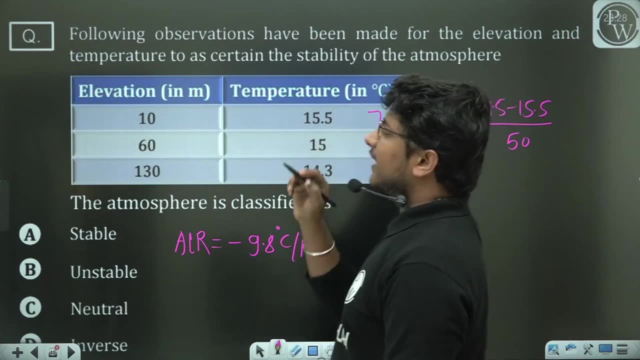 change in temperature kitna ho gaya hai 15 minus 50.5, bahut badya. divided by 2 distance ho gaya aapka kya 50 hoge aap ye 50 ke liye aap gaya matna per meter aagea. 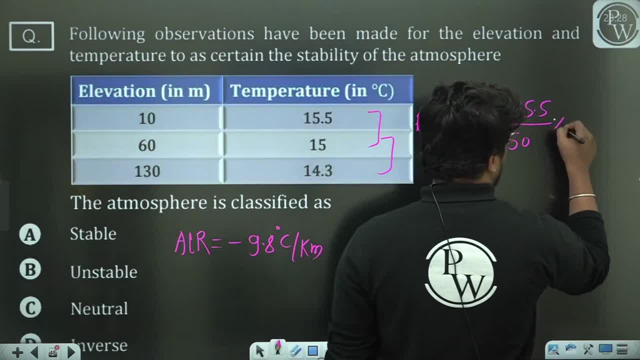 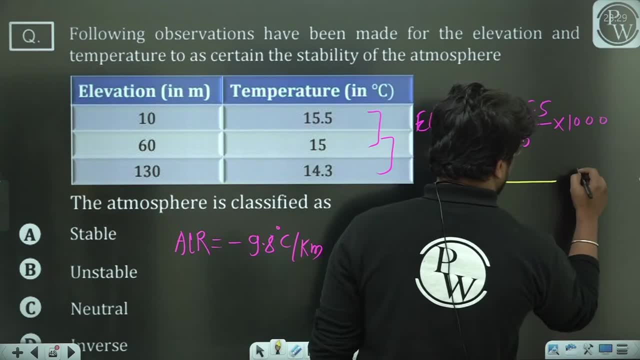 aapko nikalna hai per thousand ke liye, matna per kilometer ke liye. toh thousand se multiply kar, do kitni aayi ELR ki value. ELR ki value kitni aayi in a degree Celsius per kilometer. 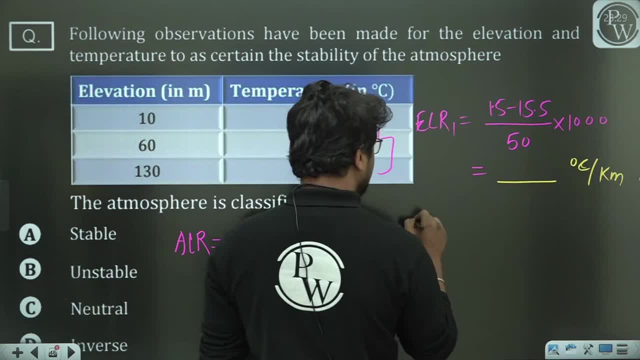 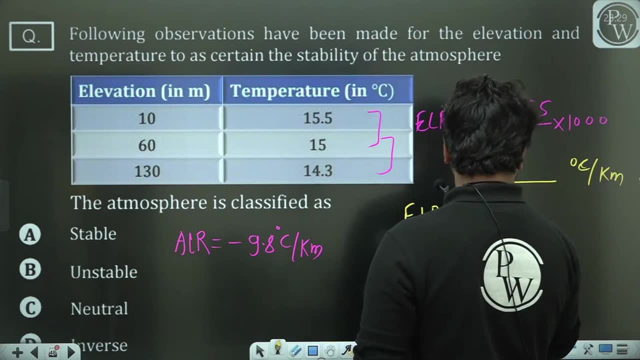 jawab: aap log doge same, agar mai baat karo aap se ELR 2 ki toh 2 ka kya ho jayega? 14.3 minus 15 divided by 17, plus 23 divided by 16. 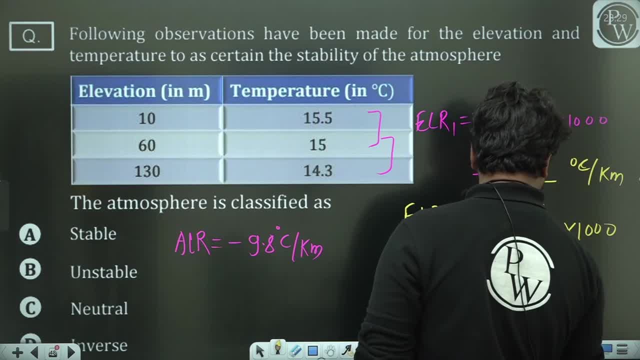 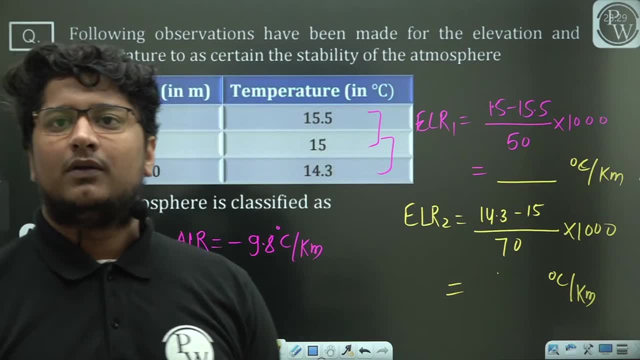 plus 18, divided by 19 minus 20, multiplied by 0. crab 40. 20 divided by 15 minus 15 plus 30 plus 11 times SUN, is 21, 12. 12 minus 10 equals 15 plus 64. 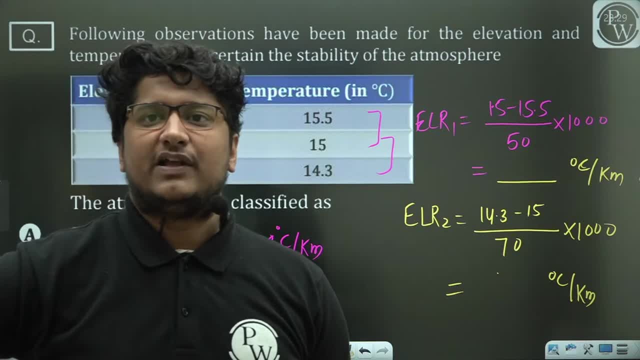 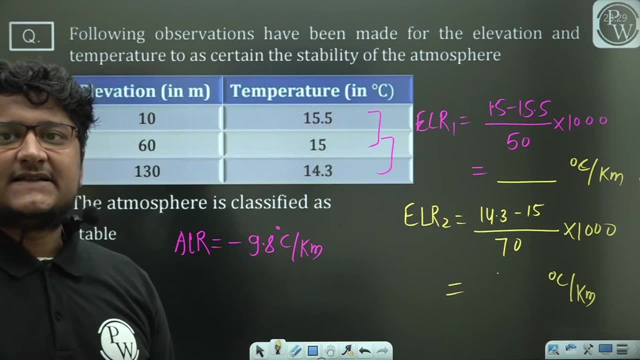 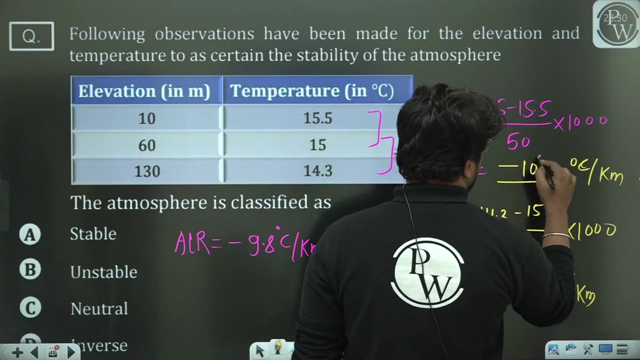 plus quickly jump for 10, 29, 80 exactly. we will consider participate in a video of 12 toh 12, 14 into 11, 12, 22, 20 degrees Celsius per kilometer minus 10 degrees Celsius per so this you are getting minus 10 degrees Celsius per kilometer here also, I think. 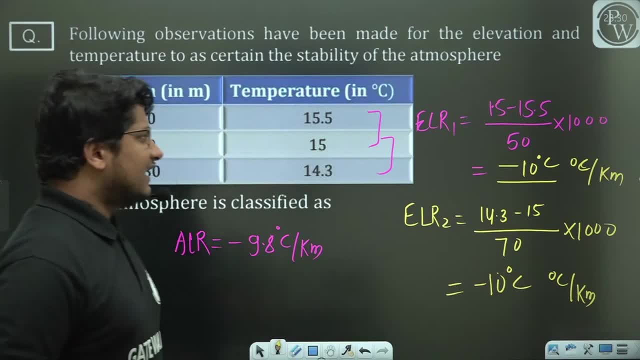 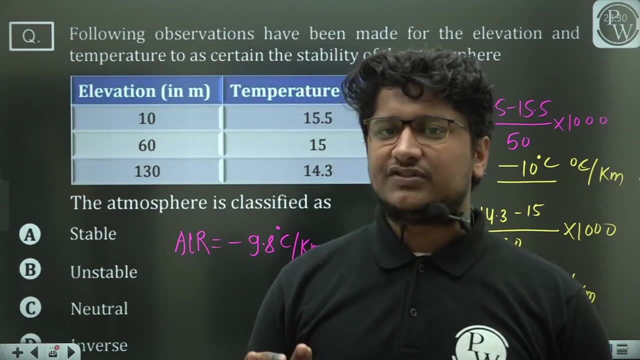 you must be getting minus 10 degrees Celsius per kilometer. so you tell me both are same. take ELR1 or ELR2, both are same. tell me that if ELR1 and ELR2 both are same, then take any one of them, it will work. 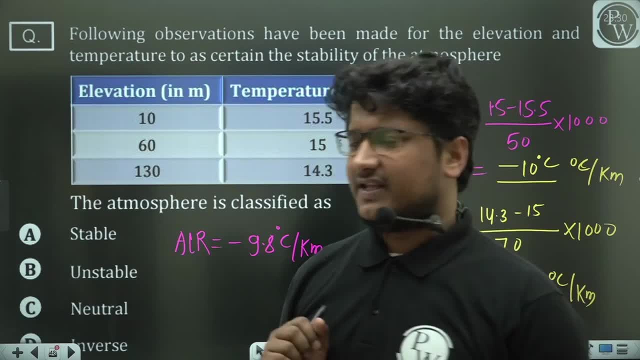 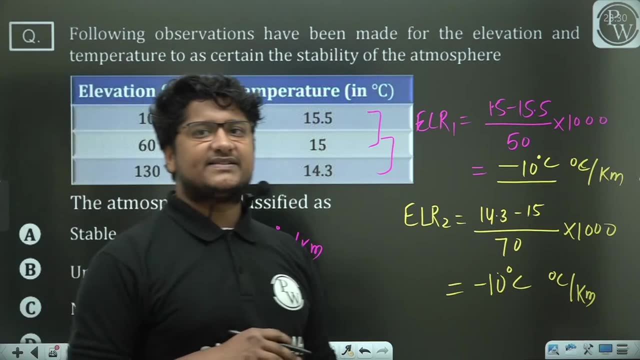 is the value of ELR more or ALR is more? tell me by commenting: you are getting ELR minus 10 degrees Celsius per kilometer and ALR is your minus 9.8 degrees Celsius per kilometer. what does this mean, ELR, if you are getting minus 10 degrees Celsius per kilometer? 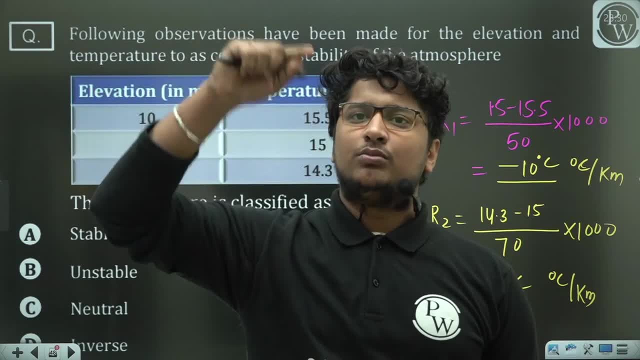 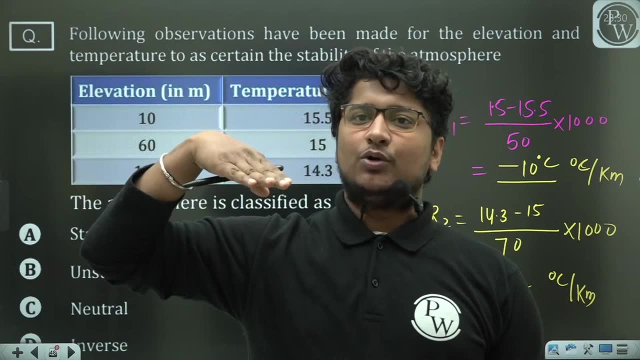 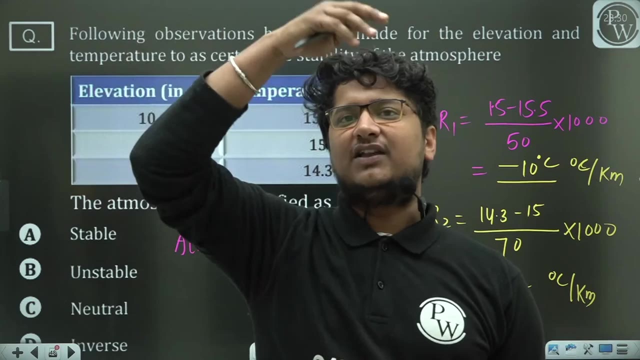 what does this mean? if you go one kilometer up, Modi ji also came. wow, greetings to Modi ji. come here, let's talk. if you go one kilometer up, please say my greetings to Modi ji. Why do I have to do this? If the name is before the surname, then Hiram Modi can also be and Nain Modi can also be. 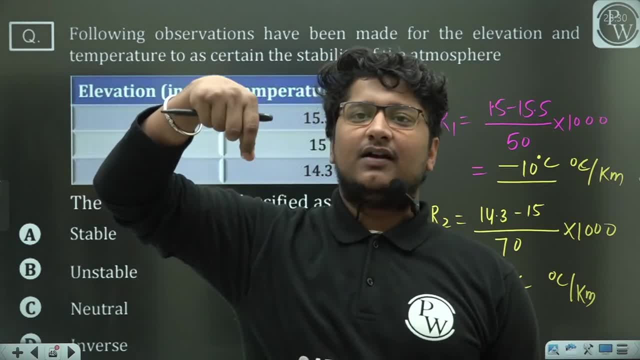 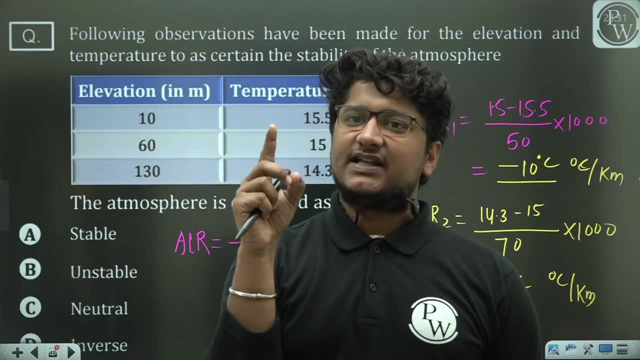 Get lost. I was bowing. What was I talking about? When you are talking about ELR, if you say minus 10 degrees Celsius per kilometer, then 1 degree Celsius means if you go up 1 kilometer, then your temperature is decreasing by 10 degrees Celsius. 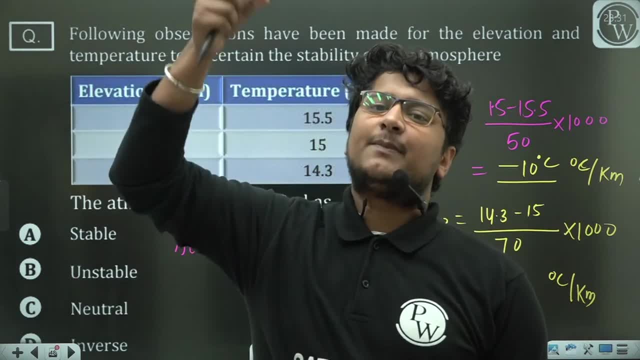 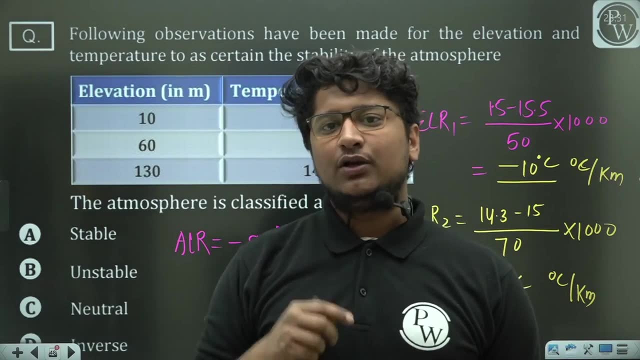 This is your meaning And what is your ELR? If you go up 1 kilometer, then it is decreasing by 9.8 degrees Celsius. So obviously, sir, ELR is more visible. So if ELR is more than ALR, then what is the condition, sir? 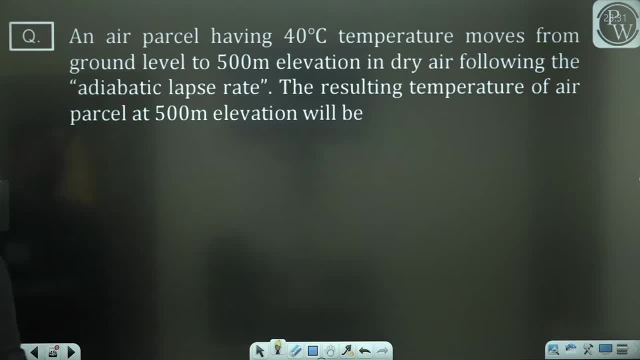 Unstable, Without any doubt. Next condition: You have to make it fast. Simple question, sir: 40 degree Celsius is the temperature. You went up 500 meters and you were following the dry air. Dry air follows the temperature, So you have to make it fast. 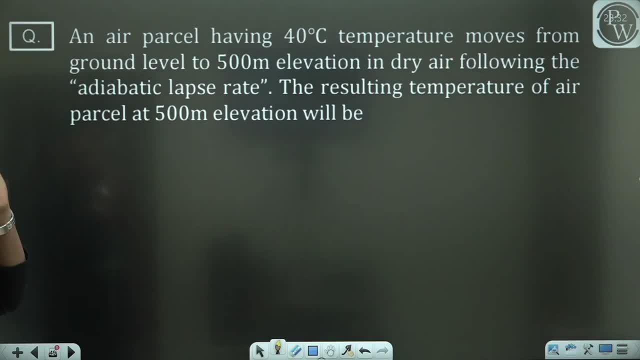 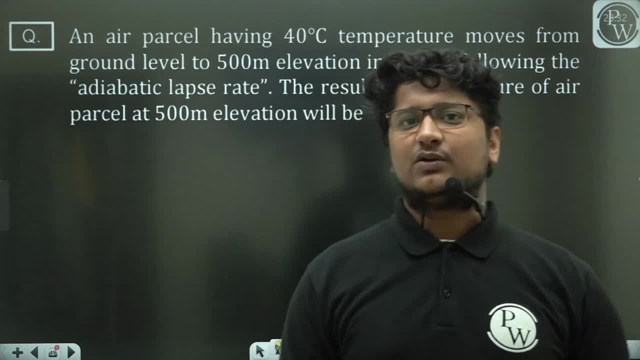 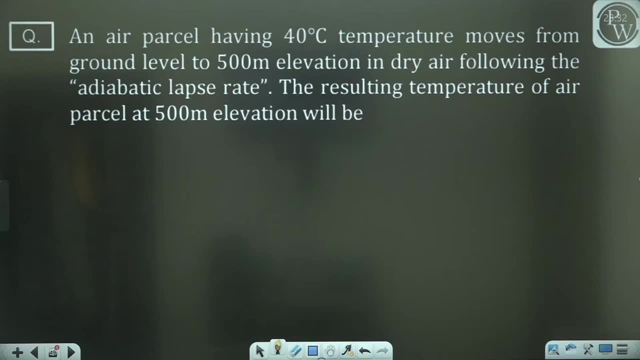 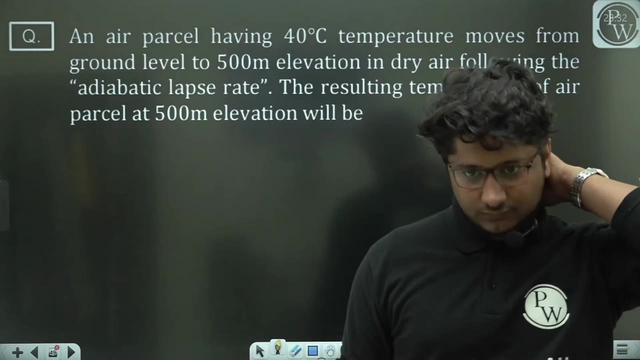 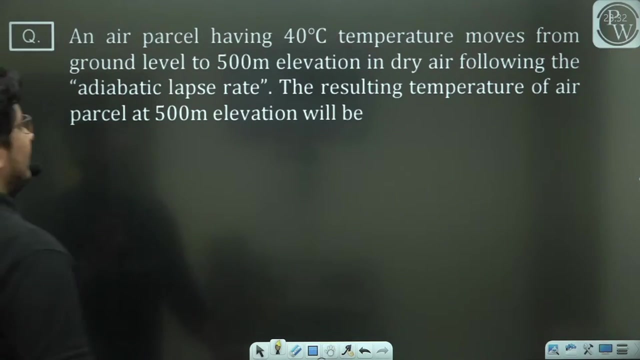 So what happens if you go up 500 something meters result in temperature. It is 1 minute, It is 1 mark. So it is an easy answer for you guys. Good Sir, it is 40 degrees Celsius. if I talk about minus, then, Sir, look here. Sir, generally, if you go, 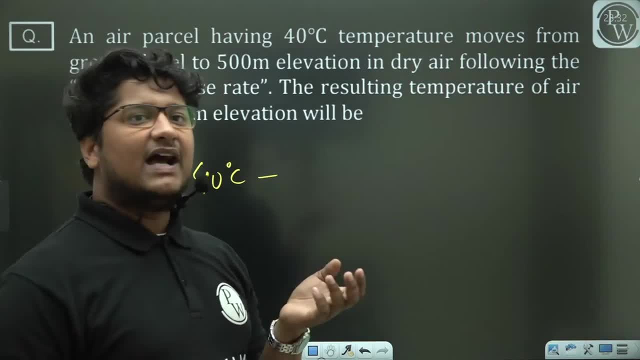 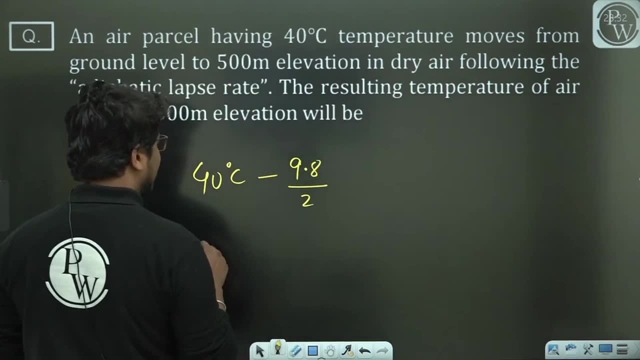 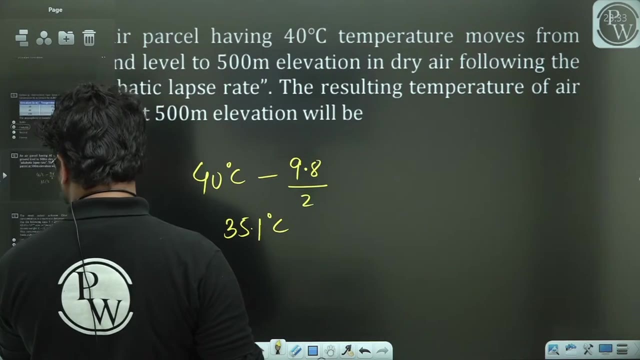 one kilometer above then 9.8 degrees Celsius used to decrease, Sir. what are you doing here, Sir, going half a kilometer above then 9.8 divided by 2, about 4.9, means 35.1 degrees Celsius. very good, next question. you have next question. 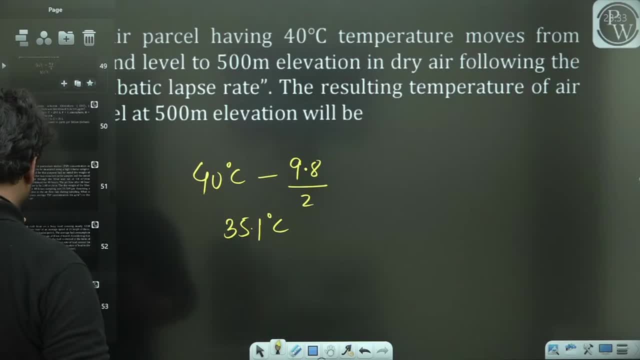 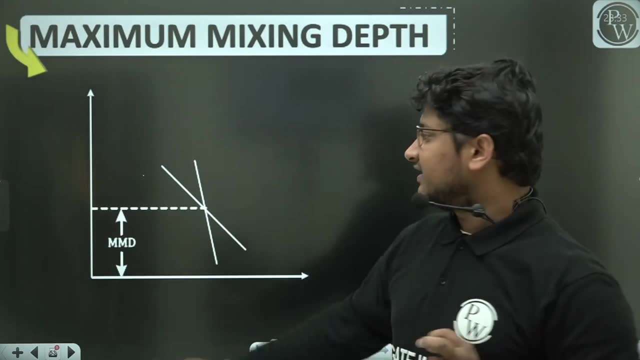 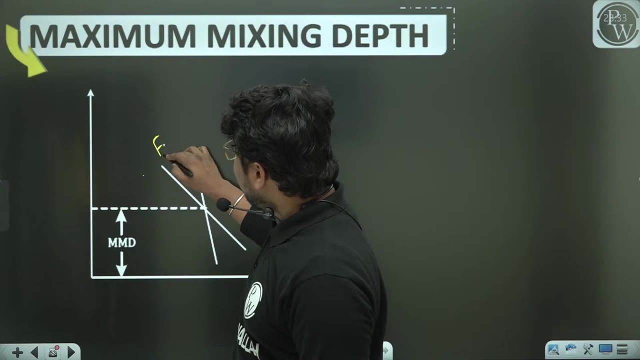 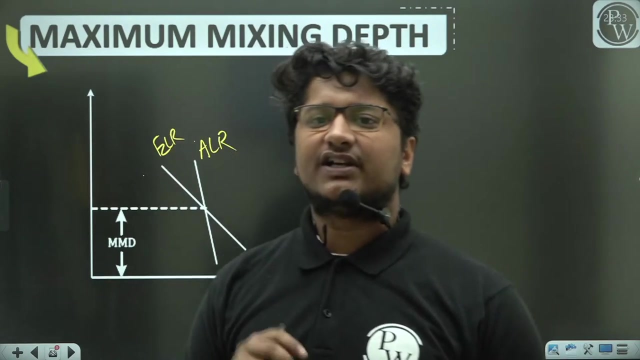 we will look at it later. it is a similar question. next term, we understand mixing depth. it is a small term. it is not a very difficult term. what is this term? basically, you just saw ALR, you saw ELR. so let us say: this is your ELR and this is ALR. if you look at both of them, it is possible that both are crossing one place, so where they cut each other. we call this height, maximum mixing depth. 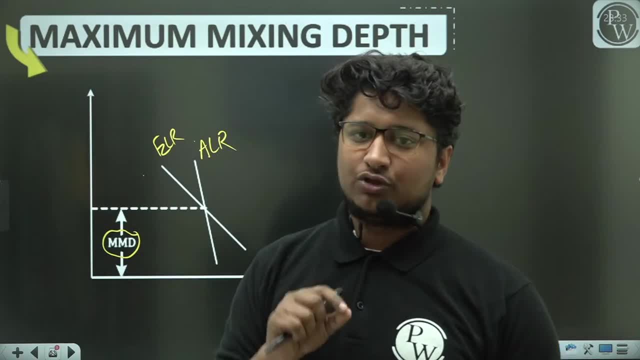 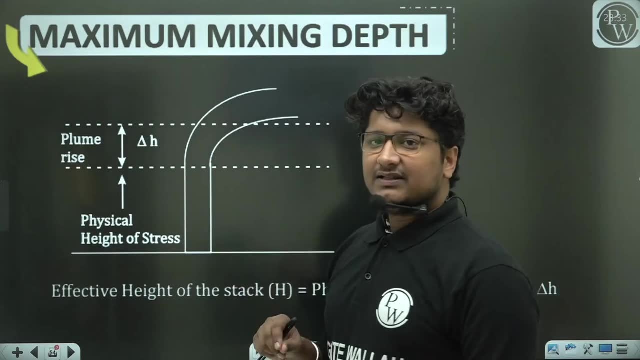 and our attempt is that you give the height of the stack above this. so you give the height above this with maximum mixing depth. take care of this. it is a small term. second thing, that if you look at the total stack height, then one is your physical height. 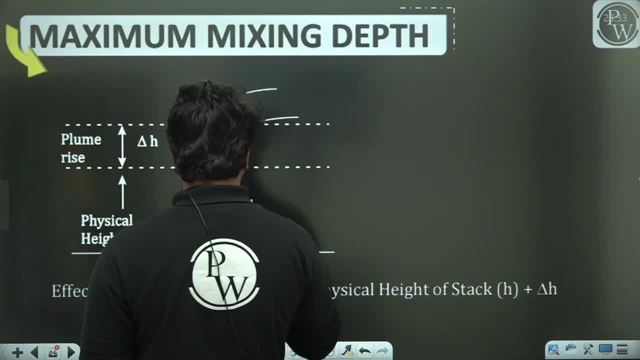 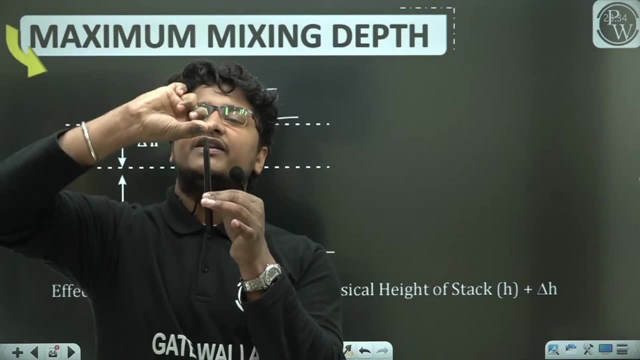 one is your physical height, which you are calling small h, and one is your plume rise. now understand this thing, that, for example, this is your chimney, so the plume comes out and does not turn from here. it goes a little up and then turns. 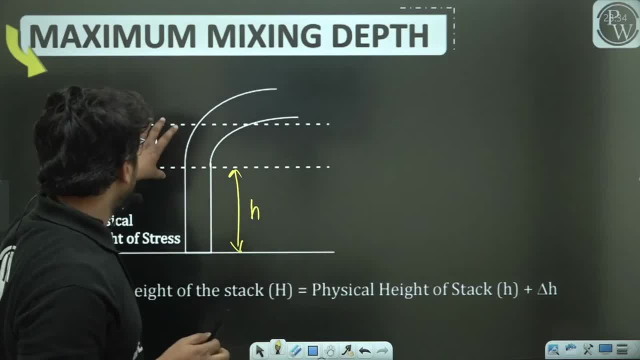 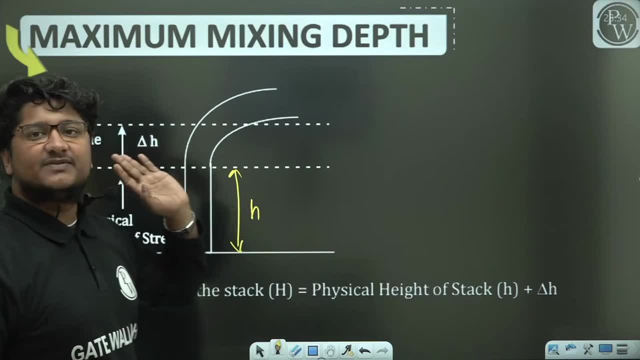 so the distance that you have gone up, you call it plume rise. you call it plume rise then the total height that you will be kept. what will be your physical height plus plume rise? you will take care of this thing. 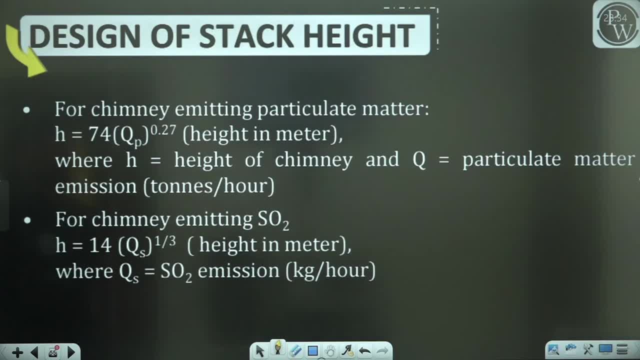 Now regarding your small h, some formulas have been given regarding it. basically, these are empirical equations, so you have to keep this in your mind. it can ask you many times in one mark. by the way, it has not been asked yet in the gate, but ask who knows. 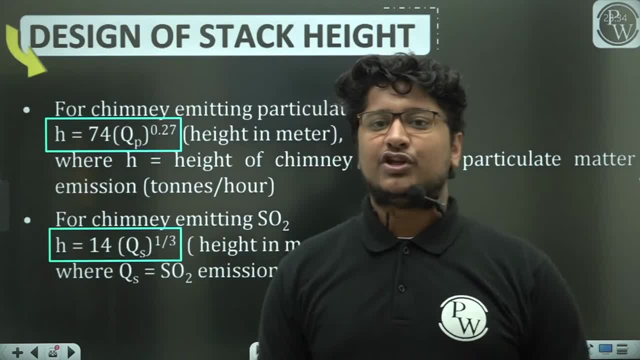 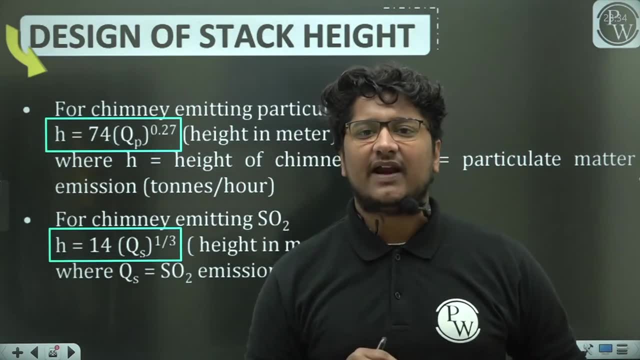 okay, so the formula given here is an empirical equation. it is given on the basis of two parameters, of two things, assuming that our pollutants are coming out, they are generally coming out of thermopower plants and the pollutants that are coming out will be more SO2 or particulate matter. so on the basis of these two, 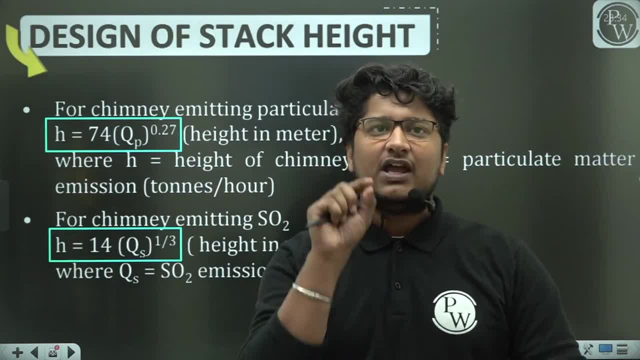 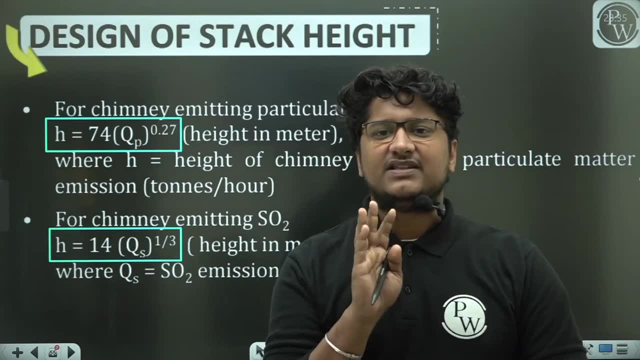 we have given an empirical equation. if you see the first empirical equation, then you have it on the basis of your particulate matter. that is, h equal to 74 qp to the power 0.27,. now you will pay attention to this. here your qp is in tons per hour. in tons per hour, and if you talk about 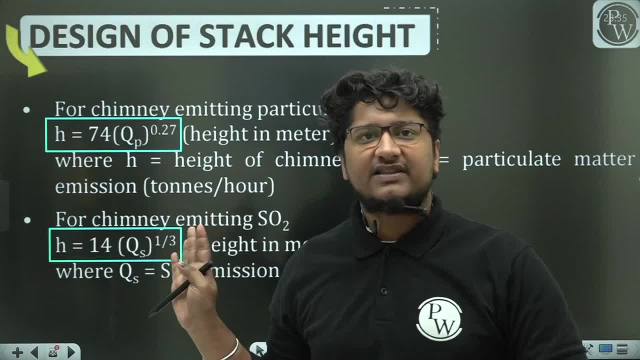 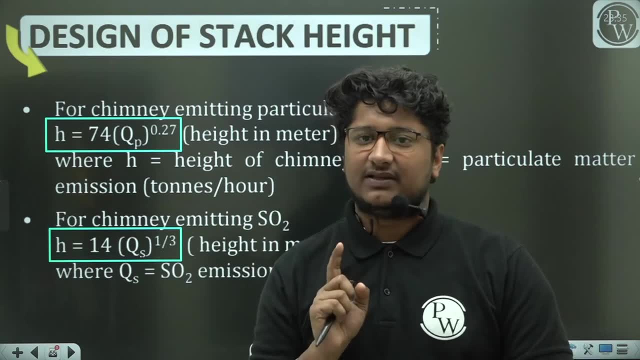 chimney SO2, then how much is your h 14 qs to the power 1 by 3? and here your qs is your SO2 emission and it is in kg per hour. so it is an empirical equation. so you have to take care of the unit, okay. apart from this, 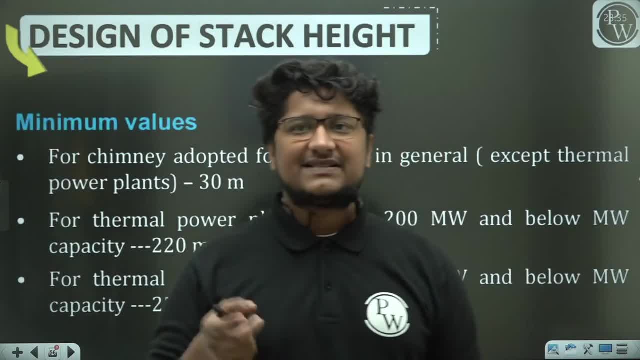 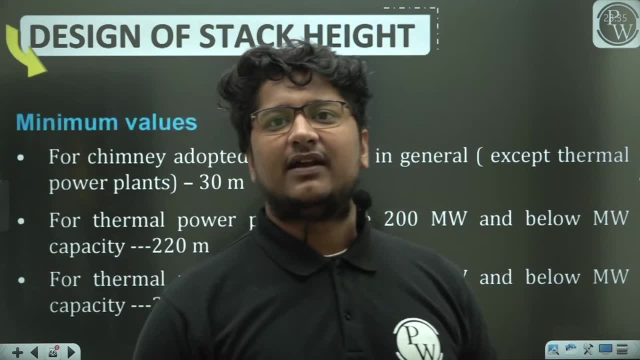 you also have. apart from this, you also have a standard. this is the value that you have taken. it has been done, but apart from this, you also have a minimum value. decide, we will take a screenshot. you will have the whole. 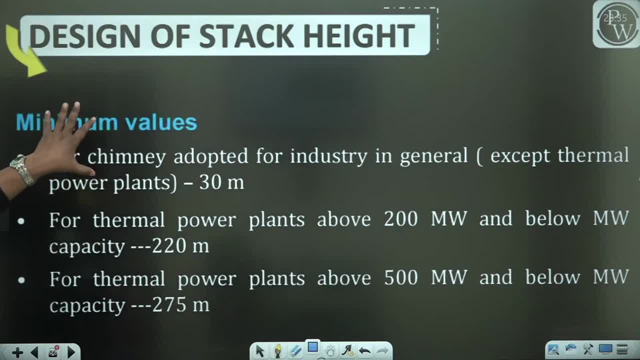 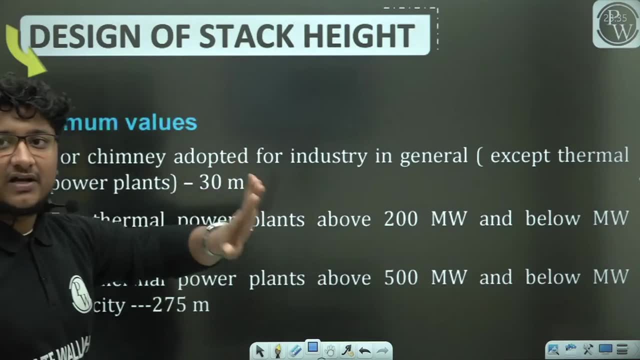 pdf. so why are you getting worried now? you have given the minimum value. see from this for chimney, adopted for industry in general, except thermopower plant, you will keep the minimum height of 30 meters, brother. if it is less than 30 meters, then also give the height of 30 meters. secondly, if the thermopower 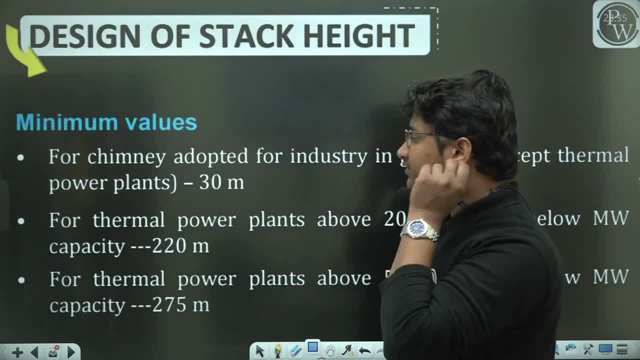 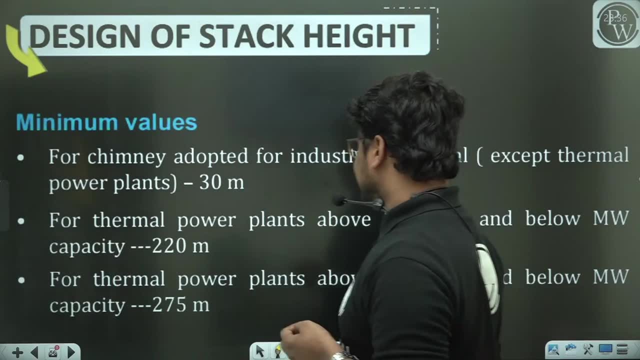 plant is more than 200 megawatts or is below that, then you will keep 220 minimum height. and if your plant is more than 500 megawatts, then what will you keep? in such a case, you will keep 275 meters. keep. 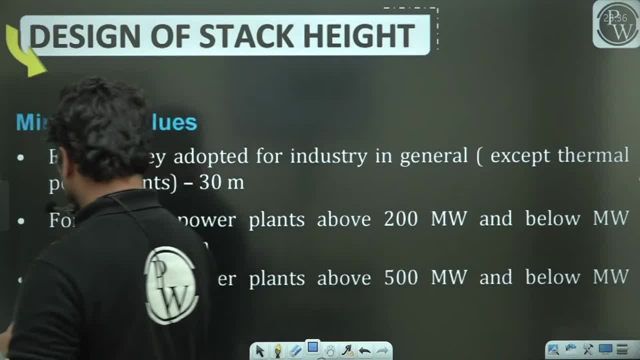 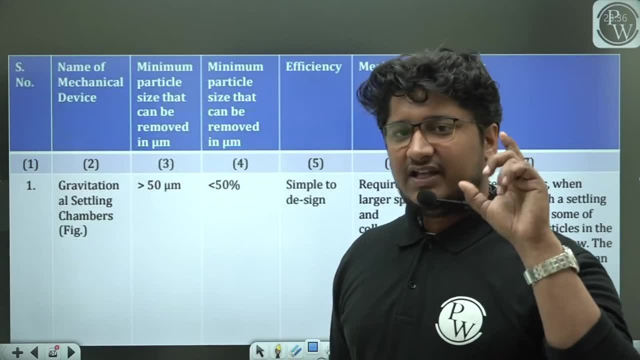 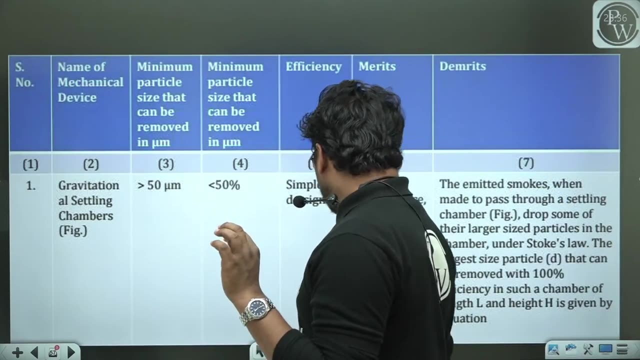 this thing in mind. this is the minimum value which is given to you in the standard. come on now, before going to the next numerical part, understand a little bit. here you have to focus. I will underline you carefully. if you keep that thing in your mind, that will be enough for gate exam. you have to study a little more for other exam also. then you can read the pdf once. 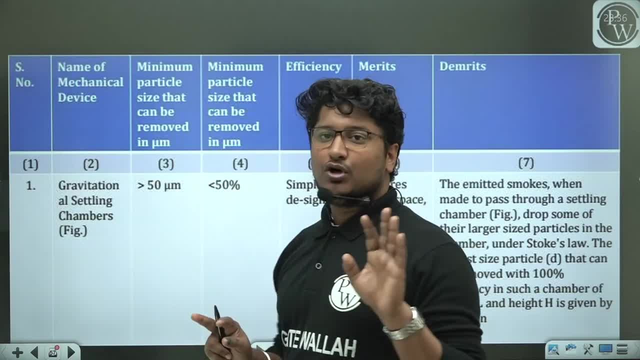 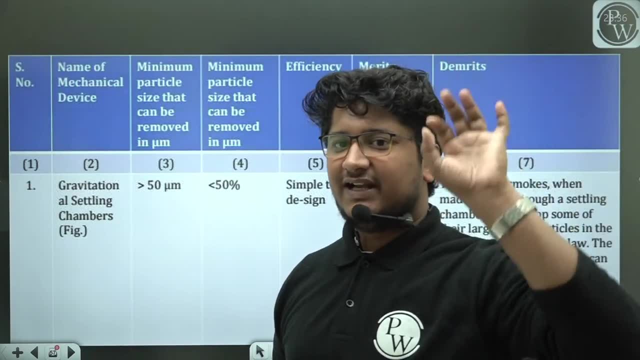 now the things that I am making you note, which I will underline. keep that in your mind, okay, once all of you stand up quickly, all of you are aligned here, ok, next 10 to 20 minutes is going to be very important. 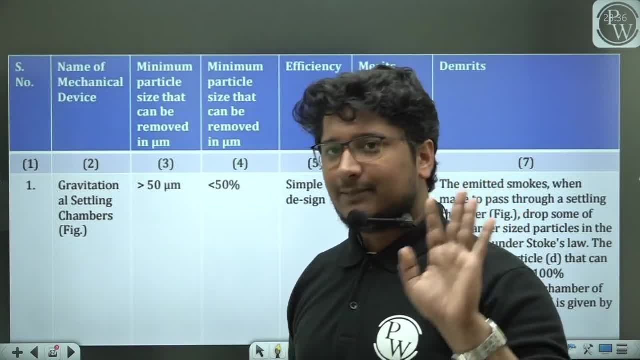 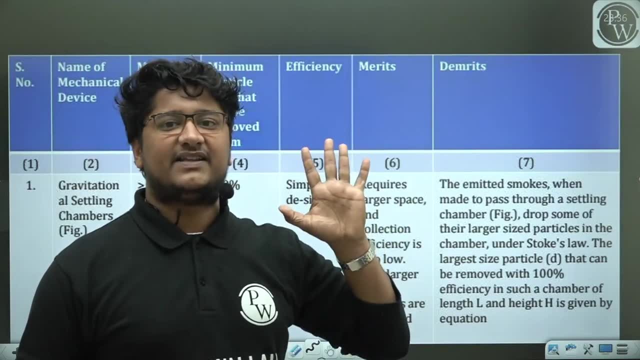 for you. so once all the children tell me quickly: all of you are aligned with me. next 10 to 20 minutes is going to be very important for you again, as you gave me support in plume behavior, by the way. 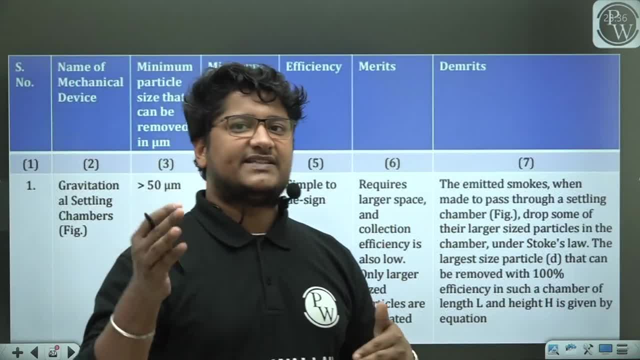 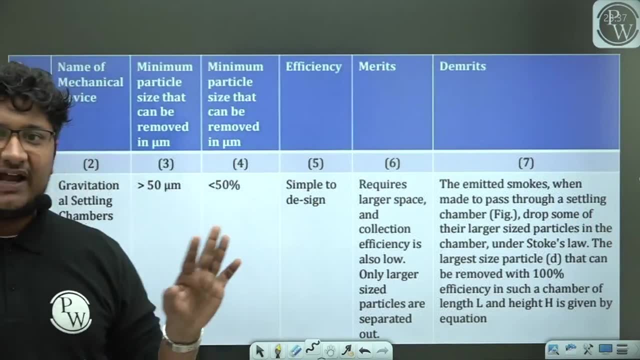 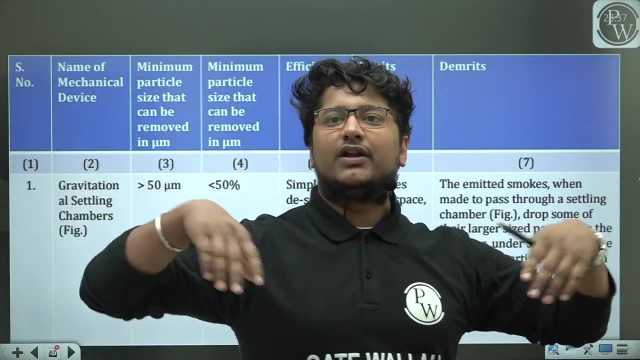 you have to give support again. once you give support, then you will understand things very easily. okay, now understand things easily. if you have said: yes, sir, we are all aligned. now we are awake, we are not sleeping. see, there are a lot of devices of yours for removal of air pollutants, our 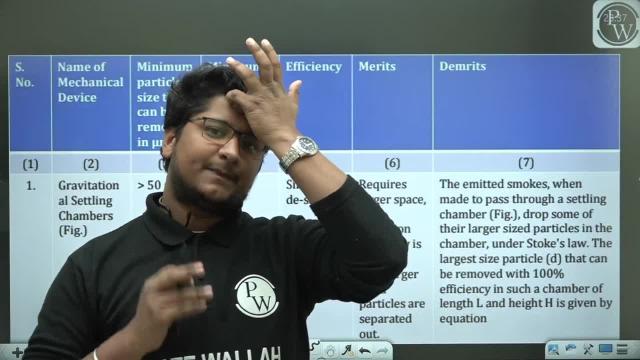 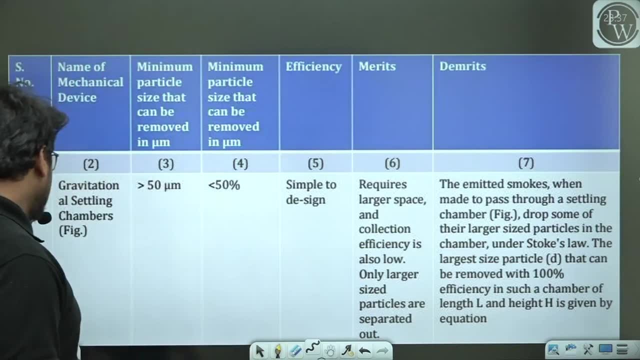 main goal will be the removal of particulate matter. so the first device of yours, we call it gravity settling chamber by name, this settling chamber, which you have read many times. so first we will see its figure, then we will talk about its story. oh, 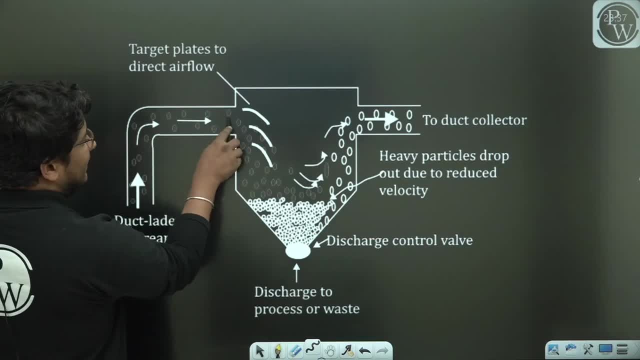 all figures what you are doing, sir, from here the�what you hear from you, you shiver if you come to the flu. what you have done, you have inserted the go in it. Now, here you have set up a second structure. 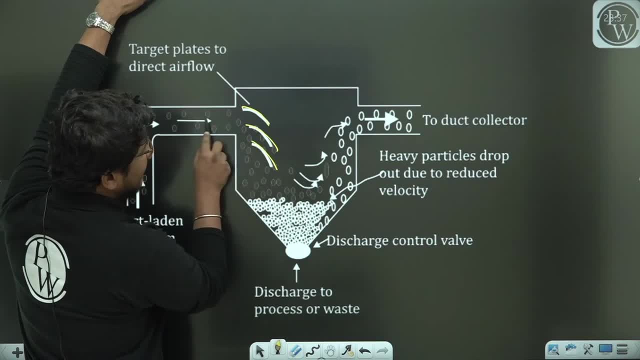 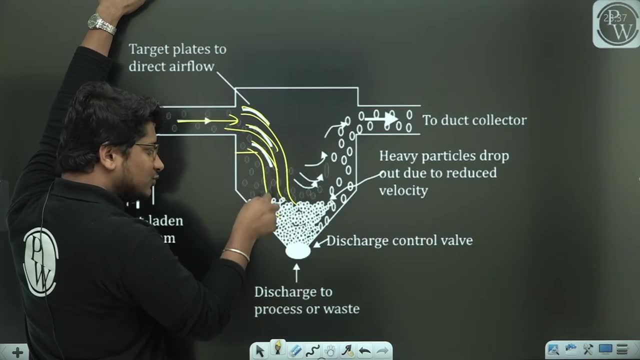 of some kind. this is the structure of your. that is why, whoever you have from here, If the bed hand hits to the bottom, it goes, Pulls and run down. Once the gas that has run down, you. the gas is hot, it is of a high temperature so it needs to get out. If there is atop, you will want to get up if there is. 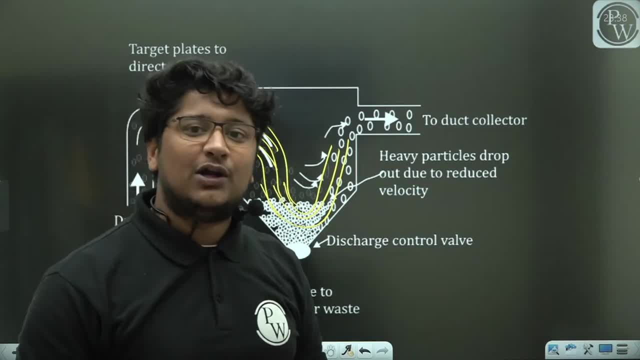 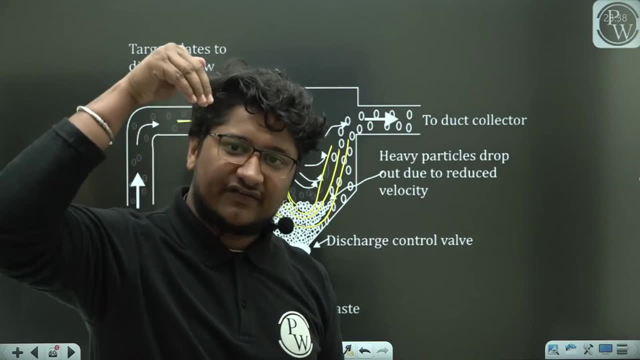 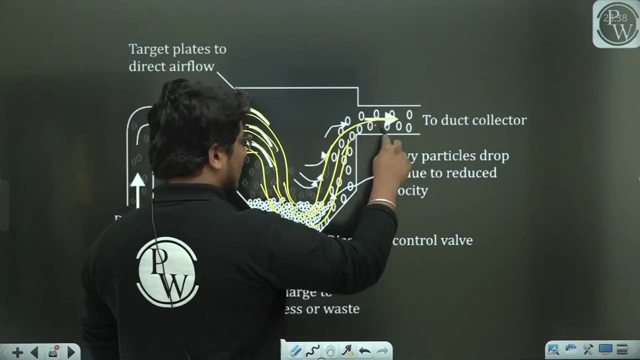 But the problem is that the particles in the gases will not be able to rise again Once they fall. they will settle down because of gravity. All the particles will not be able to go with the gas. So now your gas has come out of here and some particles will remain here. 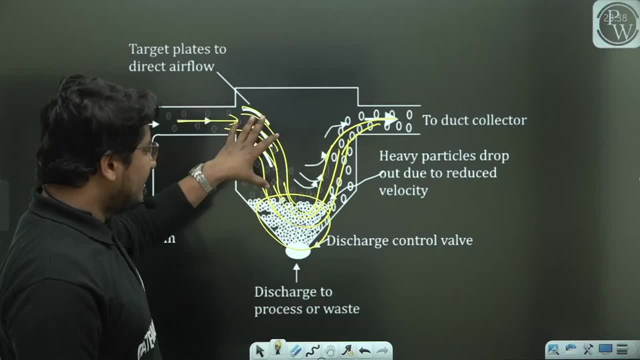 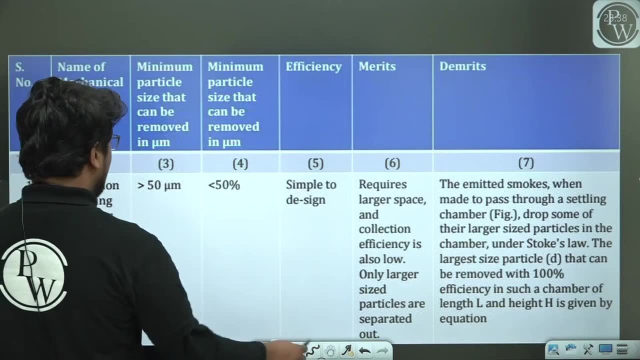 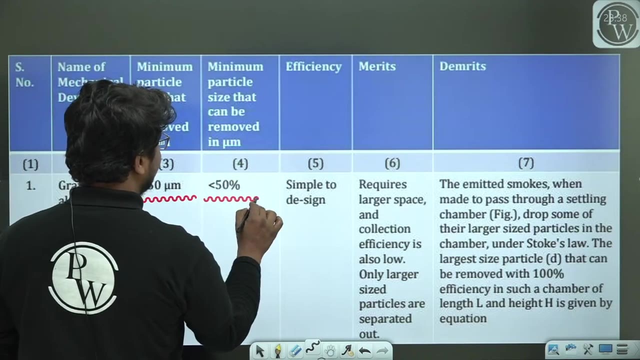 So this type of removal is called gravity settling chamber removal And the removal that you will see. this removal will be greater than 50 micrometer And its removal efficiency is also very low- less than 50%. Its removal efficiency is also less than 50%. 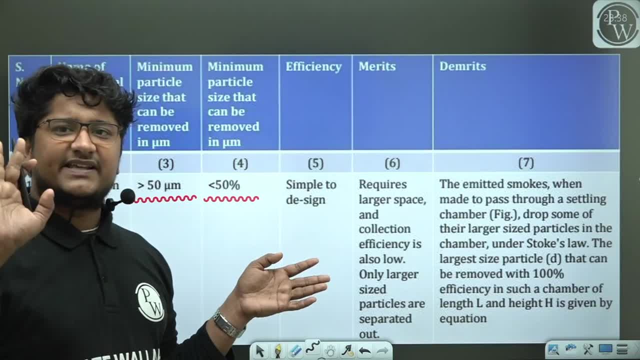 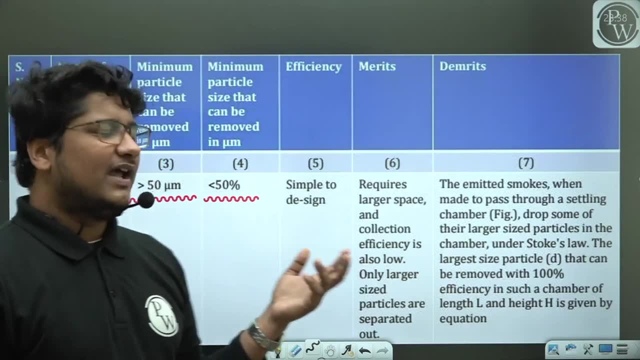 It also needs a big space. It is like a sedimentation tank. The concept is like a sedimentation tank, So it also needs a big space. This is simple to design and all, But what problem do we have to remember It is greater than 50 micrometer. 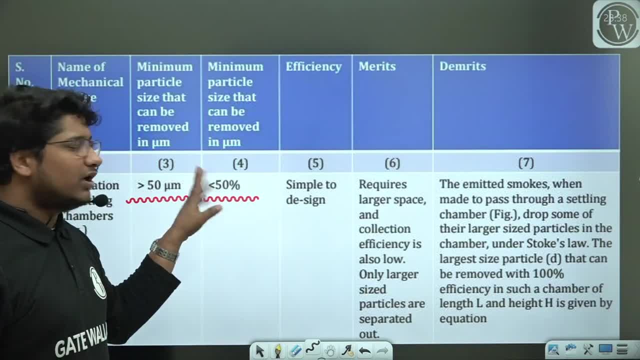 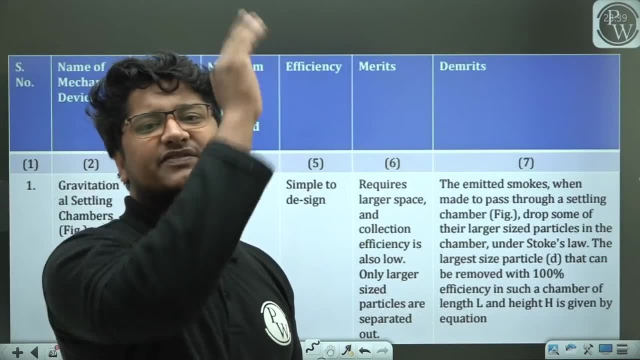 And this small size will only be able to be removed by small particles, And its efficiency is very low too, Because small particles are again removed with your air. Small particles are removed with air, So there are only large particles which you will be able to settle down. 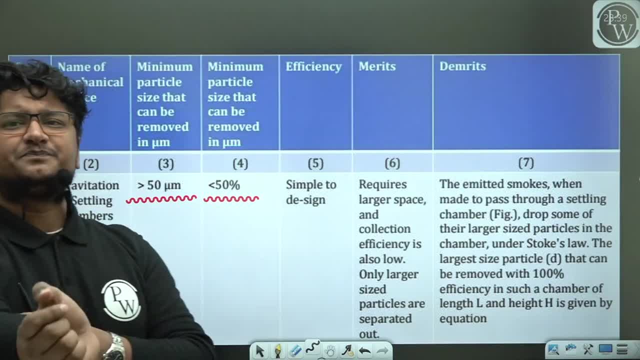 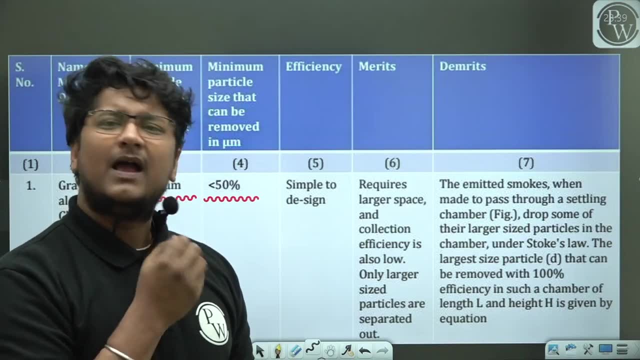 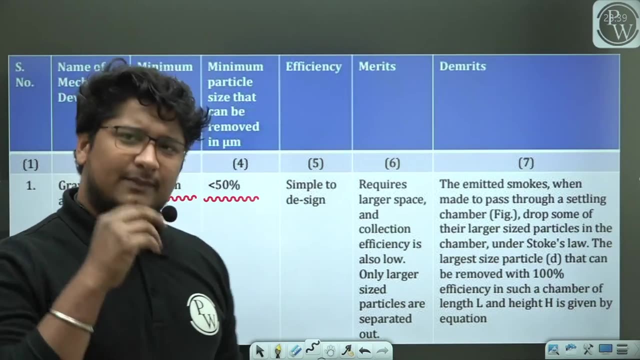 You will often see gravity settling chambers being used. It is of tane wheat. Have you seen? wheat Fans are reliably driven from the front. Ghee hoon mein hota hai, ya dhaan mein hota hai. Abhi bhool gaya, yaar kheti. 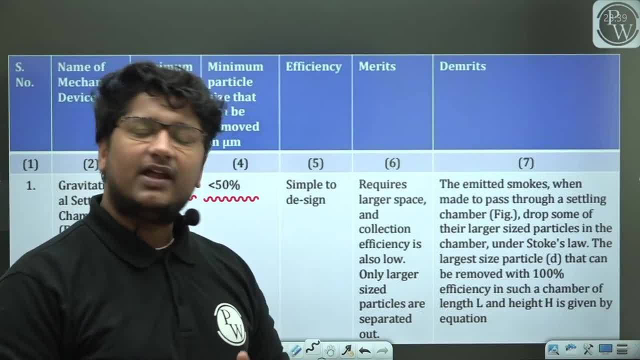 Pahele, bahut pahele mein kheto mein jaata tha. Abhi toh bahut din ho gaye, Isme saamne se fan chala dete hain. Aachkal machine bhi aage fan chalta hai. 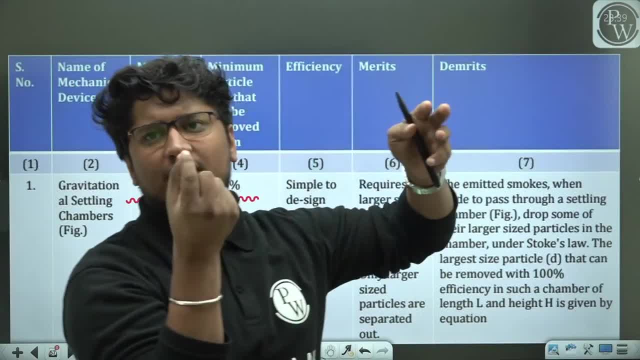 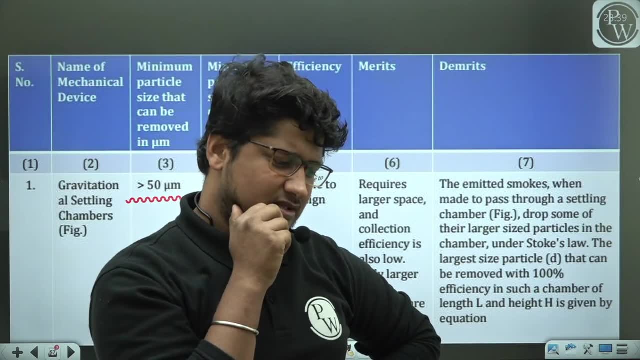 Toh jo ganda wala part hai, wo odh ke aage nikal jata hai, Aur jo, I think, dhaan mein hi hota hai, Dhaan mein hota hai, ki ghee hoon mein hota hai. 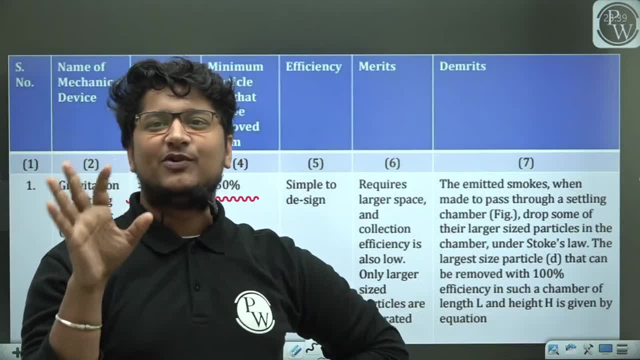 Re, yaar, main bhool gaya, Dhaan mein hota hai, ki ghee hoon mein hota hai. mujhe bhool gaya, That means rice mein hota hai or wheat mein hota hai, Jo log dhaan aur ghehu nahi jaante hoon log ke liye. 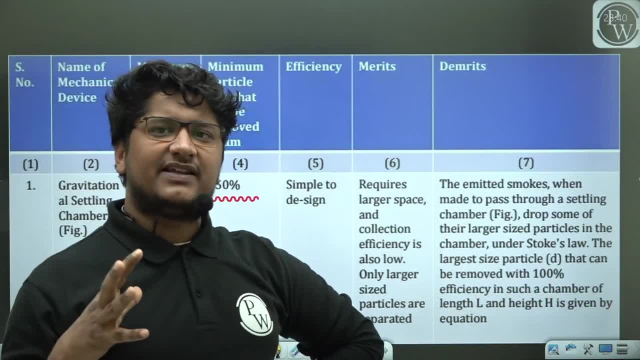 Toh wheat aur isme. I think isme saamne se fan chalate hain. na Haan sir, dhaan mein hi hota hai, dhaan mein hi hota hai, Wheat mein hi hota hai, dhaan mein hi hota hai. 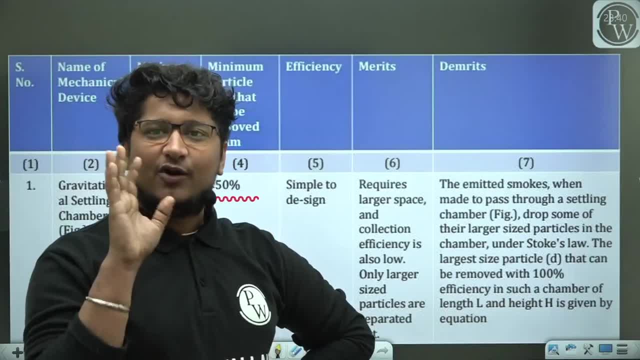 Dono mein hota hai: Arre, waa, Theek hai dhaan ghehu chhodo Usme hota hai, saamne se kya kiye Fan chalaaye Toh jo aapka halka wala part, jo uska cover rata hai. 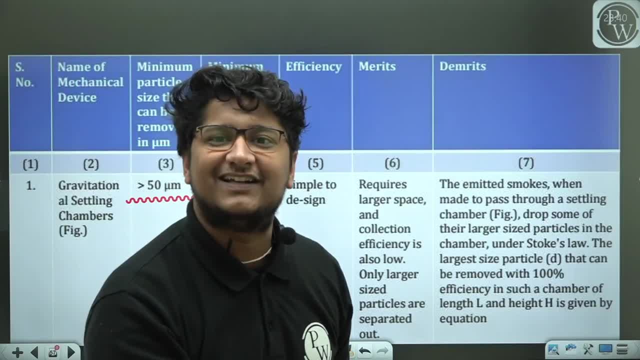 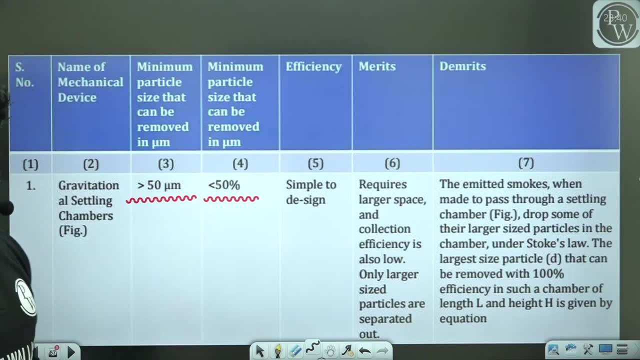 wo odh ke aage chala jata hai Aur jo heavy part hai, wo wahi niche gir jata hai. That is nothing but the gravity settling. Toh aapka first setup samajh gaye, Kya baate aapko yaad rakhna hai. wo bhi samajh gaye. 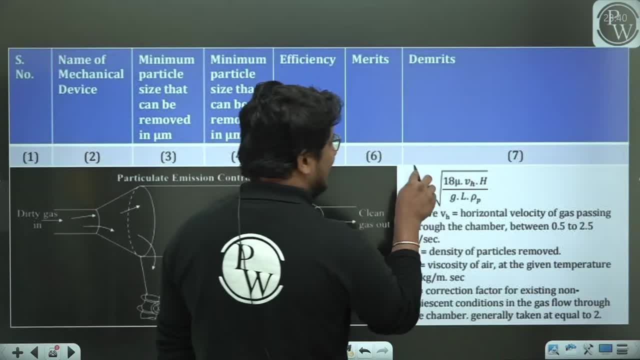 Ek cheez aur mein aapko thoda ekstra yaad rakhwa raha hu. Wo hai aapka diameter of particle? ye wala formula: So D equal to C root under 18 mu THH upon GL rupee. 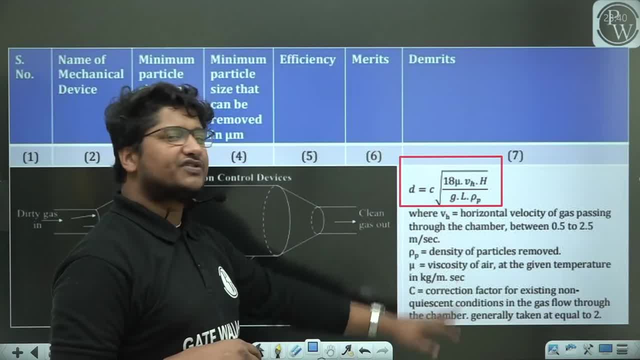 Aap log bata sakte ho ye formula kis tarike se lag raha hai. Thoda similar formula hai stokes ki tarah Toko ki usi same concept pe aa raha hai ye formula. 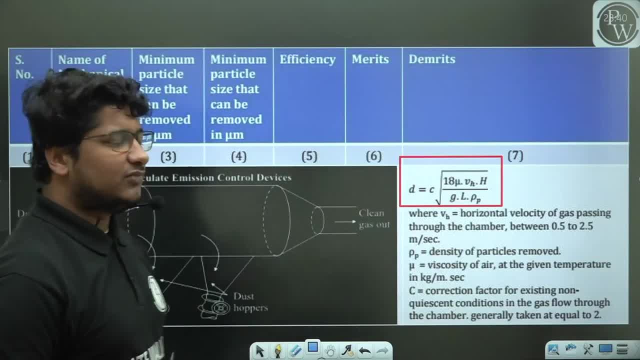 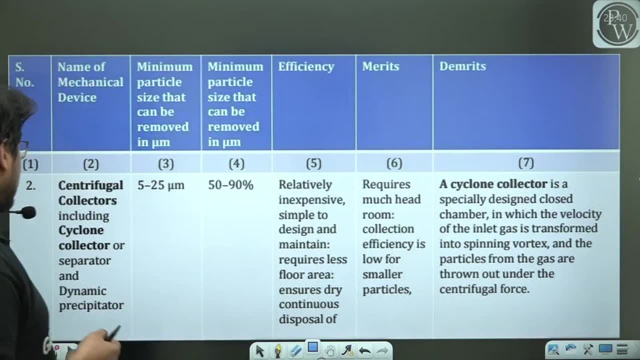 Toh, ek baar isko aap dekh lena, Waisa questions aane ke chances bilkul almost zero hi hai. Doosra hai aapka centrifugal collection. Ab isko dekho aap jo hai cyclone separator jo hai aapko. 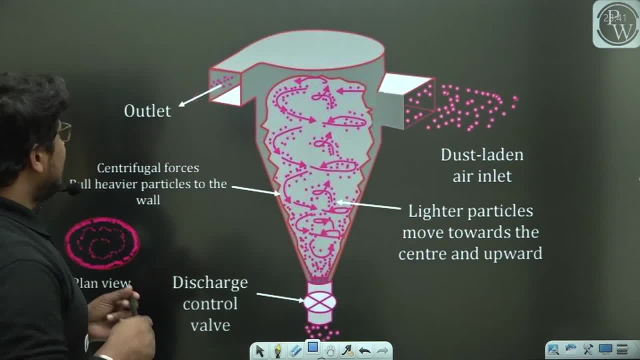 Isko, ek baar figure me pehle aap dekho, phir main aapko baat karunga. Figure me, kya dekho, aapne ek side se inlet diya. Ab aap inlet tangentially de rahe ho. 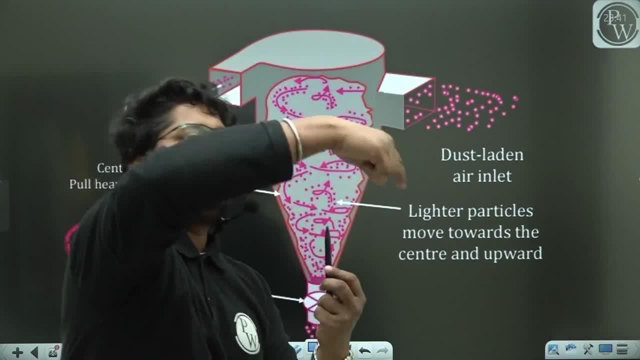 Inlet aap tangentially de rahe ho, Kisi bhi cheech me, agar aap tangentially inlet dete ho, na toh automatically rotate karne lagta hai. Ab, jab rotate kar raha hai, centrifugation ho rahi hai. 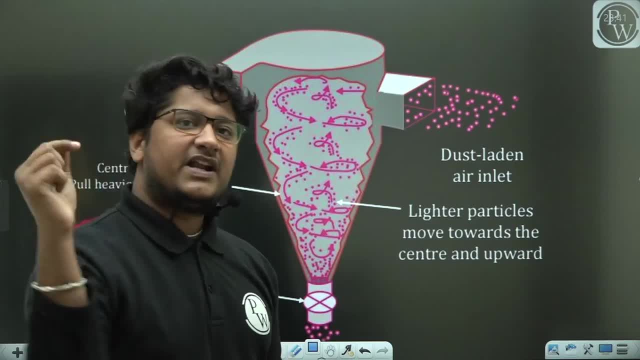 toh usme jo particles rahenge, wo bhi rotate karenge. Ab heavier particle. agar aap rotate karega, toh wo bahar ki tarah bhaagega, Kuki usme ek force lag raha hoga. 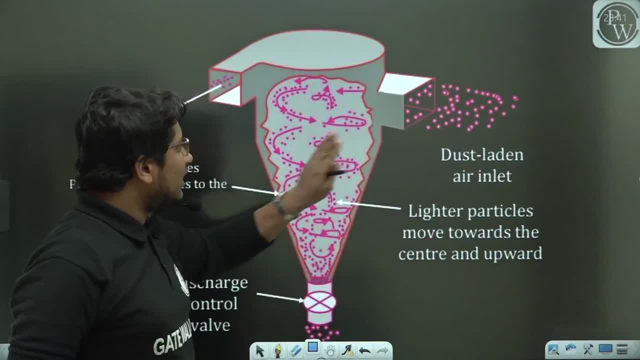 centrifugal force Bahar ki tarah bhaagega. Ab bahar toh aapne isko poora kya rakha hai. pack rakha hai, Toh takra ke kya hoga, wo niche ki tarah gir jayega. 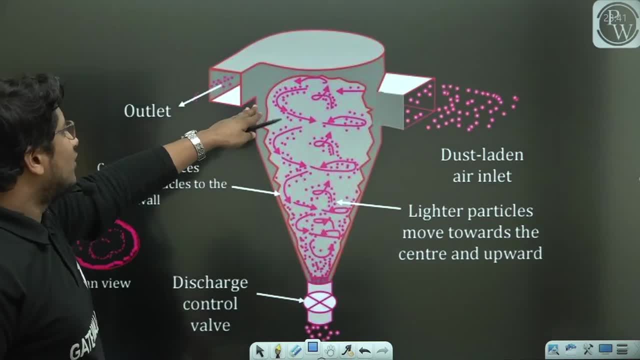 Aur niche ki tarah gira, toh usko aap collect kar lo bahar Aur jo aapka outlet gas hai, wo aapka bilkul, jo particles usme kam, jo hai particles, wo mostly particles aapke niche settle ho gaye. 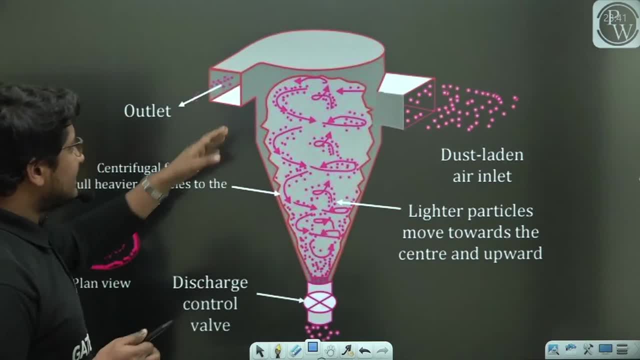 Toh jo niklega usme. kya rahega particles? toh aapko kam hi rahenge. Iss type ke separation, ko aap log bolte ho centrifugal, yaa aapko cyclonic separator bolte ho. 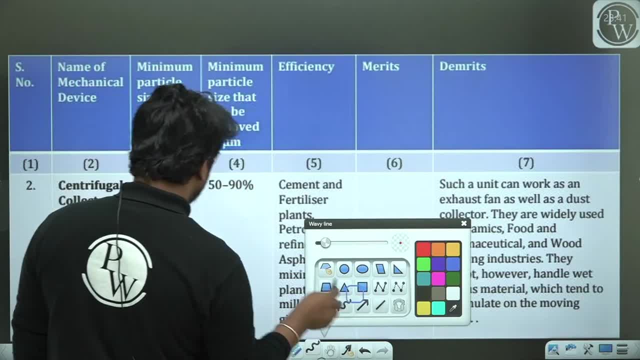 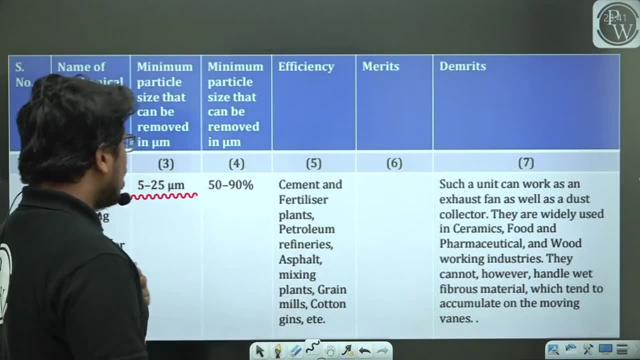 Aur iss ki jo baate aapko yaad rakhni ho. kya yaad rakhni hai? ki sir iss ka particle size, jo remove karega ho 5 to 25, matlab ek gravity settling se thora behtar hai. 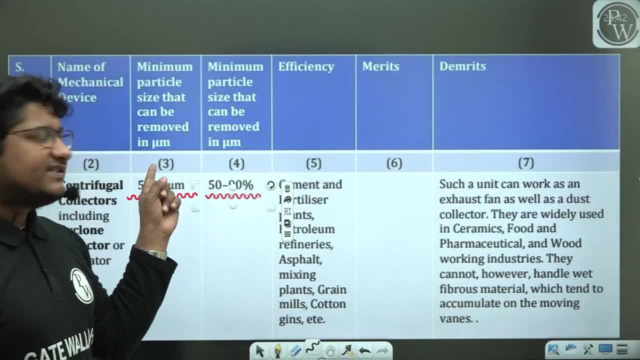 aur iss ki efficiency bhi acchi hai. 50 to 90% hai Iss ki efficiency ki itni range isli di gayi hai, kuki agar chote particles hote hai. na, bahut chote particles hote hai. 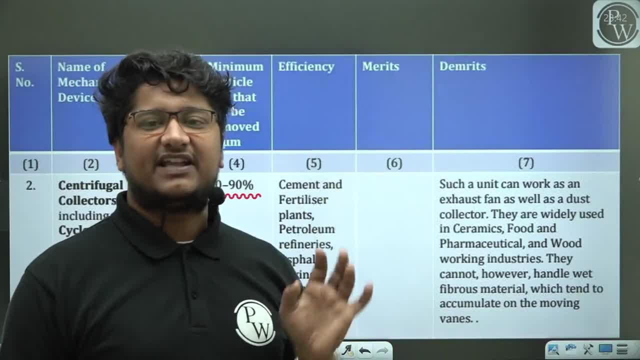 toh iss ki efficiency bhi acchi nahi aati hai. 50 k matlab, 60,, 70 k aspa chali aati hai. Agar thode bade particles ho, toh aapko, ye aapko. 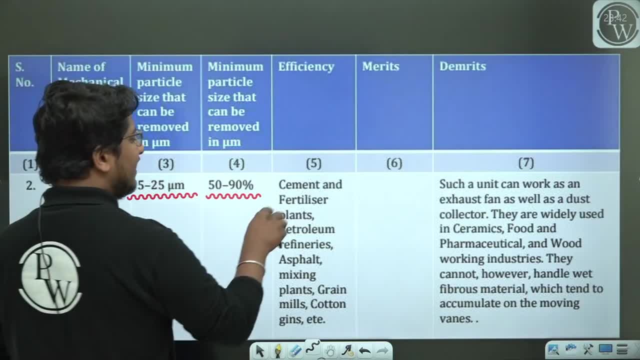 accha efficiency aapko deta hai. So generally aap dekhoge isko cement me yaa fertilizer plant me yaa petroleum refineries me yaha pe aapko use hote dekhoge Cranes mill jo hai aapko. 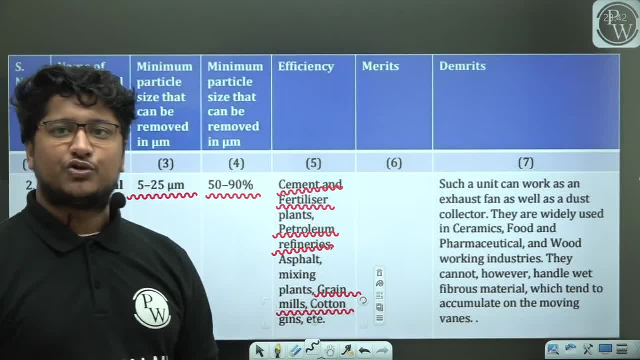 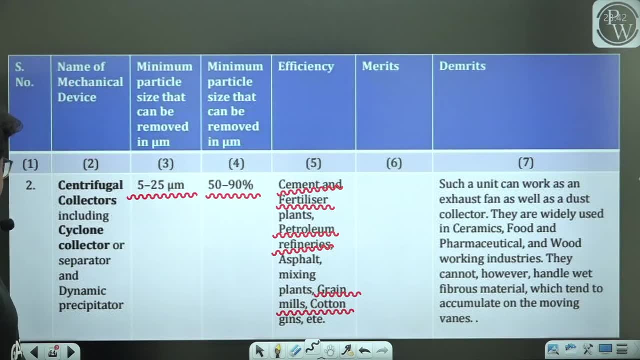 waha bhi aapko use hote dekhega. So generally in sari joga pe aapko use hote hue dikhta hai. It is 5 to 25 micrometer, aur iss ki percentage jo hai aapki 50 to 90%. 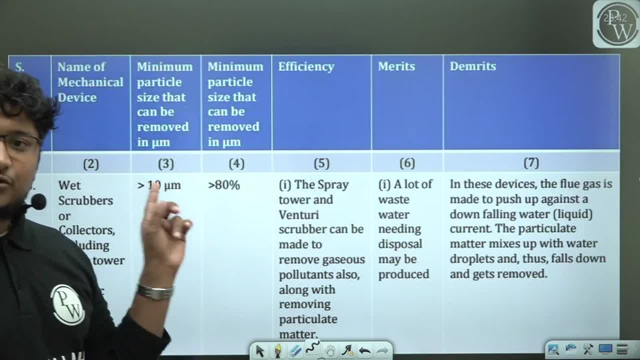 Sab ka aapko mechanism yaad rakhna hai, aur sab ka aapko. sab ka aapko mechanism yaad rakhna hai, sab ka aapko. jo data mein aapko underline kar raha ho. 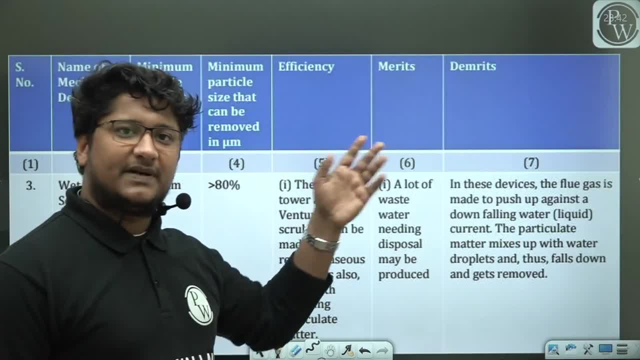 wo yaad rakhna hai. Baaki theory. agar aapko extra padhne ka mann hai, toh aap padh sakte hain for different exam kit. mein ho theory nahi puchhne bade. Next baat kar raha ho mai aap se. 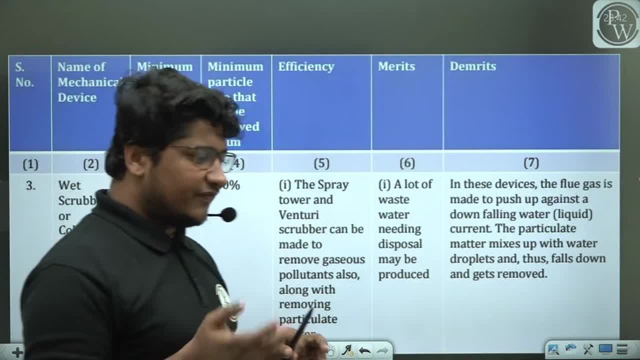 ki aap aapke paas 3 separator hai. Ek saath mai aapko 3 ho samjhaunga, fir 3 ho ka mai aapko alag lag kahaani bataunga. Ek hai aapka wet scrubber. 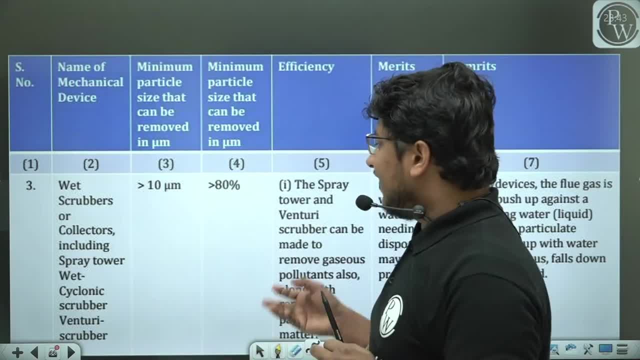 tike dusra hai aapka spray tower aur tisra hai aapka cyclonic scrubber. Matlab ek aap bol chakte ho. normal spray tower hai aapka dusra hai aapka cyclonic wala. 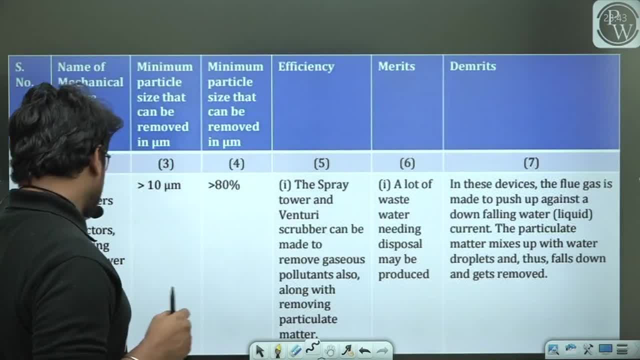 aur tisra hai aapka venturi scrubber. 3 ho ke baare mai aapko baat karunga. aur ye 3 ho aapke wet wale hai Wet matla paani dal rahe ho aapko. 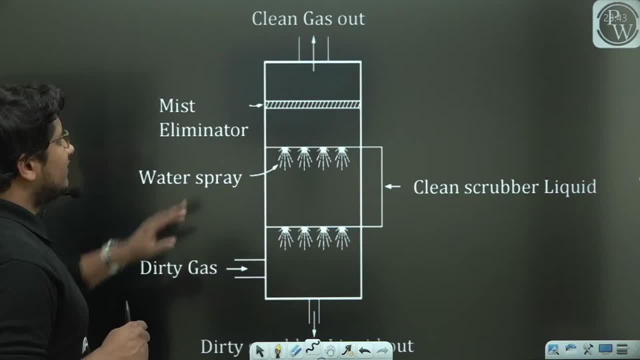 Okay me, ek ek aapko samjhata ho. Pehle pehle lete hain spray tower, Pehle spray tower ko samjhete hai, simple wala hai. Dekho kya hai spray tower mein. 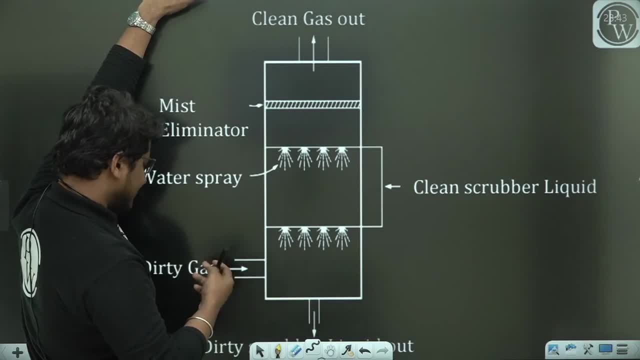 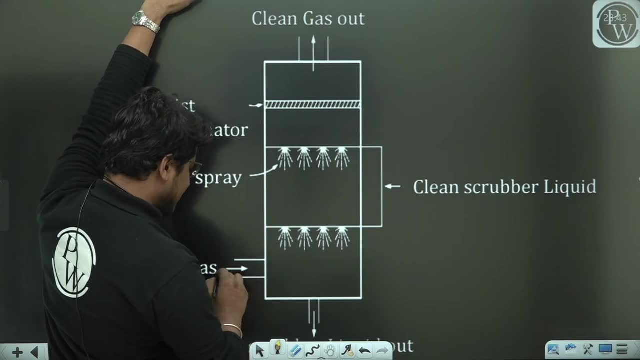 Sir, aapne inlet kahan se diya, Arre, inlet kahan gaya. dada, Inlet me haan se diya, chalo Ek mat. Ye aapka inlet hua theek hai, Yeb aap gas ko inlet doge. 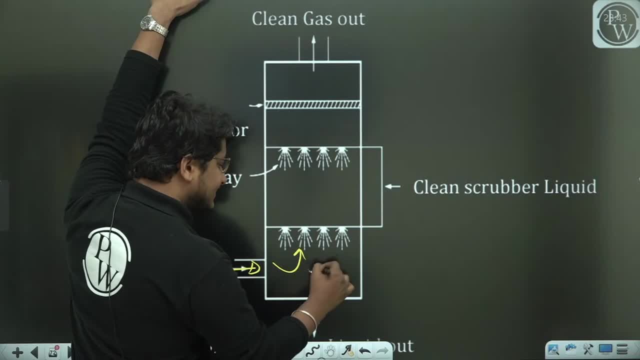 to gas. kya hai, Garam hai Woh. aapko upar ki tarah bhaagega Gas. aapko upar ki tarah bhaagega Gas. aapko upar ki tarah bhaagega. 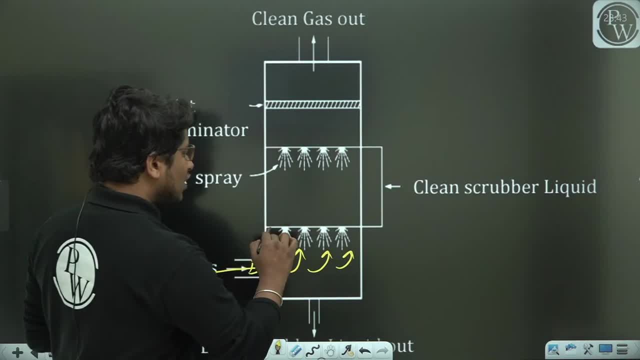 Aapne kya lagake rakha, Yehap pe spray Spray tray lagake rakha hai. Toh yehase aapne water spray kiya, Yehase aapne water spray kiya, Yeh aapne water spray kiya. 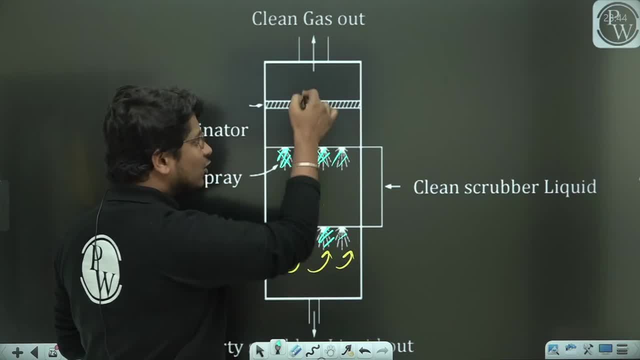 Yeh aapne water spray kiya, Kuch iss tarike se Yeh gases hai, yeh upar jaana chaah rahe hain Toh gases. jab upar jaayega, uspe agar aap water spray karoge? 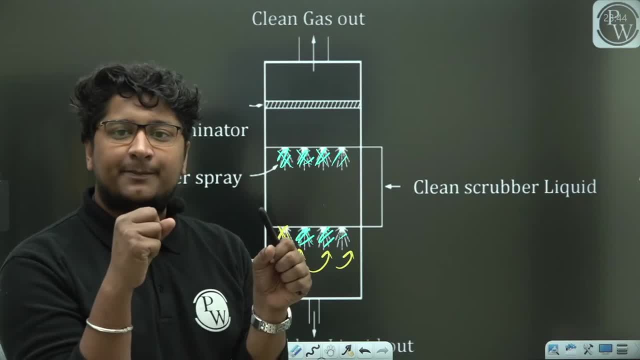 toh gas mein jo solid particles hunge, woh heavy ho jaayenge, Toh pehle saayad, woh aapko air ke saath flow kar rahe thee, lekin aap heaviness huni ki wajah se. 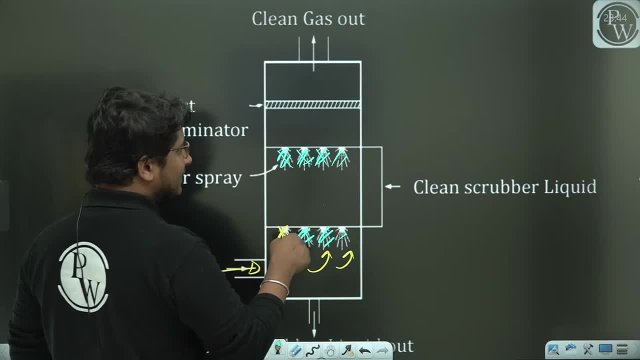 woh aapko niche settle kar jaayenge. Aap aise mein kya hoga? ki jo aapka air jaayega usme aapko thora mora mist, toh aahi jaayega. halka halka aapko water droplet, toh aahi jaayega. 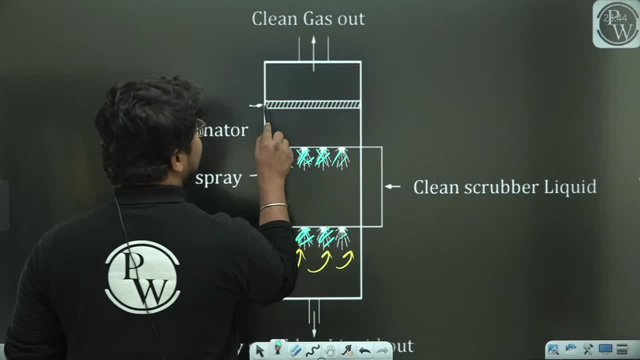 Toh, if you want to remove that mist also, toh yehap pe aap mist eliminator lagake rakhe ho. Toh aapka jo gas bahar ki tarah jaayega that is completely free from the particles. 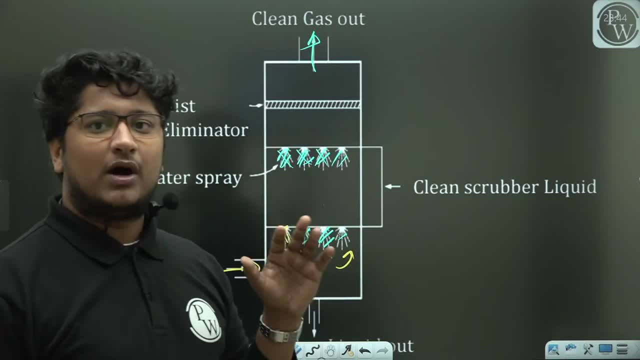 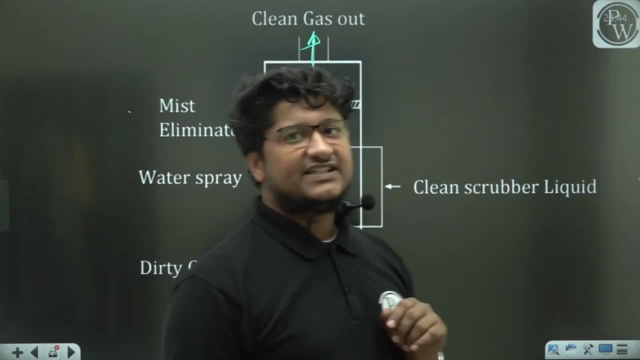 as well as jo mist aapko bana tha, usko bhi aapko hata dega. Toh yehapka clean gas outlet ho gaya Kaar samajh mein aayi. Is that clear to all of you? 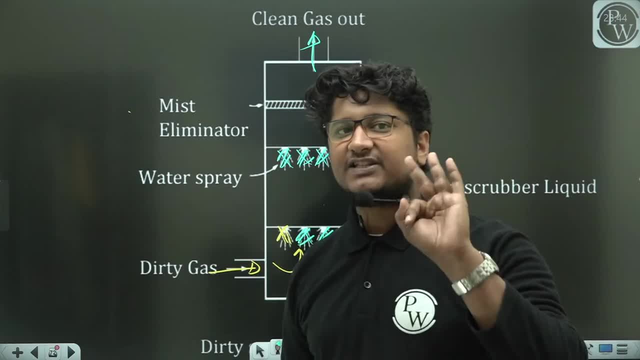 Spray tower. sab logon ko samajh mein aaya Main pehle aapko teeno ka principle samjhaunga Teno wet wala hai. teeno ka mechanism samjha diya maine aapko. 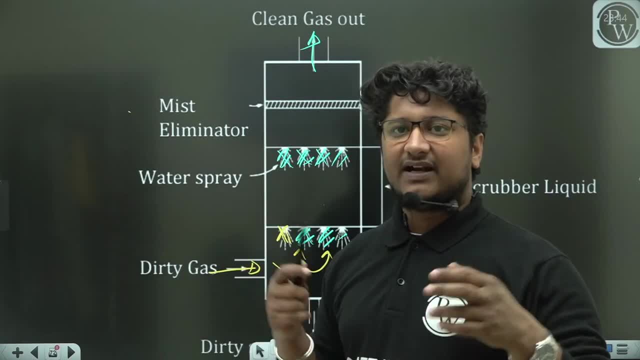 aur fir mein aapko uske kya baate yaad rakhni hai, aapko kya baate ratna hai, woh main aapko baad mein bataun. Pehle aap ek baar mujhe bata diyega ki. 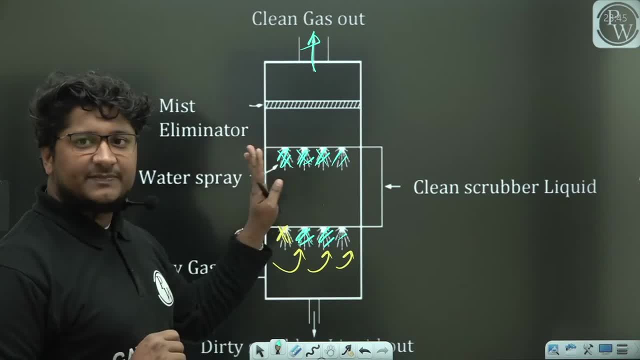 working principle samajh mein aagaya, Spray tower ka working principle sabko samajh mein aagaya, kis side se aapka air aa raha hai, beech mein kya ho rahi hai aur kaise woh nikal raha hai. 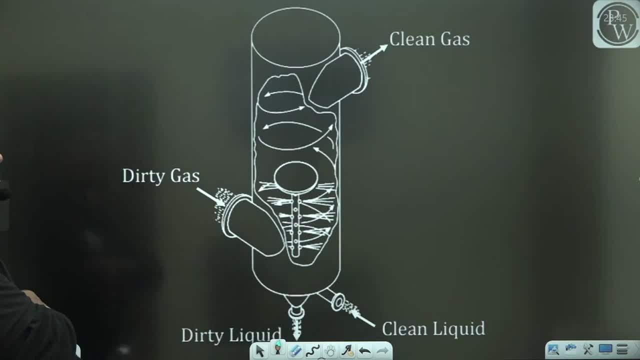 Aap dusra hai, aapka cyclonic, aapko yeh hai, toh wet scrubber hi, lekin aap yeh cyclonic action aapki ho rahi hai. Dekho kaise, Jab bhi aapko cyclonic action karwani hai na. 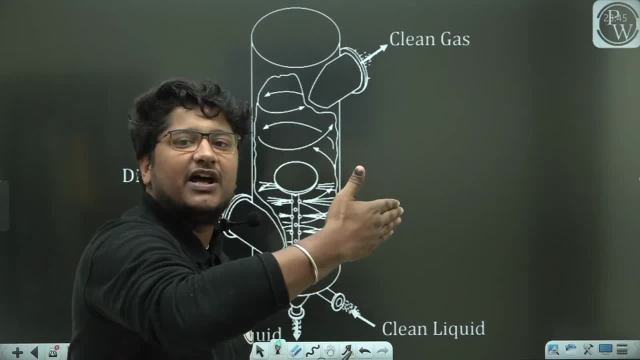 jab bhi aapko isko rotate karwana hai, aap humesa tangential daalo To tangential daane. se kya hota hai ki woh ek baar khud hi se rotate kar gaya, aur ek baar agar woh rotate kar gaya. 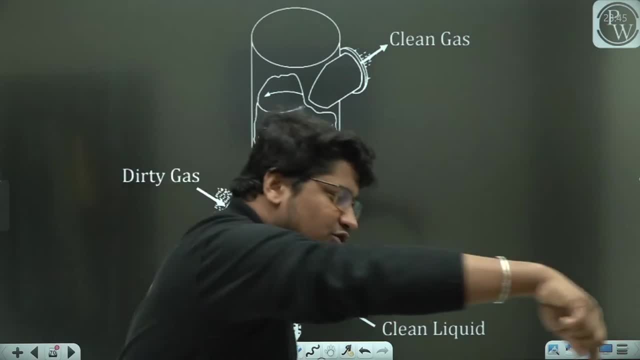 aur upar toh jaana chahta hai, yeh ko ki warm air parcel hai. upar toh jaye gaya hi ek baar rotate kar gaya, toh woh upar aapko aise, aise rotate karta hua. 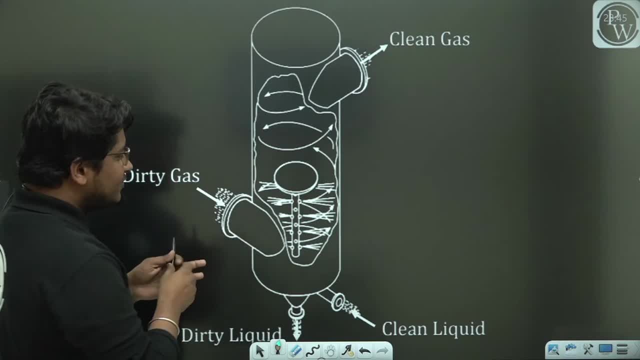 upar ki tarah badhe ga, Aap, jab yeh aapko niche rotate kar raha tha, beech mein humne kya daal ke rakha hai, aapna water, aapka sprayer daal ke rakha hai. 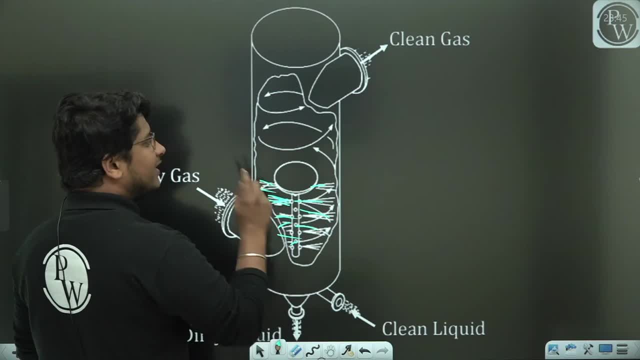 Yeh dekho aapka water spray kar raha hai. yeh dekho aapko water spray kar raha hai, Jab yeh rotate kar raha tha, tab aap kya kiye beech mein, se aapne pipe daal ke rakhi hai. 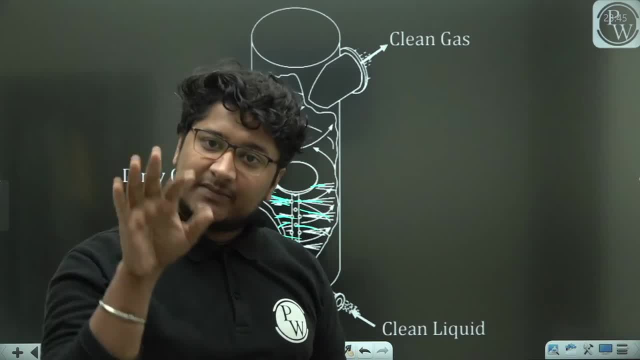 jo aapko water spray kar raha hai, Aap water spray karega, toh same kahaani hogi. kya kahaani hogi, sir? solid particle aapka heavy hoga aur solid particle heavy hoga. 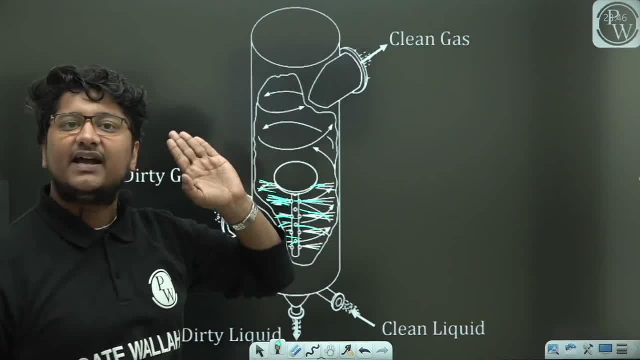 toh woh nichi ki tarah settle hoga upar se aapka clean gas, nikal jayega Baaki principle same hi hai, Lekin agar mein aap log se puchu ki comparison to spray tower: 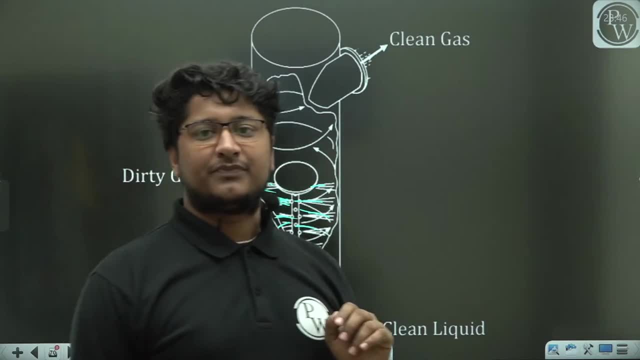 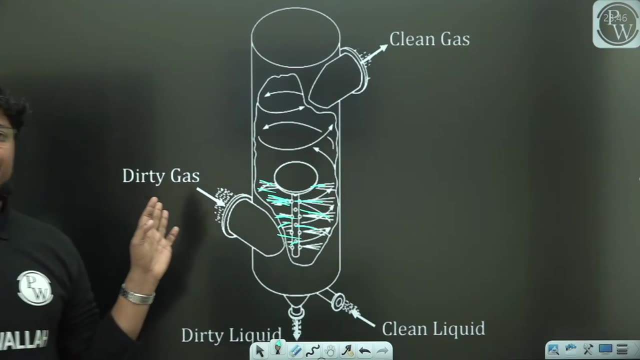 aur yeh jo aapka cyclonic action wala hai. which one will perform better? Which one will perform better? Comparison to spray tower, jo aapne pehla symbol wala dekha tha, aur yeh, jo aapka cyclonic separator wala hai. 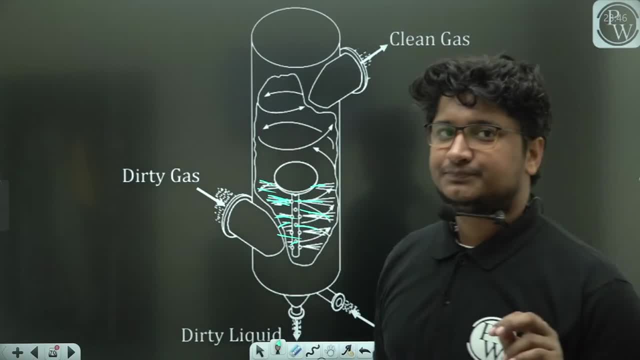 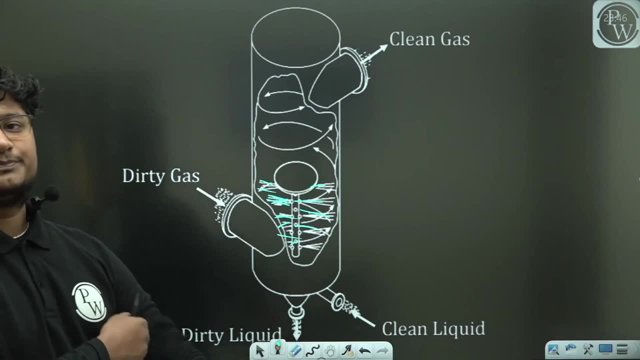 matlab cyclonic action wala hai kaunsa behtar perform karega. Kaunsa behtar perform karega. That means kis ki efficiency. achchi hogi Kota moti, yehi puchh raha hu. 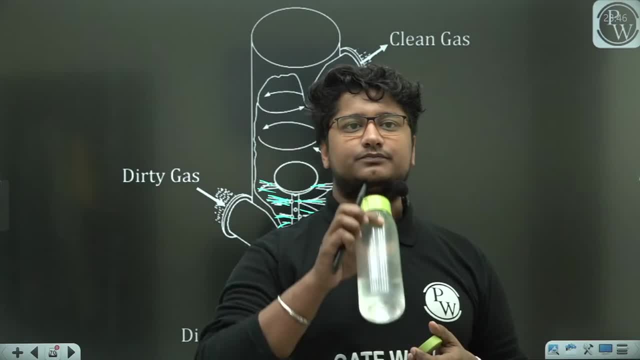 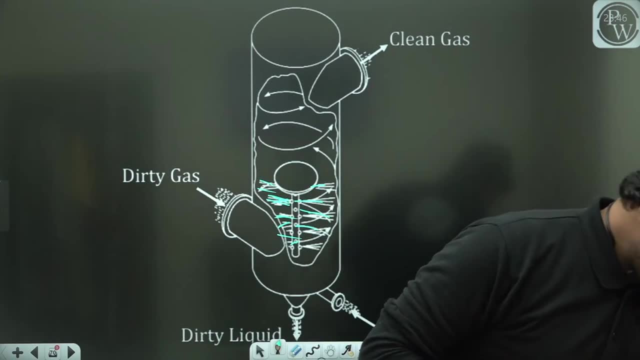 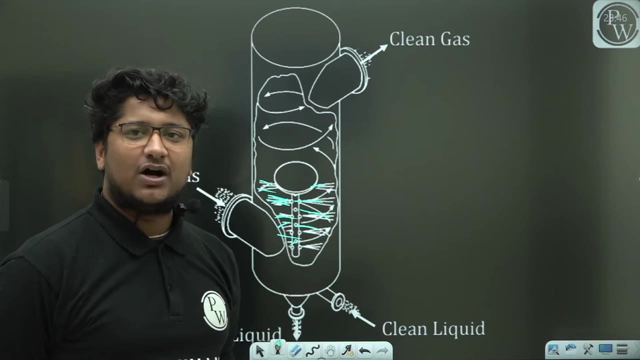 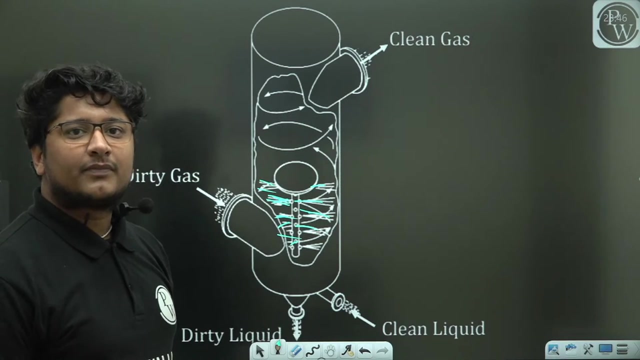 Kis ki efficiency achchi hogi. Spray wale ki Arey nalaik cyclonic action ka hoga na Cyclonic action se kuch particle aapko because of cyclonic action bhi remove hore hongi. 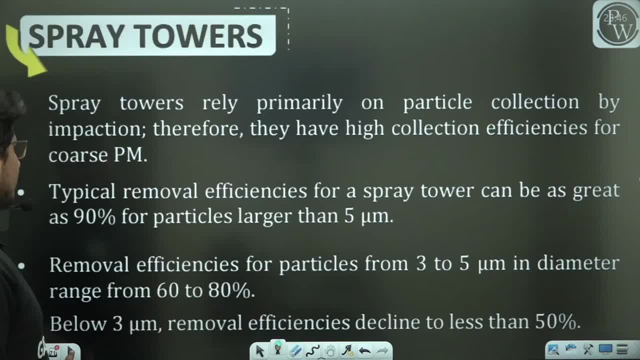 advantage milega na cyclonic wale me. advantage milega na cyclonic wale me. advantage milega na cyclonic wale me Karo. Teesra, jo aapka hai similar setup me, wohi aapka Venturi Scarab. 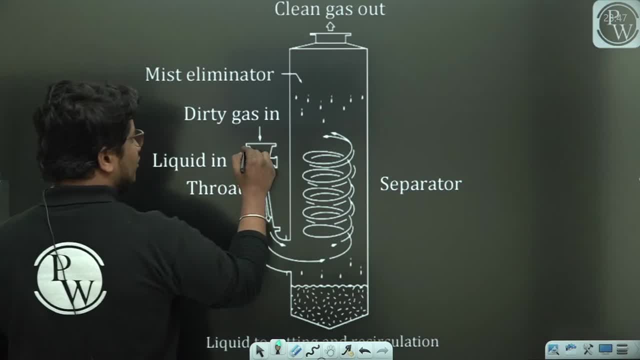 Ab yeh Venturi Scarab, dekho kya hai aap sab log na Venturi setup dekha tha kuch issi tarike, se aapko setup raha tha tha Venturi ka To aap kya kia dal. 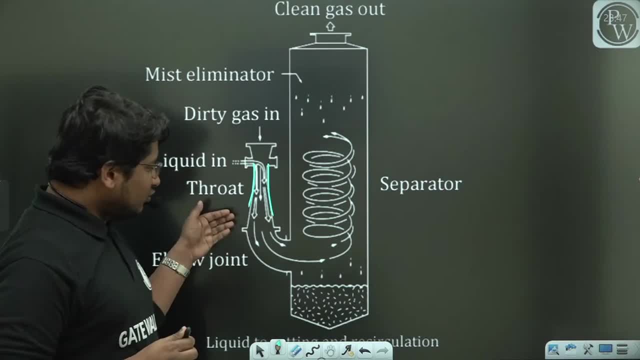 inlet to aap kya dere ho. tangentially hi dere ho inlet to aap, tangentially hi dere ho, lekin aap paani jo aap dal rahe the spray, jo kar rahe the ko aap yaha pe kar rahe the. 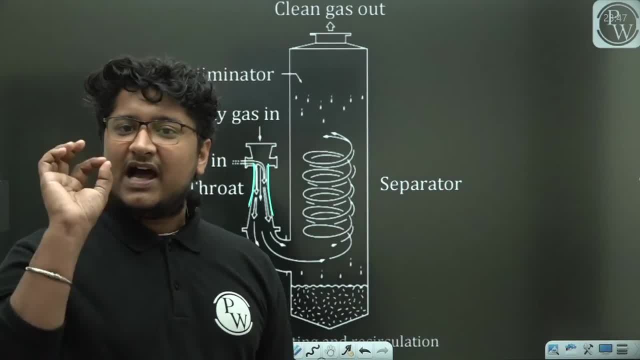 spray kar rahe the. kya hora tha ki saare particle dhang se bhing nahi rahe the har particle ko halka, halka paani aara tha. kuch particle aisa chhupke nikal jaa raha tha. 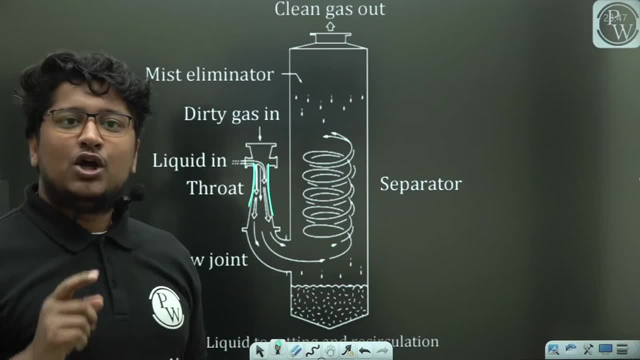 kar. bhaiya paani dhar se aara hai. mai idhar se nikal jaa to to chhupke, nikal jaa tha to waise particle phil. aapko remove nahi hongi waise mist elimination jo hai. 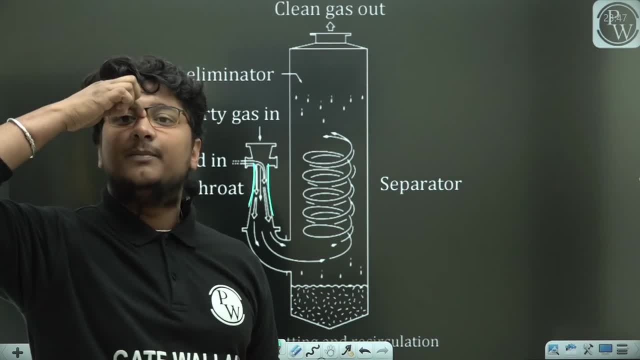 aapka mist efficiency wale part ko nahi relate karega na Vikash Bhushan mist eliminator usme hai, lekin mist jo hai. aapka particle removal efficiency me nahi mist to humne extra remove kar diya. 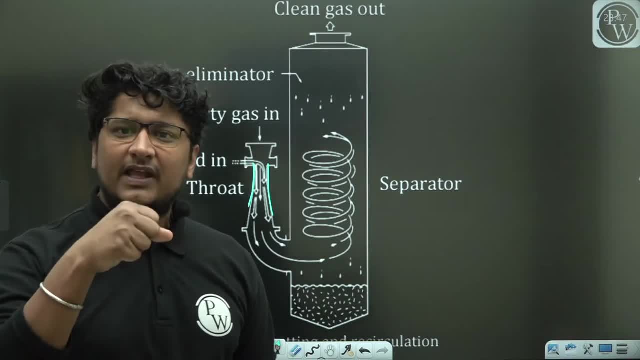 lekin particle removal nahi ho paaya. na part apni apni bullet ko servicing ki jaga. aap usme velvet ki cover laga doge to theek. hai. achchi baat hai, achchi dikhegi ho. 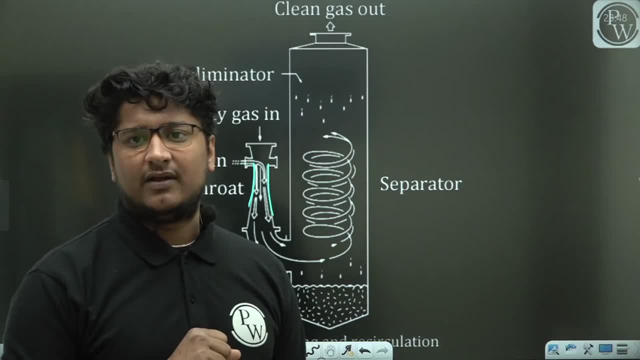 lekin chalegi tabhi na usme servicing. achchi karvaoge baat, samchh pahare to bhai. bhali baat hai, ki aapka particle removal efficiency mist eliminator se depend nahi karta na. 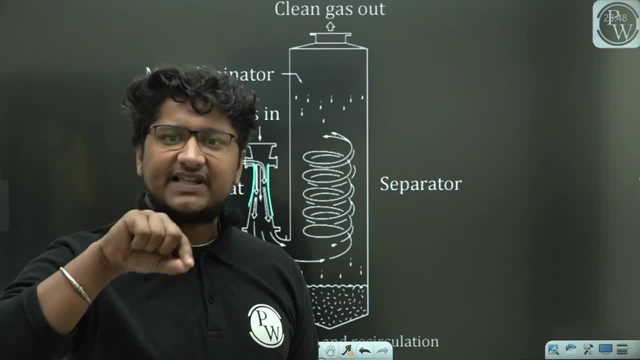 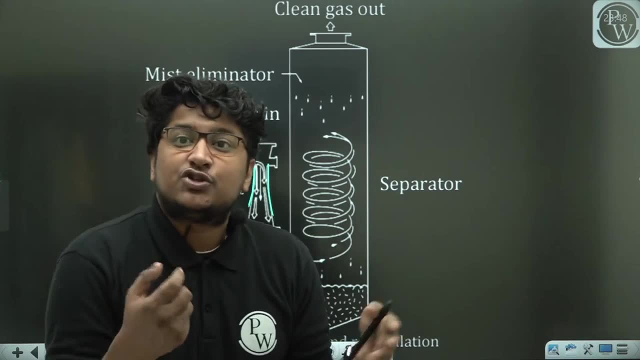 particle removal efficiency aapki mist eliminator me depend nahi karegi na theek hai aap. mai kya bola aapko ki ye kuch particle, the jo dhigi nahi rahe, the chhupke nikal jaate the. 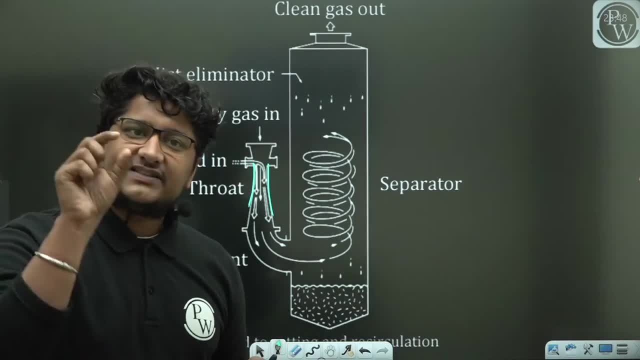 ki bhaiya, mere pe paani nahi aaya, mere pe paani nahi aaya to waise particle ko bhi bhingane ke liye, unko achche se geela karne ke liye, hum kya karte hai? 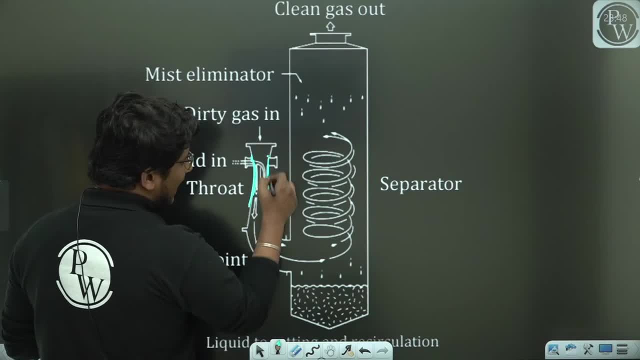 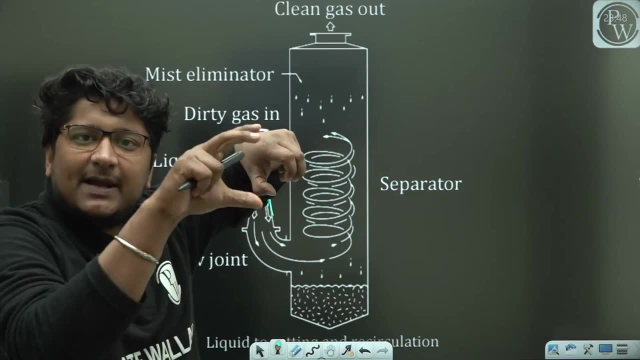 ki bhaiya inko yahan pe dalo. ab yahan pe aapko malum hai, ventrometer me beech ka area ek throat area hota hai, jahan chhota cross section hota hai. ab yahan se air aapko nikal raha hai. 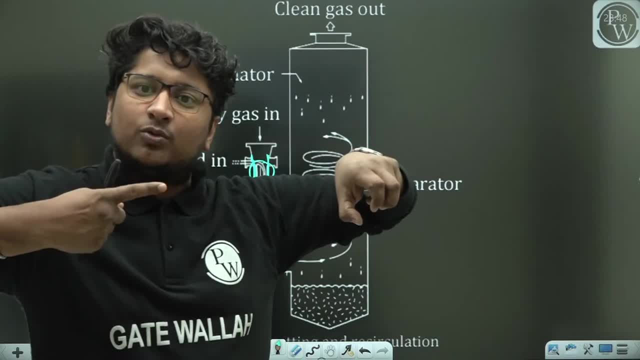 yahan, se aapka inlet air jaa raha hai, yahi pe paani ka spray maro, yahi pe paani ka spray maro. ab aisi jaga pe, agar aap paani ka spray maroge. 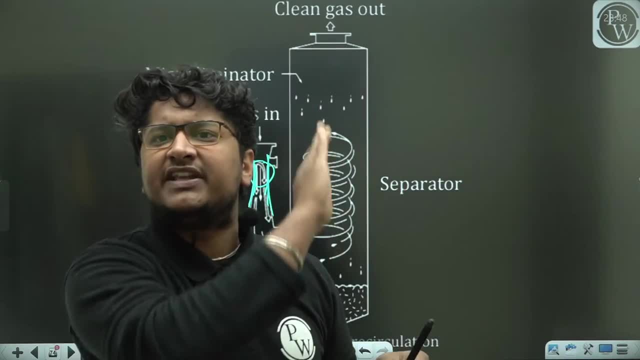 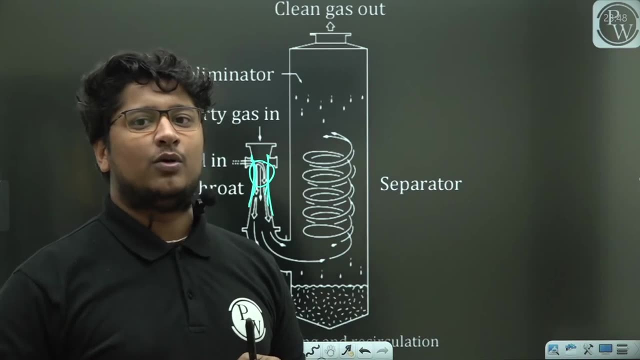 itna chhota cross section hai, to aap uniformly achche tarike se mar sakte ho, koi bachke nahi jayega ek to Zindasand samjho ki holi me, agar kisi chhote corner pe aap khade ho. 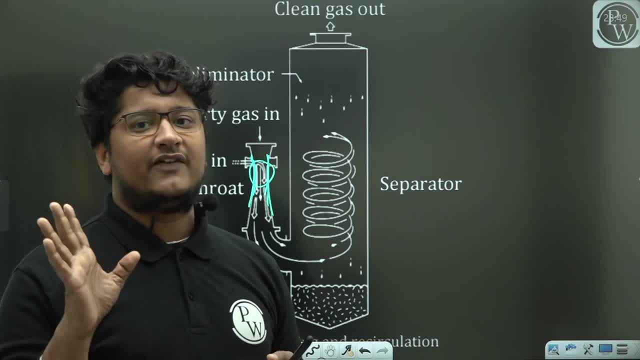 yahan se to sabko jana hi hai. to ek ekko rang. aap lagaoge ek bhi chhutne wala hai nahi, aur bade se 8 feet road me khade ho to koi ne koi chhuti jayega. 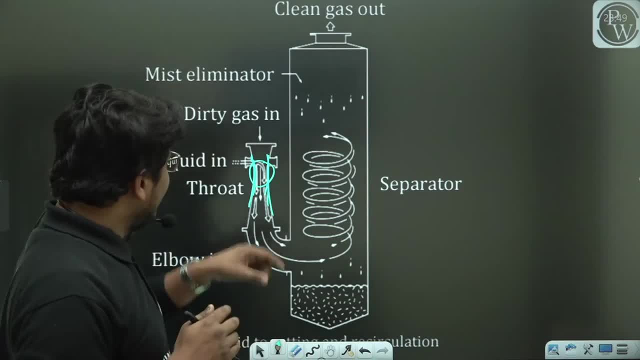 ek dam gali me khade raho, ek ekko rang lagake hi aage bhejna hai to wahi wali baat hai, ki yahan itne chhote area se aap usko gujar rahe ho. 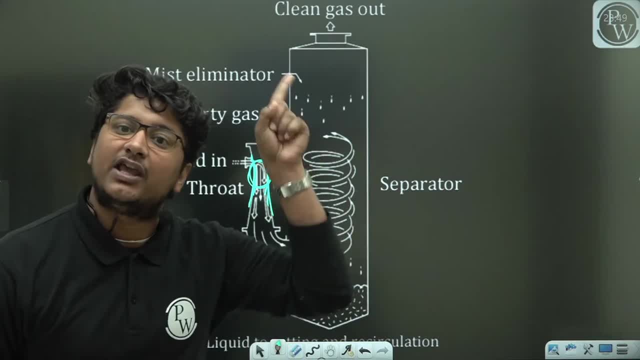 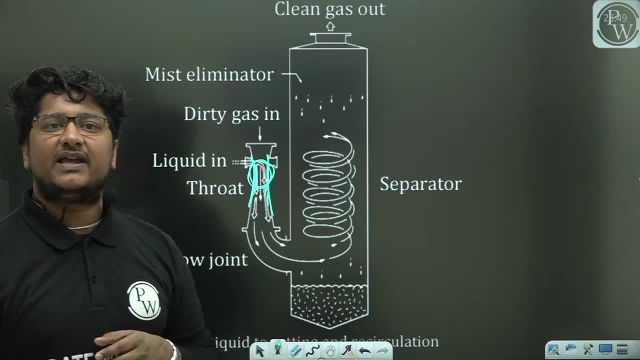 ki yahan, agar aap paani daloge to har ek particle geela hi hoga. option nahi unke paas bachke jaane ka to aise case me ab ye particle. yahan aega to aapko behtar removal efficiency milegi. 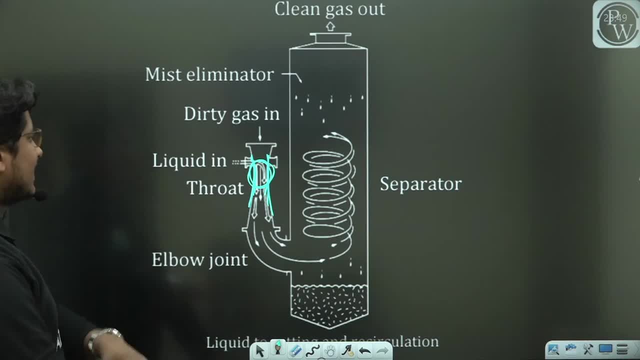 isme koi doubt nahi hai to Venturi Scarver, jo aapko jyada behtar kaam karega. isme koi doubt nahi, aap loko ab yahan bhi mist elementor lagaya hua hai. 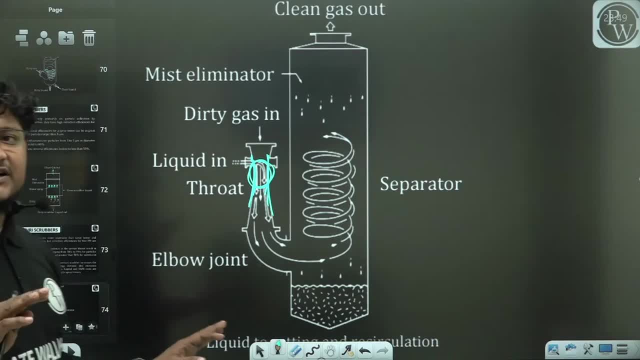 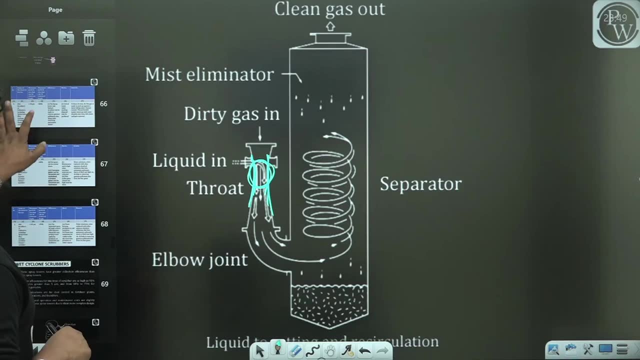 to isme koi problem nahi hai. mist elementor ka particle removal efficiency. se aapko koi khasa fark nahi padta ab ye chiche, maine aapko working principle bata di. ab teeno ka mai ek bar aapko ye bata deta hu. 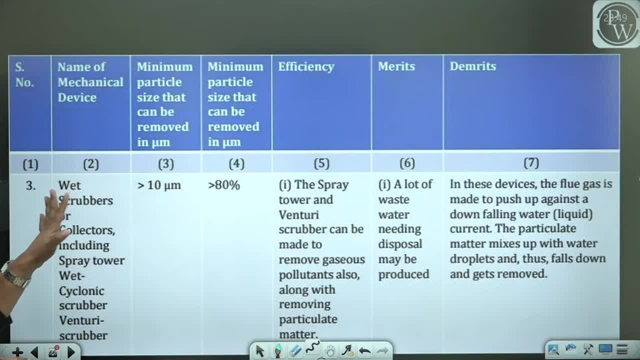 jo aapko dimaag me rakhna hai. sabse pehle me aapko baat kar raha hu, spray tower ki the basic one to uska. aap dekho ye 10 micrometer particle, se jyada rakhda hai bada. 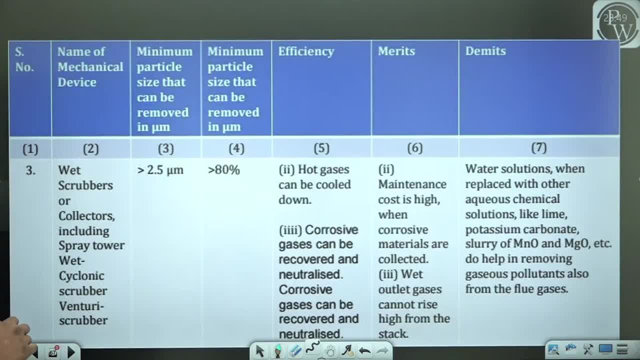 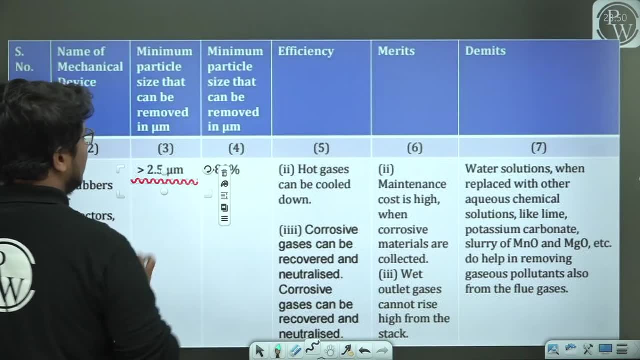 aur uski efficiency aapka 80% se thodi upar rahegi. next aapko baat karu, me to aapka ho gaya cyclonic wale ka to cyclonic wale ka, jo aapki particle hai. wo. 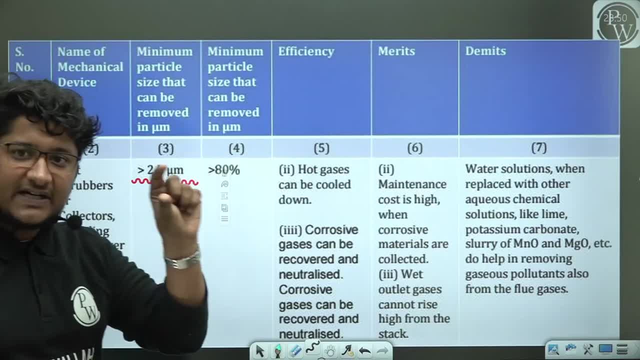 greater than 2.5 micrometer dekh sakte. uski thote particle ko bhi remove kar raha hai, wo aur uski efficiency bhi greater than 80% hai. next, jo aapko loko dimaag me rakhna hai. 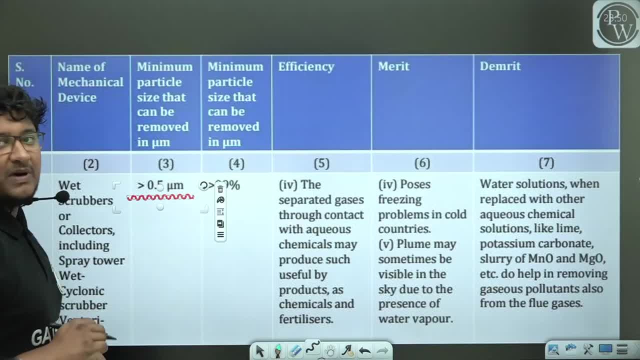 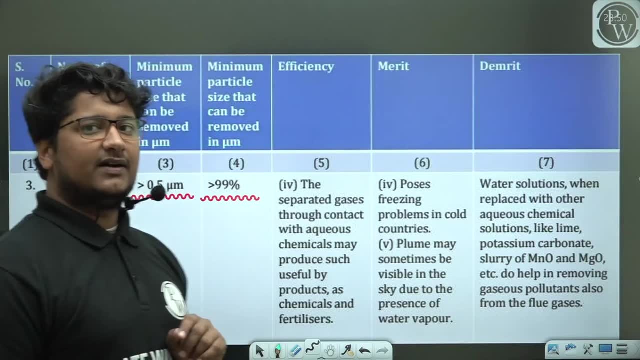 wo hai aapka Venturi Scarver to 0.5 micron particle se bhi jyada ko aapko remove kar raha hai, aur uski efficiency aapki greater than 99%. this baat ko aap log dhyan me rakhye ga. 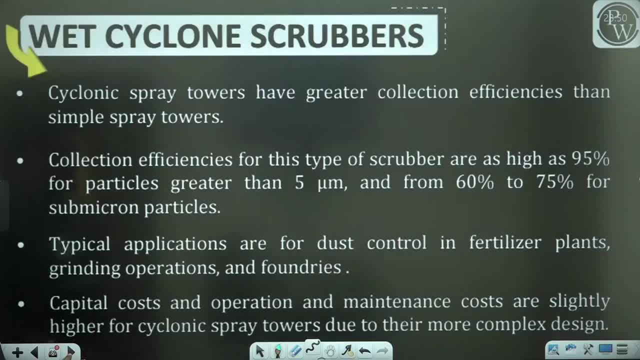 jo bhi baate me aapko underline karwa raha hu, usko aap jyadur dhyan me rakhye ga baaki, ek baar padhna jyarud hai. ek baar padhna jyarud hai. 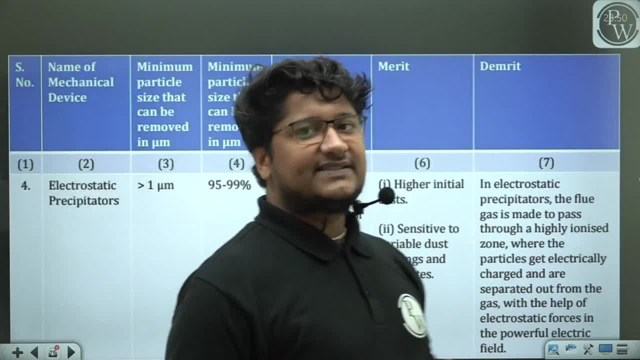 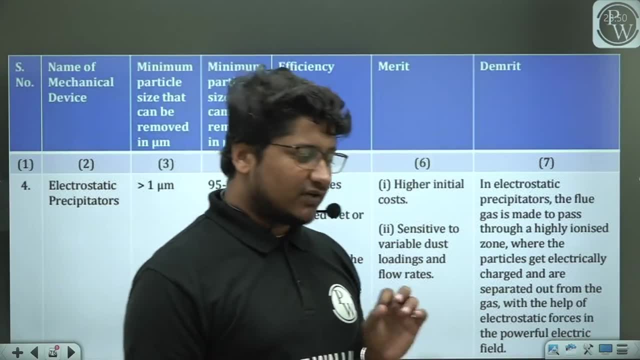 chill. ye. now the next thing comes, that is electrostatic precipitator generally bohot jyada use hota hai. short form, me isko am log ESP bolte hai, aur ye khas kar wahan use hota hu. dekhay hoge. 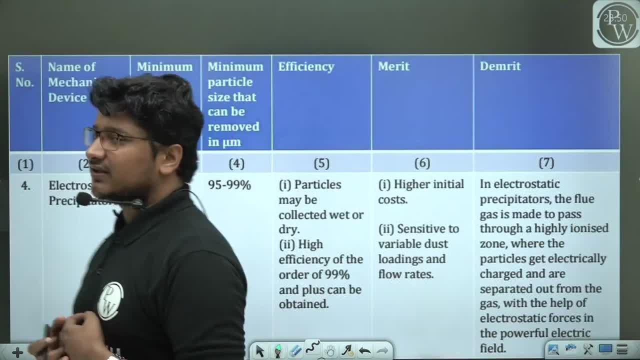 jyahan aapka thermopower plant hai, ki fly ash vey gara, ye achcha remove kar kaam. kaise karta hai? pehle wo dekhte hai, phir iske data pe aayenge, ham log. 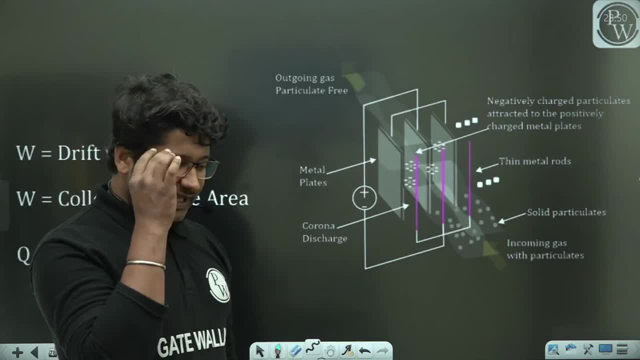 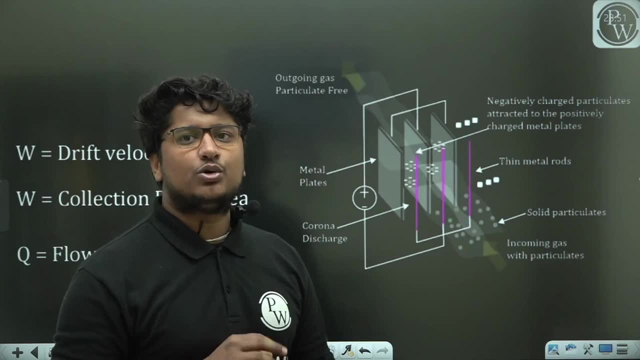 basically, humne kya bana ke rakha hai. humko malum hai ki har particle me kuch na positive, kuch negative charge toh rehte hi hai. jo bhi aapke particles rahenge, jisko aap remove karna chahte ho. 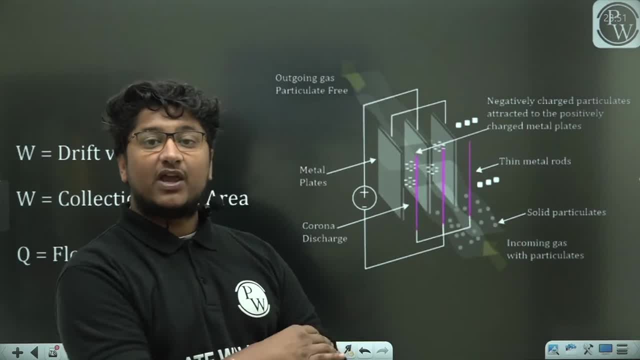 toh kuch positive, negative charge toh rahenge. saayad, wo apna charge show nahi kar rahe hai, wo jagye hue nahi hai, unko jagaani ke liye kya karte hai, unko ek charge wala design develop kar dete? 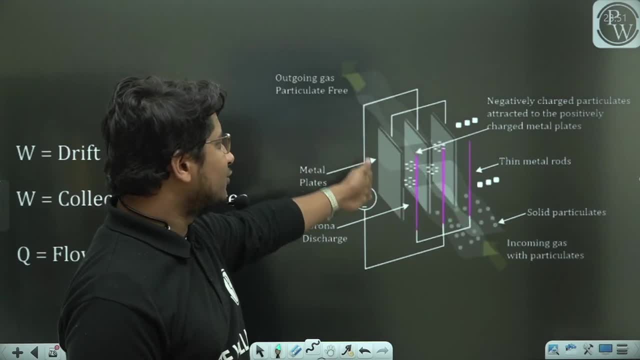 kaise develop karoge, sir, hum kya karte hai? ek plate liye positive wala part. 2ra aapka plate hai usme aap negative wala part, aur beech me aap ek reason develop kar diye. 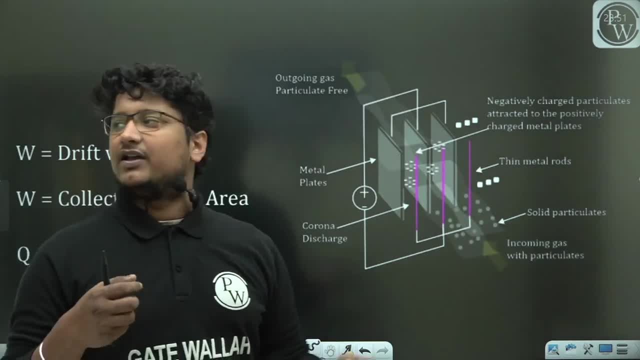 jahaan pe aapka charge koi bhi particle aayega, toh khud jag jayega ki aad bhaiya yahan toh positive, negative dono hai. toh hum, kya hai, sir? hum toh positive hai. 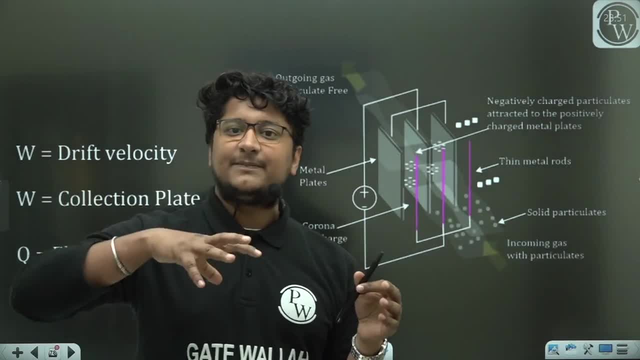 toh bhaiya positive wale part me de in a sense, wo aise normally charge particle tha. lekin jaise aapko pata chalta hai, ki jaise for example samjho, ki aap kahin gaye. 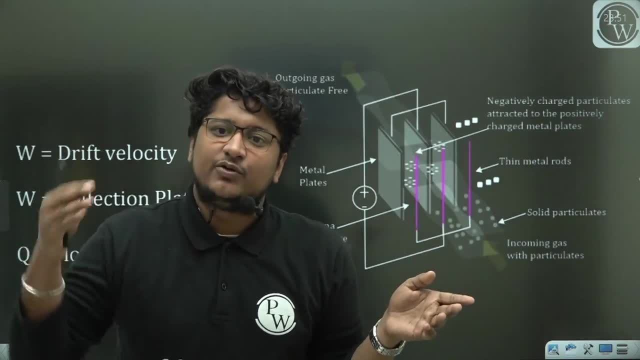 jaise aapko pata chalta hai ki bhaiya, ye toh Bihar hai, toh bahutte hu, ki me Bihari hu, ya Chhattisgarhi hu, ya Nepali hu ya, lekin jahaise kahin baat aati ki bhaiya. 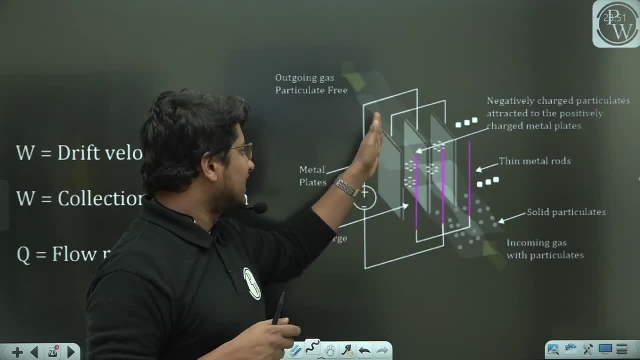 yahan toh alag lag batte hu hai. toh wahi wali baat hai, ki aapka jo collection plate hai, aapko alag, alag, in a sense ek collection plate aapko yahan bataya hu. 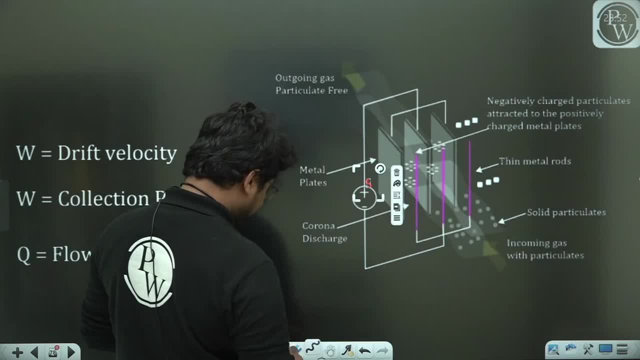 dekho yahan pe dono plate ko hum ne kya kiya hai. power se connect kar diya hai. power se connect kar diya hai. toh aise me kya hoga, ki jo aapka negatively charged particle hai. 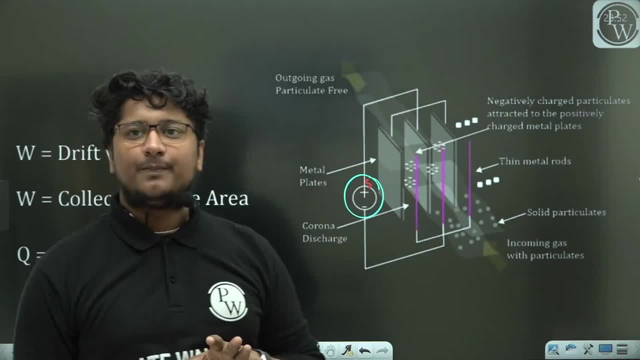 wo aapko attract ho jayega, positively charged metal plates pe. aur opposite bhi ho sakta hai aapko. let us say, aapka jo plate hai, wo positive charged particle hai, aur aapke particle kya huwe uspe attract ho gaye. 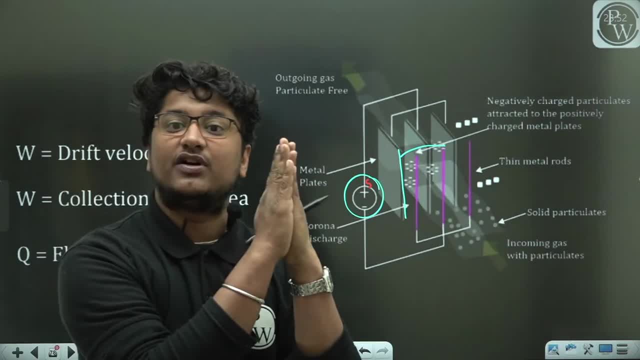 ab ye particle aapko uspe attract ho gaye, just because kisli attract ho gaye, toh ki abhi aapne waha pe charge develop kiya hua hai, aapne ekko positive, ekko negative banaya hua hai, dono rod me. 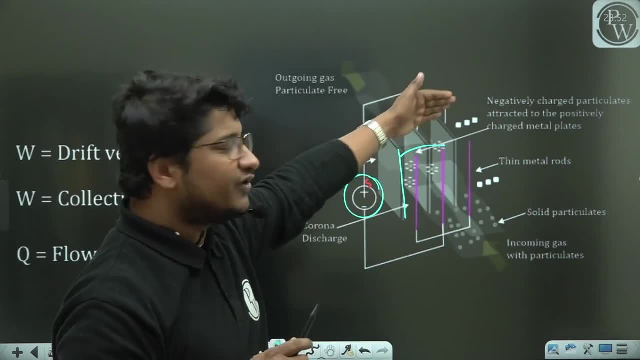 toh jo plate hai aapne. for example, usko aapne positive banaya hua hai, toh negative charged particles uspe attract ho rahe hai, toh ye tab tak attract rahenge, jab tak aapne light on ki hui hai. 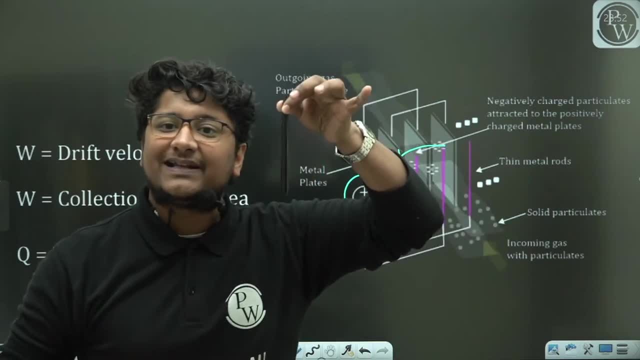 jaise hi aap light off karoge, jaise hi aap light off karoge. in plate ka jo tha charge wo khatam, toh ye jo particles usme se attract the chipke huwe the, wo bhi aap chipakna khatam. 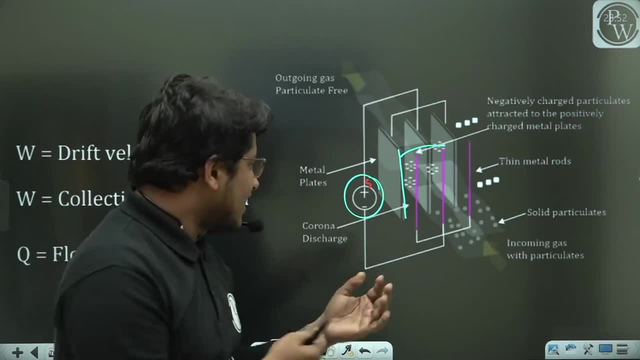 ab wo attachment rahegi nahi, toh kahan niche gir jayenge, niche hum ek hopper laga, ke rakhenge usme saare particle ko collect kar liye, jab ye on tha, tab hum isse air mass gujaare. 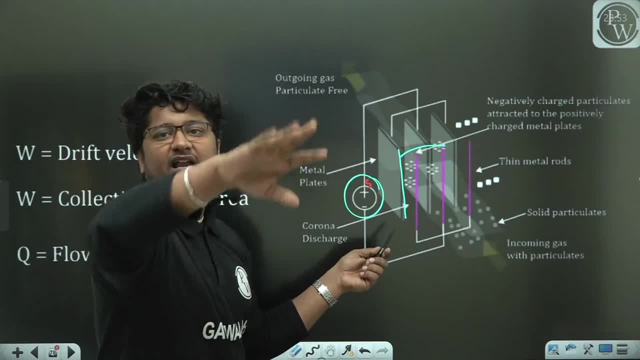 aapke particles isme chipak gaye air mass jo bahar nikla ekdum completely free mila aapko particles se jaise hi aapka saara air. aapko gujar gaya light off kijiye. 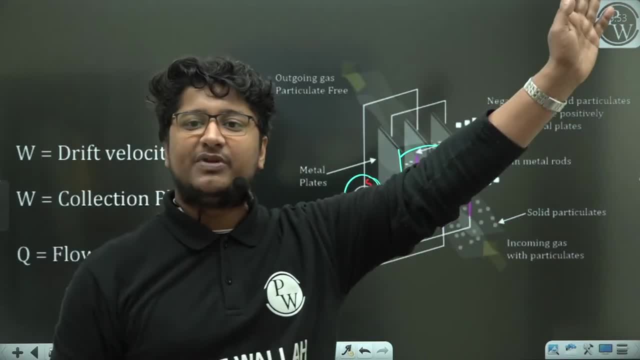 niche hopper hai, usse collect kar liye. jo bhi aapka particle mila aage, usko, jo bhi karna hai, aap kar liye. toh ye aapko kuch is tarike, se aapko ESP kaam karta hai. 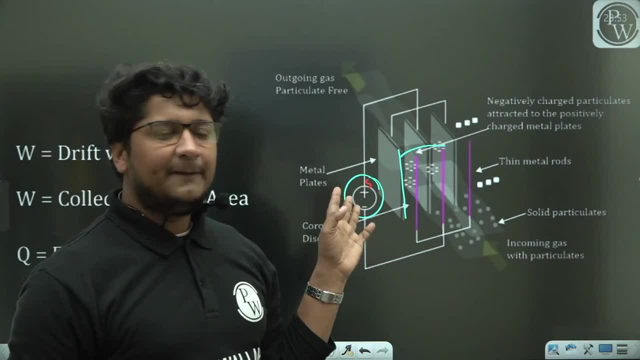 obvious hi baat hai. dekho, kharcha jyada nahi hai isme initial kharcha thoda hai. baaki isme kuch equipment jyada raha te nahi hai plates hai itna hi kharab hongi. 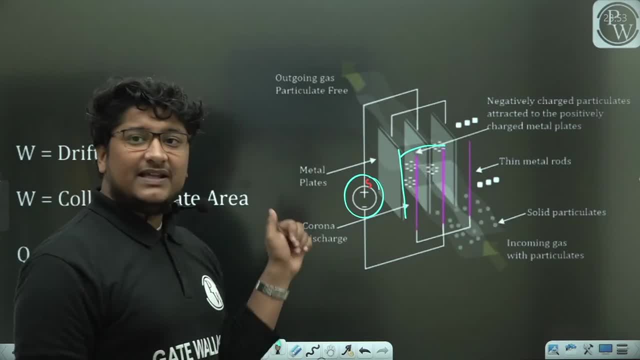 toh aapko maintenance thoda lower cost padta hai iska, but initial cost jyada padta hai. initial cost jyada padta hai. is baat ka dhyana rakhiye. chaliye toh iske regarding. 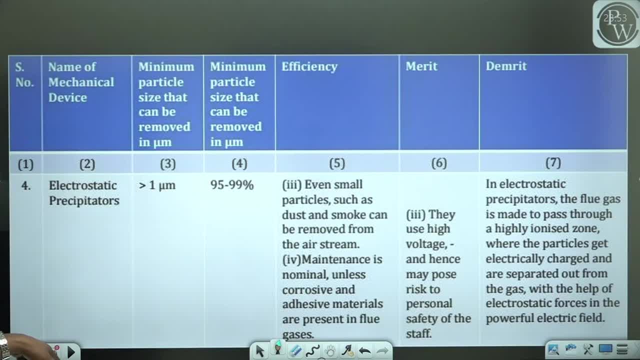 agar baat dekhiye, kuch, kuch baate, jo aapko dimaag me rakhni hai. toh pehli baate, jo aapko dimaag me rakhni hai, woh hai ki bhaiya ye. 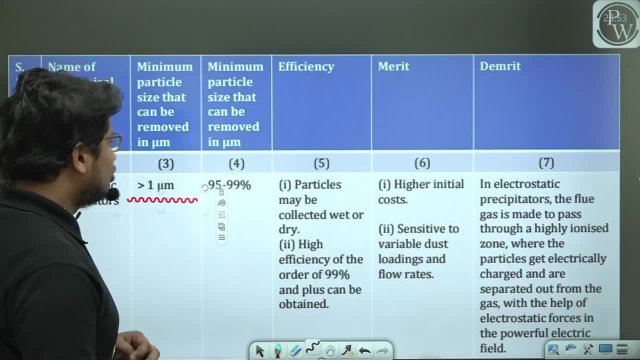 greater than 1 micrometer particles ko remove karta hai. dhusra ki, sir, ye 95 to 99% jo aapka particle isko ye remove karta hai. efficiency bhi achchi hai, dhusra, dekho dhyana do ki particle. 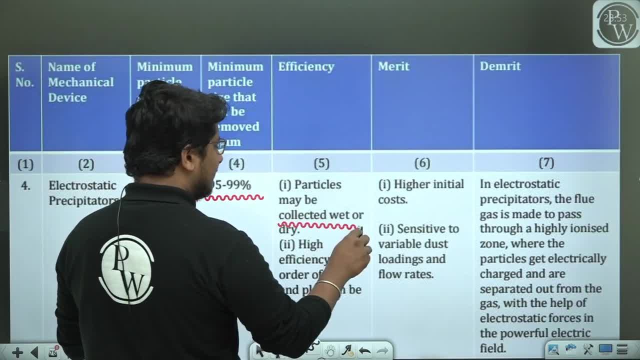 may be wet, may be collected wet or dry. toh aapko dono condition mein aapka kaam kar raha hai, tisra aapko kya hai? dekho aapka ki higher initial cost hai jo mai aapko. 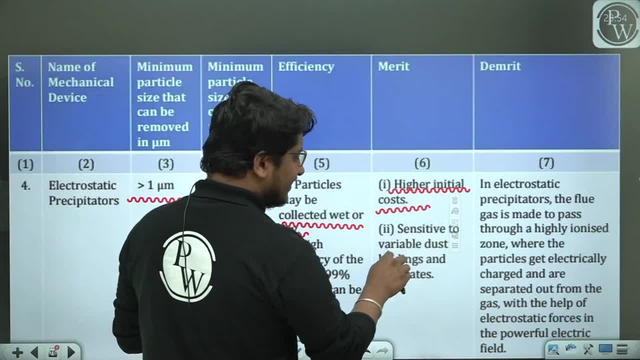 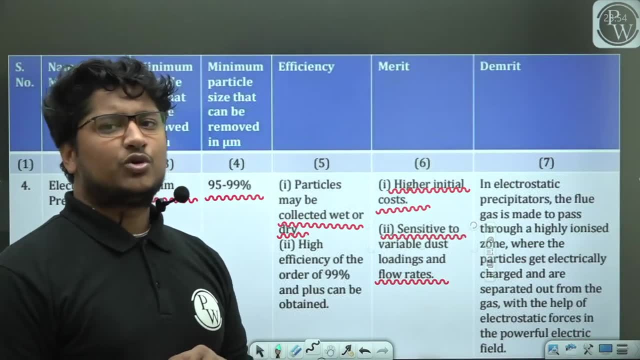 already bata chuka hu. aur tisri point: density variable to the dust loading and flow rates. agar aap variable dust loading doge, toh thora sensitive hai ki bahut jyada aap variation kar sakte. ho load me. 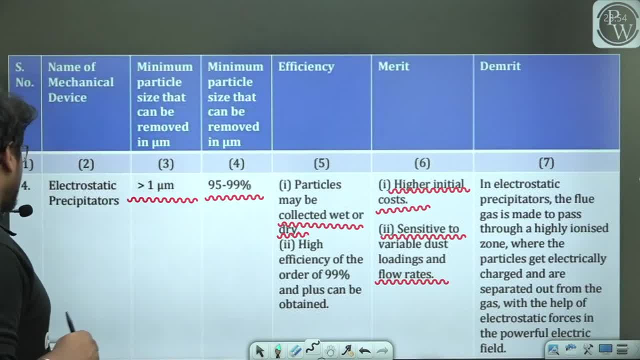 aisa nahi thora aap ispe dhyana rakhega. next jo point: aapko dimaag me rakhna hai: woh ek aur cheez jo dimaag me rakhni hai, yeh wala, jo mai aapko bata chuka tha. 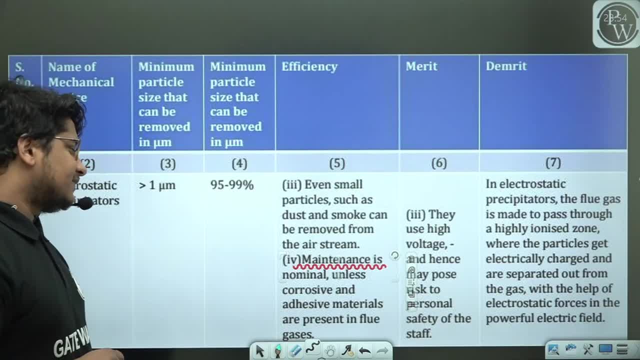 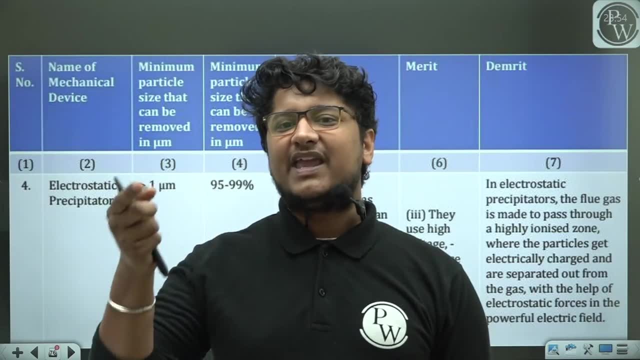 maintenance is nominal, unless corrosive and adhesive materials are present in the flue gas matlab. generally aapka maintenance ka kum hai, generally aapka maintenance kum hai. but problem hai ki agar aapki air mein koi corrosive metal rahega, toh 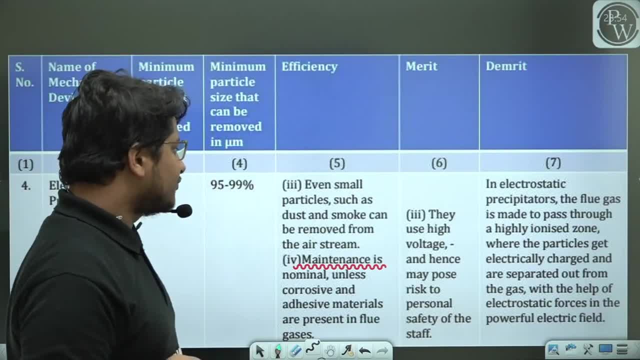 aapke plate ko corrode kar dega, toh phir aapko plate badalna parta hai. yeh ek problem hai, aur ek aur isme hai ki bhaiya, they use high voltage, they use high voltage. aur. 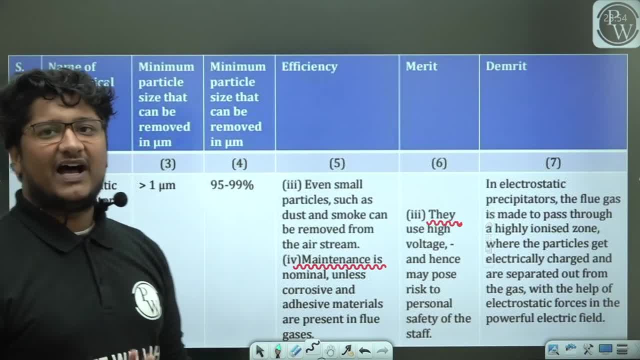 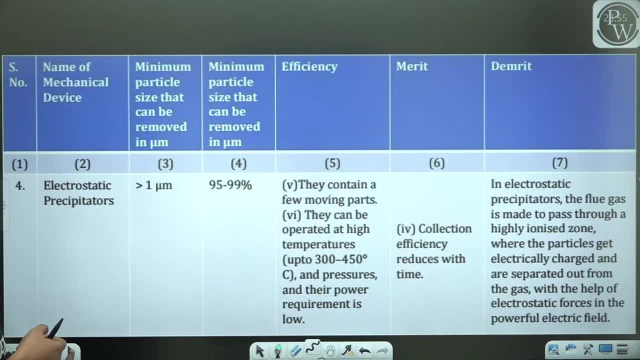 hence may pose risk to the personal safety of the staff. a bhaiya, high voltage se kheloge, toh high voltage ka jhatka toh laghi sakta hai. na chali acha yeh ESP itna jyada famous. 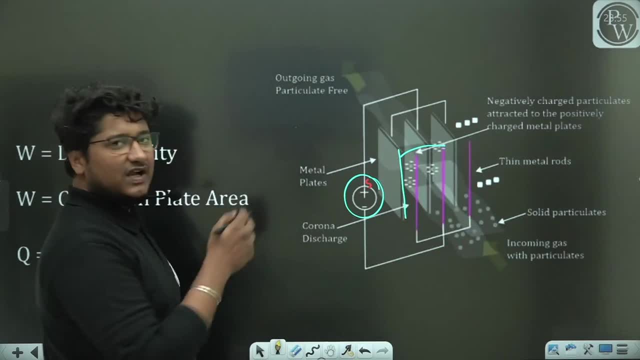 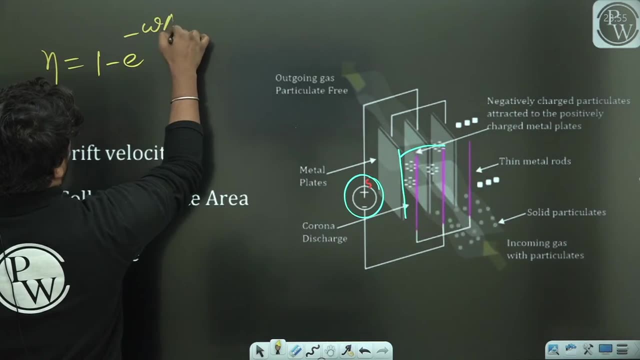 hua hai. na ki iska ek formula bhi banaya hua hai: efficiency, inka ek formula banaya hai, jo aap loko dimaag me rakhna hai: kita equal to 1 minus e. power. omega a by q. 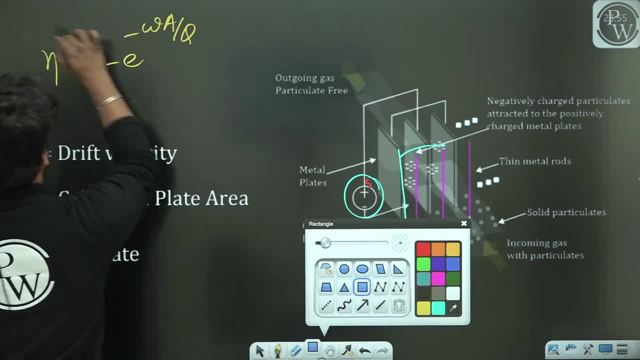 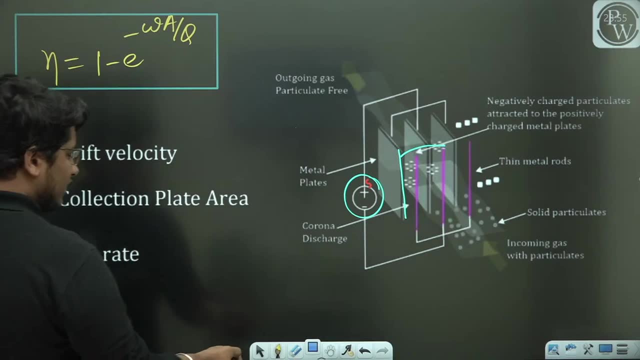 is formulae ko dimaag me rakhna hai. bholna mat important formula hai: eta equal to 1 minus e to the power omega a by q. agar koi efficiency pooch raha hai percentage mein, toh aap isko multiply kar lena. 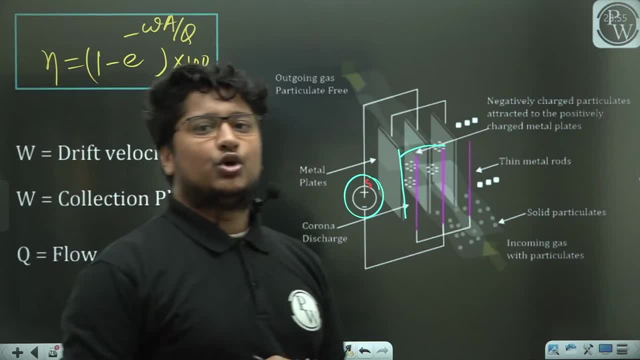 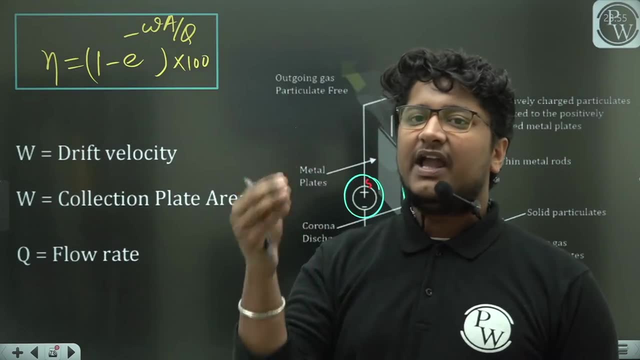 100. se tike toh formula. kya bini gaya: 1 minus e to the power, omega a by q, where omega is the drift velocity, a is the collection plate area and q is the rate of flow. jo aap. 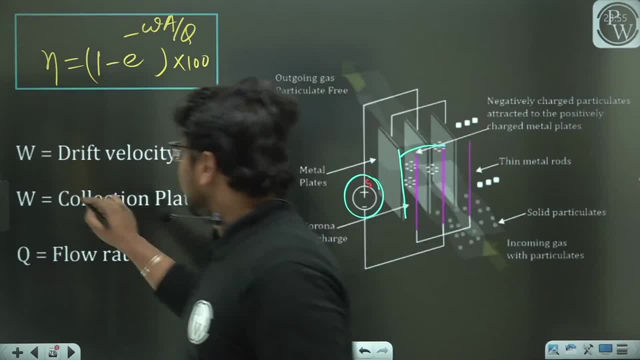 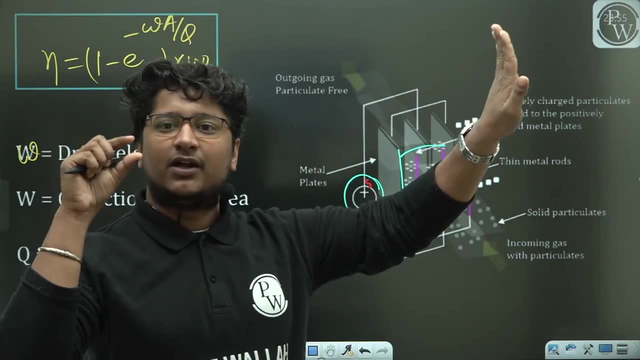 de rahe ho ab drift velocity. kya hoti hai? isko samajhna ki omega hai bahute simple cheeje ki collection plate hai aur particle hai collection plate aur particle jo hoga collection plate ki taraf attract hoga jo. 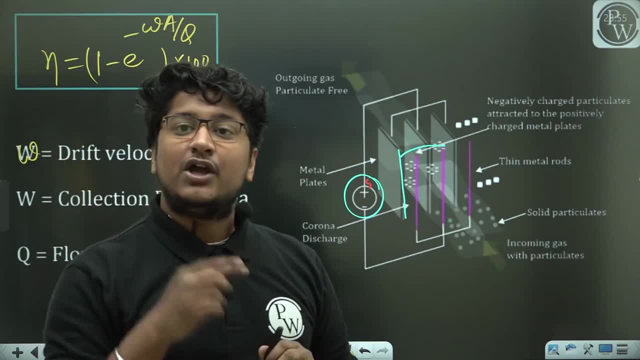 particle attract hoga. toh kya hoga? move karega collection plate ki taraf toh, wo jis speed se move karta hai, usko hum bolte hai drift velocity, ab yaha ek sawal banta hai conceptually. 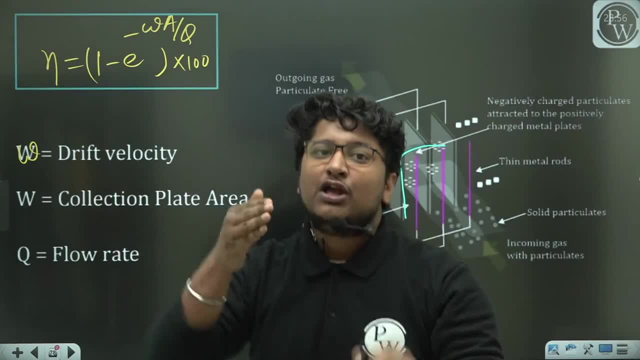 ki sir, ek bada particle hai aur ek chhuttu particle hai. tono ki drift velocity: me kya antar rahega, kaun kiski velocity jyada hogi? drift velocity, ek chhota conceptual. 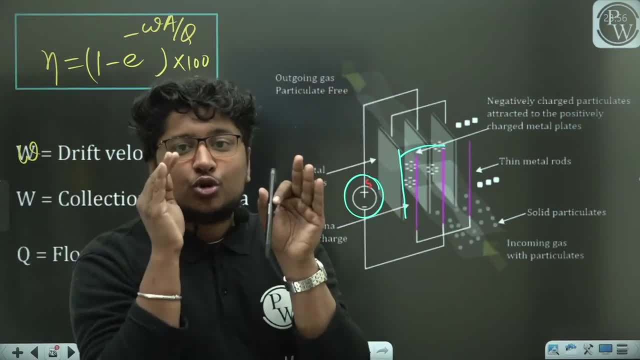 question: banta hai ki sir ek bada particle hai aur ek chhuttu particle hai. tono ki drift velocity me kya antar rahega? Mahesh singh bol rahe hai, sir, aapne jo environment engineering ki youtube padhaya tha? 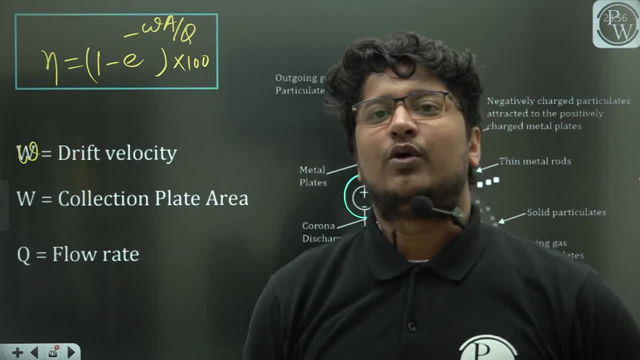 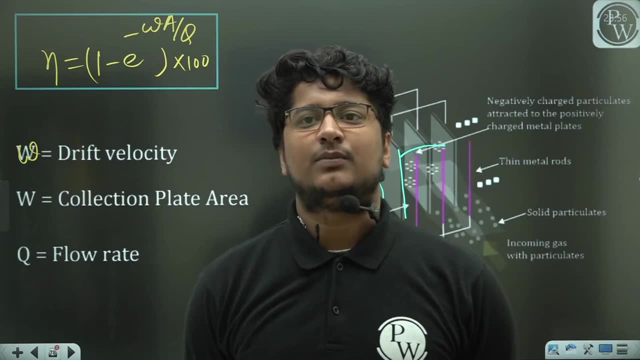 bohot accha tha aaj hi exam dekar aaya hu guda ho gaya kaunsa exam diye. bache aaj for that good thing, aapke exam. by the way, kaunsa exam dekhe aaye bhai. 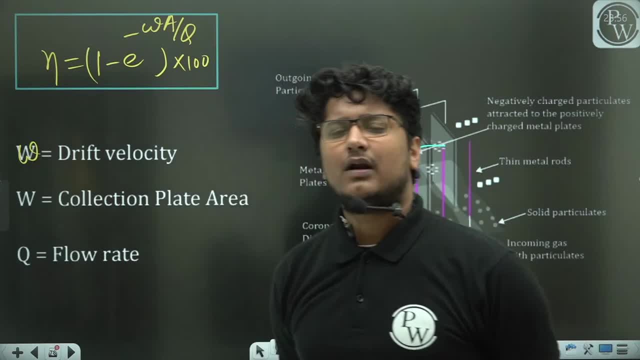 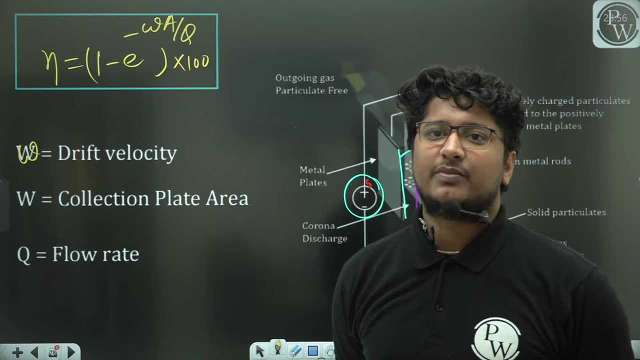 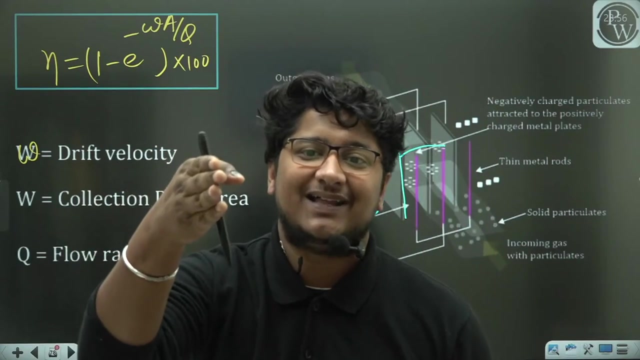 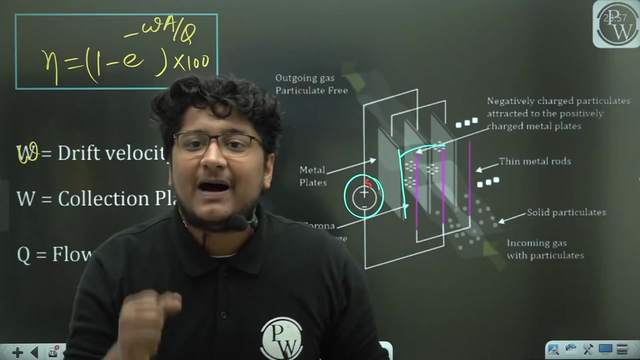 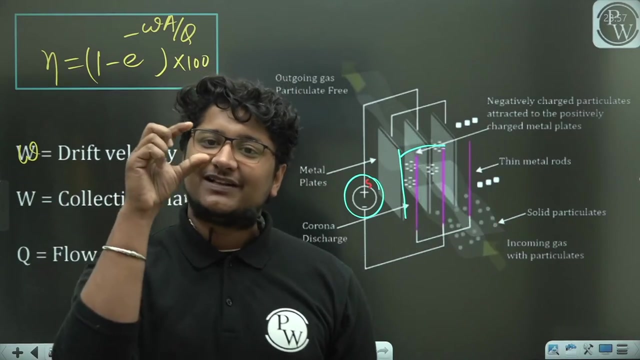 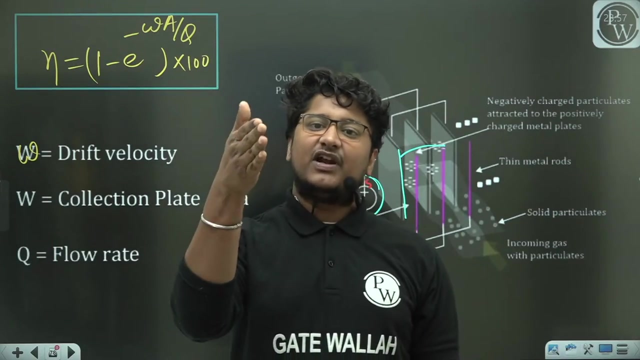 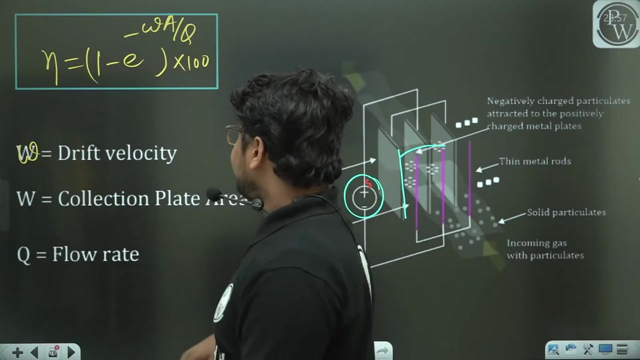 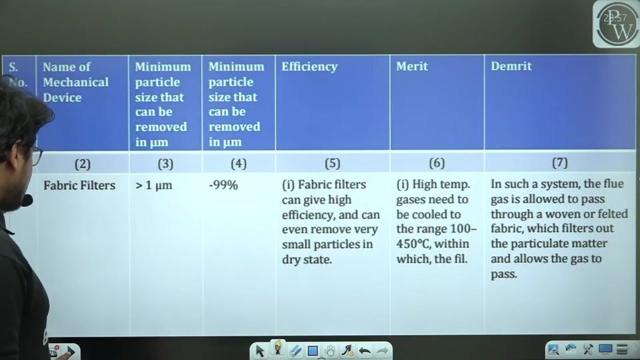 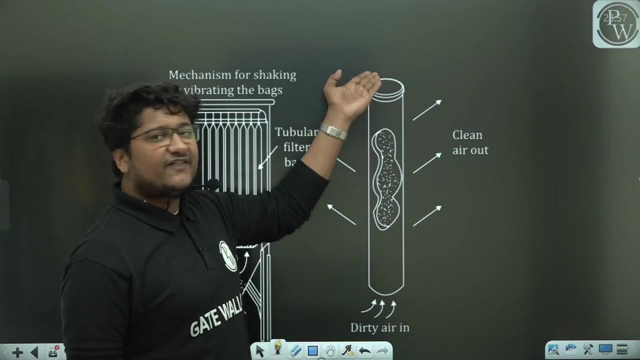 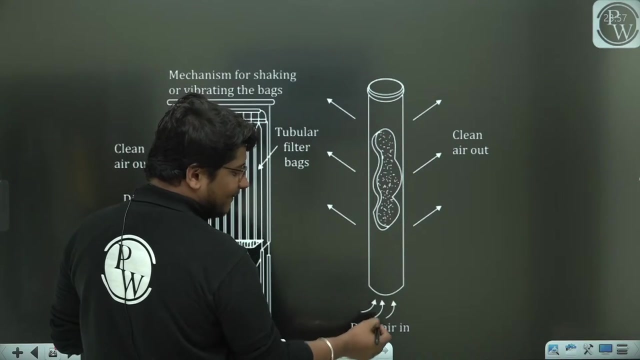 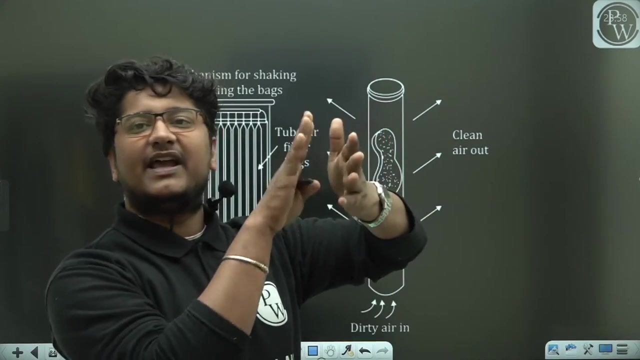 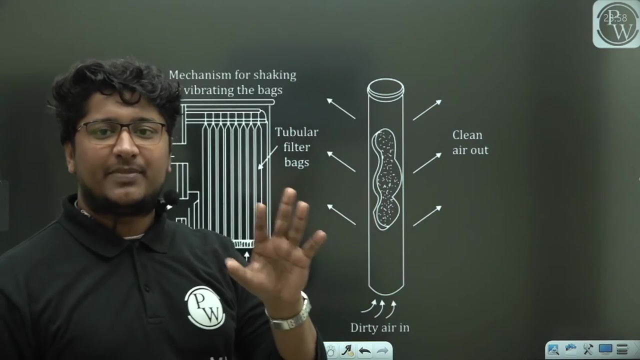 abhi recent koi exam tha kya. So this is your one fabric filter. something like this is a fabric filter. now see how your fabric filter works. you have given dirty air from the bottom. your whole fabric filter is made of a whole fabric in which air passes, but solid will not pass. it is like you understand cloth. you see the cloth. sometimes if you pass air through it then dirt stops on the cloth and air comes out. so normal cloth is not used here. the fabric is of good quality so that it can withstand a little temperature. 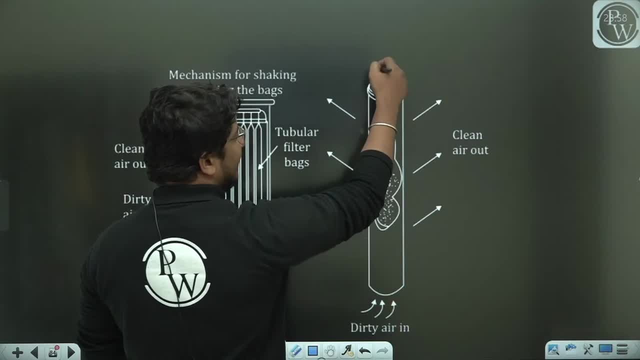 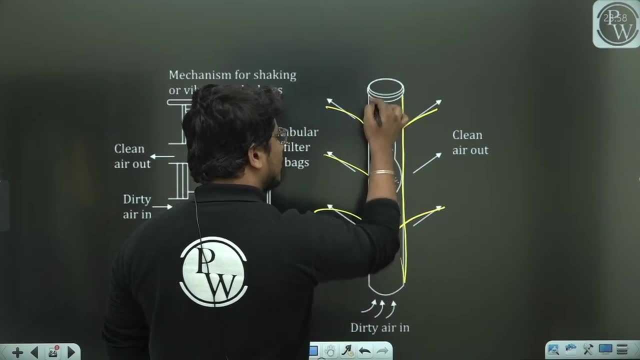 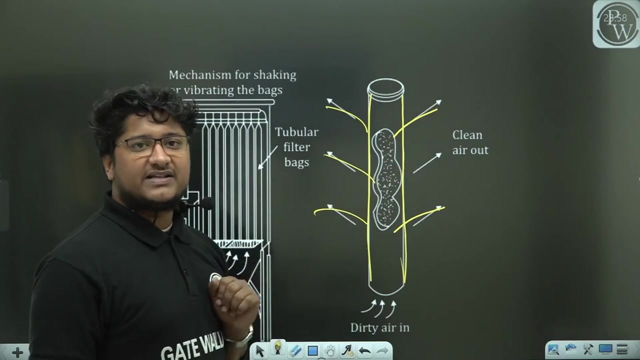 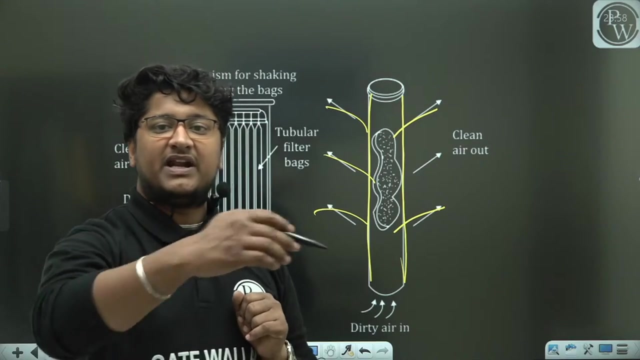 okay, now the air you put from here, then the air does not wait to go up. wherever it gets space from the side, it comes out. and when it comes out, what will it do? it will leave its dirt on its surface, it will leave its pollutant matter and clean air will come out. now, if you want to make a big tube, then what is the problem? instead of making a big tube, we make a lot of small diameter tubes. 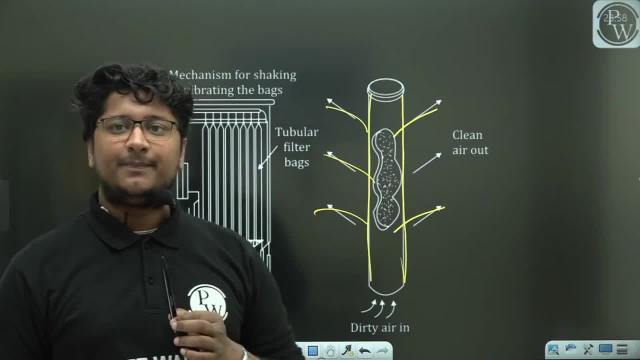 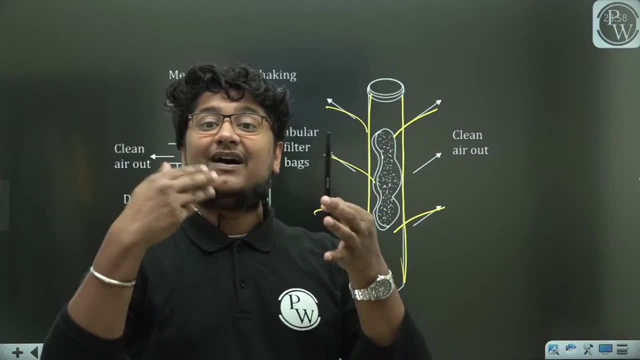 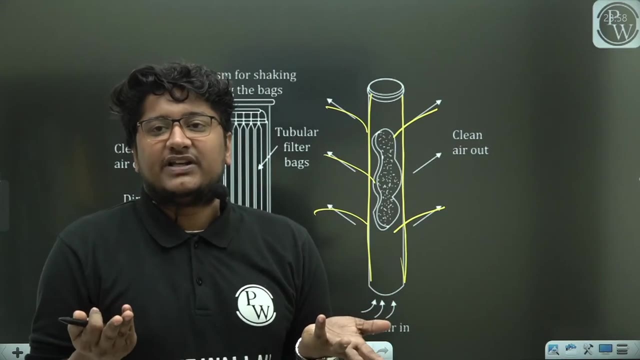 means we carry multi tubes. we keep multi filter bags. what is the benefit of it? the benefit is that if you keep a multi filter bag, then you will provide more surface area in the same space. you will provide much more surface area, the better your efficiency will be. you will understand it very clearly. 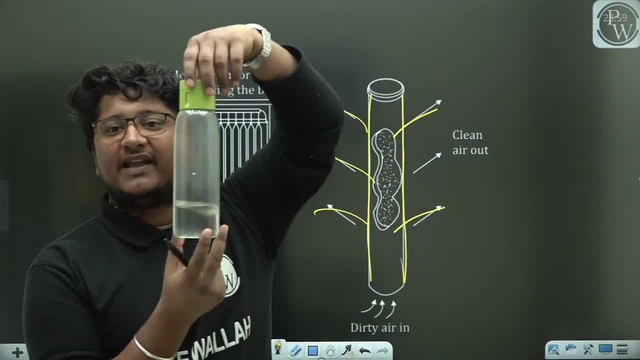 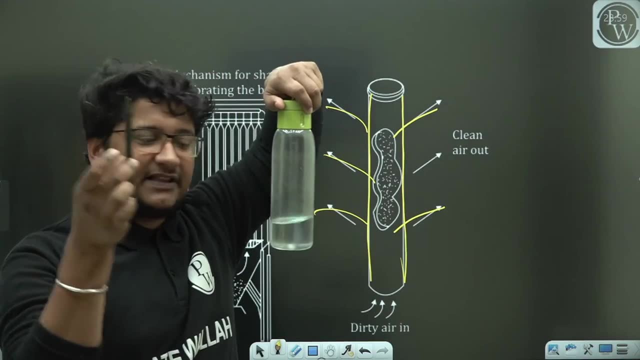 that, if you understand that I took this bottle now, this will be the surface area of this, this surface area. in place of it, I will make such thin, many thin, thin, many small, thin tubes, make all these cylindrical shaped tubes here. then the obvious thing is that its surface. 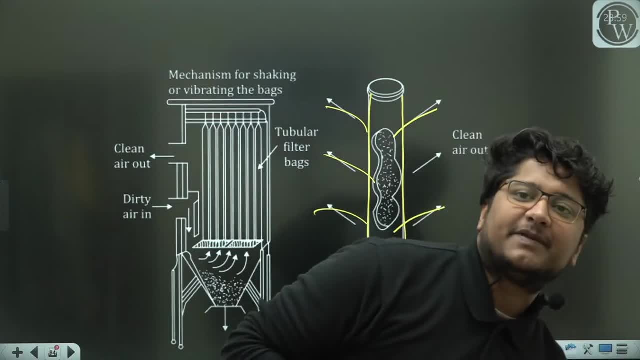 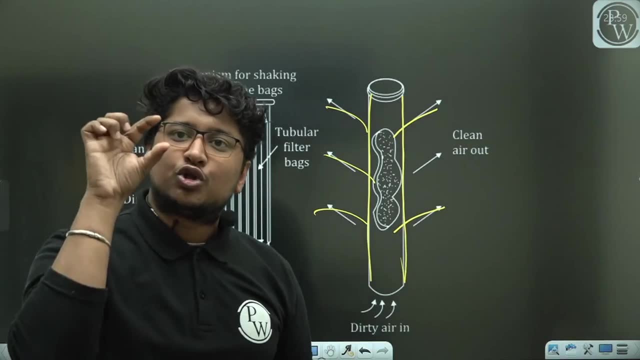 area will be more. the smaller the tubes are, the more the surface area will be. it is like you took a cube of 1 meter x 1 meter x 1 meter. you broke it and changed it to a small 1 cm. 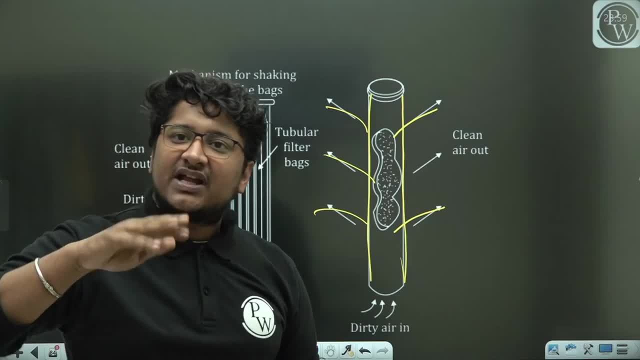 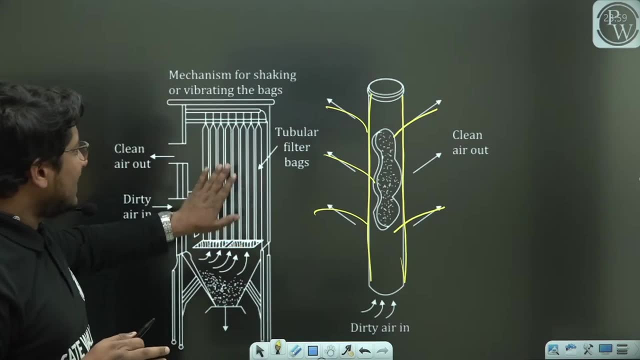 cube. so the obvious thing is that your surface area will increase. the more your surface area increases, the more your efficiency will increase. is that clear? now understand in this matter that you are doing this work like this, so whatever you put in it from here, your air. 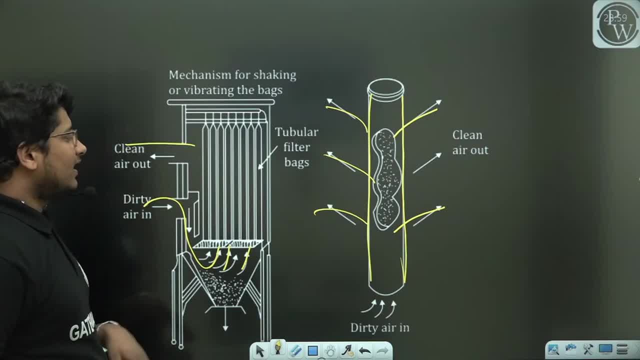 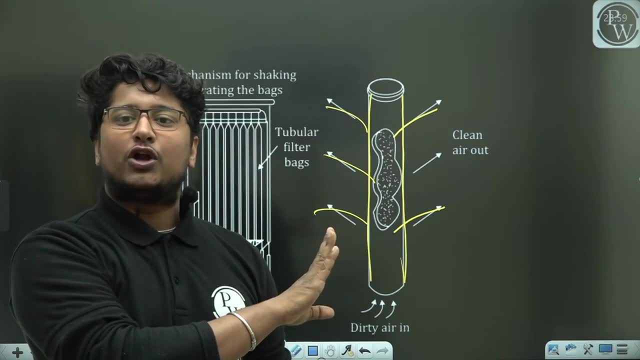 came in. it went in from above. you got clean air output. now what happened that? a time will come when the entire filter bag of yours will be choked. so you said that now stop the air inlet a bit and see how the mechanism is placed in it. we will vibrate it a little. 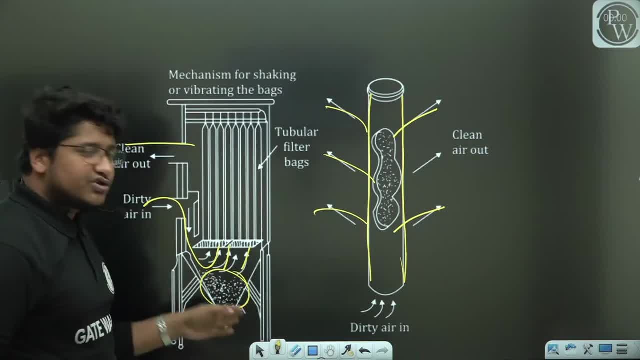 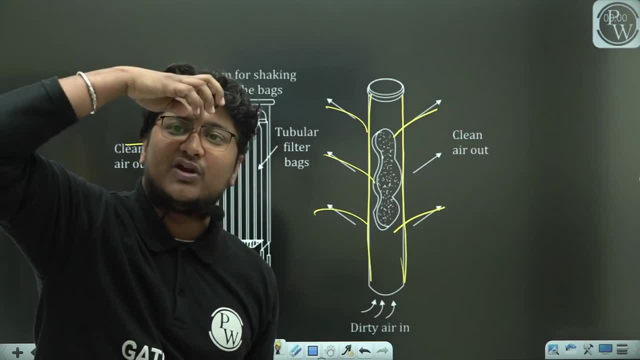 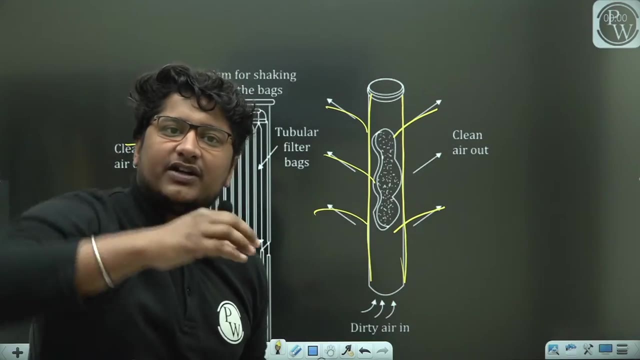 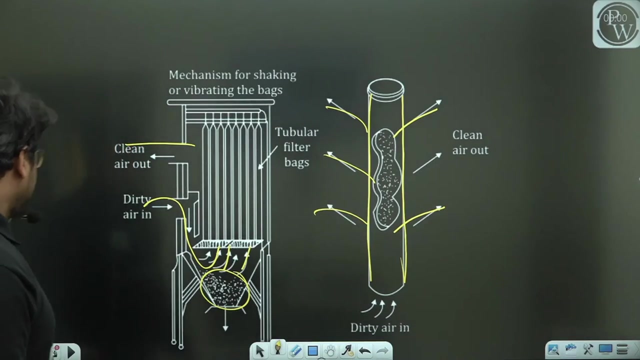 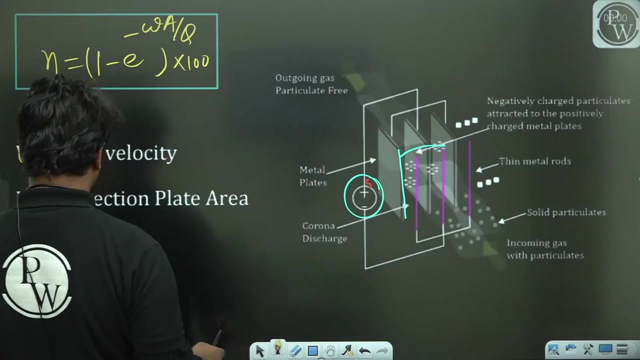 when you vibrate it, then all the dirt will come down. it will be stored here in the hopper which you can clean later. so what happens to this? when the dirt comes down, then it, When this is completely choked, you show that you need a little cleaning. then stop the air a little and vibrate it completely, vibrate it completely, vibrate it completely. when you vibrate it completely, it will fall down and fall down and then you use it. then again you use it through it. you understand it is a little better. if you look at its efficiency, you will like it if you look at the efficiency. once your efficiency is greater than 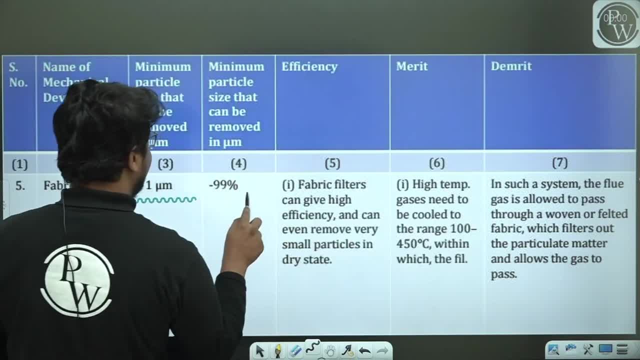 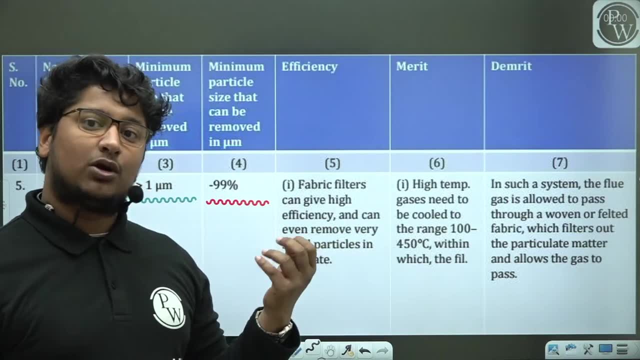 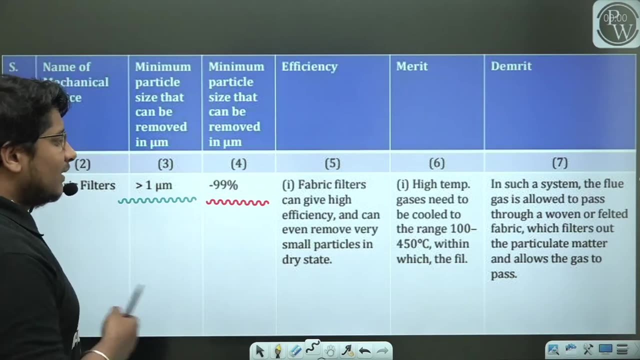 one micrometer and its particle size removes it means till one micrometer. it removes any bigger particle than that will remove everyone. and efficiency also goes up to 99%, so you can keep it in the best efficiency part. there are some problems that you will keep in your mind, like high temperature. gases need to be cooled. you can't keep it at high temperature. 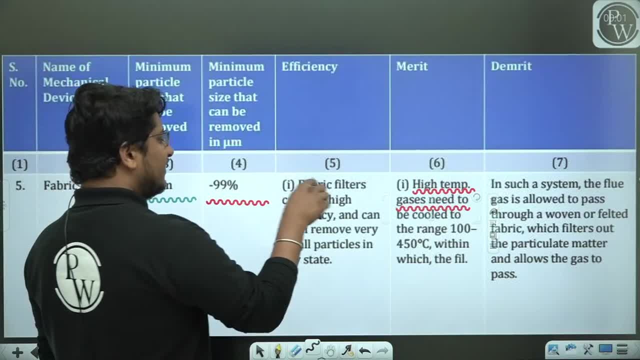 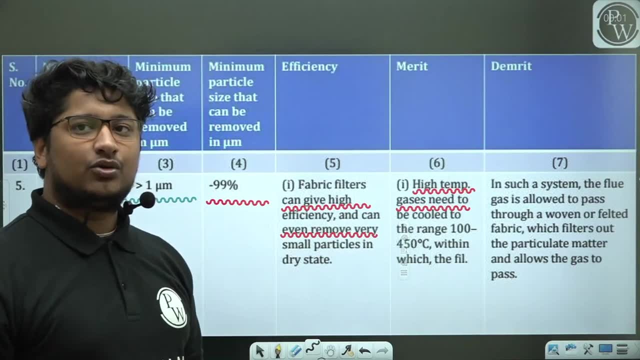 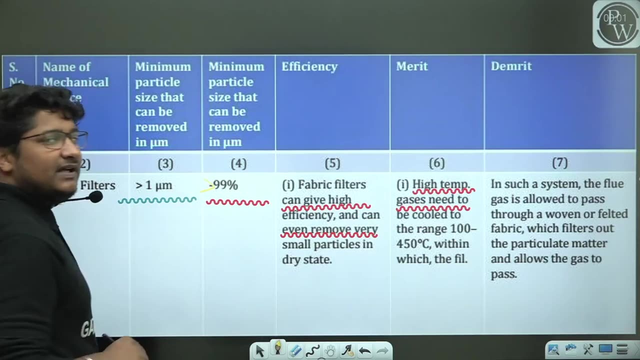 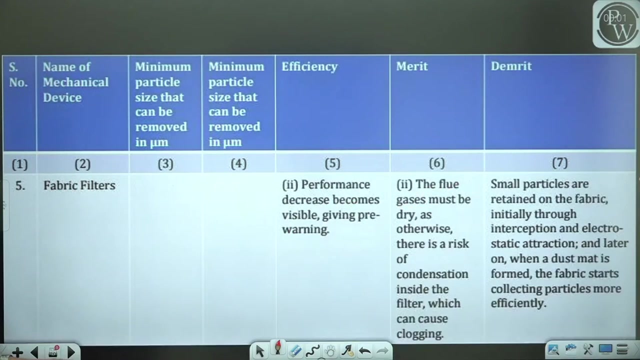 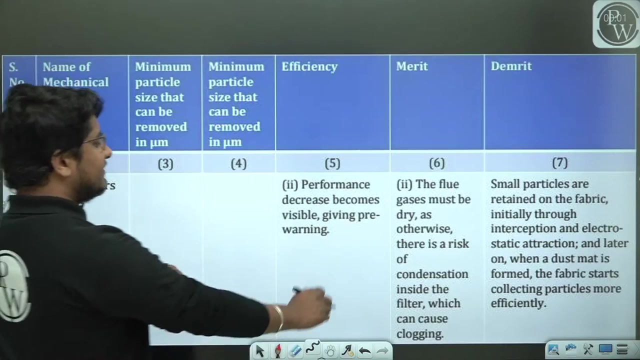 third, fabric filter can give high efficiency and can even remove small particles. you know this now. here you can work in dry state. here you can work in dry state. so here you can see that 99% is sometimes more than 99,. sometimes more than 99, so some people are saying that more than 99, yes, sometimes more than 99, you will see. the only problem is that you will see that its performance is decreasing. performance decreases becomes visible. giving pre-warning. 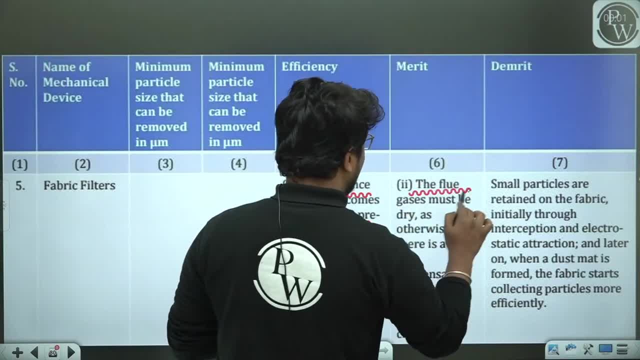 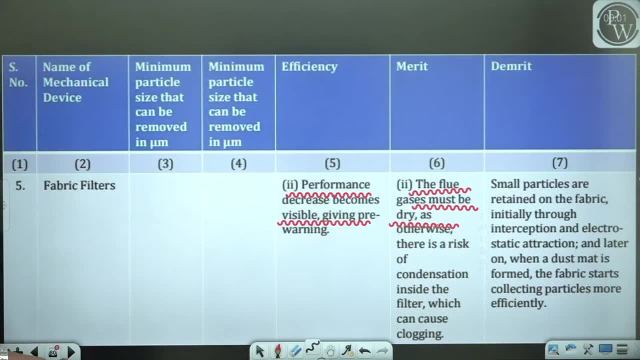 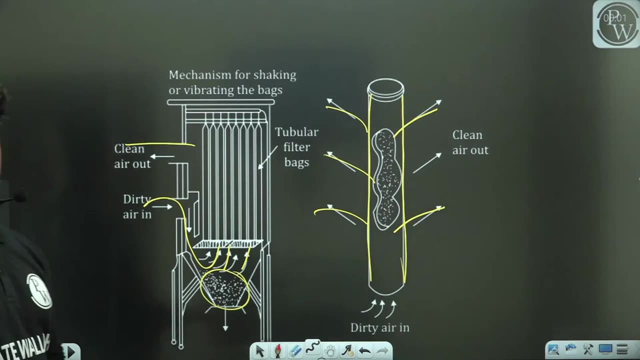 and here you will only use the dry one. the flue gas must be dry, otherwise what will be the problem, brother? you will have more choking. then you will take care, and this means that even the gases that will remain there should not be any chemicals in it, otherwise your fabric can be damaged due to chemical attacks. 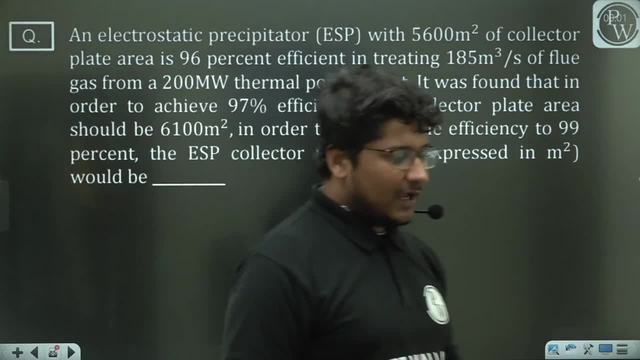 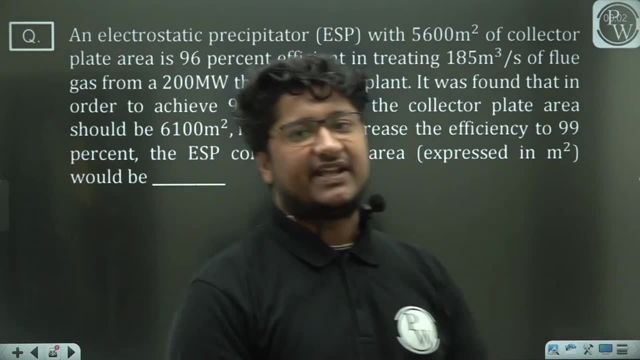 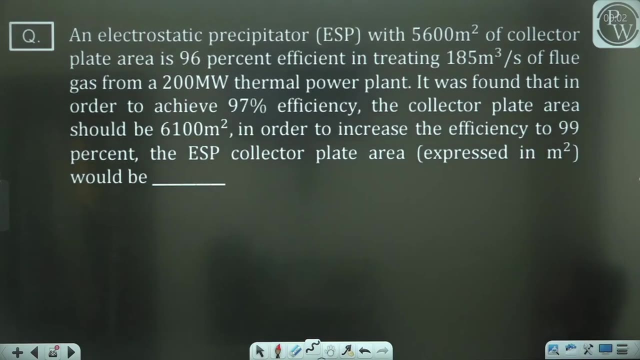 there is one question. let's do it quickly now. the theory part is not much to ask. now we will do the questions and then this chapter of yours will end. we will do 4-5 questions. so we will do it. do it slowly, there is no hurry. 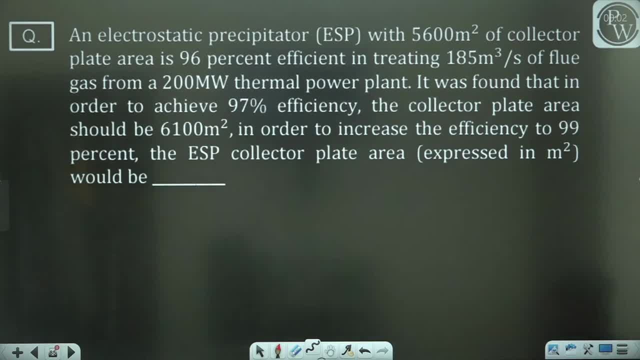 sir, just now, just give me half an hour more, your chapter will be completed. only half an hour, not even half an hour. if you make the problem fast, then not even half an hour. sir, now the bus is in the class from 4 o'clock. no one will catch. we will see for another half an hour. 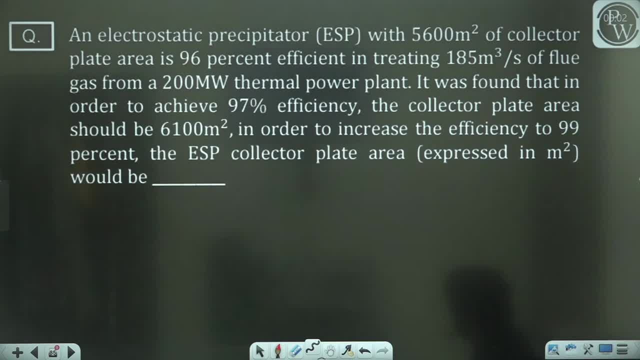 let's go, brother, I am tired. tell me which is the latest good movie you have seen. which is the last good movie you have seen which is a favorite movie? which is a favorite movie which is also good in the language of language? 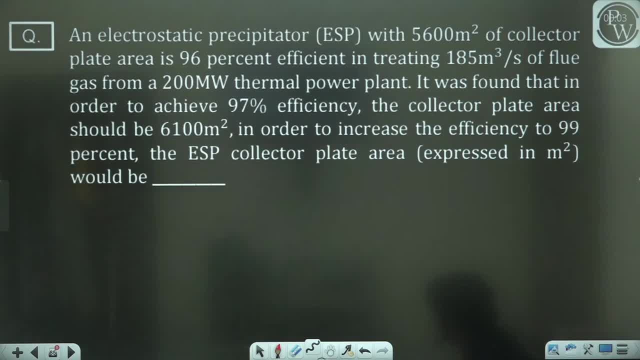 which is also good, because in the language of language, language and the language, we have a group of people, the middle class people or the people who are in front of you. give us a good reply. read it, it is not difficult. 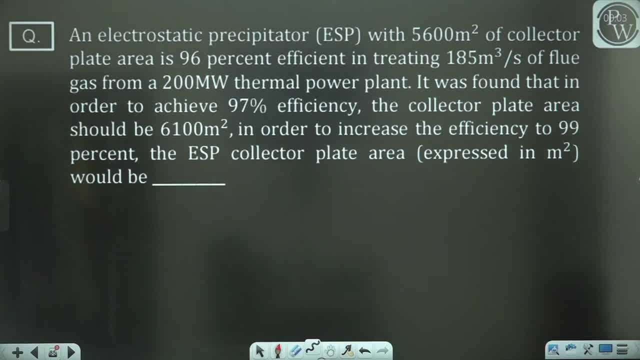 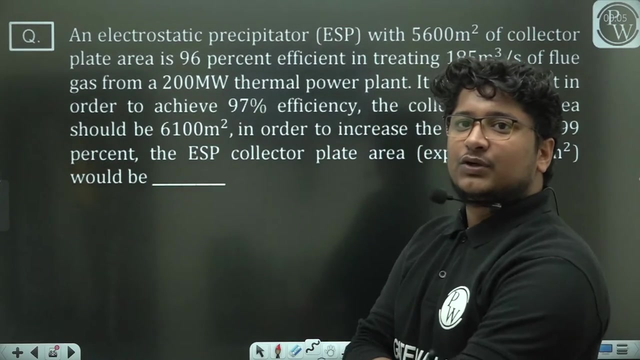 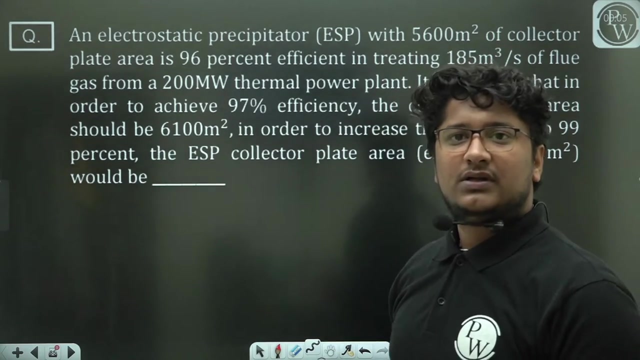 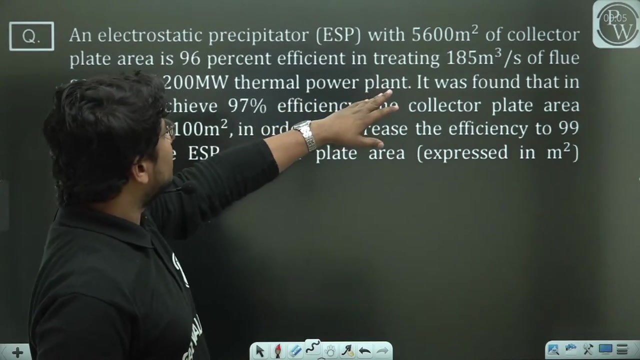 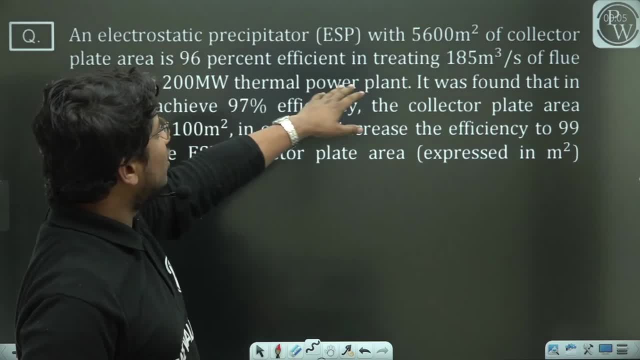 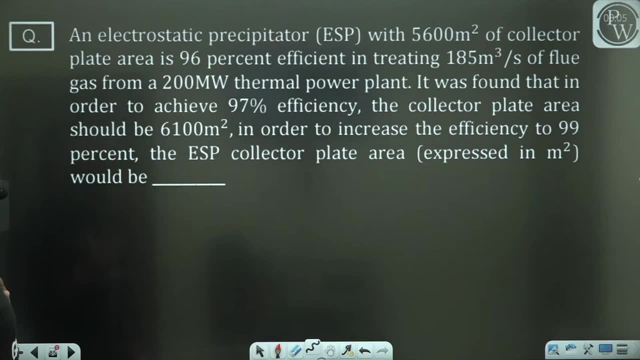 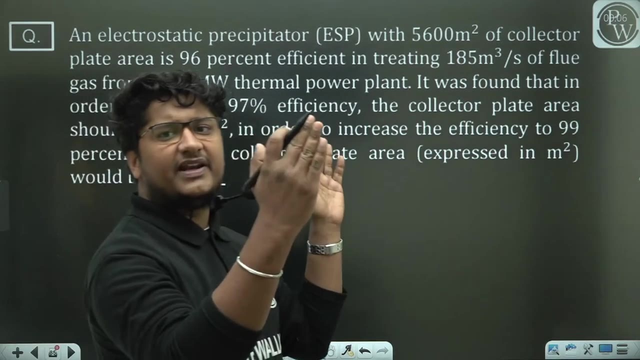 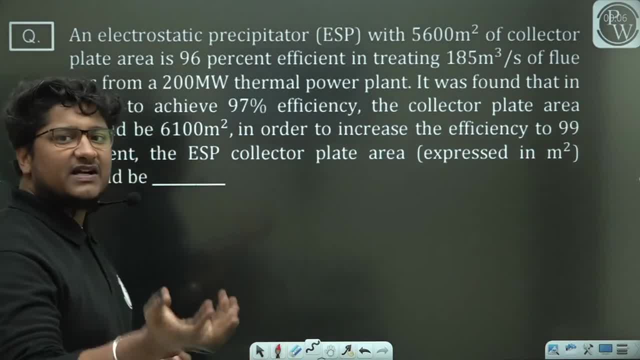 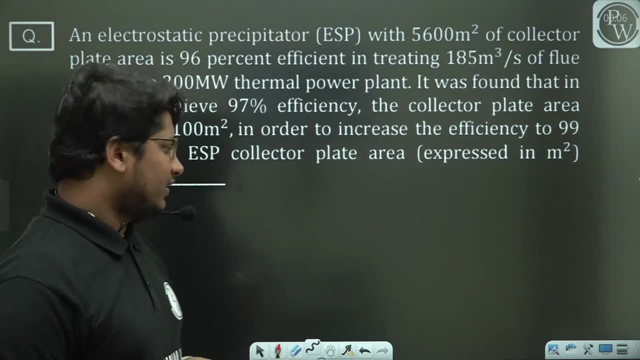 I am asking: collection plate area. there is no doubt you can attract more particles. so if you want 99% efficiency, then what is the collection plate area? okay, no problem, we know the formula. let's talk about the first case. the first case you have given is 96%. 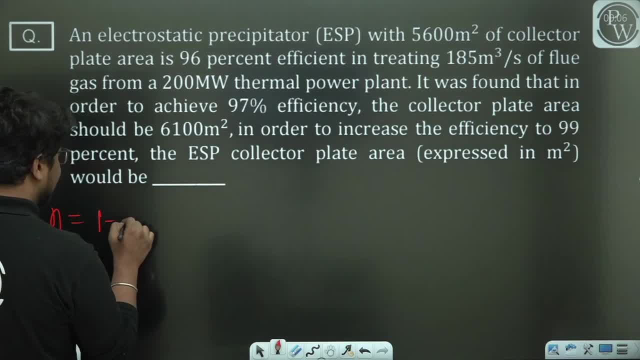 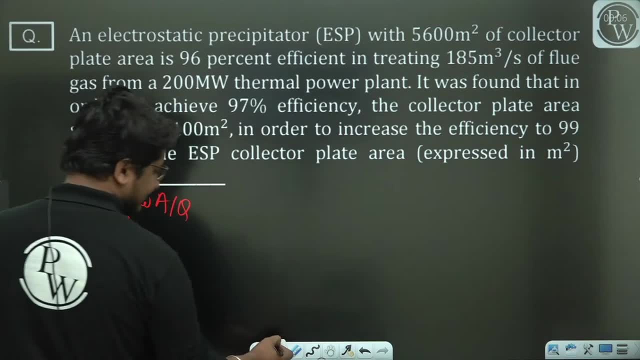 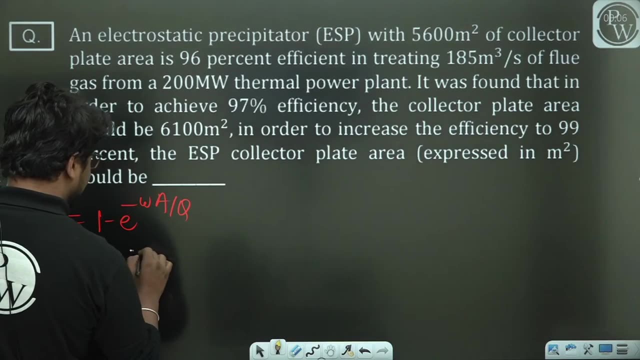 so if we see the formula of efficiency, then what do we write? 1 minus e to power omega a by. this is something we write. so if we see the first case, how much is it 96, so in the first case, 0.96 equal to 1 minus e to power omega by q into area was 5600,. 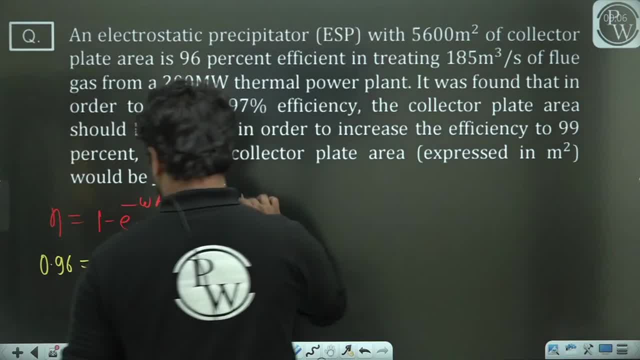 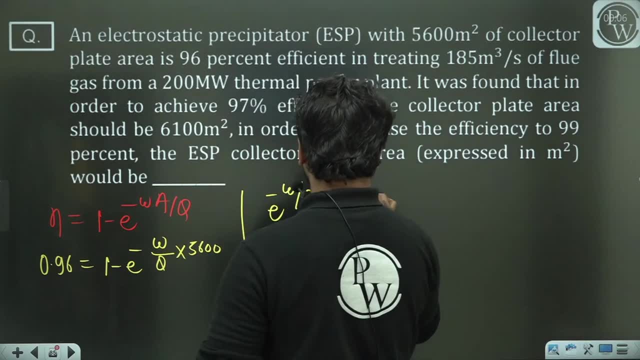 I am changing it a little, I am writing it in a better way. so e to power omega by q into area is 5600, and that will be equal to your 1 minus e to power omega by q into area is 5600,. 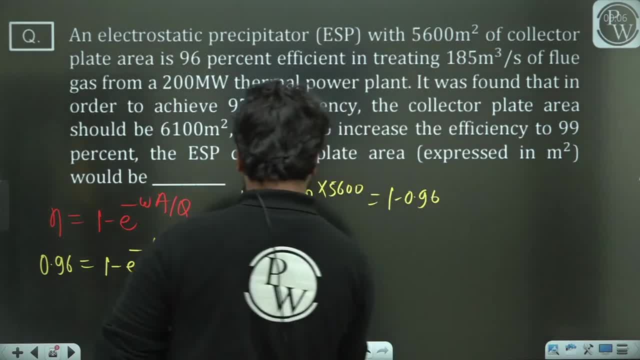 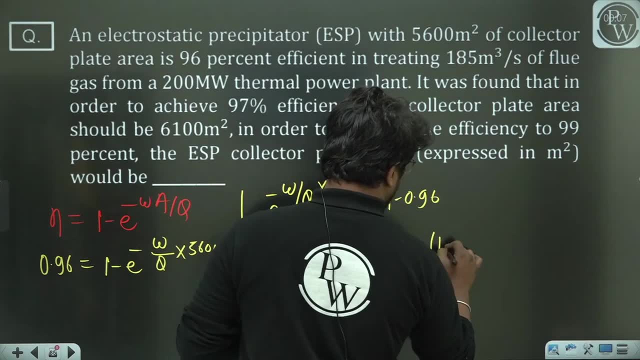 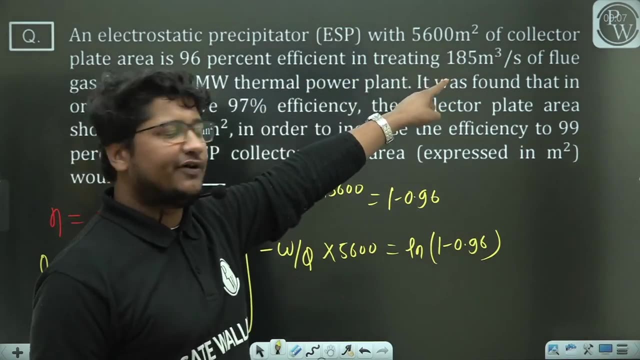 1 minus 0.96, which I can write like this: minus omega by q into 5600 is equal to ln 1 minus 0.96,. now I have written this according to the first one, according to the 5600 meter square you had given. 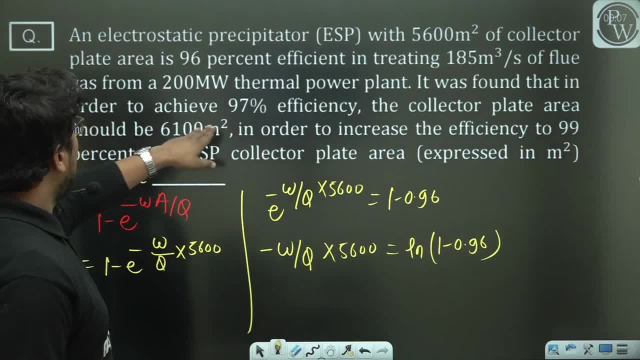 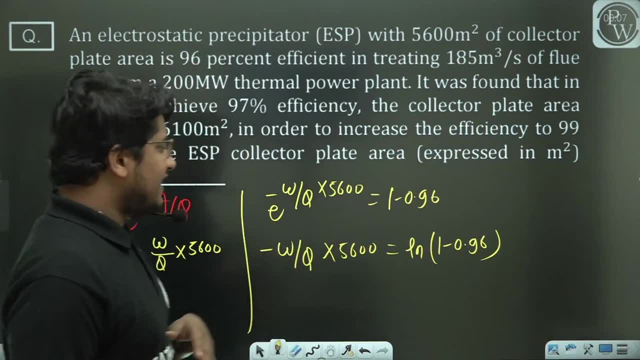 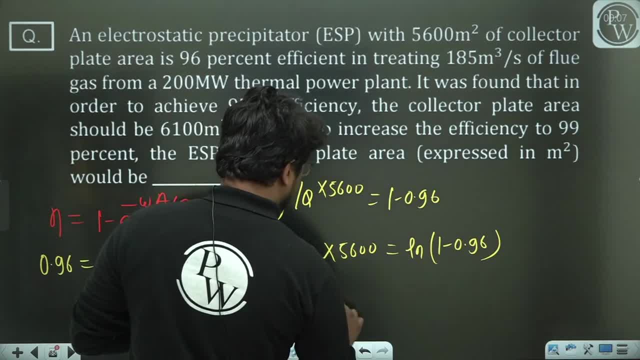 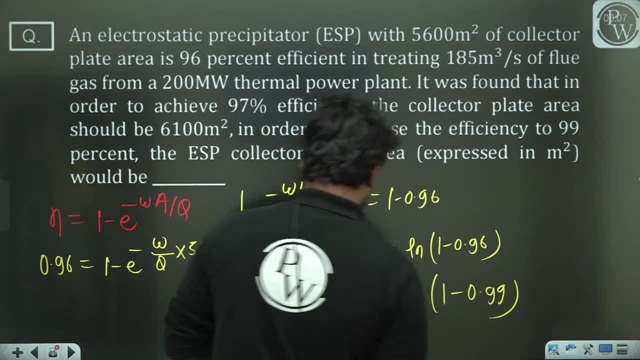 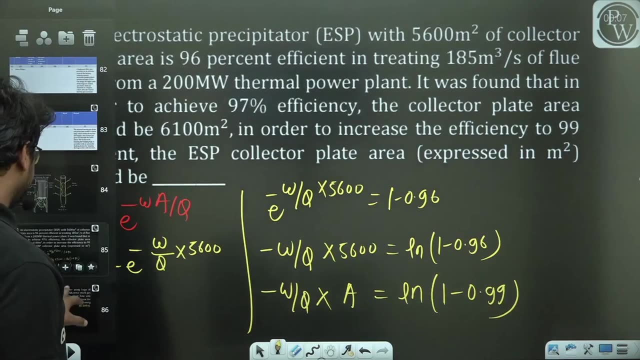 what will happen for 99%? again, your formula omega by q into area. you do not know that ln 1 minus 0.99, so divide both omega by q. omega by q will be cancelled. will you have? will you have, 56 hundred divided by area? 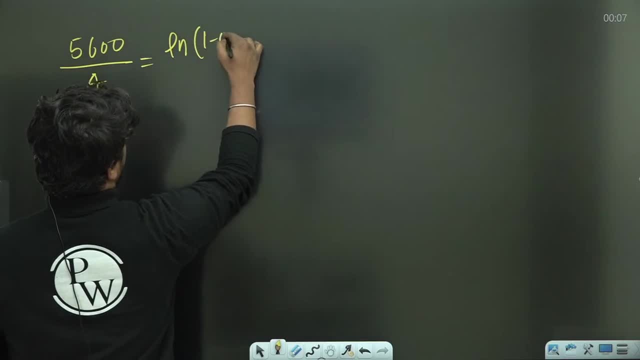 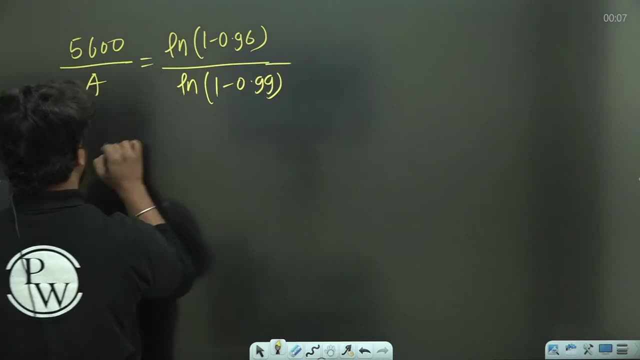 it will come here again ln 1 minus 0.96, and here will come ln 1 minus 0.99,. so what will be the value of area comment and tell me. what will be the value of area comment and tell me. 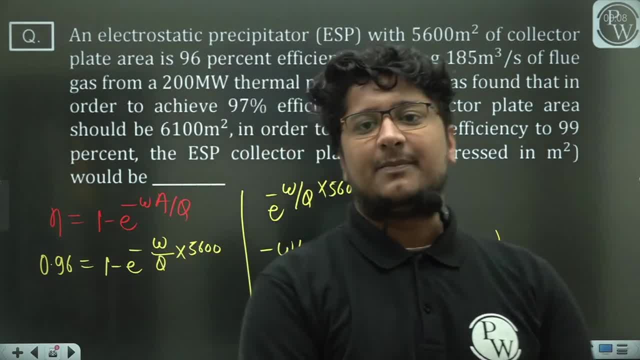 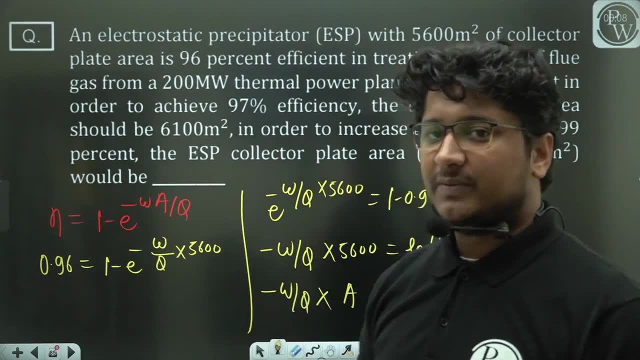 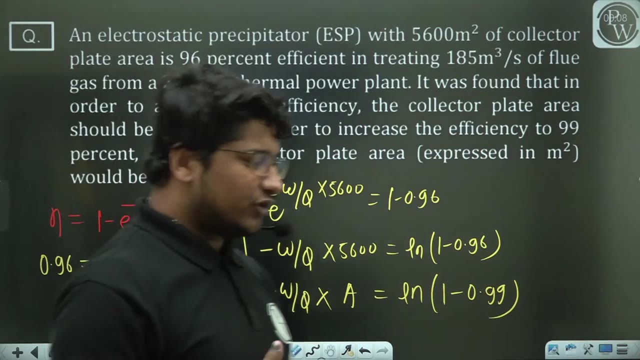 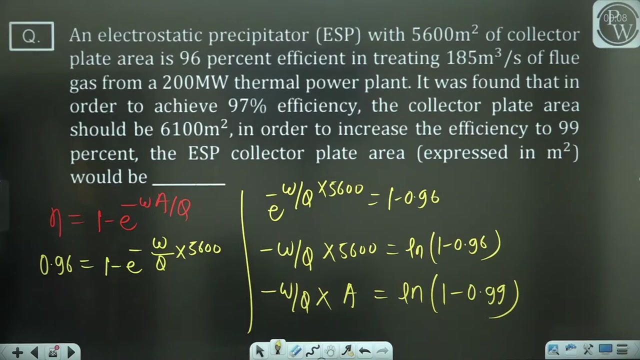 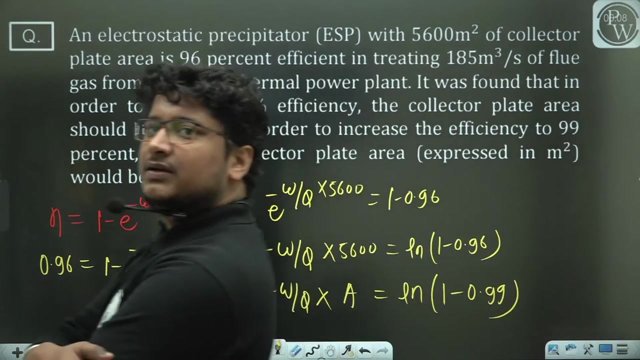 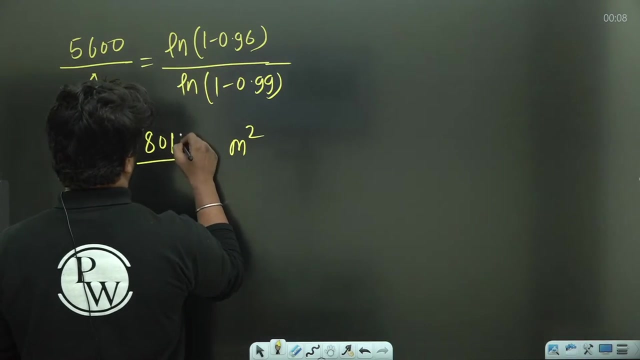 omega by q will remain same in both your particles collection created area will increase. your omega is not changing. your q is not changing. it is the same. so it is the same. omega and q will be constant. that is not changing. so your answer is 8011.78, 8011.78 meter. 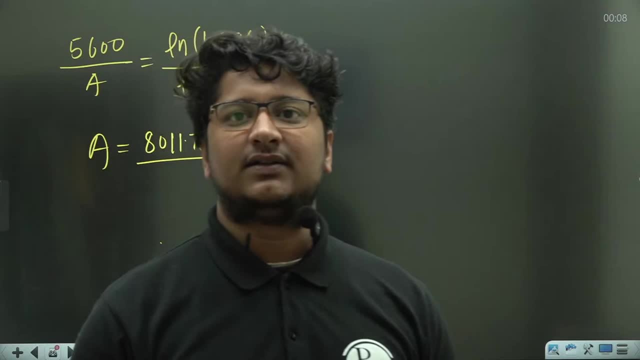 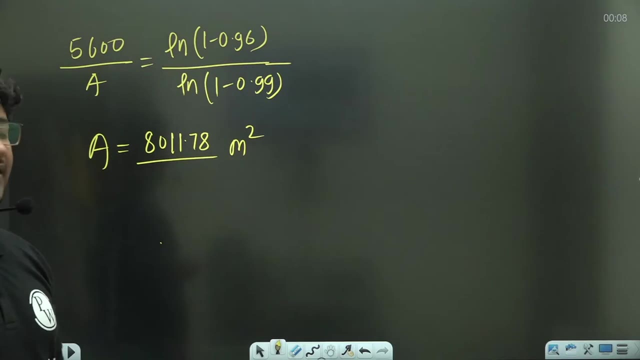 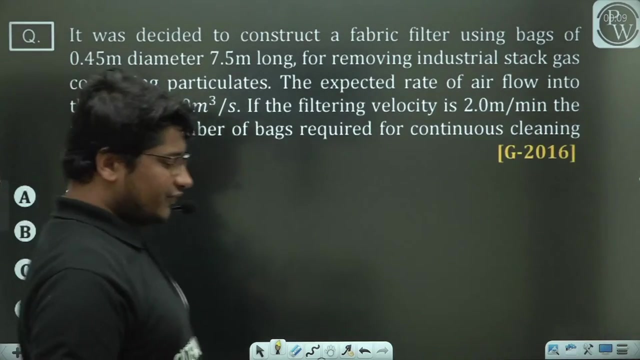 did you understand Faisal Akhtar? did you understand child? did you understandGIRA hills? América, Neur�atuk. OK, now we will discuss aboutICHIL, we will discuss aboutIH1QR, we will discuss about Whorecraft. 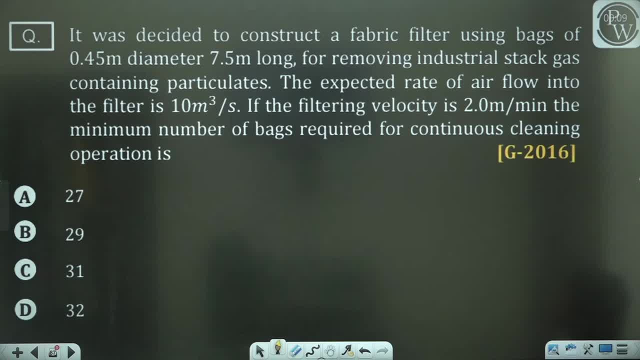 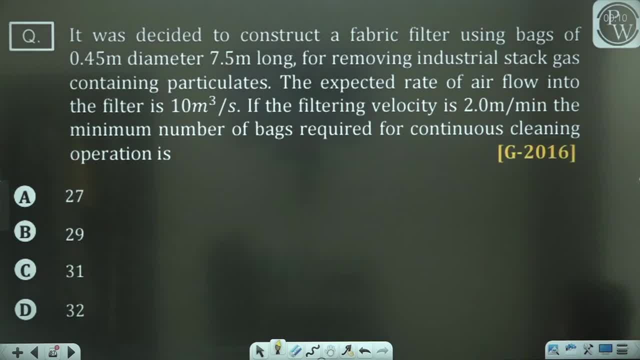 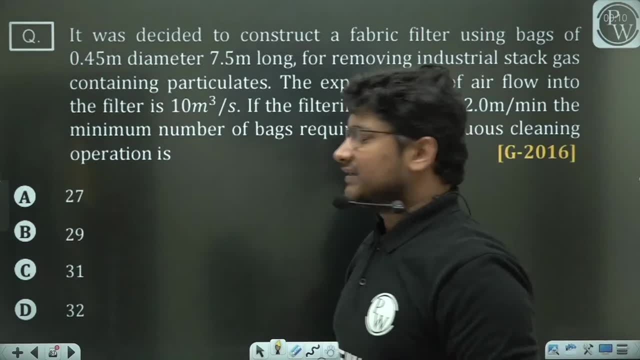 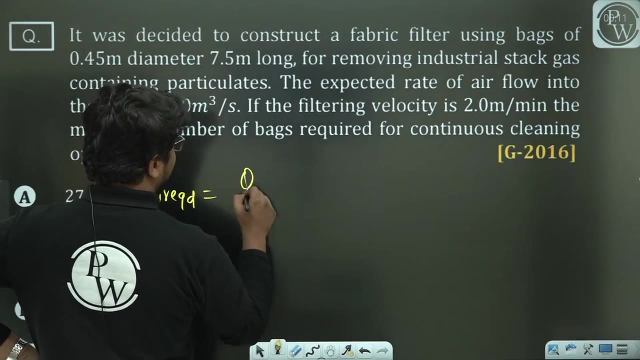 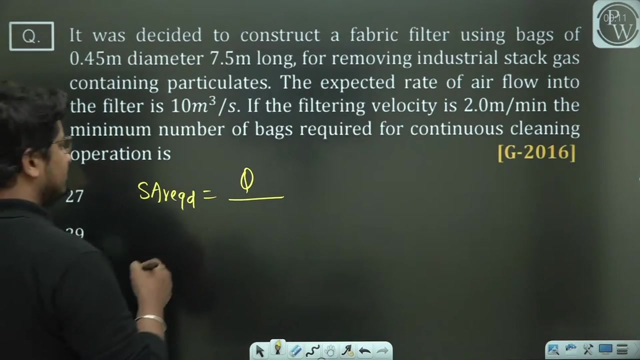 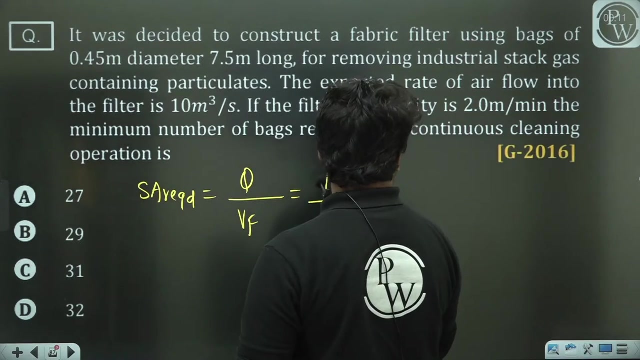 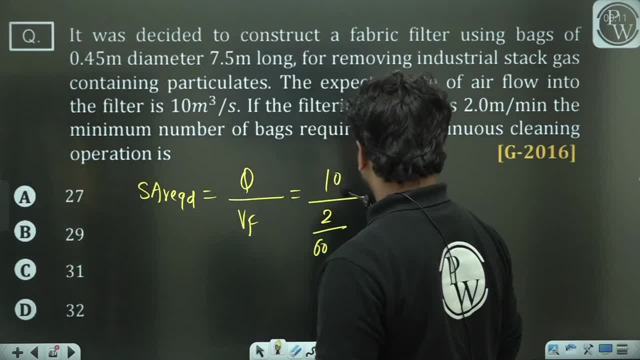 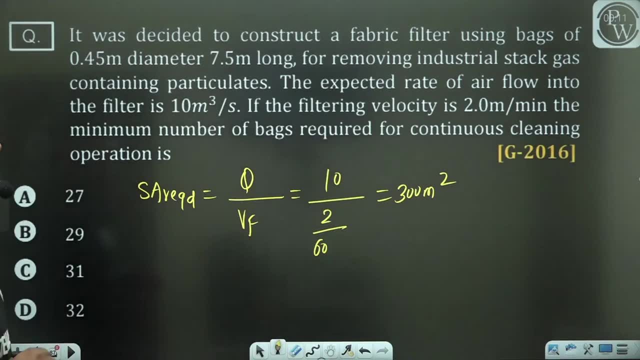 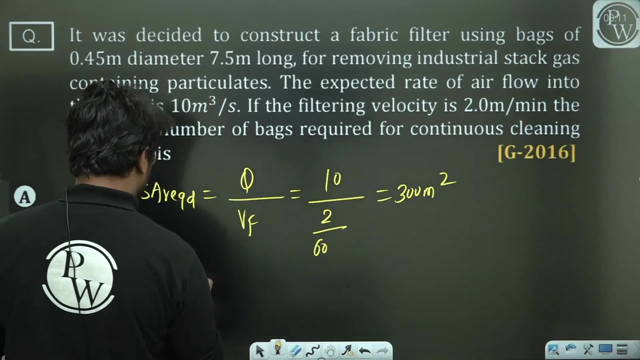 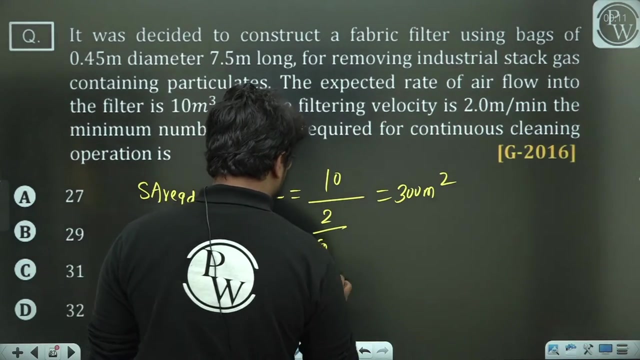 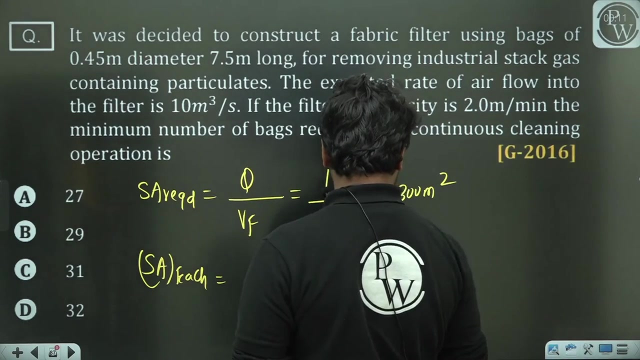 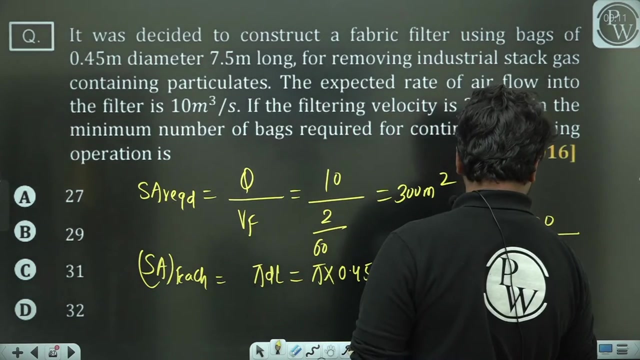 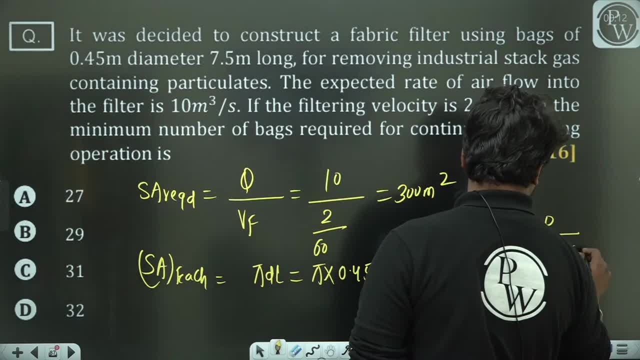 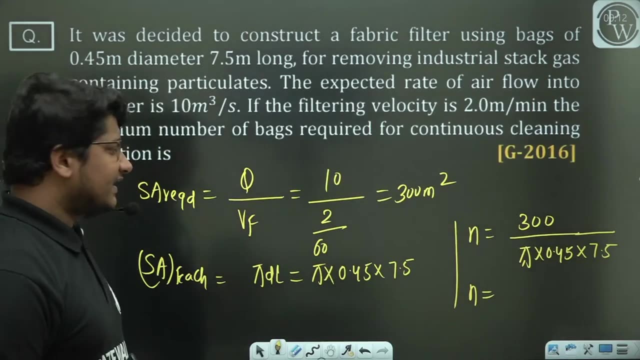 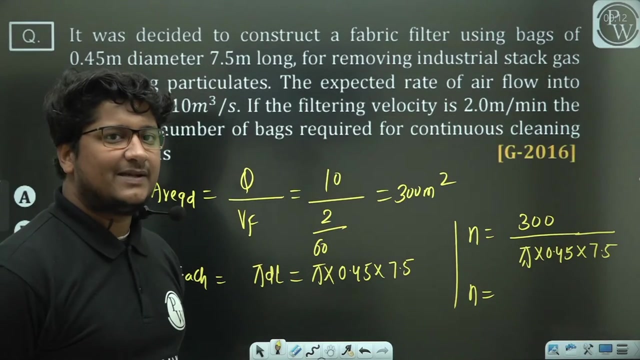 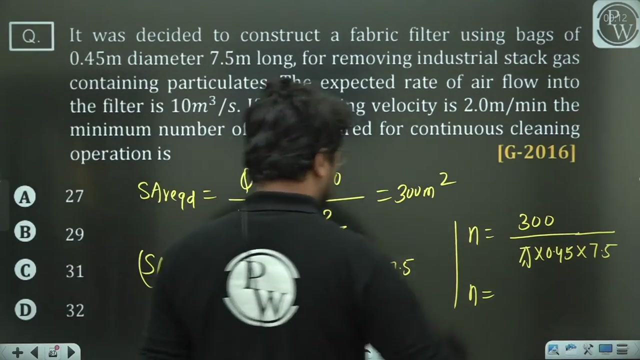 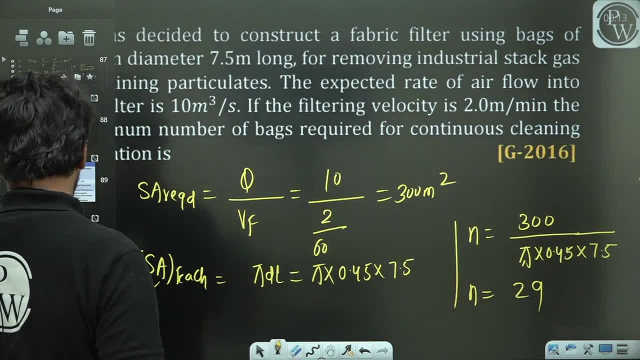 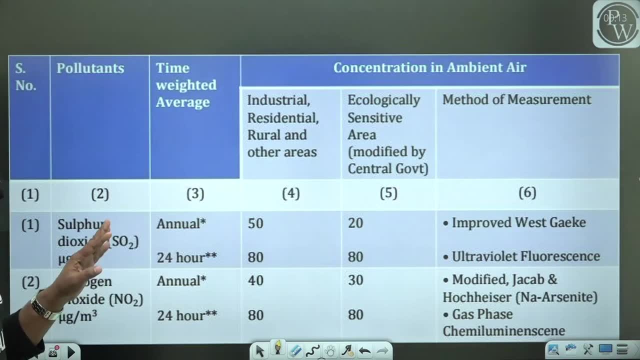 number of filter bags. so when this sir cannot, ok, I switch over. data will be mentioned to you and your 24 hour data will also be mentioned. keep this table in your mind. I have given you the whole table in this PDF. you don't have to wander anywhere. okay, what is the total? 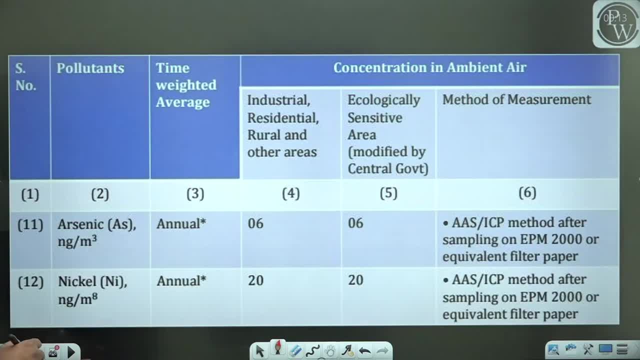 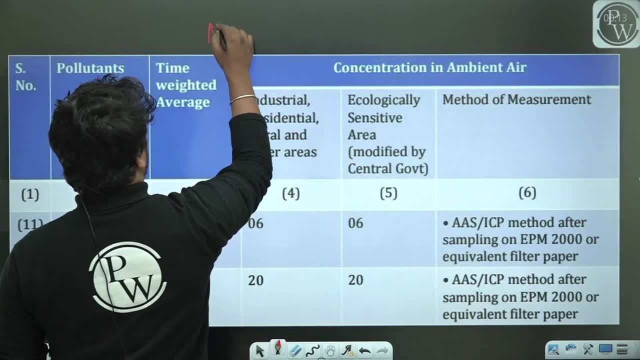 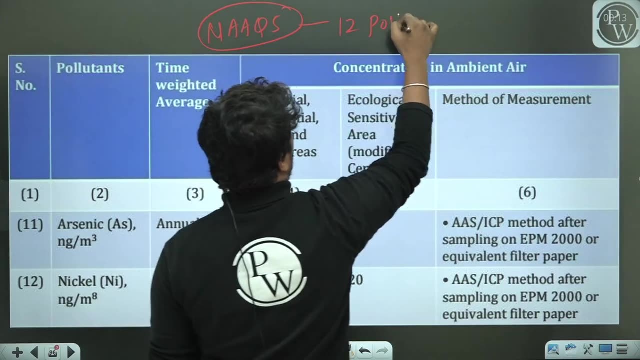 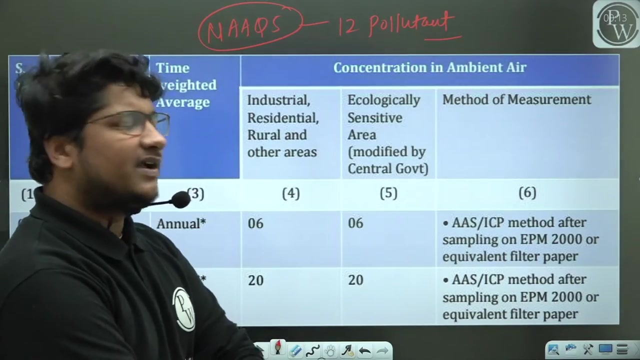 the table that has been given to you has been given to you for a total of 12, total 12 are your NOCs A, a, 12 pollutants of which you have given data. keep it in your mind once: I don't ask about gate, but sometimes you. 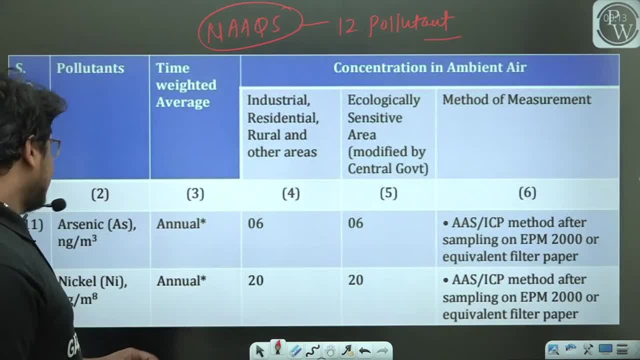 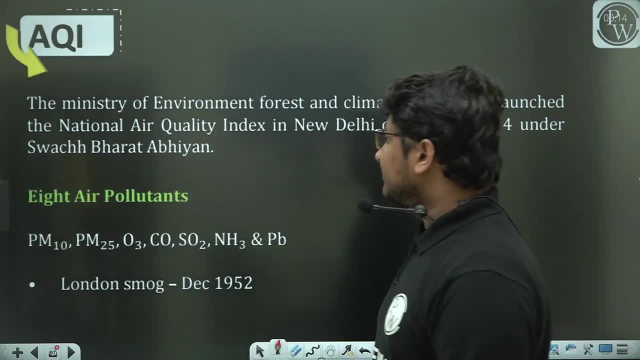 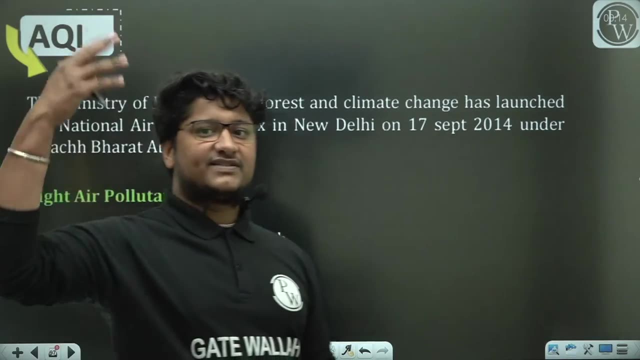 see on the AC. now I don't ask, but still I'm telling you I don't know. ask the second thing regarding yourself, your air quality index, basic things. So in the air quality index you generally keep 8 pollutants. total 12 are given by NOX. 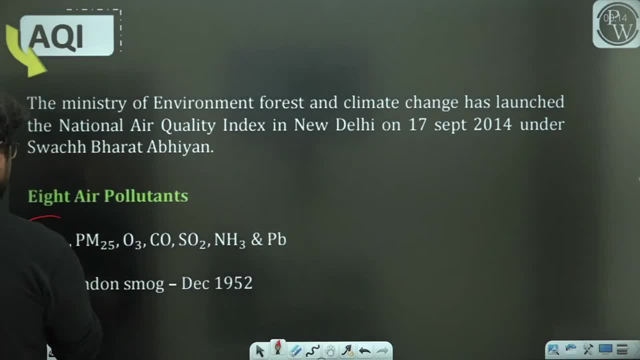 But in the air quality index only 8 are considered. Only these 8 are PM10, PM2.5, ozone, CO2, SO2, NS3 and PV. Tell me one pollutant which is very important, but you don't have it. 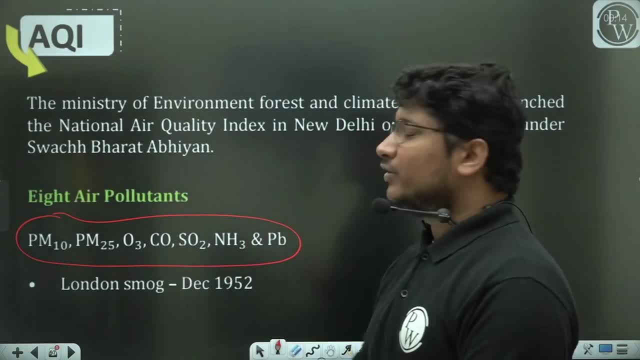 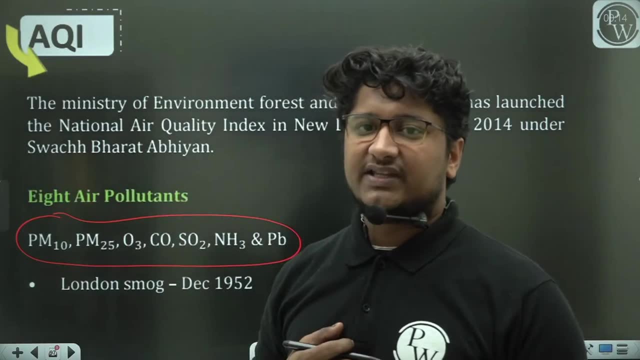 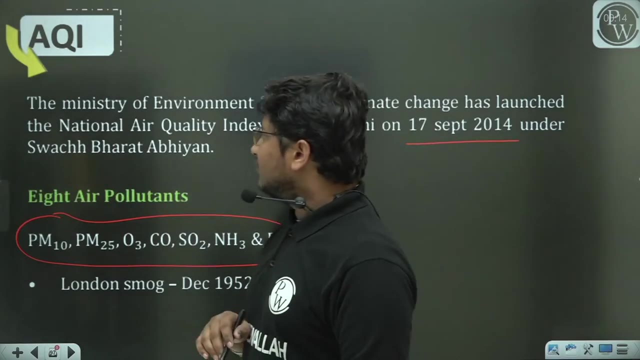 It is not very important now, but you don't have one pollutant in AQI And we didn't have AQI before. we used to follow the European air quality index, But after 17th September 2014,, under Swachh Bharat Abhiyan, your AQI came. 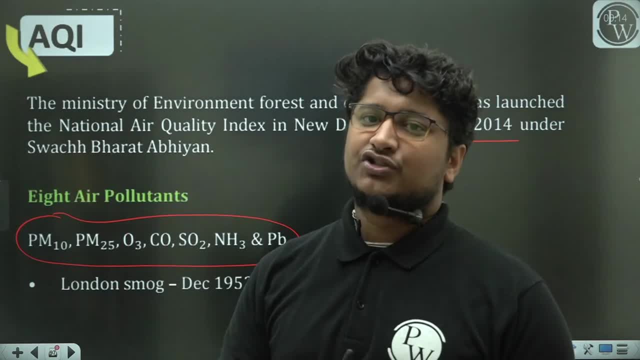 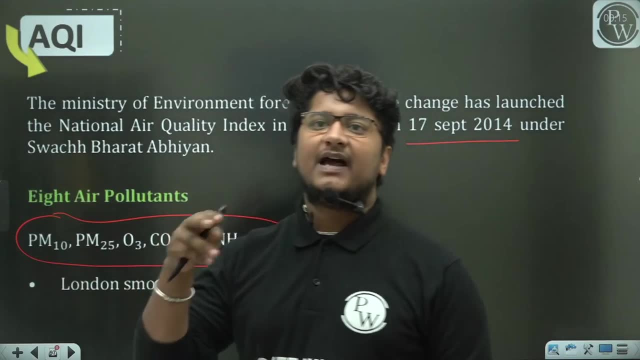 People who talk on social media. Sir, nothing has gone in Swachh Bharat Abhiyan. So there was money fraud. so it is not like that. A lot of things have come in Swachh Bharat Abhiyan. Now the latest municipal solid waste: 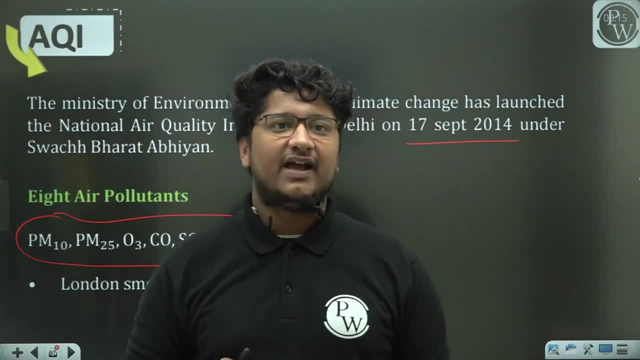 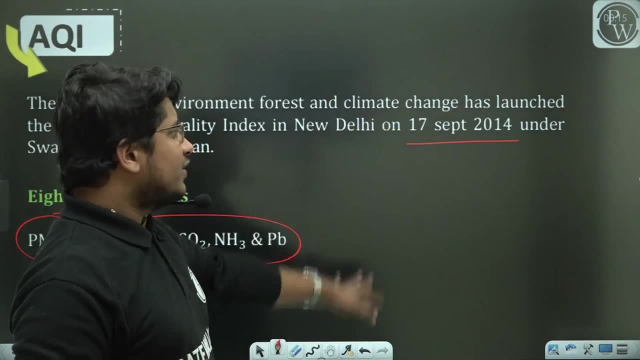 While reading the manual. it has come in Swachh Bharat Abhiyan in 2016 And the AQI which we used to be based on foreign. now it is our own AQI of India, So your AQI is also ours. 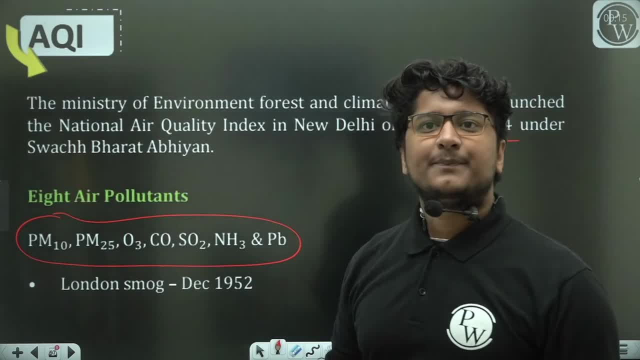 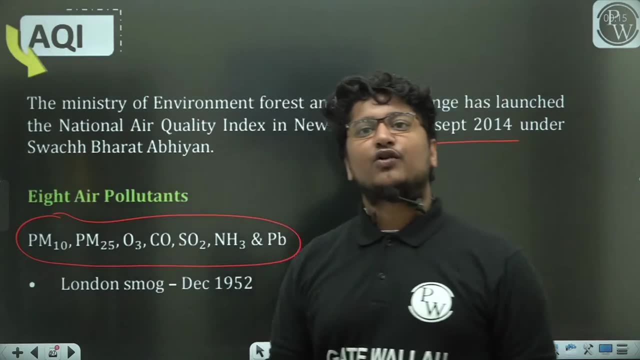 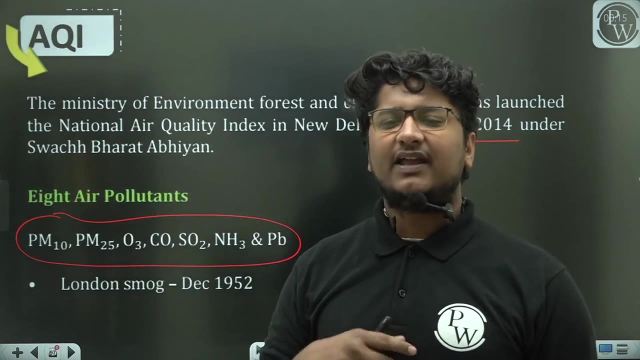 So after 2014,. you will get it. Your child got CFC and Chlorofluorocarbon- Okay, but there is no Chlorofluorocarbon. We didn't need Chlorofluorocarbon to do this. Now we don't mean to take carbon in AQI. 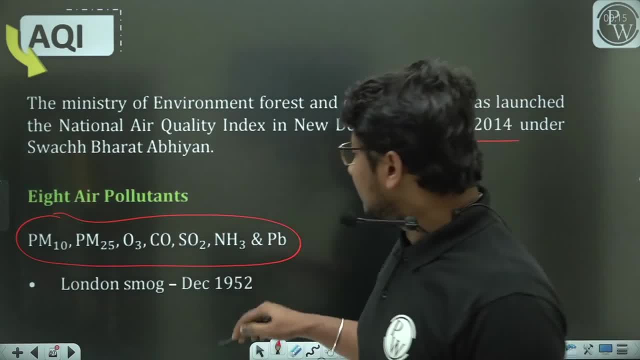 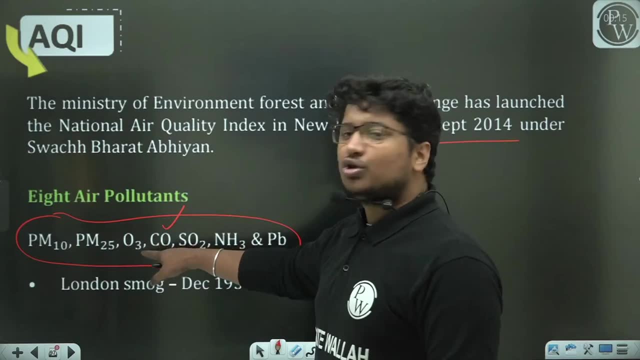 There should have been one more thing in AQI: CO2. But their term is that if CO is given, then CO2 will not be kept. So carbon monoxide is not in it. CO is kept. O3 is there, child, Very good, O3 is there. 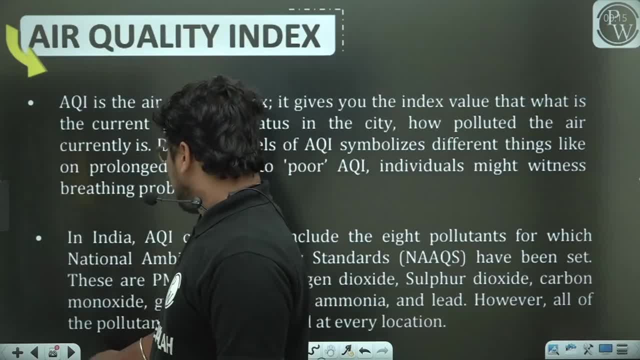 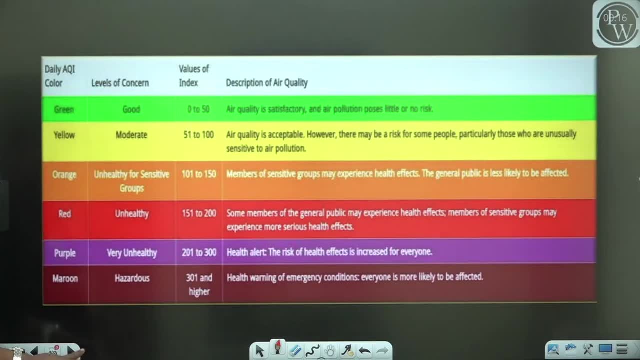 So remember these 8 names. sometimes you will be asked And remember one more thing regarding this, This table. Keep this table in your mind. Keep this table in your mind, Okay, So the green condition is 0 to 50. The yellow condition is 51 to 100. 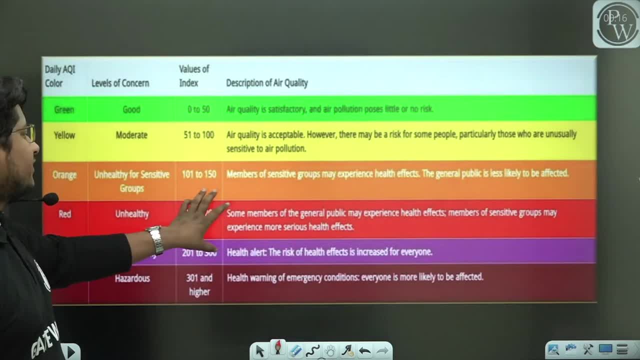 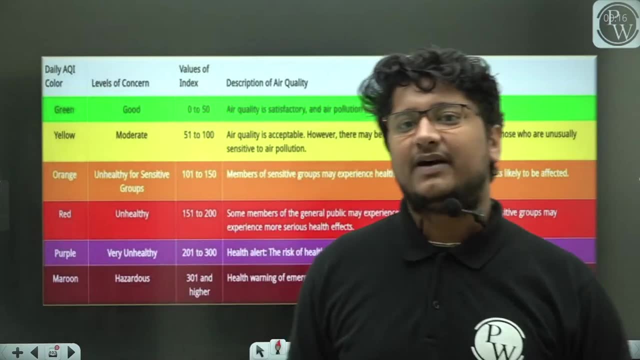 The orange condition is 1 to 1. The red one is 151, 2 to 300, 0 to higher. So keep all the remarks given in your mind. Sometimes you will be asked directly: So your AQI. this topic has been added recently. 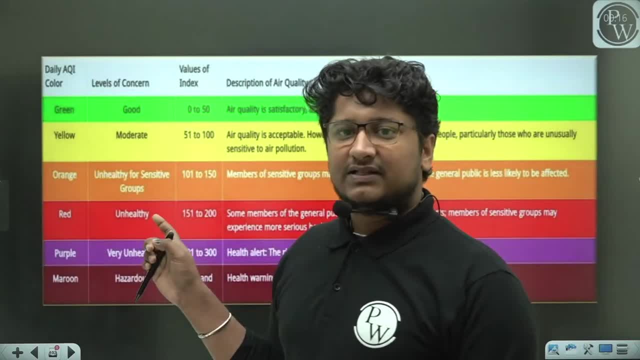 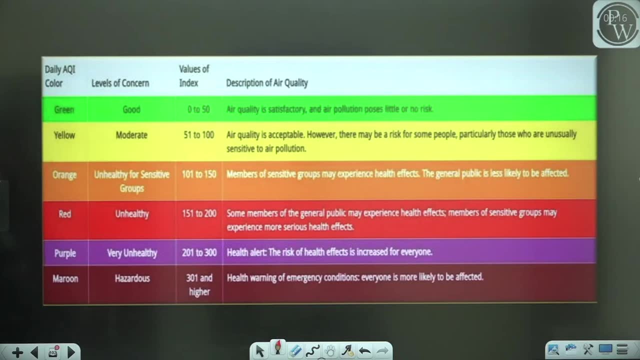 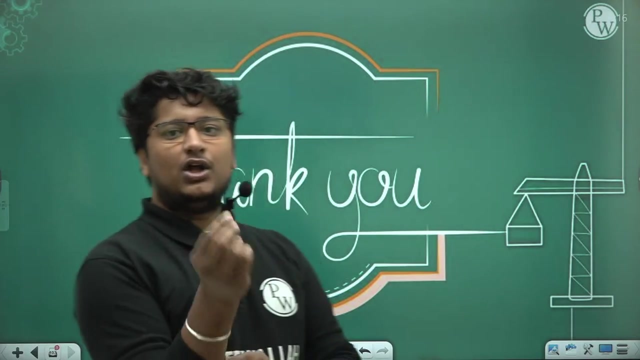 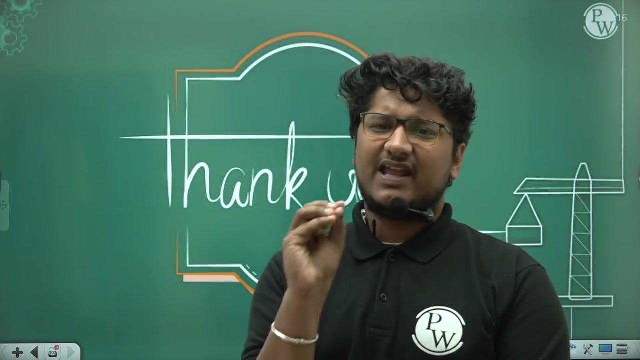 So sometimes you will be asked in such a range. Okay, Keep this in mind. So with this, your chapter of air pollution is completed. There are some things that I have left for you for reading, So whenever you have time, just read it once. Even if you read it once, that is enough, no problem. 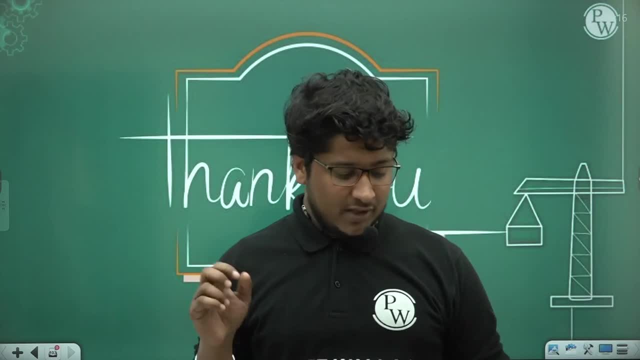 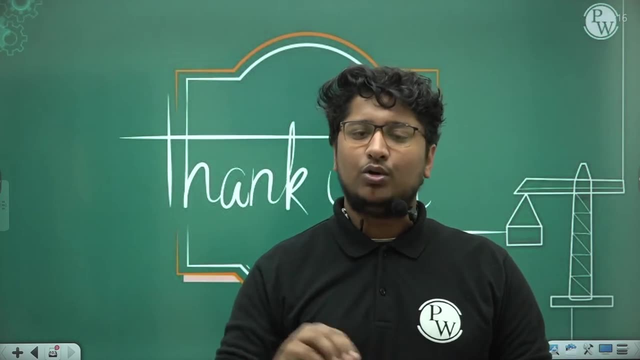 But you have to practice the questions more. Try that: your DPP and your previous year questions: You have to apply all of them well. When the chapter is complete, then DPP and previous year questions: You have to apply all of them well Whenever you get time. 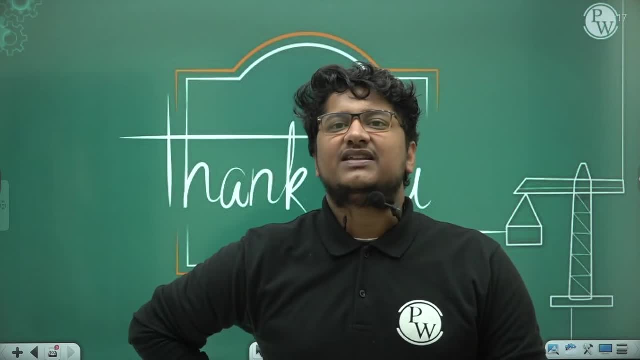 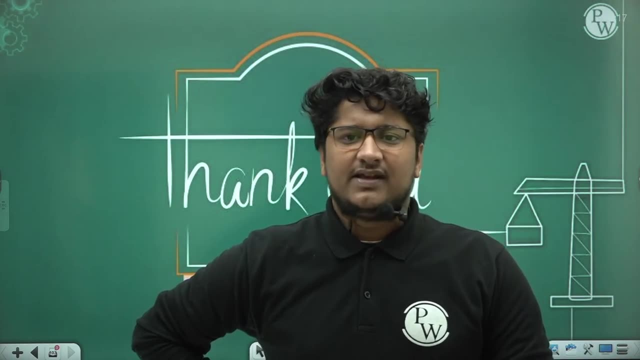 Is there any trick to remember all this data? The trick is the same: my child Don't do too much database, So GATE exam, NOT SSC exam, and RBI exam Where you don't have a database, Okay, That's why I tell you to read a lot of databases. 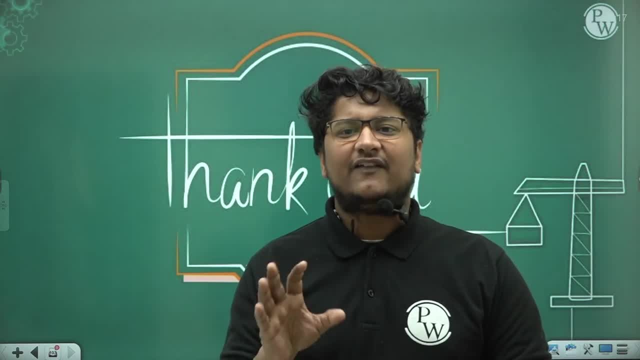 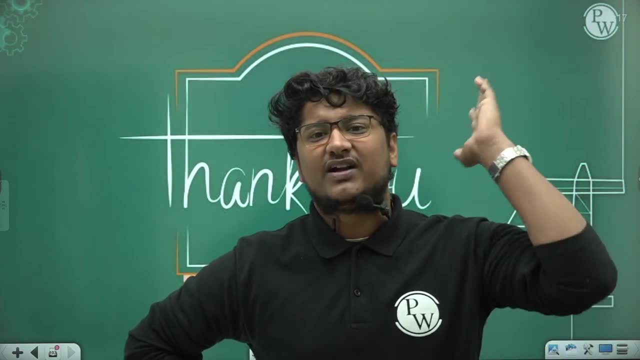 I don't make you do it in the class, Because GATE is never the part of Ratta, And if you ask one or two questions, then don't do it completely. Now, for that one mark You have to write the whole story, So that's your loss. 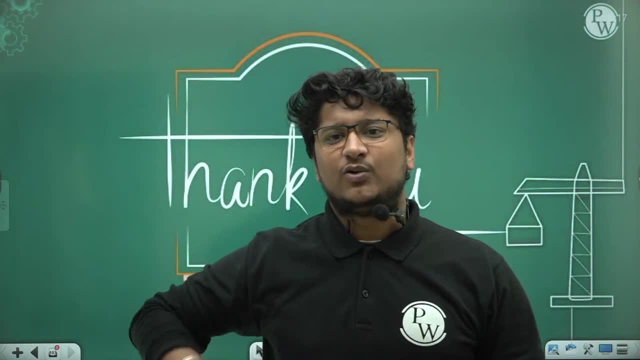 Instead of writing, you read some concept. You will get more than one mark. So it is not about solving all 65 questions. It is about solving those questions which you know, And that, too, with the maximum accuracy. No one goes to GATE to solve 65 questions. 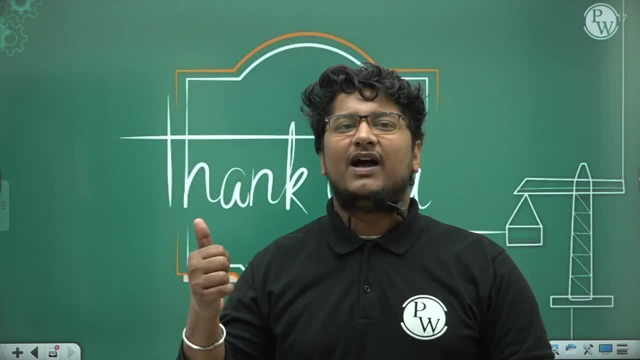 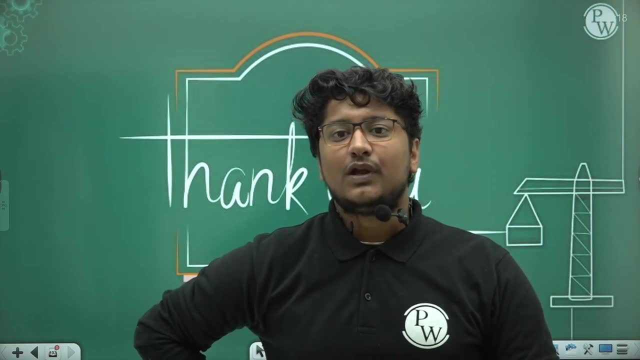 That I have to solve 65 questions. So you got one question. Now, because of that one question, you have to write all the data of the environment. It doesn't make any sense. The waste is of time For GATE point of view If you are preparing for ESC. 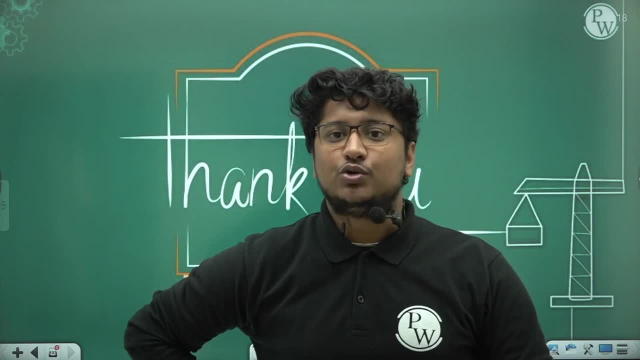 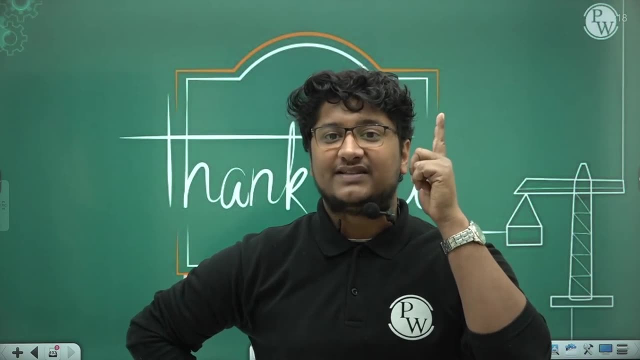 If you are preparing for SSC, Then each and every data is important for you. You need to remember. So keep one mindset clear in GATE: See before giving the exam. catch the mindset of the exam. What does the exam say? So GATE exam never gives a big formula. 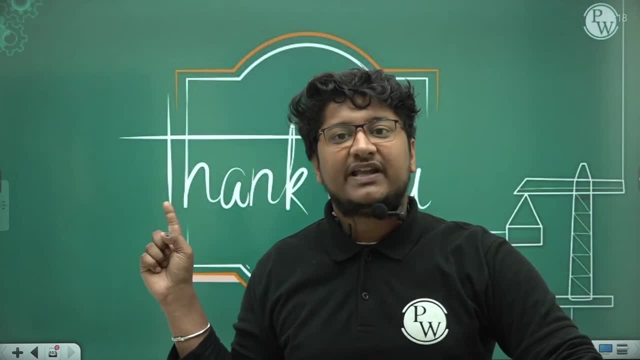 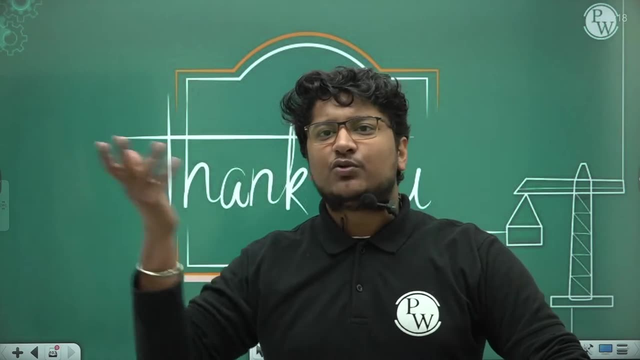 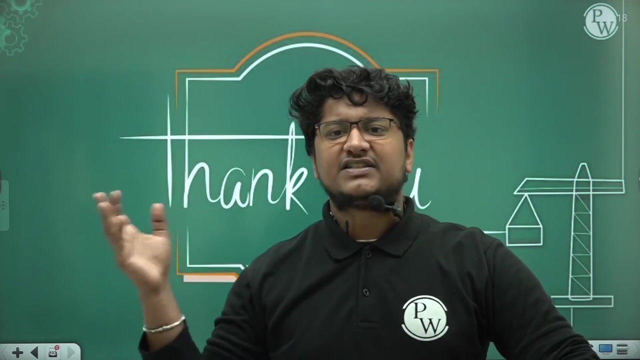 As I told you all, Peter Phillips equation in yesterday's class. No question has come from Peter Phillips equation till today Because sir GATE never gives such a big formula. Your head loss during filtration, Carbon Kozeny equation: Big formula, I told you all, But there is no meaning of questions. 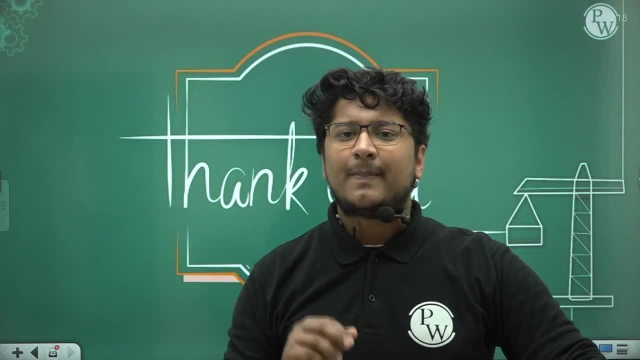 Because GATE has never come from me. Do you understand the point? The Hazen formula which I told you in sedimentation, Newton's formula, which I told you. So questions have not come till now. In the grid chamber, I told you the formula to get Vs. 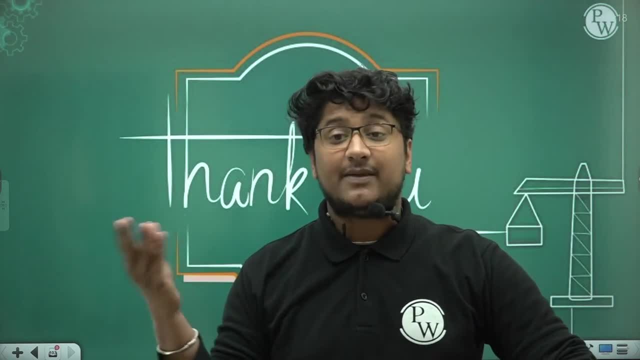 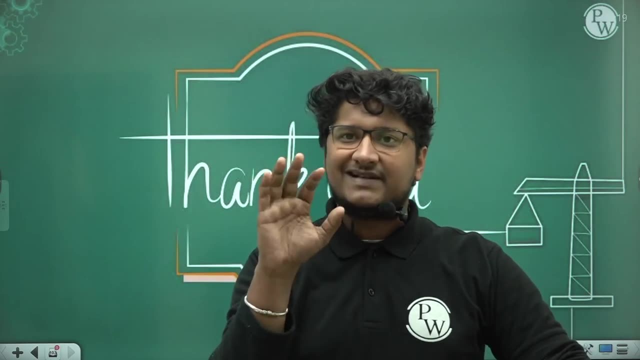 60.1. So no question has come till now, And may be it will not come in the future. May be I am keeping it in the future Because it is there. But the trend says, The mindset of GATE says, The bigger your questions will be. 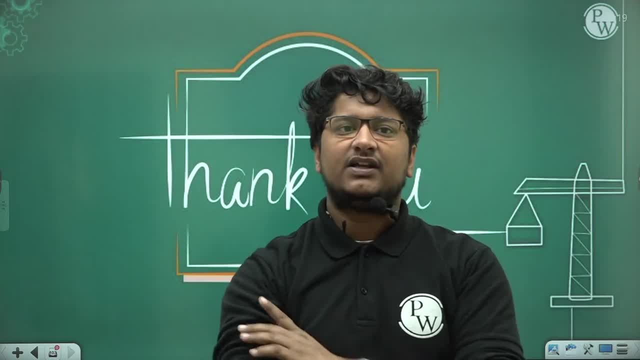 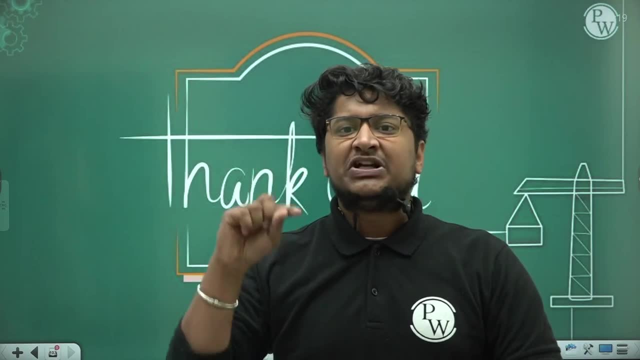 The bigger your formula will be, The chances of getting less. Why? Because the things which are outdated, The things which are outdated, GATE does not like them. So questions have not come from the trickling filter. If you check the PYQ from the trickling filter, 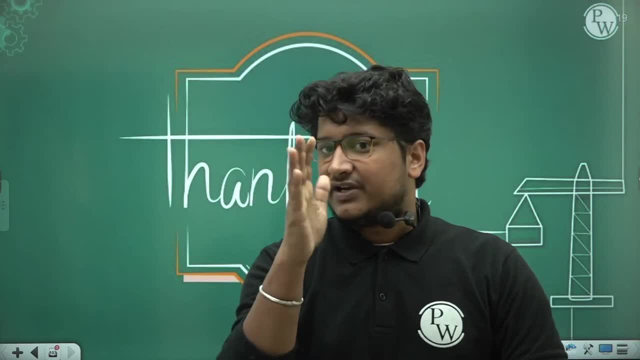 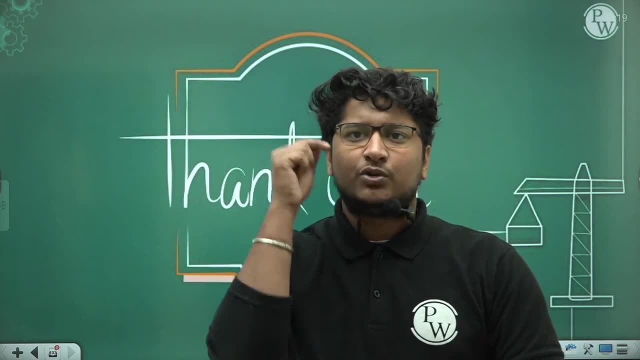 Then you will not see any question from the trickling filter. You will see from ASP. You will not see the question from the trickling filter. Leave the question of one mark. That can be anything. I am talking about the question of two marks. So keep this little trick in your mind. 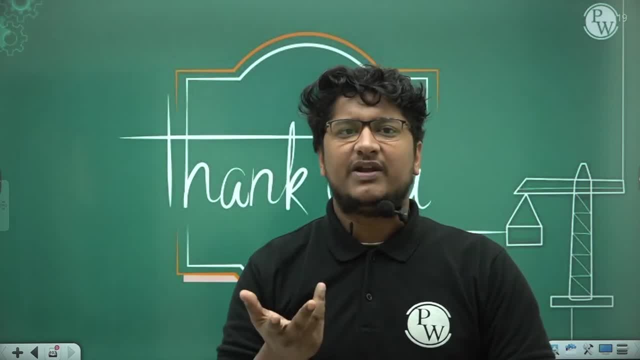 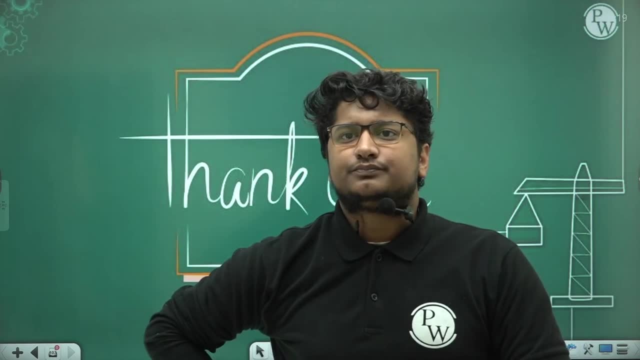 I can give you these tricks. I don't have the tricks of writing. Write it in paper, Throw it, Drink glass water. I will give you all these useless tricks. So read a little bit of the exam. About the exam, Where the regarding of my subject is needed. 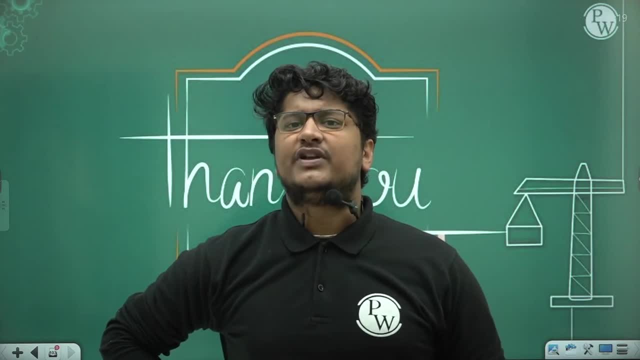 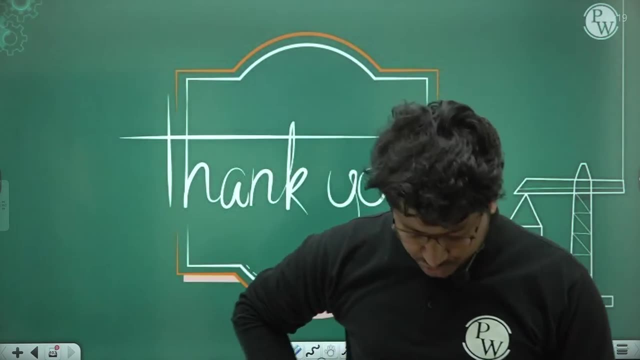 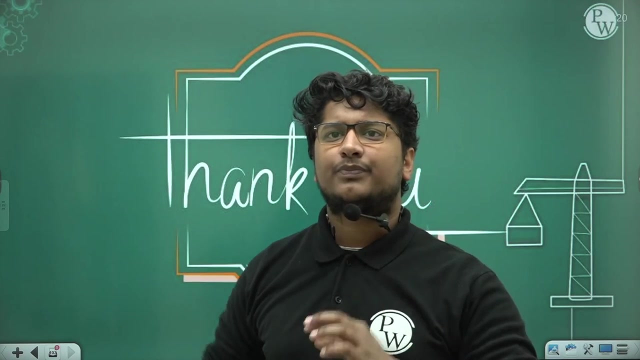 I keep telling you- Rest of the faculties also How to work regarding their subject. They must have told you: See you tomorrow. Tomorrow will be the last class of your environment And tomorrow we will complete the solid waste management easily. We will also do the problems And Will you take any assignment?